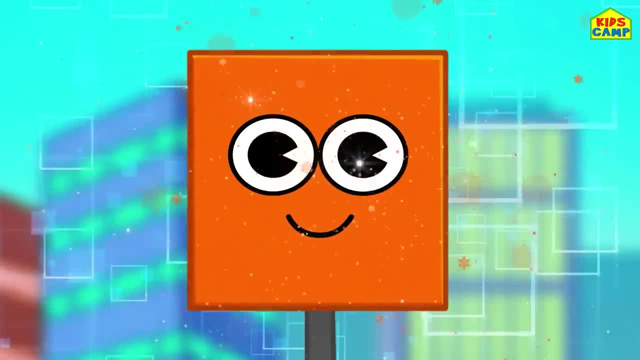 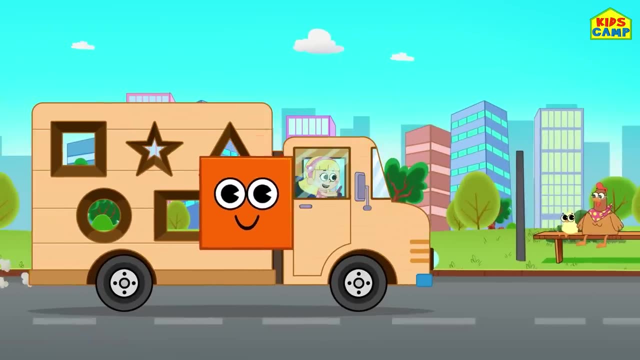 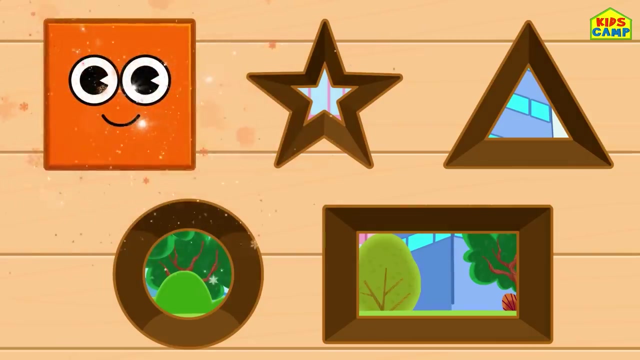 Four equal sides. Yes, this is a square, That is right. Let me collect this shape and place it on my wooden truck. No, no, This is not right. Let's keep moving the square. Yes, this fits. Wonderful Honk, honk. 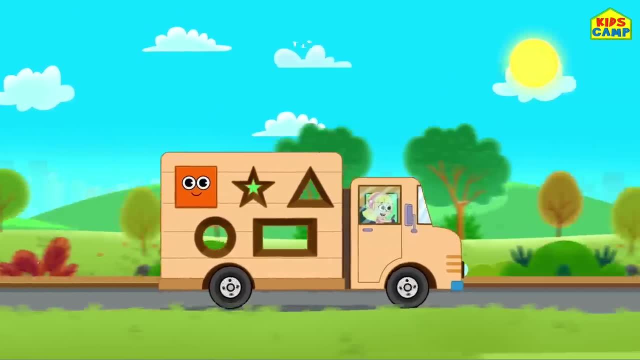 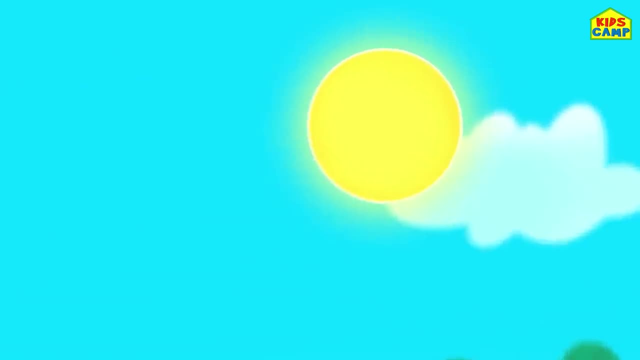 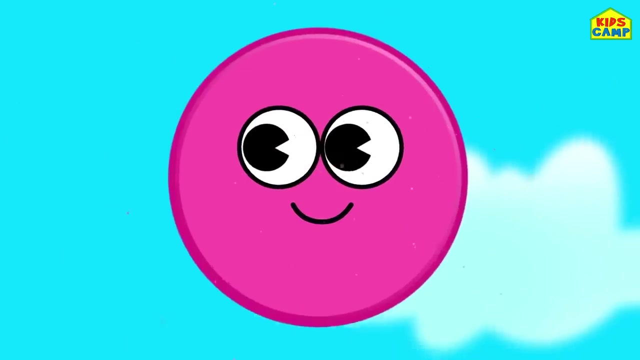 Let's find the next shape. Here I go in my truck. Honk, honk, honk goes my wooden truck. Aha, The sun, It's round, It's a circle. Let's place it on my wooden truck. 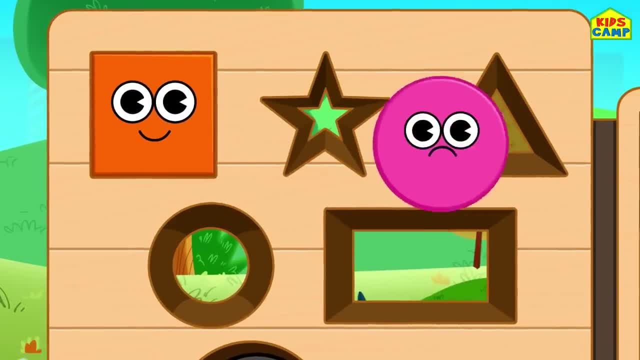 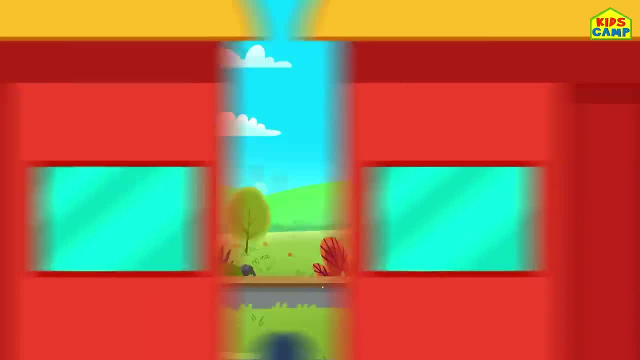 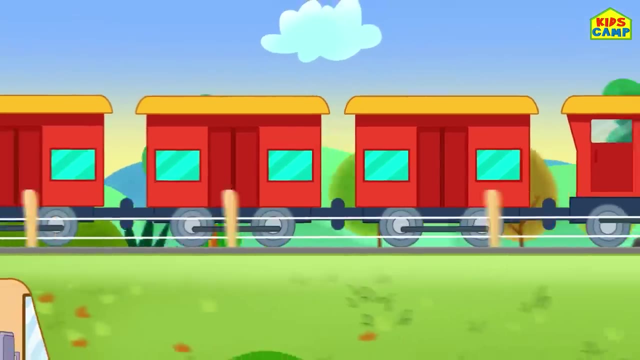 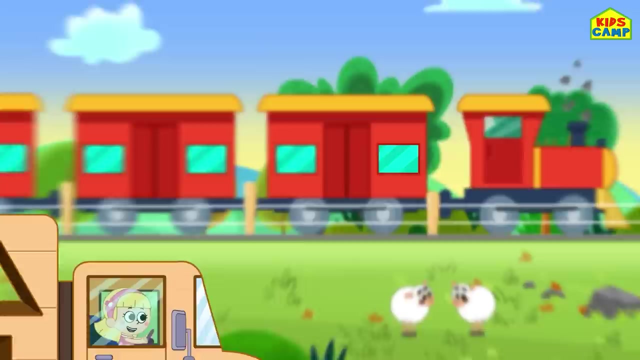 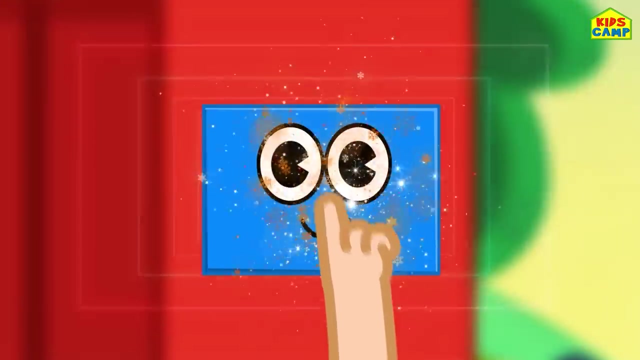 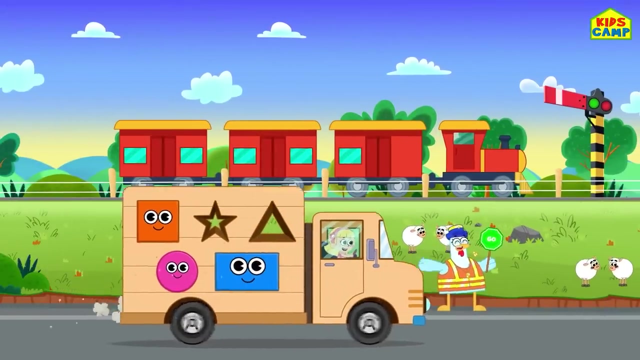 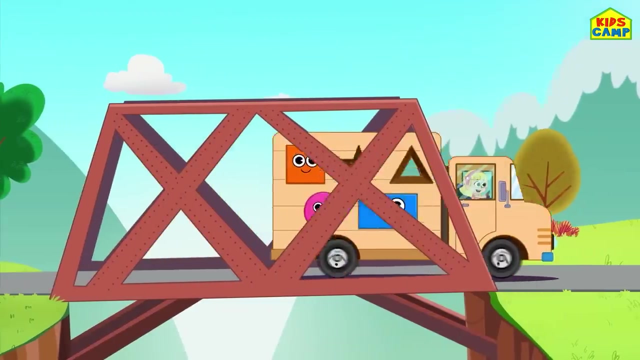 Uh-oh, Not there. No, Aha, It fits correctly, Let's go ahead. Wow, A train. Aha, Do you see what I see Our next shape: Rectangle. Amazing, It fits correctly. Woohoo, Over the bridge, Here I go. Honk, honk, honk, Here I go. 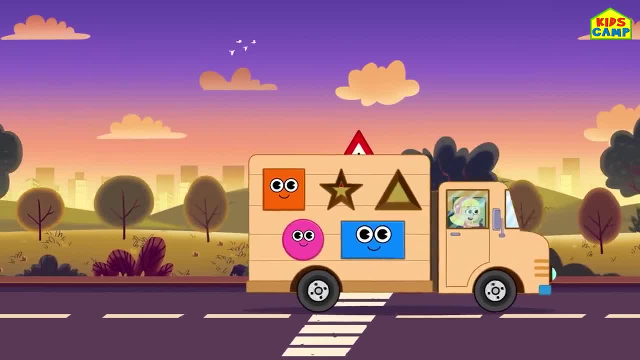 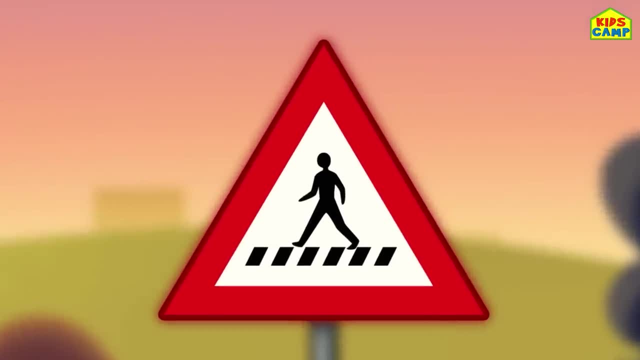 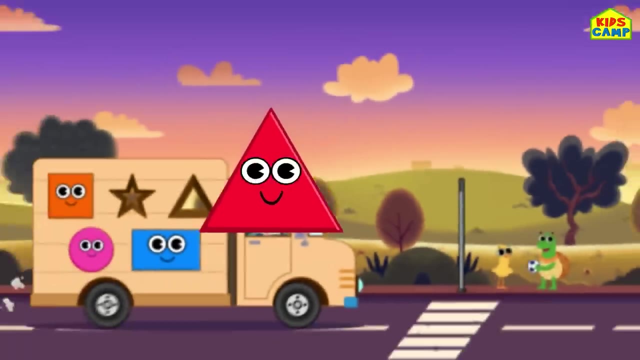 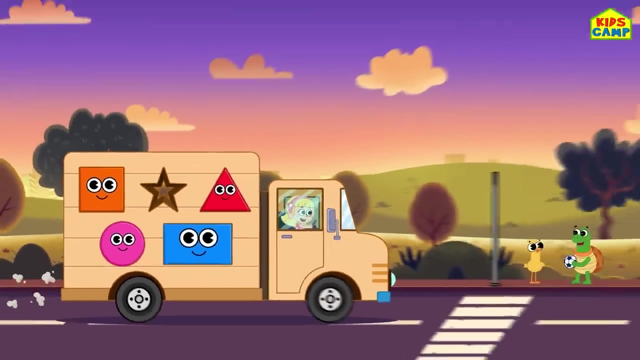 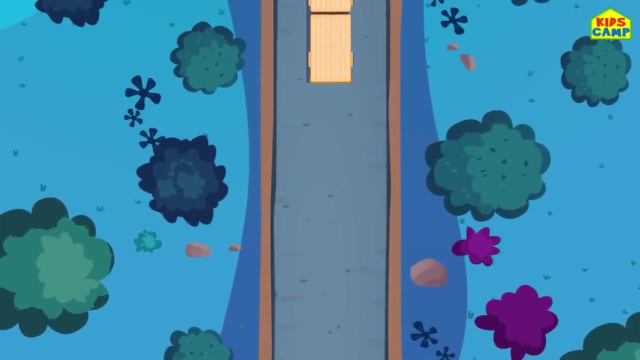 Oh, we almost missed that. Hmm, Is that a triangle? Yes, it is. Wow, Let's place it on my wooden truck. No, Aha, It fits. Let's look for another shape. Where could it be? Wow. 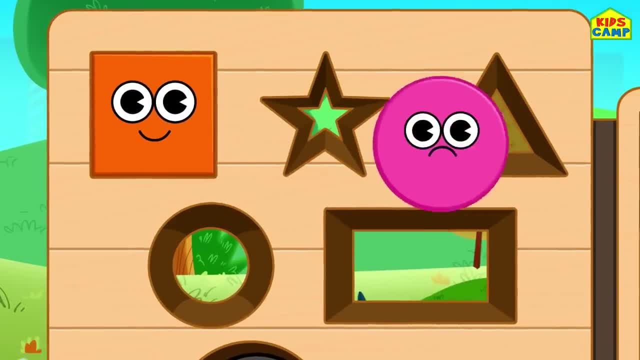 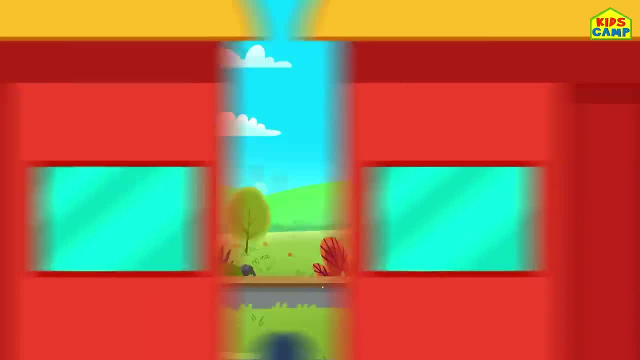 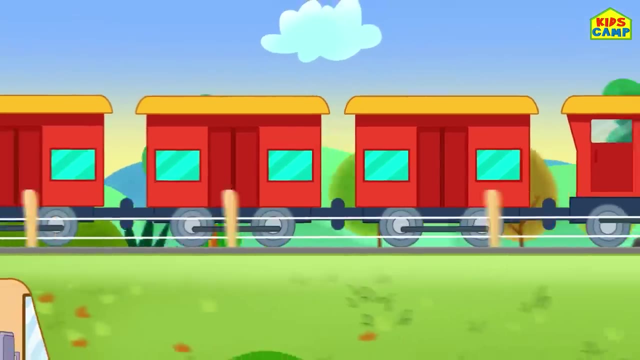 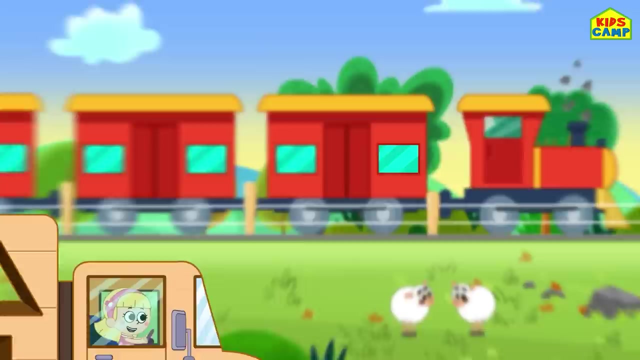 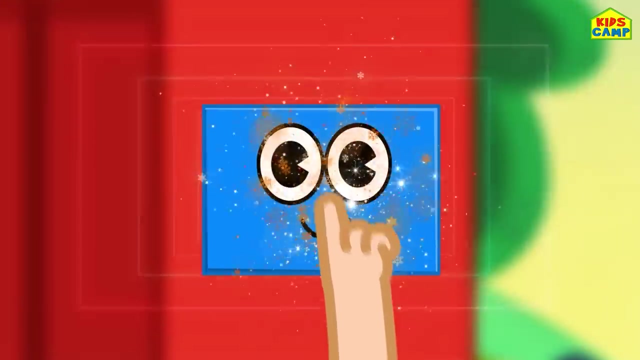 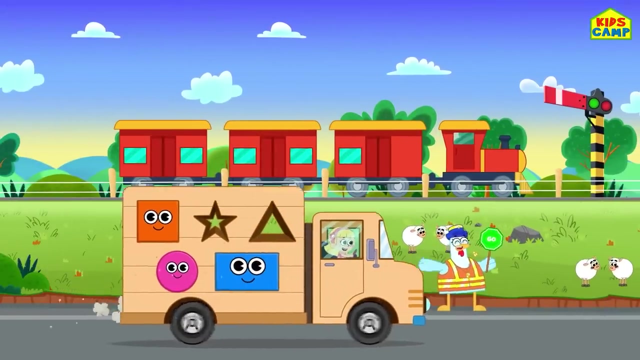 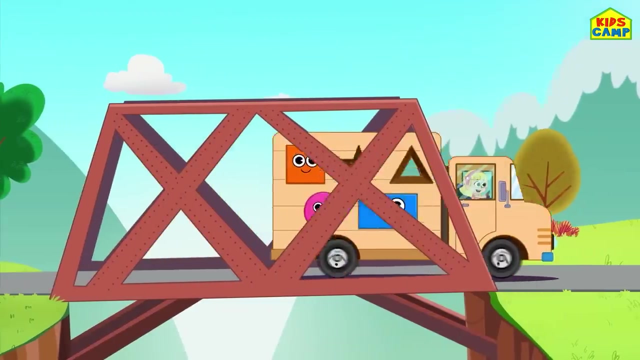 Uh-oh, Not there. No, Aha, It fits correctly, Let's go ahead. Wow, A train. Aha, Do you see what I see Our next shape: Rectangle. Amazing, It fits correctly. Woohoo, Over the bridge, Here I go. Honk, honk, honk, Here I go. 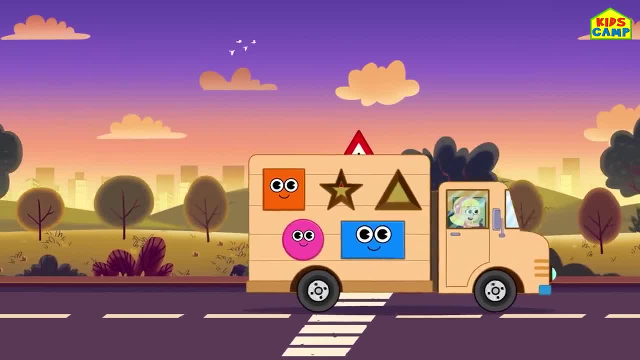 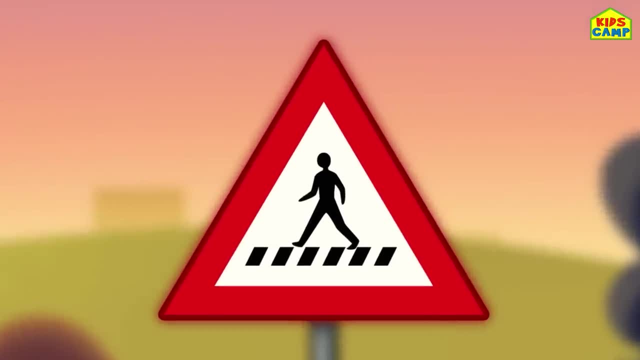 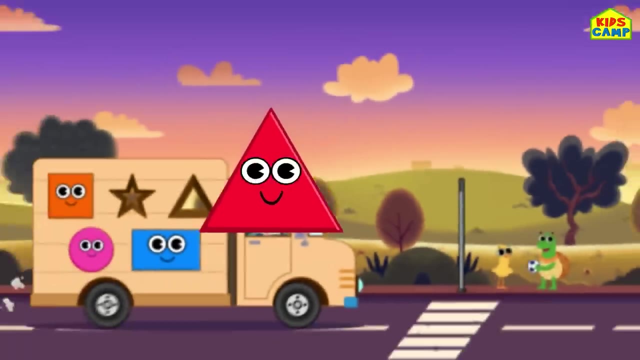 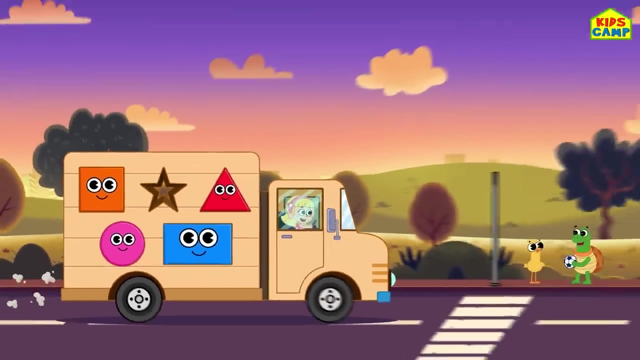 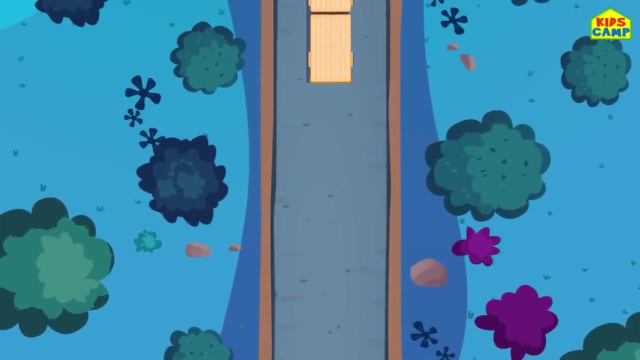 Oh, we almost missed that. Hmm, Is that a triangle? Yes, it is. Wow, Let's place it on my wooden truck. No, Aha, It fits. Let's look for another shape. Where could it be? Wow. 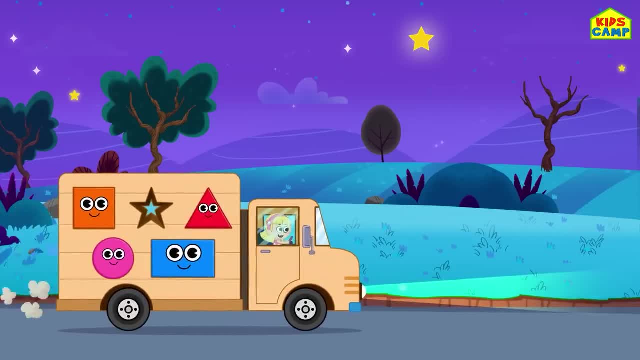 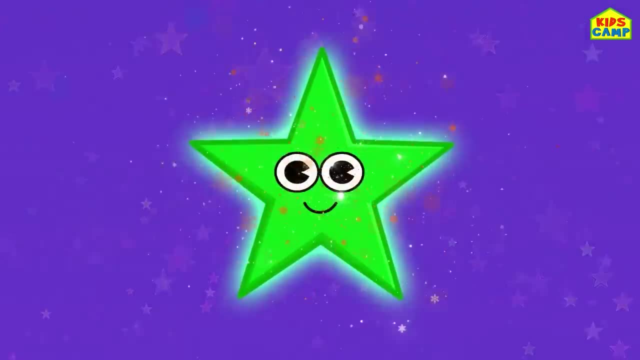 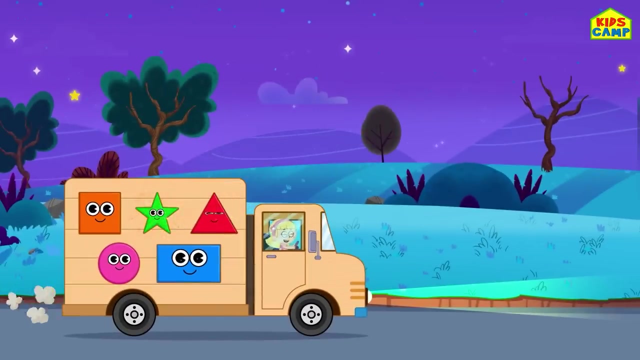 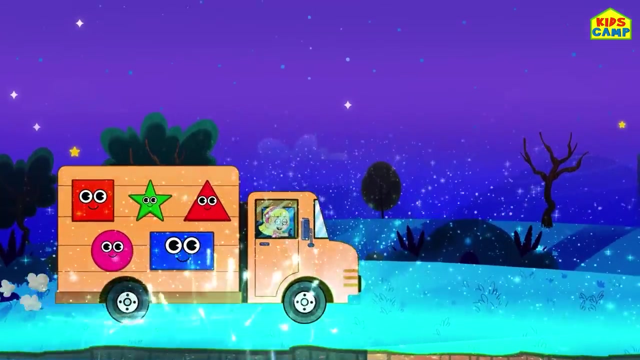 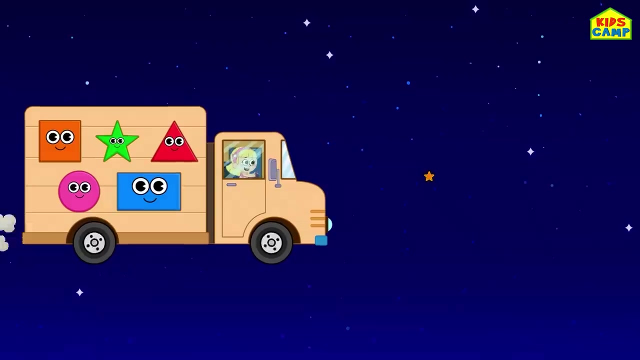 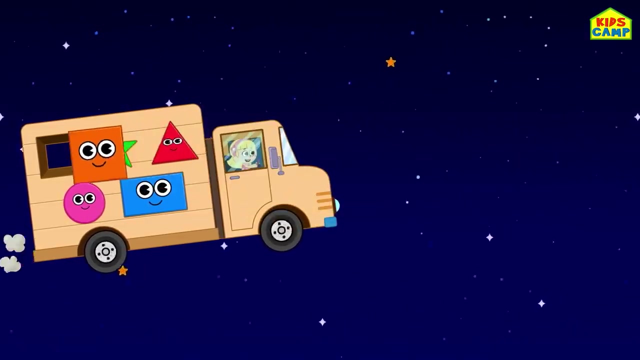 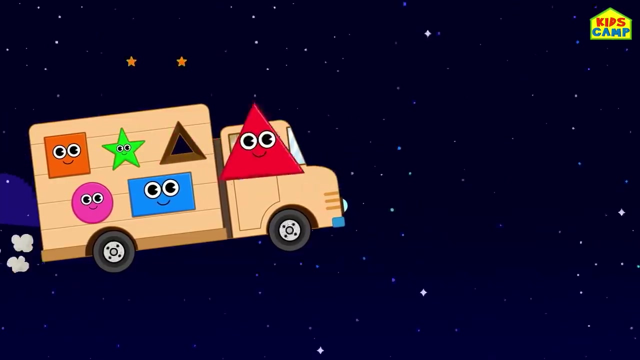 I see it, It's a star Wonderful. Let's place the star on my wooden truck. We've done it. We've collected all the shapes. Oh magic, Wow, Wow, Here I go. Square Star Triangle. 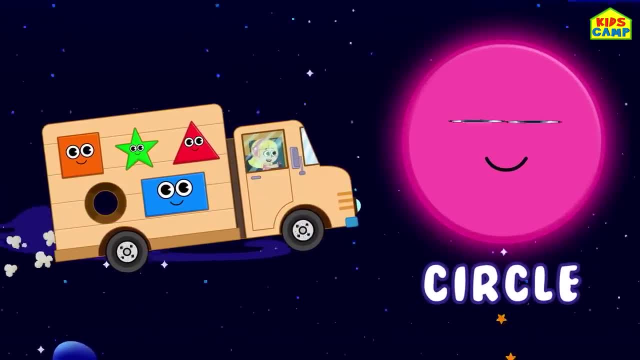 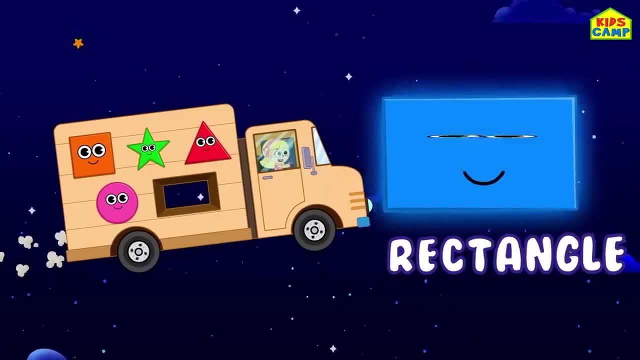 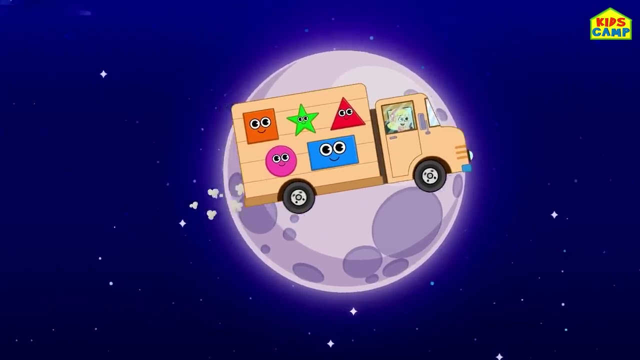 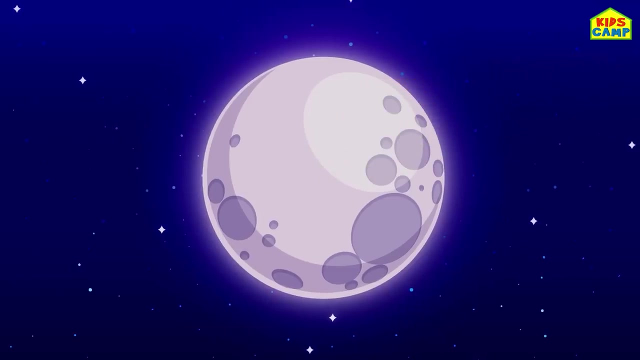 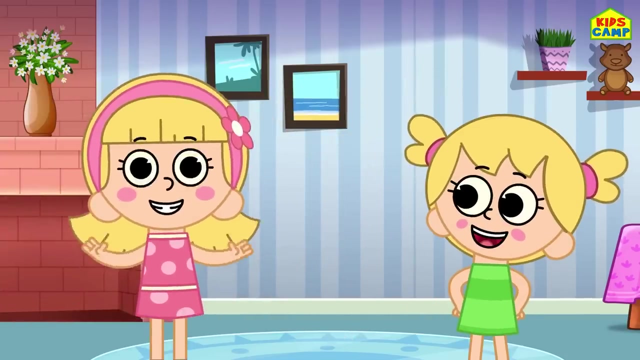 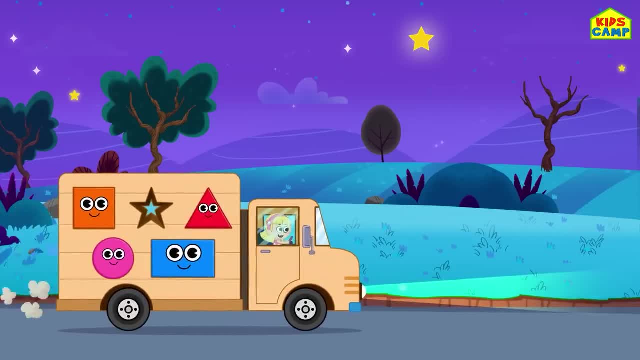 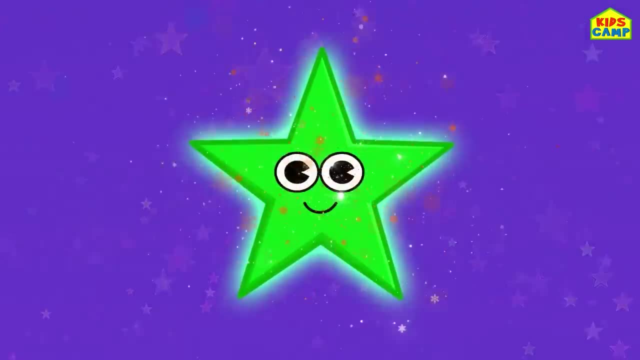 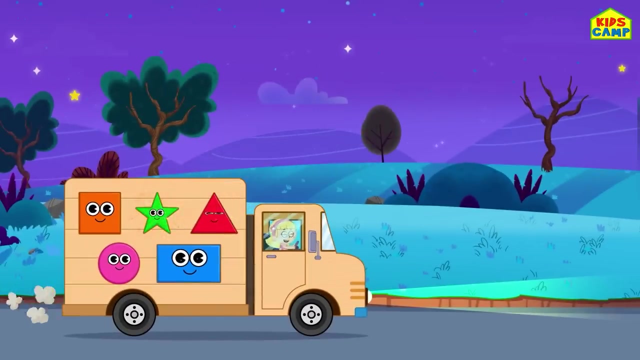 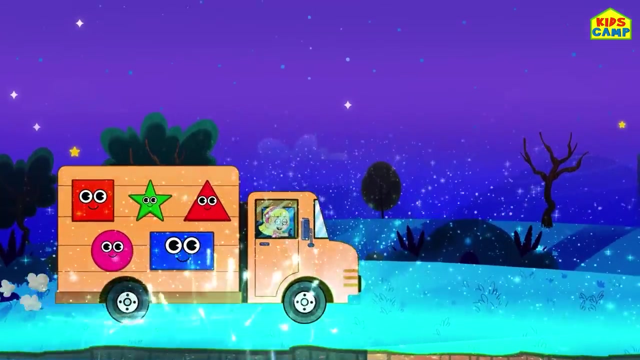 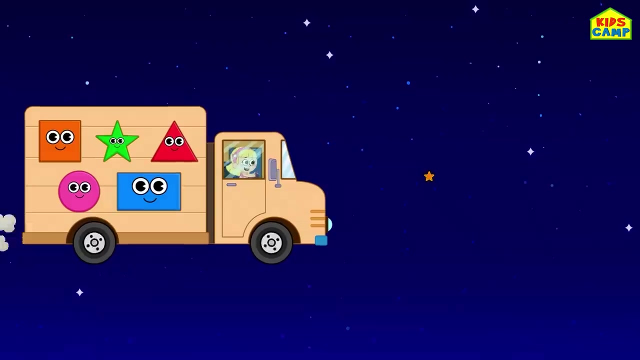 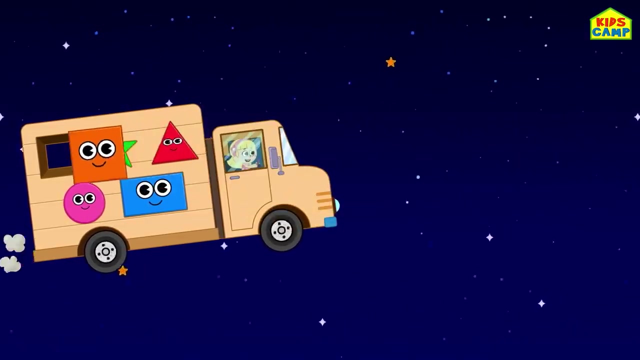 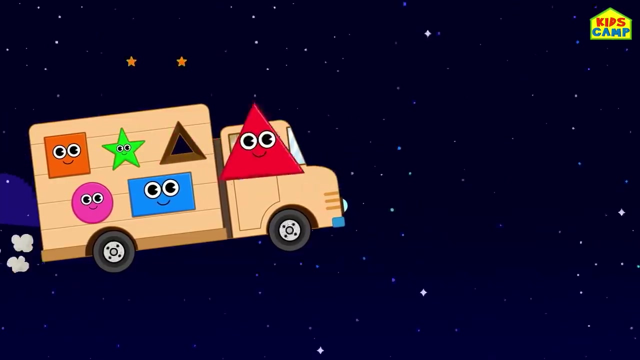 I see it, It's a star Wonderful. Let's place the star on my wooden truck. We've done it. We've collected all the shapes. Oh magic, Wow, Wow, Here I go. Square Star Triangle. 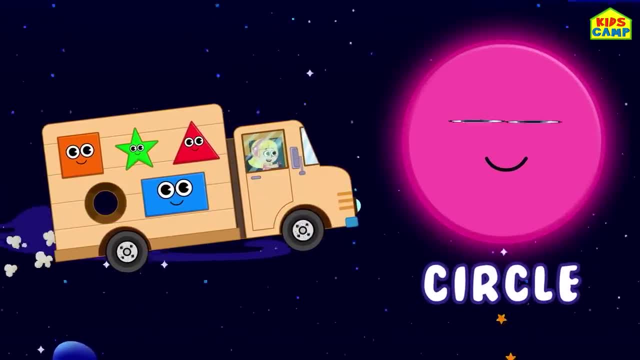 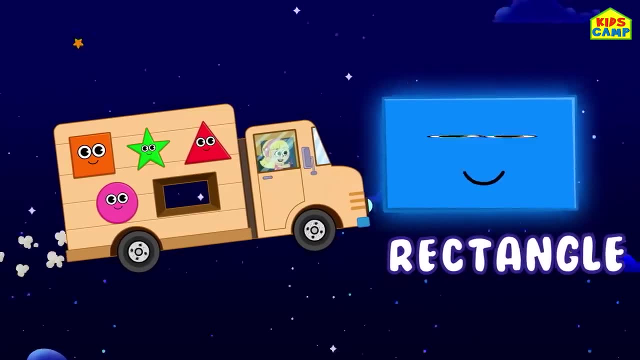 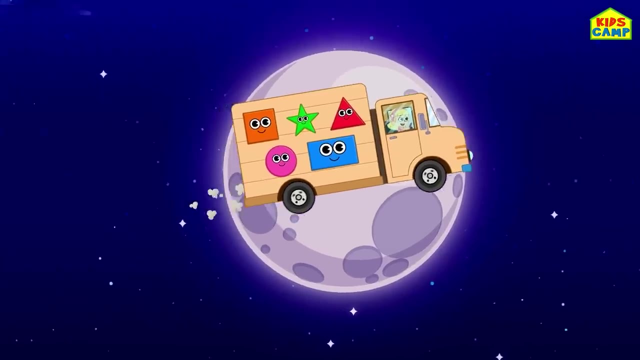 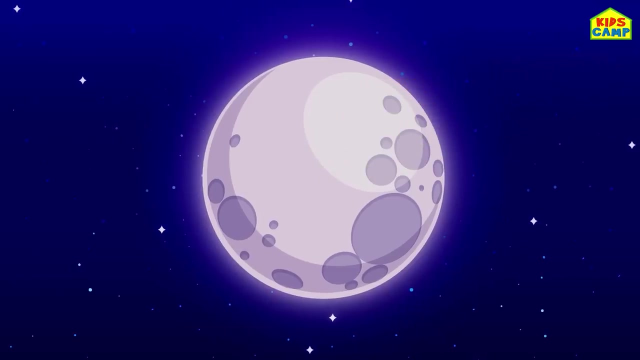 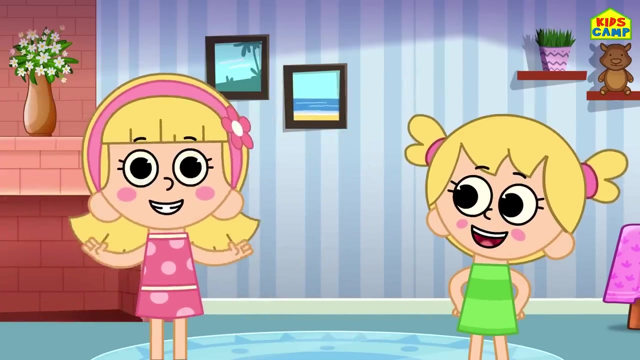 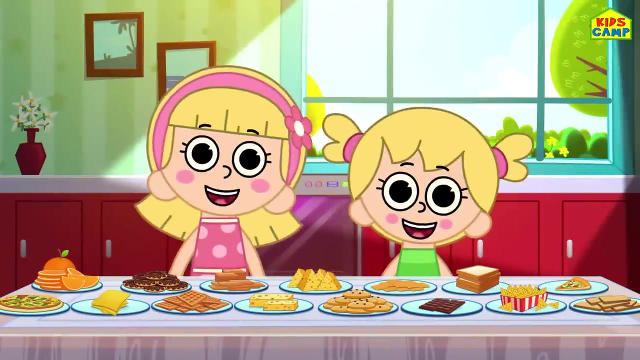 Circle And rectangle Over the moon, Here I go. Hi kids, I'm Ellie. Hi kids, I'm Ellie, and this is Eva, and today we are going to have a party. Yay Ooh, Look at all this food. 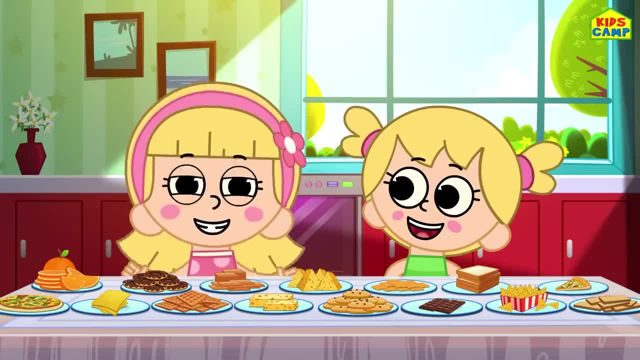 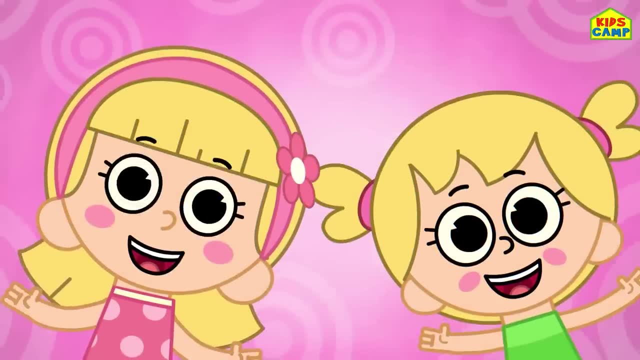 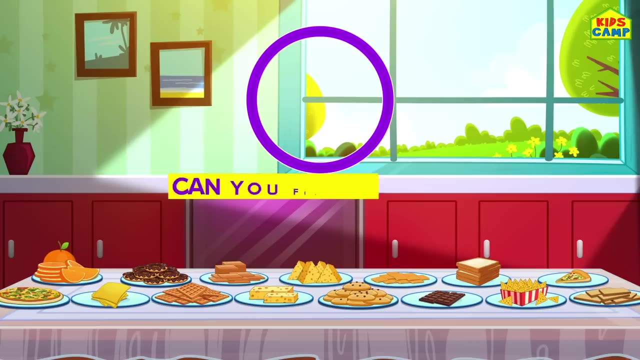 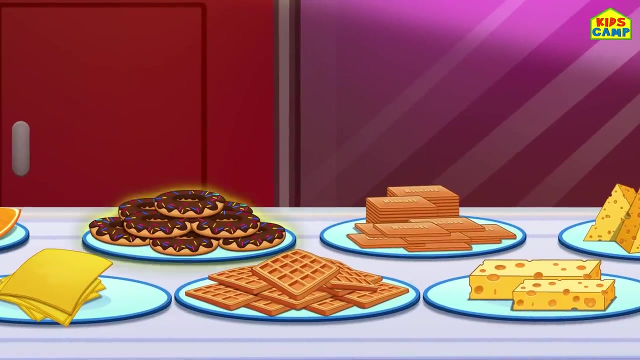 So delicious. We are also going to learn our shapes. Ready, Eva. Let's match the shapes with the food Circle. Can you find a circle? Where's a circle? What food is the shape of a circle? That's right, A doughnut. 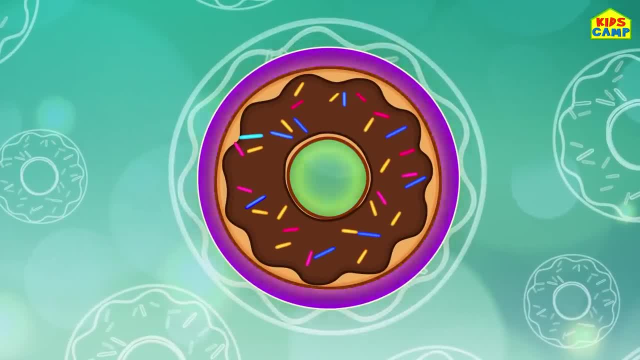 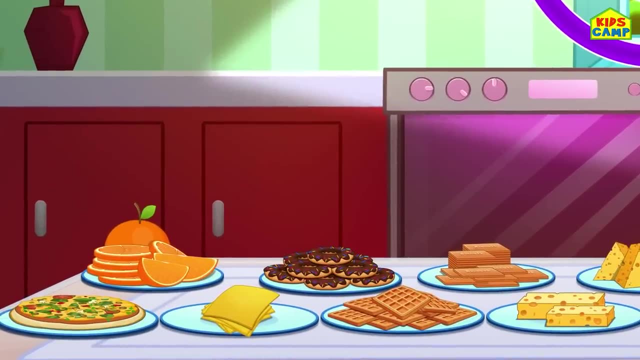 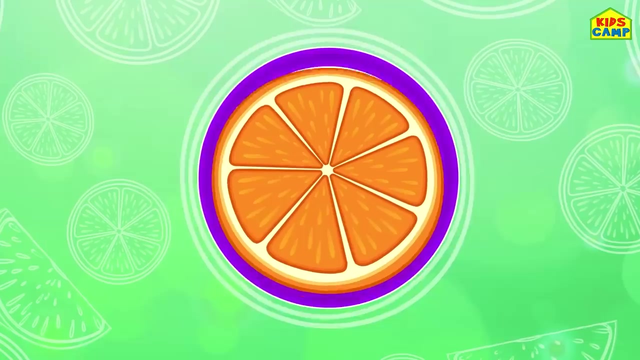 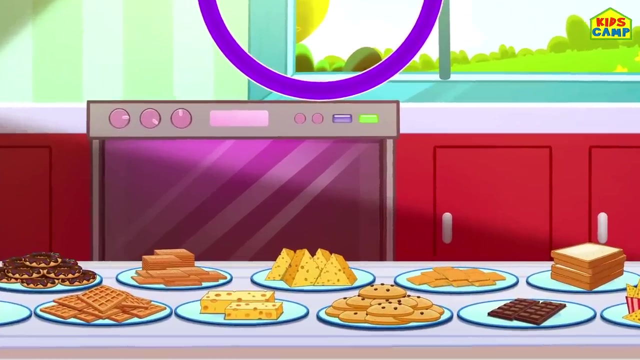 A doughnut is in the shape of a circle. What else? Hmm, That's right, An orange slice. Woohoo, An orange slice is also a circle. What else can we find? That's a circle? Hmm, A cookie. 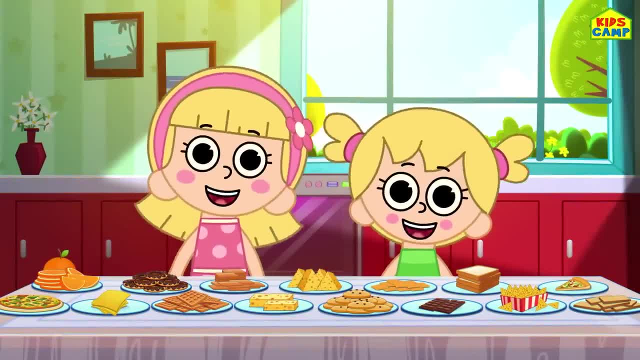 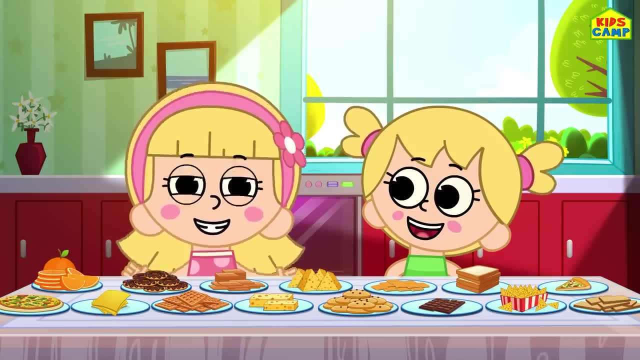 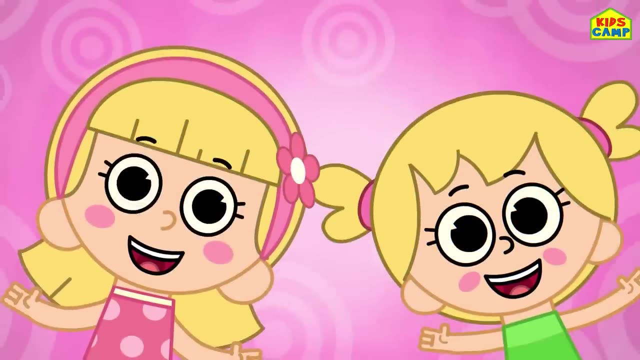 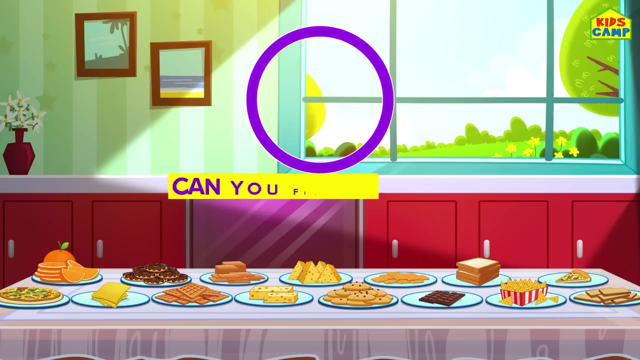 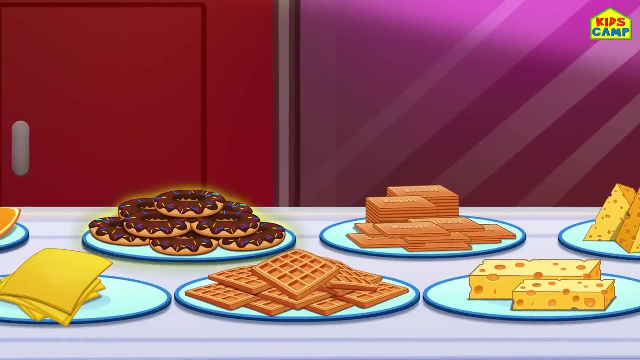 Yay Ooh, Look at all this food- So delicious. We are also going to learn our shapes. Ready Eva. Let's match the shapes with the food Circle. Can you find a circle? Where's a circle? What food is the shape of a circle? 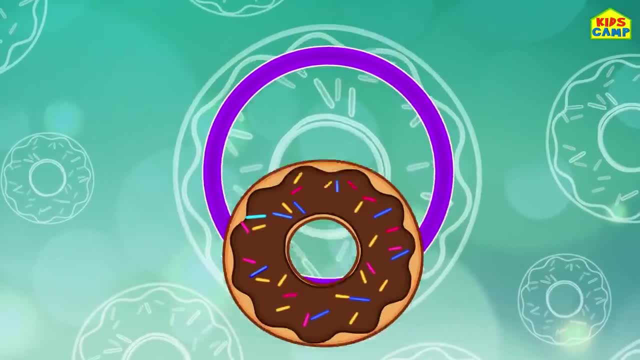 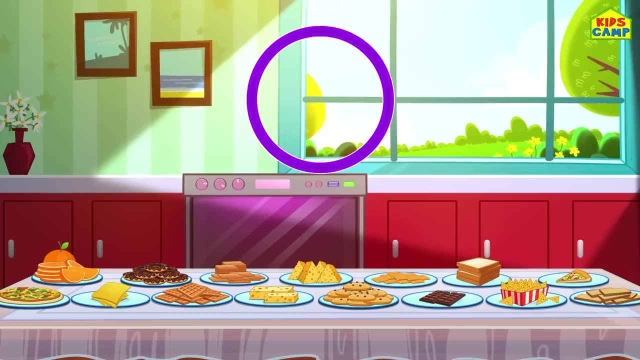 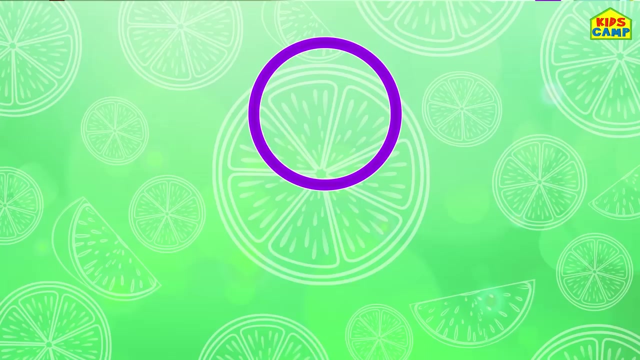 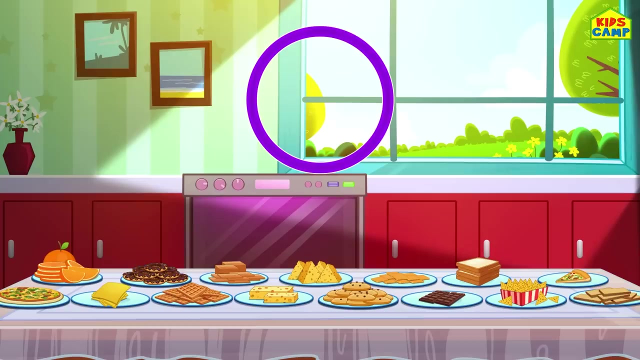 That's right, A doughnut. A doughnut is in the shape of a circle. What else? Hmm, That's right, An orange slice. Woohoo, An orange slice is also a circle. What else can we find? That's a circle. 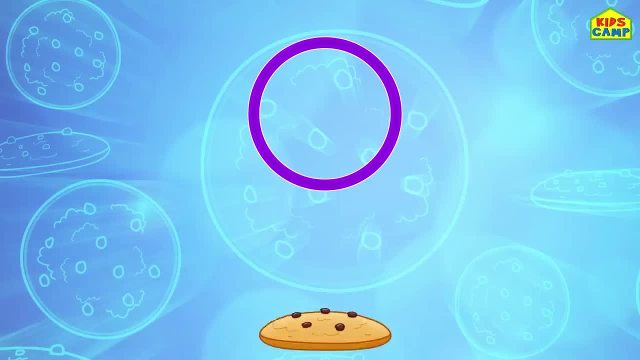 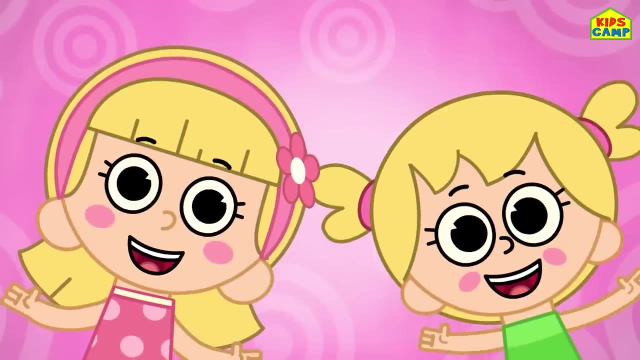 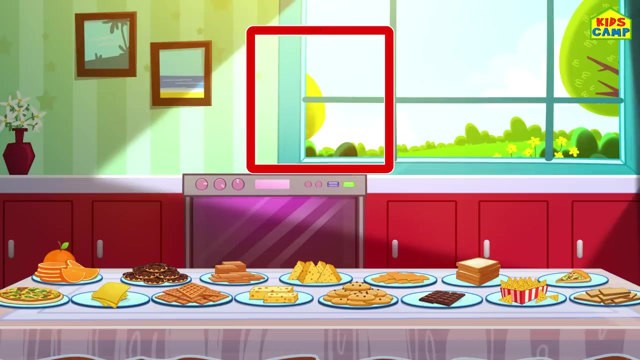 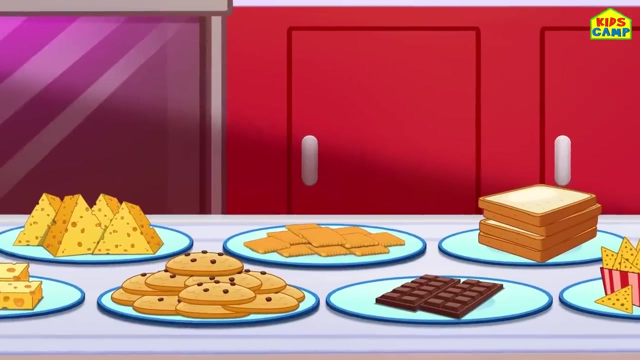 Hmm, A cookie. Yummy, A cookie is also a circle. Yay, What's the next shape? A square. Hmm, Can you find a square? kids, What food is in the shape of a square? Hmm, That's right, A craggle. 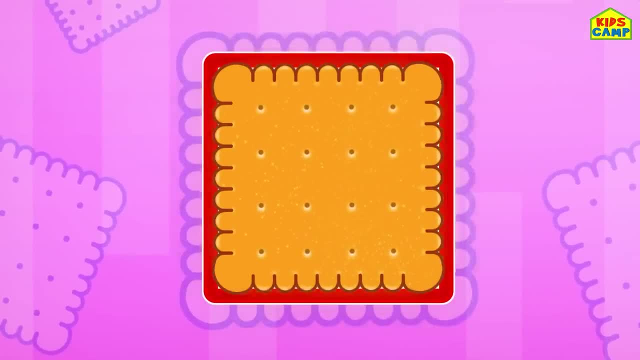 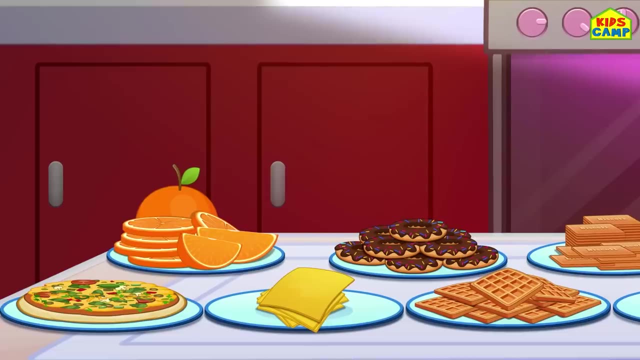 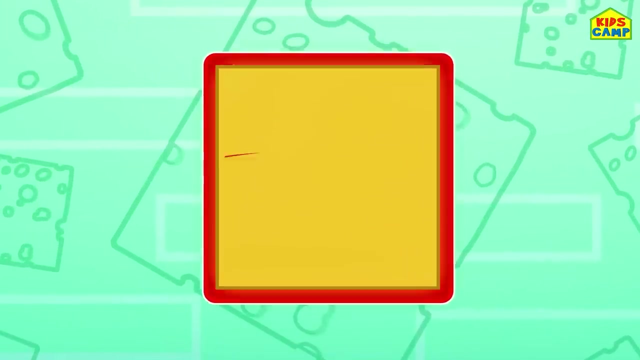 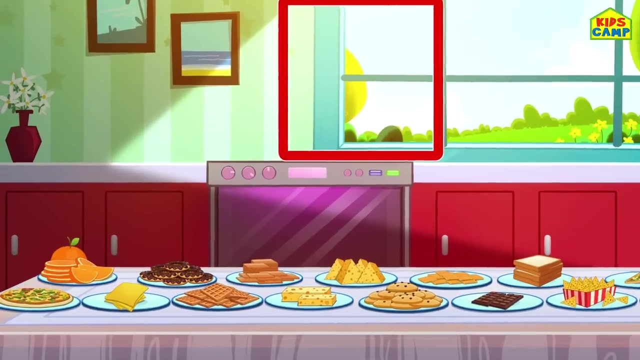 Yummy, That's the shape of a square. What else can we find that's a square? Aha, A slice of cheese. That's right, A slice of cheese is also a square. What else is a square? Aha, I see it. 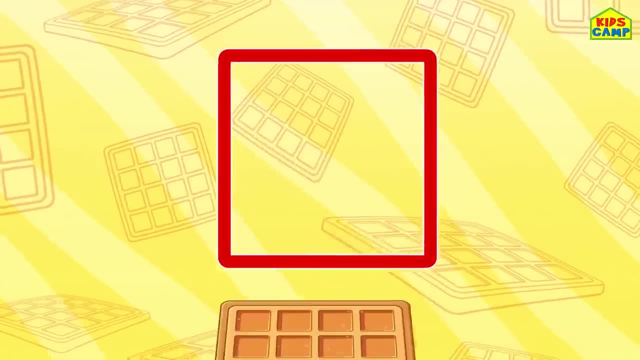 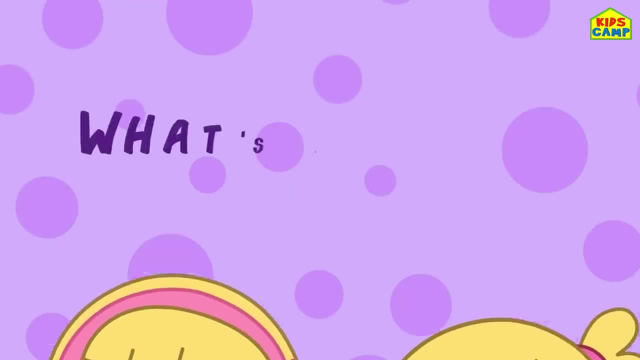 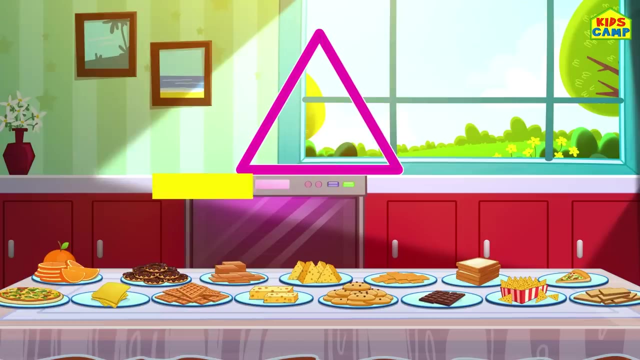 A waffle. A waffle is in the shape of a square. Yay. What's the next shape? A triangle. Can you find a triangle? Hmm, Do you see it? I see it too, Nachos, Yay. 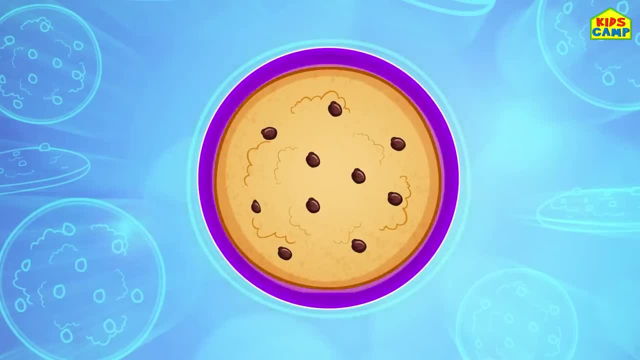 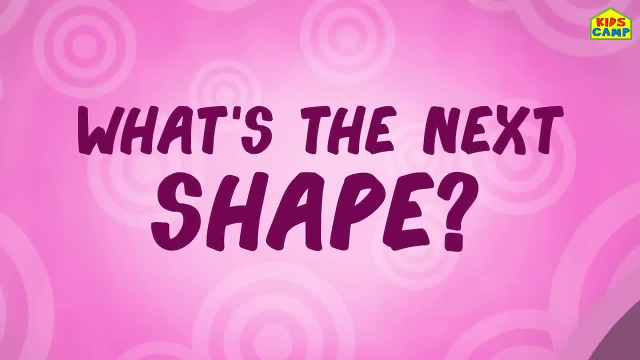 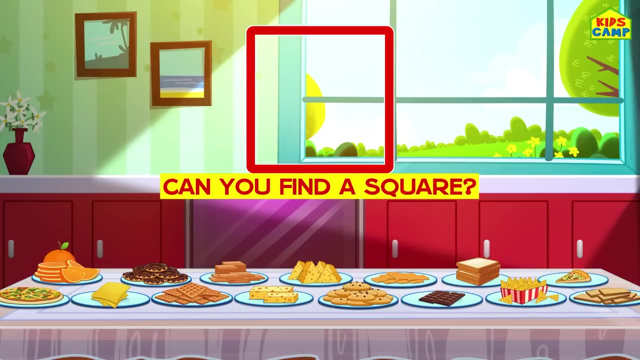 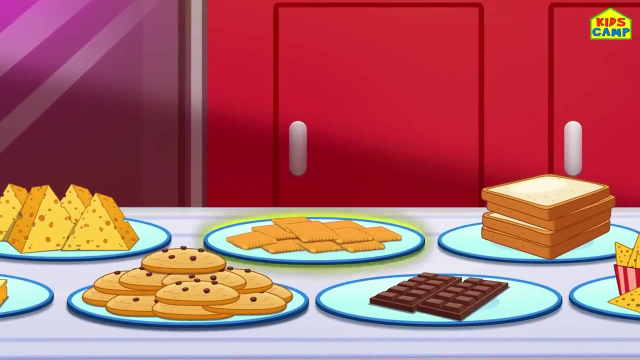 Yummy, A cookie is also a circle, Yay. What's the next shape? A square, Hmm. Can you find a square, kids? What food is in the shape of a square? Hmm, That's right, A craggle. 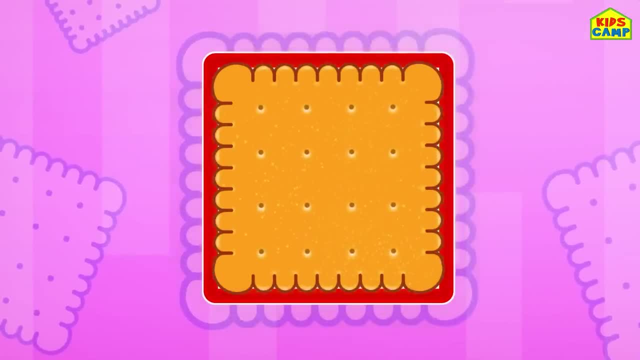 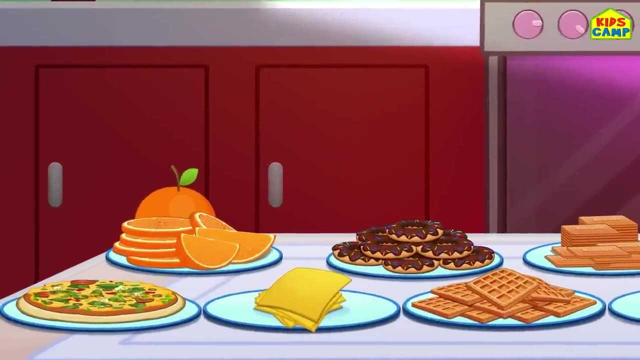 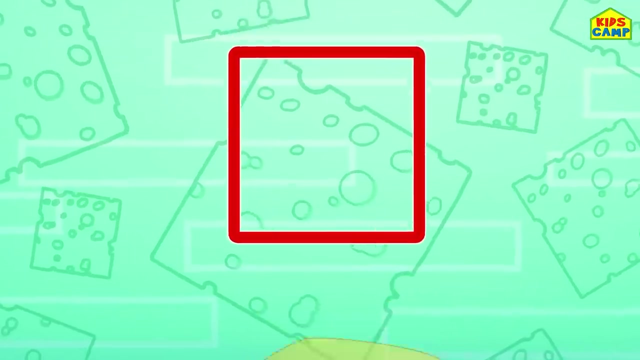 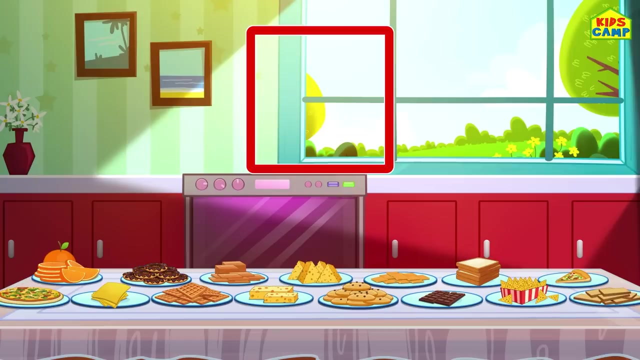 Yummy, That's the shape of a square. What else can we find that's a square? Aha, A slice of cheese. That's right, A slice of cheese is also a square. What else is a square? Aha, I see it. 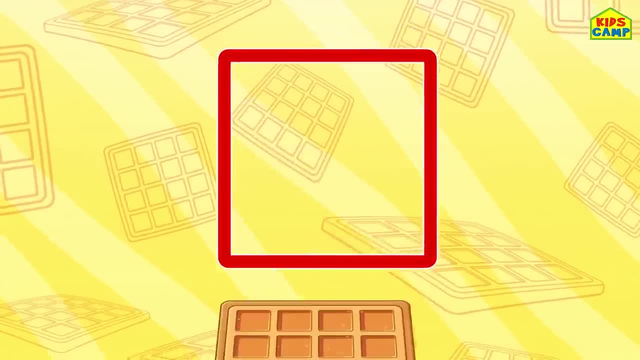 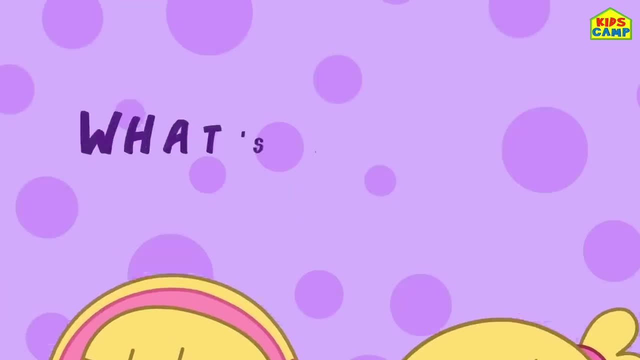 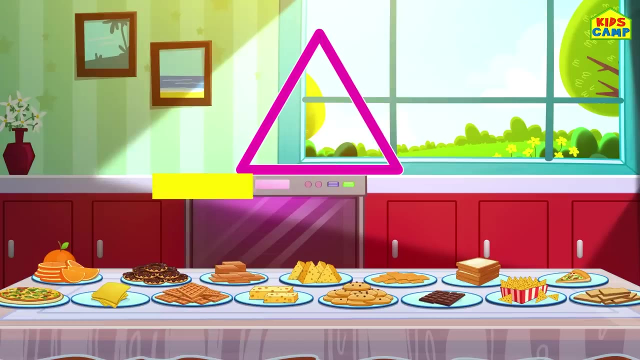 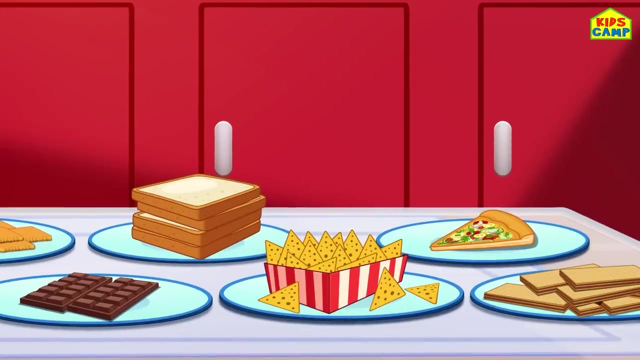 A waffle. A waffle is in the shape of a square. Yay, What's the next shape? A triangle, A triangle. Can you find a triangle? Hmm, Do you see it? I see it too, Nachos. 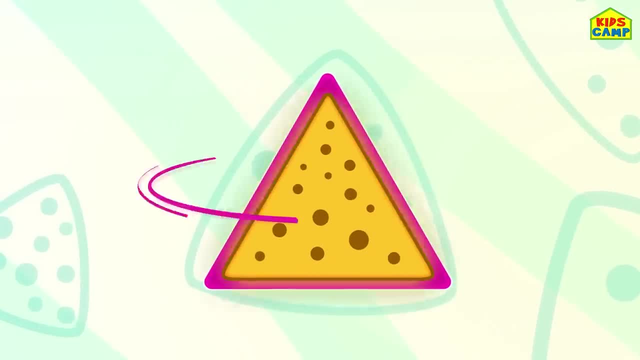 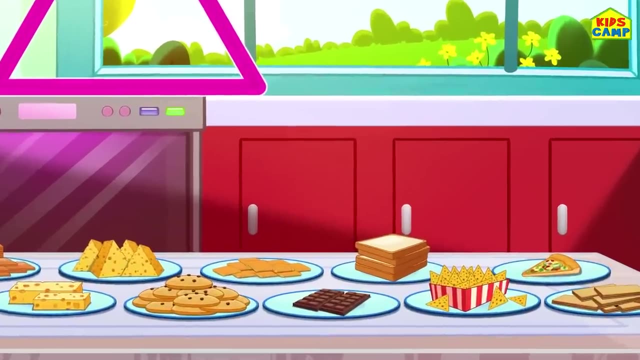 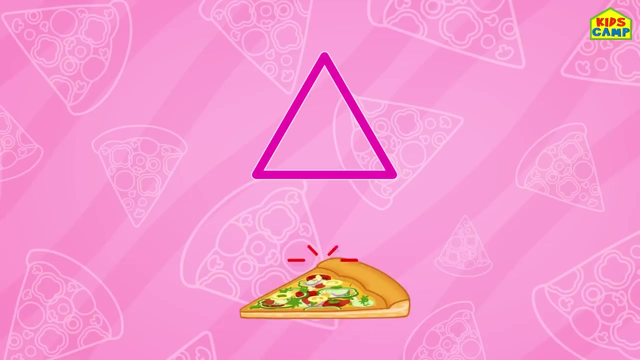 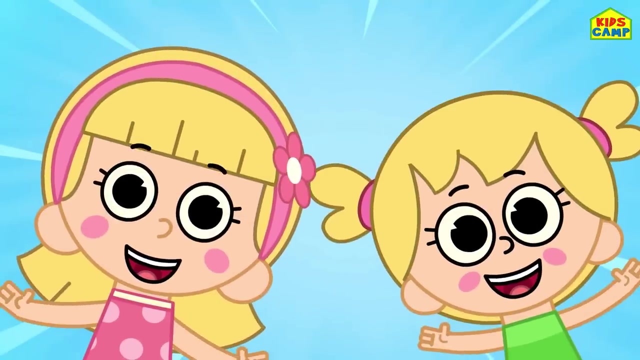 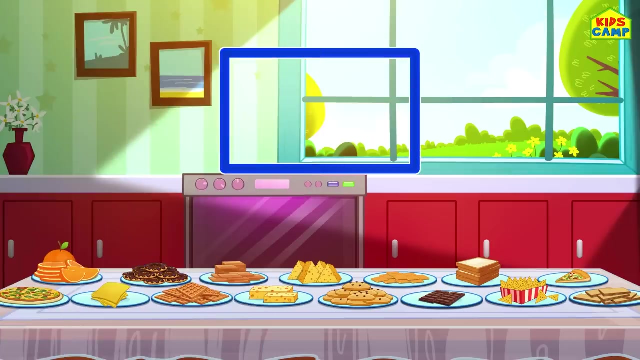 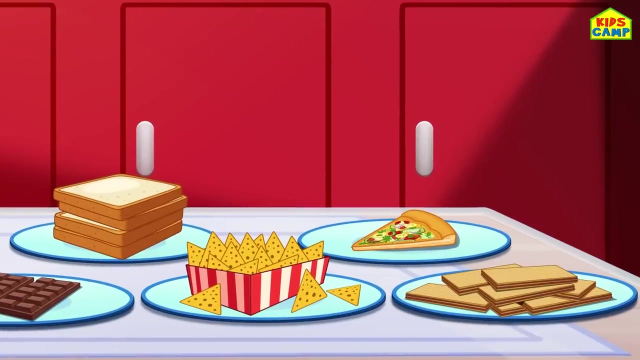 Yay, A nacho is in the shape of a triangle. What else That's right? Everyone's favourite, a slice of pizza. that sure is a triangle. what's the next shape? a rectangle. can you find a rectangle, kids? ah, I see it. 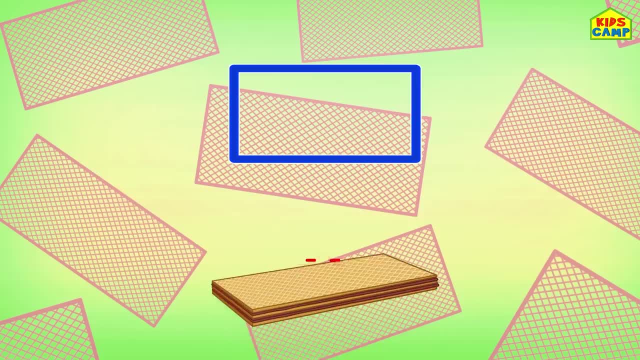 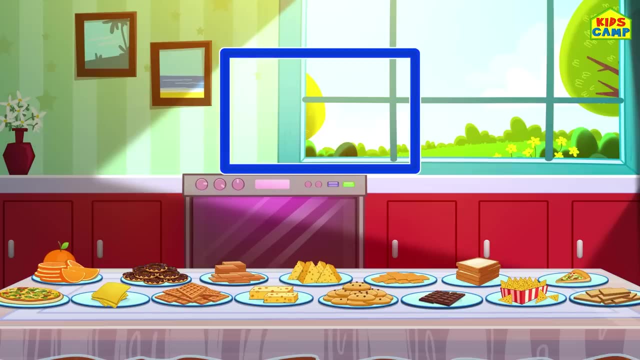 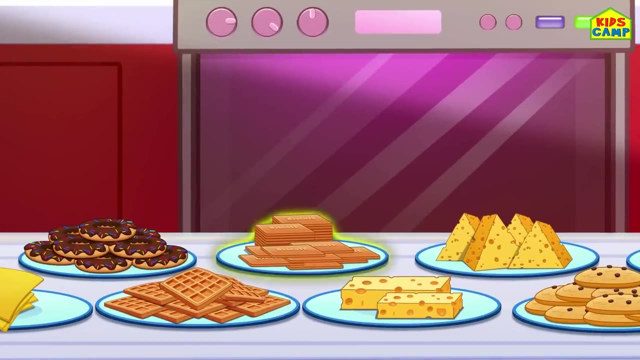 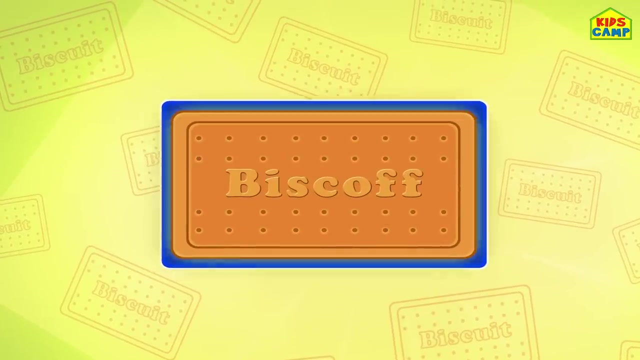 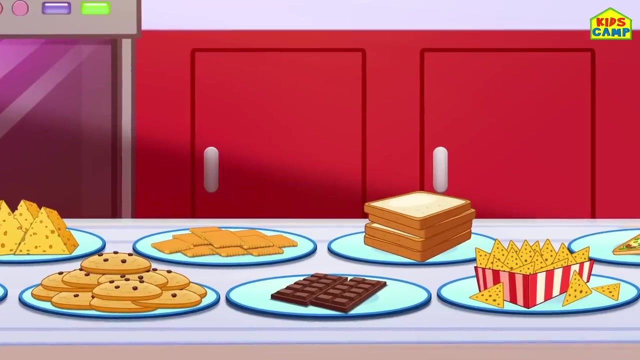 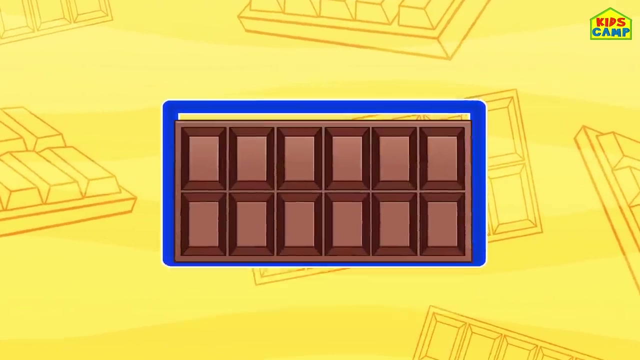 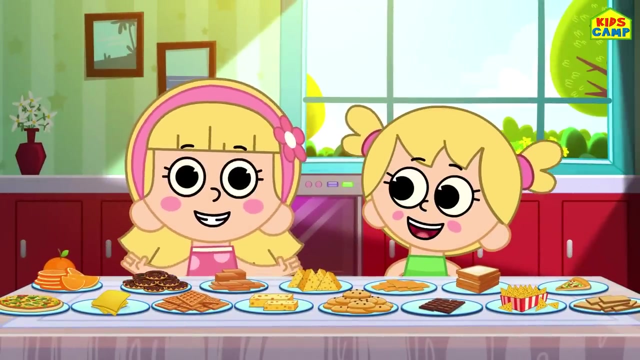 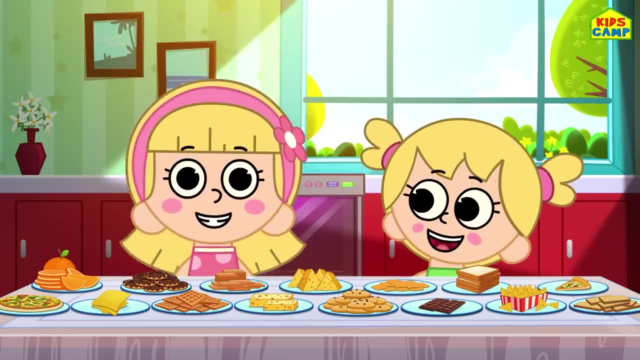 to a chocolate wafer. that also is a rectangle. that sure is the shape of a rectangle. anything else? uh-huh chocolate, a bar of chocolate. that's right, kids, we did it. this all looks so good and you found all the shapes. good job Eva, good job kids. bye-bye, what a. 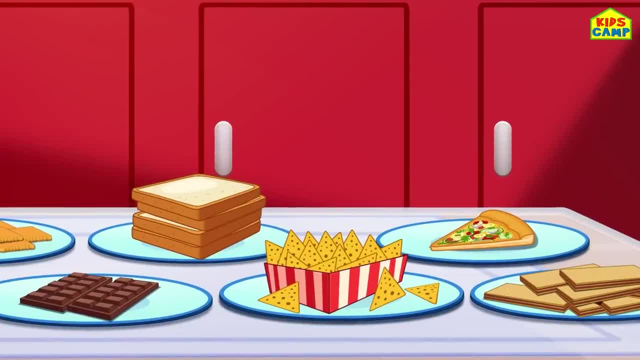 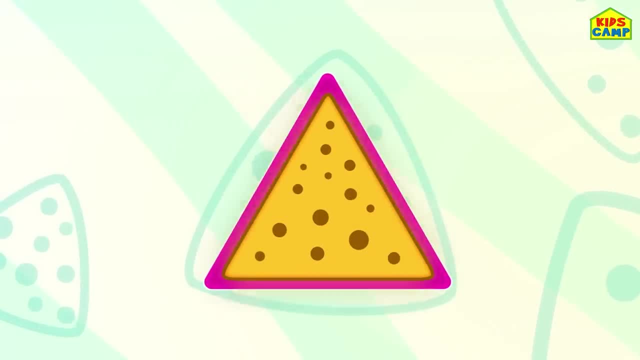 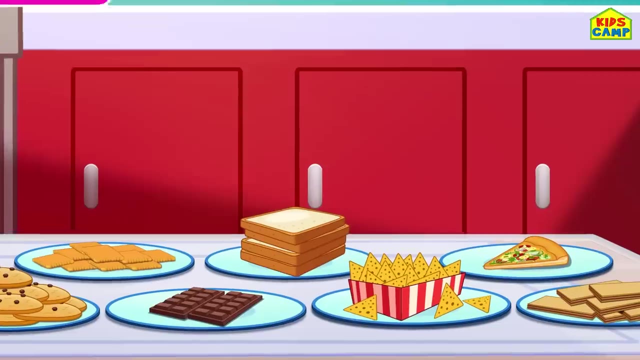 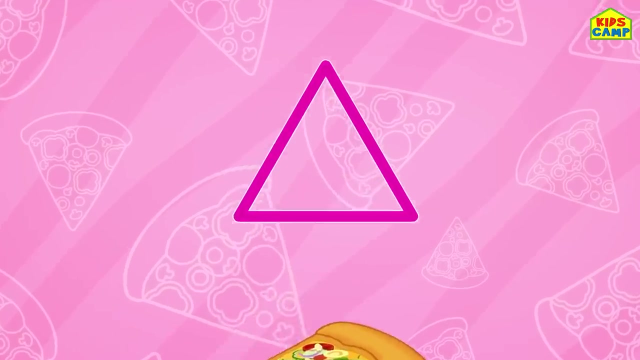 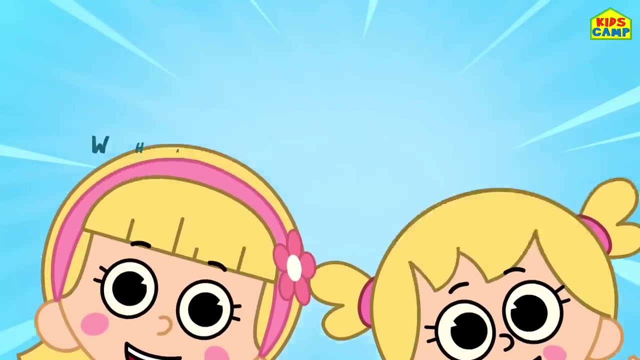 A nacho is in the shape of a triangle. What else? That's right, Everyone's favourite. A slice of pizza, A slice of pizza, Yay. A slice of sausage- A slice of sausage, That's right, one's favorite slice of pizza. that sure is a triangle, yay. what's the next shape? 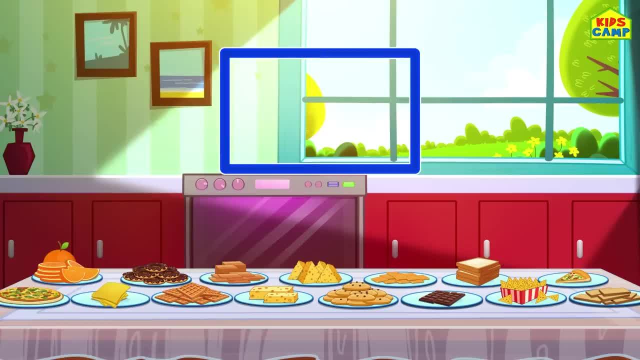 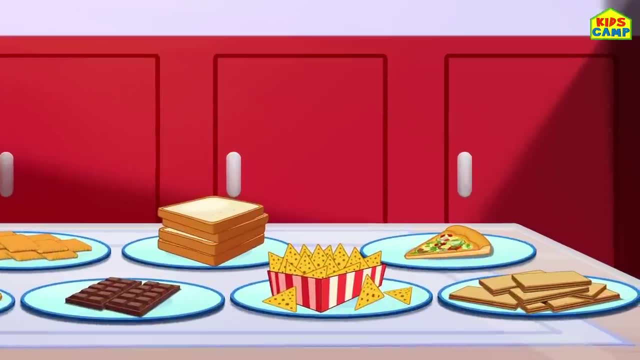 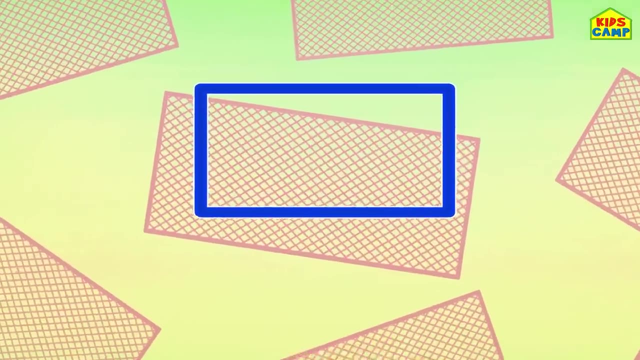 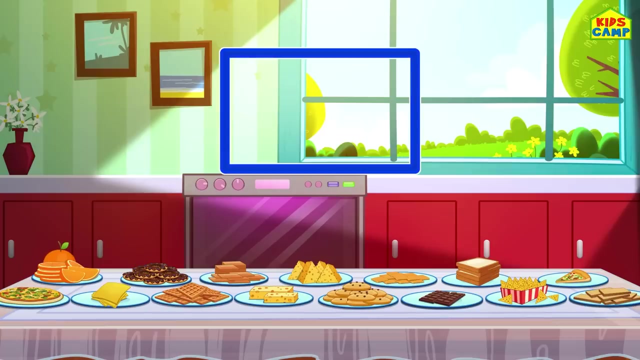 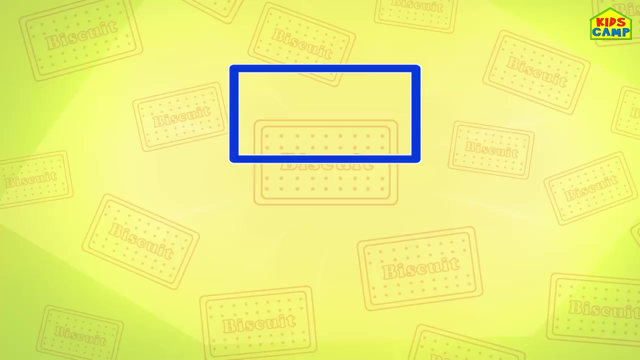 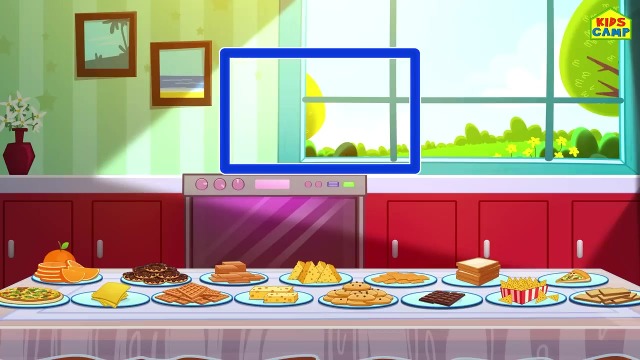 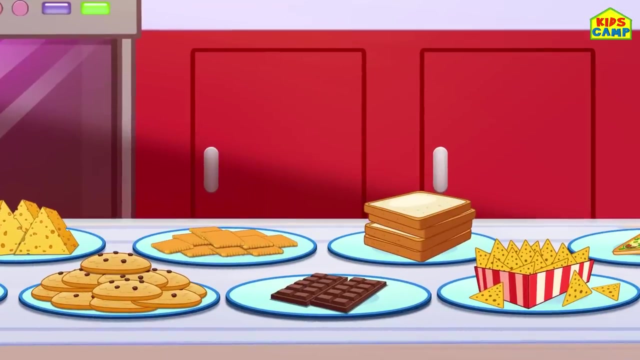 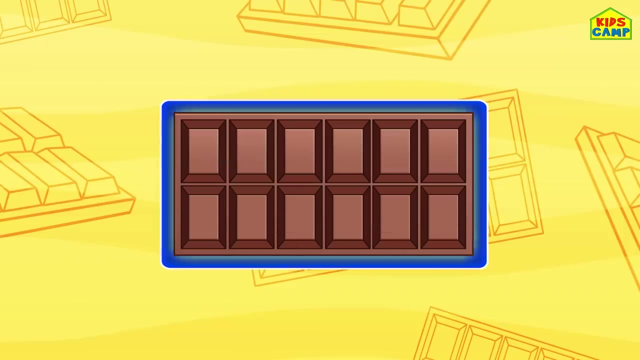 a rectangle. can you find a rectangle, kids? ah, I see it too. a chocolate wafer, that also is a rectangle. yay, what else? what's that yummy biscuit, that sure is the shape of a rectangle. anything else, uh-huh, chocolate, a bar of chocolate. that's right, kids, we did it this all. 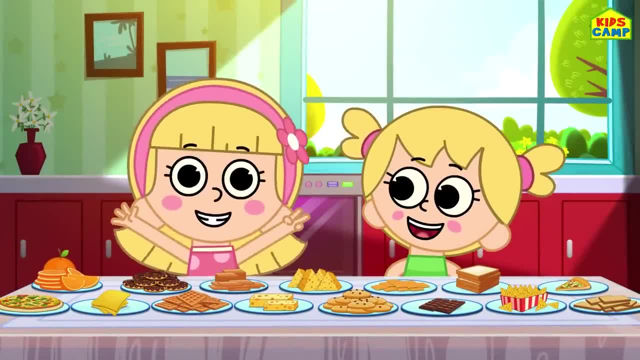 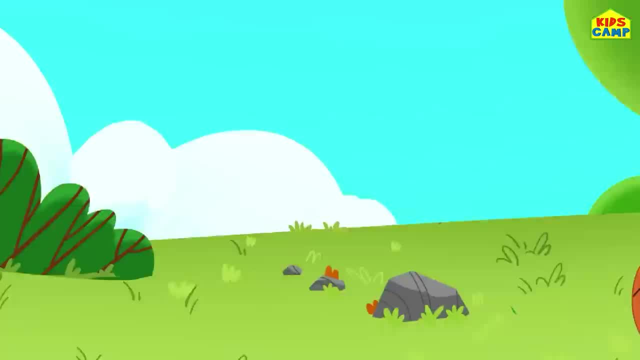 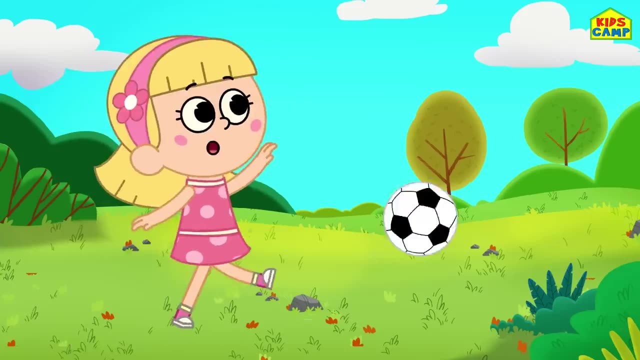 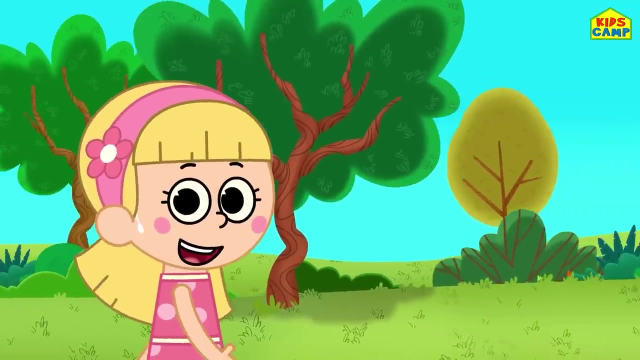 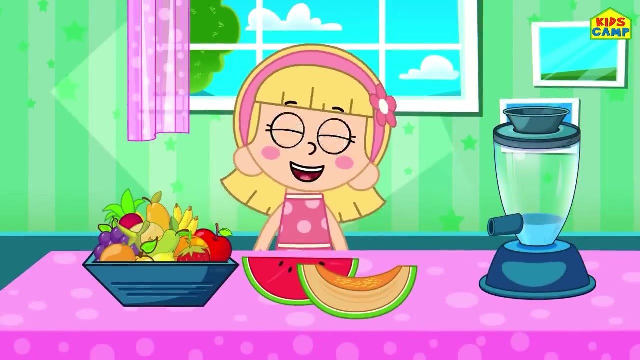 looks so good and you found all the shapes. good job, Eva. good job kids by by. what a perfect sunny day to play outside, oh yay. what should we do to beat this heat? I know let's make summer coolers. hey friends, what food should we pick today? 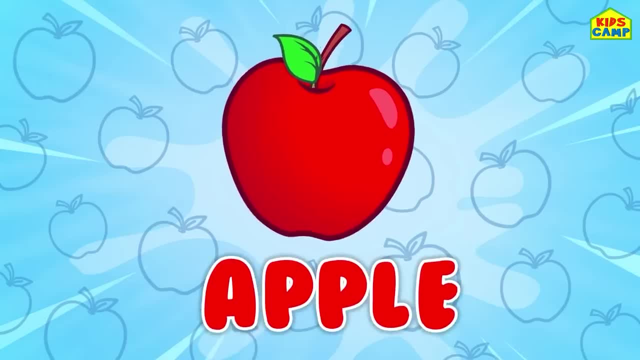 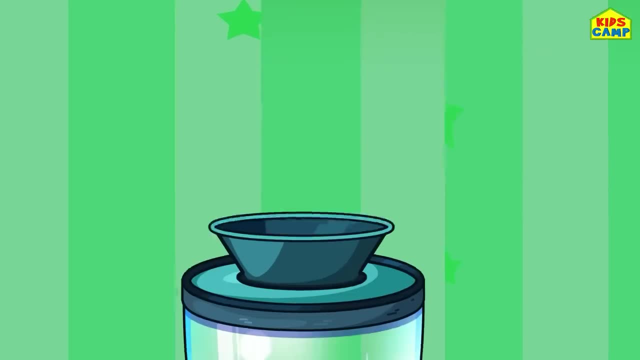 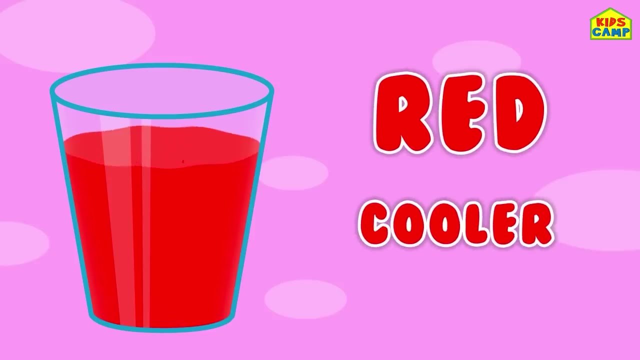 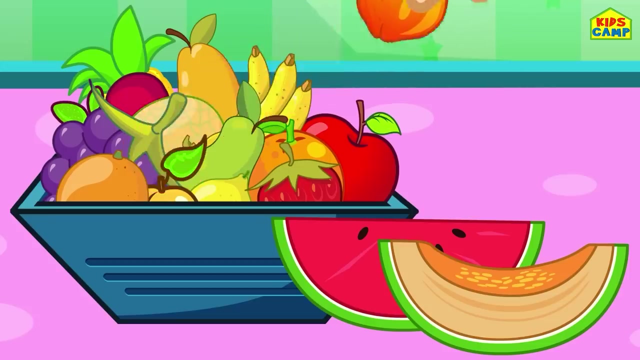 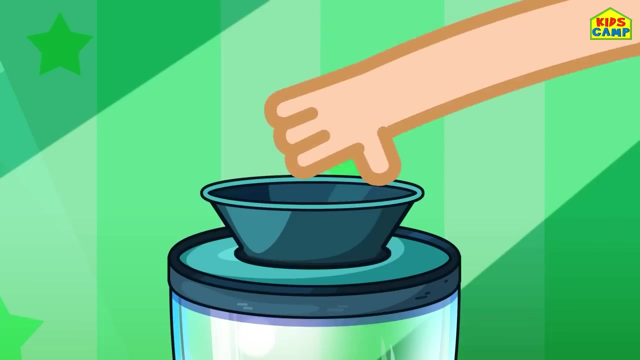 First a scrumptious apple, a yummy strawberry and a juicy watermelon. Let's blend them up. Yay, A red cooler. Let us give them another go. I'm going to take a yummy papaya, an orange and a juicy melon. 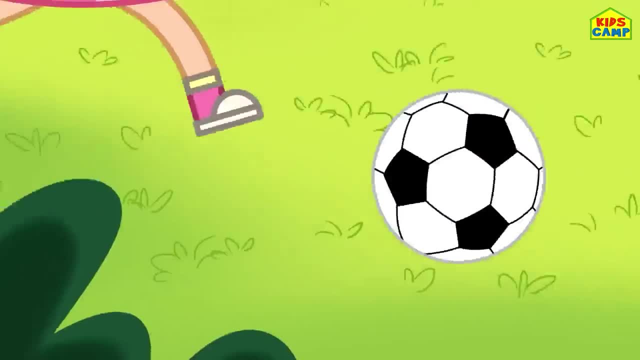 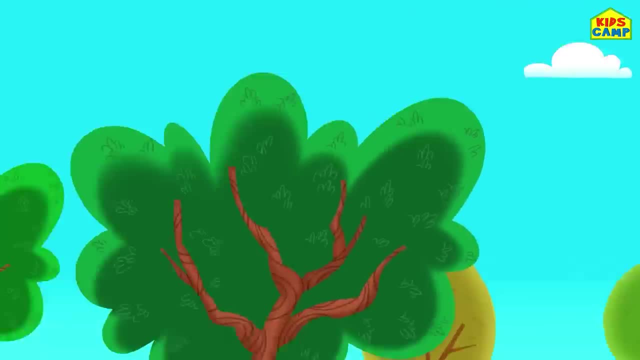 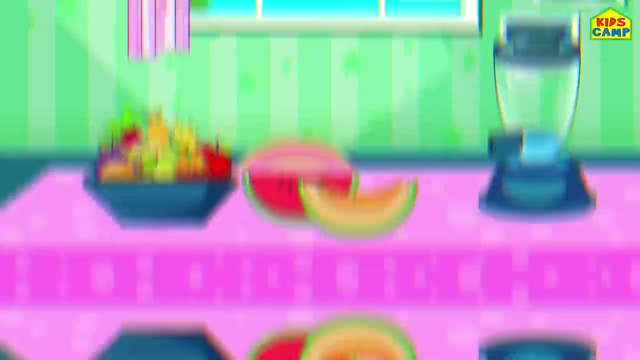 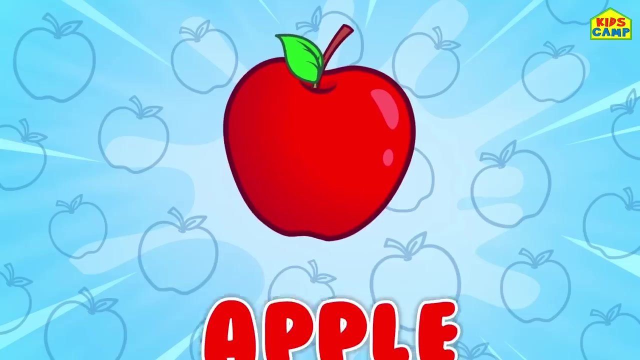 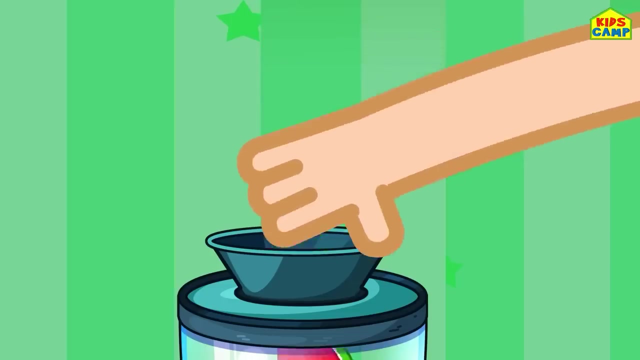 perfect sunny day to play outside. oh yay. what should we do to beat this heat? I know let's make summer coolers. hey friends, what fruit should we pick first? a scrumptious Apple, a yummy strawberry and a juicy watermelon. let's blend them up, yay. 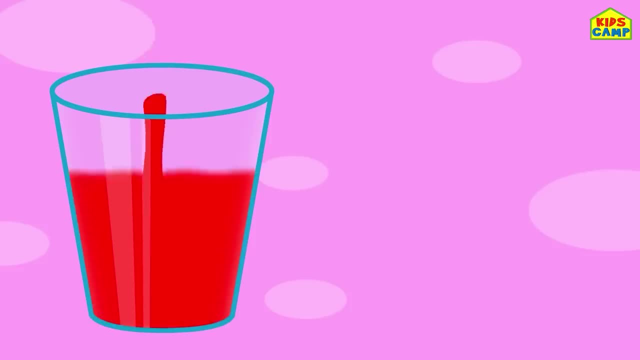 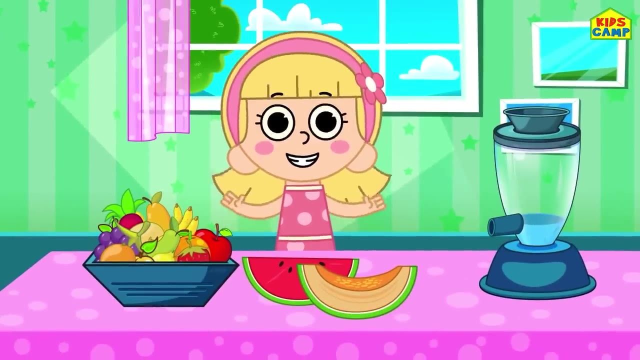 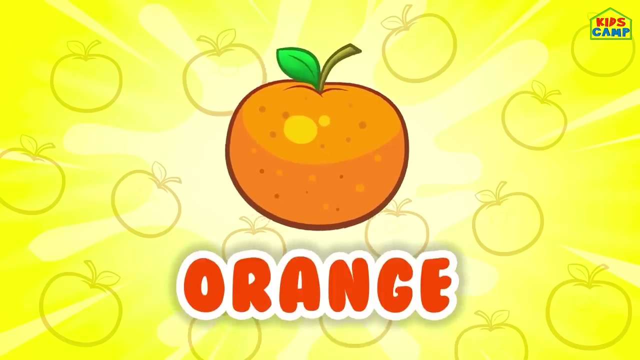 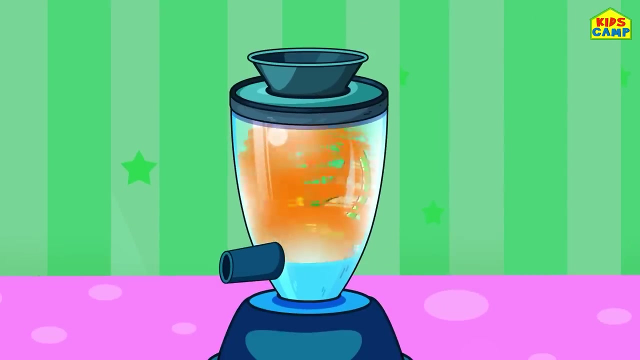 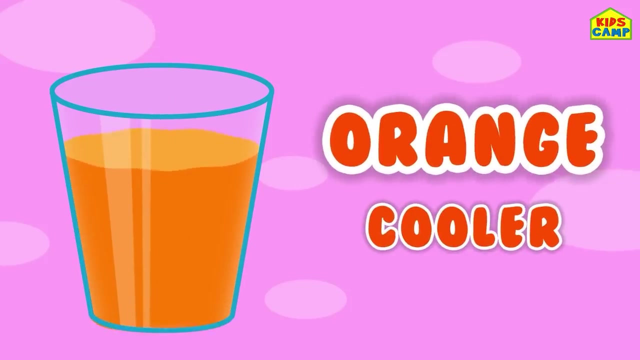 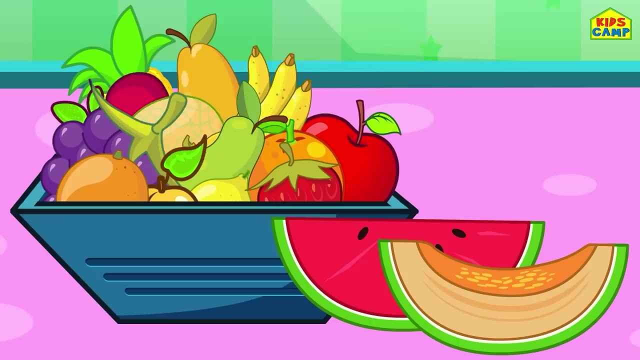 a red. cooler, let us give them another go. I'm going to take a yummy papaya and orange and a juicy melon. in they go. let's mix them up. whoohoo and orange- no, 77 percent. ya, baby, orange Cooler, let's try another one. this time I'm going to take a banana and a. 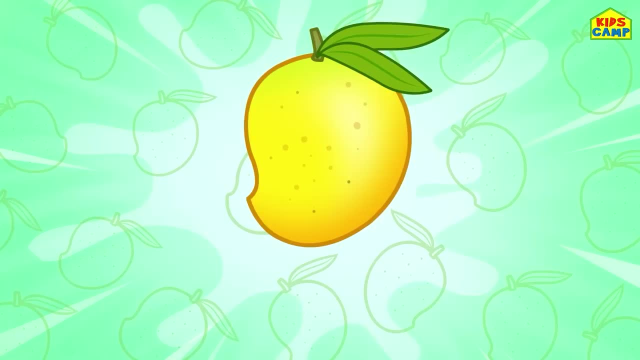 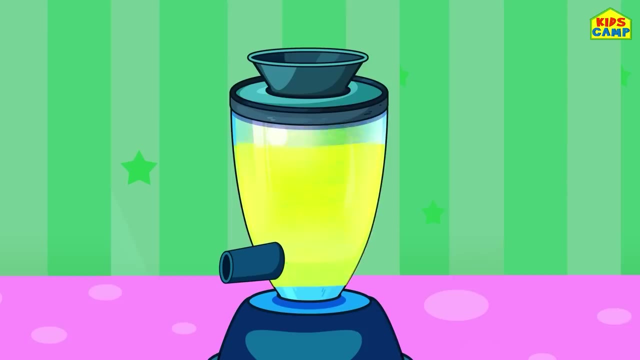 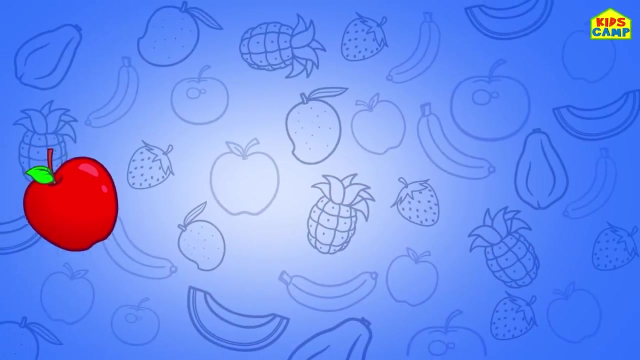 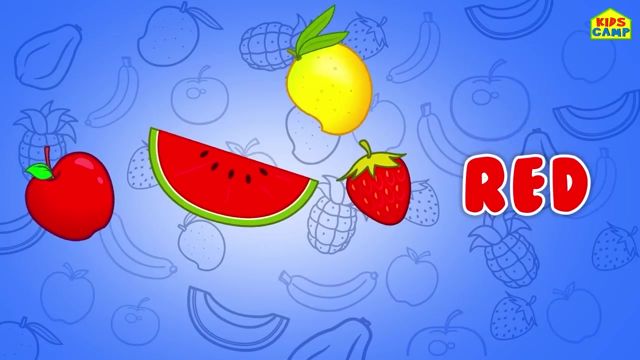 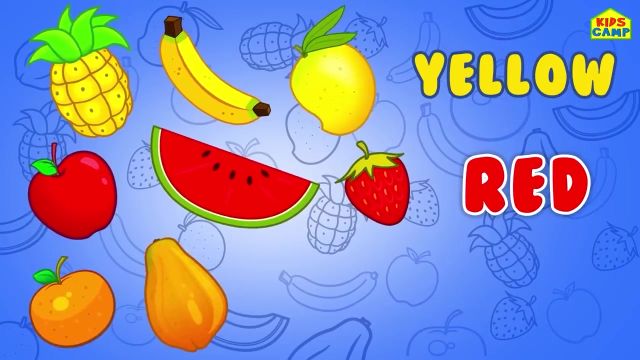 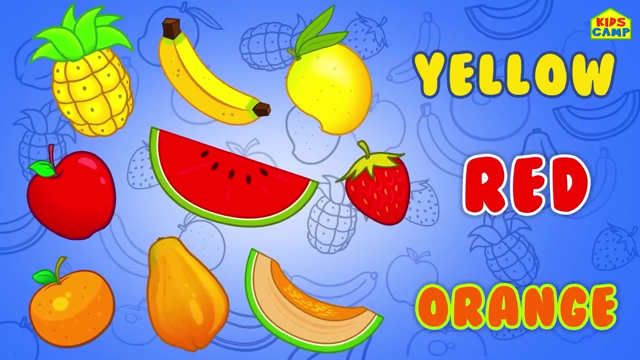 pineapple and a yummy mango. in they go. let's mix them up a yellow cooler. today we learned that apples, watermelons and strawberries are red, mangoes, bananas and pineapples are yellow, oranges, papayas and melons are orange in color. we had a fun learning day and delicious summer. 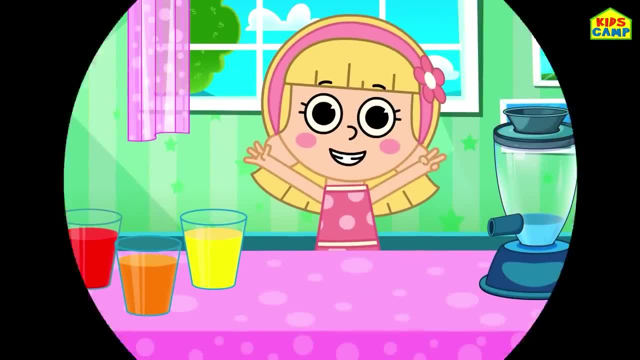 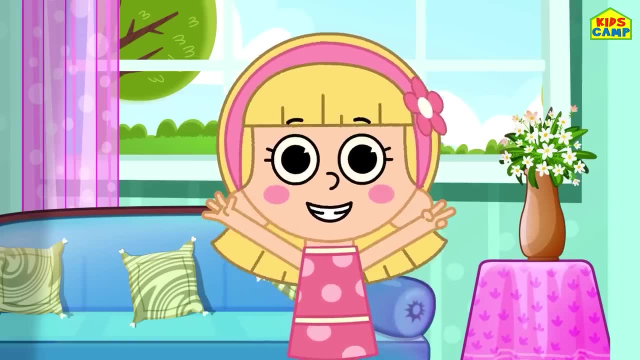 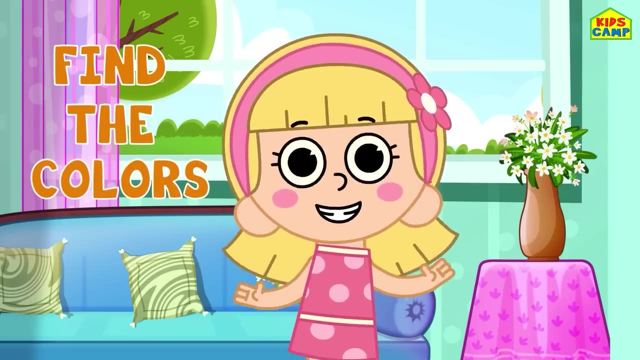 cooking colors to drink. yay, hi, I'm Ellie, and today we're going to play a fun game with colors. that's right, we all love colors, don't we? we have to find all the different types of colors, as mentioned on the buckets. the first color that we 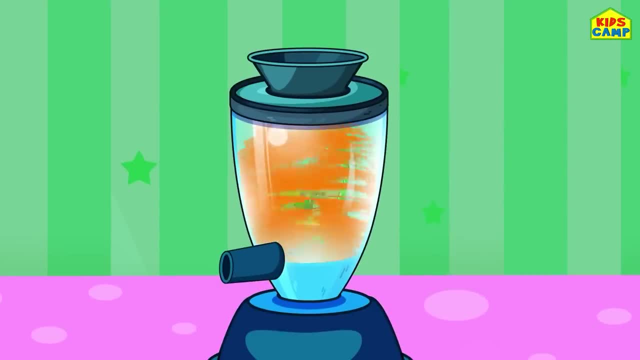 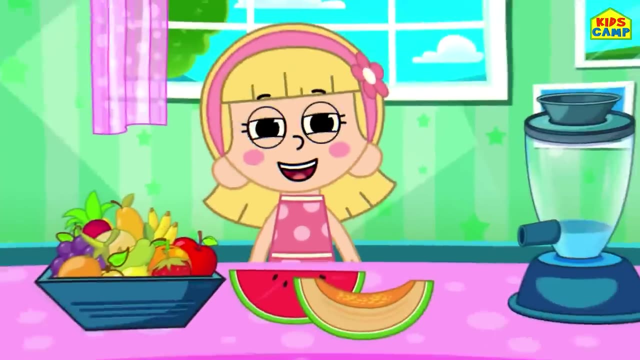 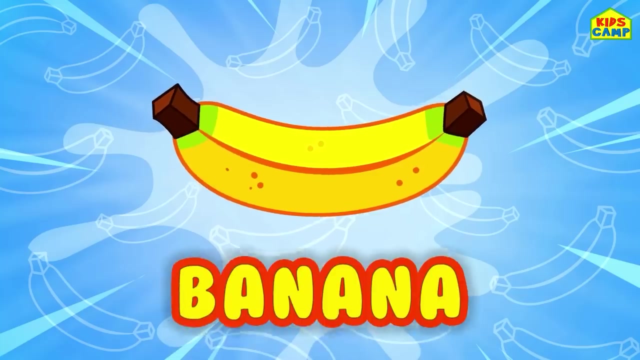 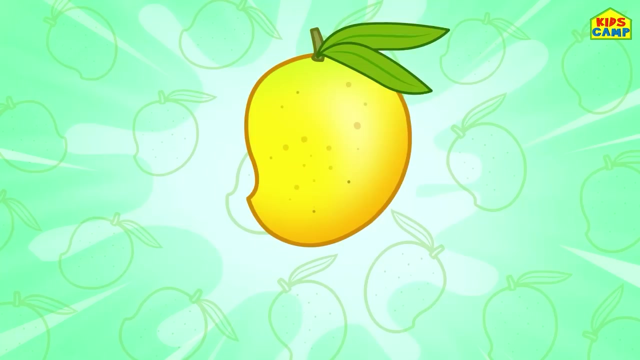 In they go. Let's mix them up. Woohoo, An orange. cooler, Let's try another one. This time I'm going to take a banana and a pineapple and a yummy mango. Woohoo, In they go. 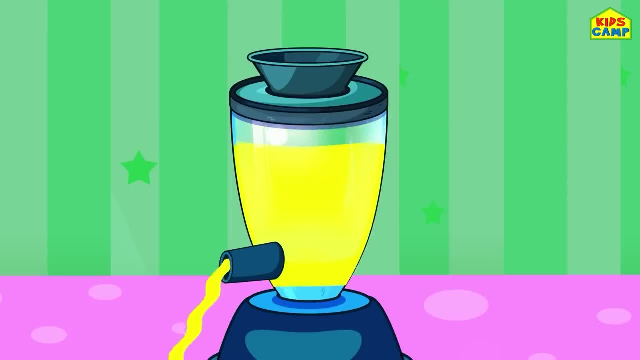 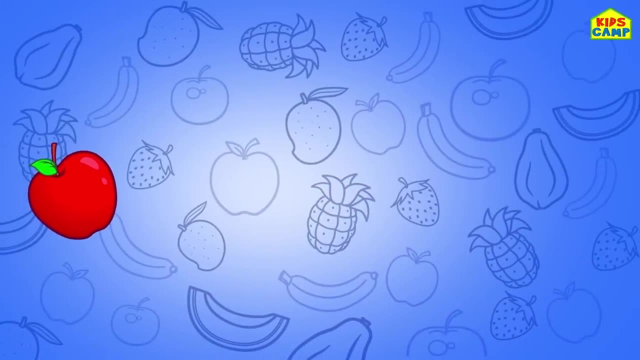 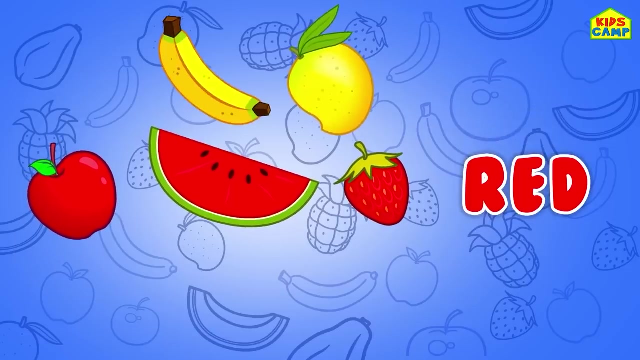 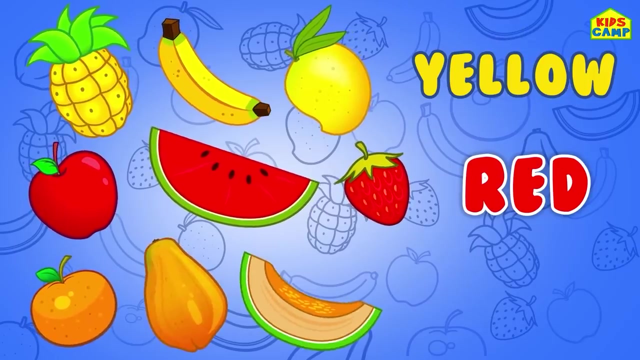 Let's mix them up. A yellow cooler: Wow. Today we learned that apples, watermelons and strawberries are red Mango, Tomatoes, bananas and pineapples are yellow Oranges, papayas and melons are orange in color. 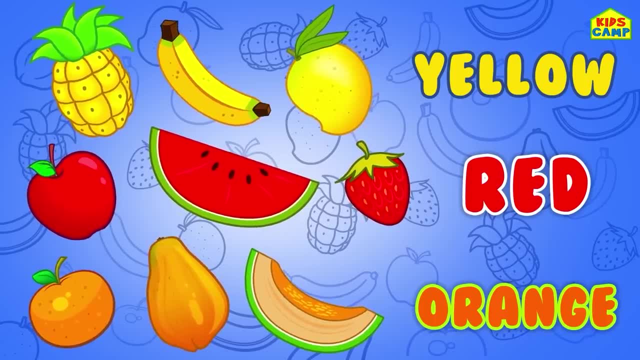 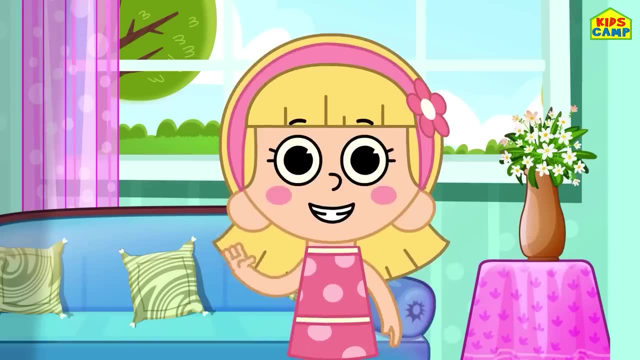 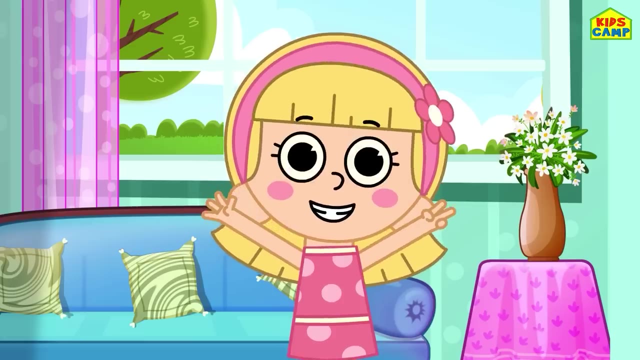 Yay, We had a fun learning day And delicious summer coolers to drink. Yay, Hi, I'm Ellie, And today we're going to play a fun game with colors. That's right, We all love colors, don't we? 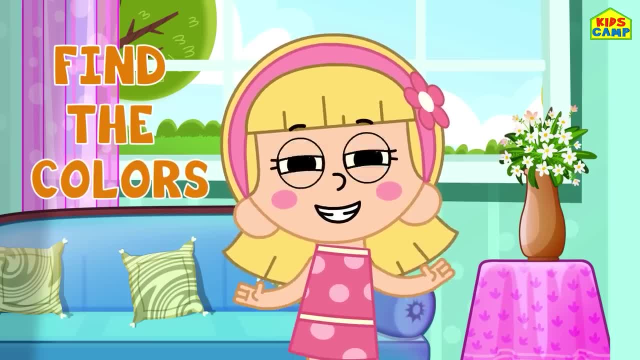 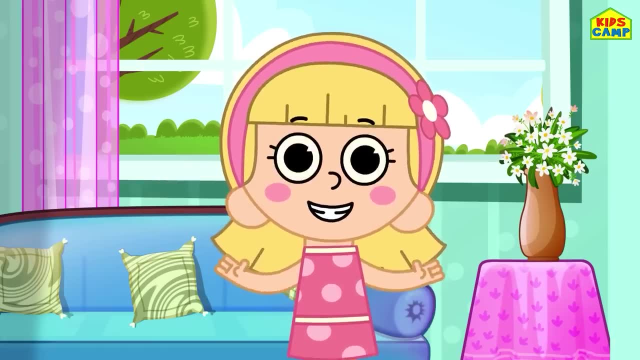 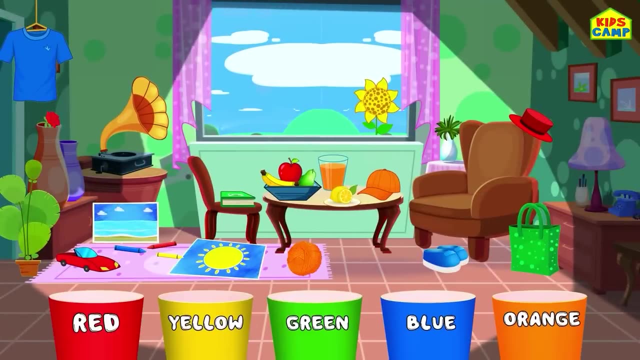 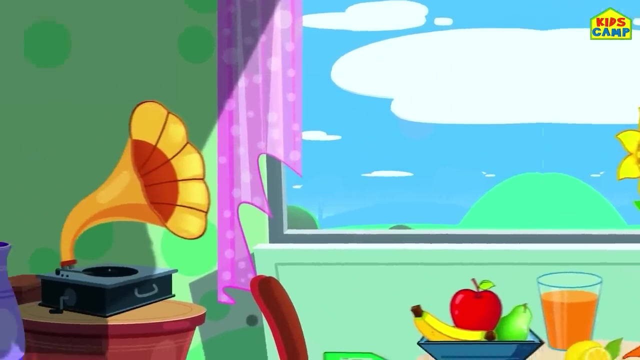 We have to find all the different types of colors, as mentioned on the buckets. The first color that we have to find is red. Can you spot everything red? Let's get started. Can you find anything red? Umm, that's right. 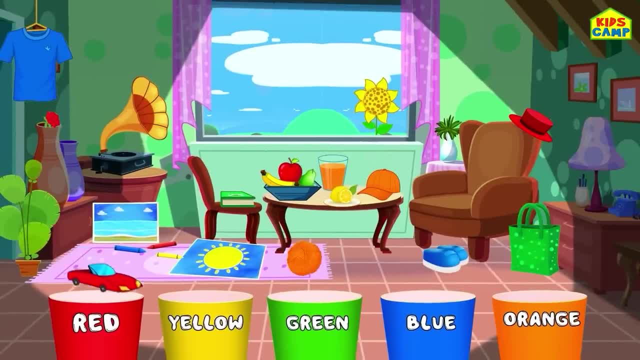 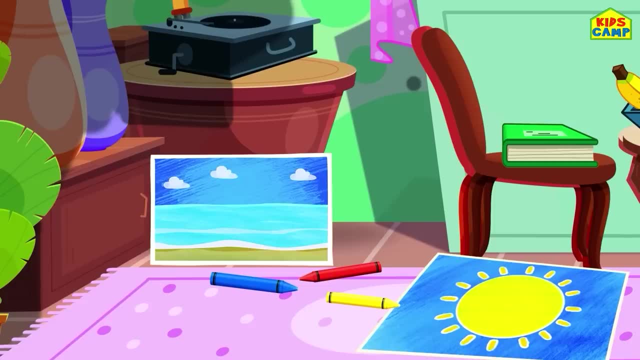 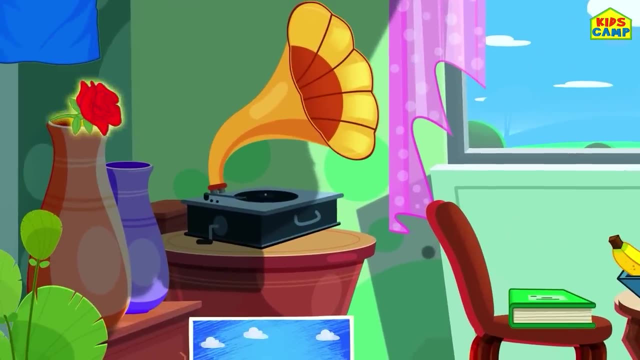 A toy car. Yes, it's red. Let's add it to the red bucket. What next? What else is red? Aha, I see a red crayon. That's right. Wow, A red rose. What else is red? 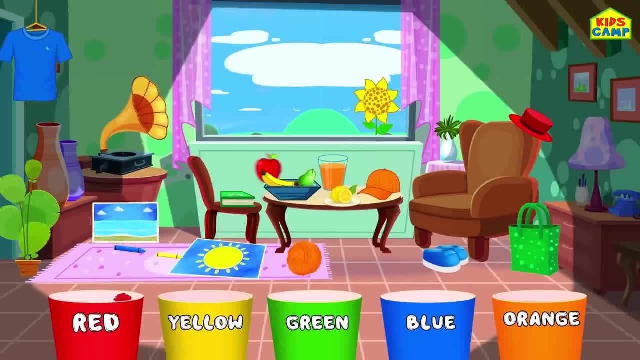 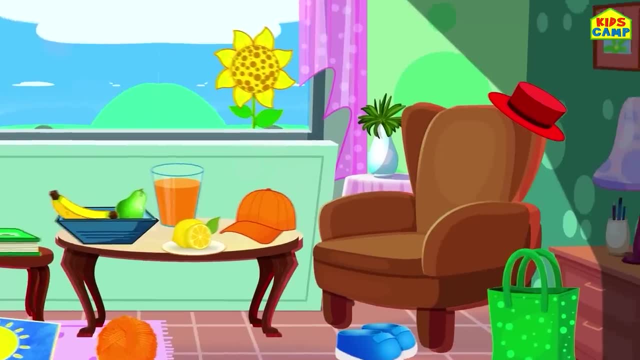 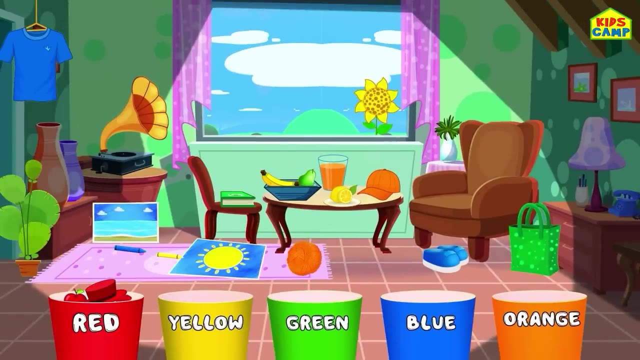 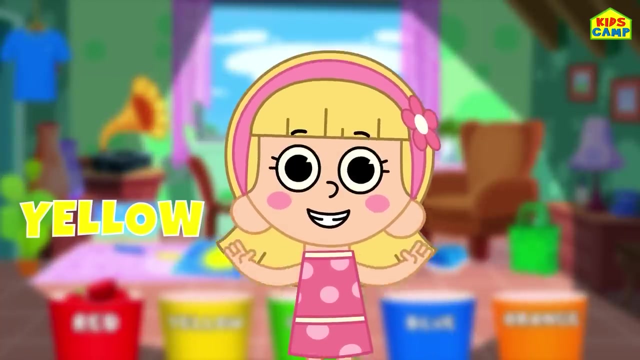 An apple. We'll add that to our red bucket. Keep looking for something else that's red. That's right, A red hat. Woohoo, We found everything that was red. What's the next color? Yellow, My favorite. 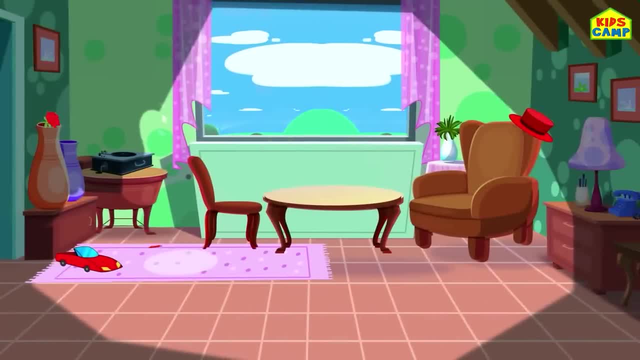 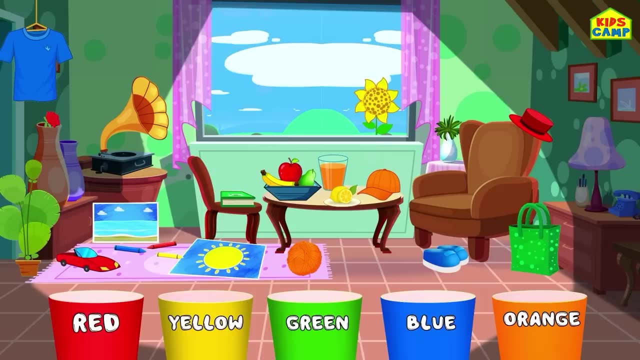 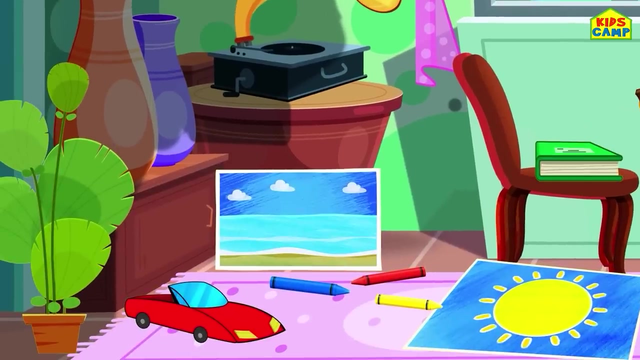 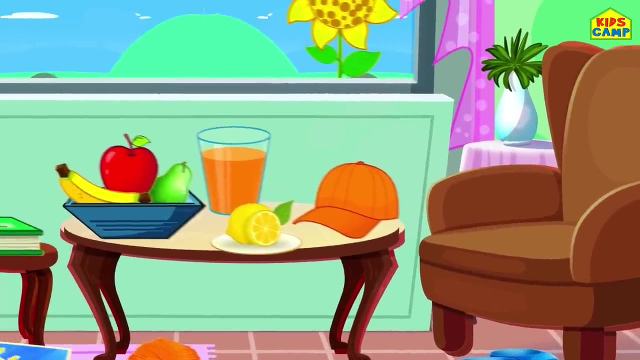 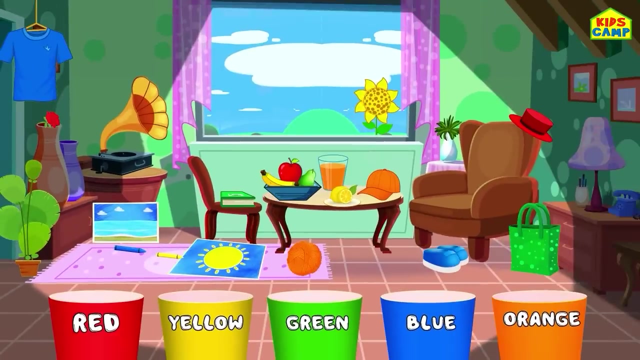 have to find is red. can you spot everything red? let's get started. can you find anything red? that's right, a toy car? yes, it's red. let's add it to the red bucket. what next? what else is red? uh-huh, I see a red crayon. that's right. Wow, a red rose. 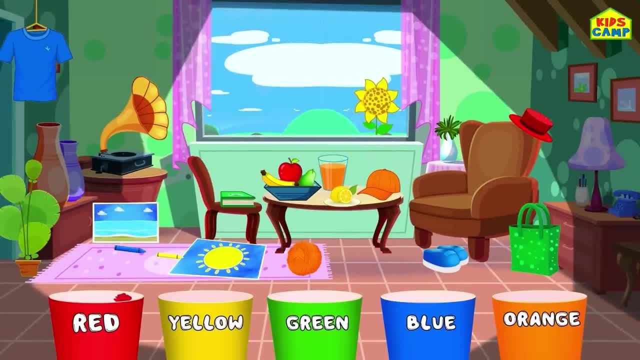 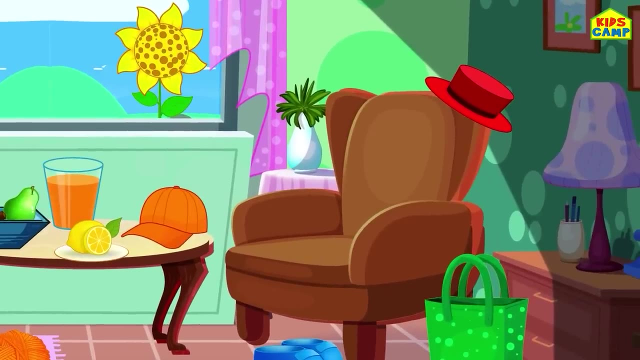 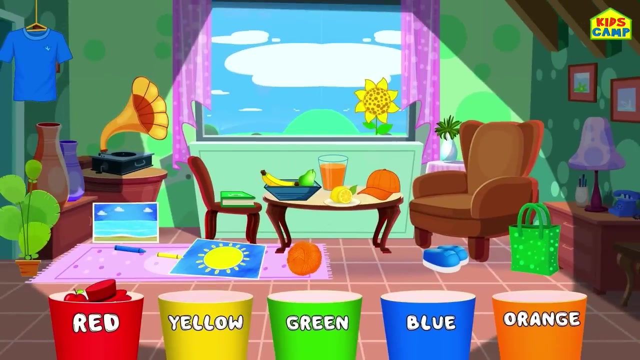 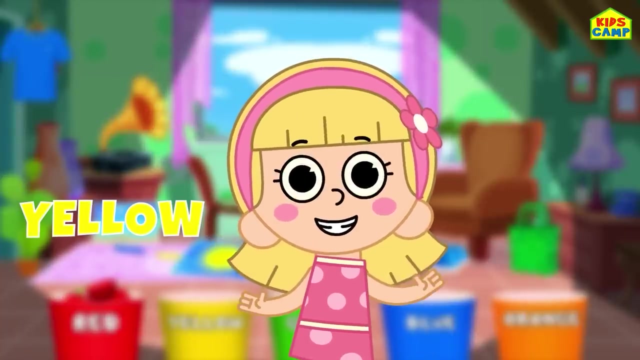 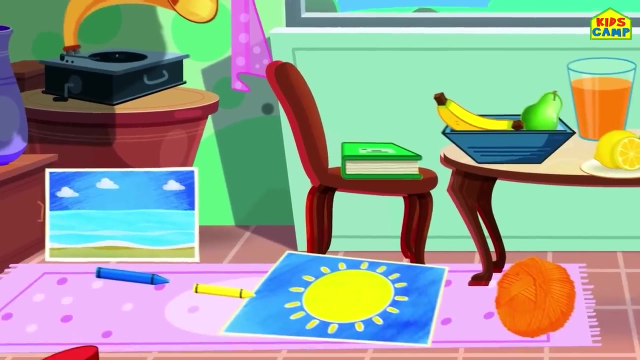 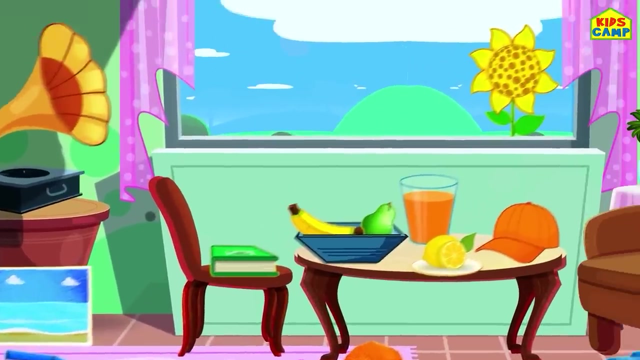 what else is red? an apple, we'll add that to our red bucket. keep looking for something else that's red. that's right, a red hat. we found everything that was red. what's the next color? yellow, my favorite. what do you see? that's yellow. uh-huh, my drawing of the Sun, the sunflower, that's. 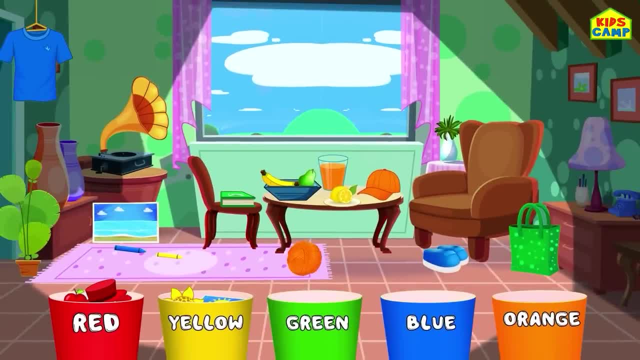 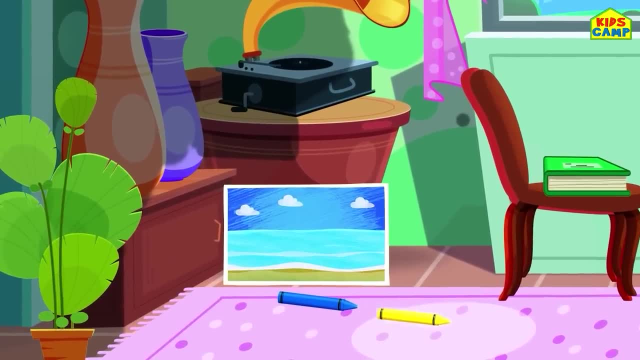 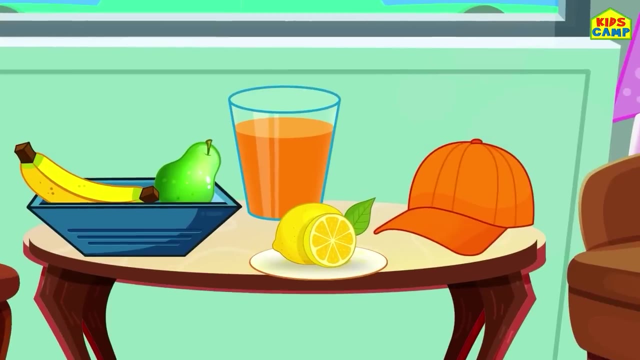 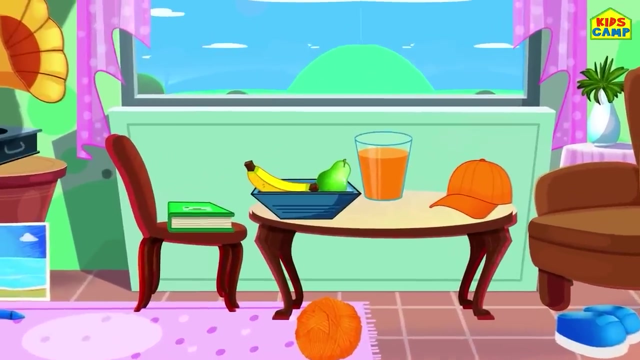 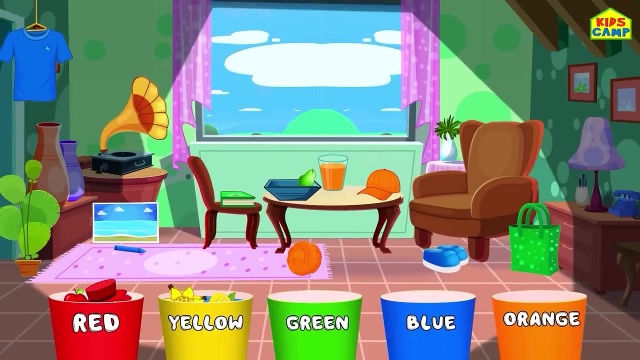 yellow too, into the bucket. good job, friends. what else is yellow? a yellow crayon, that's right. what else do you see? ah-ha, lemons, wonderful. what else? aha, a banana. the banana is yellow. into the yellow bucket, it goes. let's go to the next color, which is green. 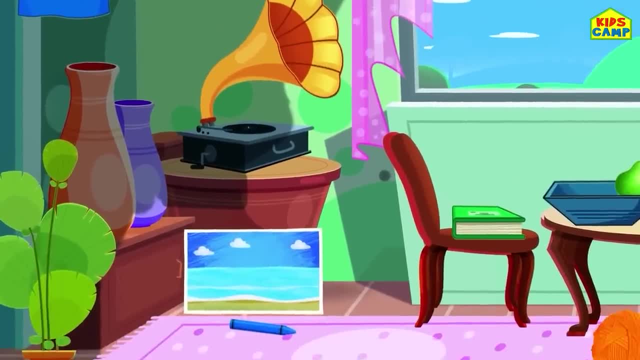 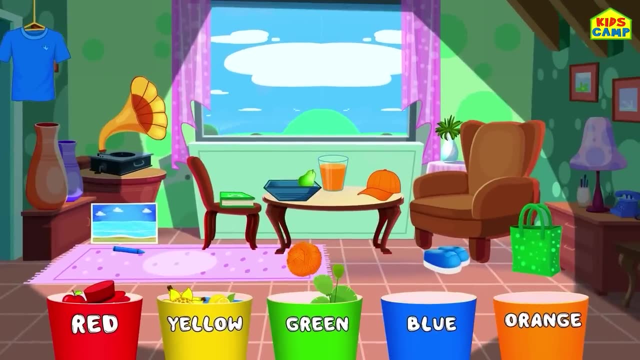 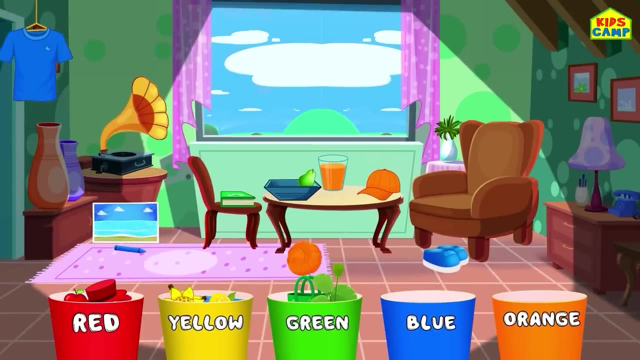 can you look for something that is green in my room? can you look for something that is green in my room? Uh-huh, I see it. the plant Into the bucket, it goes. What else is green? That's right, the green bag, Anything else. 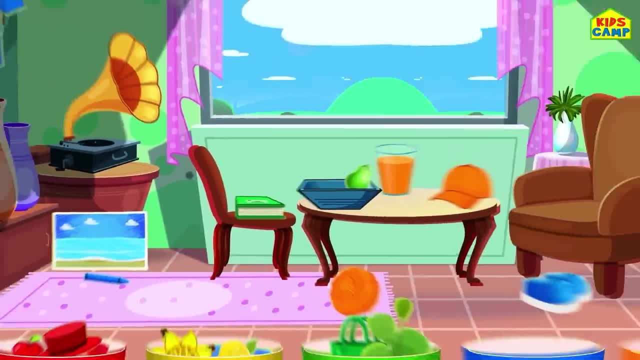 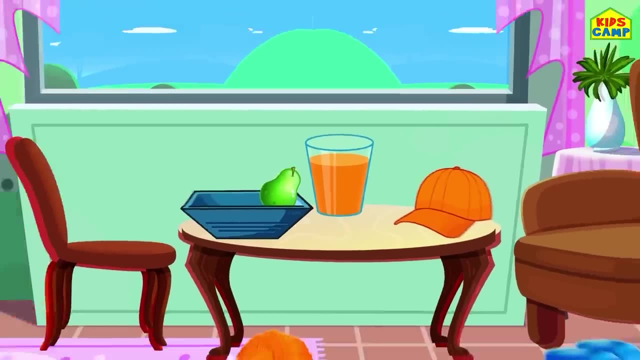 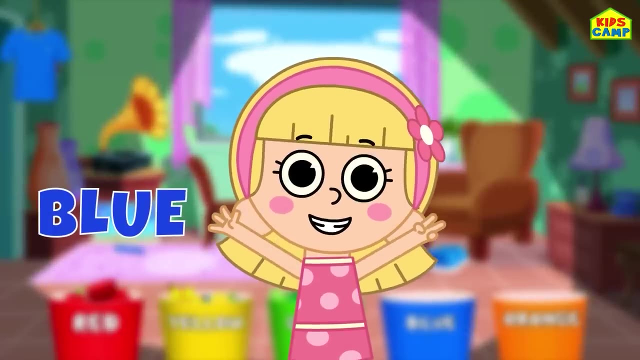 I see it too. the green book- Woo-hoo, What else? The pear, that's green too. Into the green bucket. Yay, Let's move on to the next color. It's blue. Woo-hoo, What's blue-colored here? 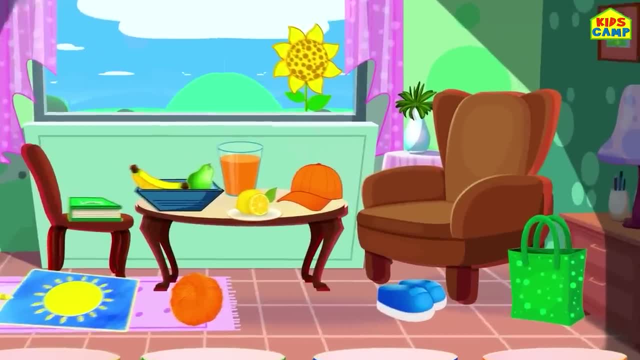 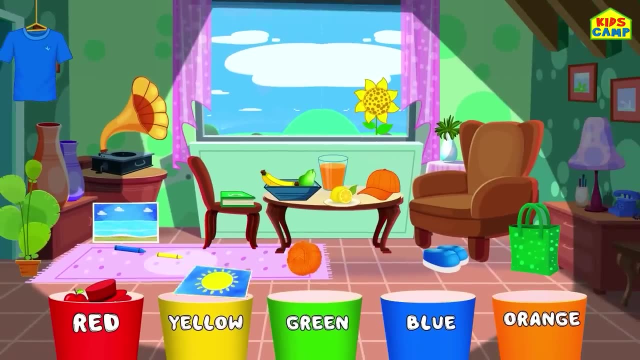 What do you see that's yellow? Aha, My drawing of the sun, My drawing of the sun, My drawing of the sun, The sunflower, The sunflower, That's yellow too. Into the bucket. Good job, friends. What else is yellow? 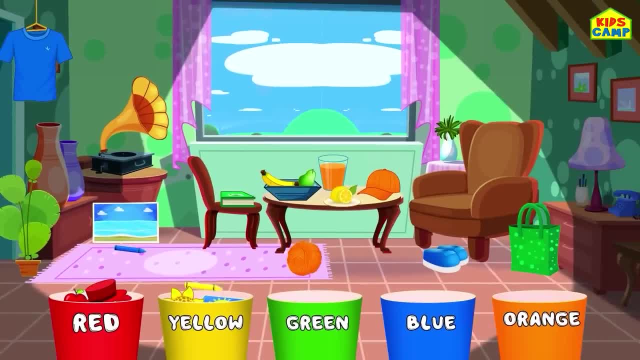 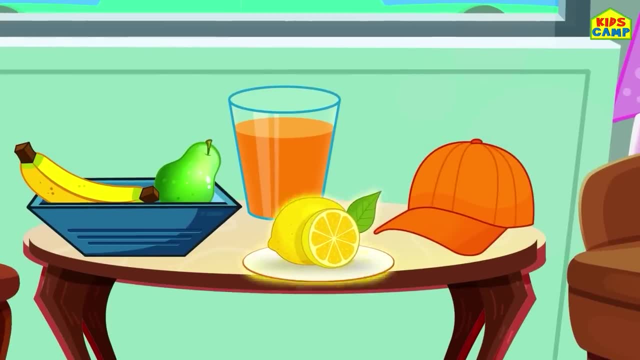 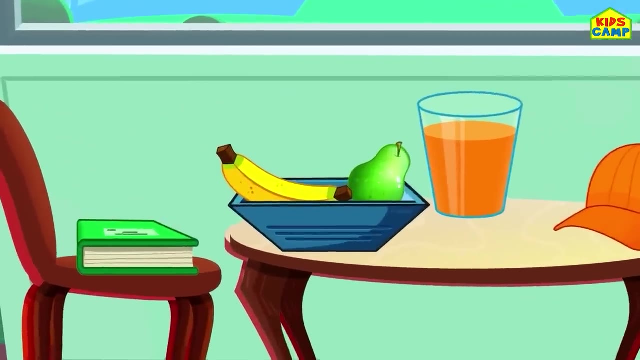 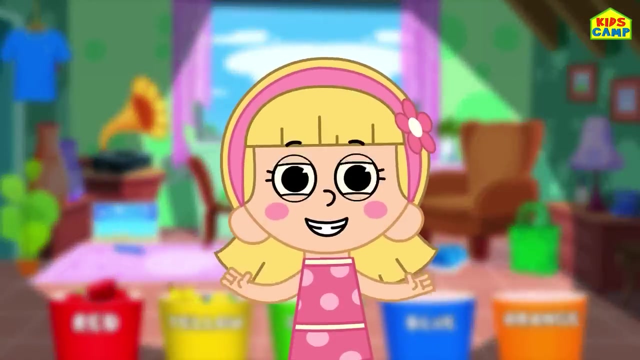 A yellow crayon, That's right. What else do you see? Aha, Lemons, Wonderful. What else? Aha, A banana. The banana is yellow. Into the yellow bucket it goes. Let's go to the next color. 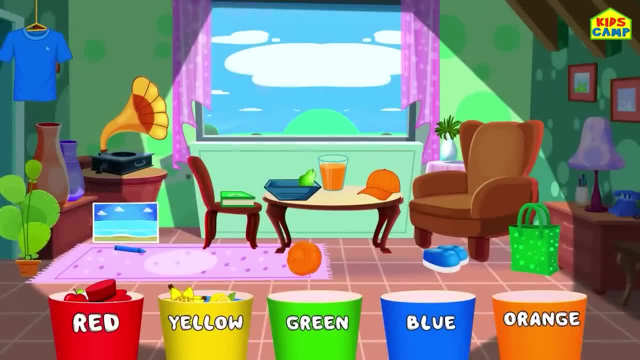 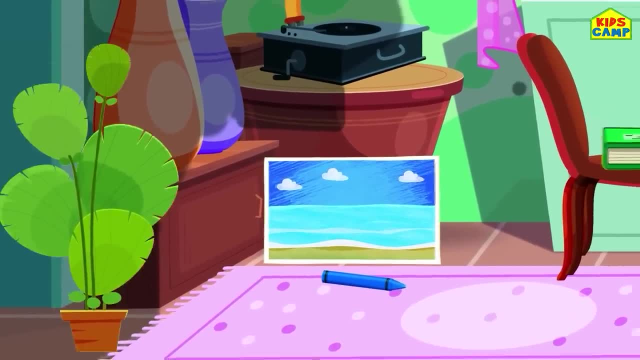 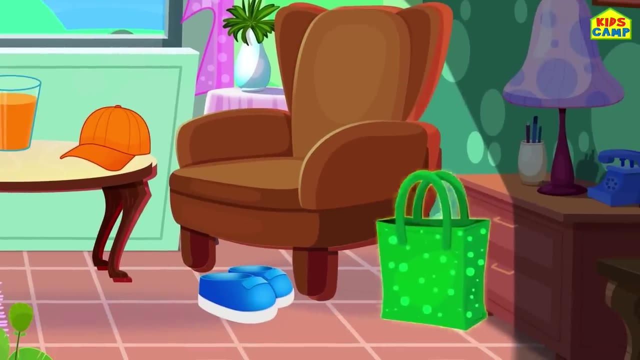 which is green. Can you look for something that is green in my room? Aha, I see it. The plant Into the bucket it goes. What else is green? That's right, The green bag. Anything else? I see it too. 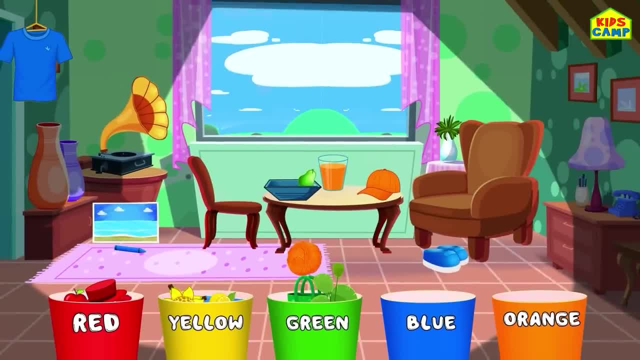 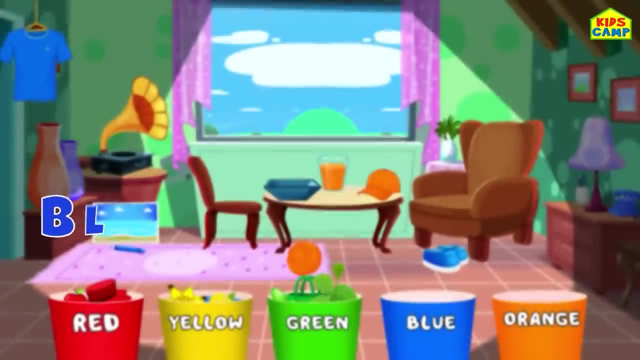 The green book. Woohoo, What else? The pear, That's green too- Into the green bucket. Yay, Let's move on to the next color. It's blue. Woohoo, What's blue colored here? The blue crayon. 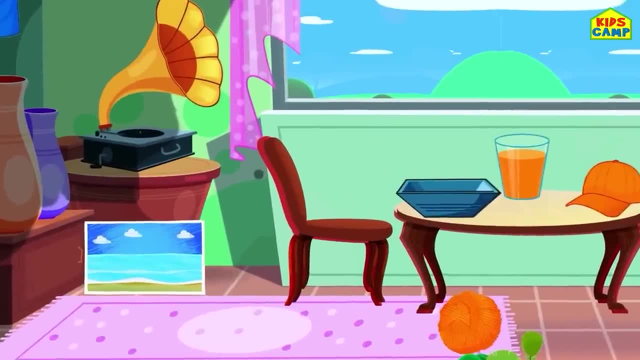 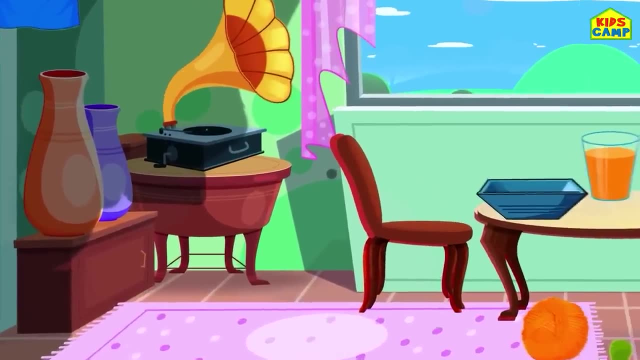 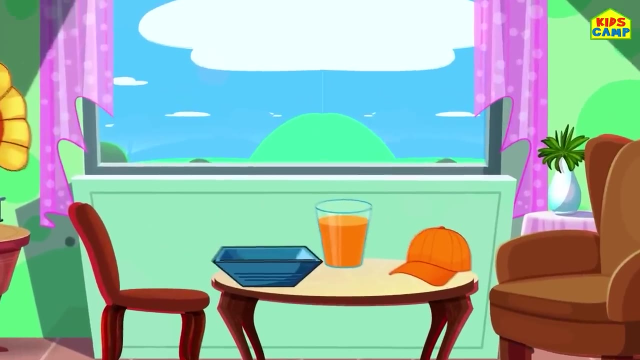 Anything else? My drawing of the blue sky? What else? The blue t-shirt Into the bucket? Aha, I see My pair of blue shoes. We found everything blue. What's next, It's orange, That's right. 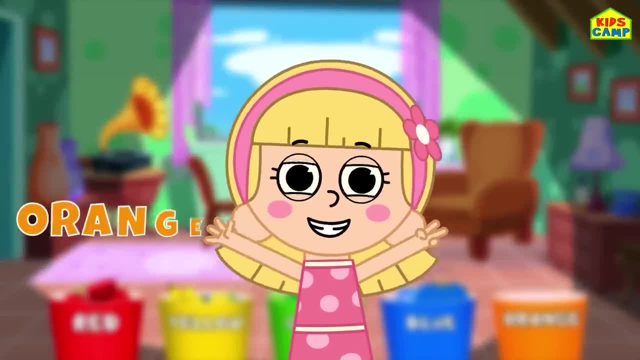 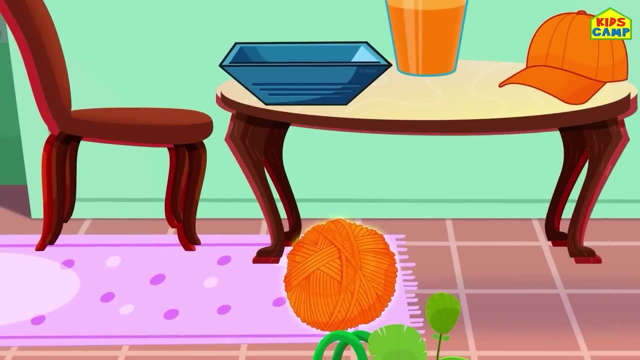 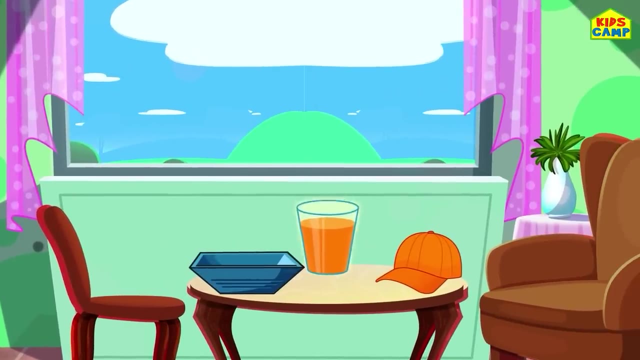 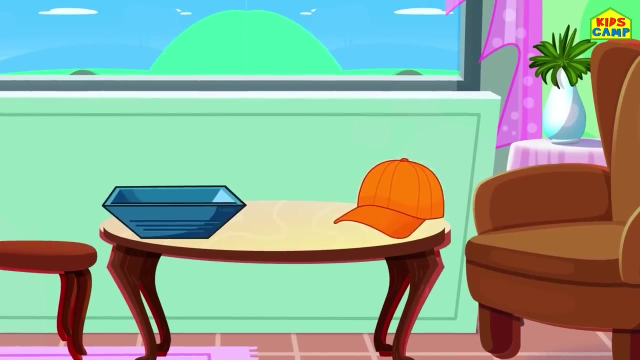 Can you spot something that is green? That's right. Can you spot something orange? An orange yarn of wool? That's right. What next? I see it: A glass of orange juice And An orange cap. Yay, Into the orange bucket, it goes. 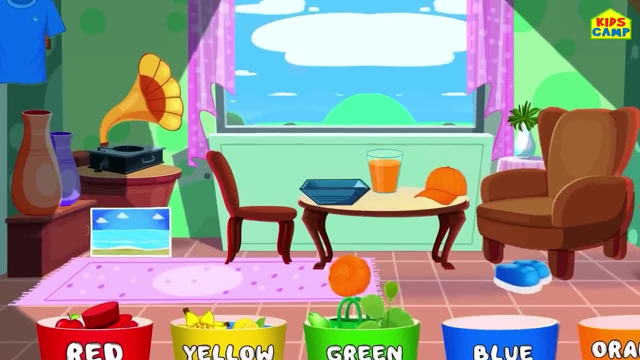 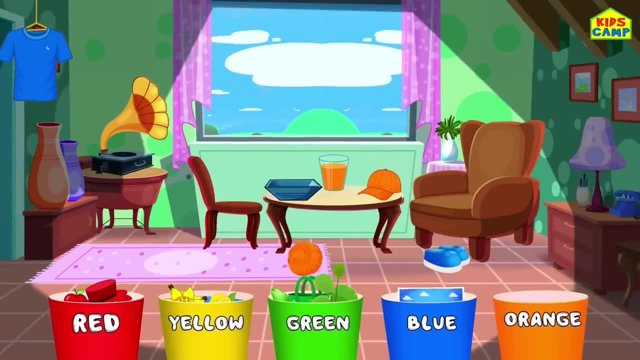 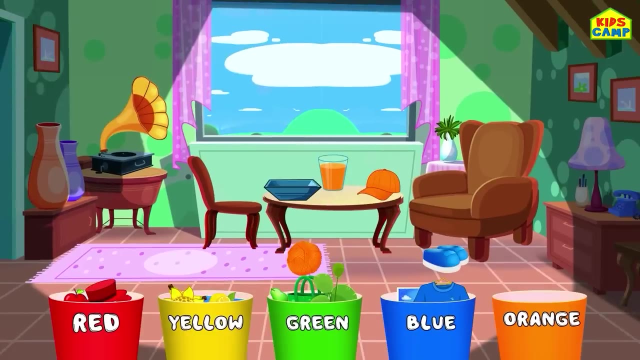 The blue crayon, Anything else? My drawing of the blue sky, What else? The blue T-shirt Into the bucket, What else? Uh-huh, I see my pair of blue shoes. We found everything blue. What's next? It's orange, That's right. 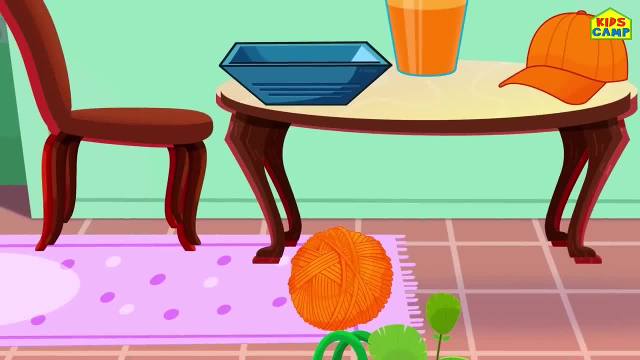 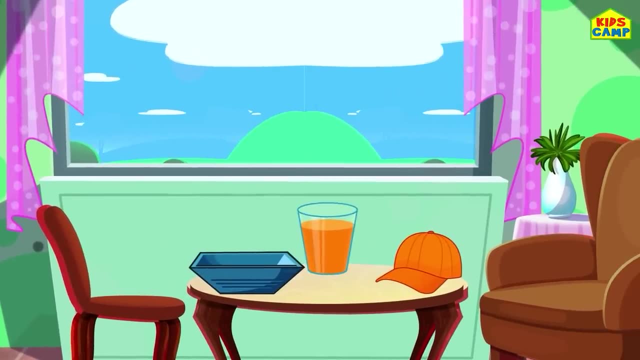 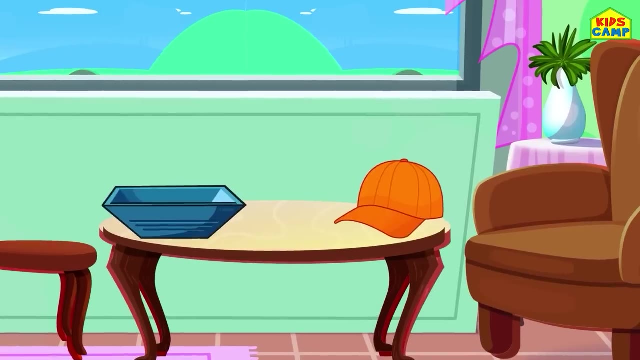 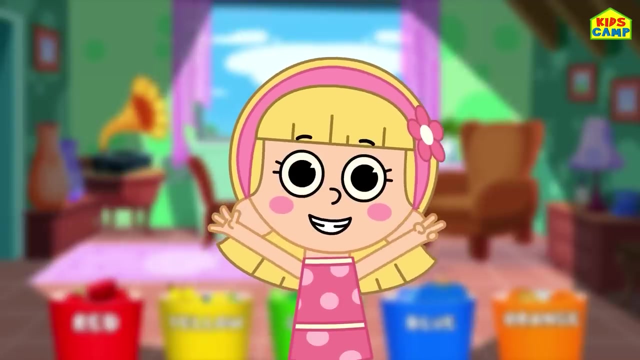 Can you spot something orange? An orange yarn of wool, That's right. What next? I see it: a glass of orange juice And An orange cap. Yay Into the orange bucket. it goes. Wonderful kids, we found all the colors. Bye. 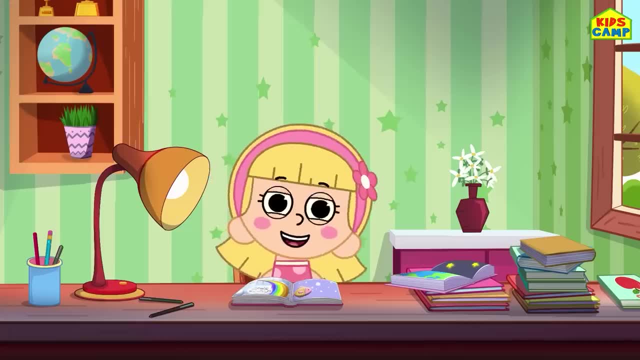 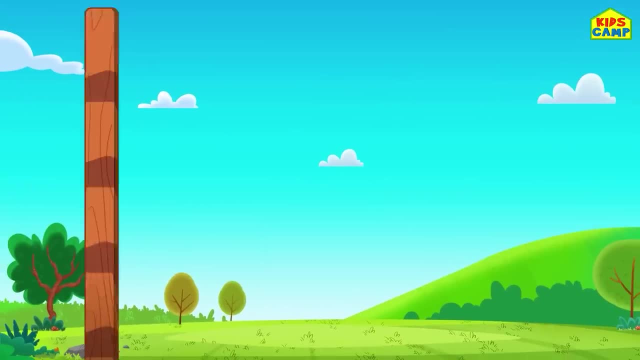 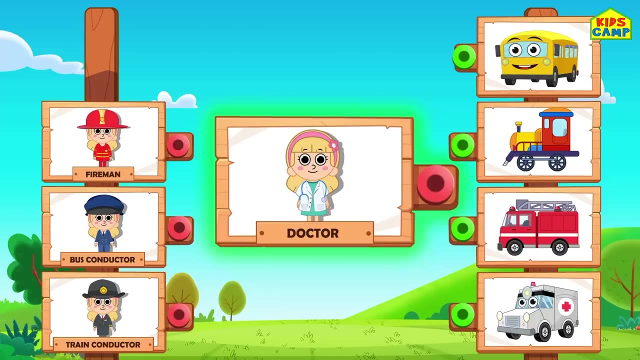 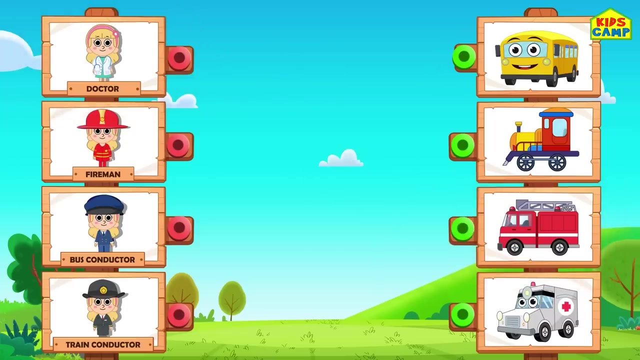 Bye, Hi friends, I'm Ellie. Let's play a fun game where we match the pairs. Let's match the professions to their vehicles. What vehicle will a doctor use? A fire truck, No. A train, No, No. Hmm, I know. 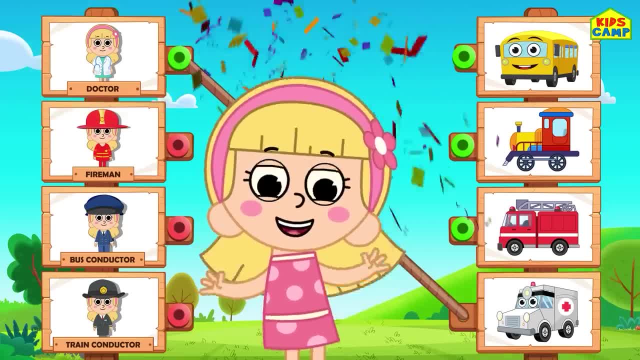 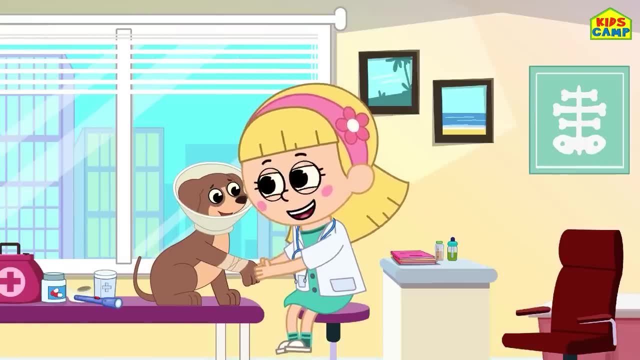 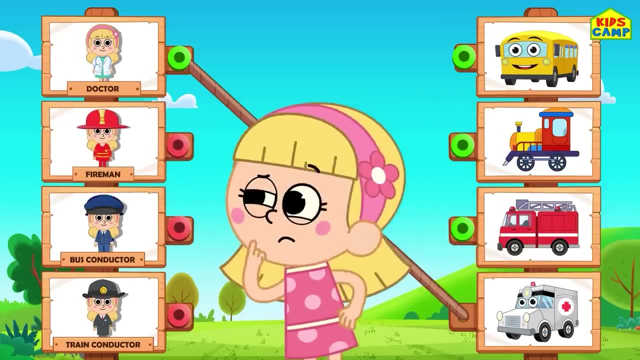 The doctor will use an ambulance. That's right, Yay. A firefighter will use A firefighter will use A firefighter. will use Which vehicle? Hmm, a bus. No, no, A fire truck. That's right, Yay. 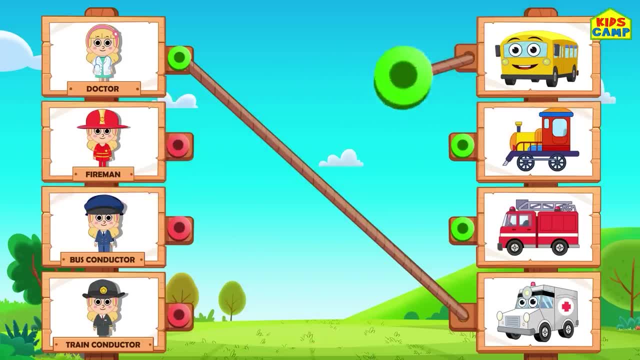 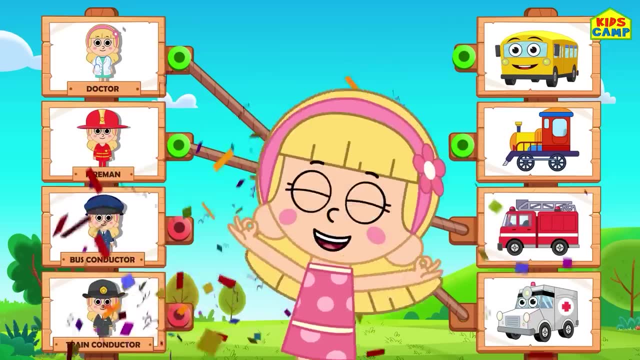 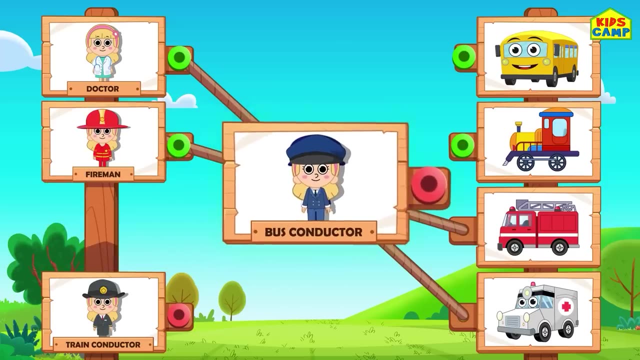 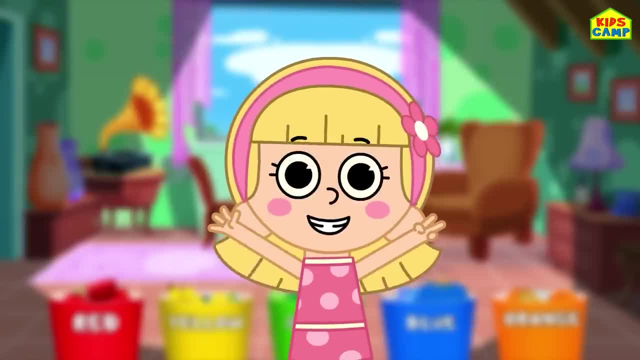 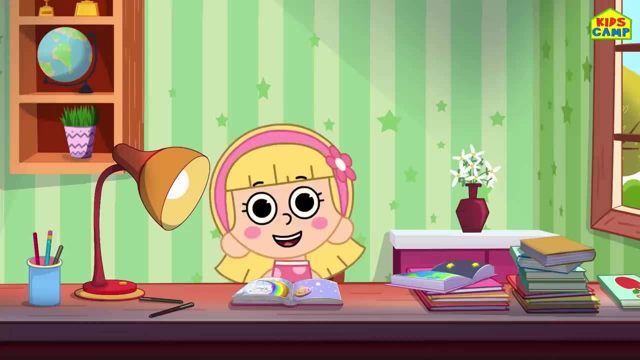 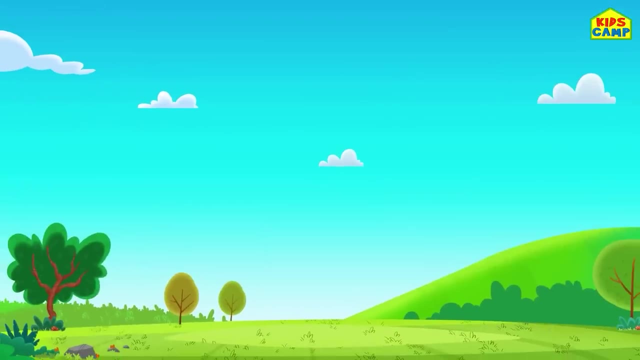 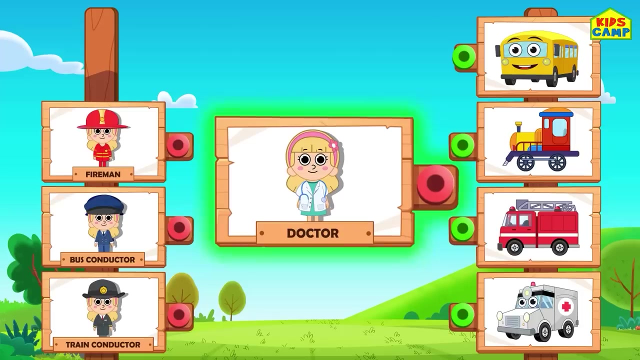 Wonderful kids. We found all the colors. Bye, Hi friends, I'm Ellie. Let's play a fun game where we match the pairs. Let's match the professions to their vehicles. What vehicle will a doctor use? A fire truck, No. 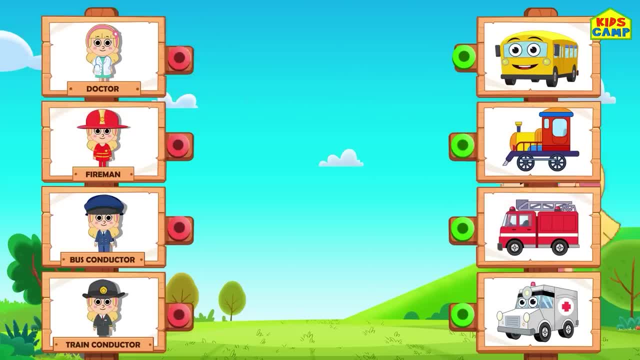 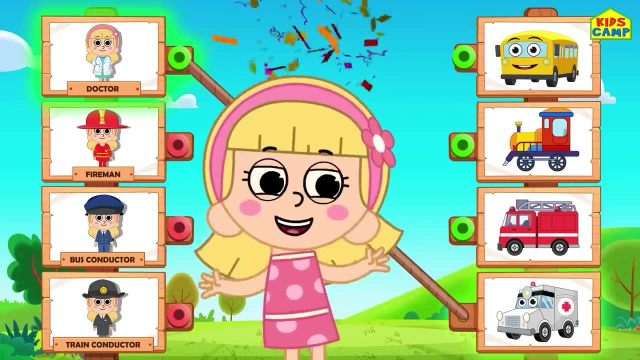 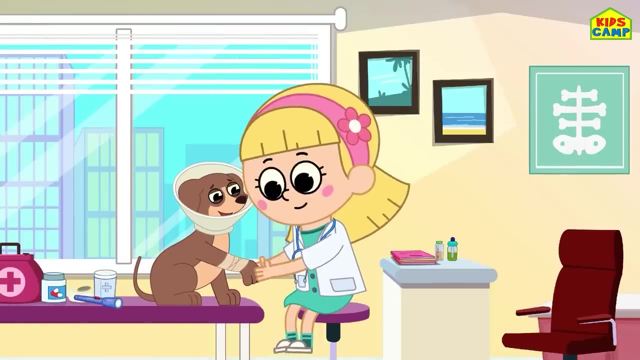 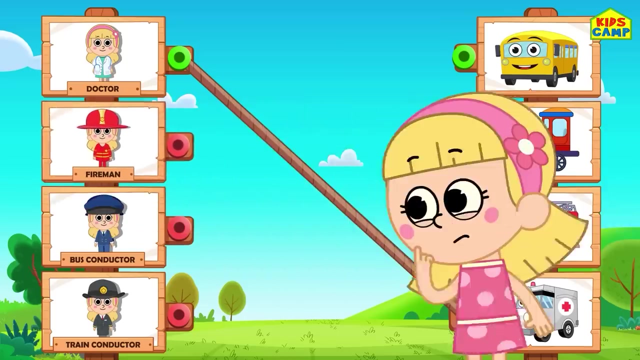 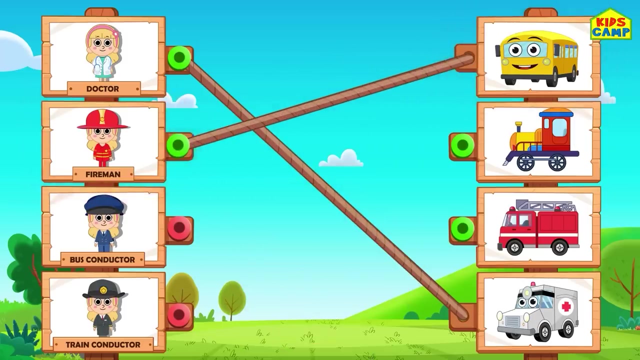 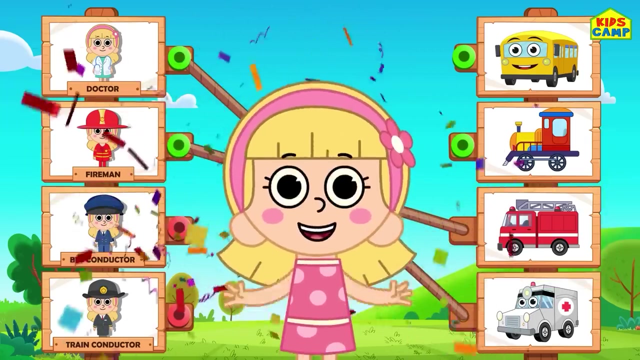 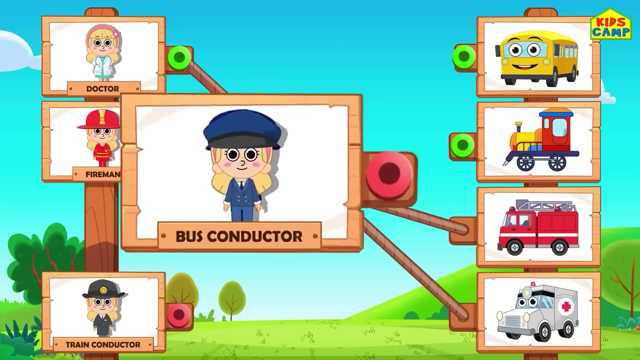 A train? No, Hmm, I know The doctor will use an ambulance. That's right, Yay. A firefighter will use Which vehicle? Hmm, A bus. No, A fire truck, That's right, Yay, A bus driver. 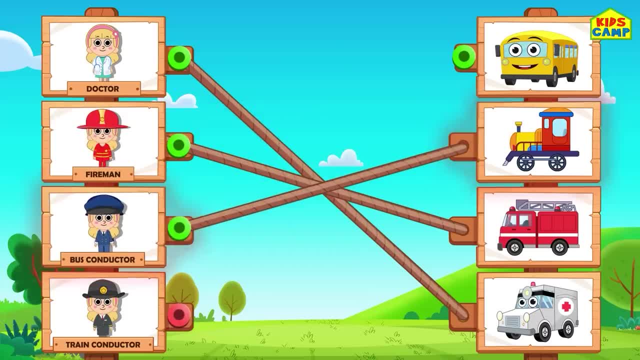 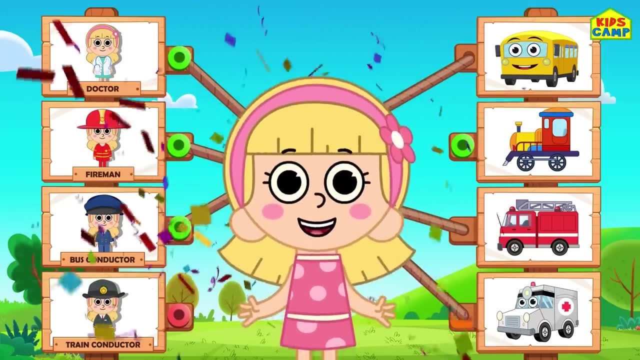 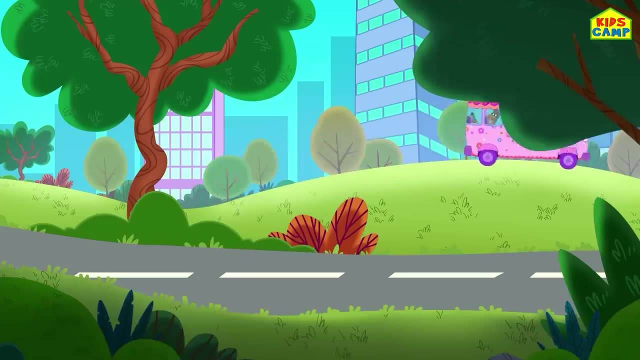 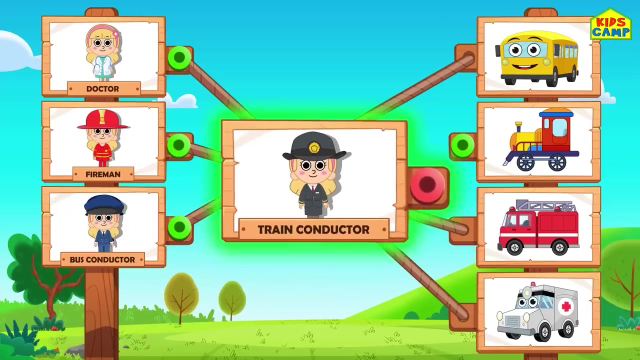 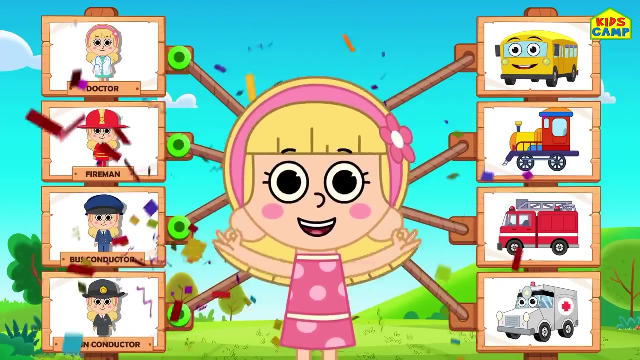 will use A train, No A bus. That's right. Good job, friends. Yay. What's next A train conductor? What's next A train conductor? Which vehicle will he use? The train, That's right. 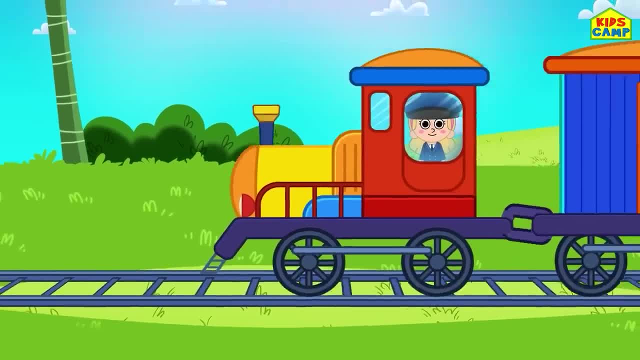 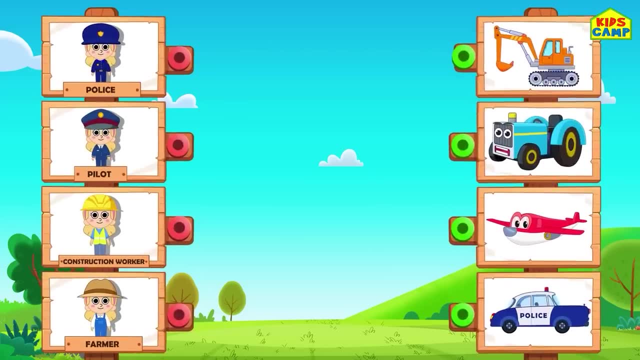 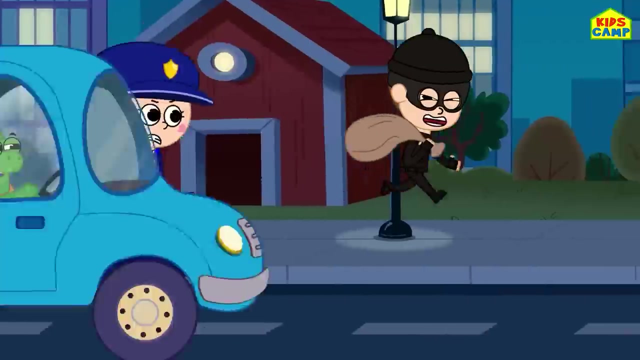 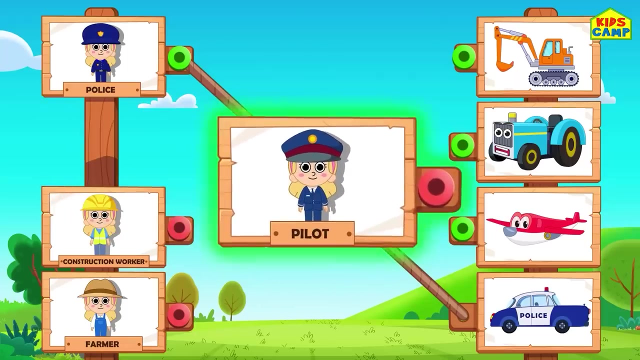 All aboard. Ooh, What will the police use? An airplane? No. A tractor? No way. Hmm, I know A police car, That's right, Yay, A pilot will use Which vehicle? Hmm, A digger. 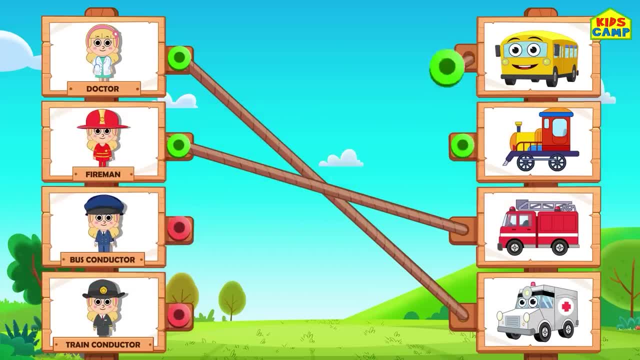 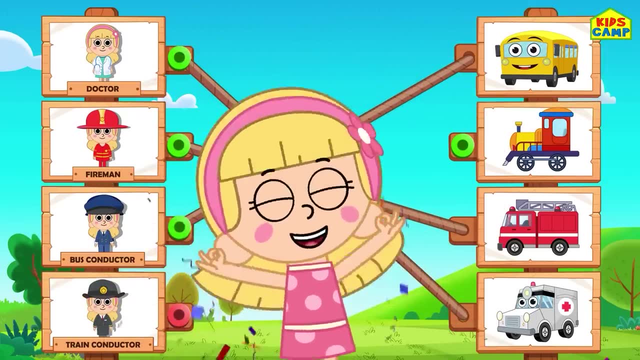 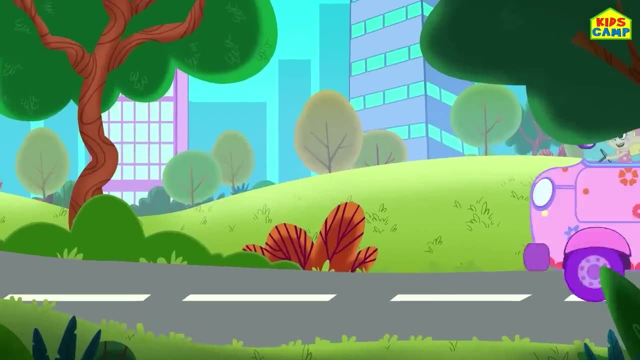 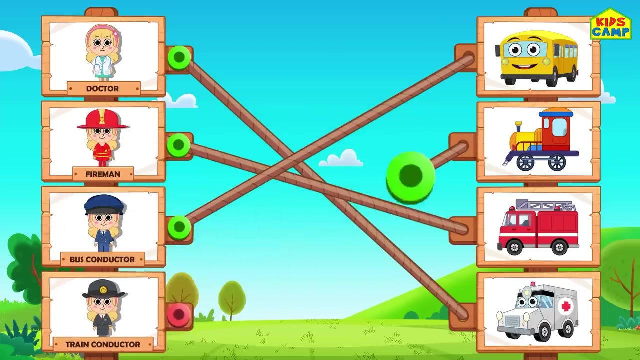 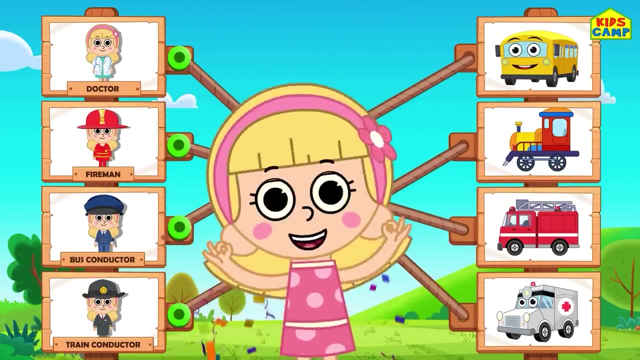 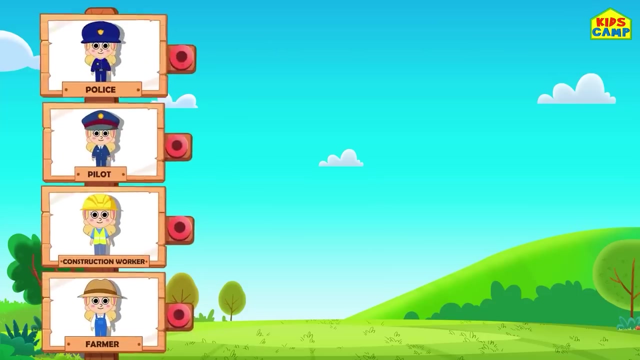 No, No, No. A bus, A bus, That's right. Good job, friends. Yay. What's next A train conductor? Which vehicle will he use? The train, That's right, All aboard. Ooh, Which vehicle will the police use? 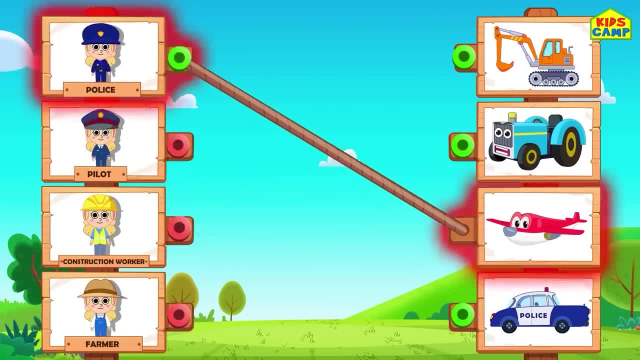 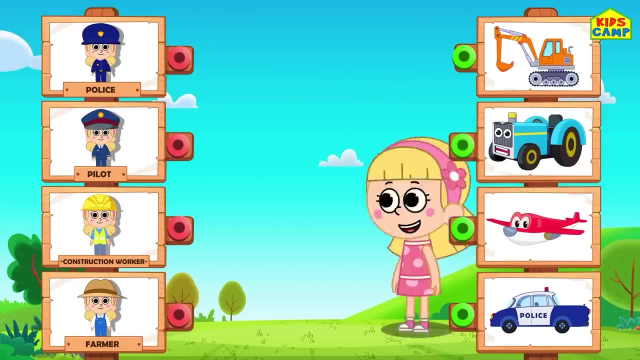 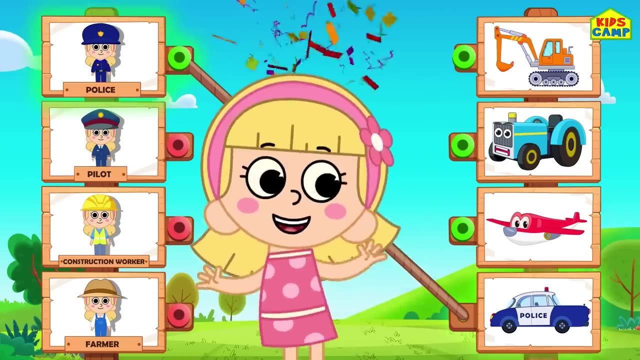 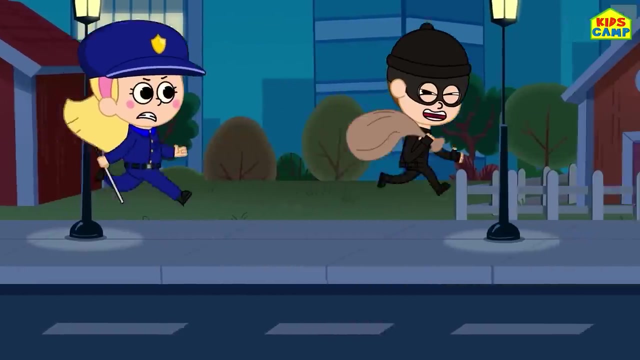 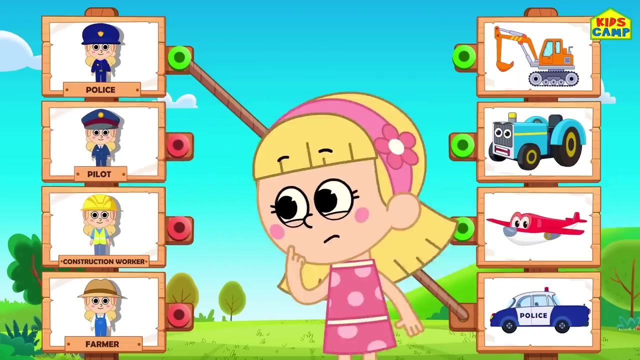 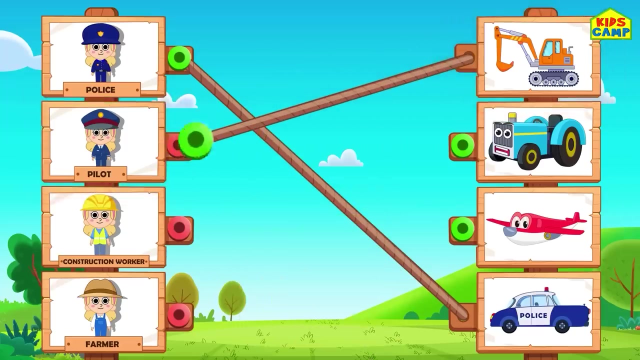 An airplane: No. A tractor: No way. Hmm, I know A police car, That's right, Yay, Yay. A pilot will use Which vehicle? Hmm, A digger: No. An airplane: Yes. 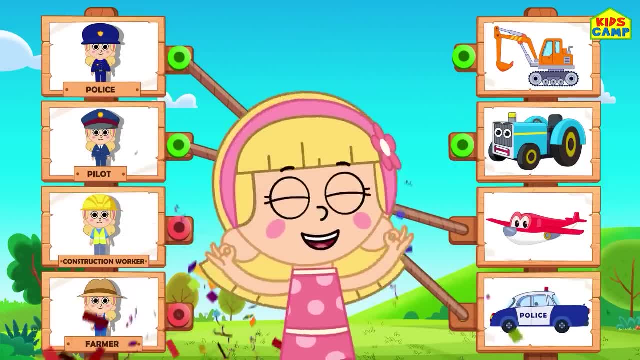 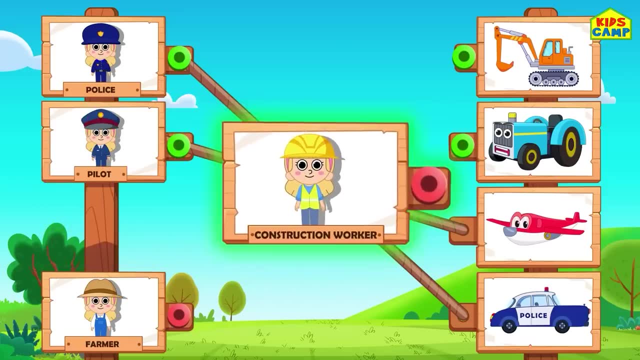 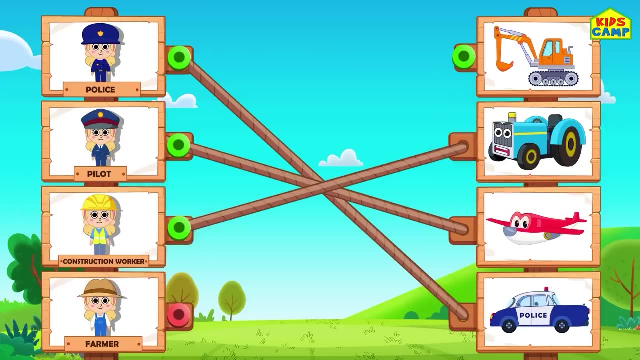 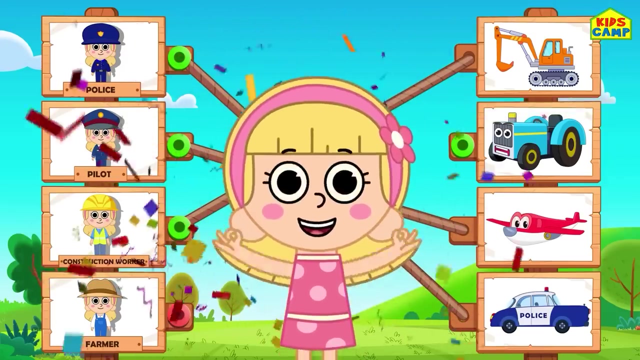 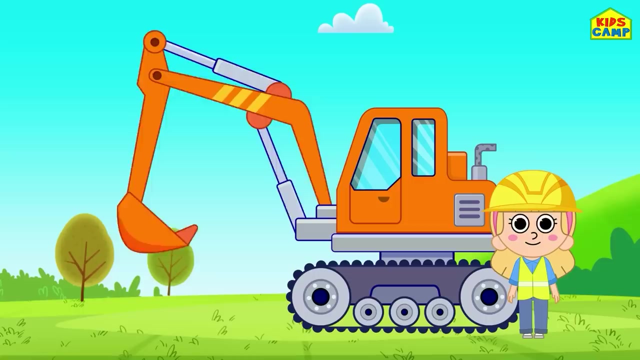 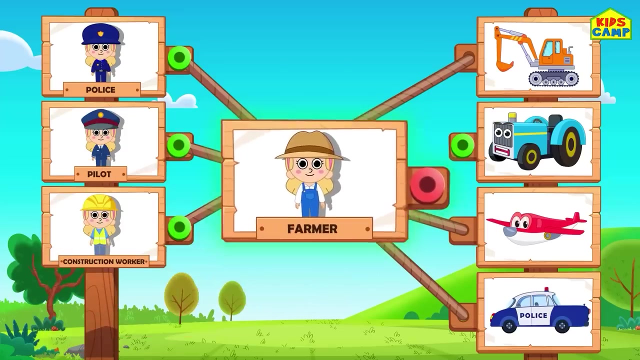 Fly away, Yay. A construction worker will use which vehicle? A tractor. No, A digger, That's right. Yay, Yay, Yay, Yay. What vehicle will a farmer use? A tractor, That's right. 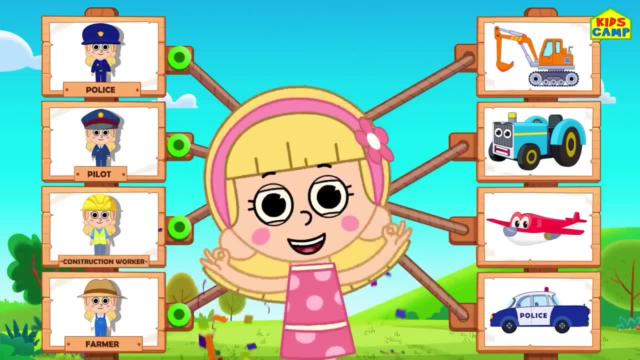 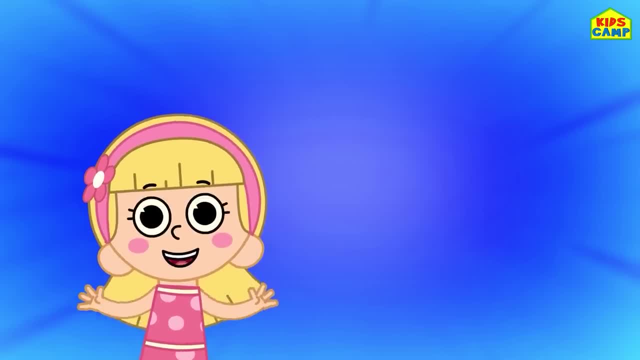 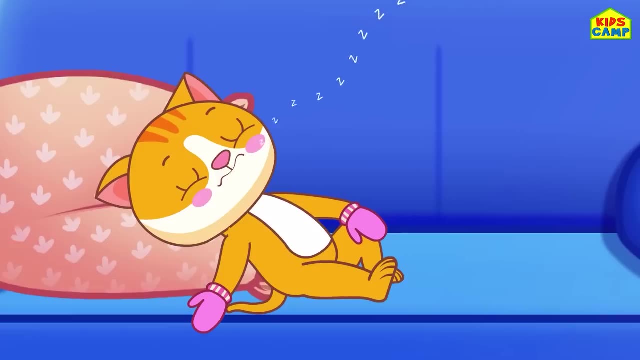 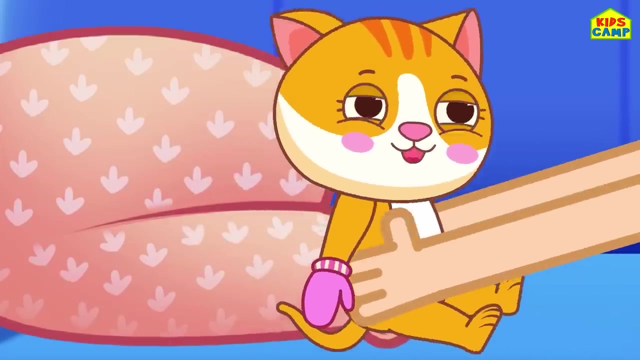 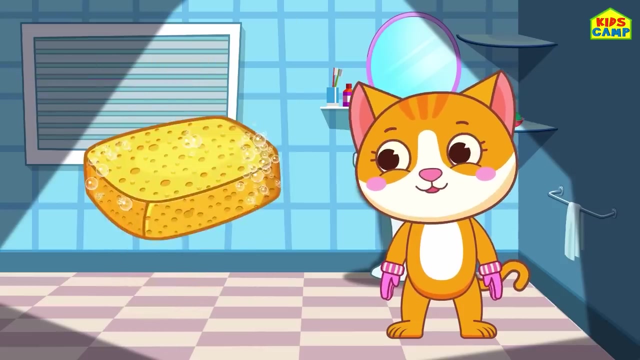 Yay, Superb, That was so much fun. Keep watching Kids' Camp. Bye, Good morning Kitty. Wake up, Let's brush your teeth Ready. What do we brush your teeth with? Is this a toothbrush? No, 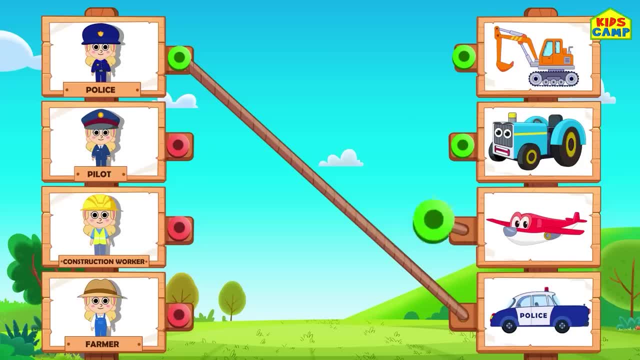 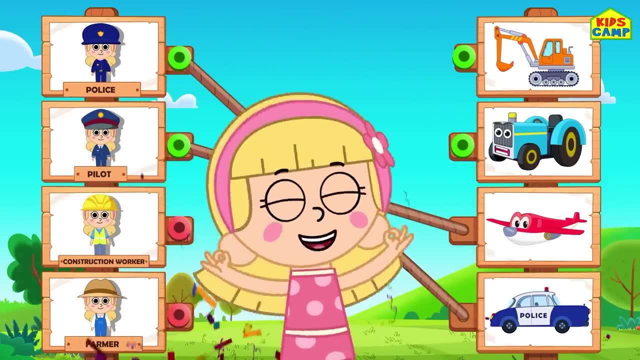 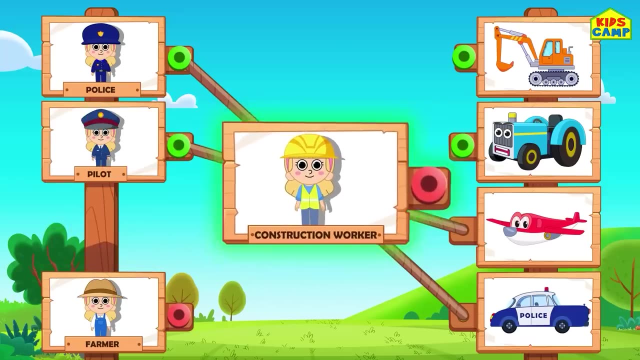 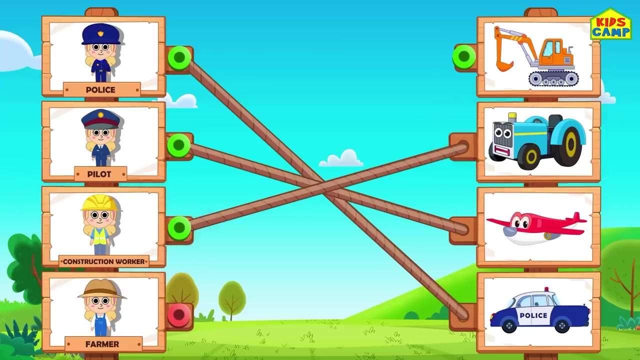 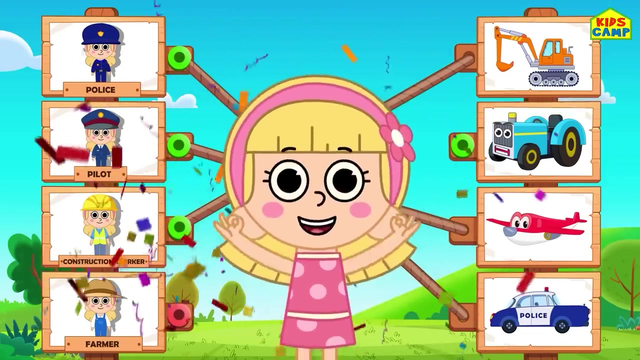 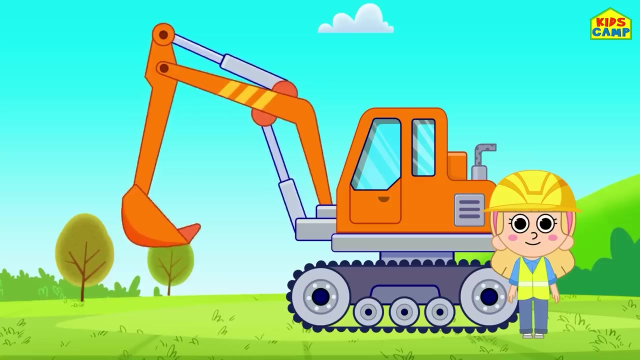 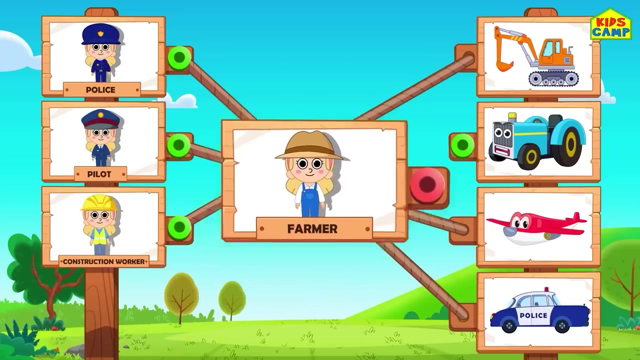 No, An airplane. Yes, Fly away. Yay. A construction worker will use which vehicle? A tractor. No, A digger, That's right, Yay. What vehicle will a farmer use? A tractor, That's right. 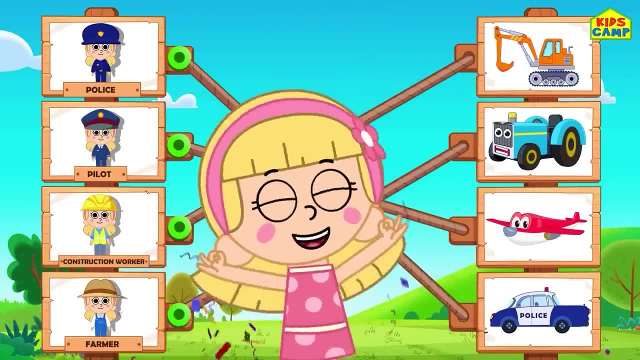 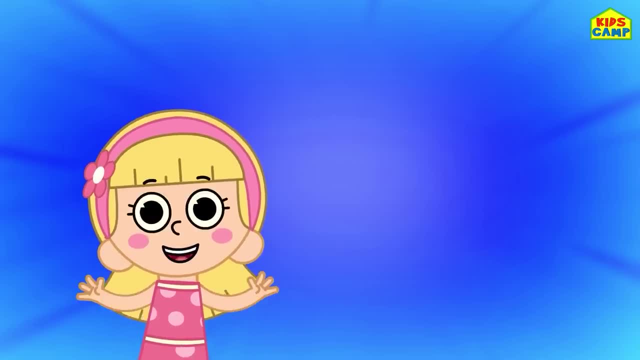 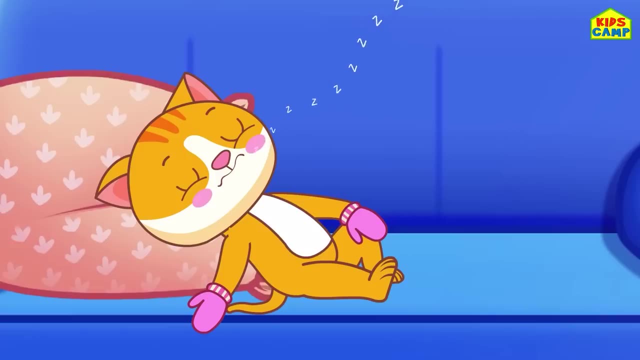 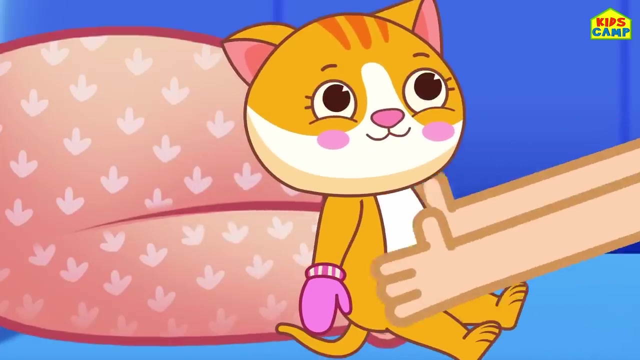 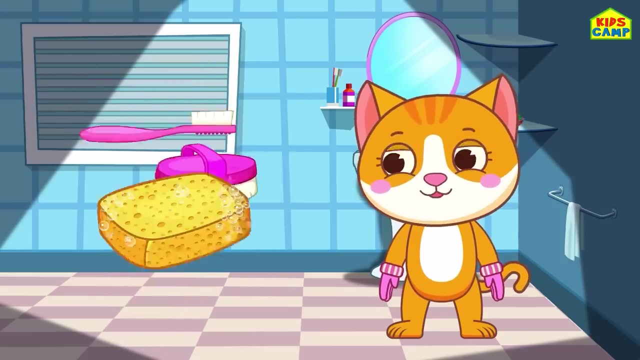 Yay, Superb, That was so much fun. Keep watching Kids' Camp. Bye, Good morning Kitty. Wake up, Let's brush your teeth Ready. What do we brush? What do we brush our teeth with? Is this a toothbrush? 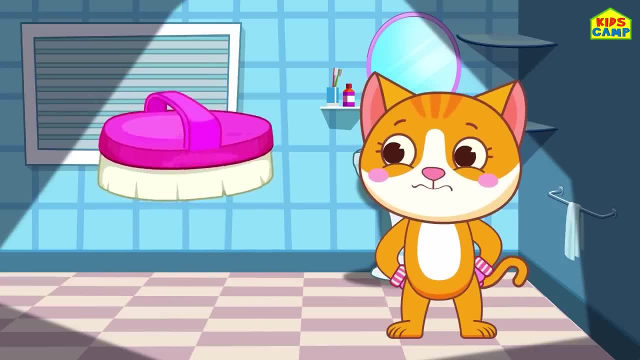 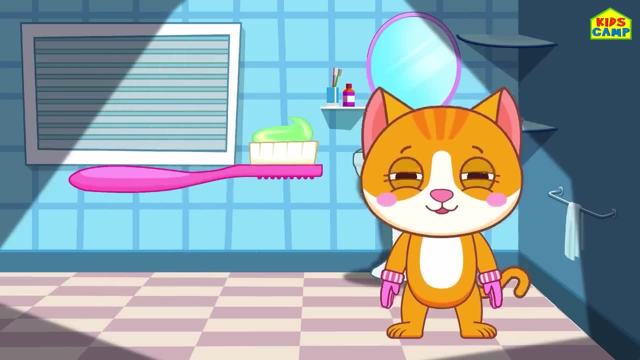 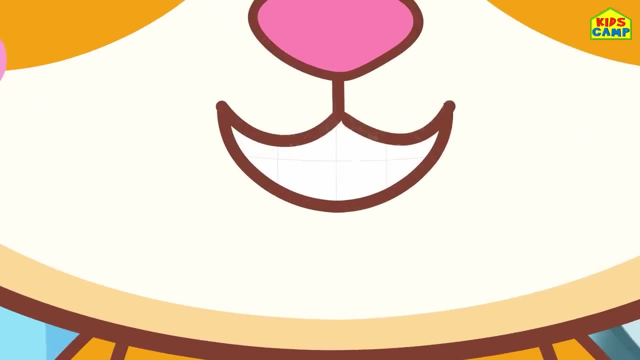 No. Is this a toothbrush? No, no, Is this a toothbrush? Yes, it is, Yay. Wow, Your teeth are sparkling white. Now let's have a bath. What do we have a bath with This one? 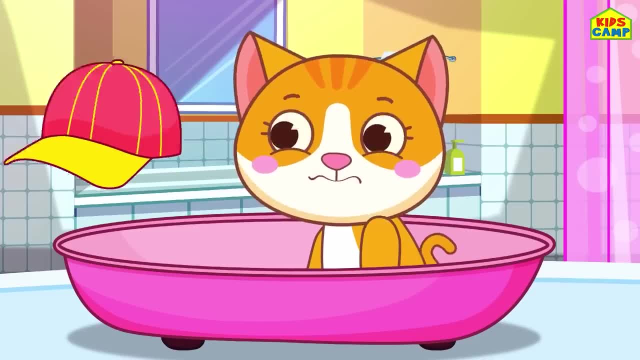 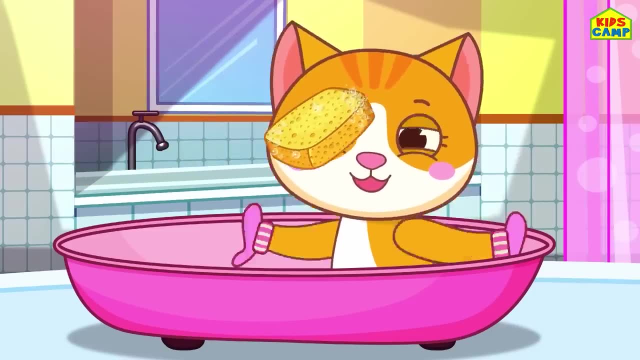 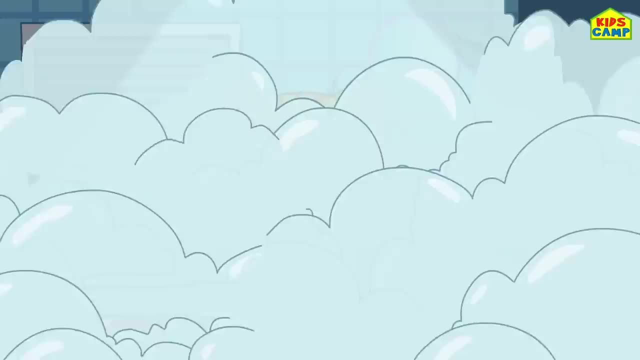 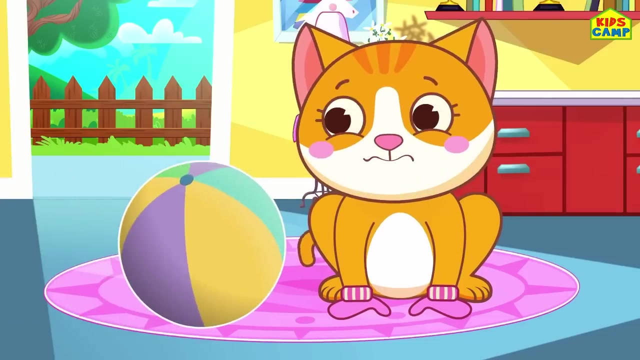 No, This one, Definitely not This one. Yes, Yay, Don't you love taking a bath? Wow, You are neat and clean, Kitty. Now let's have breakfast. What do we have for breakfast? This one, No. 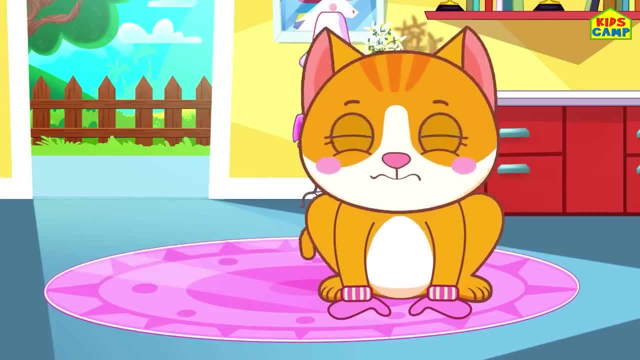 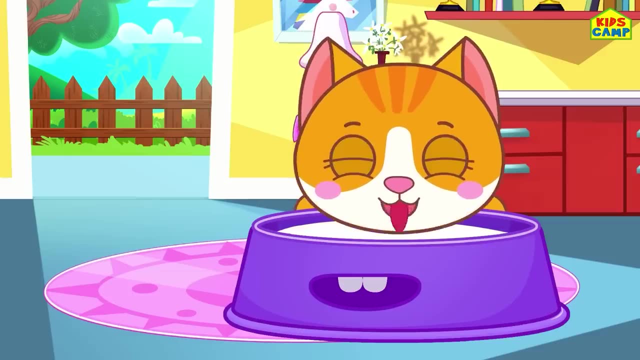 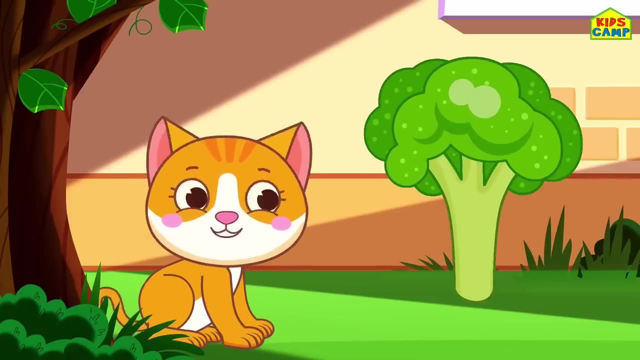 This one? No, Then let's have milk. Yes, Milk is good. Don't you love drinking milk? Now let's play. What do we play with This? No, It's a broccoli. No, we can't play with this, It's a candy. 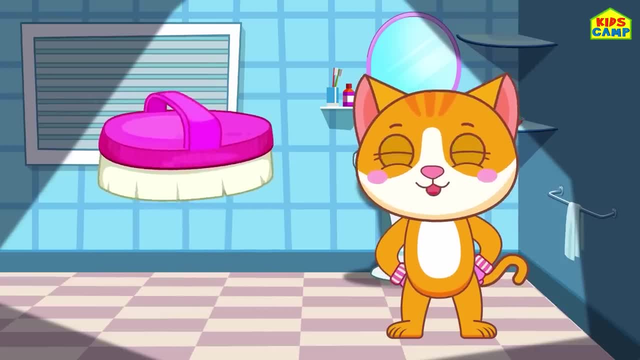 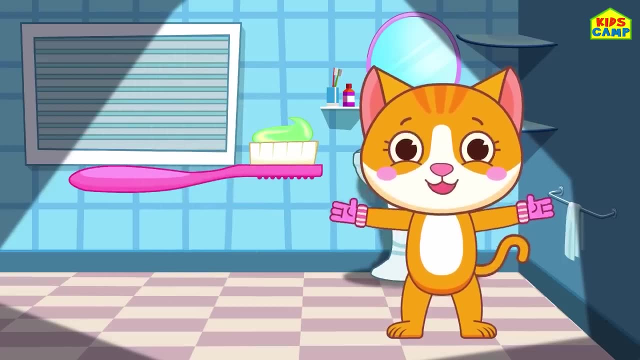 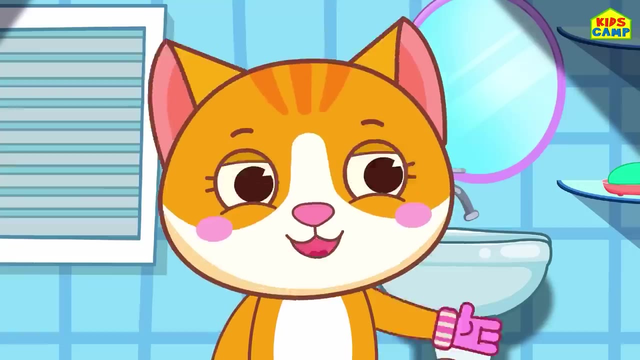 Is this a toothbrush? No, no, Is this a toothbrush? Yes, it is, Yay, Yay, Wow, Your teeth are sparkling white. Now let's have a bath. What do we have a bath with This one? 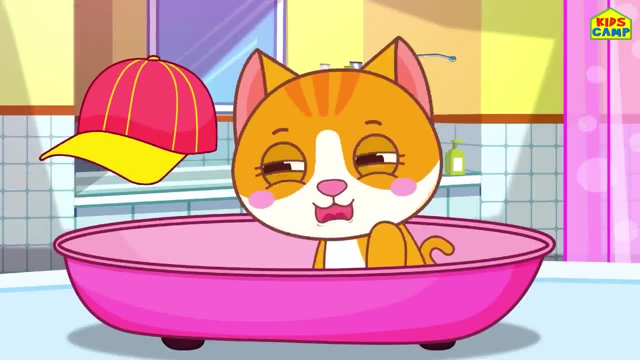 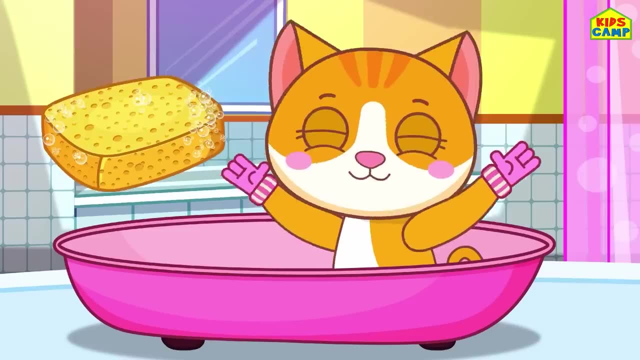 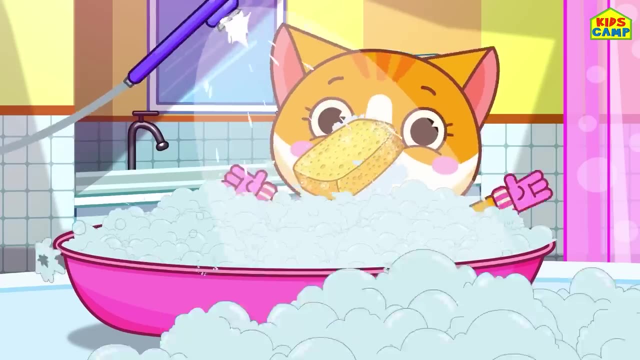 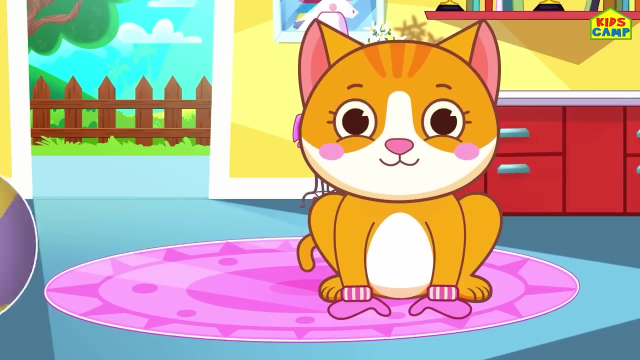 No, This one, Definitely not This one. Yes, Yay, Don't you love taking a bath? Wow, You're neat and clean, Kitty. Wow, You're neat and clean, Kitty. Now let's have breakfast. What do we have for breakfast? 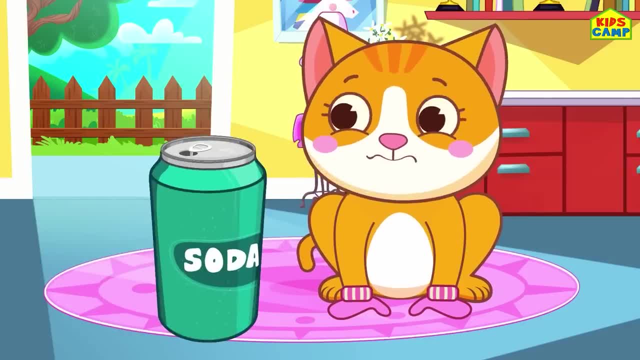 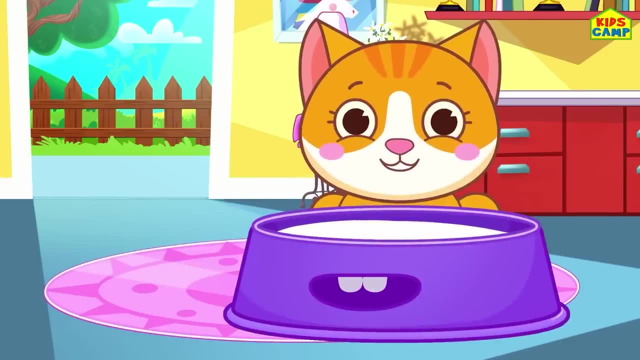 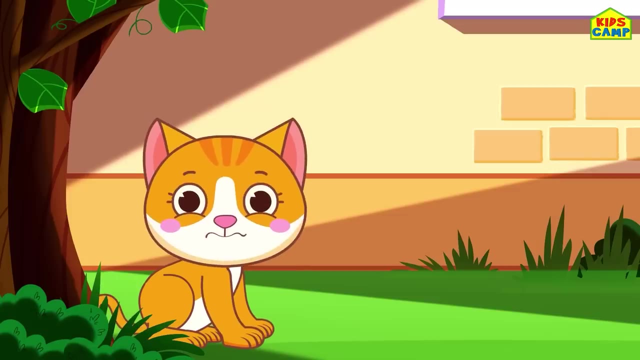 This one, No. This one, No, no. Then let's have milk. Yes, Milk is good. Don't you love drinking milk? Now let's play. What do we play with This? No, it's a broccoli. 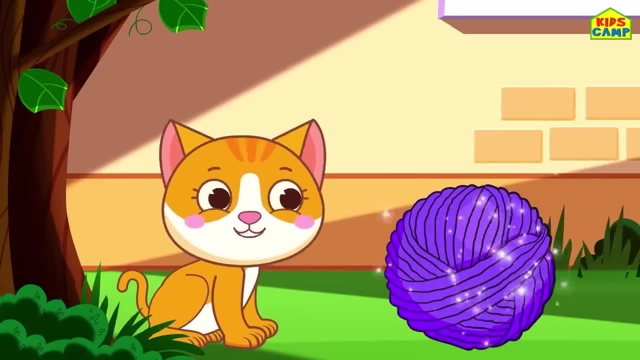 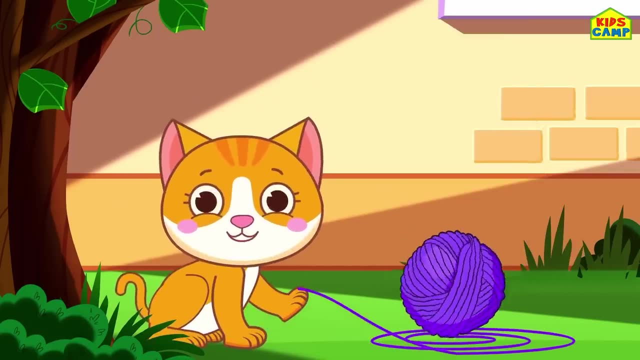 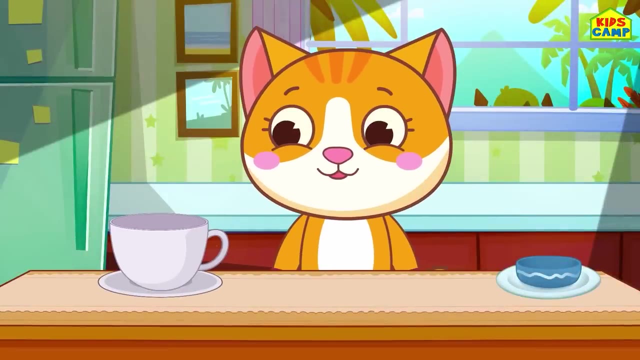 No, it's a candy. Yes, we can play with this. It's a ball of string. Wow, So much fun. Now let's eat something. Are you hungry? Can you eat this? No, Can you eat this? No, no. 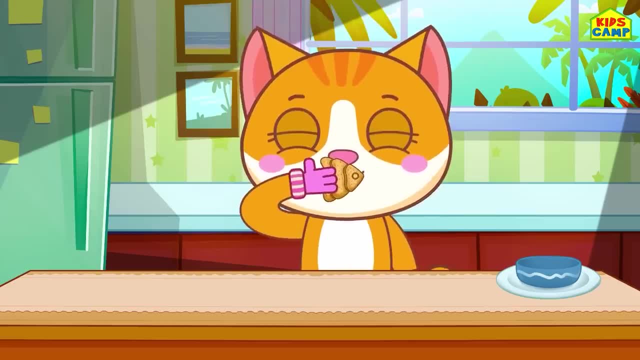 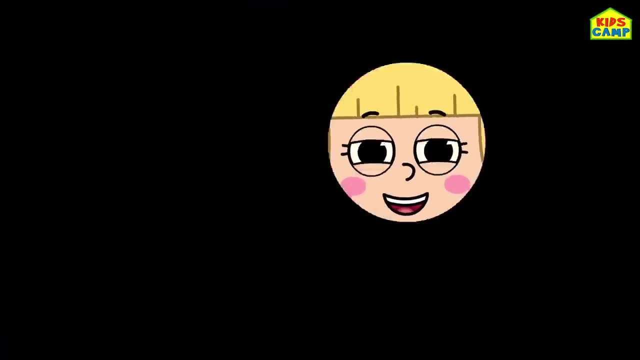 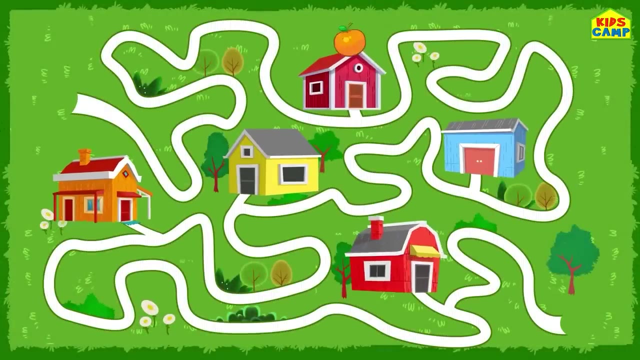 Yes, you can eat this. Don't you love the fish biscuit? Yummy. Wasn't it a fun day with my kitten. See you soon. Bye, Hi, I'm Ellie And I have to collect all the fruits into the basket. 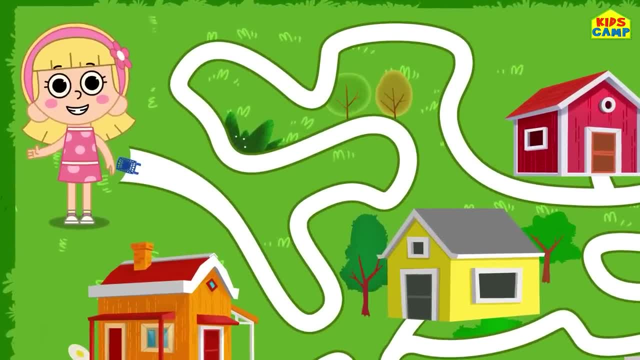 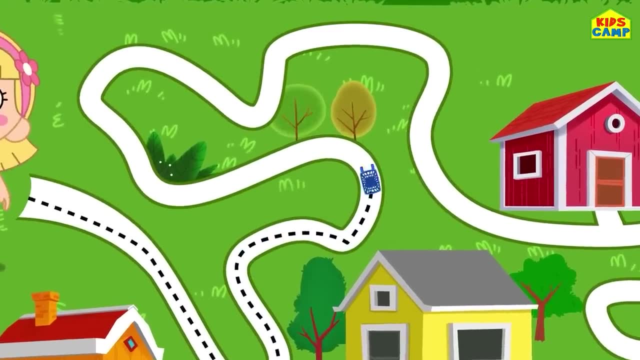 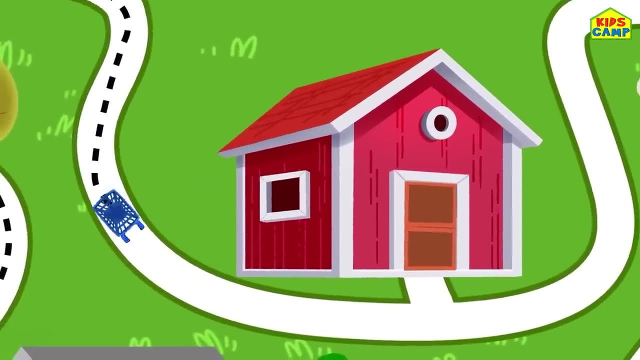 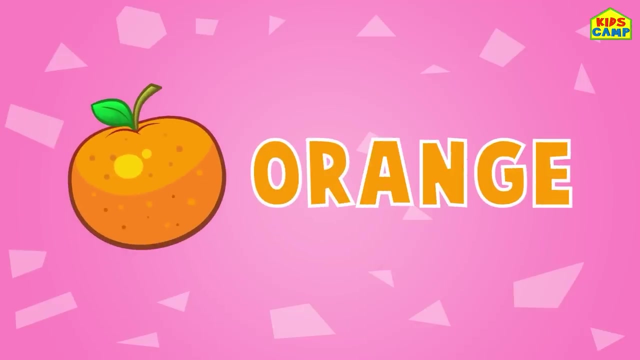 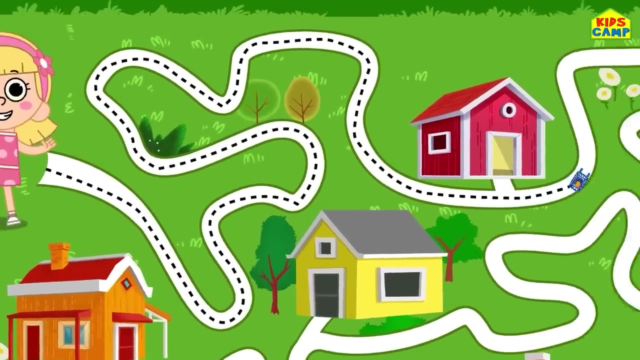 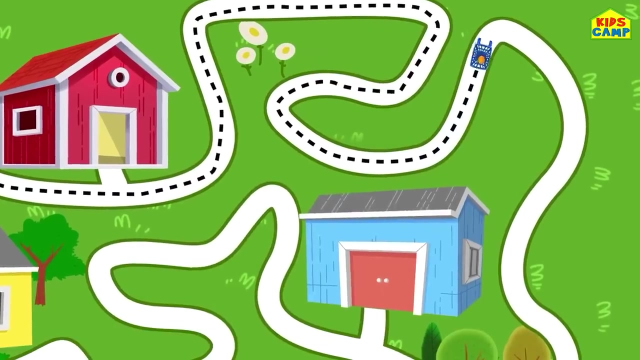 That's right. Here goes my cart, Let's collect fruits. Knock, knock, Hi, Do you have any fruit? Oooh, An orange Into my cart, Wonderful, Let's keep going. Ooh, Knock, knock. 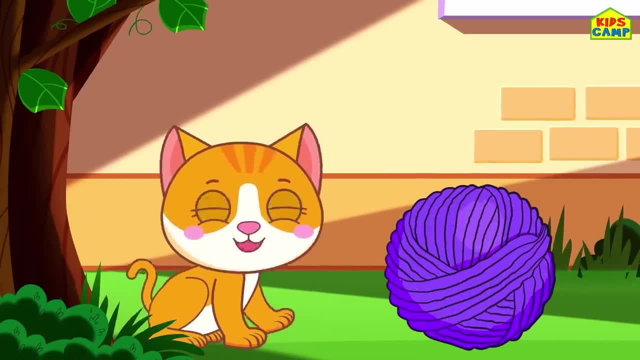 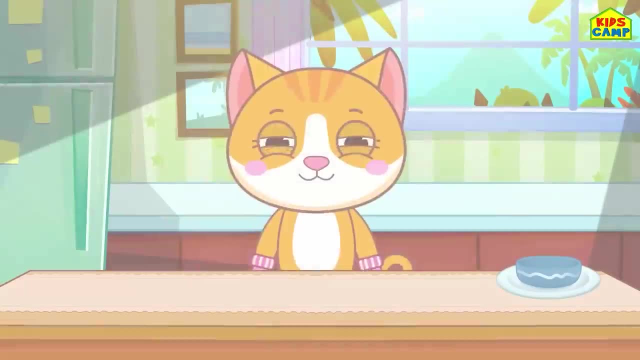 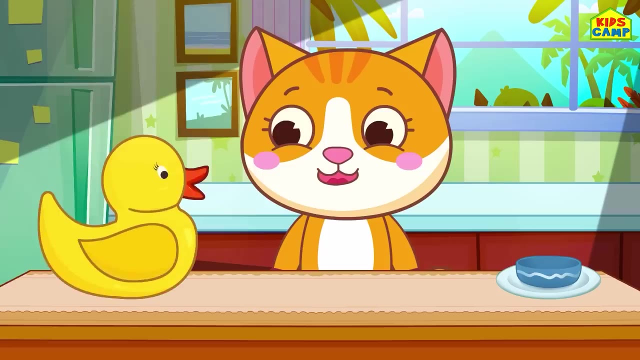 Yes, we can play with this. It's a ball of string. Wow, So much fun, So much fun. Now let's eat something. Are you hungry? Can you eat this? No, Can you eat this. No, No, Yes, you can eat this. 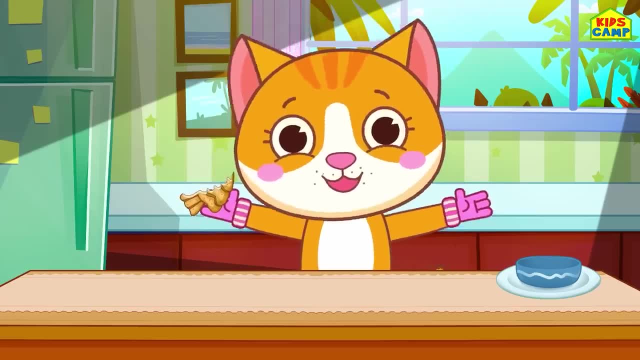 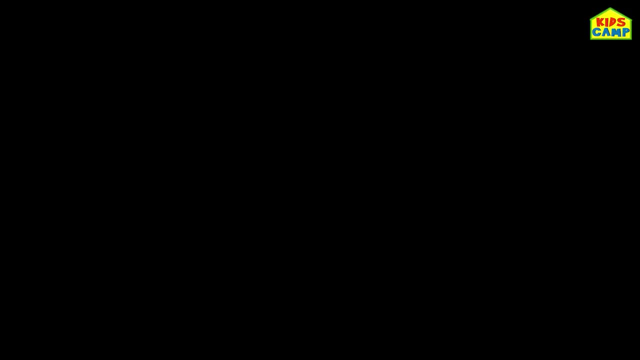 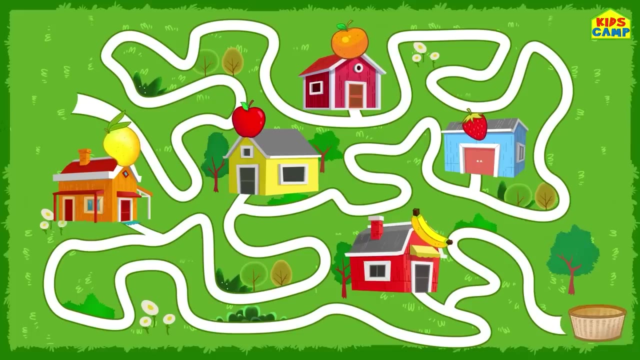 Don't you love the fish biscuit? Yummy, Wasn't it a fun day with my kitten. See you soon. Bye, Hi, I'm Ellie And I have to collect all the fruits into the basket. That's right. 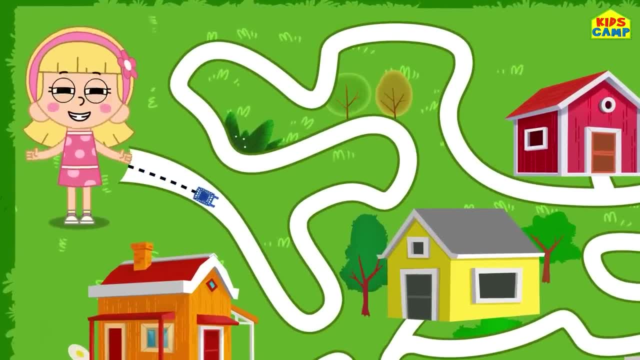 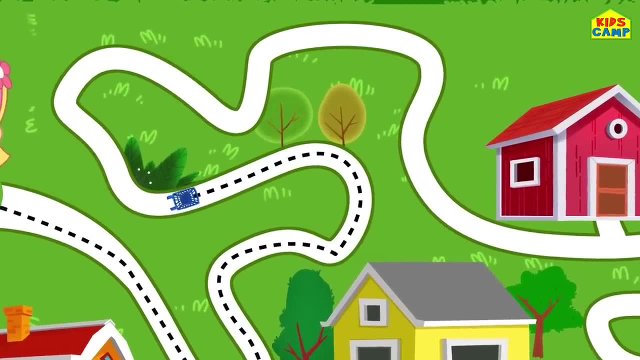 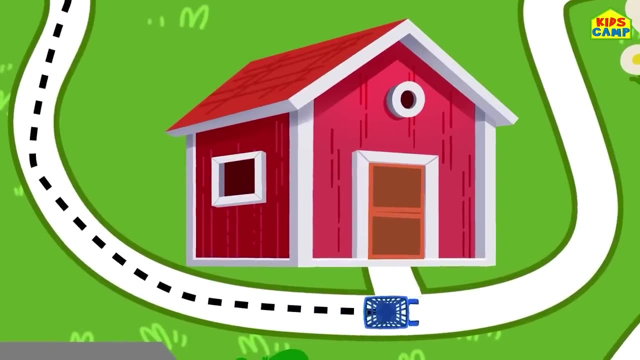 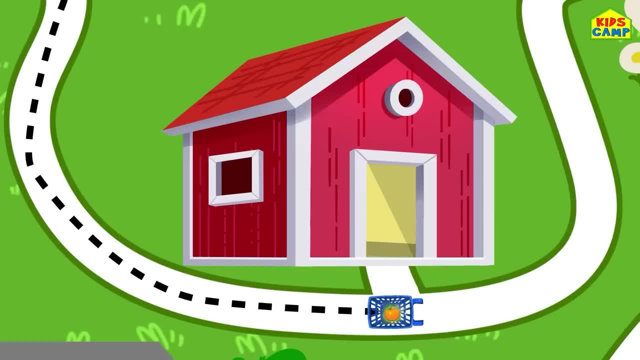 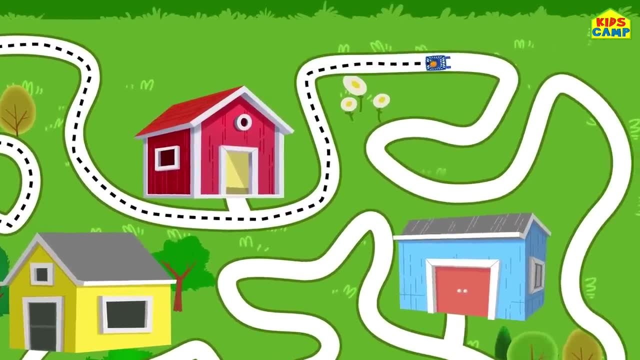 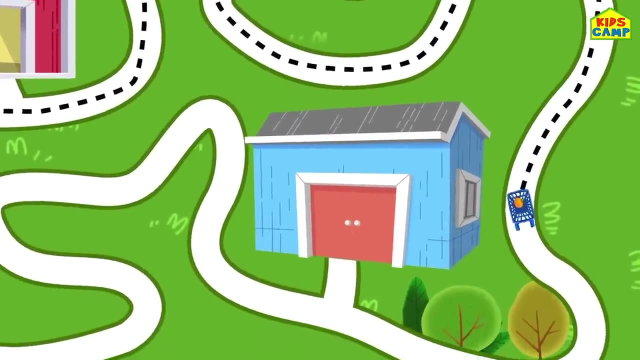 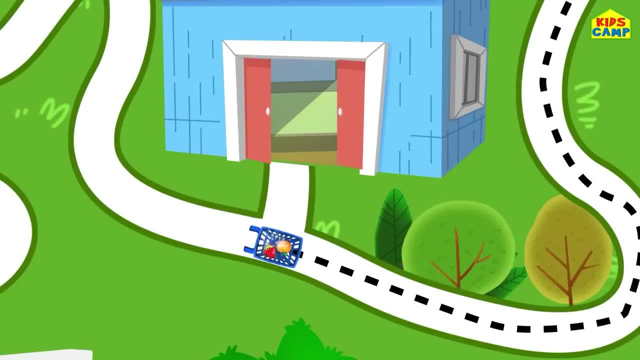 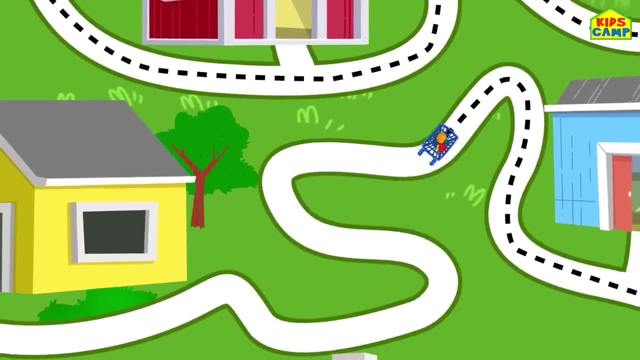 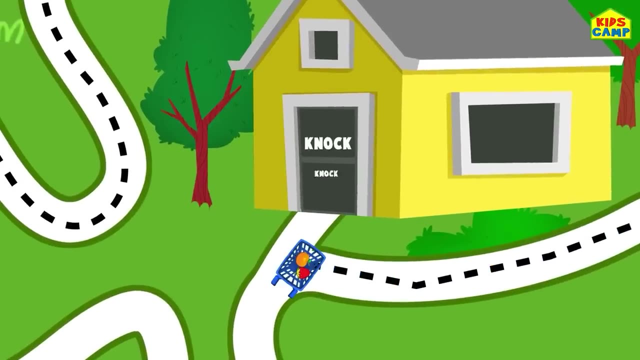 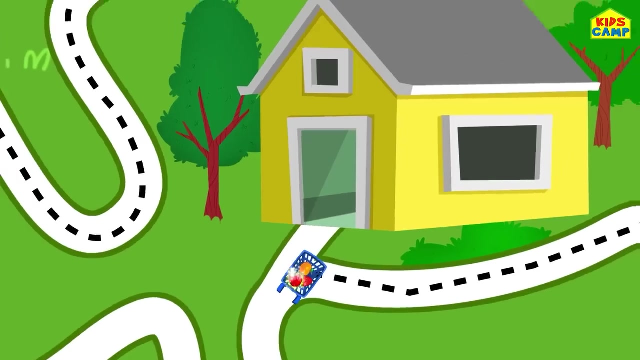 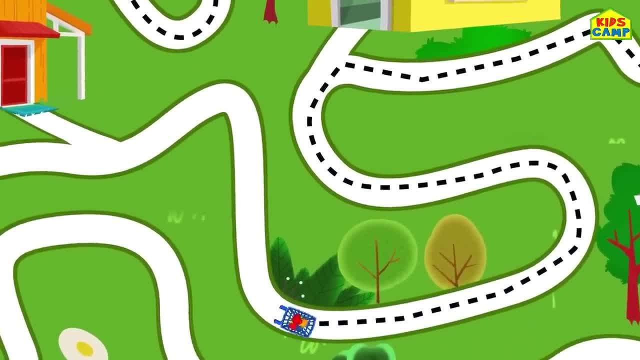 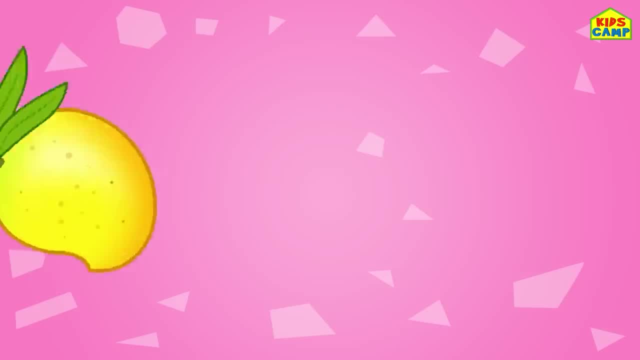 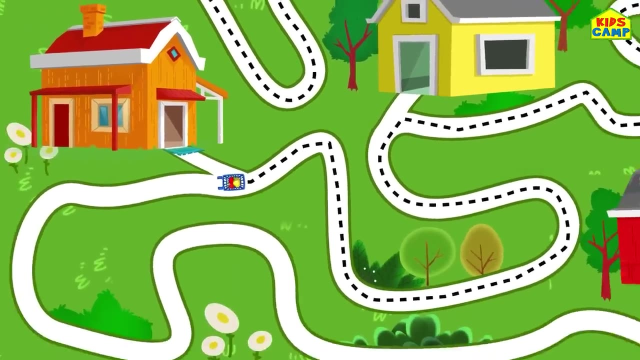 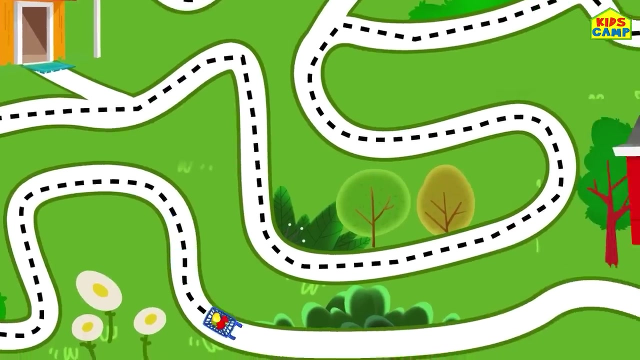 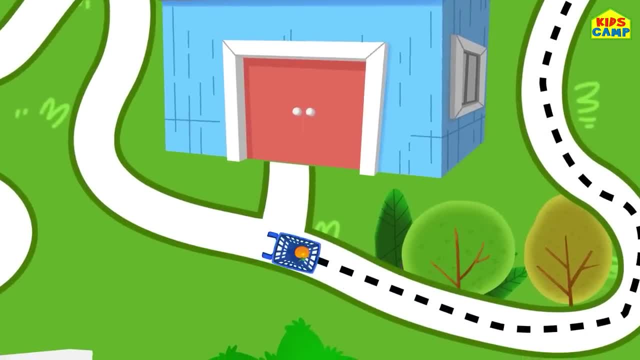 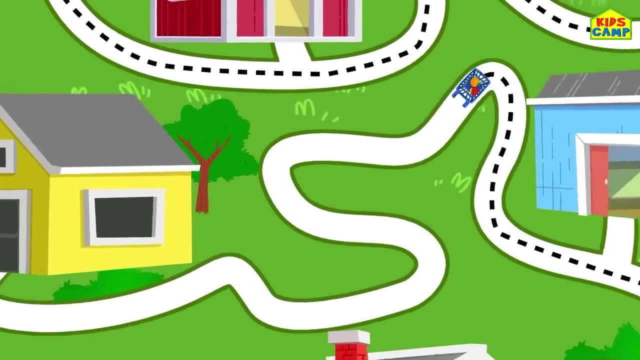 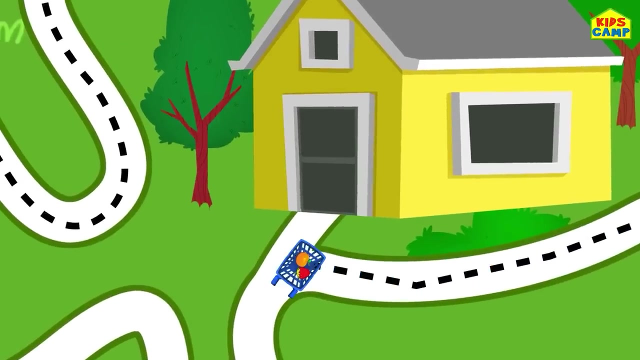 Do you have any fruit? Aha, A strawberry Into the cart. Wonderful, Let's get going. Knock knock, Hi. Do you have any fruit? Ooh, Knock knock. Do you have any fruit? Ooh. 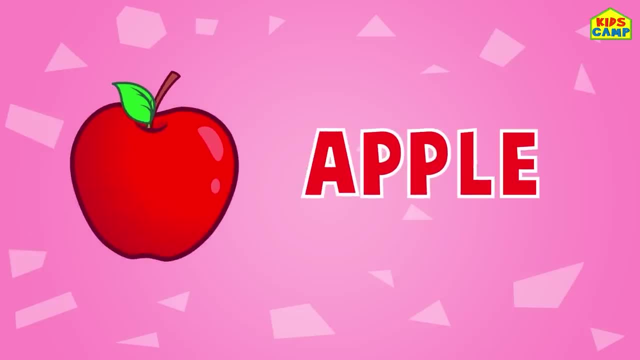 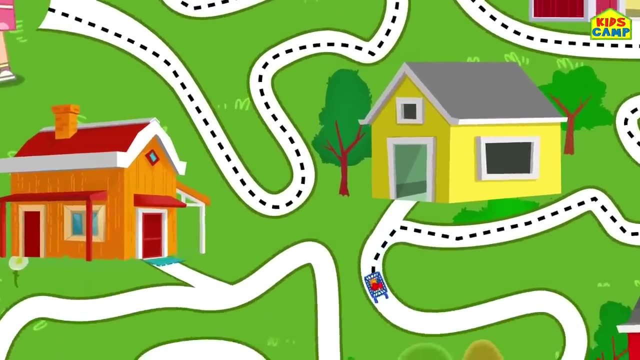 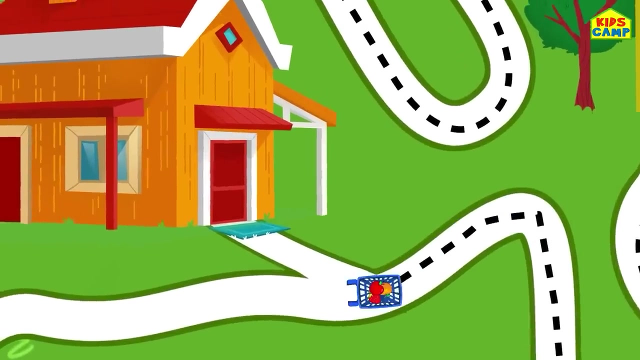 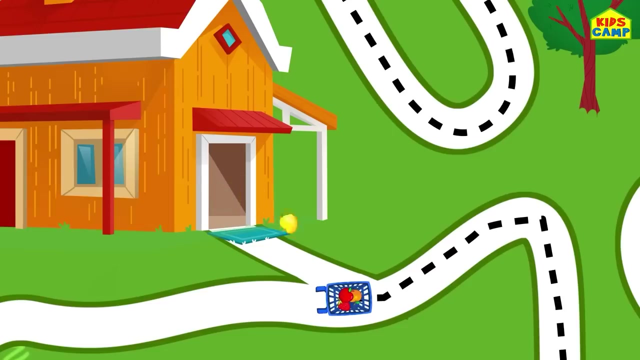 Knock knock, Hi. Do you have any fruit? Ooh, My favorite, An apple Into the cart. Yay, Let's keep going. Knock knock. Do you have any fruit? Ooh, A mango Into my cart. 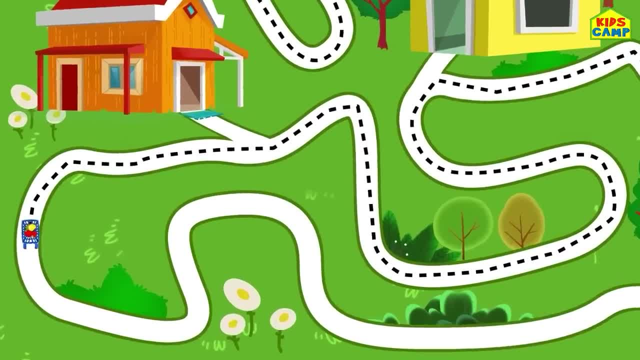 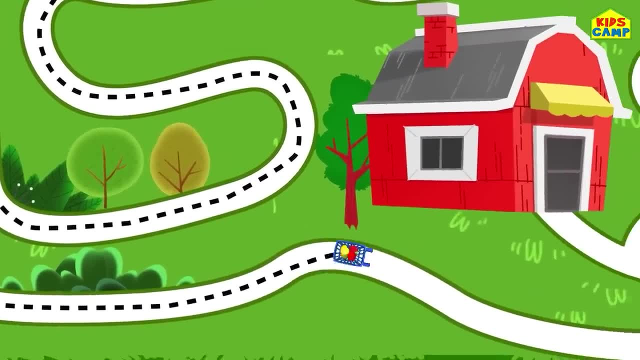 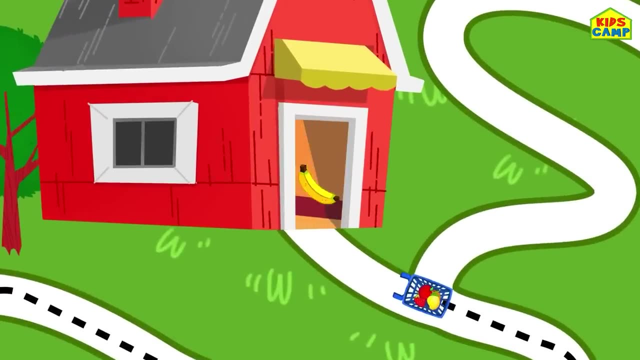 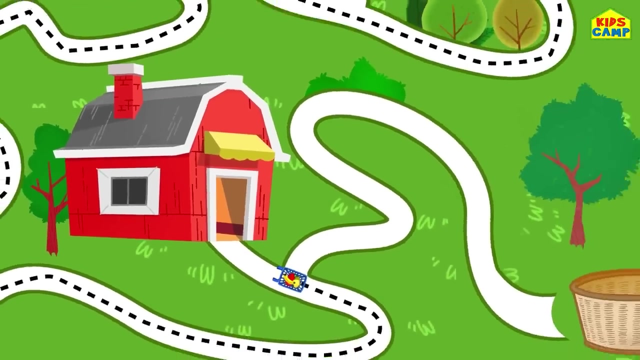 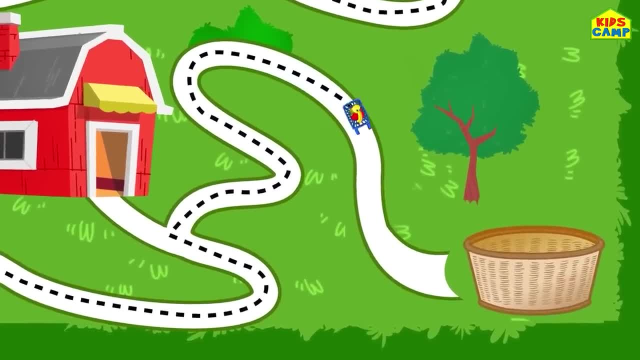 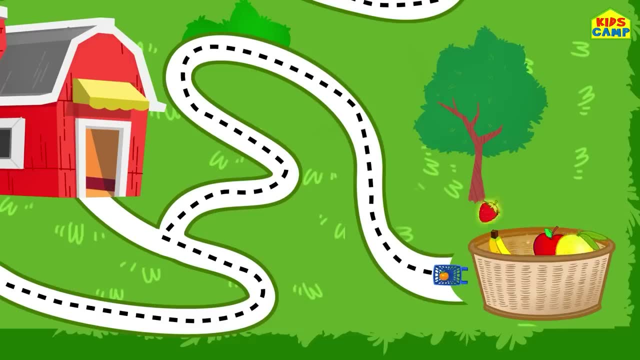 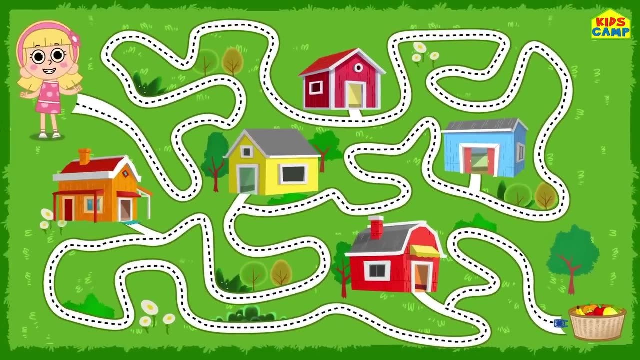 Let's keep going. Yay, We've collected all our fruits. What did we get? A banana, a mango, an apple, a strawberry and an orange. Good job, Thank you so much for helping me find my fruits and collecting them in my basket. 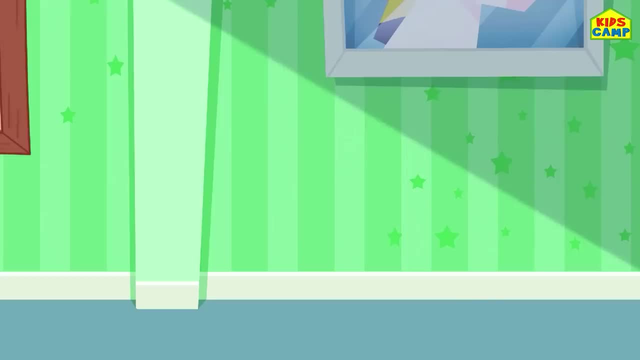 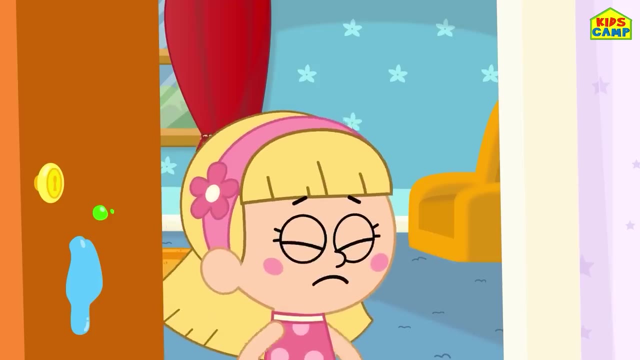 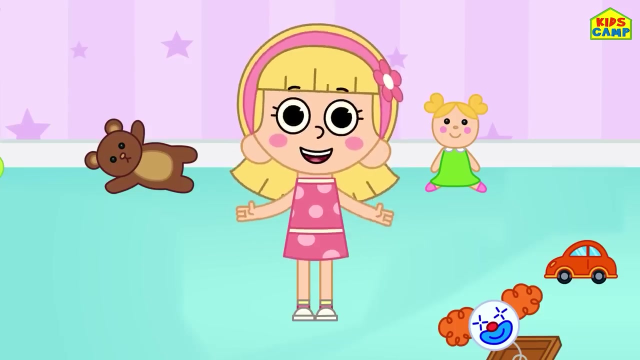 Thank you. Knock knock, Knock knock. Hi friends, I'm Elli and this is Eva. Eva, look at your room. You have to clean the room now. I know a fun way to clean our room: Let's find the objects and put them where they belong. 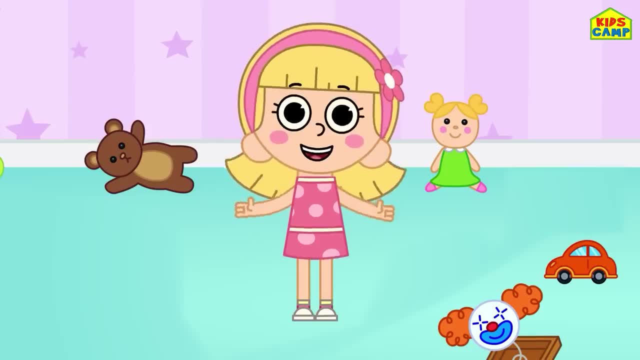 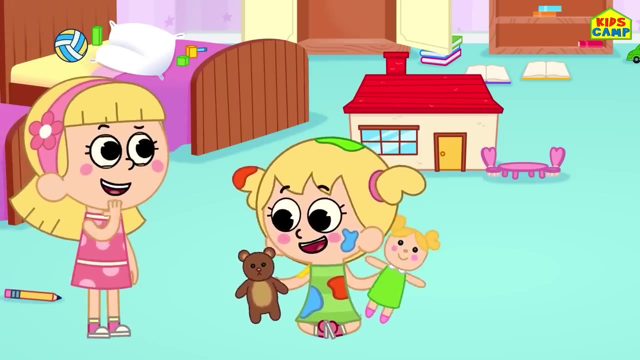 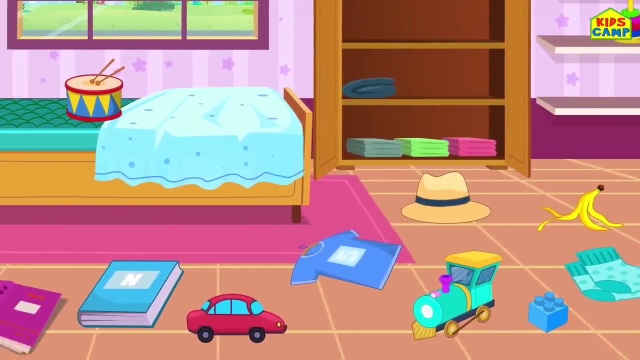 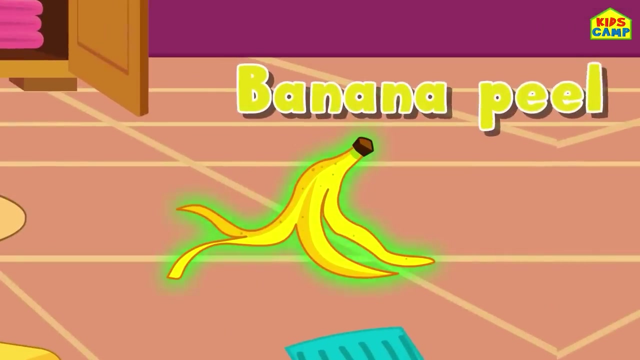 Eva, let's clean our room. Let's do this. friends Ready, Let's get started. Yay, Come on, Eva. Eva, you know what you have to do. That's right, Let's first pick up the banana peel. 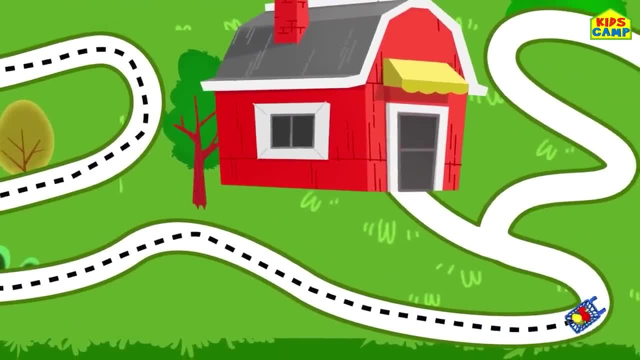 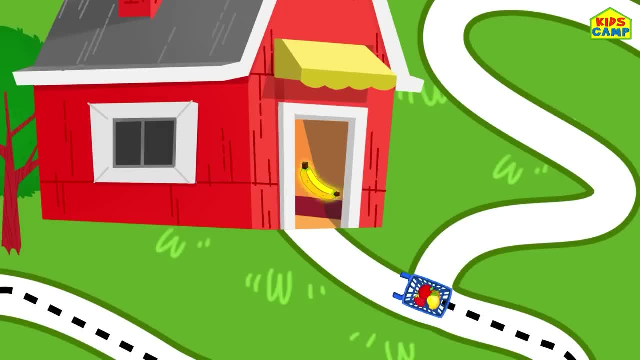 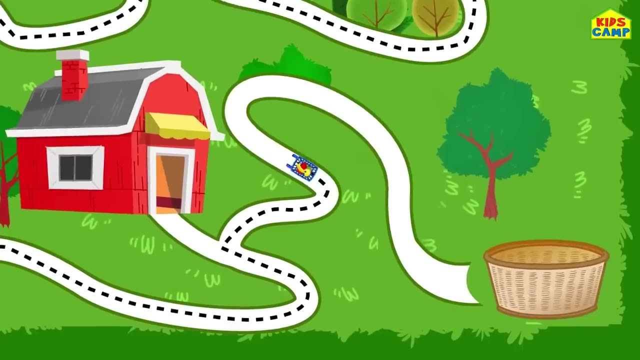 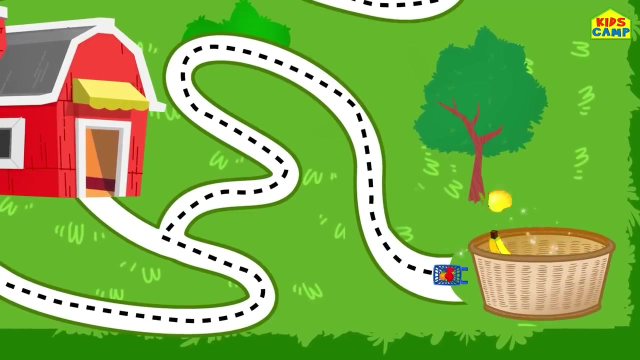 Keep going, Knock-knock. Hi, Do you have some fruit? A banana, Yay, Into the cart, Let's keep going. Yay, We've collected all our fruits. What did we get? A banana, a mango, an apple, a strawberry and an orange. 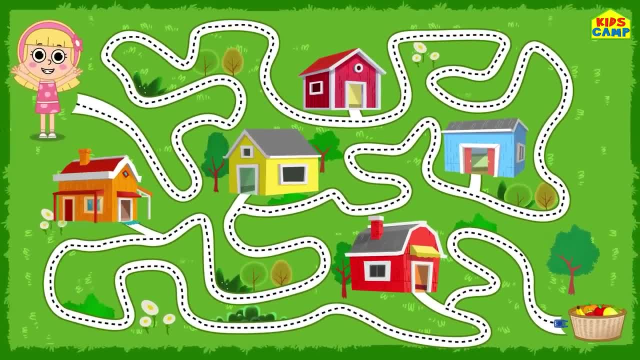 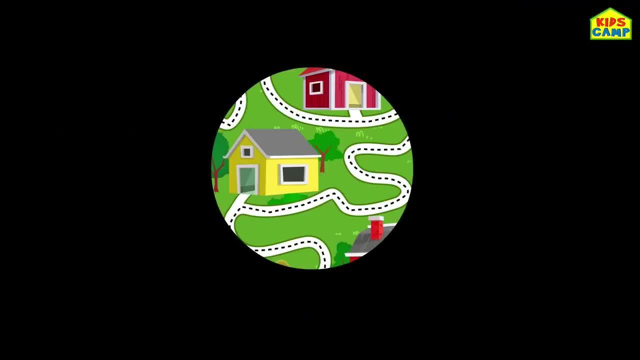 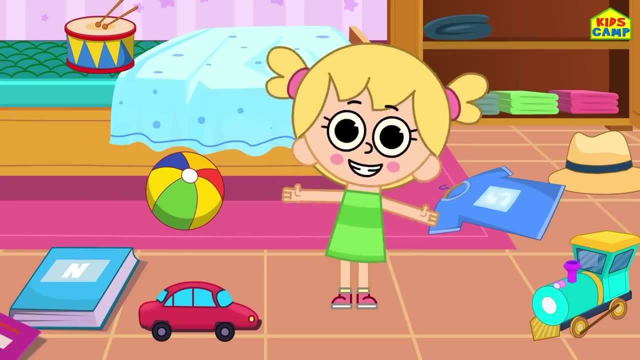 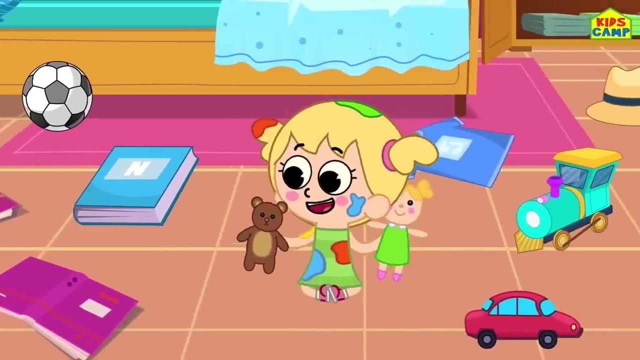 Good job. Thank you so much for helping me find my fruits and collecting them in my basket. Thank you, Hi friends, I'm Ellie and this is Eva. Eva, look at your room. You have to clean the room now. I know a fun way to clean our room. 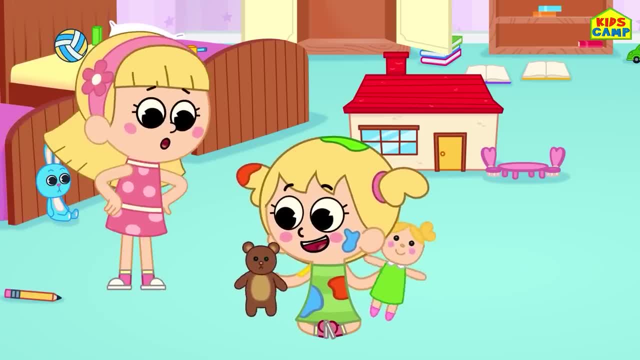 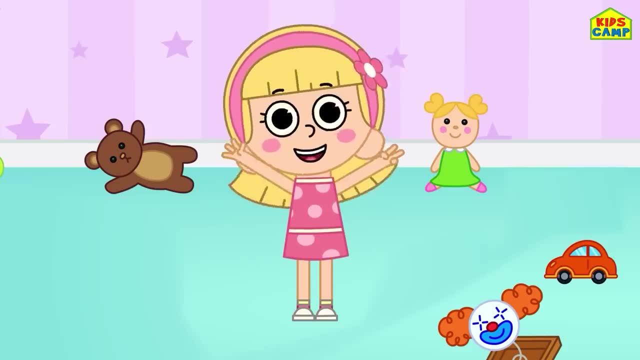 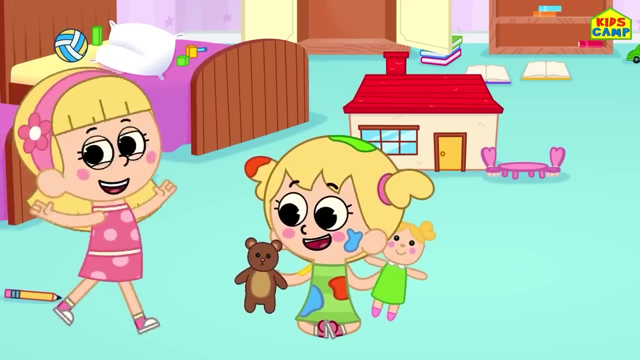 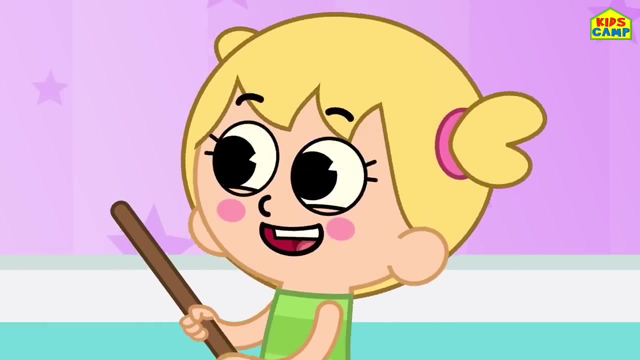 Let's find the objects and put them where they belong. Eva, let's clean our room. Let's do this. friends Ready, Let's get started. Yay, Come on, Eva. Eva, you know what you have to do, That's right. 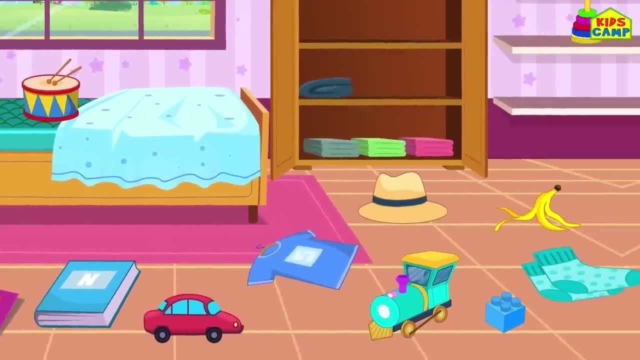 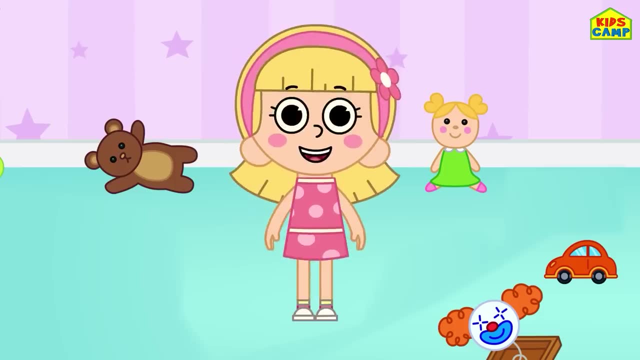 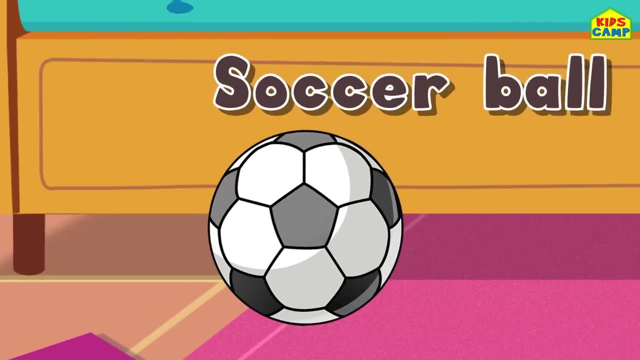 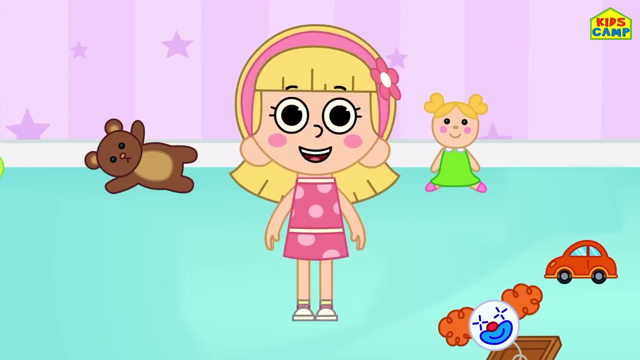 Let's first pick up the banana peel Into the dustbin. Good Job. Now what else? Let's pick up the soccer ball and keep it on our shelves. Good job, Eva. Very good, Let's clean some more. 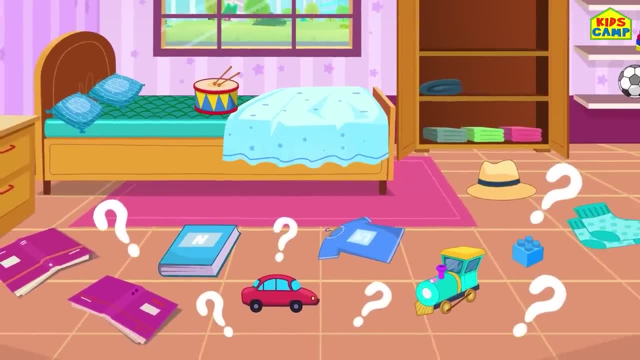 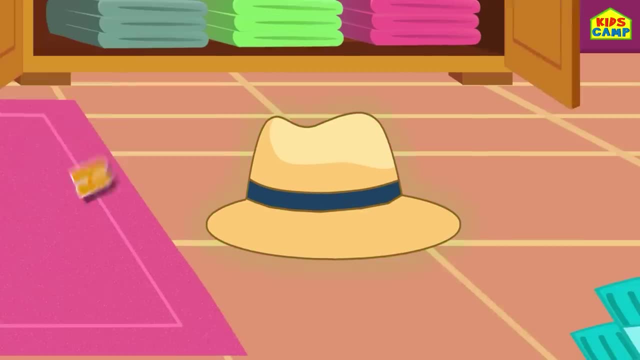 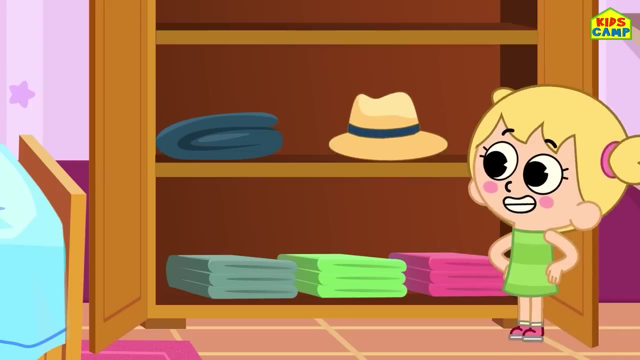 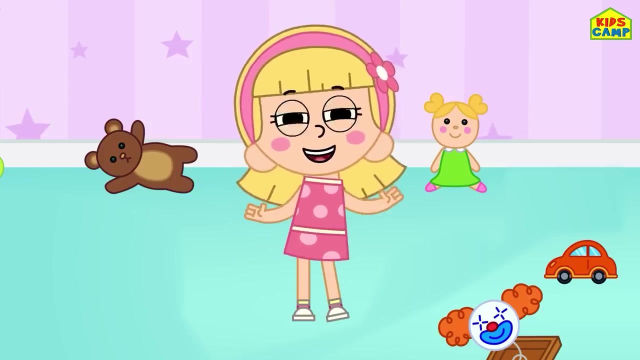 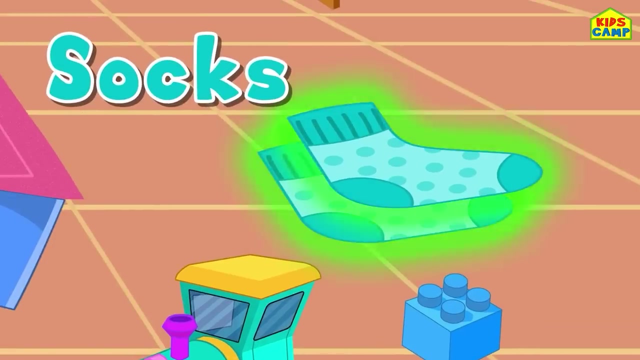 Good job, Eva. Very good, Let's look for the hat. Where is it? No, That's not a hat. No, That's a hat. That's right On to the shelves. Good job, Wow, Let's clean some more. Now let's look for the socks. That's right. 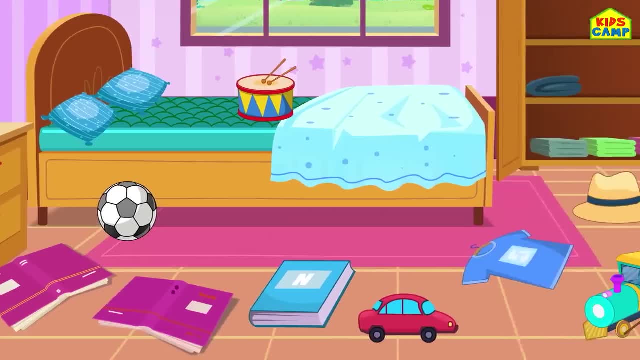 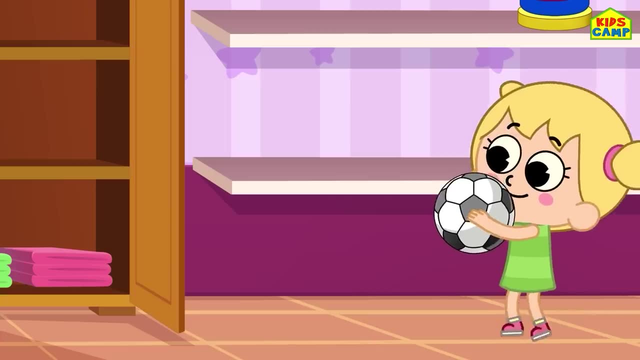 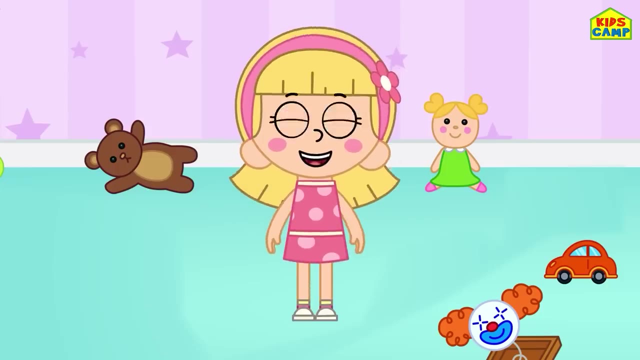 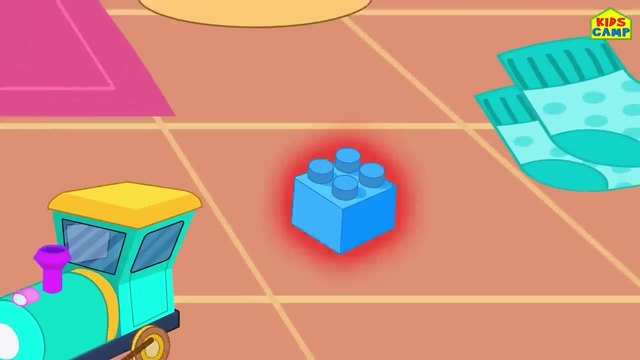 Into the dustbin. Good job. Now what else? Let's pick up the soccer ball And keep it on our shelf. Good job, Eva. Very good, Let's clean some more. Let's look for the hat. Where is it? 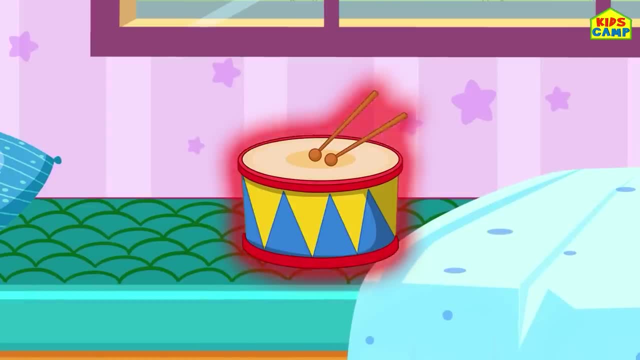 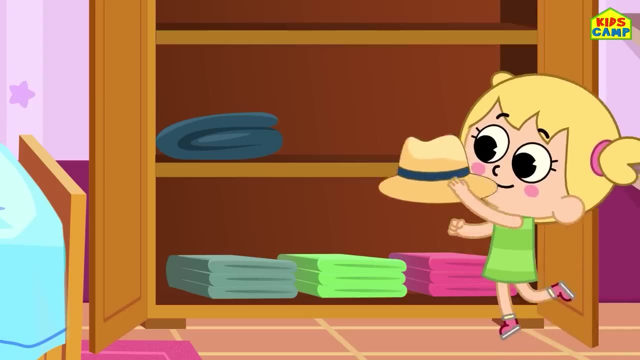 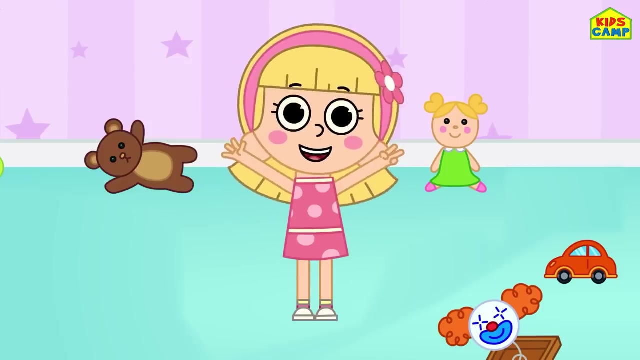 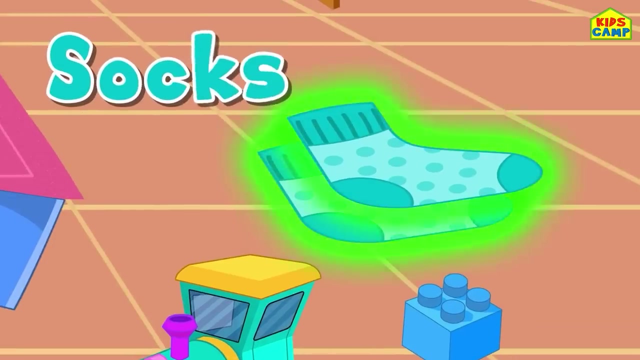 No, That's not a hat. No, That's a hat That's right On to the shelves. Good job, Let's clean some more. Now let's look for The socks. That's right Into the drawer- Wonderful. 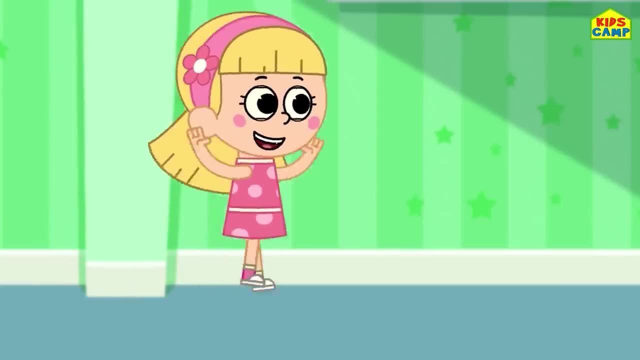 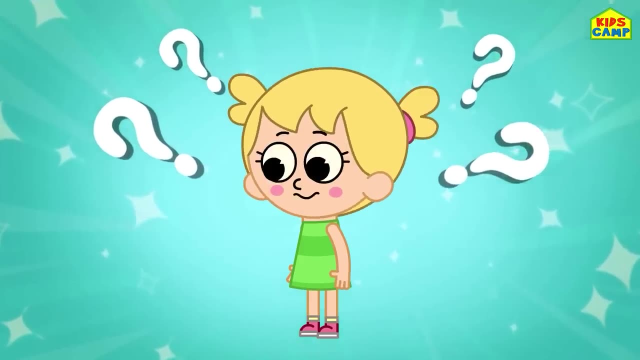 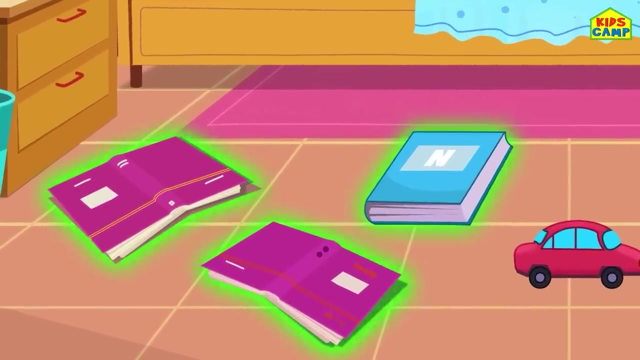 Very good, Eva. where are your books? Look for them. That's right, Here are the books. Let's see what's inside. Let's see what's inside. Here are the books. Let's see what's inside. Let's pick them up. 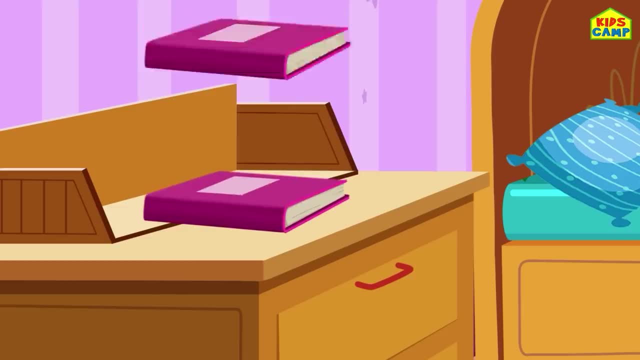 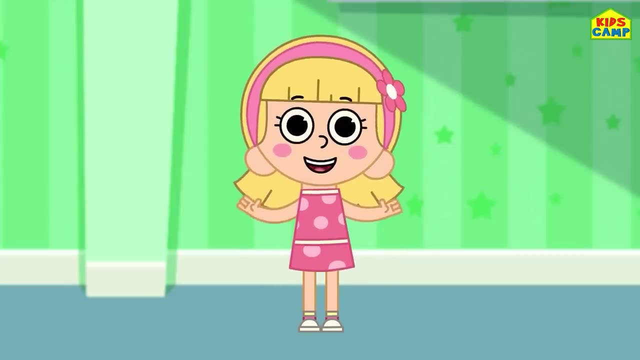 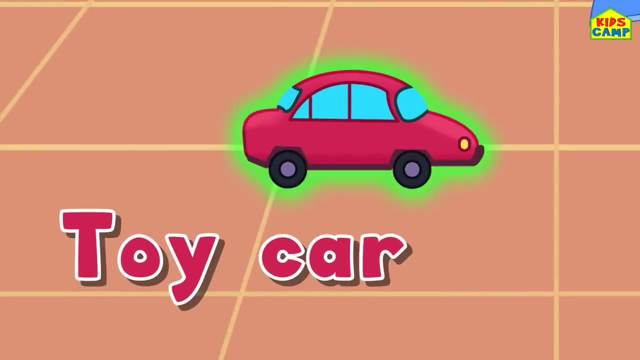 Very good, Stack them together. The room already looks clean, Wonderful. Now let's look for the toy car. That's right, Amazing. On to the shelf. Good job, Eva. Let's clean some more. That's right, Amazing. 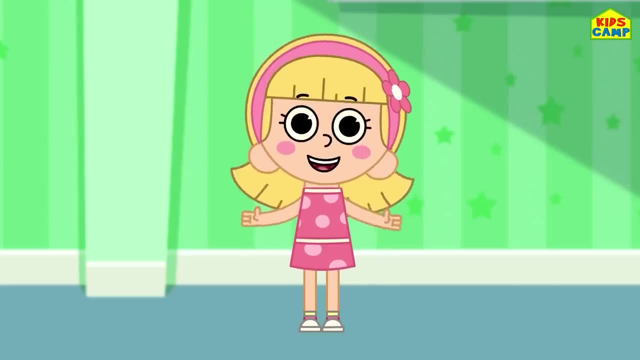 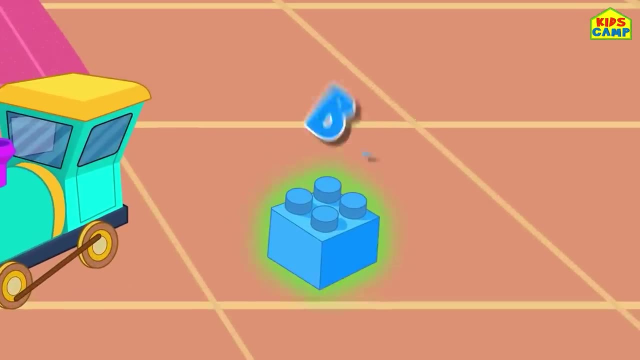 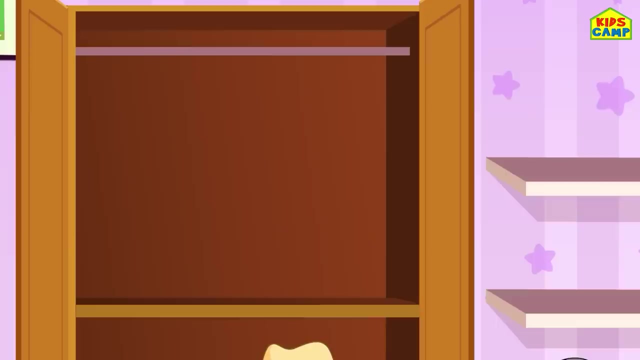 On to the shelf. Good job, Eva. Let's clean some more. Let's clean some more. The block, The block, And the t-shirt, And the t-shirt. Eva, let's pick them up, Eva, let's pick them up. 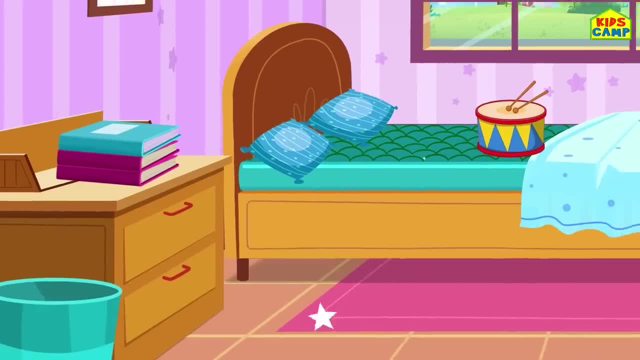 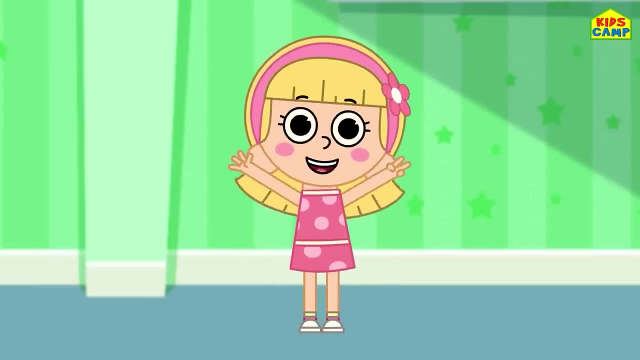 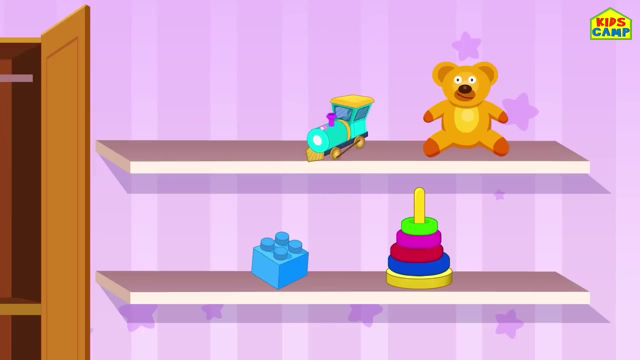 Into the cupboard And on the shelf. Good girl, Wonderful, Wonderful, Let's clean some more. Let's clean some more. The juju train On to the shelf. We did it, We're almost there. Good job, friends. 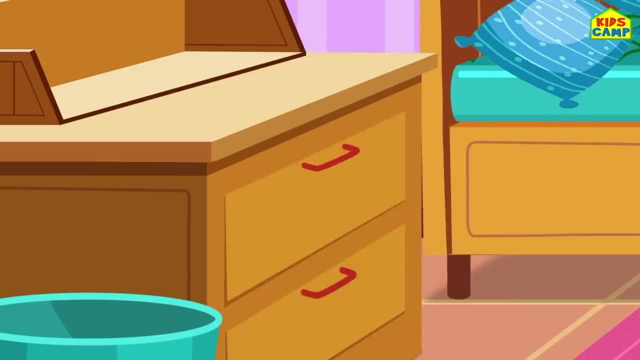 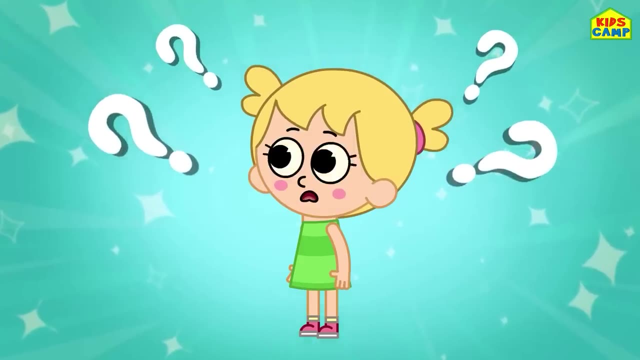 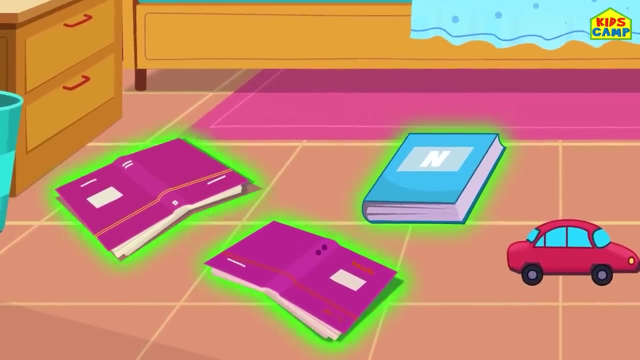 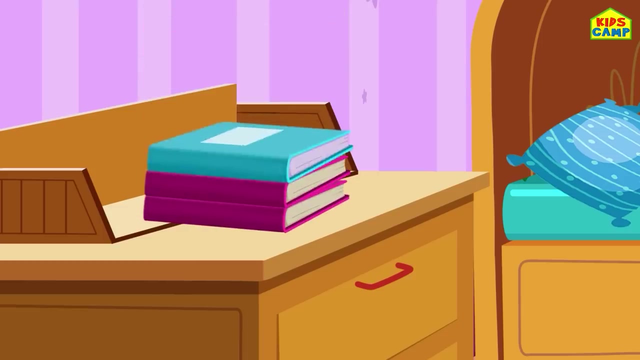 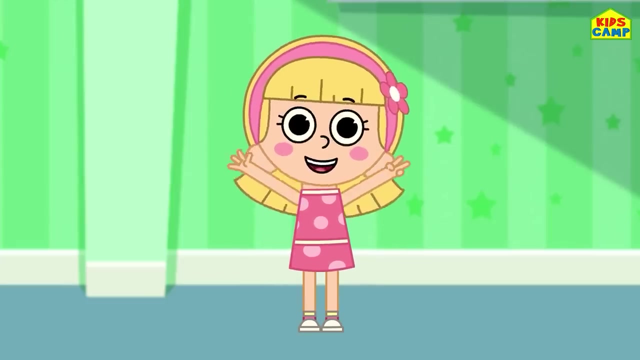 Into the drawer, Wonderful. Very good, Eva. where are your books? Look for them. That's right. Wow, Here are the books. Let's pick them up. Very good, Stack them together. The room already looks clean, Wonderful. 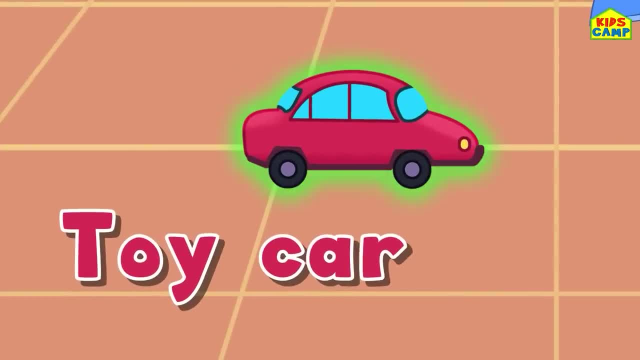 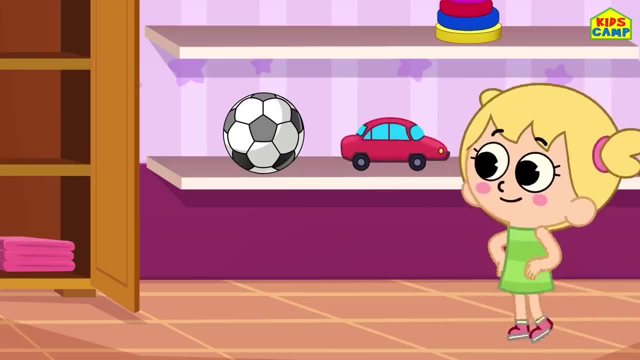 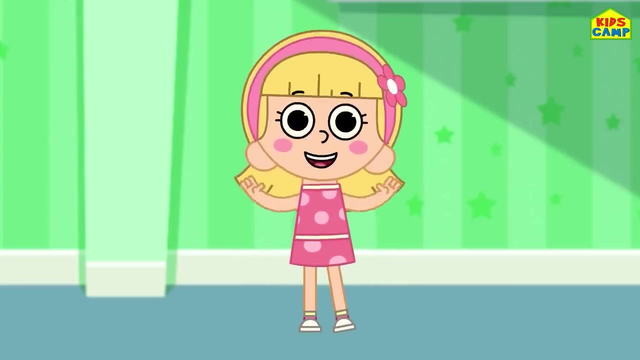 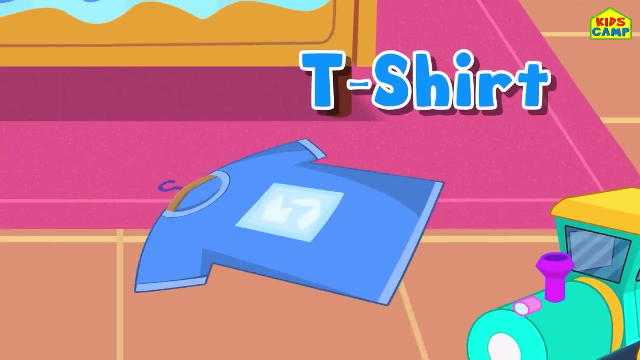 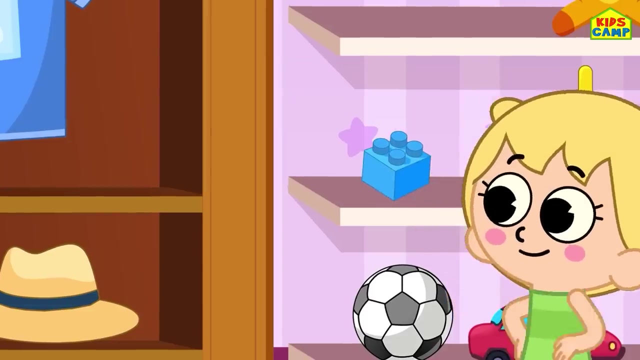 Now let's look for the toy car That's right- Amazing- On to the shelves. Good job, Eva. Let's clean some more: The block and the t-shirt, Eva. let's pick them up Into the cupboard and on the shelves. Good girl, Wonderful. 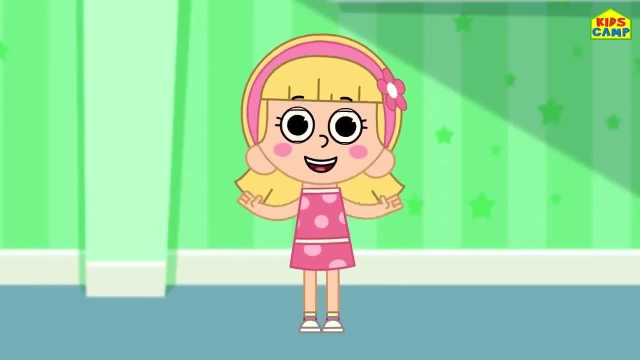 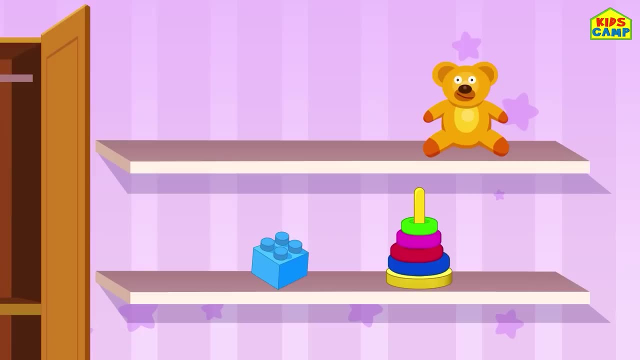 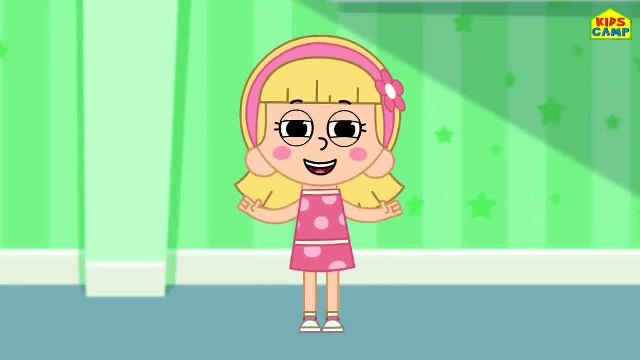 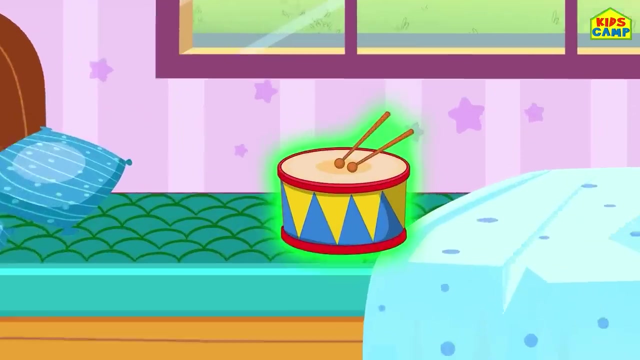 Let's clean some more. Good job, Some more. The couple keeps things clean, The Choo Choo train On to the shelf. We did it, We're almost there. Good job, friends. Wonderful C'mon The to y drum. 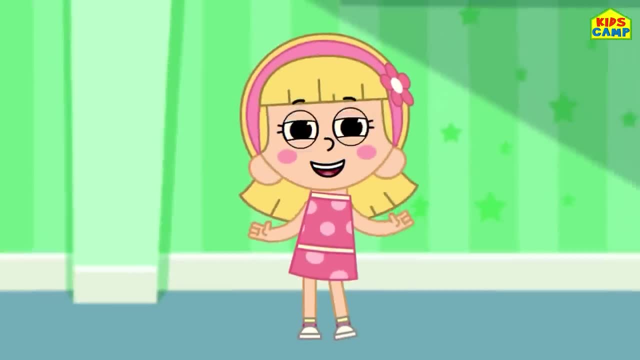 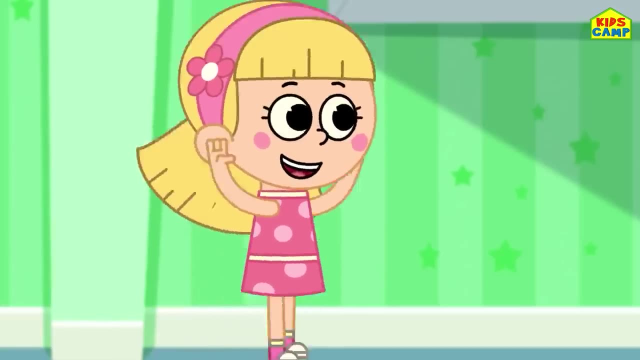 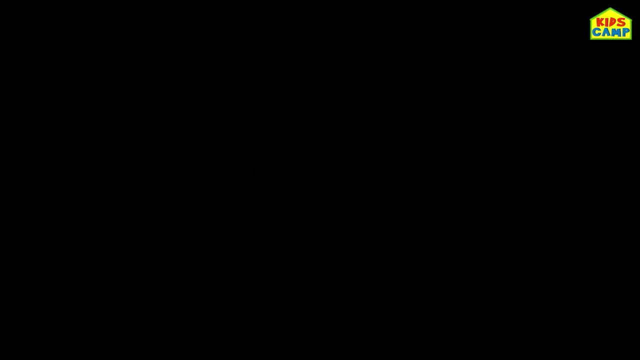 Let's pick it up And put it on the shelf. That's right, Our room looks clean. Yay, Good job, Eva. Wonderful, That's how you clean your room, Wasn't that fun kids? Bye, Hi friends. I'm Ellie. 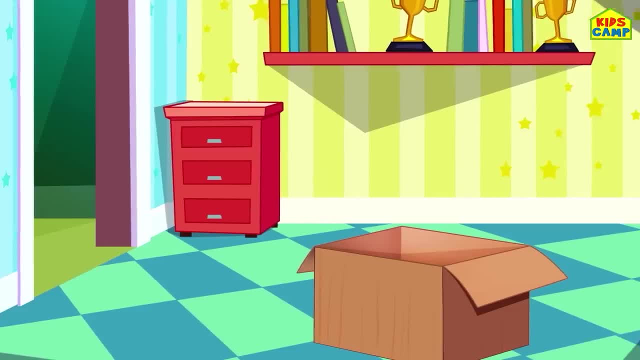 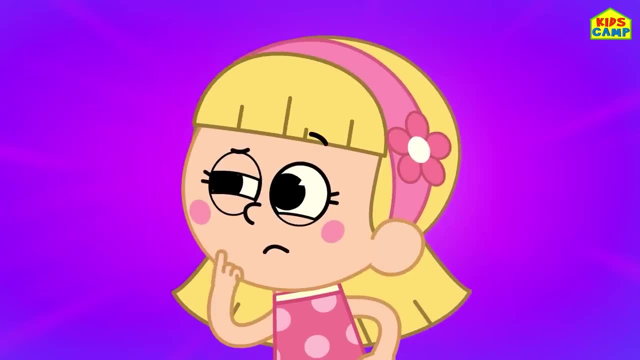 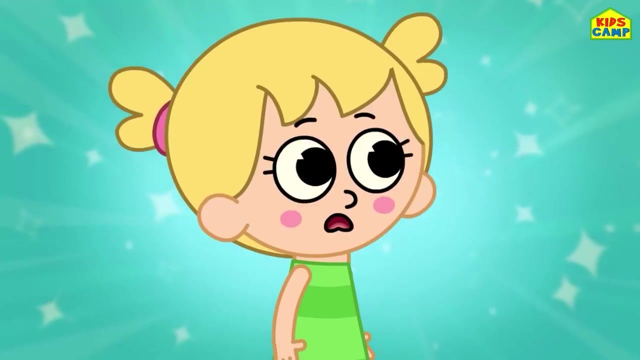 But I can't find my cat. I don't know where she's gone. Can you help me look for her? Hi Eva, Where's our cat? That's right, She's in the box. Eva seems to be confused, Don't worry. 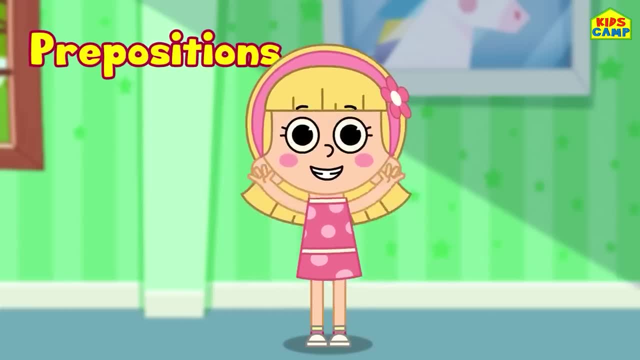 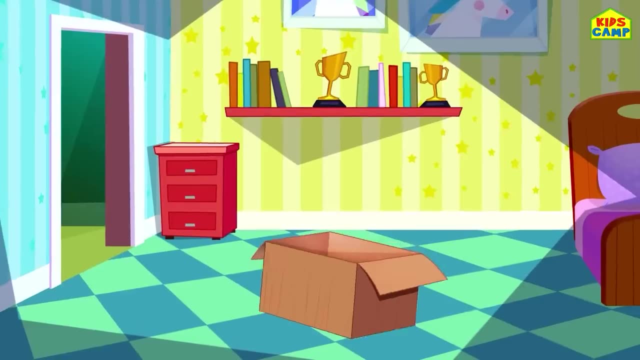 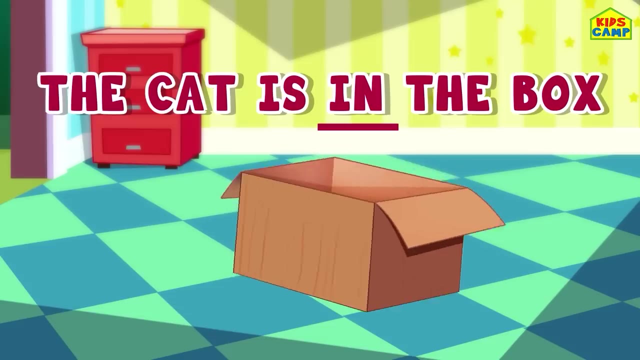 Today we are going to learn prepositions And how and where to use them. Ready, Let's start. The first preposition is IN. The cat is in the box. Do you see that, Eva? Eva, She's in it. 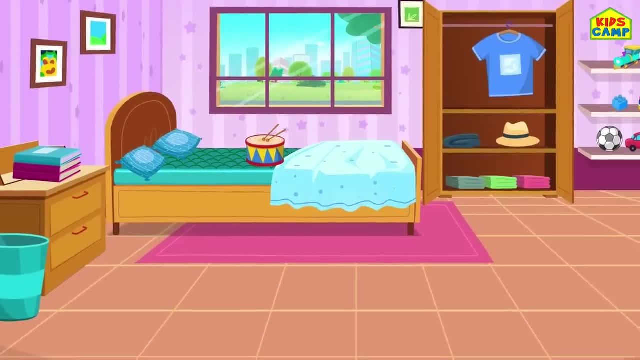 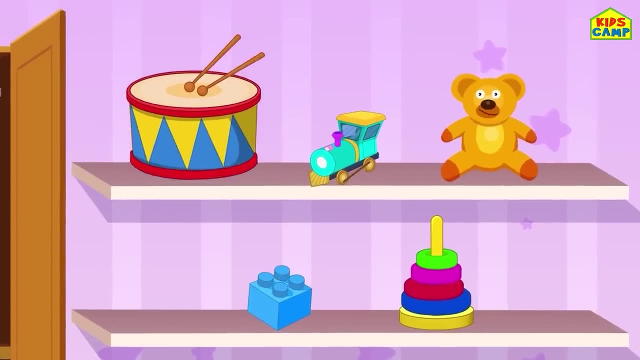 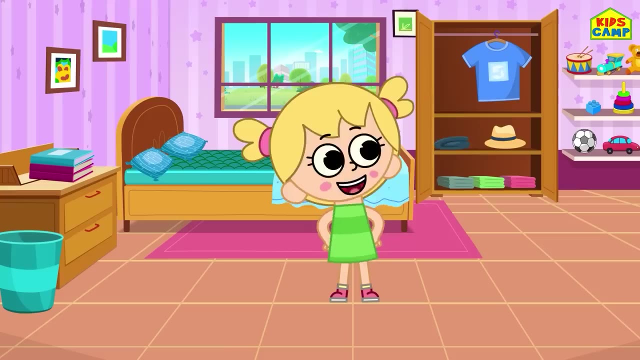 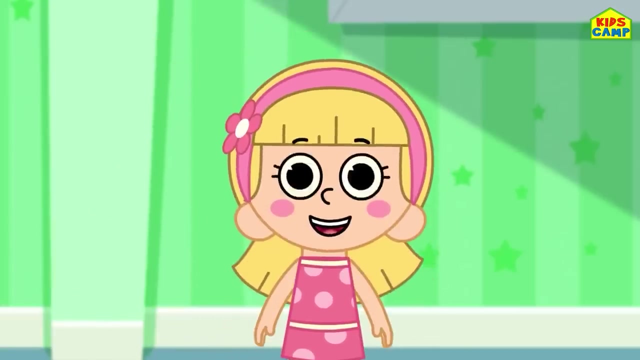 Wonderful, The toy drum. Let's pick it up And put it on the shelf. That's right, Our room looks clean. Yay, Good job, Eva. Wonderful, That's how you clean your room. Wasn't that fun kids. 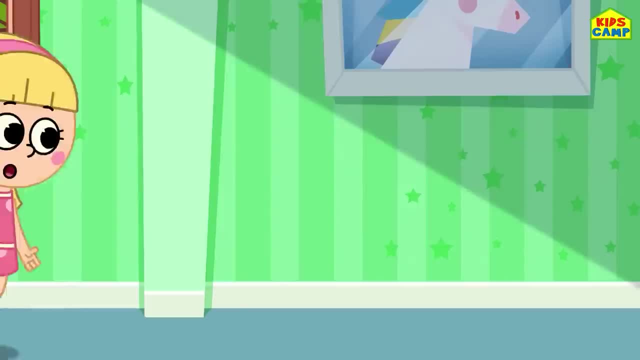 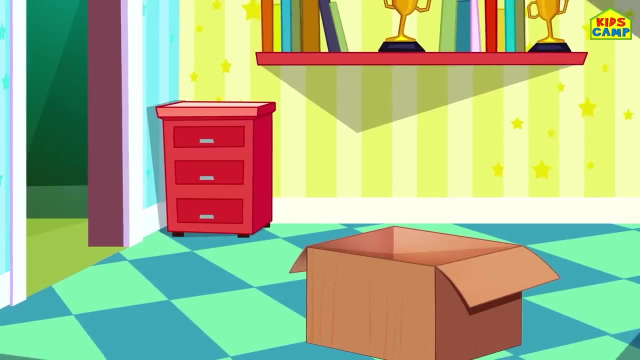 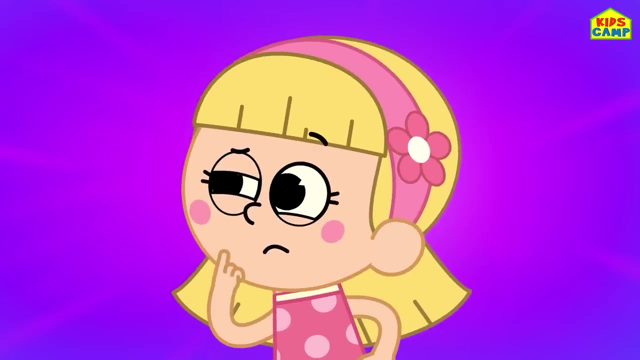 Bye, Hi friends. I'm Ellie, But I can't find my cat. I don't know where she's gone. Can you help me look for her? Hi Eva, Where's our cat? That's right, She's in the box. 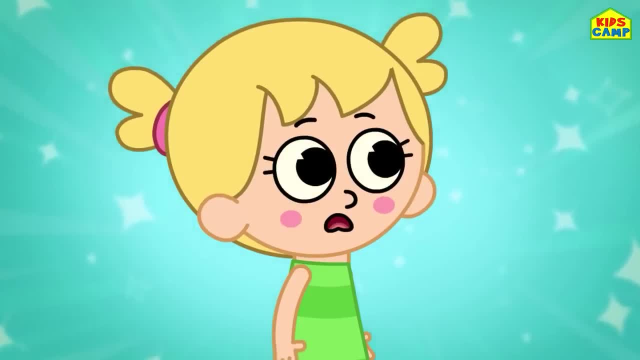 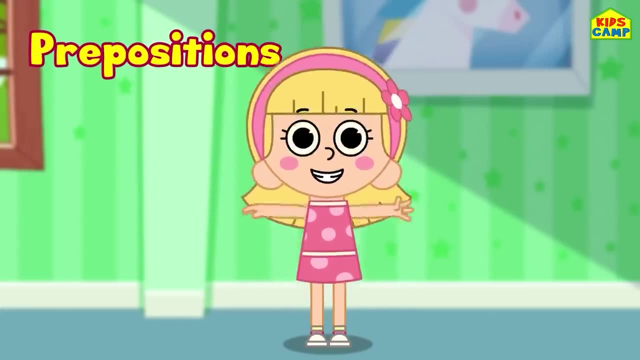 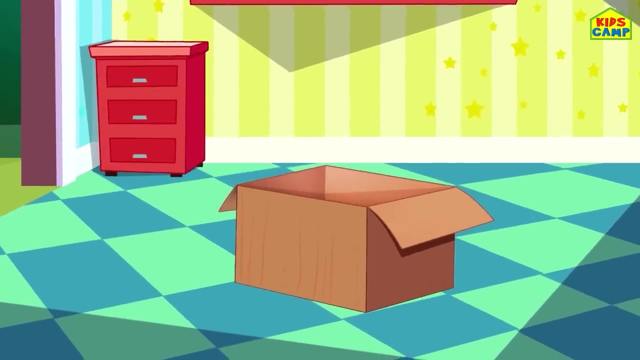 Hmm, Eva, seems to be confused. Don't worry, Today we're going to learn prepositions And how and where to use them. And how and where to use them. Ready, Let's start. The first preposition is In. The cat is in the box. 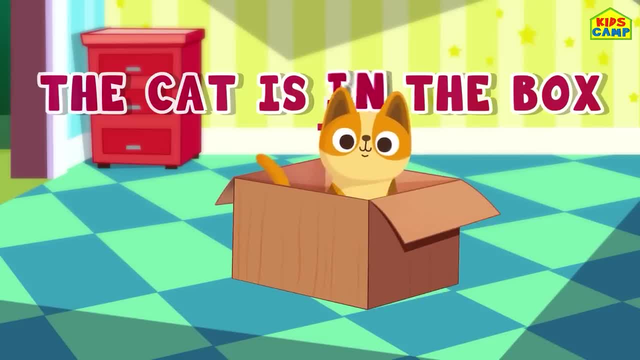 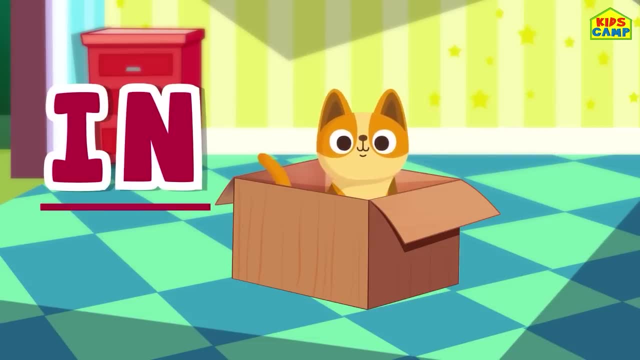 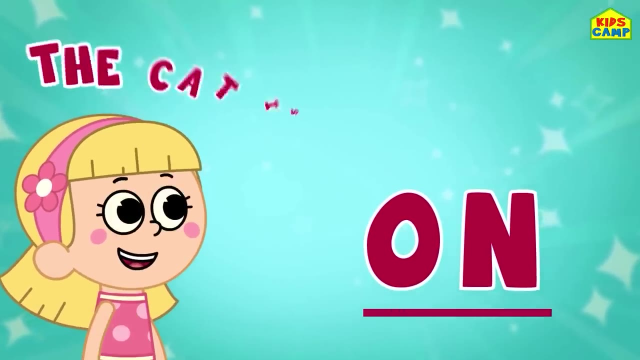 Do you see that, Eva? She's in it. In is the preposition, And this is how we use it To show the position. The next one is On. That's right. The cat is on the box, Yay. 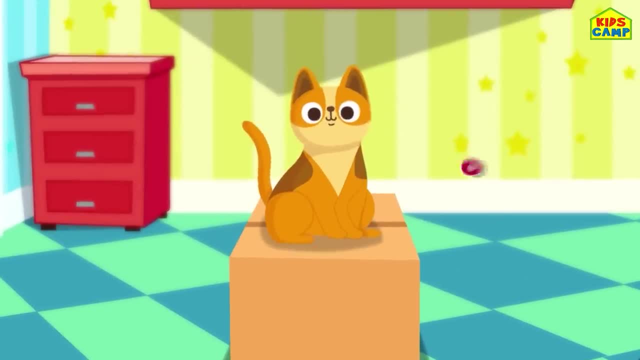 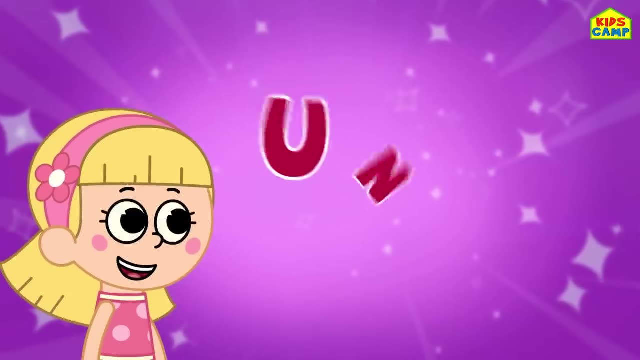 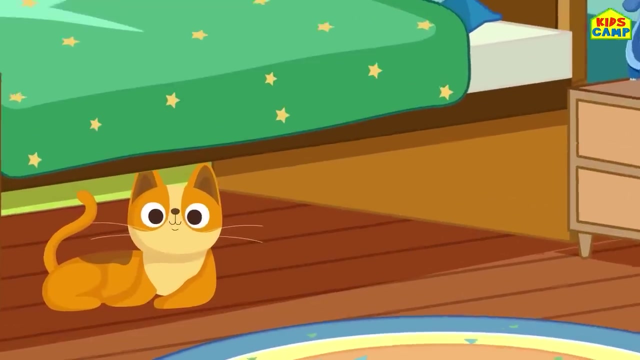 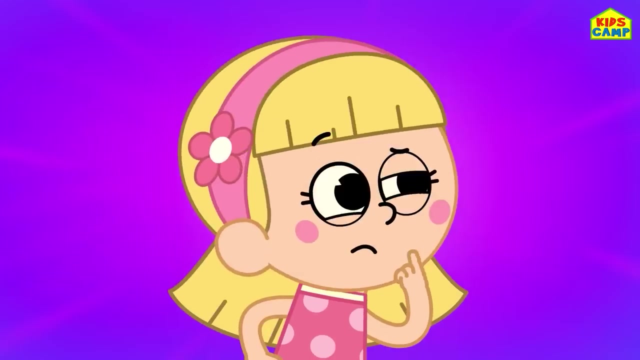 This is easy, Isn't it? This is how we use the preposition On. Next is Under or Beneath. The cat is under the bed. There she is. We found her. Good job, friends. Where is the cat now? 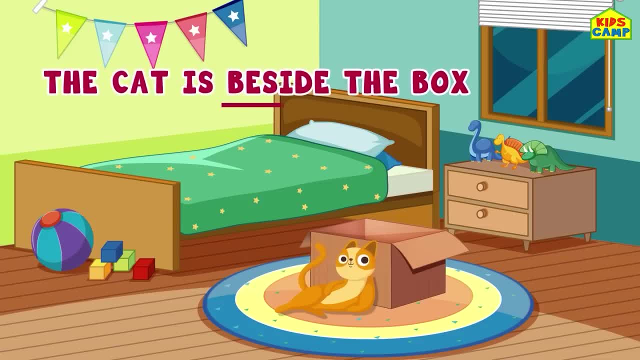 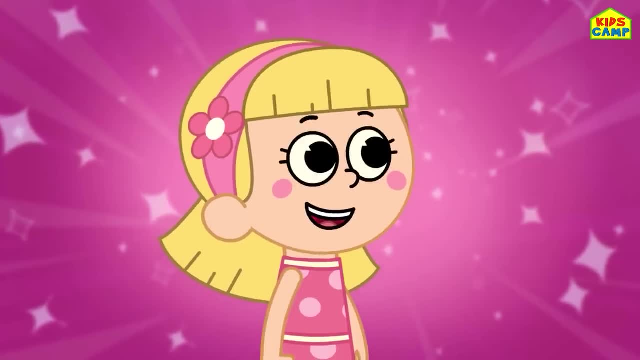 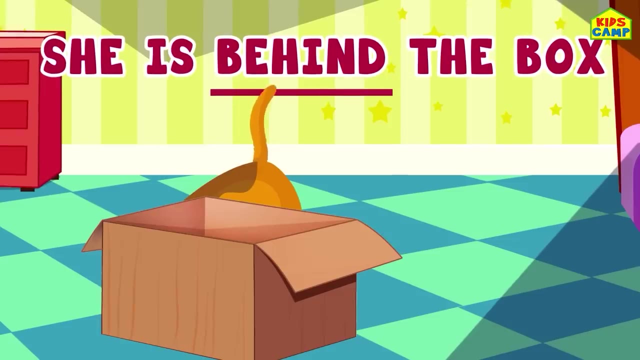 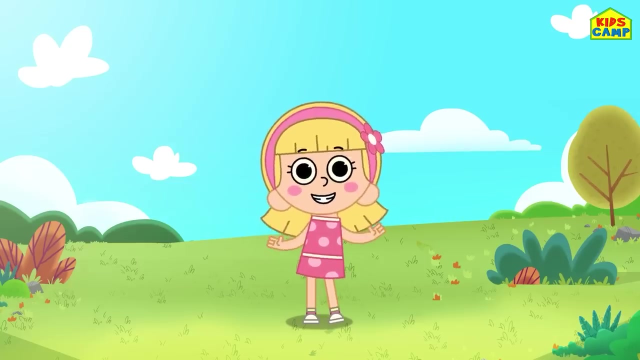 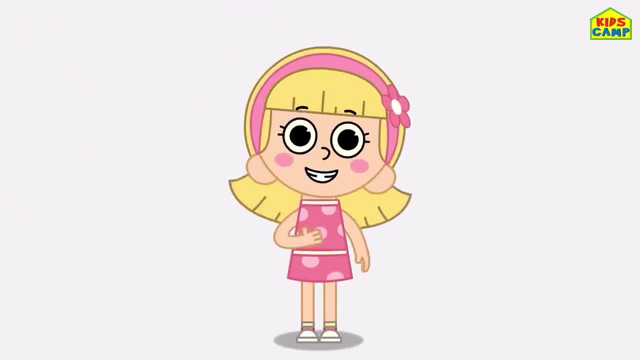 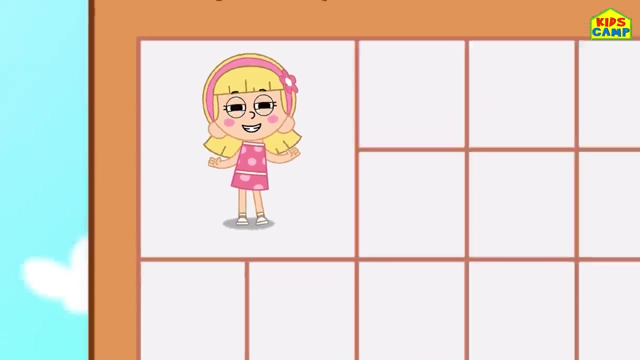 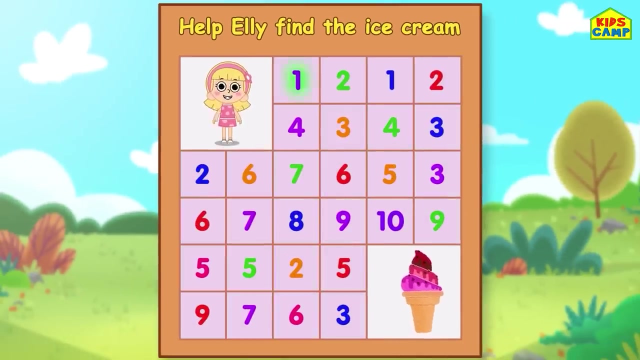 The cat is besides the box. She's beside it, Right. Where is the cat now? She is behind the box. There she is. Come back for more games and keep watching Kids' Camp. Until then, bye-bye On number one. 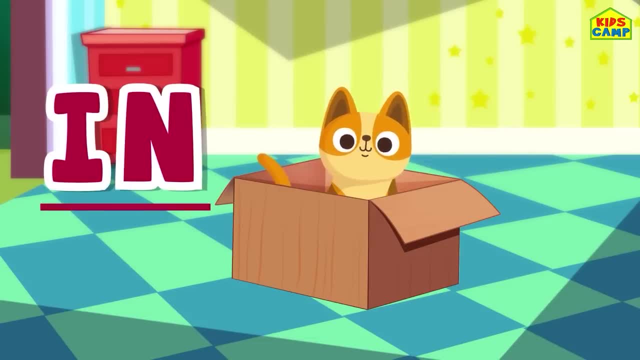 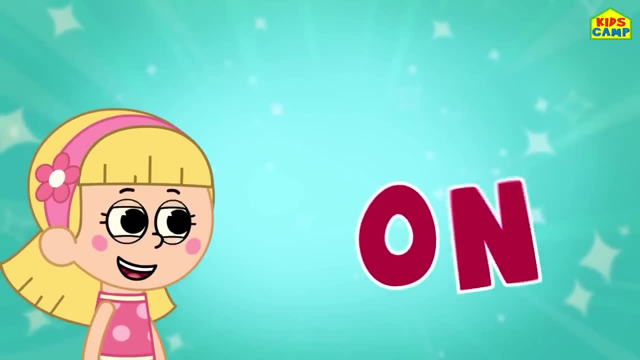 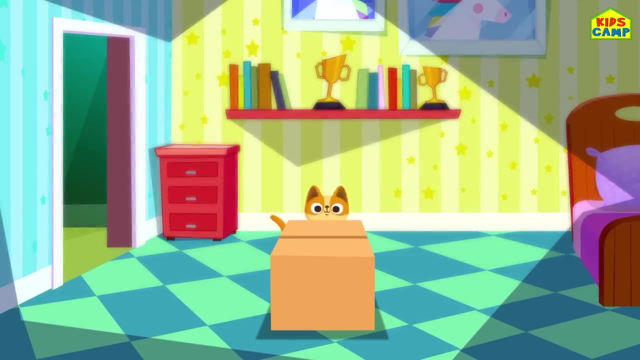 IN is the preposition, And this is how we use it To show the position. The next one is ON. That's right, The cat is on the box. Yay, This is easy, isn't it? This is how we use the preposition ON. 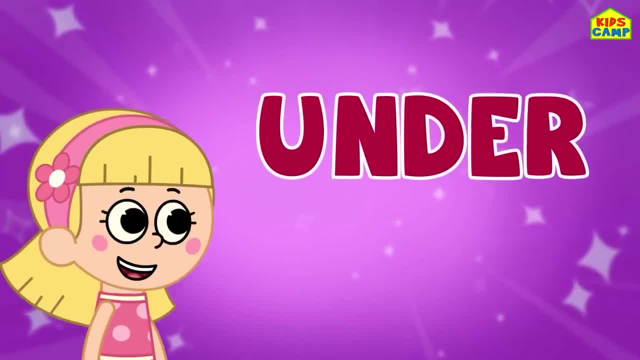 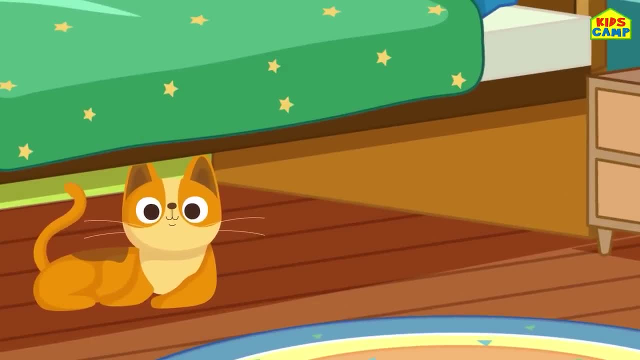 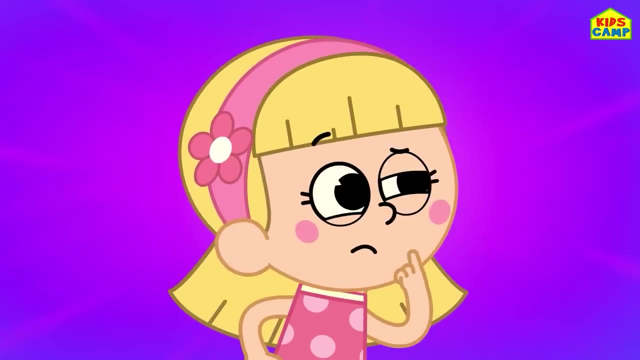 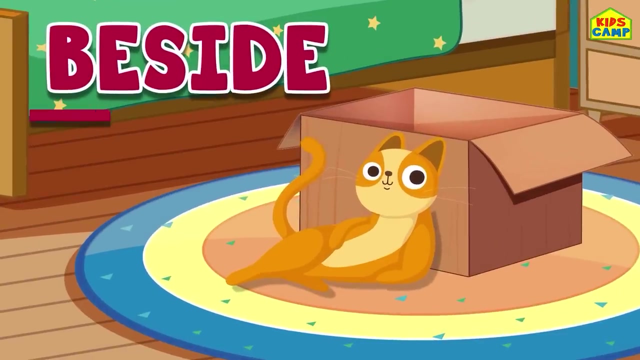 Next is UNDER Or beneath. The cat is under the bed. There she is. We found her. Good job, friends. Where is the cat now? The cat is besides the box. She's beside it, Right. Where is the cat now? 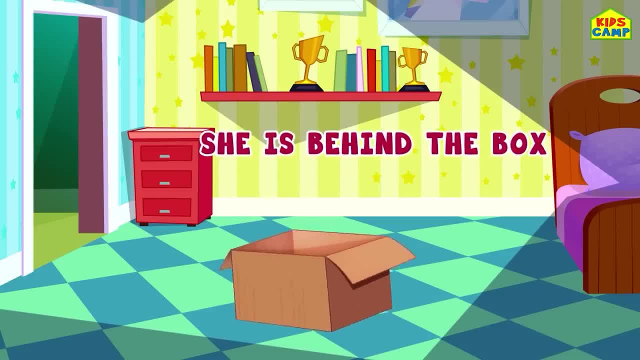 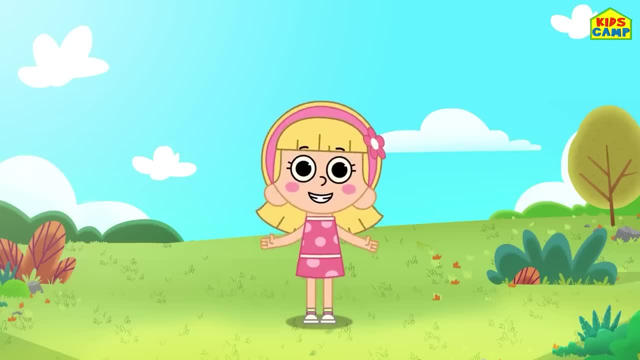 She is behind the box. There she is. She's behind the box. Yay, Yay, Yay, Yay. Come back for more games and keep watching Kids' Cam. Until then, bye-bye, Bye, Bye. 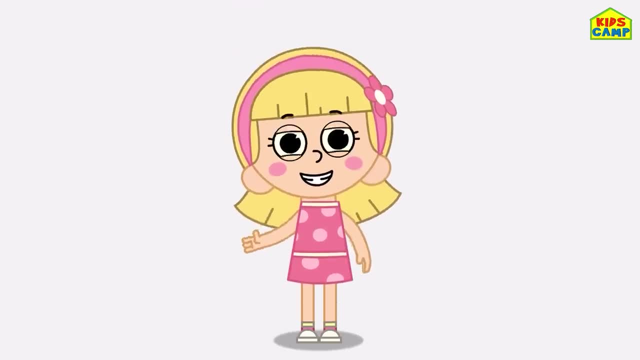 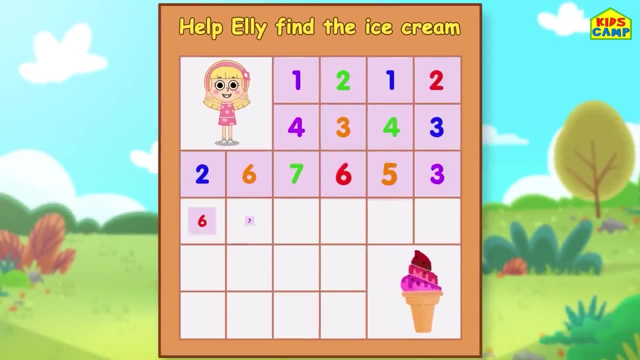 Hi friends, I am Ellie. Would you like to help me reach the ice-cream? Yes, Then let's get started with this amazing number maze. Let's get started. Let's start with the number. start with the number one. yes, i'm on number one. let's go to the next number two. yay. 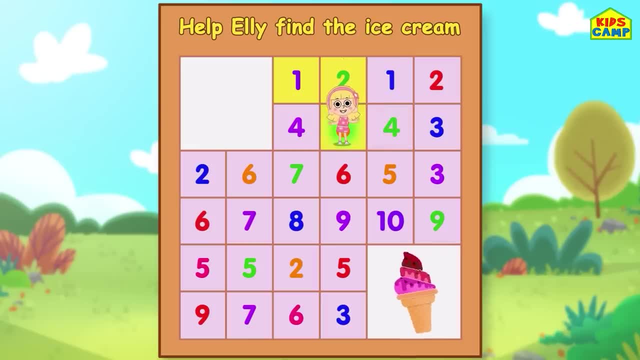 oh, that's not right. aha, that's right, that's three. let's go to the next one, number four. yay, aha, number five. good job friends. oops, that's not right. the next number is six. that's right, wonderful. next seven, we're almost there. and eight, yay. 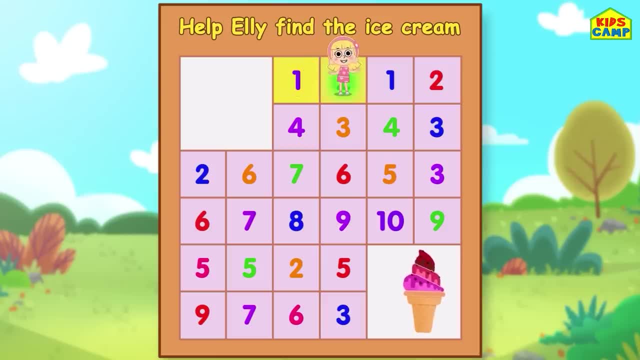 Let's go to the next number Two. Yay, Oh, that's not right. Aha, That's right. That's three. Let's go to the next one, Number four. Yay, Aha, Number five: 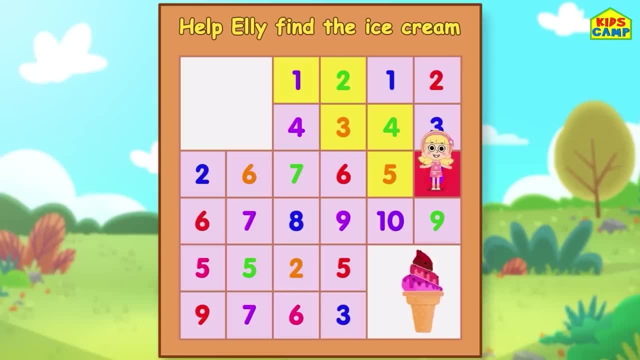 Good job, friends. Oops, That's not right. The next number is six, That's right, Wonderful. Next Seven, We're almost there. And eight, Yay, Uh-oh. No, That's right. Nine: 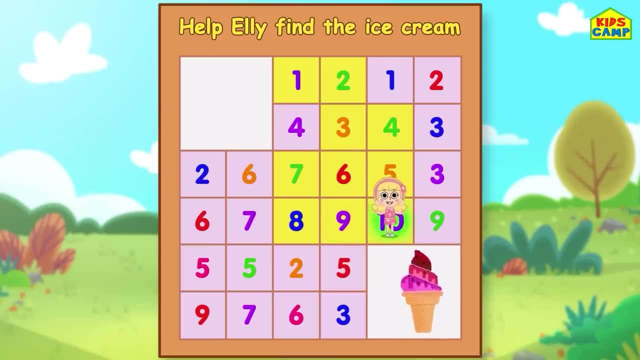 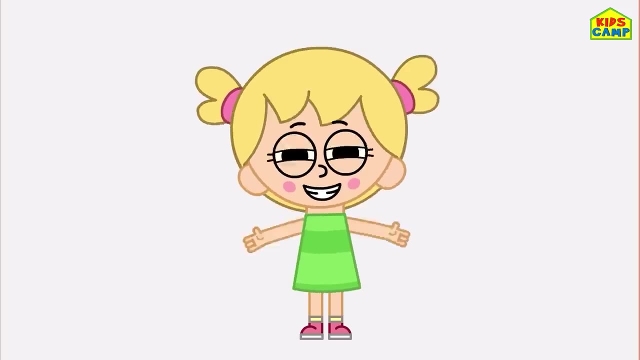 And ten: Yay, We did it. You helped me reach the ice cream, Thank you. Oh, it's Eva's turn now. Can you help her reach the donuts? Let's get started. Yay, Let's start with number one. 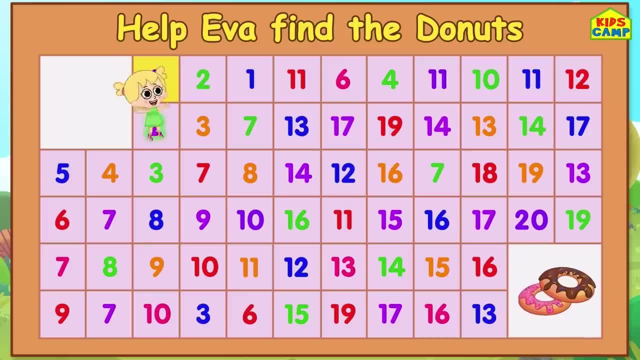 One, Two, Three, Good Four, Uh-oh, No, no, no, That's right. Number five, Good Six, Keep going. Seven, Eight, Yay, Oops, That's not right, That's right Nine. 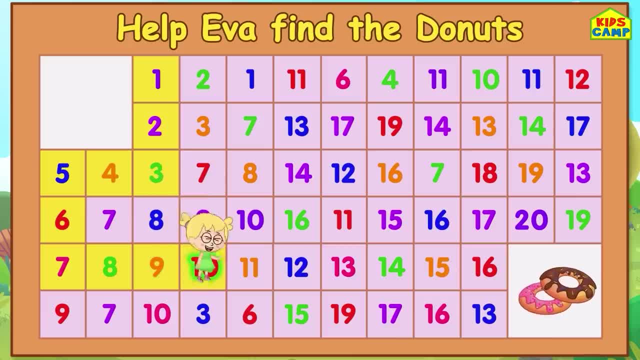 And ten, Eleven, Keep going. Yay, We're on twelve. What comes after twelve? Uh-oh, No, not that one, That's right. Thirteen And fourteen. Next is fifteen, Only five more to go. 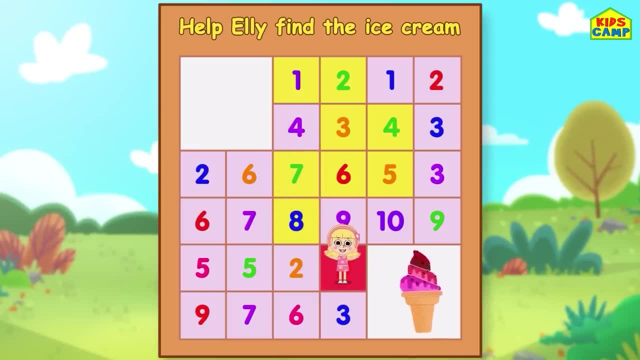 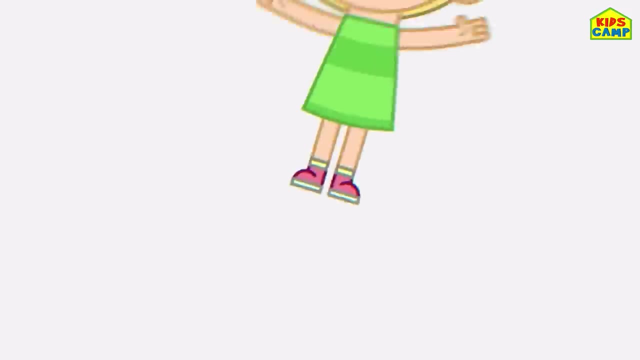 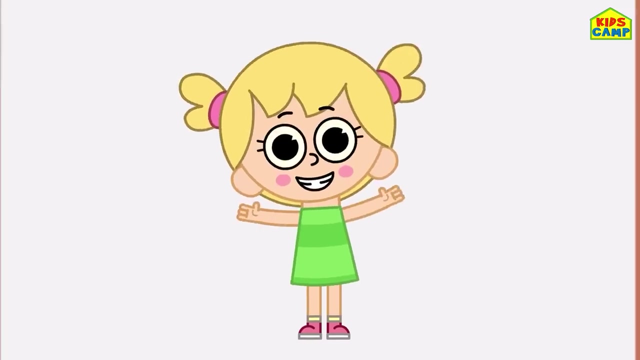 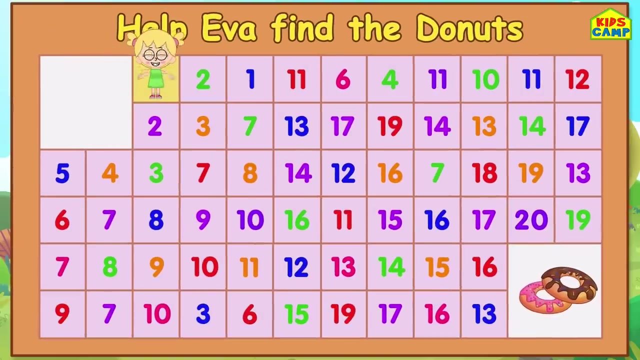 oh no, that's right. nine and ten. yay, we did it. you helped me reach the ice cream, thank you. oh, it's eva's turn now. can you help her reach the donuts? let's get started. yay, let's start with number one. one, two: three: good four. oh no, no, no, that's right. number five: good six. keep going seven. 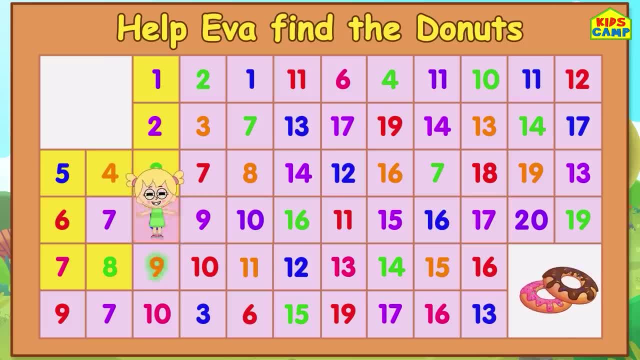 eight. yay, oops, that's not right, that's right. nine and ten eleven: keep going. yay, we're on 12.. what comes after 12.? oh, no, not that one, that's right. 13 and 14.. next is 15.. only five more to go. 16.. 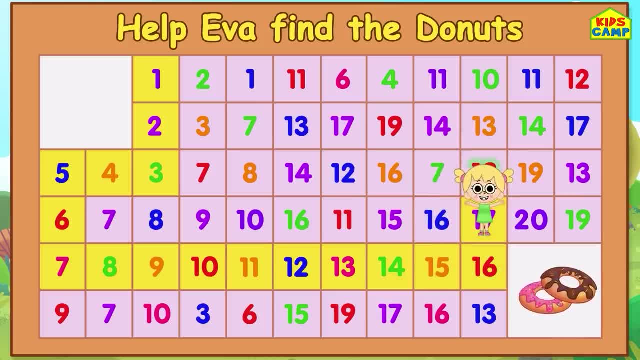 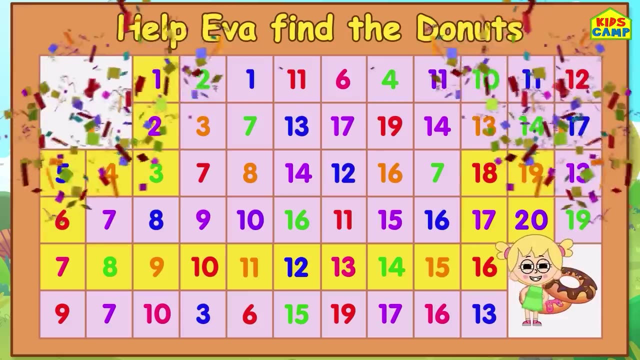 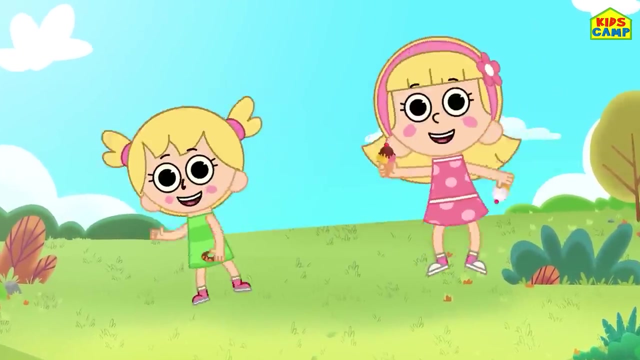 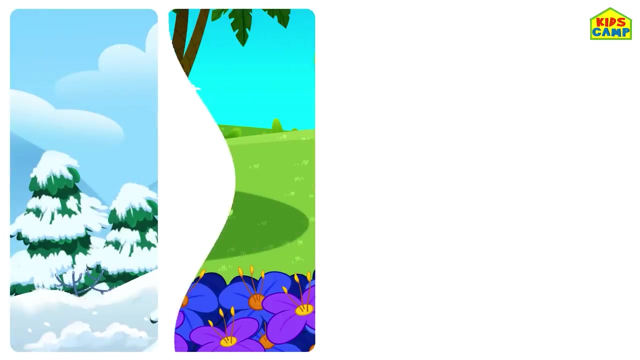 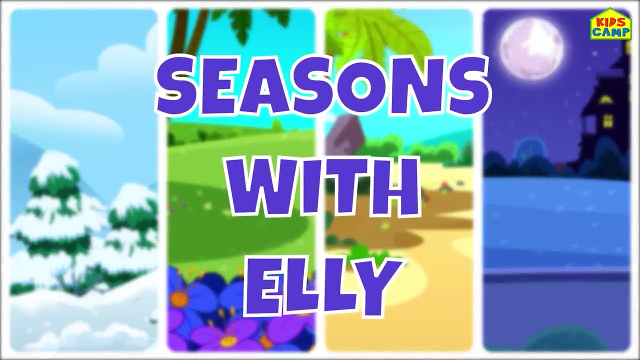 that's right. 17.. next is 19.. that's right, 19. we're almost there. and 20.. that's right. we did it. we helped eva find the donuts. Good job, friends. Bye Seasons with Elli. What season is this? 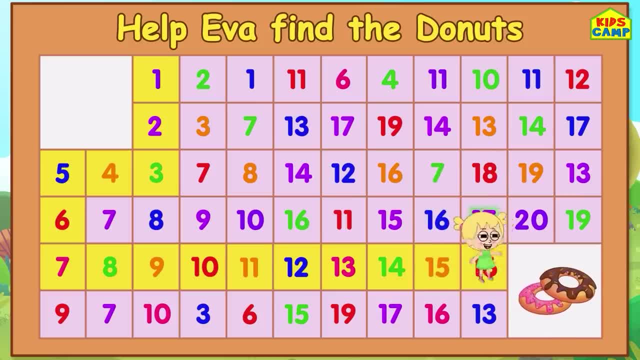 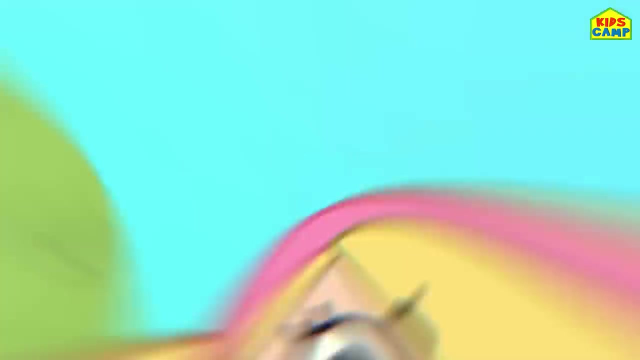 Sixteen, That's right. Seventeen. Next is eighteen, That's right. Nineteen, We're almost there. And twenty, That's right. We did it. Woo-hoo, We helped Eva find the donuts. Good job, friends. 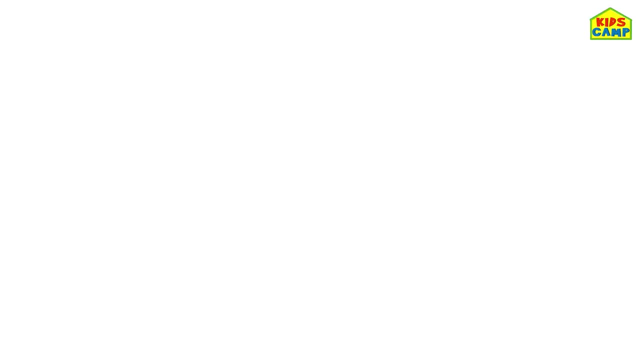 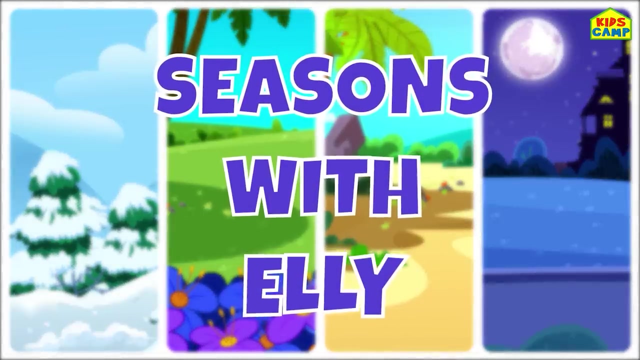 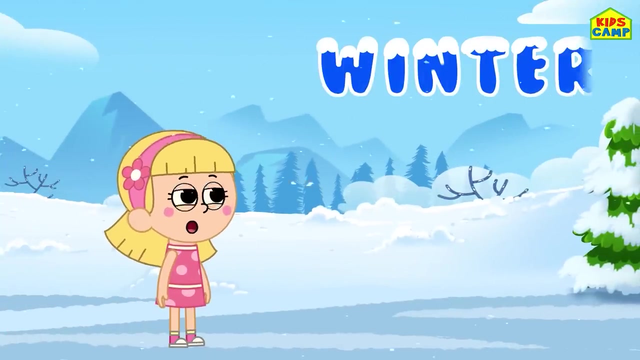 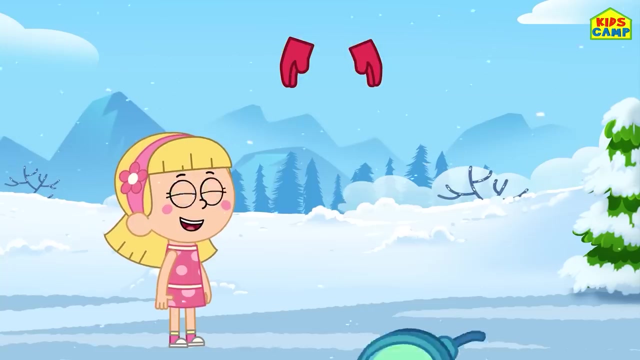 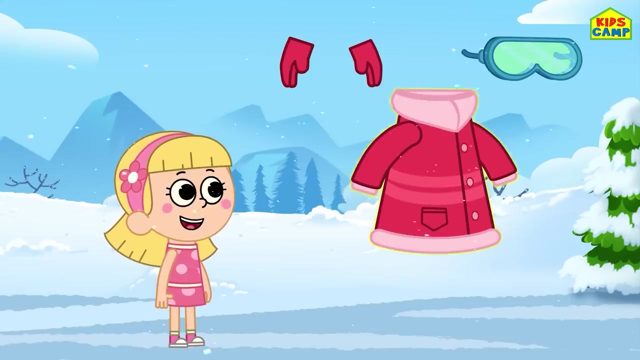 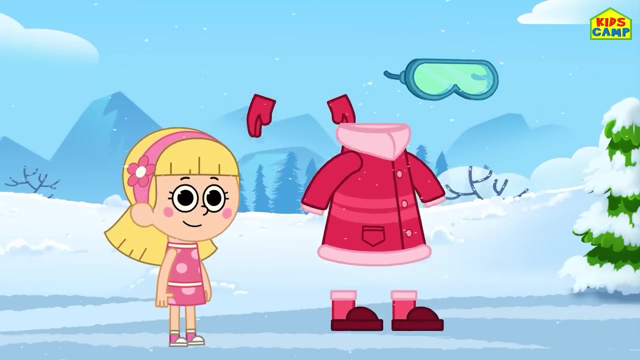 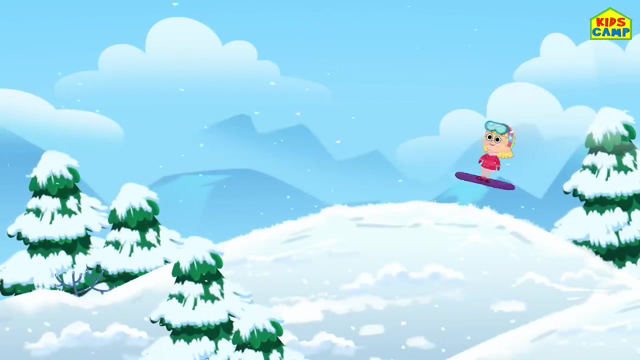 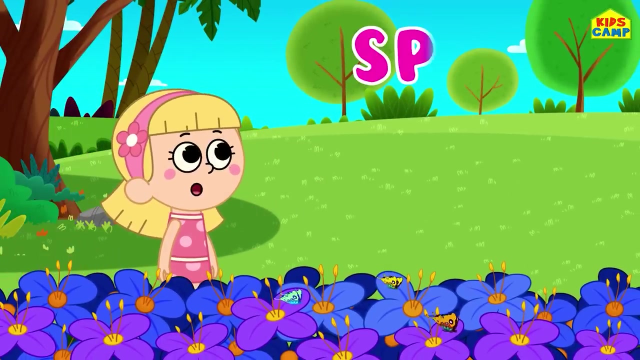 Bye Seasons with Ellie. What season is this? Winter Gloves, Snow goggles, Coat, Boots, Yay, Yay, Whee, Woo-hoo. What season is this? What season is this? What season is this? It's spring. 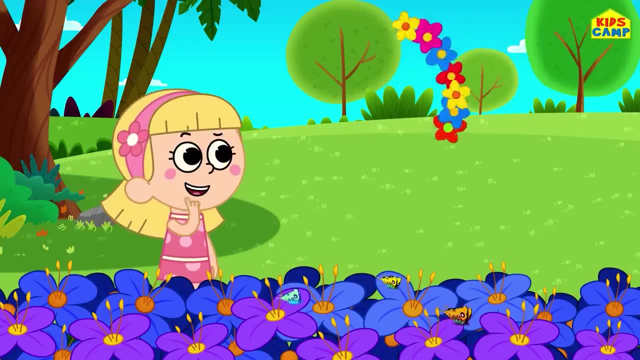 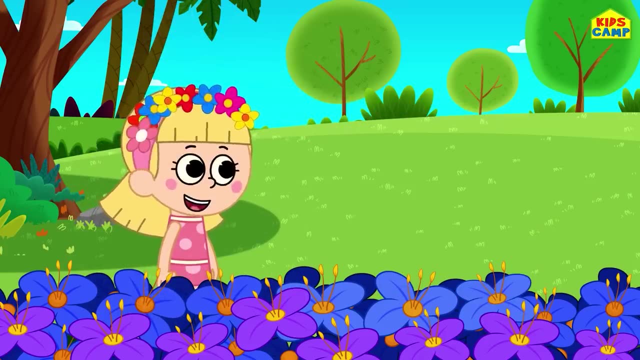 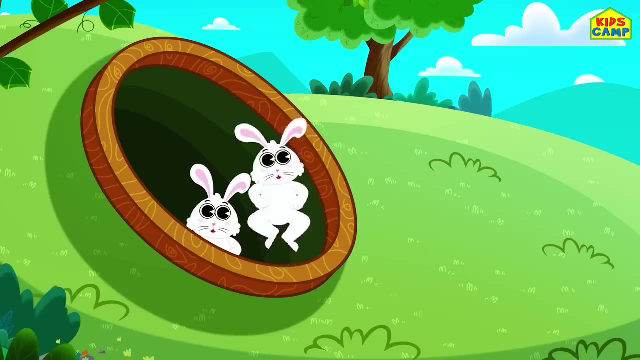 It's spring. Flower headband, Flower headband, Flower headband. Wow, Look at the flowers bloom. Look at the flowers bloom And the birds sing. The bunnies have come out to play And the sun is shining bright. 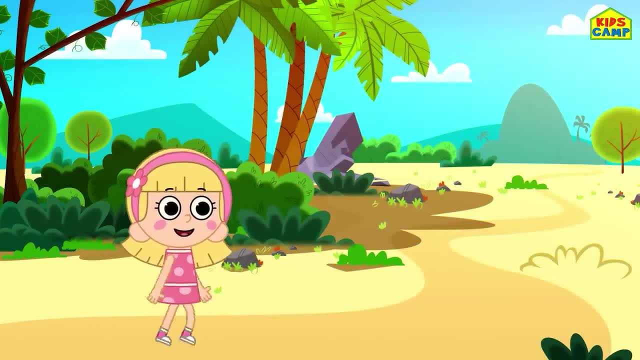 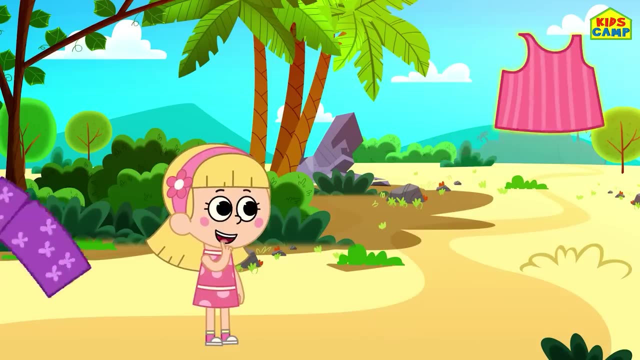 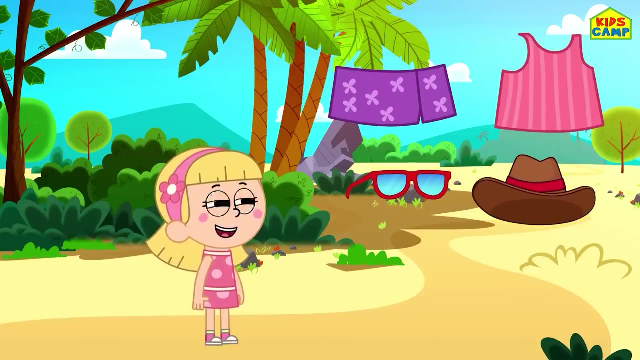 And the sun is shining bright. What season is this? It's summer. It's summer. Swimsuit, Sarong, Sunglasses, Hat, Yay, We're ready to go to the beach. We're ready to go to the beach. 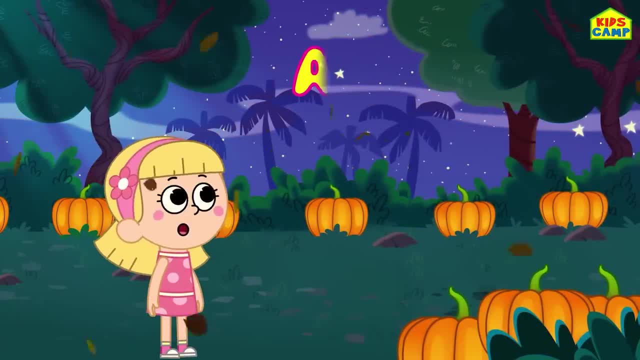 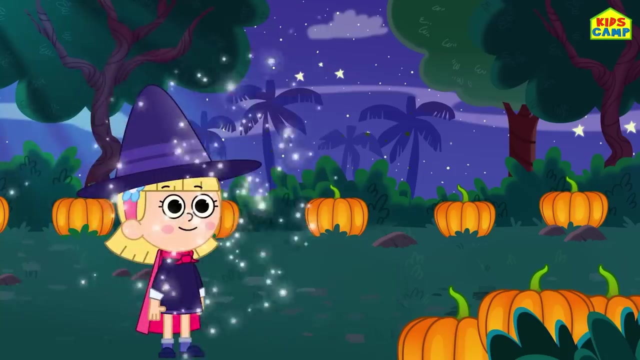 Ooh, It's nearly Halloween. That means it's autumn. That means it's autumn- A witch's hat, A witch's hat, A dress with a cloak And witch's shoes. Yay, I'm a witch. Today. we learned our seasons. 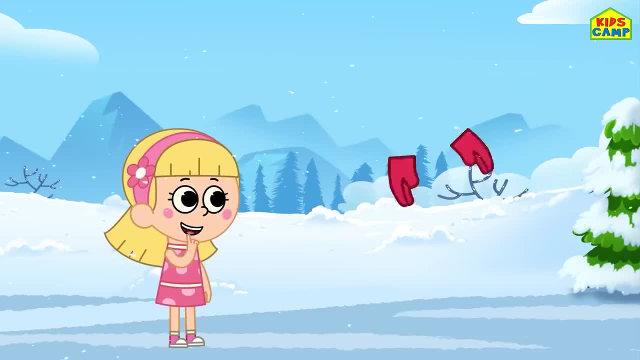 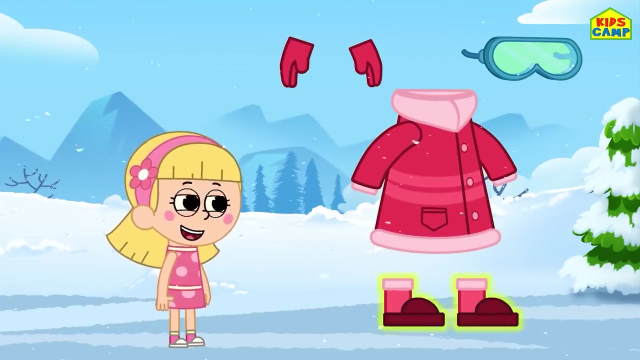 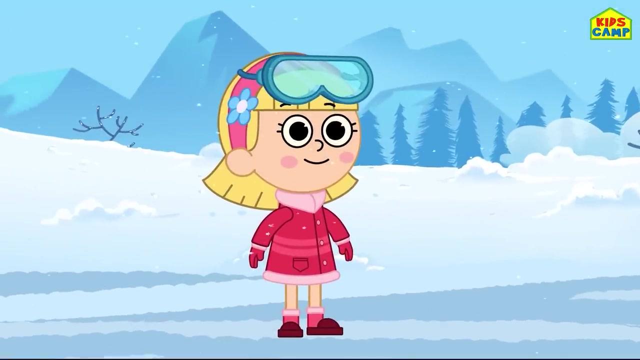 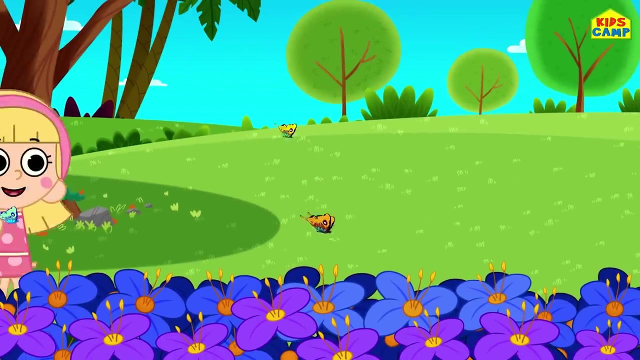 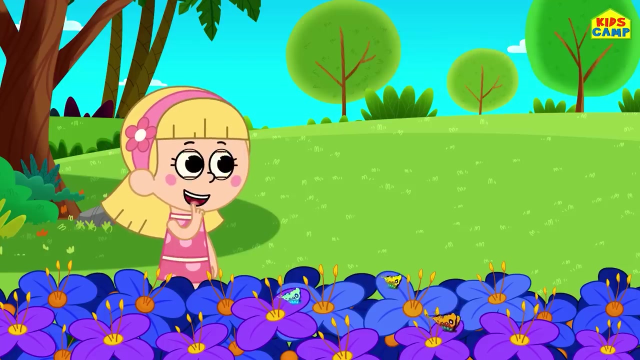 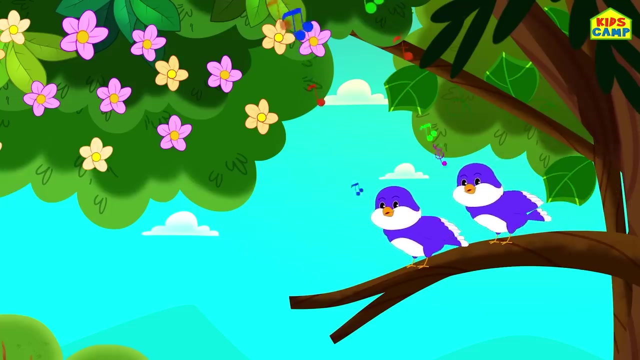 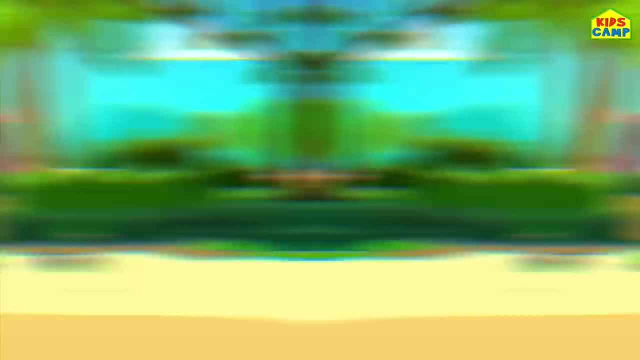 Winter Gloves, Snow goggles, Coat, Boots. Yay, What season is this? It's spring, Flower headband. Wow, Look at, the flowers bloom And the birds sing. The bunnies have come out to play and the sun is shining bright. What season is this? 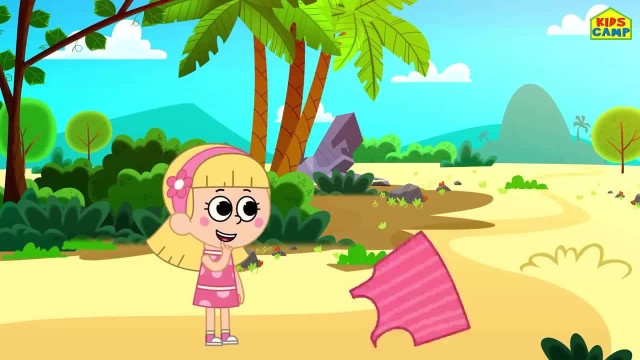 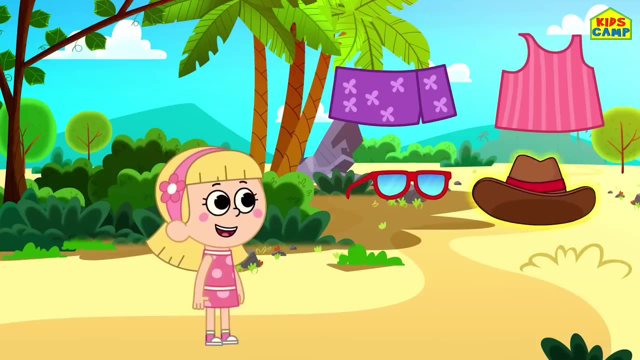 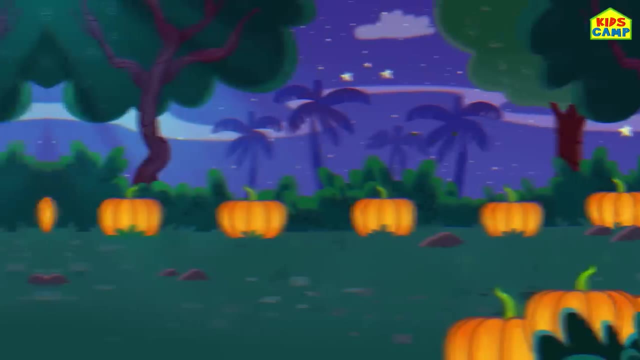 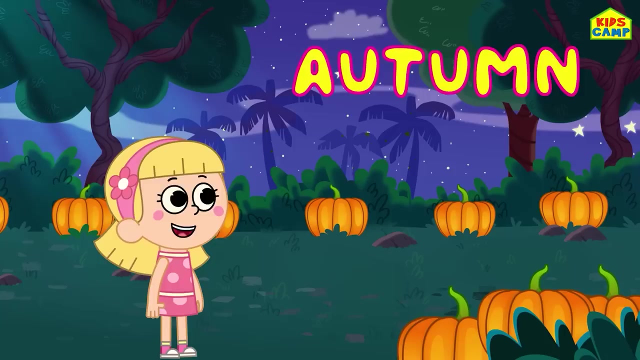 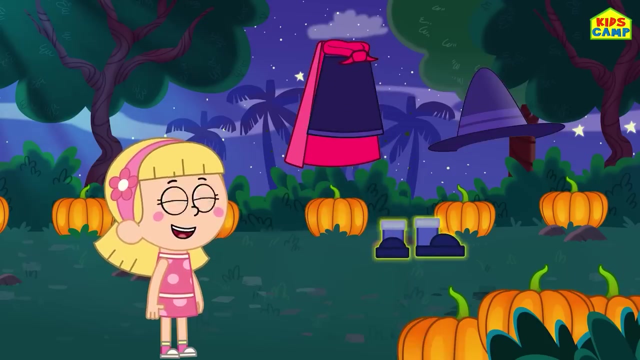 It's summer: Swimsuit, Sarong, Sunglasses, Hat- Yay, We're ready to go to the beach. Oooh, It's nearly Halloween. That means it's autumn. A witch's hat, A dress with a cloak And witch's shoes. 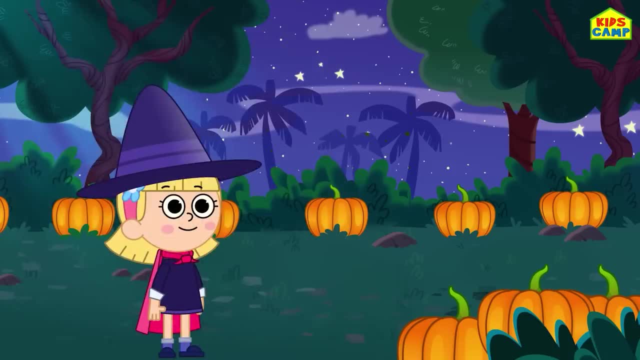 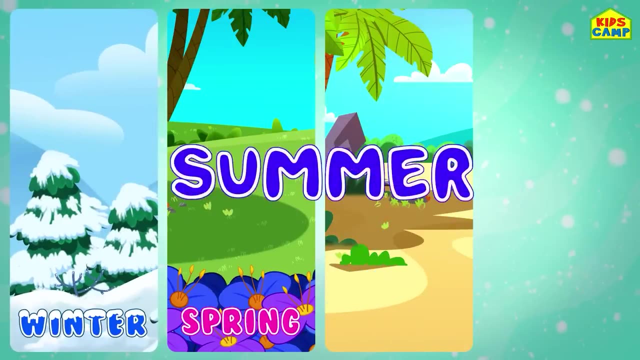 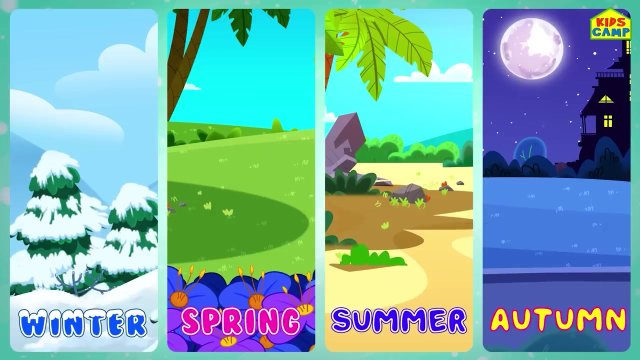 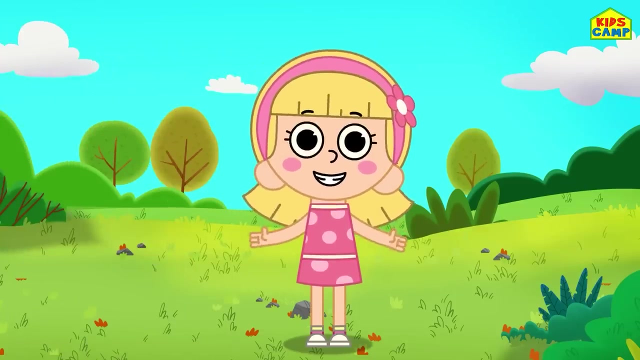 Yay, I'm a witch. Today we learned our seasons: Winter, Spring, Summer And Autumn. Woohoo, Hi friends, I'm Elli, And today we are going to build a house. Excited So am I. Let's go. 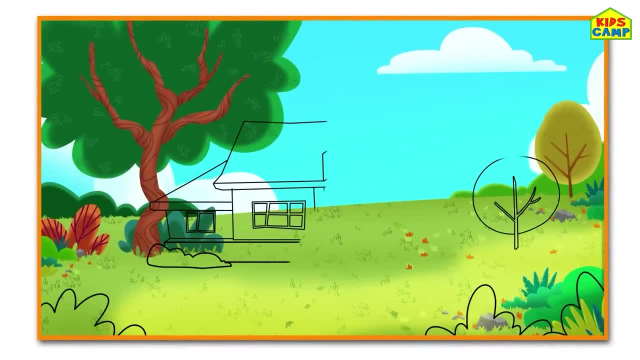 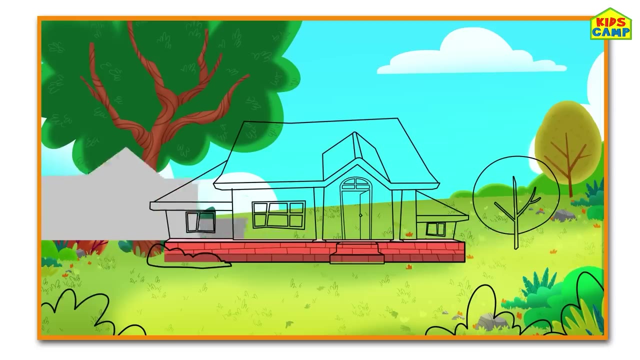 Oooh, That's the outline. Let's fit the different parts of the house right there. Let's figure out what goes where. First, the foundation, The base. Wow, That was easy. Now let's add the walls. Shhhh. 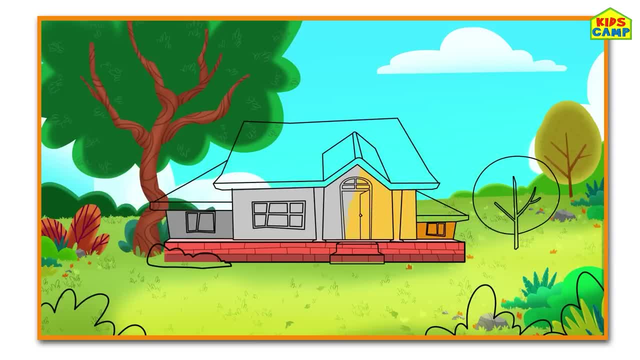 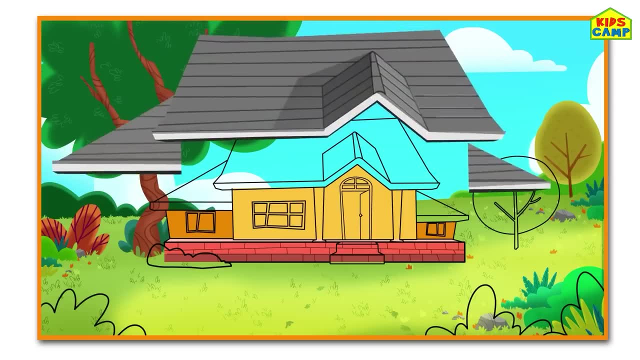 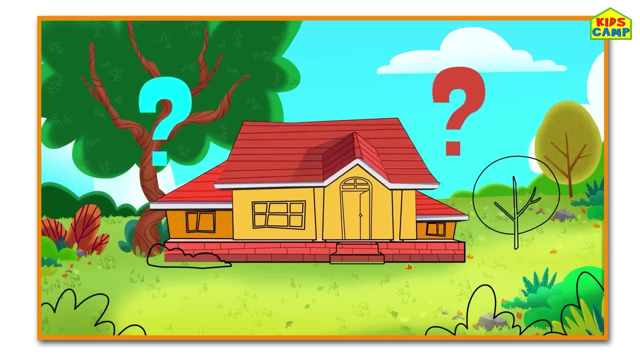 I love yellow paint on my walls. This looks great. Next, let's add the roof. Shhhh, Perfect. It's starting to look like a house. What's missing, That's right A door, Yes, And lovely windows to look outside. 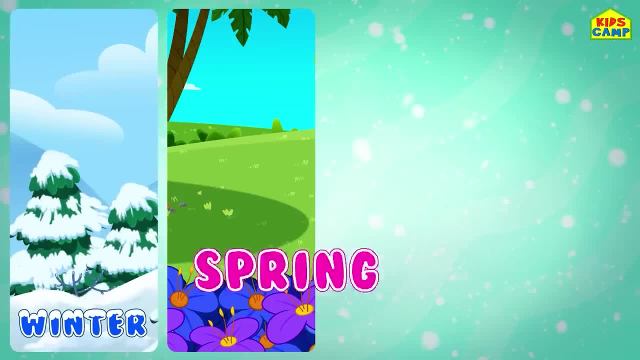 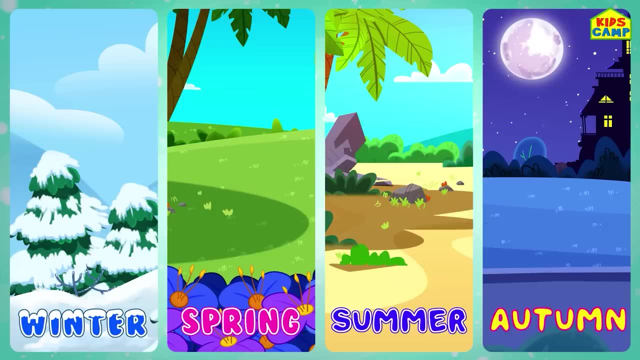 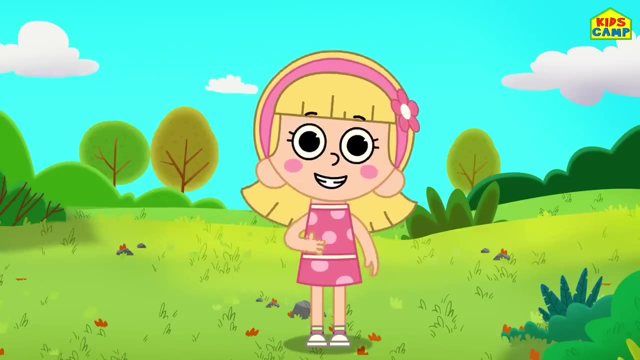 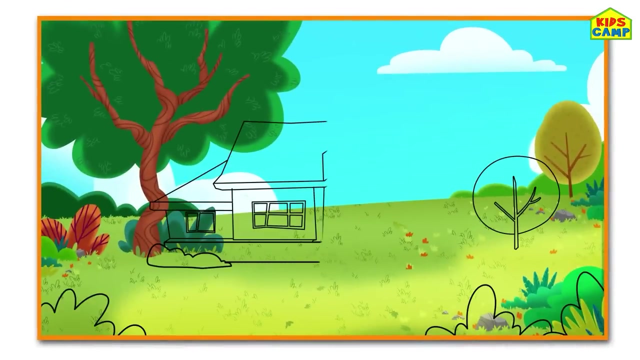 Today we learned our seasons: Winter, Spring, Summer And autumn. Woohoo, Hi friends, I'm Elli And today we're going to build a house. Excited So am I. Let's go. Ooh, That's the outline. 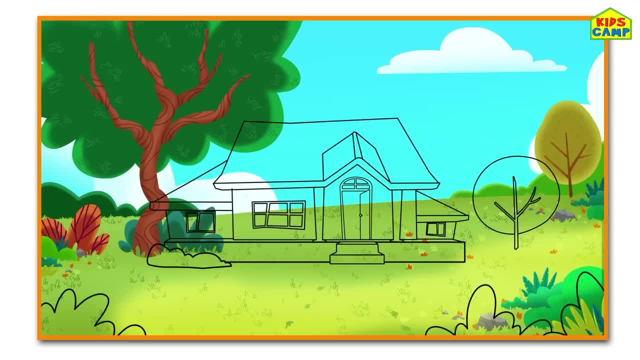 Let's fit the different parts of the house right there And figure out what goes where. First, the foundation, The base. Wow, That was easy. Now let's add the walls. Now let's add the walls. I love yellow paint on my walls. 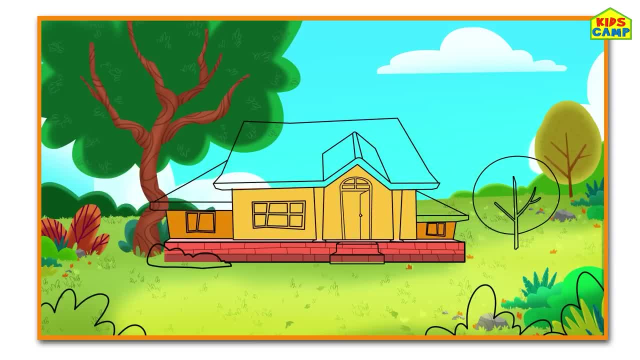 I love yellow paint on my walls. This looks great. Next, let's add the roof. Next, let's add the roof. Perfect, It's starting to look like a house. It's starting to look like a house. What's missing, That's right, A door. 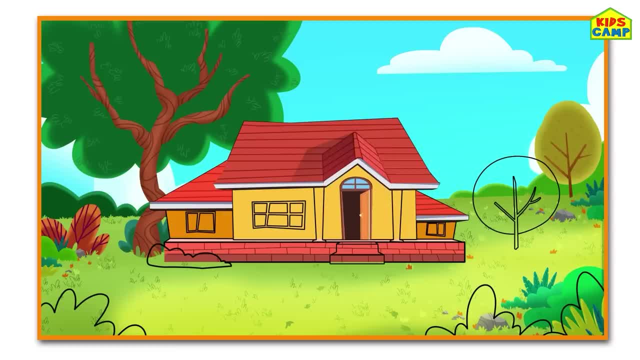 Yes, And lovely windows to look outside, And lovely windows to look outside And for sunshine to come in, And for sunshine to come in. Next we need steps, Next we need steps. Perfect, And now let's add the pillars. Going good. 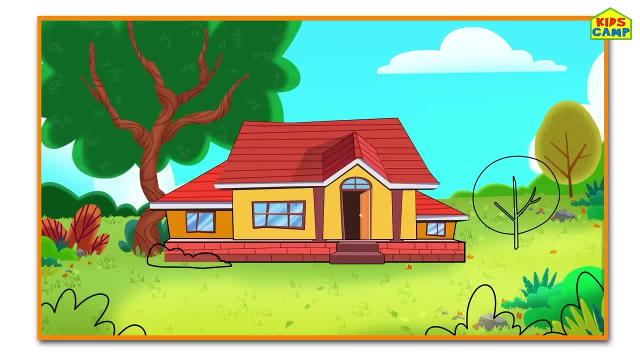 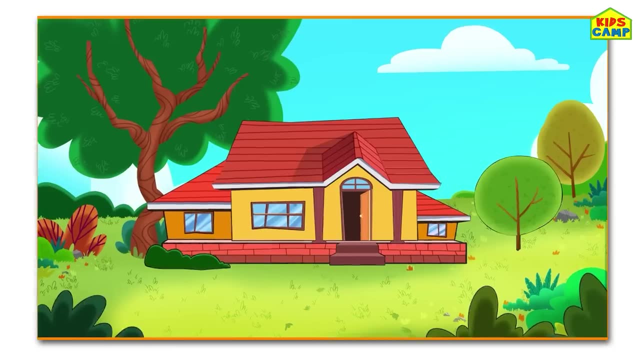 This is such a beautiful house, But what else is missing? Let's add color to my garden. Let's add color to my garden. Let's add color to my garden. Wow, It looks beautiful. Wow, It looks beautiful. That's my house. 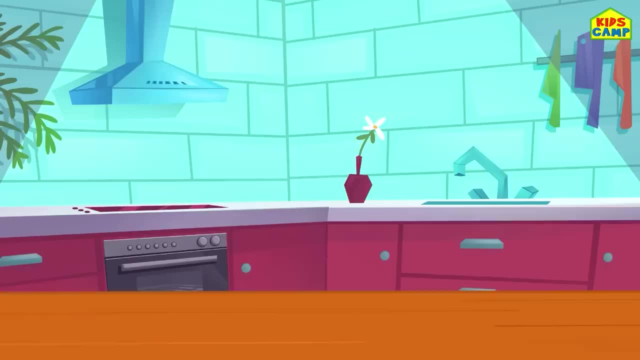 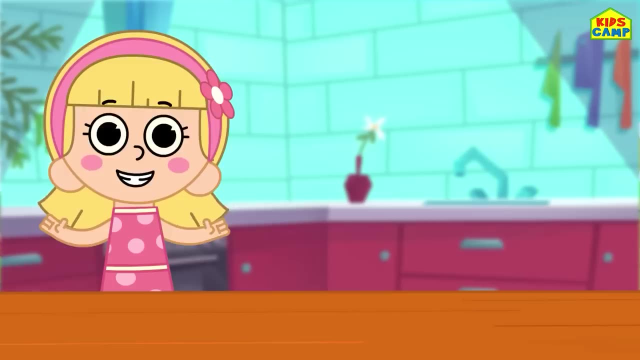 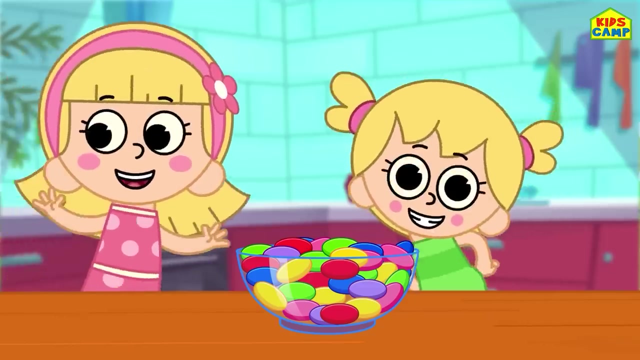 Okay, friends, I'm going home. See you. Bye, Hi friends. Hi friends, I'm Ellie and I love jelly beans, Don't you too? That's right, And this is Eva. We have to sort the jelly beans by their color. 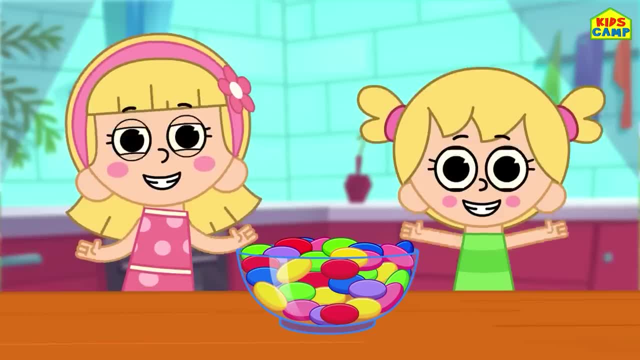 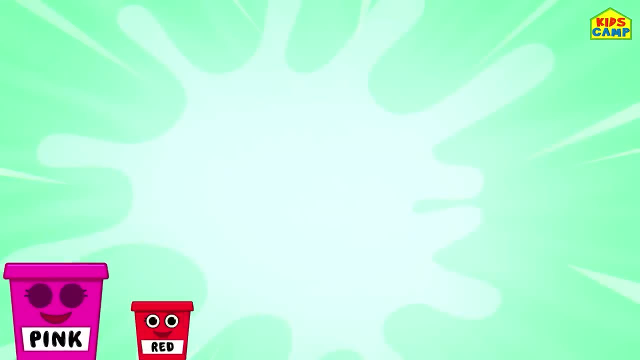 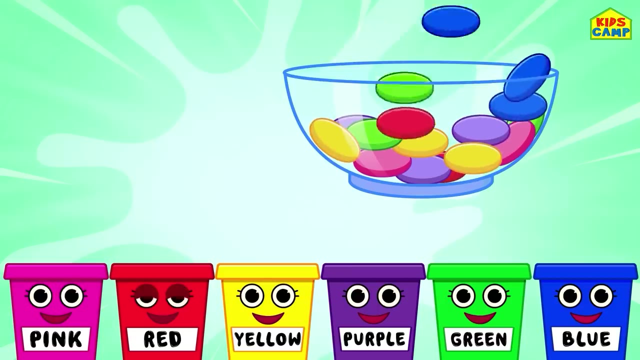 We have to sort the jelly beans by their color. Yay, Will you help us? Let's get started. Let's get started. Ooh Jelly beans, Ooh Jelly beans. Let's sort the pink jelly beans. Let's sort the pink jelly beans. 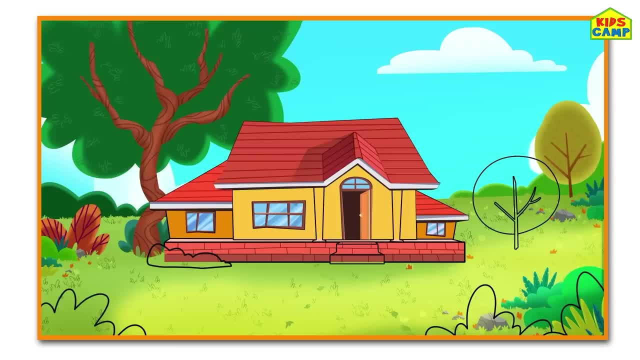 And for sunshine to come in. Next we need steps. Perfect, And now let's add the pillars. Going good, This is such a beautiful house, But what else is missing? Let's add color to my garden. Wow, It looks beautiful. 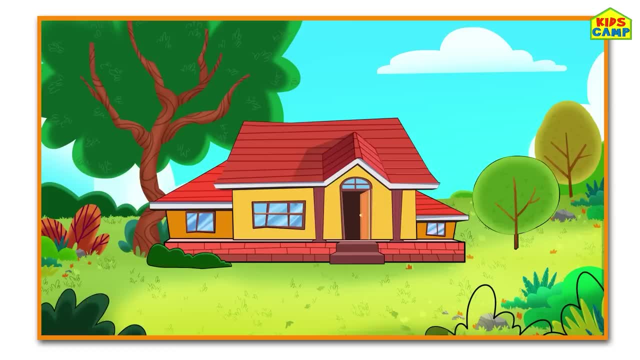 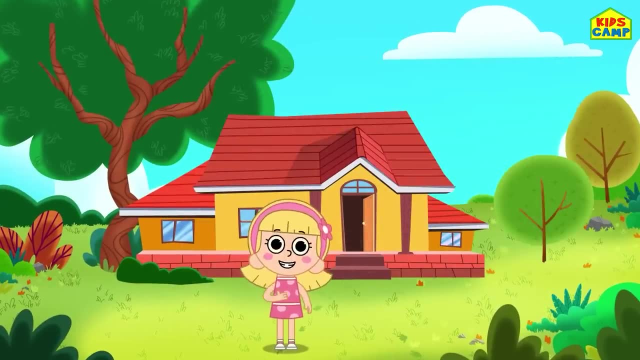 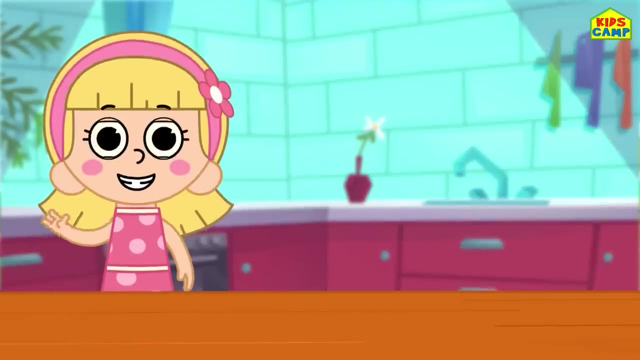 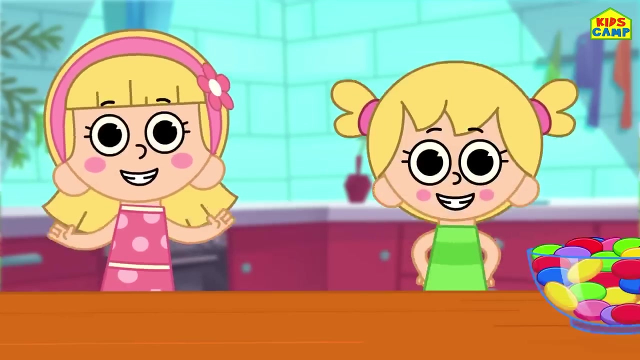 That's my house. Okay, friends, I'm going home. See you, Bye, Hi friends. I'm Ellie and I love jelly beans, Don't you too? That's right, And this is Eva. We have to sort the jelly beans by their color. 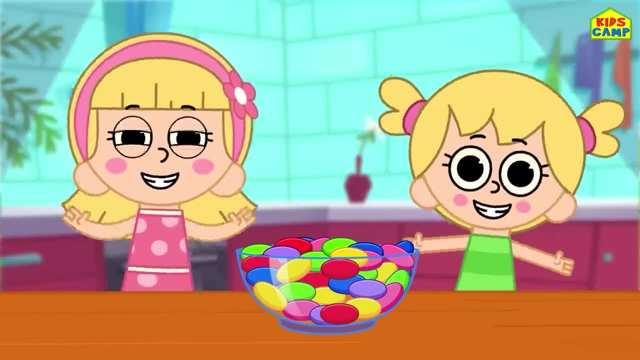 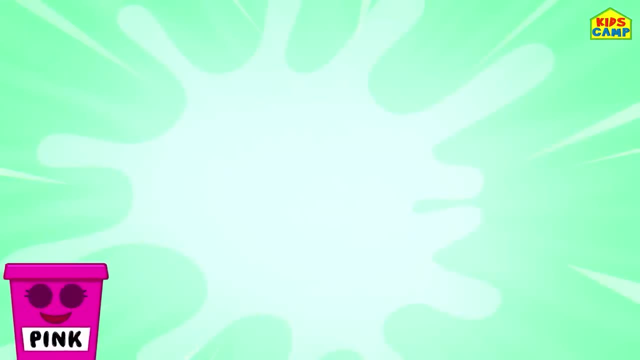 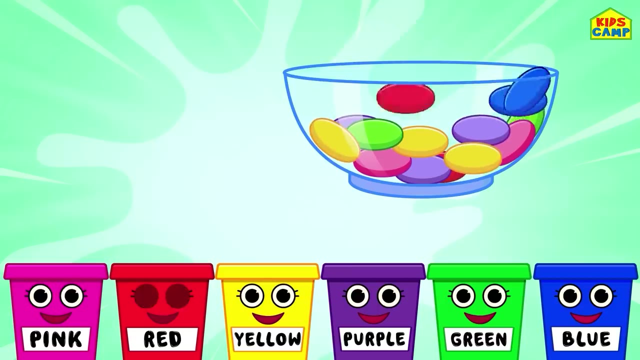 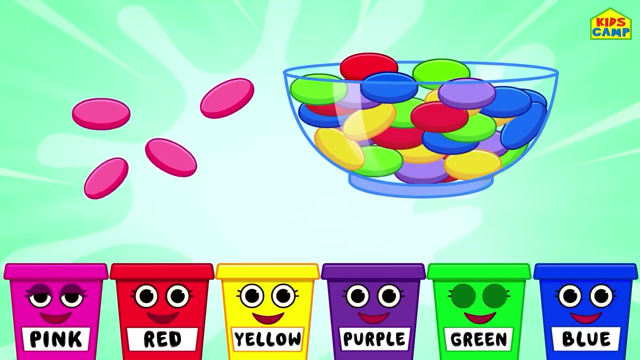 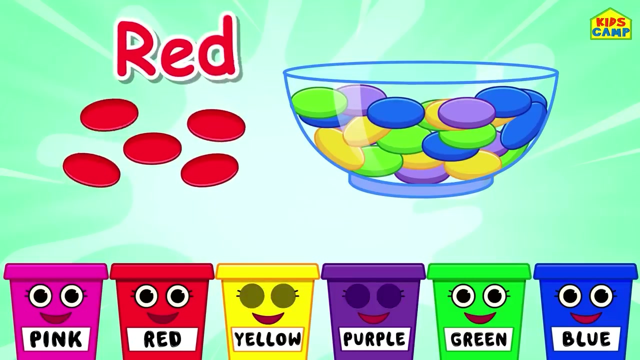 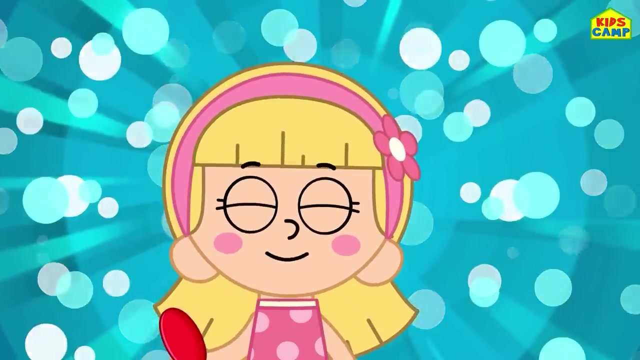 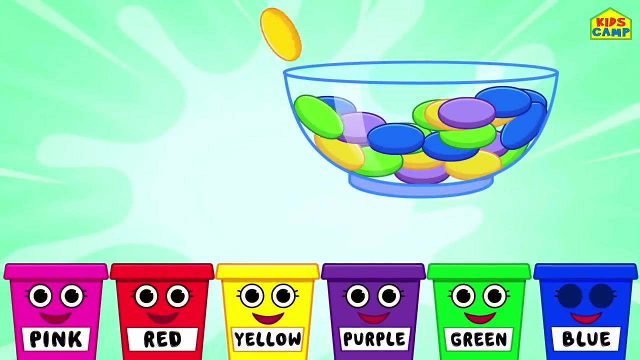 That's easy. Yay, Will you help us? Let's get started. Let's sort the pink jelly beans- Yummy. Into the pink bucket- Wonderful. Next up is red. Let's sort the red jelly beans Into the bucket- Yummy. Next up is the color yellow. Let's sort all the yellow jelly beans. 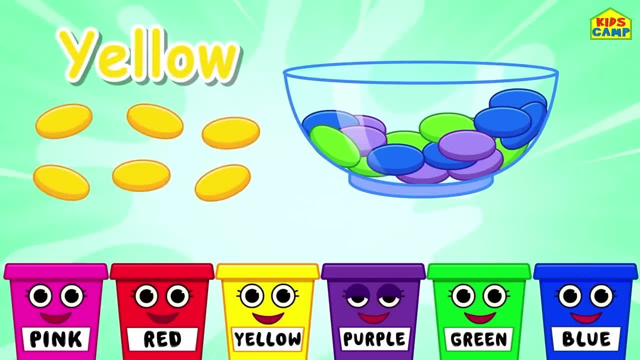 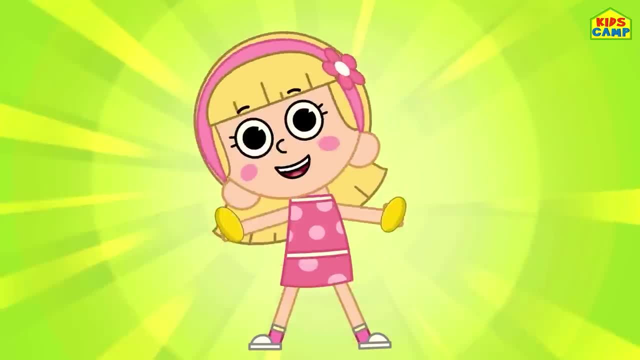 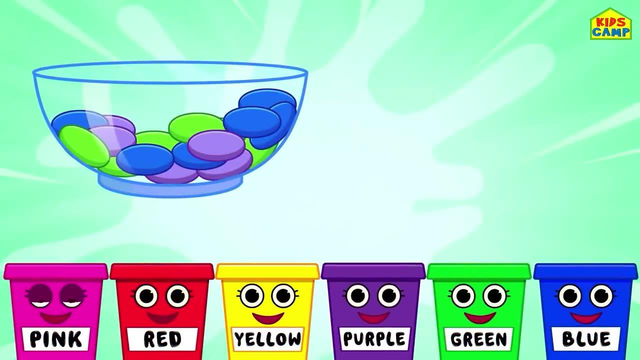 That's right Into the bucket- Wonderful. Next up is yellow. Let's sort the yellow jelly beans. Next up is yellow. Let's sort the yellow jelly beans- Wonderful, I love the yellow. Next up is purple. Look for all the purple jelly beans. Yes, that's right. 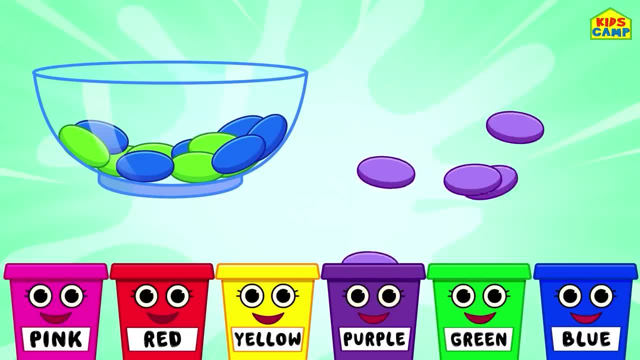 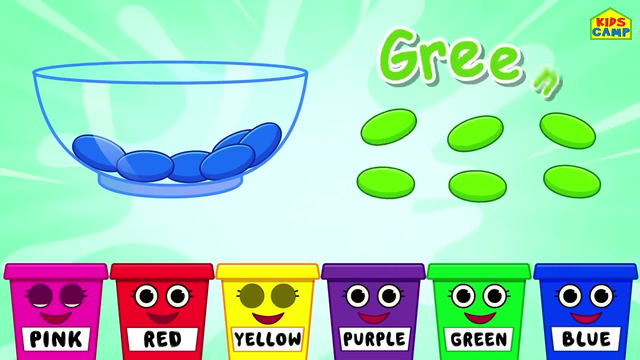 Into the bucket. Great job, friends, Wonderful. We all love jelly beans, don't we? Next up is green. Let's sort all the yellow jelly beans, Thank you, Yeah, the green jelly beans. Yummy Into the bucket. Wonderful, Yummy. And the last one is blue. 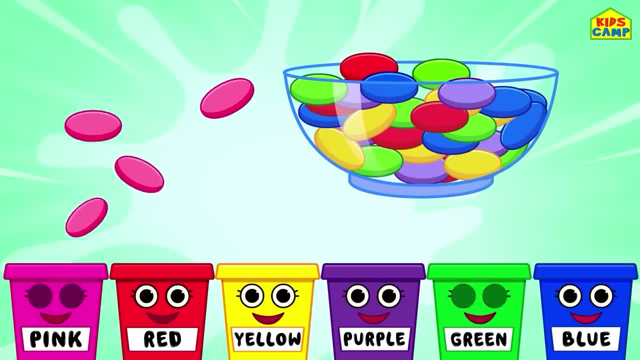 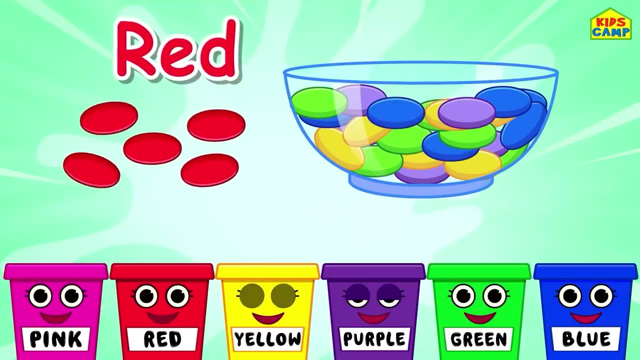 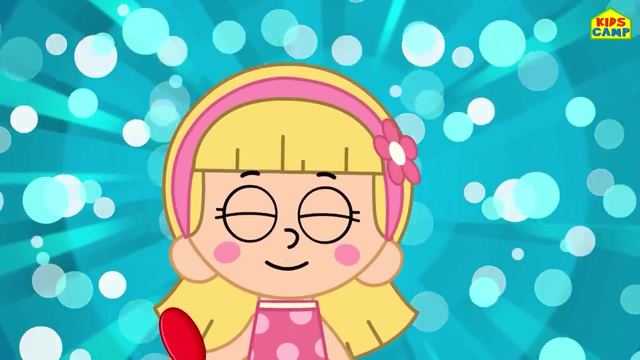 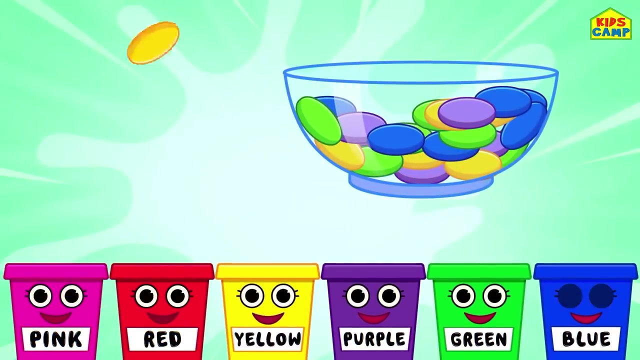 Yummy Into the pink bucket. Wonderful, Yay, Yay. Next up is red. Let's sort the red jelly beans. Woohoo Into the bucket, Yummy. Next up is the color yellow. Yummy, Let's sort all the yellow jelly beans. 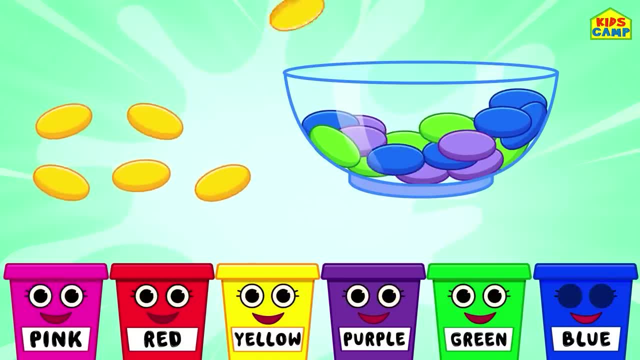 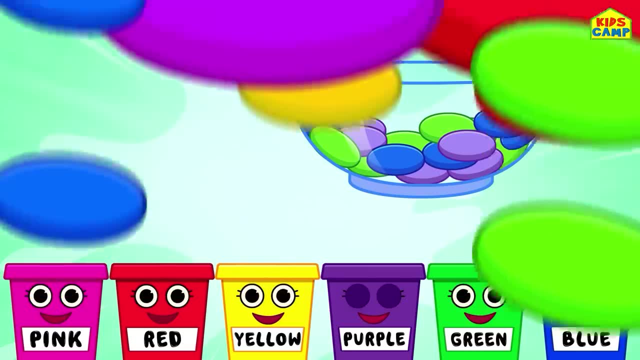 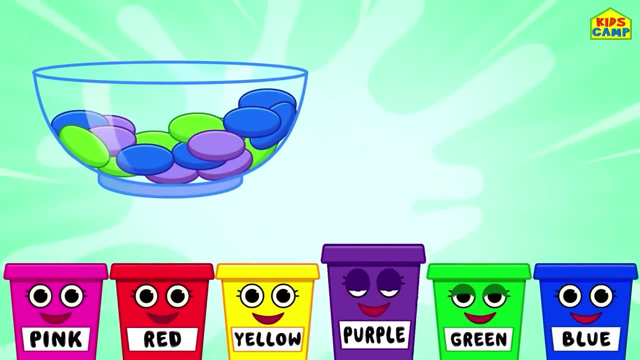 Let's sort all the yellow jelly beans. That's right. That's right Into the bucket. Into the bucket. Wonderful, I love yellow. I love yellow. Next is purple. Look for all the purple jelly beans. Look for all the purple jelly beans. 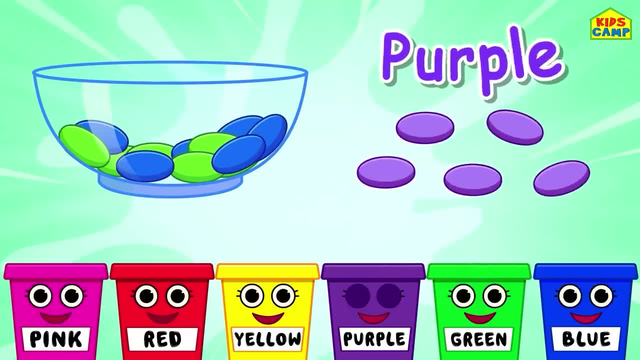 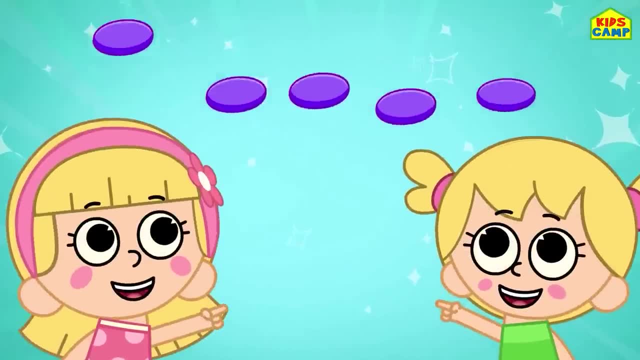 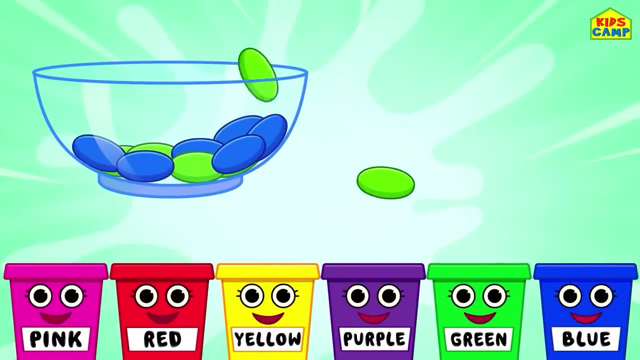 Yes, That's right Into the bucket. Great job, friends. Wonderful. We all love jelly beans, don't we? Next is green. Let's sort all the green jelly beans. Let's sort all the green jelly beans- Yummy. 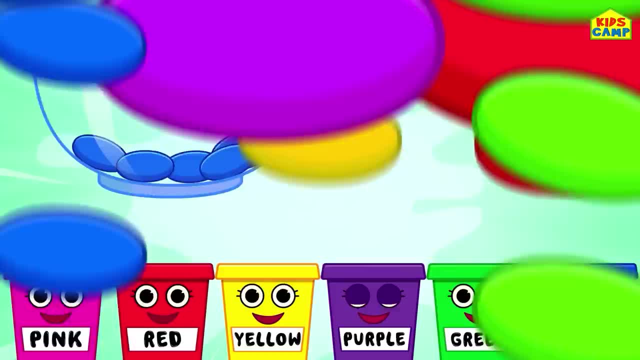 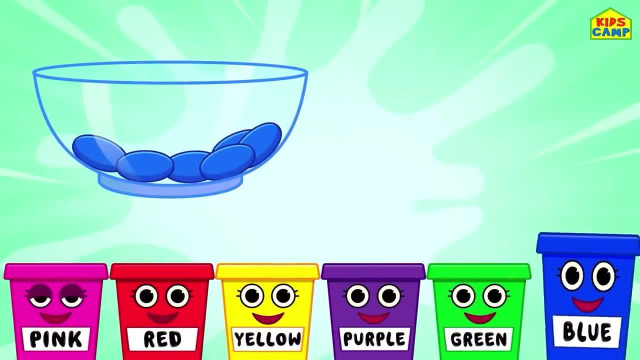 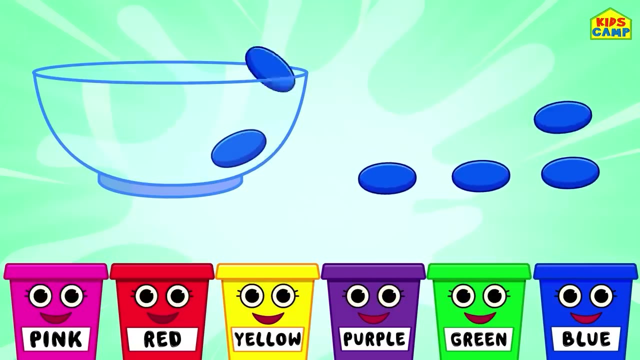 Into the bucket. Wonderful, Yummy, Yummy. And the last one is blue. That's right. We have only the blue jelly beans remaining. That's right Into the blue bucket And we're done. Good job, friends. 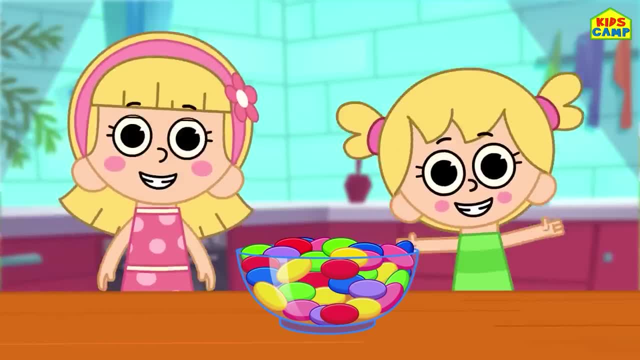 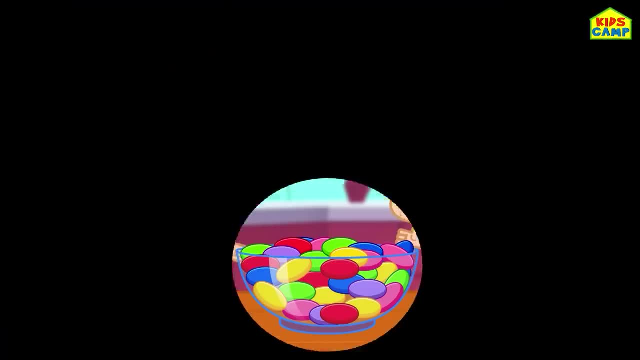 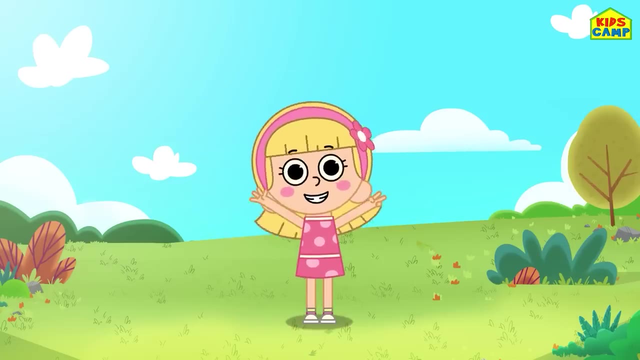 That was such a fun time sorting the jelly beans. Come back for more on Kids' Game. See you soon. Bye-bye, Hi everyone. What a beautiful day. I'm Ellie And we are going to play a new game called. 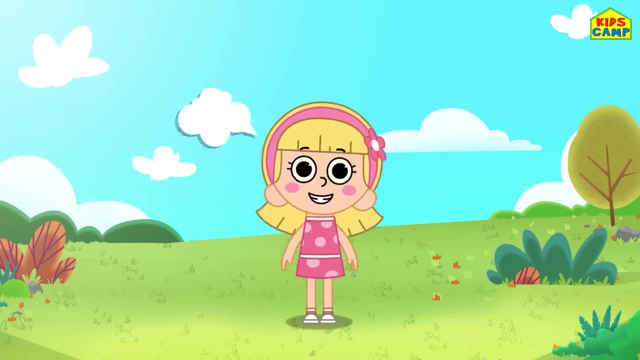 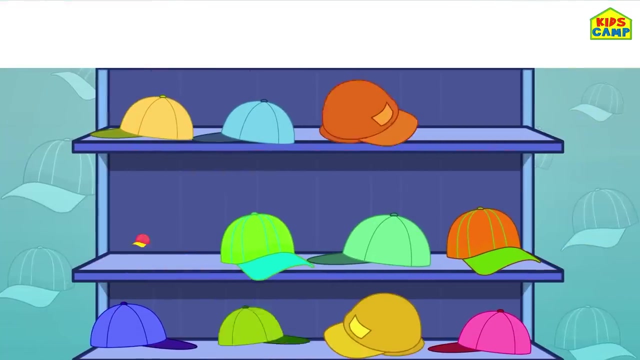 Find the Matching Pear. That's right. We have to find two similar objects and that's the game. That's simple, Ready, Let's get started. Find the Matching Pear, Find the Matching Pear, Find the Matching Pear. Can you spot two? 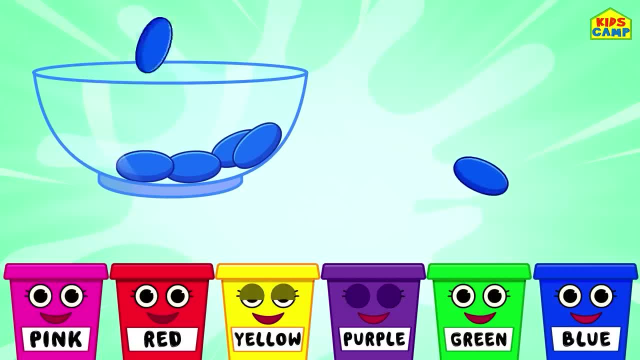 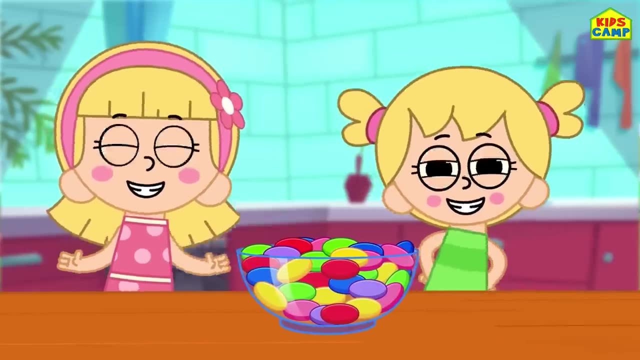 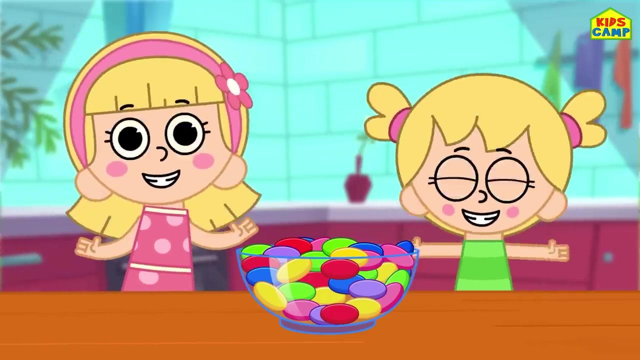 That's right. We have only the blue jelly beans remaining. That's right Into the blue bucket And we're done. Good job, friends. That was such a fun time sorting the jelly beans. Come back for more on Kids' Camp. See you soon. Bye-bye. 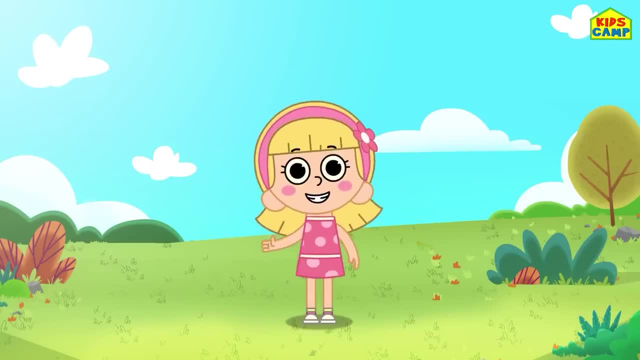 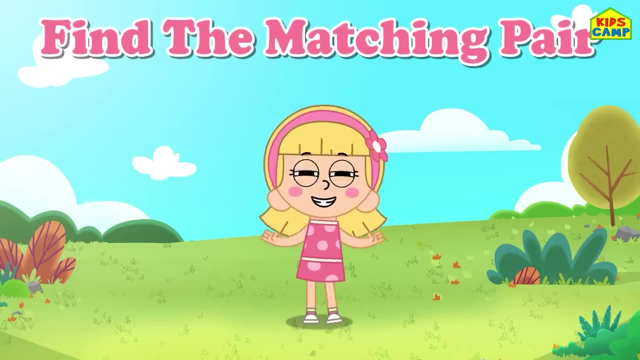 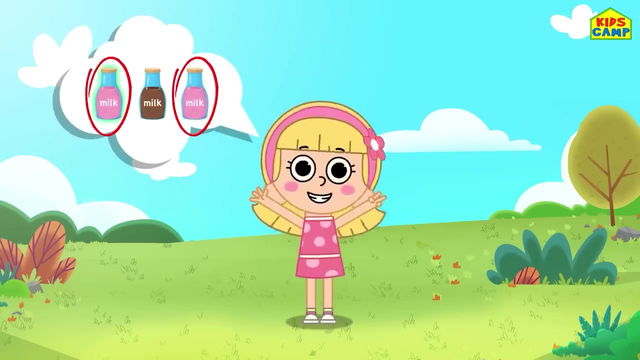 Hi everyone, What a beautiful day. I'm Ellie And we are going to play a new game called Find the Matching Pair. That's right, We have to find two similar objects and that's the game. That's simple, Ready, Let's get started. 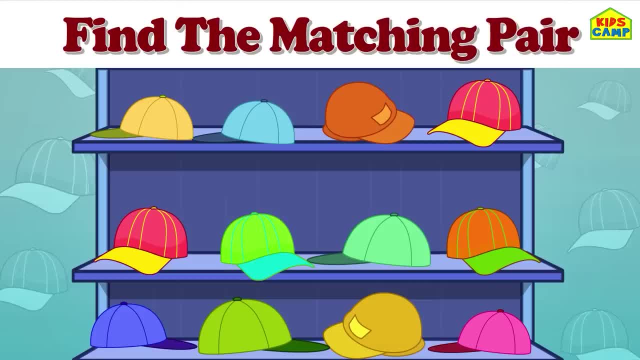 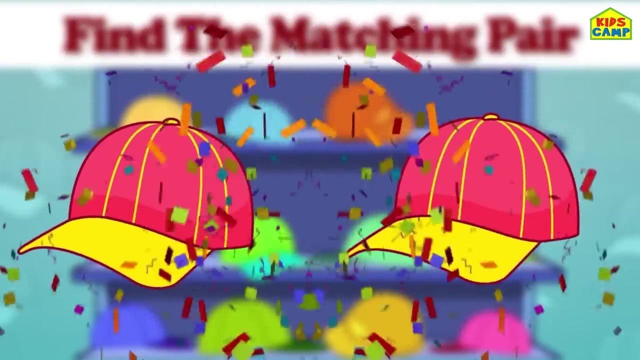 Find the Matching Pair. Can you spot two identical caps? No, they're not identical. No, Yes, Yay, We found them. They are two identical caps. Good job, Good job, Let's find another pair. Find the matching rockets. 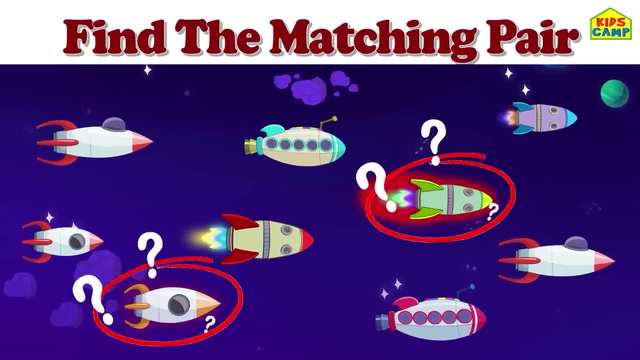 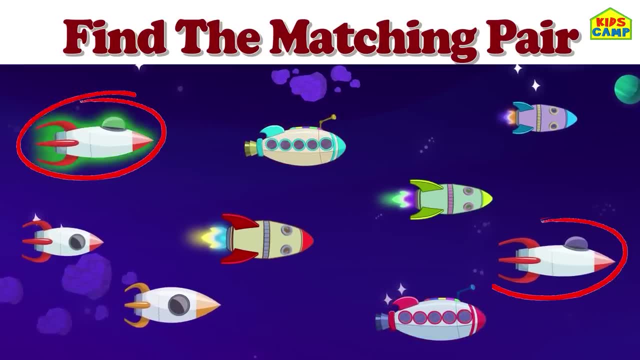 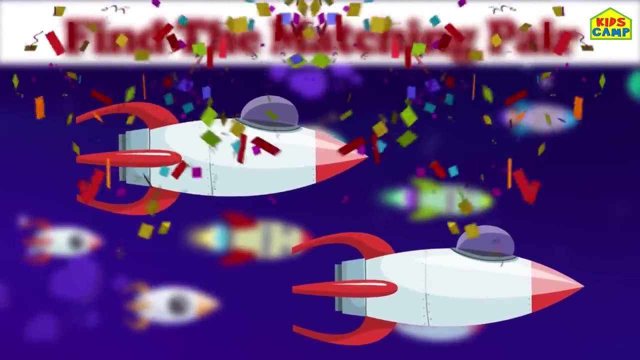 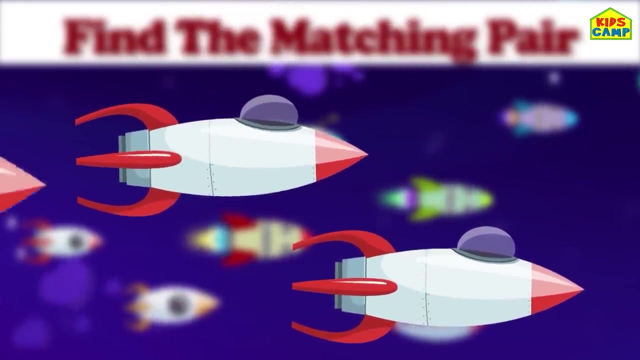 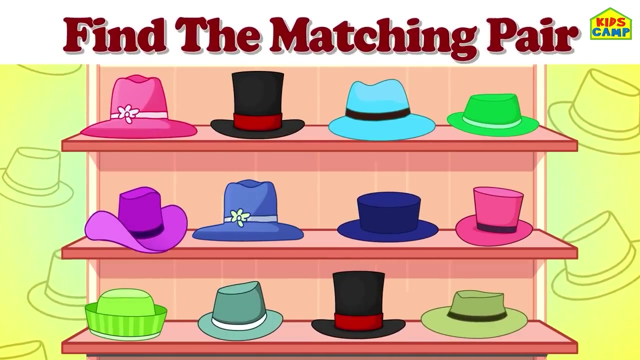 Can you? No, not this one. No, Yes, That's right, They match. Perfect, We found them. This was easy. Let's go to the next one: Find the matching hats. No, Yes, We found them. 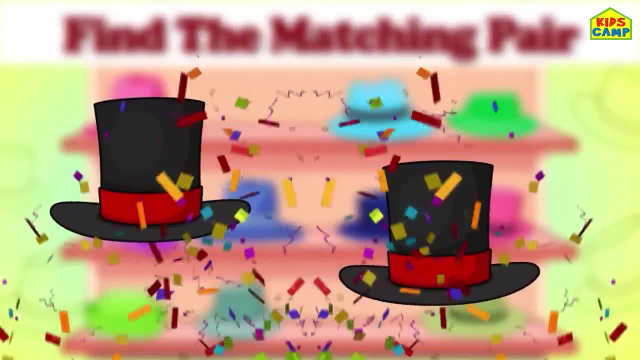 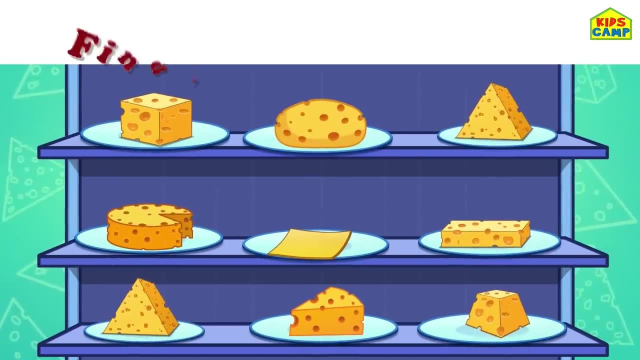 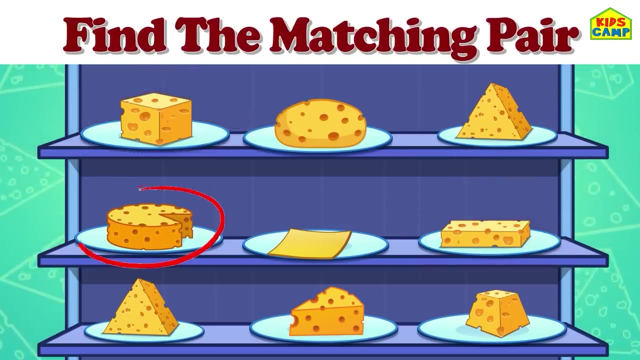 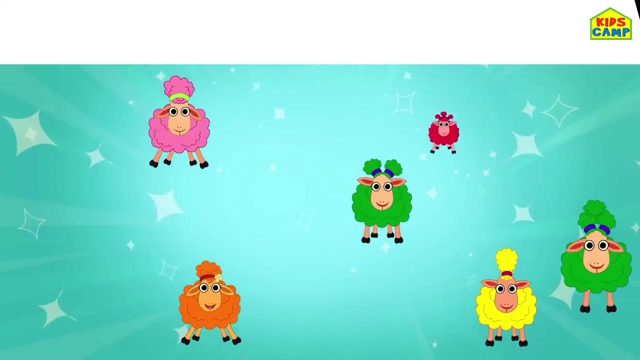 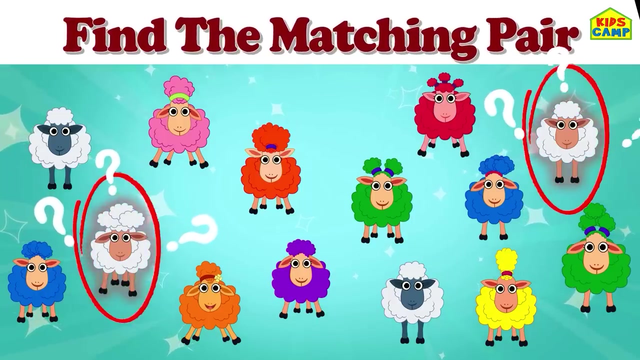 Perfect pair. Good job, friends. Can you find the matching cheese? No, Definitely no, That's right, These match Perfect Good job. Can you find the matching pair here? No, They are not identical. Yes, They match. 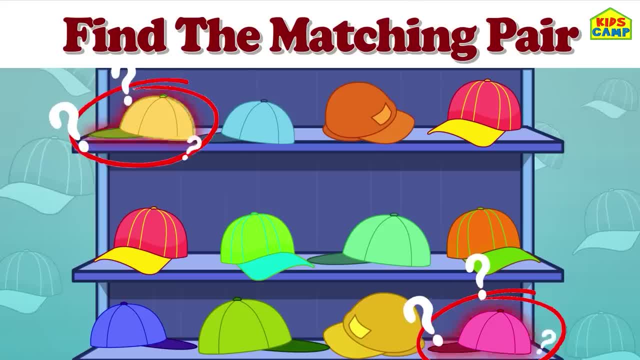 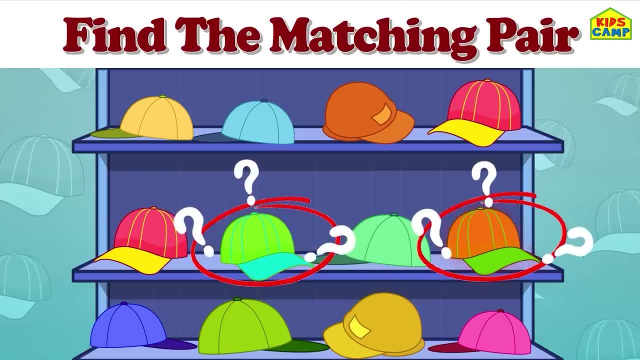 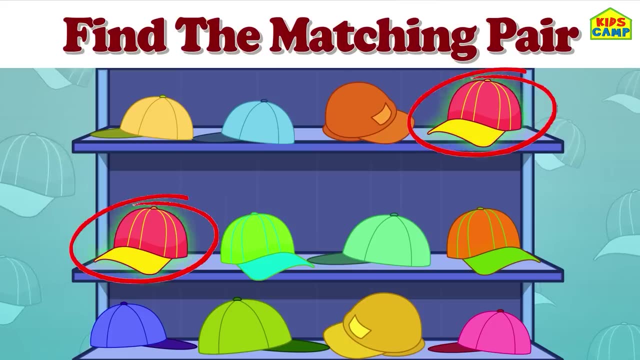 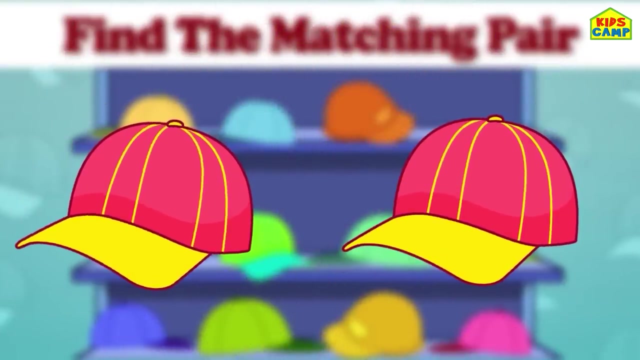 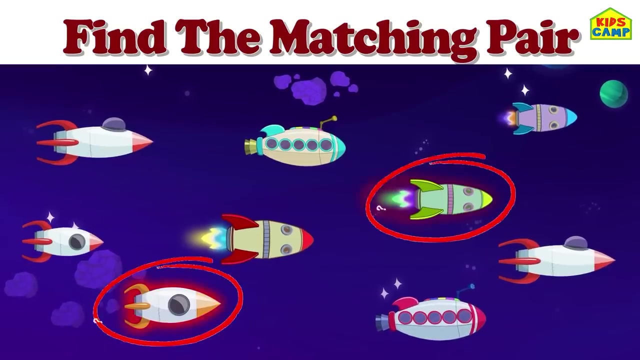 identical caps. Can you spot two identical caps? No, They're not identical. No, They're not identical. No, No, Yes, Yay, We found them. They're two identical caps. Good, job, job, let's find another pair, find the matching rockets, can you? no, not this one. 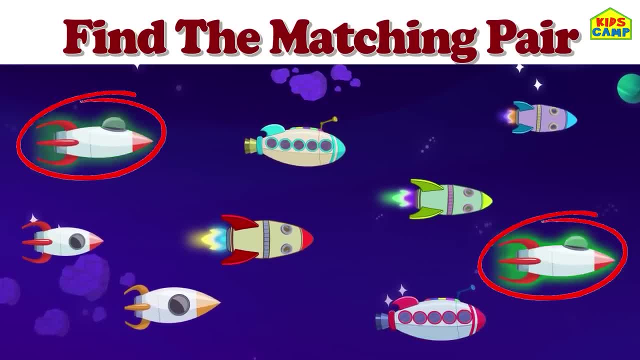 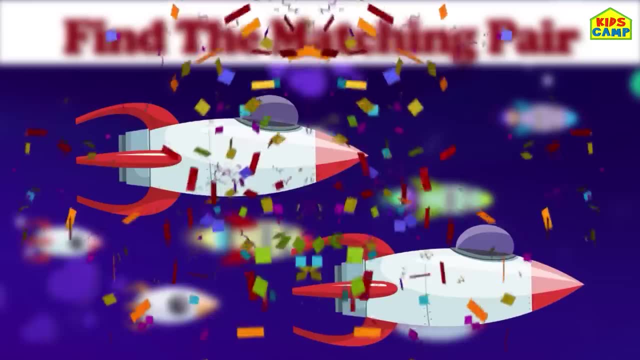 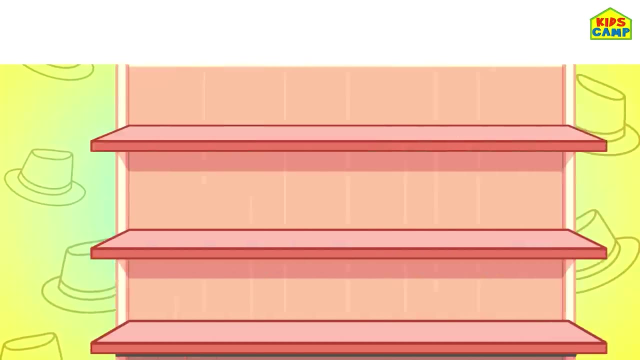 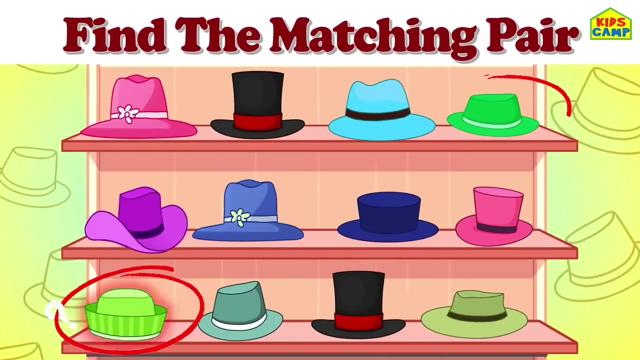 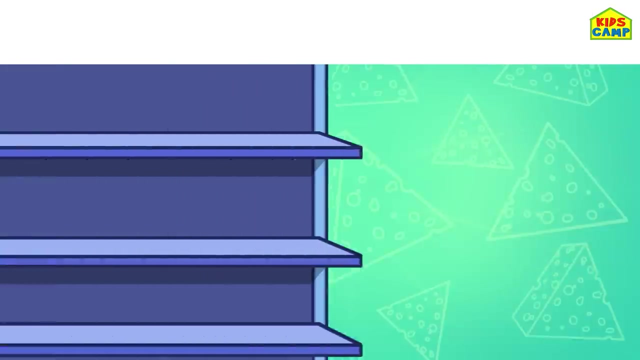 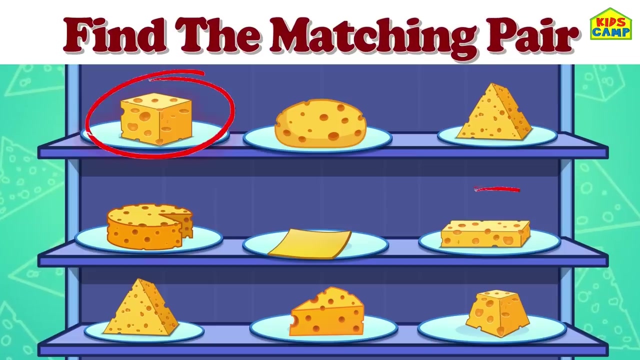 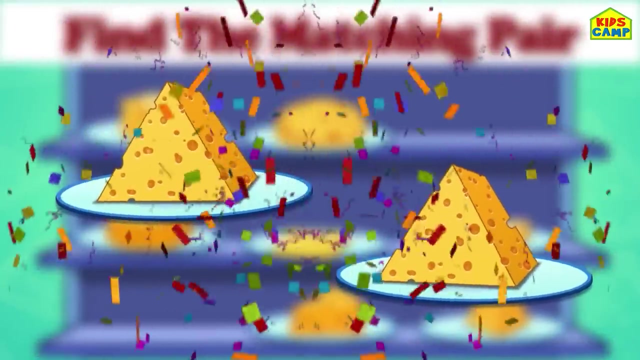 no, yes, that's right, they match perfect. we found them. this was easy. let's go to the next one: find the matching hats. no, yes, we found them, perfect pair. good job, friends. can you find the matching cheese? no, definitely. no, that's right, these match perfect, good job. 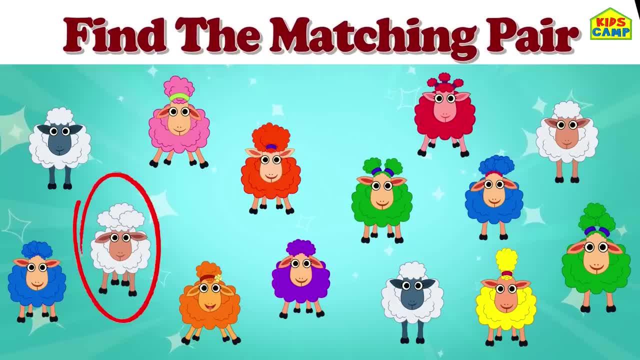 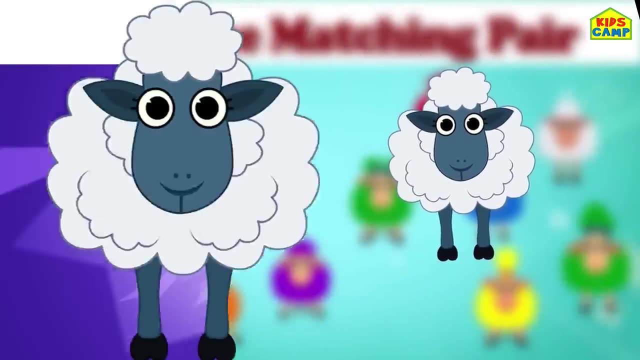 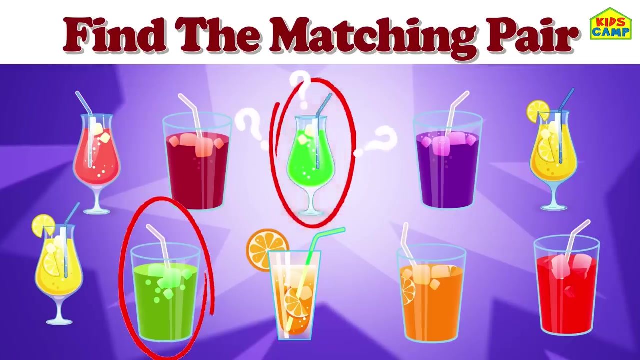 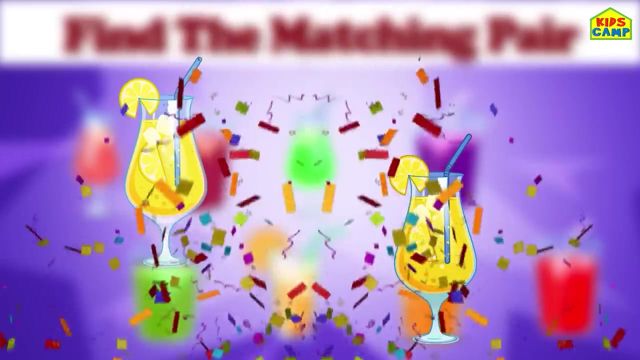 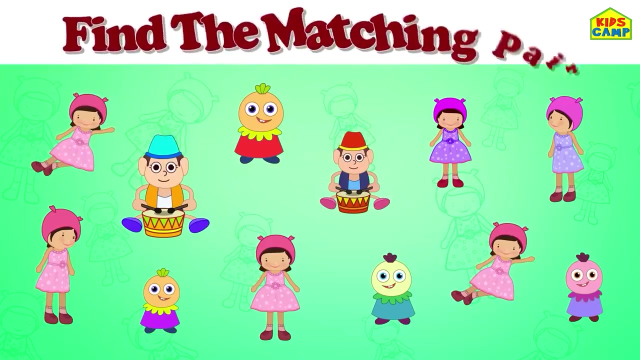 can you find the matching pair here? no, they're not identical. yes, they match. that's right. these sheep match. perfect. find the matching coolers. do these match? no, do these match? no, yes, we found the pair. good job, friends. find the matching pair. let's look for one. 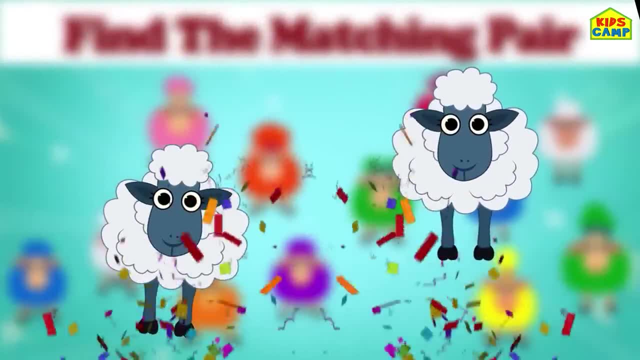 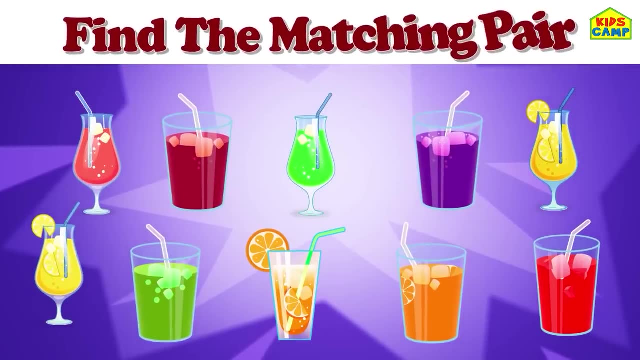 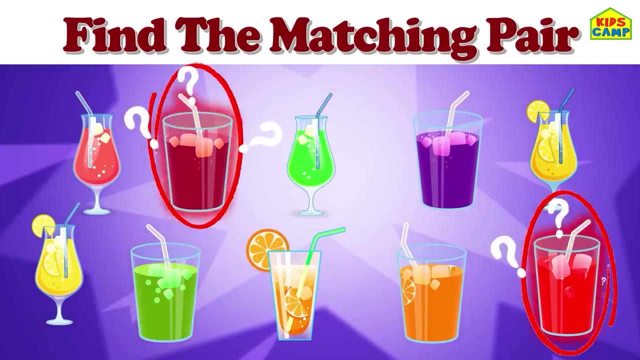 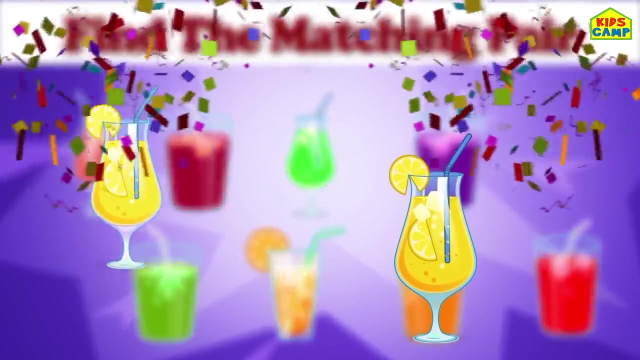 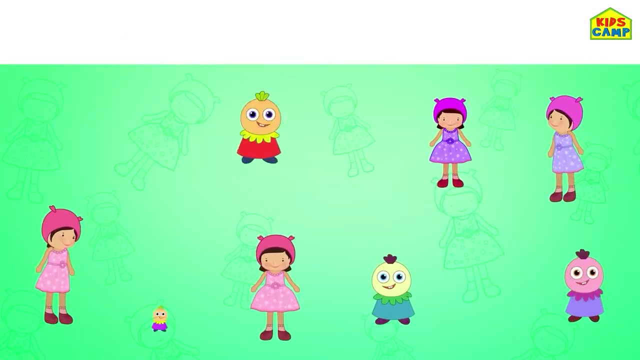 That's right, These sheep match Perfect. Find the matching coolers. Do these match No, Do these match No? Yes, We found the pair. Good job, friends. Find the matching pair. Let's look for one. 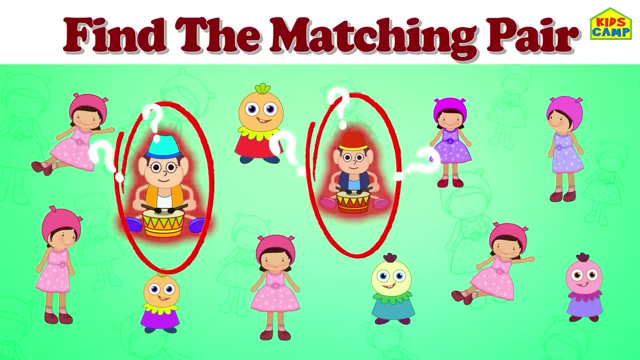 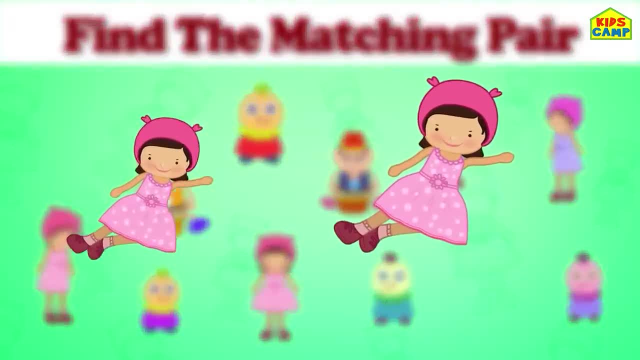 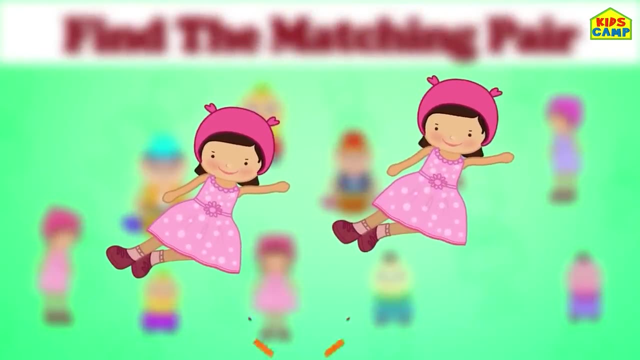 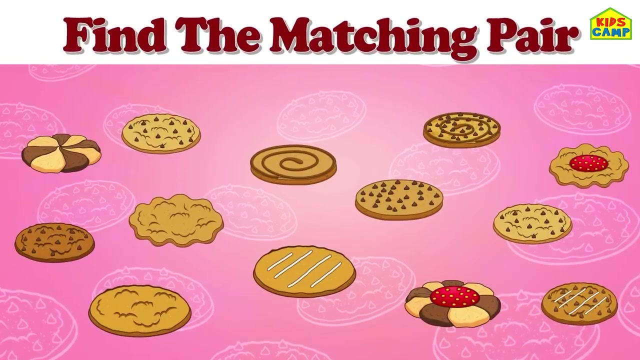 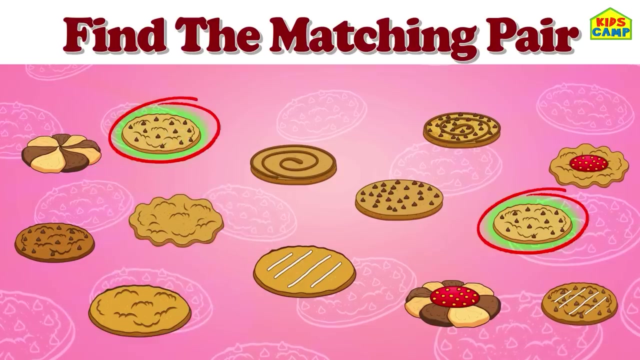 No, No way, That's right, We found the pair. Yay, Good job, friends, This game is so much fun. Ooh Cookies, Find the matching pair. No way, Yes, We found them. I love cookies. 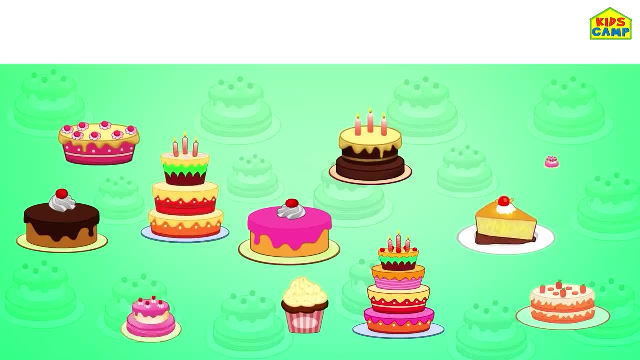 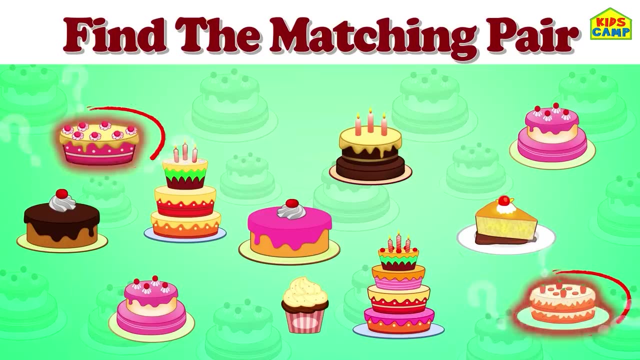 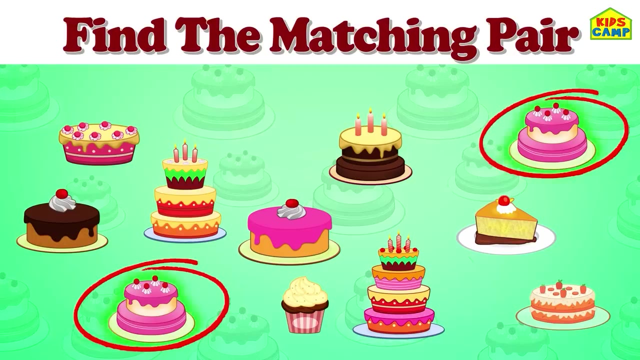 Yummy, Let's go to the next one. Hmm, Cakes. Find the matching pair. No, No, No, Yes, That's right, The matching pair of cakes. Yummy, Wonderful, Ooh Donuts. Find the matching pair. 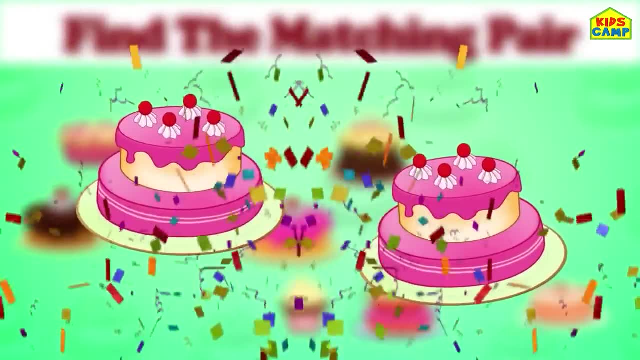 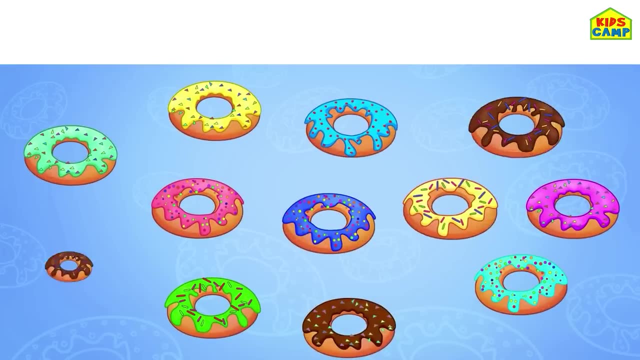 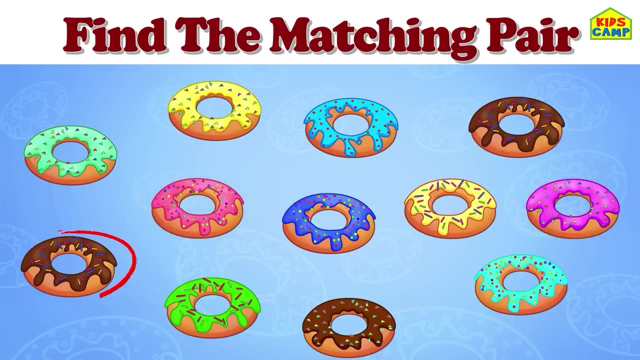 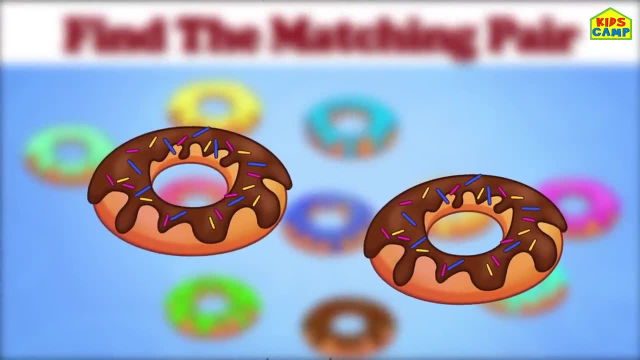 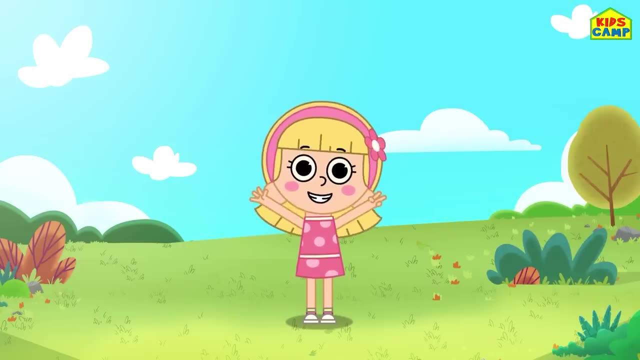 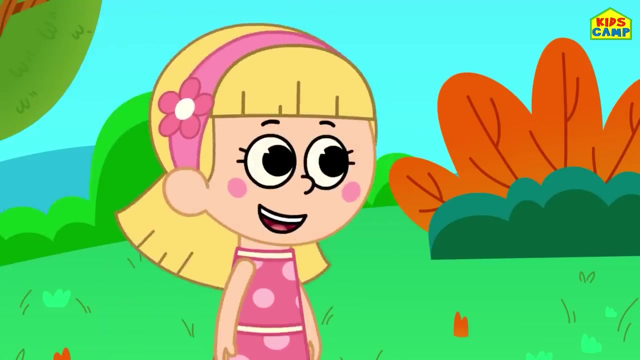 No, No, No, No, No, No, Yes. Find the matching pair These match. This was such a fun game, friends. Keep watching Kids' camp. Bye-bye, Hi friends. I'm Ely and this is Evah. 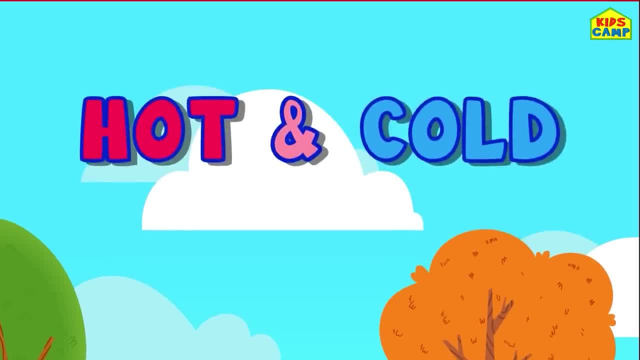 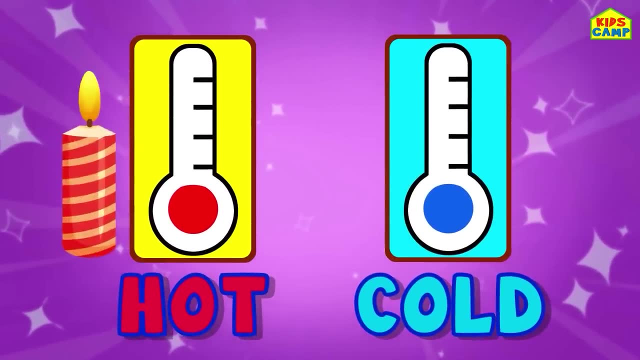 Today we're going to play a fun game of hot and cold. That's right. We have to sort according to what we're going to focus on today. So short notice, According to what is hot and what is cold. For example, a candle is hot. 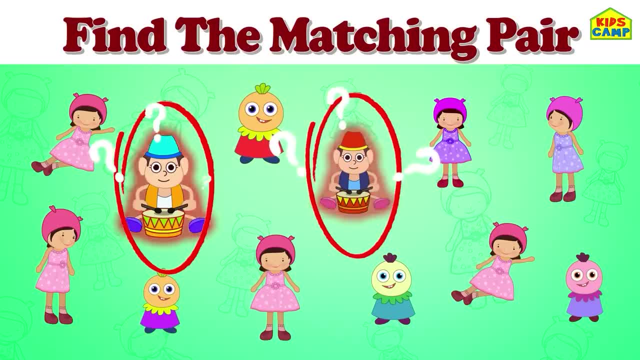 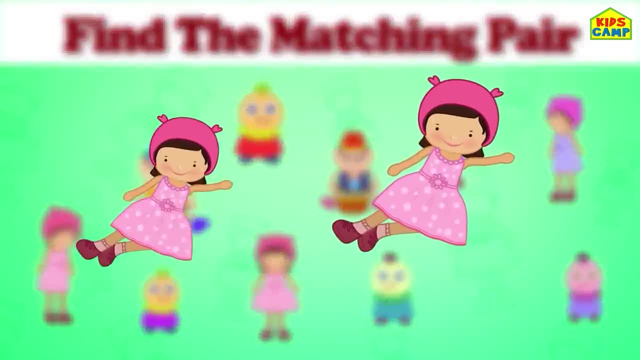 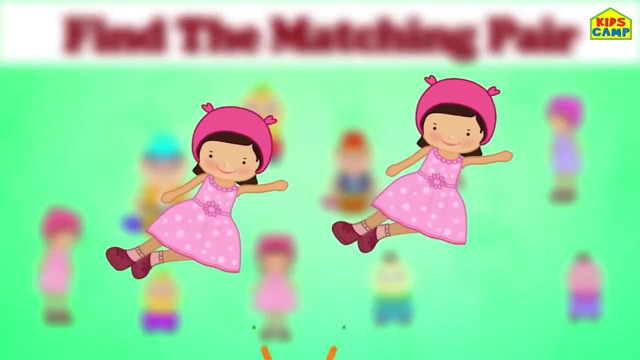 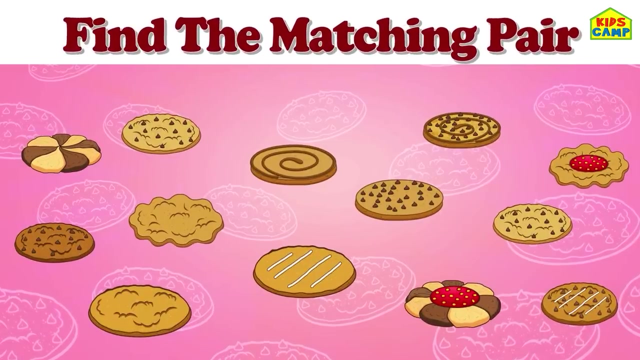 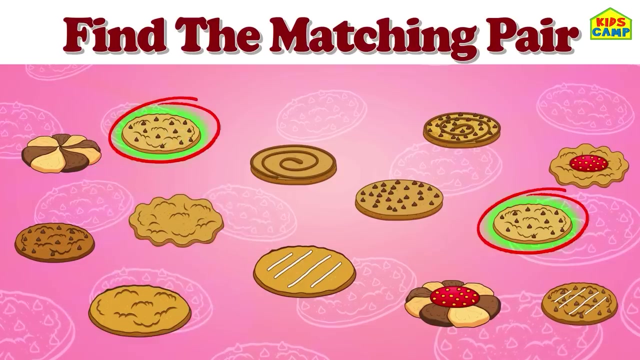 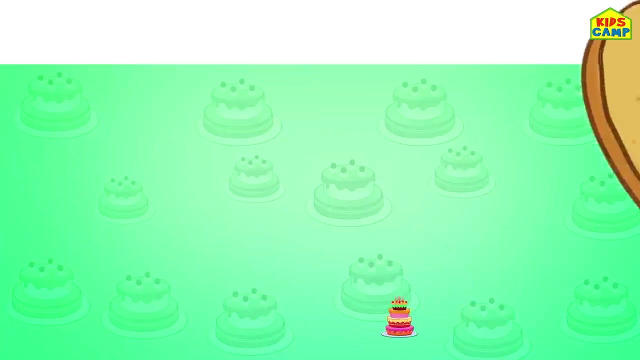 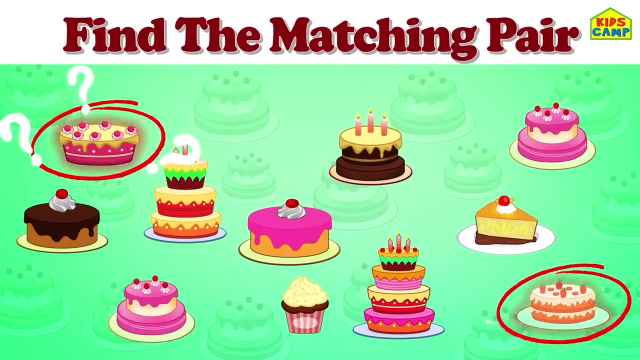 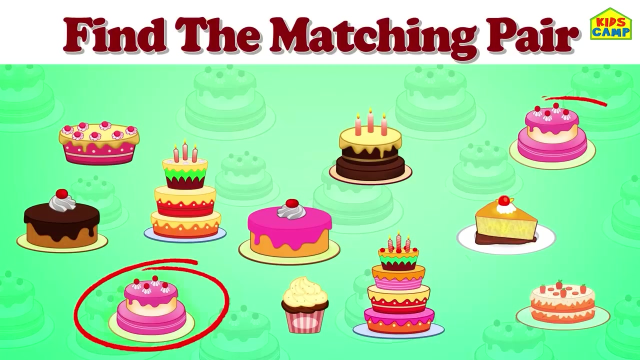 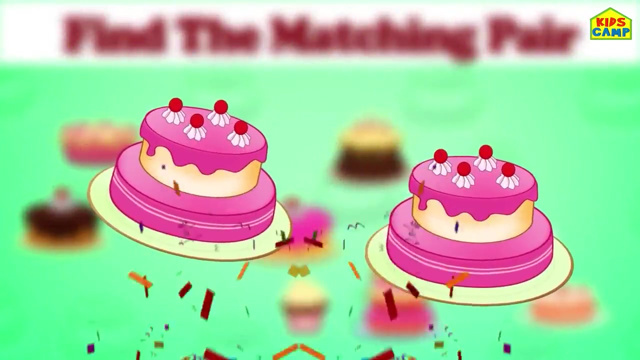 no, no, no way, that's right, we found the pair. yay, good job. friends, this game is complete. so much fun. find the matching pair: yummy. let's go to the next one: cakes. find the matching pair. no, no, yes, that's right. the matching pair of cakes, yummy, wonderful. 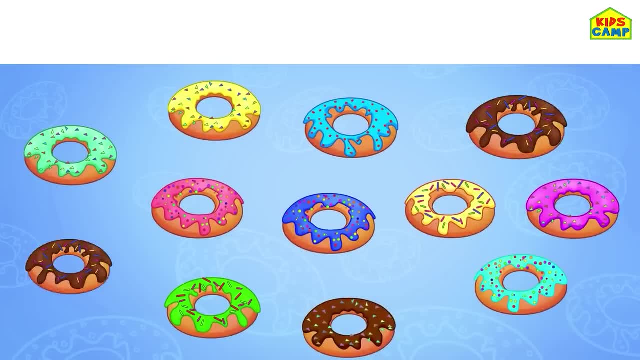 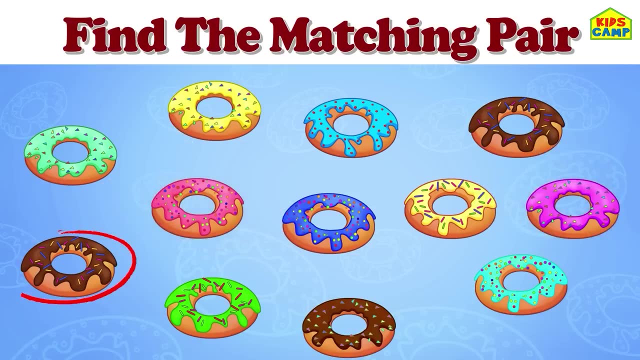 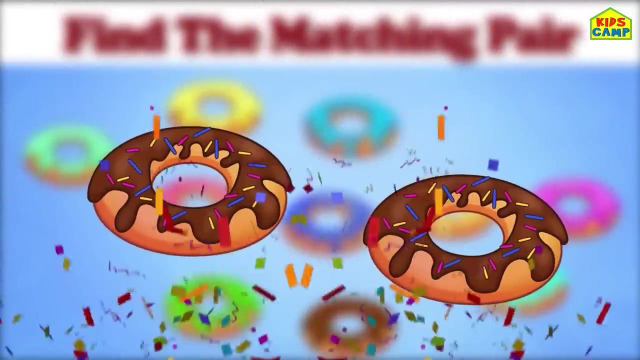 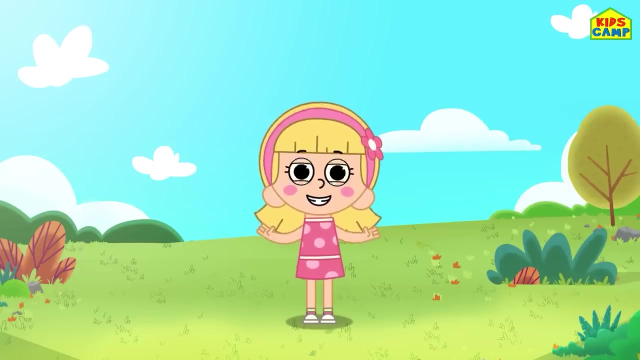 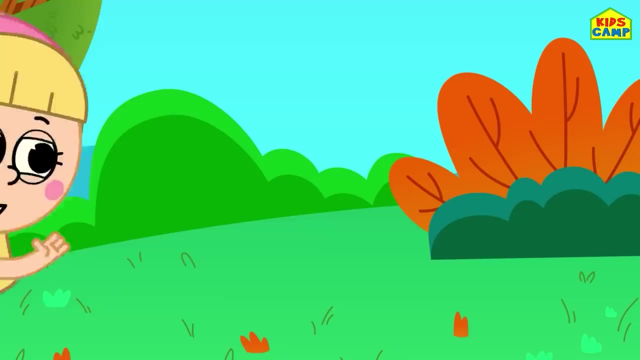 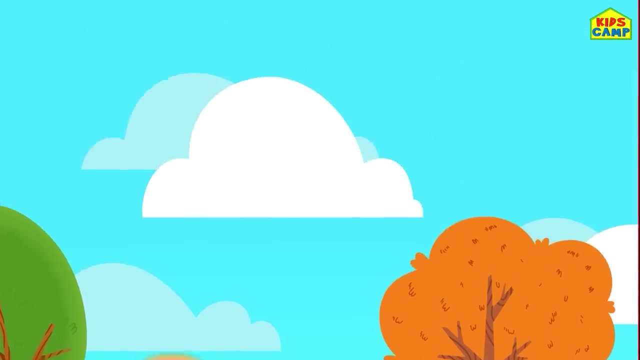 oh, donuts, find the matching pair. no, no, yes, we found the matching pair. these match. this was such a fun game. friends, keep watching kids camp, bye, bye, hi friends, i'm ellie and this is eva. today we're going to play a fun game of. 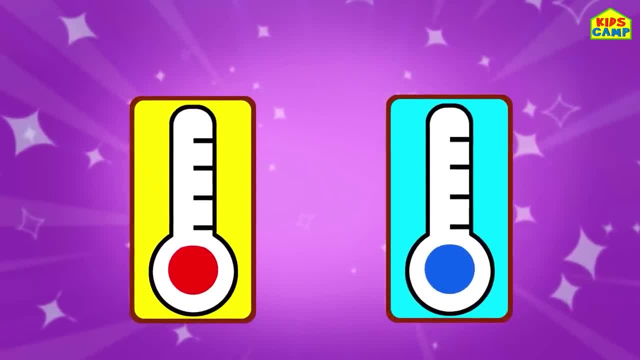 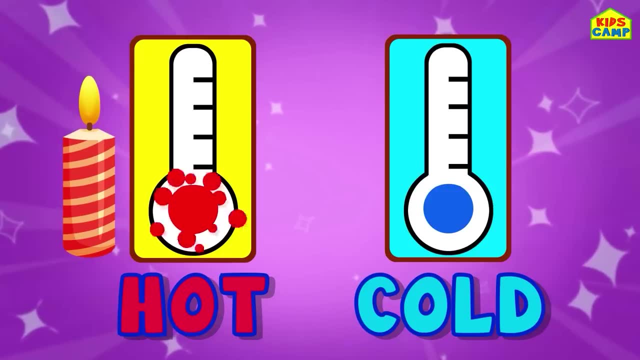 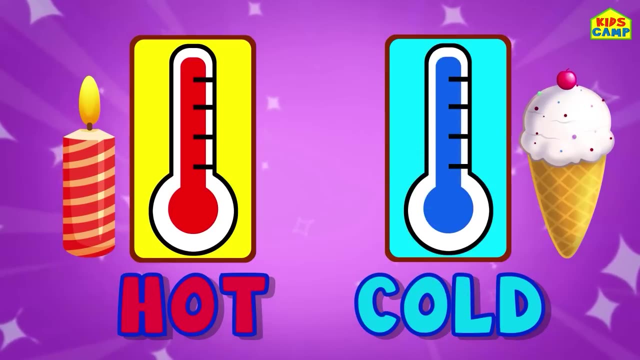 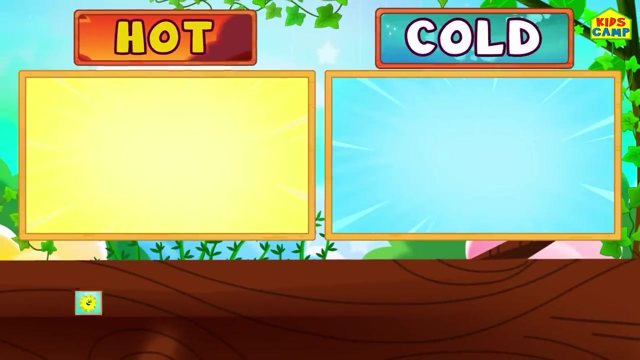 hot and cold. that's right. we have to sort according to what is hot and what is cold. for example, a candle is hot, that's right, and an ice cream is cold, that's right. wonderful, this is going to be easy. let's get started. is sun hot or cold? 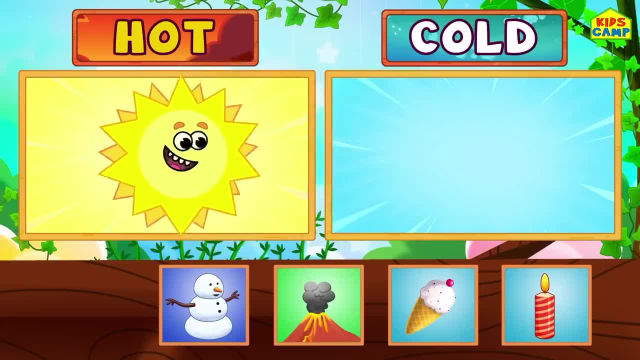 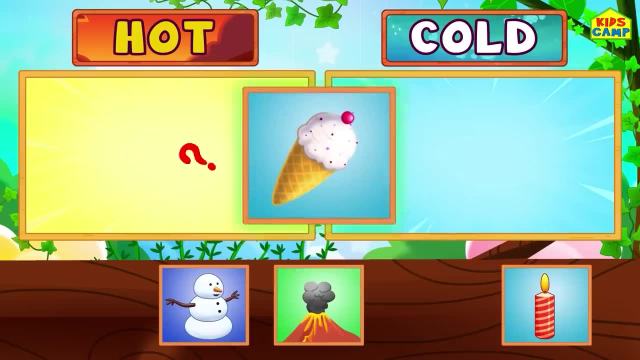 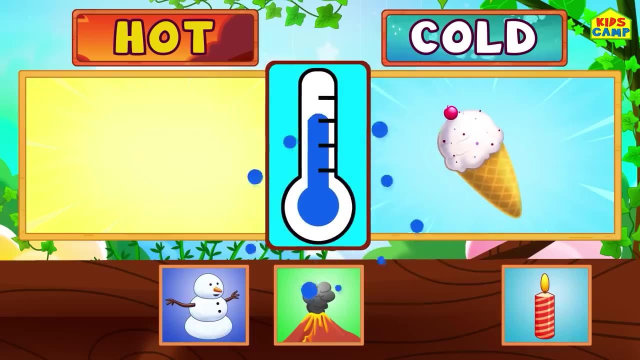 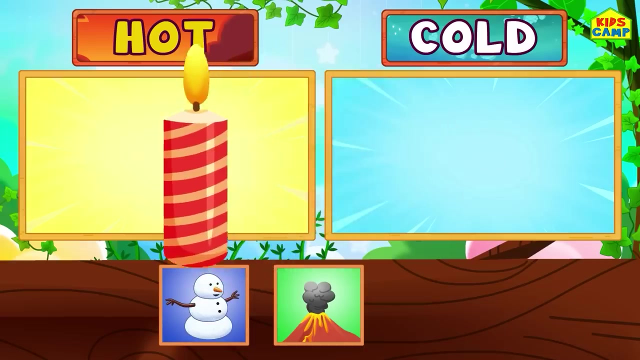 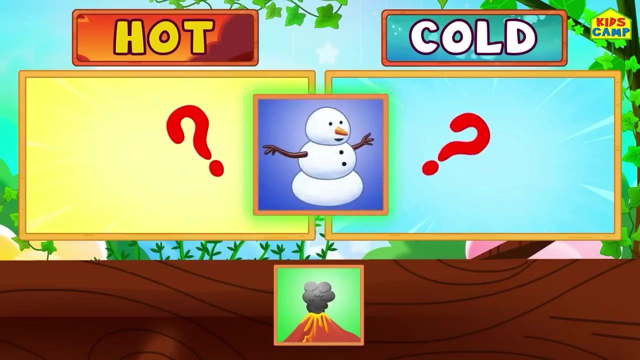 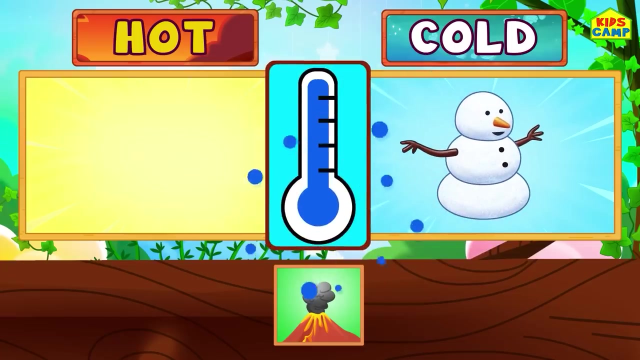 that's right. sun is hot. Anti- expiration of sun, very, very hot, that's right. ice cream, yeah, very, very great. and then a candle, hot or cold, hot, good job, that's right. говорю 하, Yes, Cold, That's right. A volcano- Hot or cold. 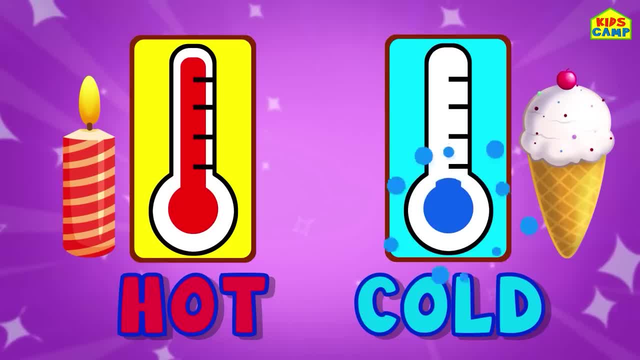 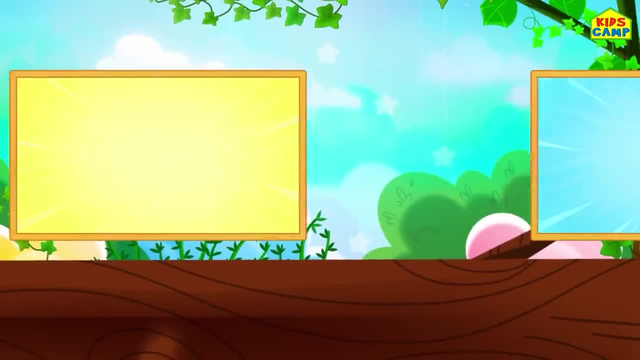 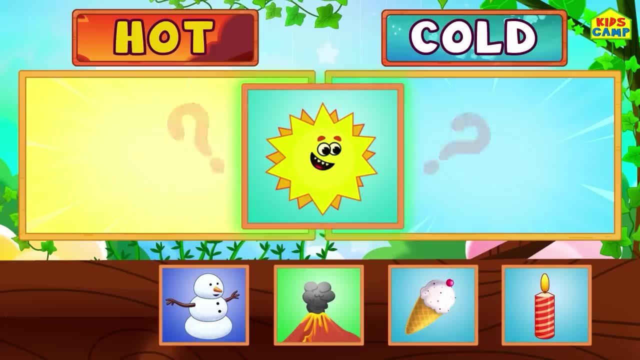 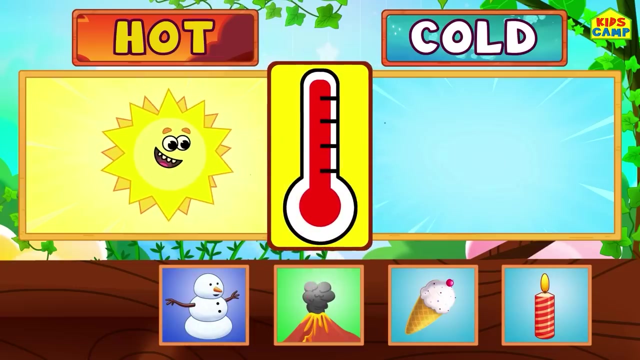 That's right. And an ice cream is cold, That's right. Wonderful, This is going to be easy. Let's get started. Hmm, is sun hot or cold? That's right. Sun is hot, Very, very hot, That's right. 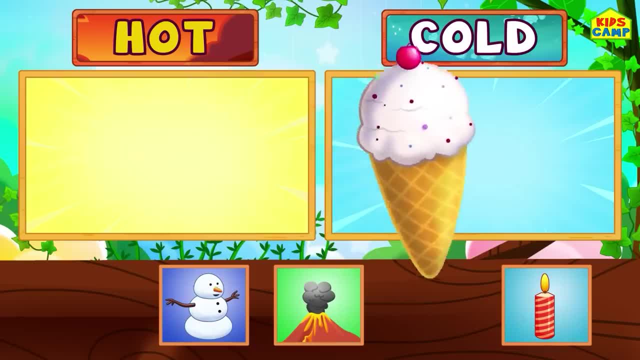 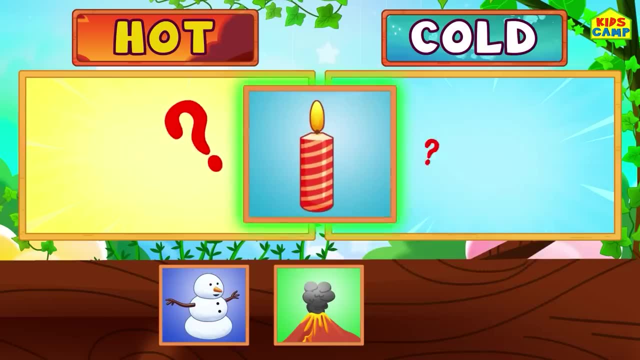 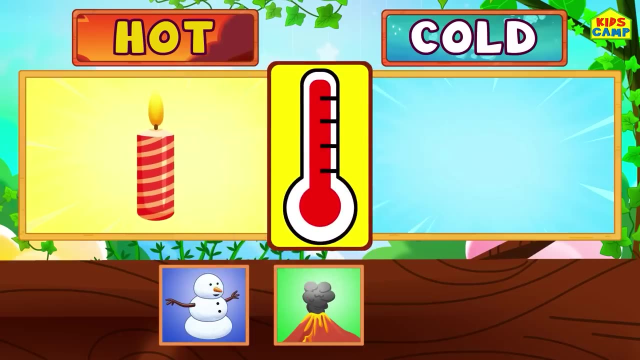 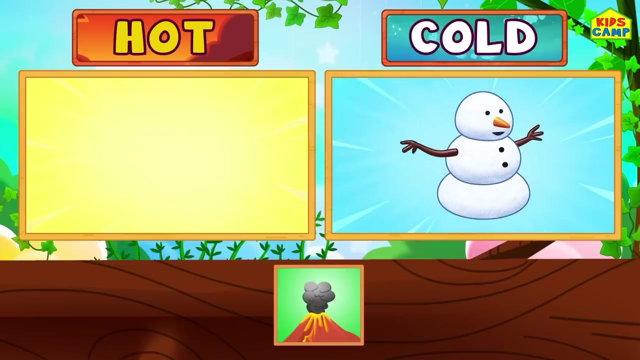 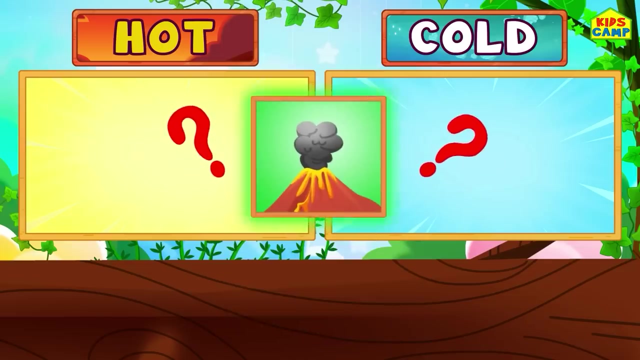 An ice cream, It's cold, Yummy. A candle- Hot or cold, Hot, Good job. That's right. A snowman- Yes, A snowman is very cold. That's right. A volcano- Hot or cold. 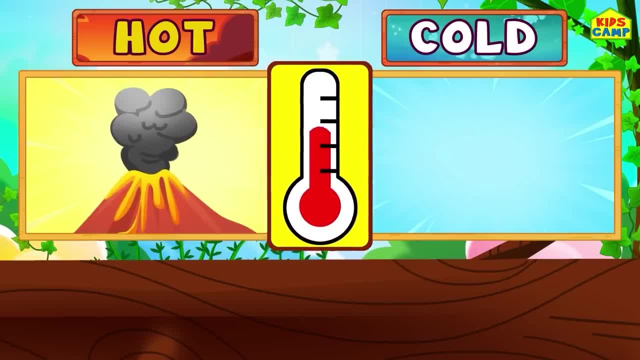 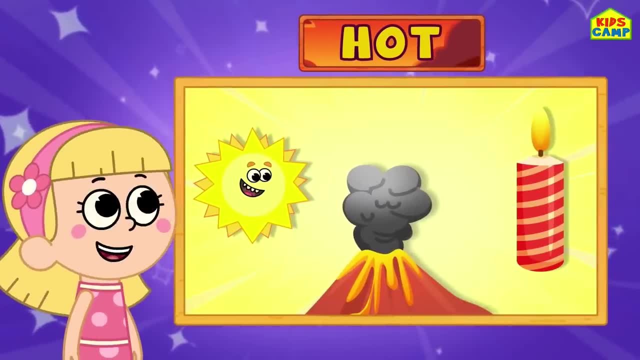 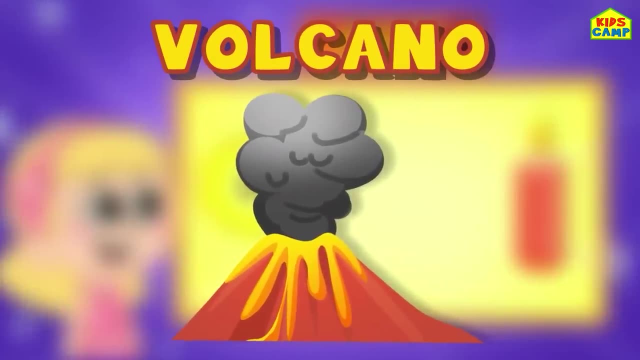 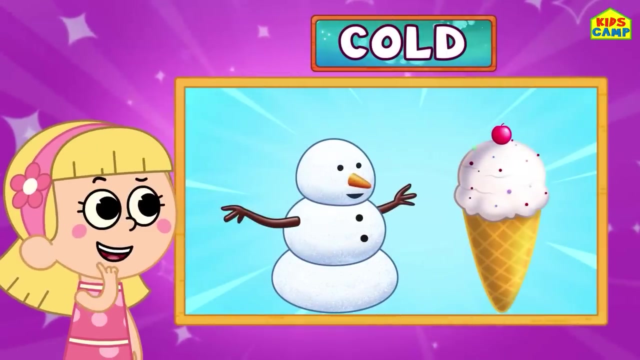 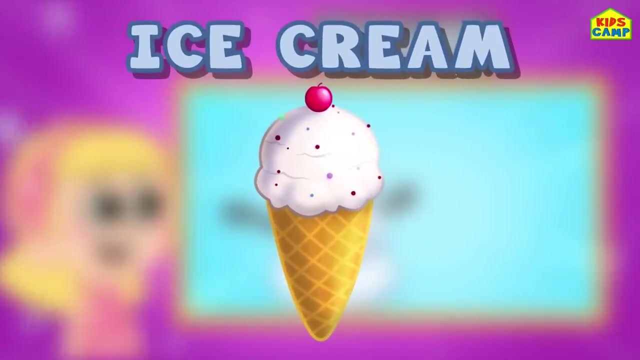 It's hot, That's right, Very hot. Yay, We found the hot objects, The sun, The volcano And the candle. And we found the snowman And the ice cream, All cold. Yay, What's next? 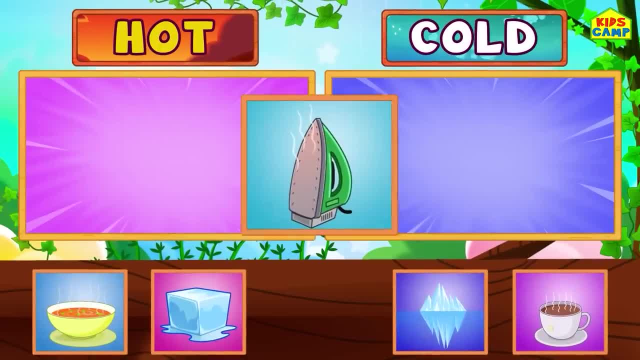 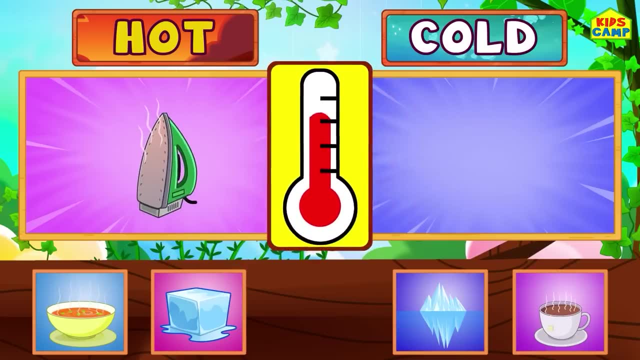 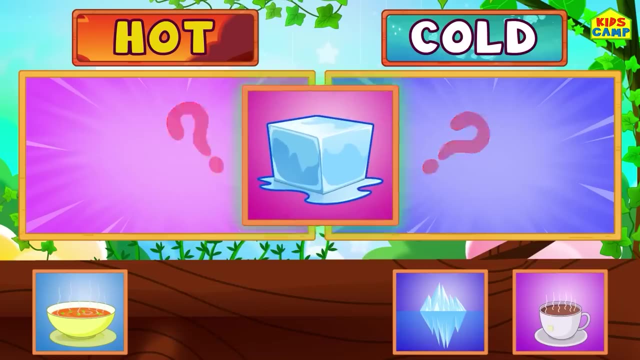 This is an easy game. An iron: Hot or cold, Hot, That's right, That's right. An ice cube, An ice cube, Hmmcold, Very cold. A cup of coffee: Hot or cold, Hot, That's right. 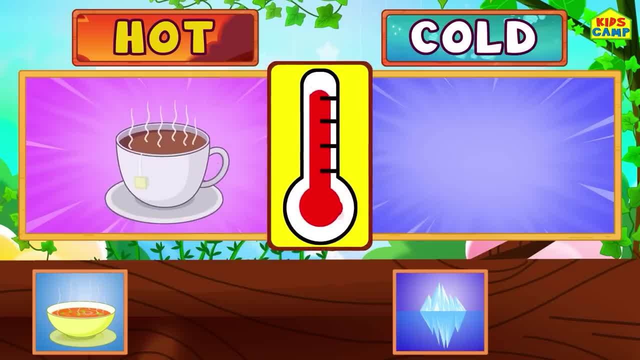 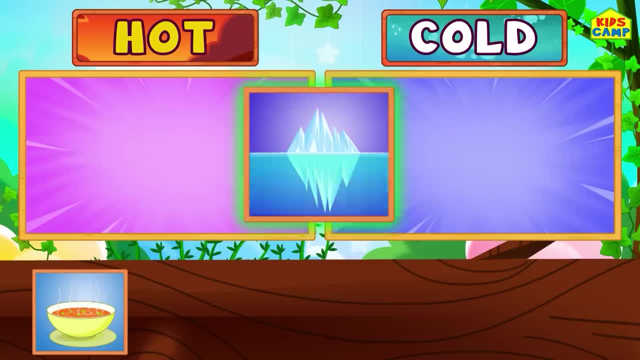 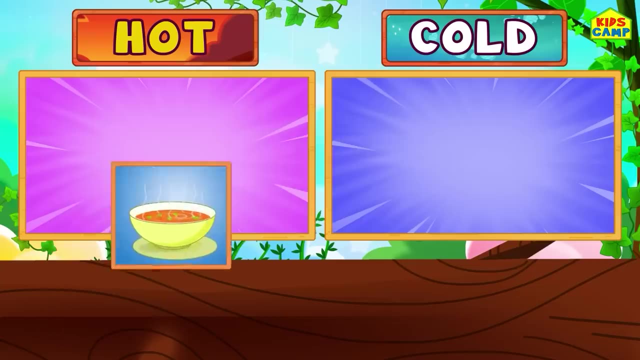 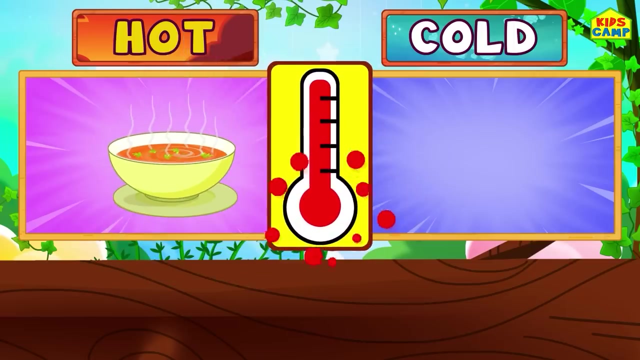 An iceberg, It's cold, That's right, An iceberg, It's cold, It's cold, Good job, Good job. A bowl of soup, A bowl of soup, That's right, Hot, Wonderful. What did we learn? 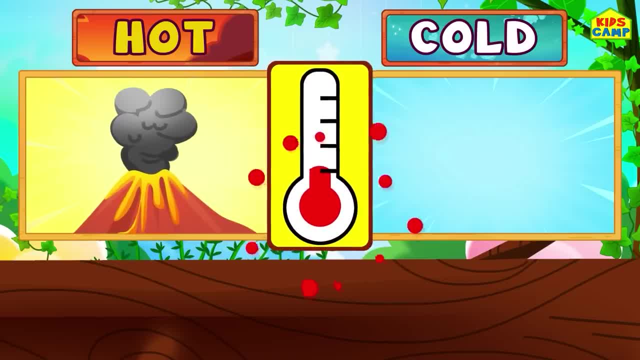 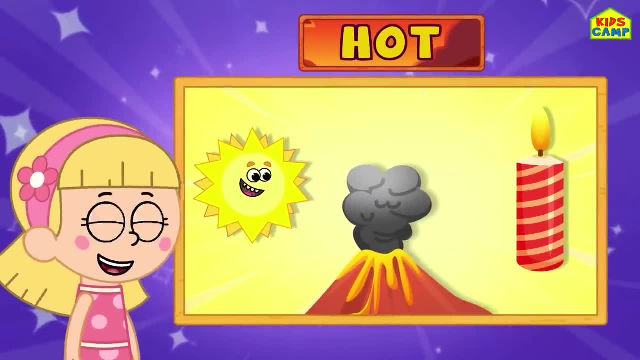 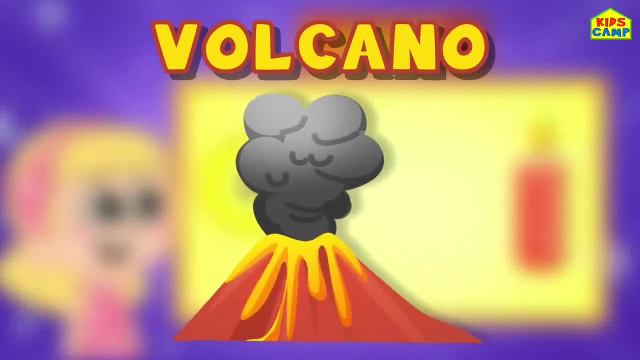 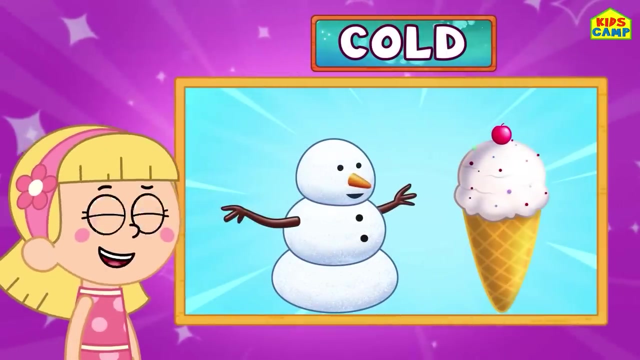 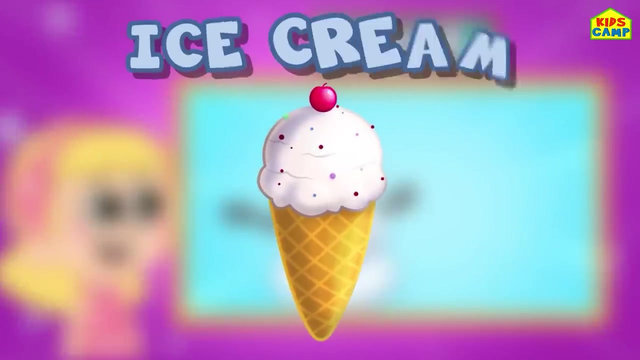 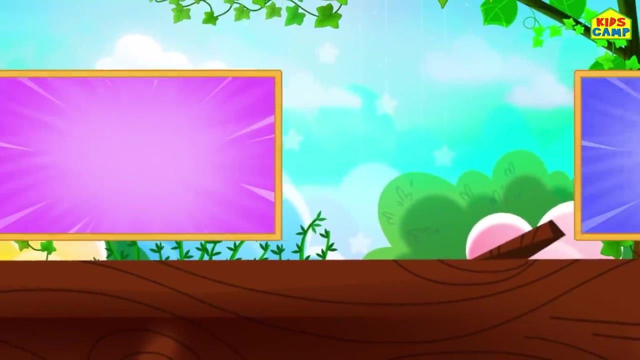 It's hot, That's right, Very hot. Yay, We found the hot objects, The sun, the volcano and the candle. And we found the snowman and the ice cream, All cold. Yay, What's next? 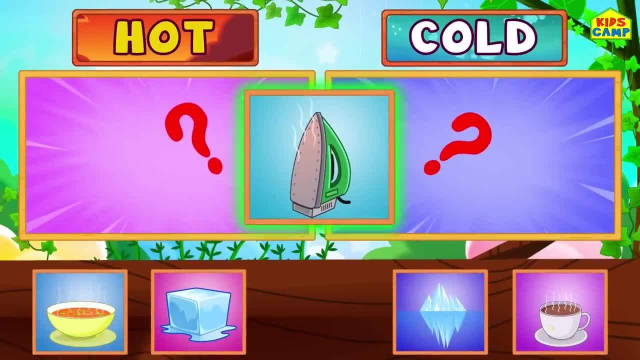 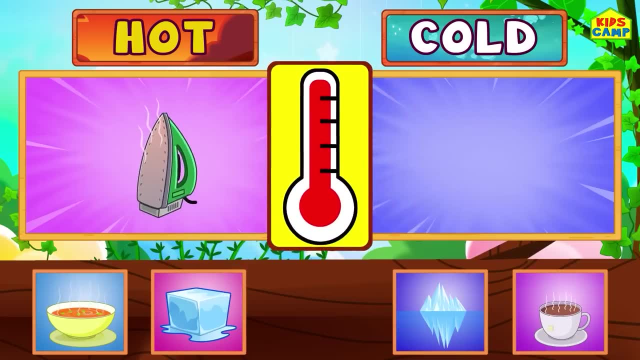 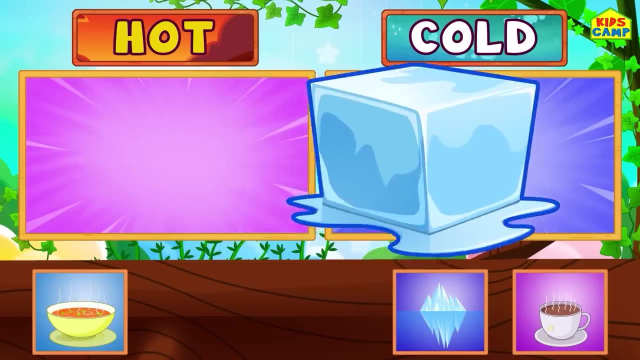 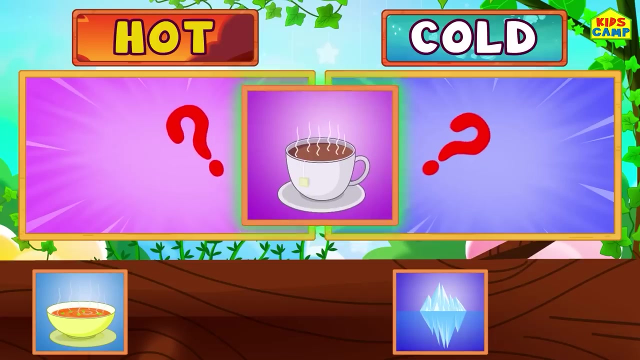 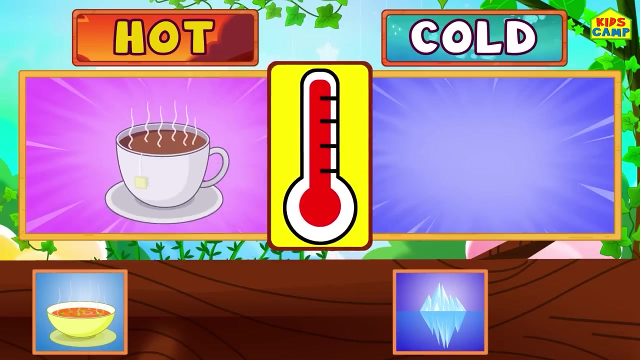 This is important Easy game. An iron, Hot or cold- Hot, That's right. An ice cube, Hmm, Cold, Very cold. A cup of coffee: Hot or cold- Hot, That's right. An iceberg, It's cold. 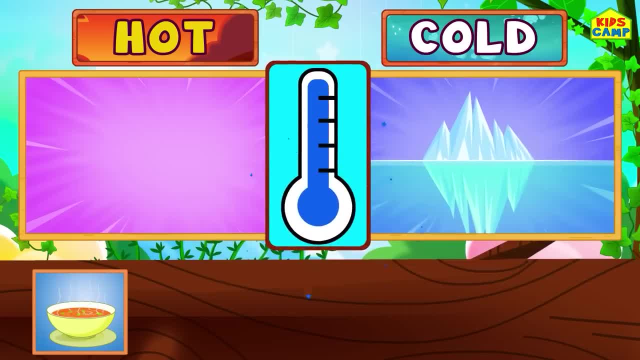 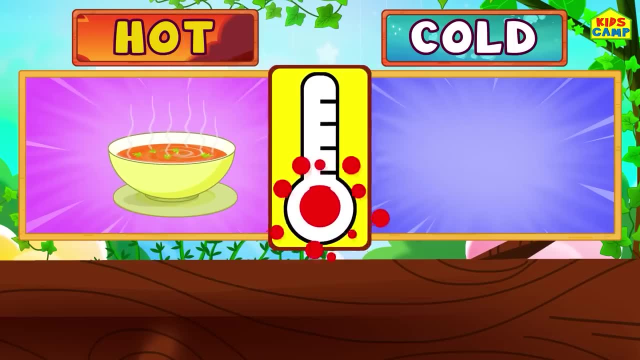 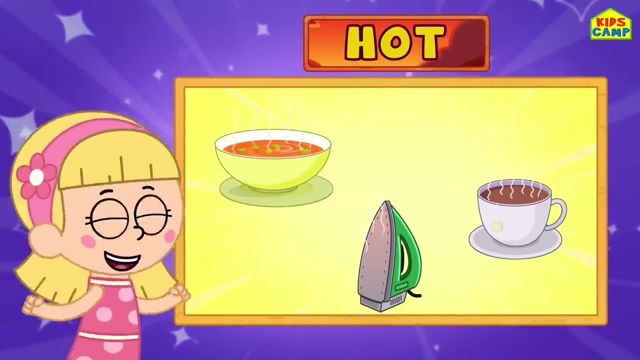 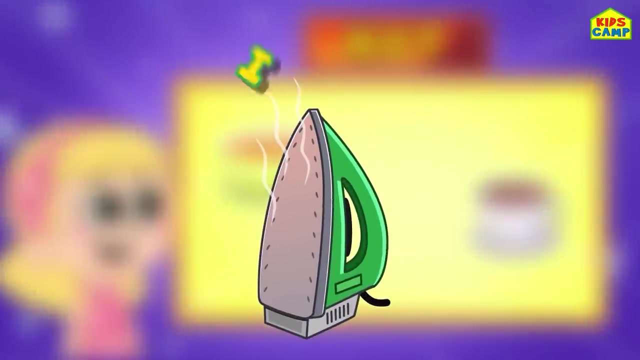 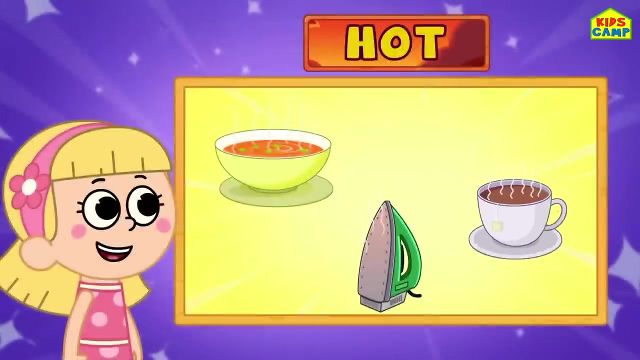 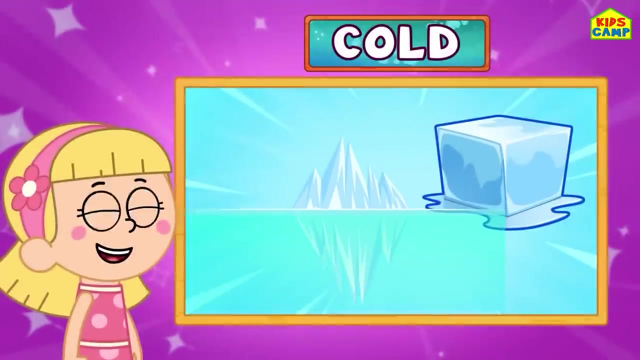 Good job. A bowl of soup, That's right. Hot, Wonderful. What did we learn? A bowl of soup is hot, An iron is hot and a cup of coffee is hot as well. An iceberg is cold and an ice cube is cold too. 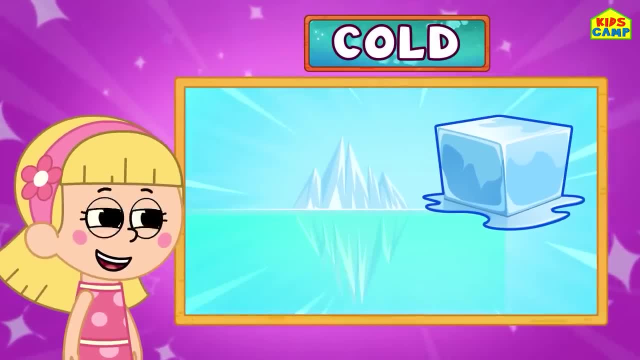 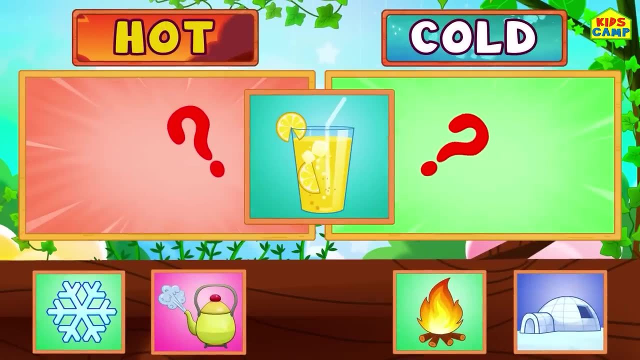 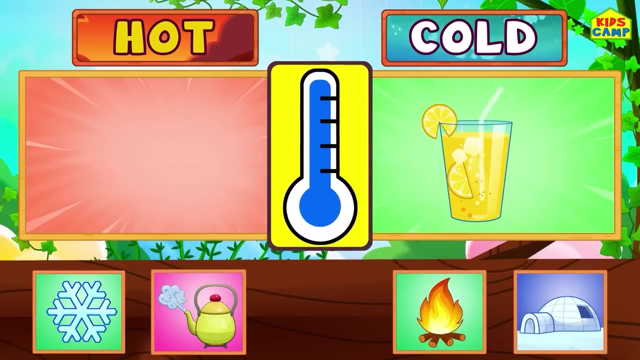 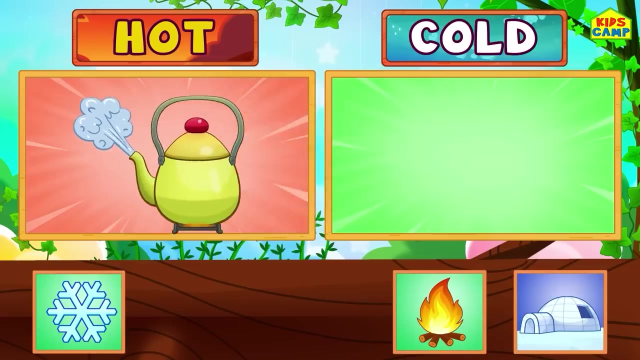 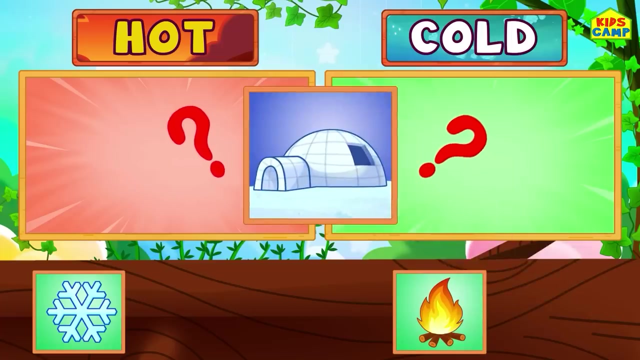 That's right, Yay, What's next? We're getting good at this game. Let's play with a lemonade. It's cold, Definitely cold. A kettle, It's hot, That's right, Hot kettle, An igloo. 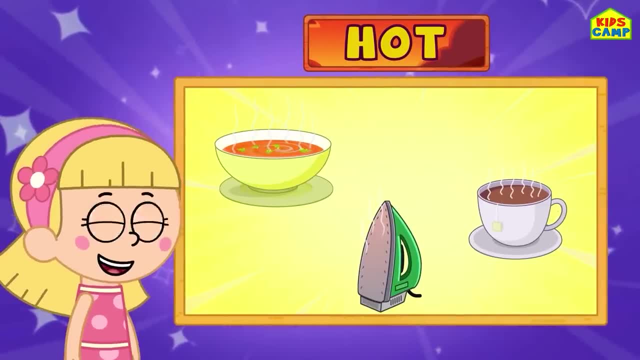 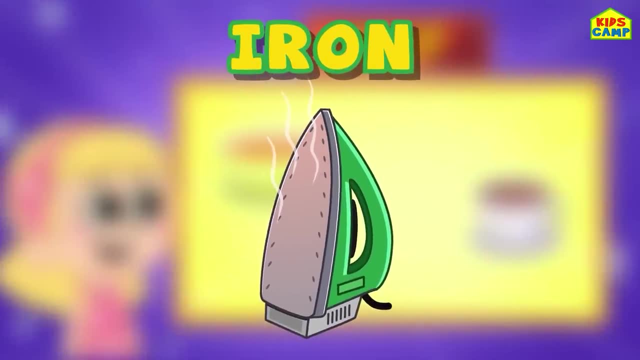 What did we learn? A bowl of soup is hot, A bowl of soup is hot, Iron is hot, And the cup of coffee is hot as well. And the cup of coffee is hot as well, And the cup of coffee is hot as well. 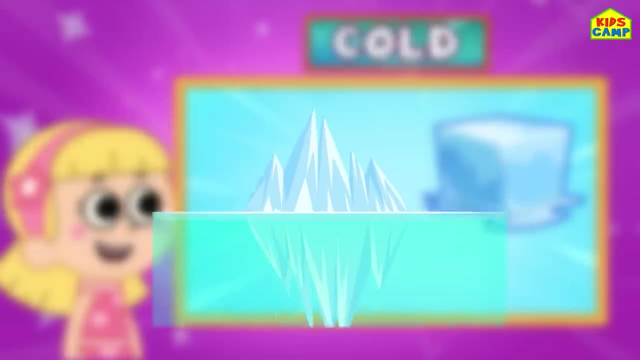 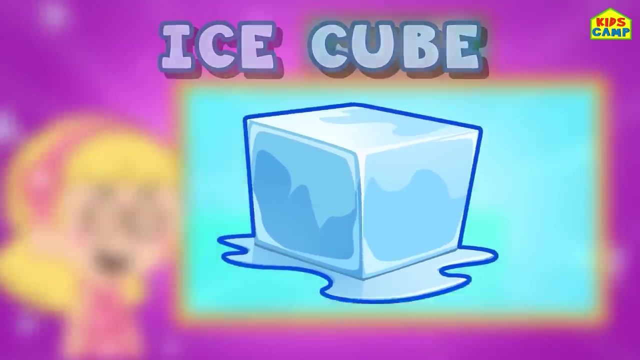 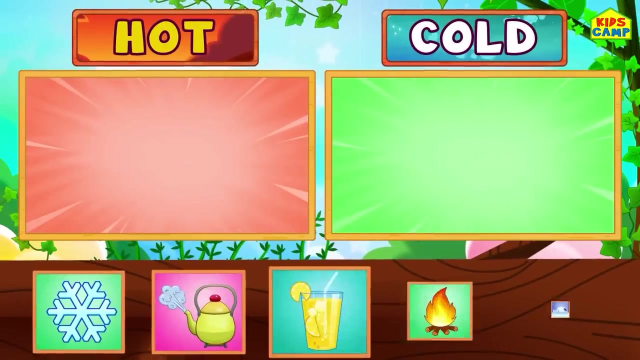 An iceberg is cold. An iceberg is cold. An iceberg is cold. And an ice cube is cold too. And an ice cube is cold too. That's right, Yay, What's next? We're getting good at this game- A lemonade. 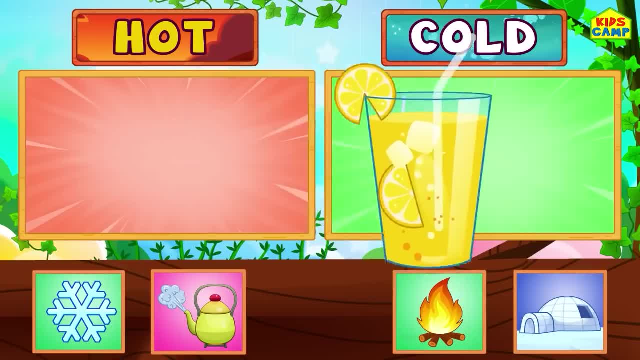 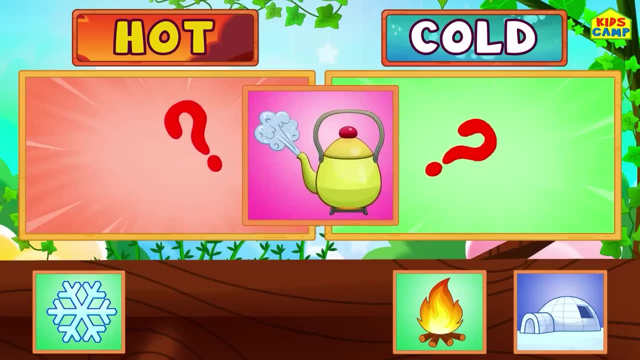 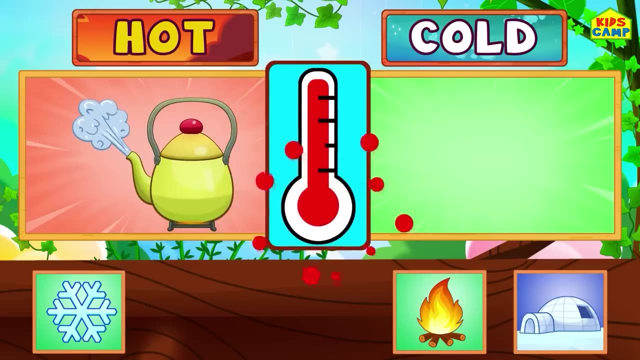 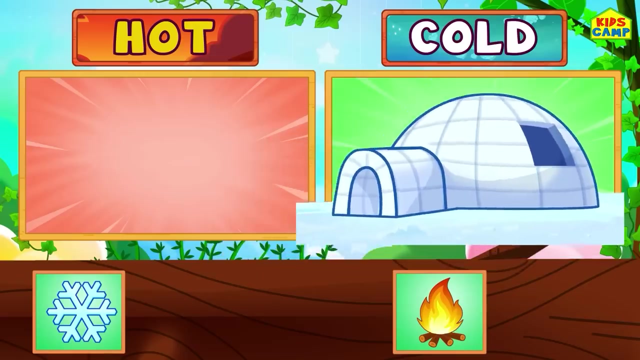 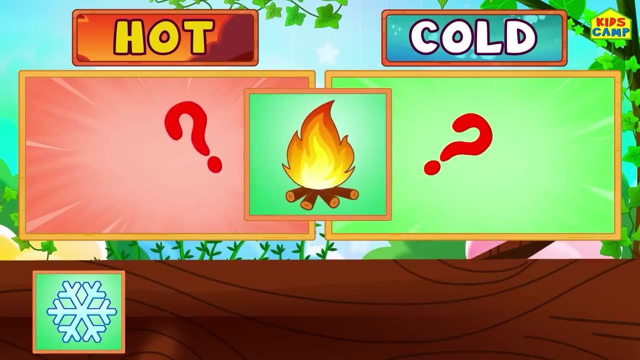 Hmm, It's cold, Definitely cold, Definitely cold. A kettle, A kettle, It's hot, It's hot, That's right, Hot kettle, An igloo, An igloo, That's cold, That's cold Fire. 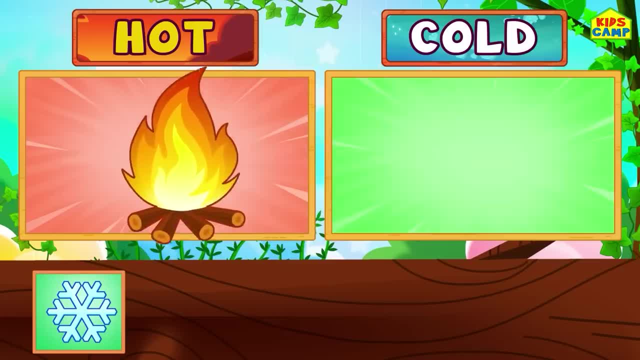 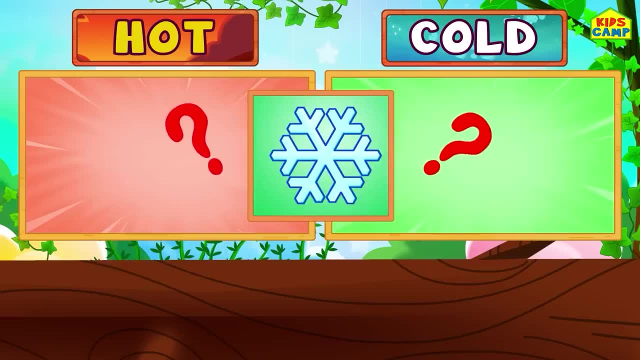 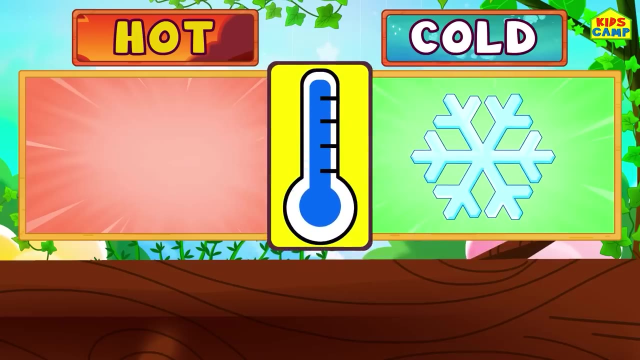 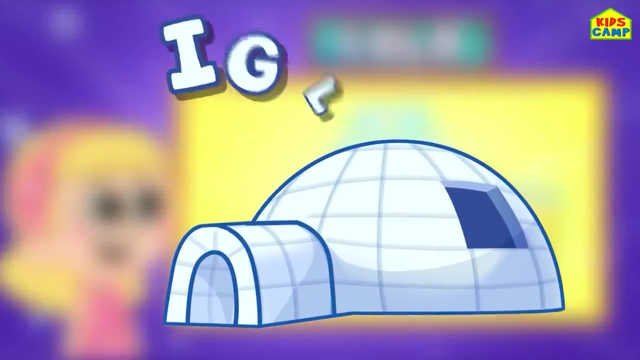 That's hot, That's hot, Definitely hot. Good job, friends. And a snowflake, And a snowflake, That's cold, That's cold. Wonderful, What did we learn? An igloo is cold. An igloo is cold. 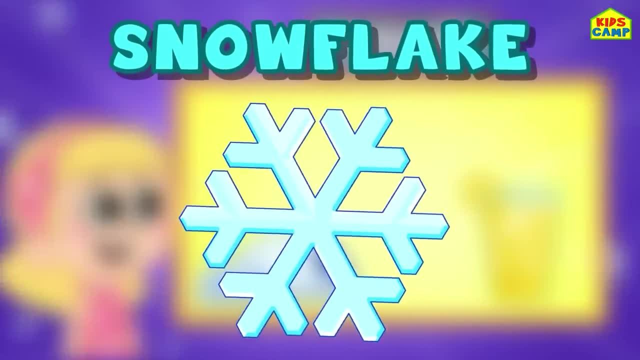 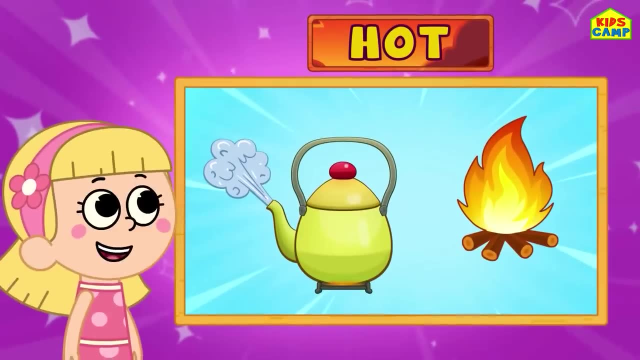 A snowflake is cold. A snowflake is cold And a glass of lemonade is definitely cold, And a glass of lemonade is definitely cold. A snowflake is cold And a glass of lemonade is definitely cold. A kettle is hot. 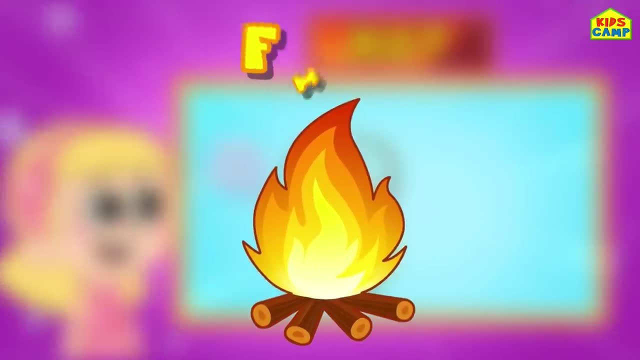 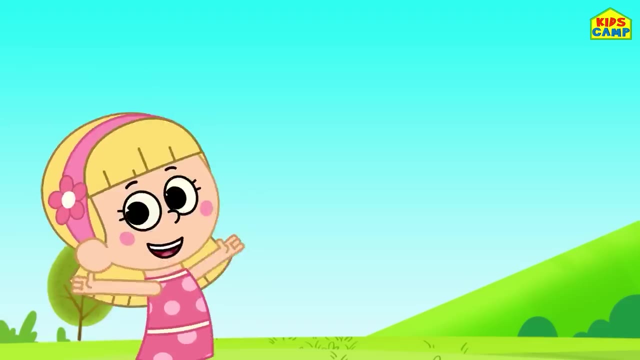 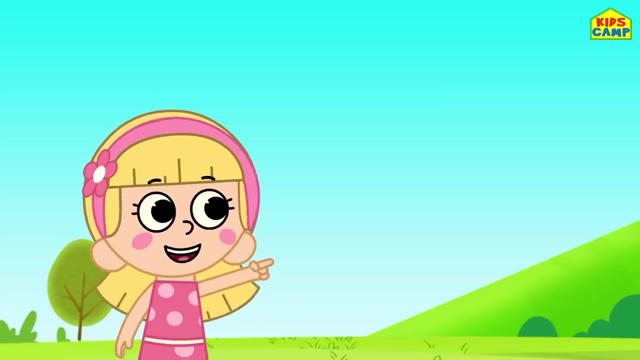 A kettle is hot And fire is hot, And fire is hot, Wonderful, Wonderful, Yay. This is so much fun learning. Come back for more. Until then, keep watching Kids' Camp. Until then, keep watching Kids' Camp. 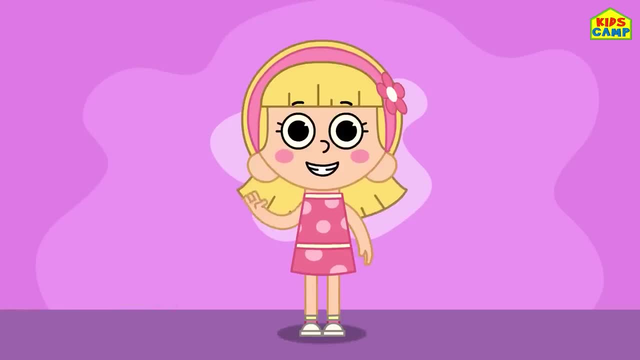 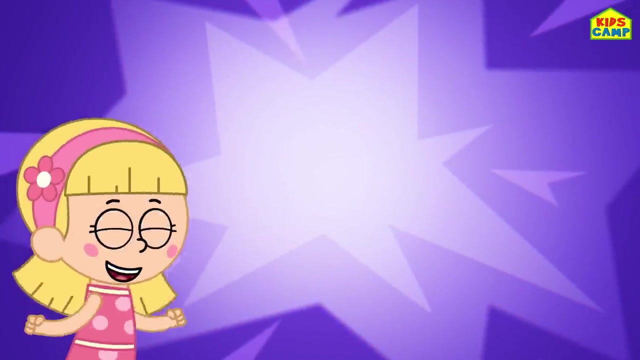 Bye, Hi kids. I'm Ellie And today is Eva's birthday. Yay, Will you help me plan a birthday party for her? Will you help me plan a birthday party for her? Yes, Let's go First. we'll need a birthday cake. 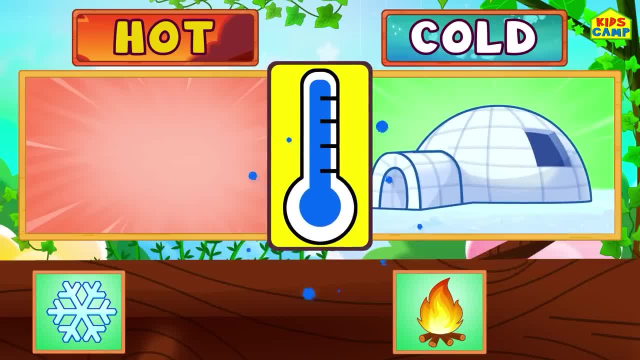 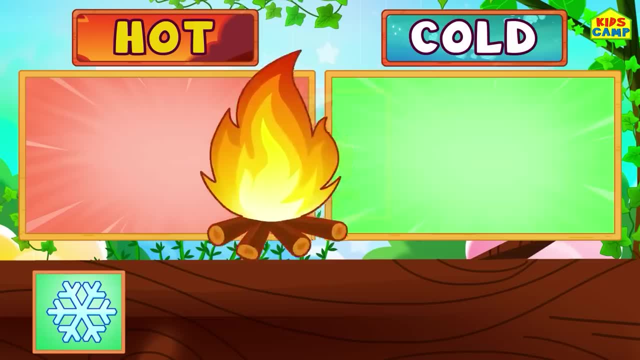 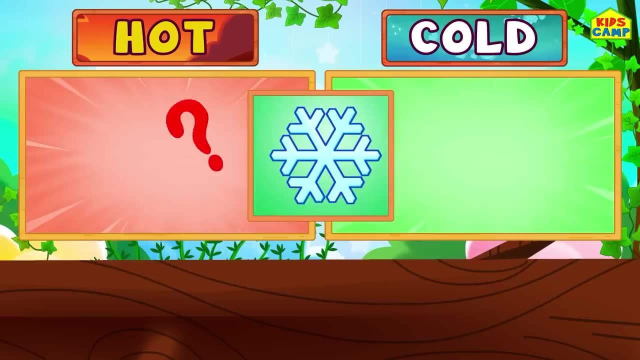 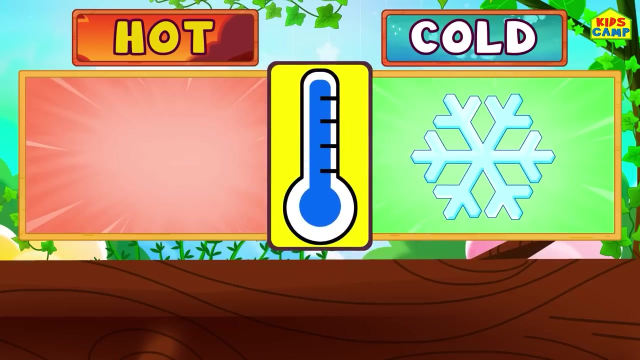 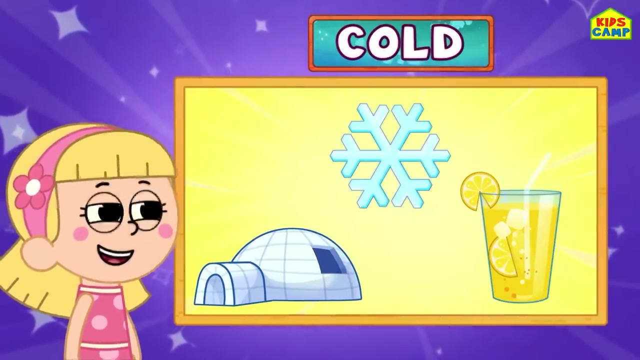 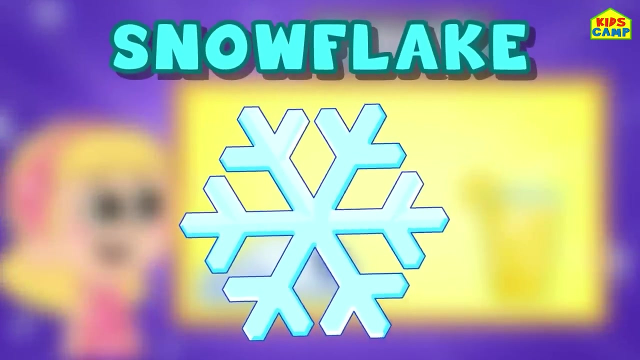 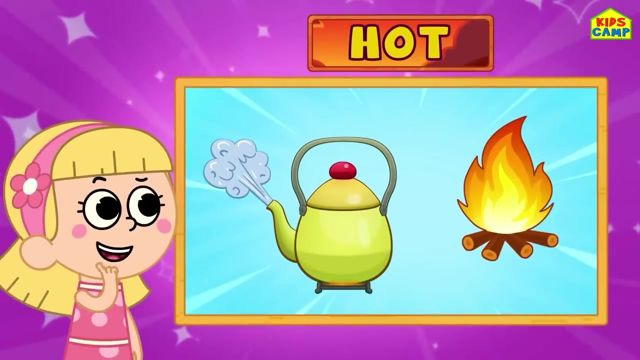 That's cold. Fire, That's hot, Definitely hot. Good job, friends. And a snowflake, That's cold. Wonderful, What did we learn? An igloo is cold, That's right, A snowflake is cold And a glass of lemonade is definitely cold. 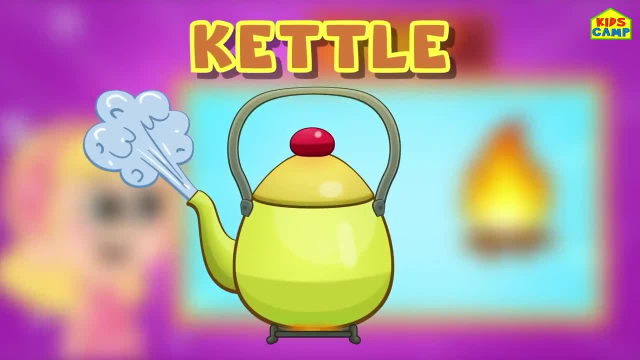 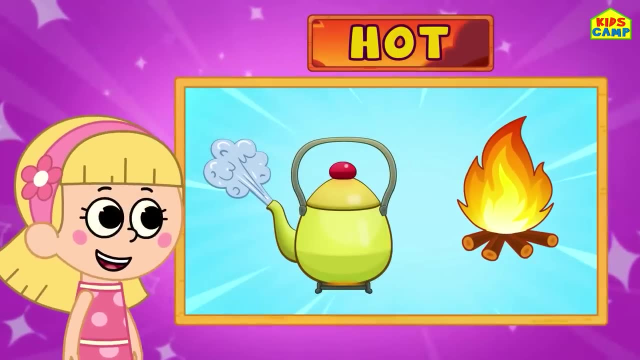 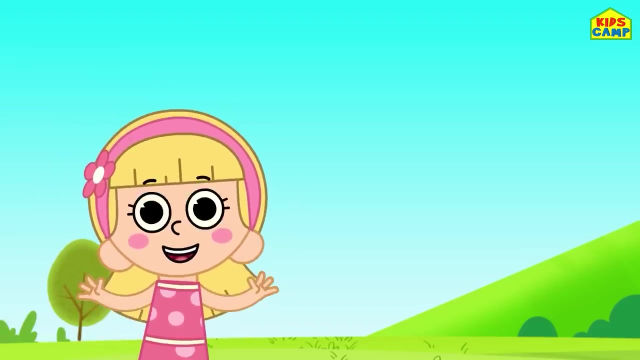 A kettle is hot And fire is hot. Wonderful, Yay. This is so much fun learning. Come back for more. Until then, keep watching Kids' Camp. Bye, Hi kids. I'm Ellie And today is Eva's birthday. 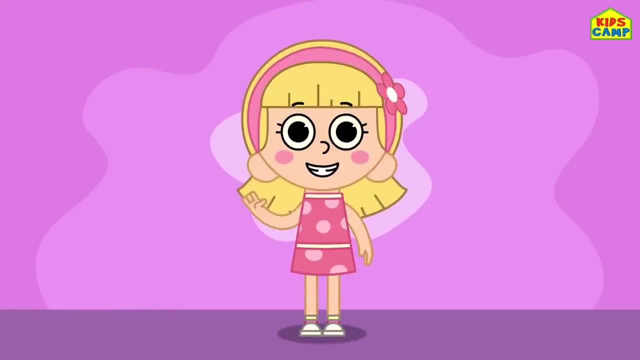 Yay, Will you help me plan a birthday party for her? Yes, Let's go First. we'll need a birthday cake. Let's bake one. Hmm, How many layers of sponge do we add to Eva's birthday cake? One? 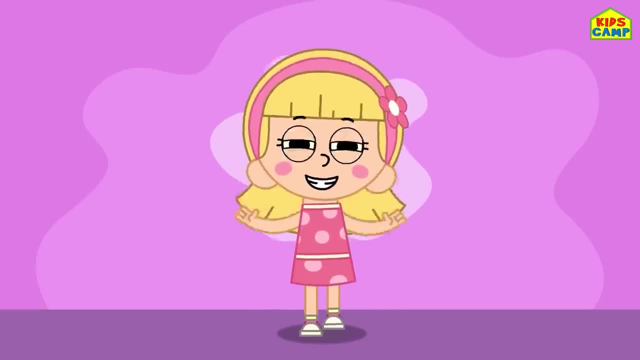 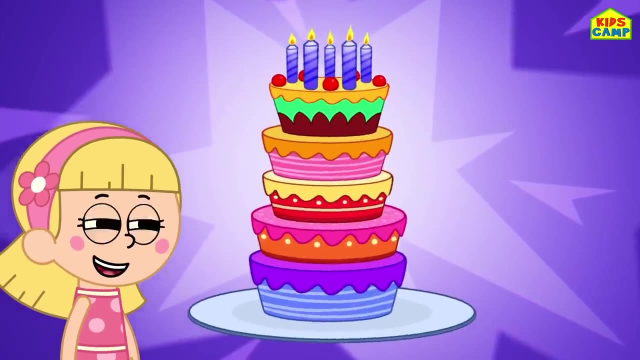 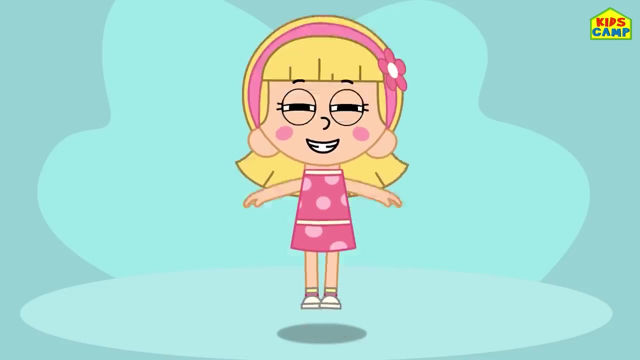 Two, Three, Four, Five, Six, Seven, Eight, Nine, 10!, 11!, 12!, 13!, 14!, 15!, 16!, 17!, 18!, 19!, 20!, 21!. 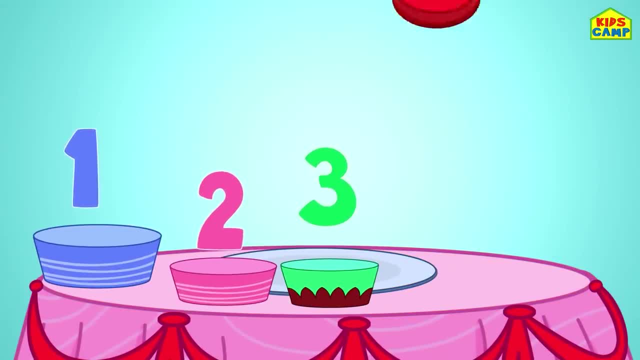 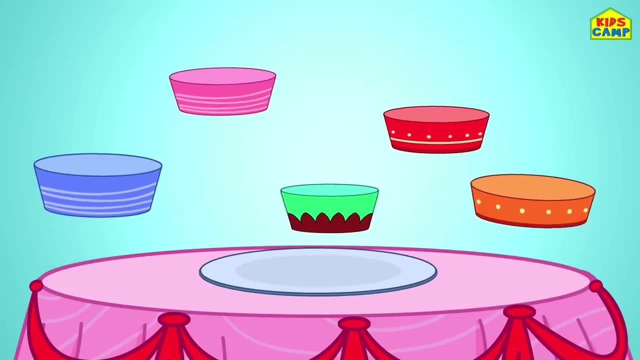 22!, 23!, 24!, 25!, 26!, 27!, 28!, 29!, 30!, 31!, 32!, 33!, 34!, 35!, 36!, 37!, 38!. 39!, 40!, 41!, 42!, 43!, 44!, 45!, 46!, 47!, 48!, 49!, 50!, 51!, 52!, 53!, 54!, 55!. 56!, 57!, 58!, 59!, 60!, 61!, 62!, 63!, 64!, 65!, 67!, 68!, 68!, 69!, 69!, 70!, 70!. 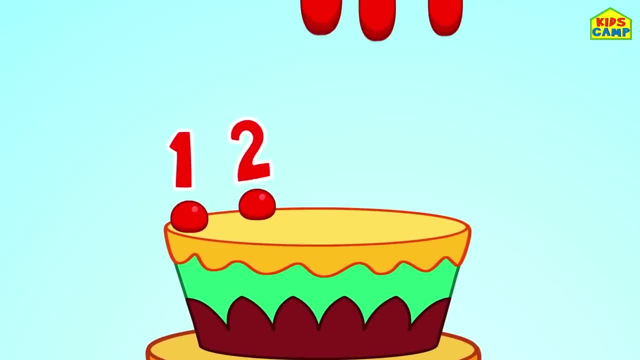 71!, 72!, 72!, 73!, 74!, 75!, 76!, 77!, 78!, 78!, 79!, 79!, 80!, 80!, 80!, 81!, 81!. 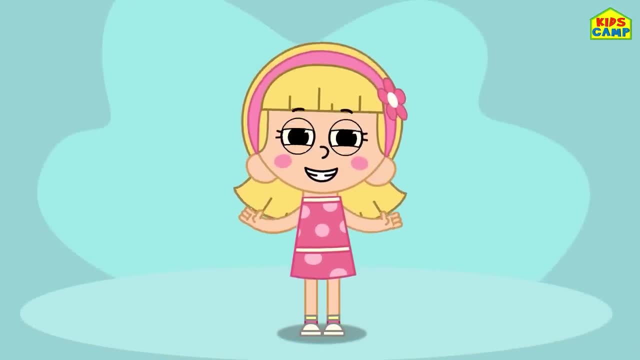 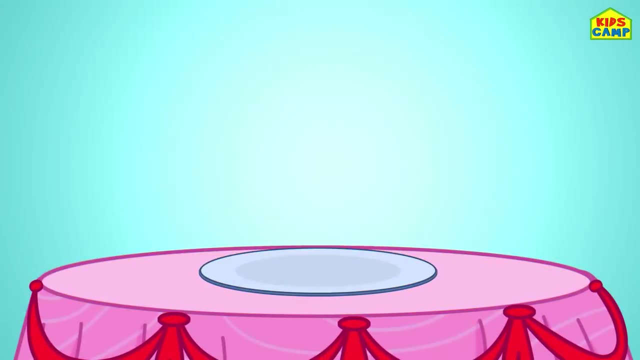 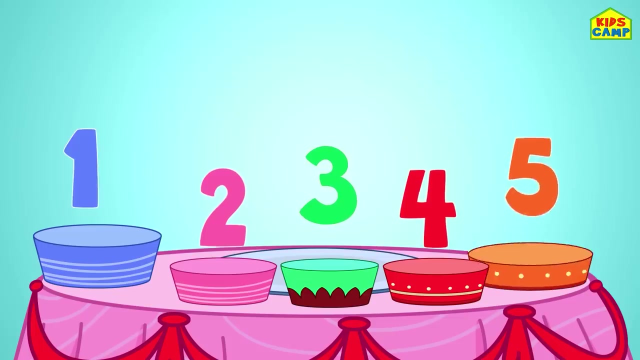 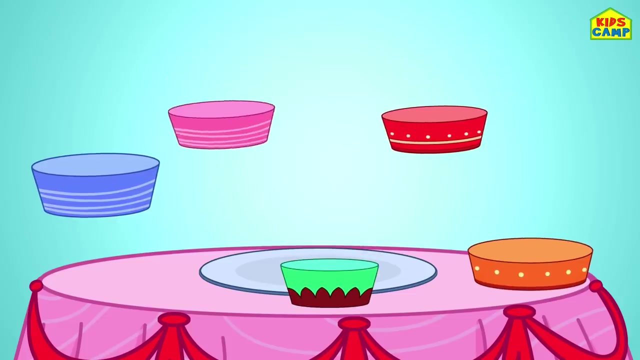 First, we'll need a birthday cake. Let's bake one. How many layers of sponge do we add to Eva's birthday cake? Let's count One, Two, Three, Four, Five, Five layers of cake, Yay, What else can we add on the cake? 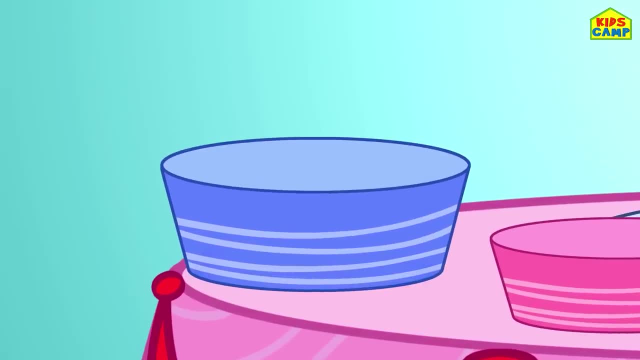 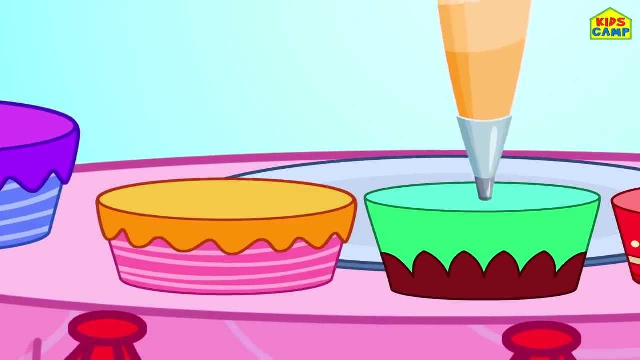 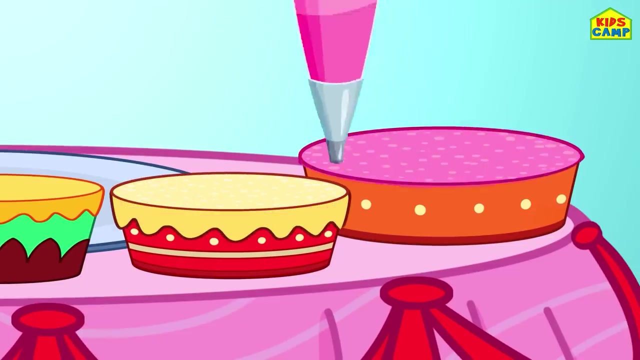 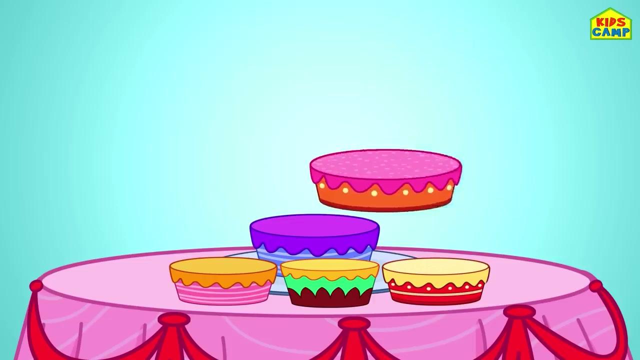 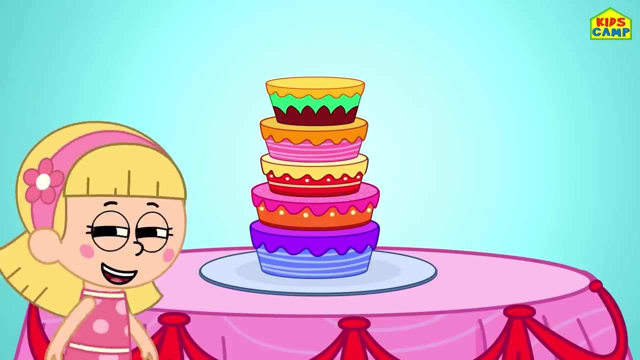 That's right. Icing, Let's add. on the first layer, on the second, on the third, on the fourth and the fifth and the fifth: Woohoo, Five layers of icing. It looks yummy, Wow. Now let's add toppings, Let's add. 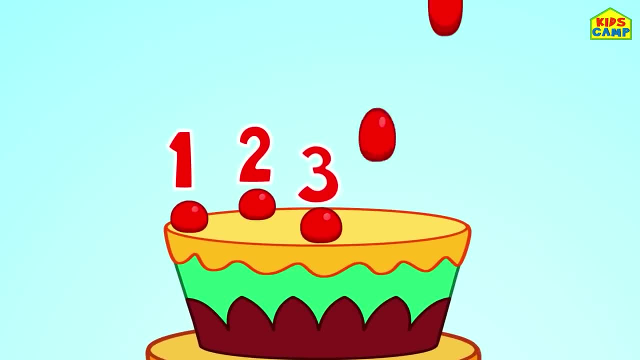 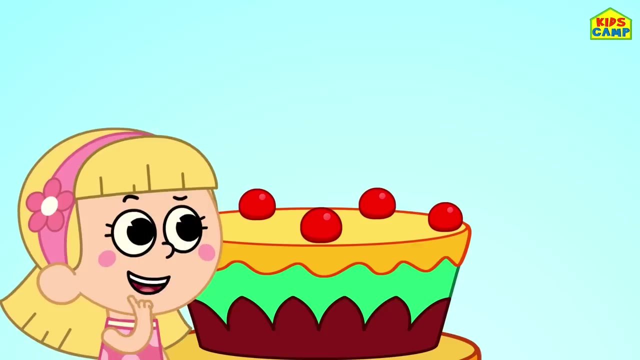 one cherry, two cherries, three cherries, four cherries, five cherries, Yay, Five cherries, Woohoo, Hmm, What do you think is missing? Hmm, Candles. That's right, Let's add candles. 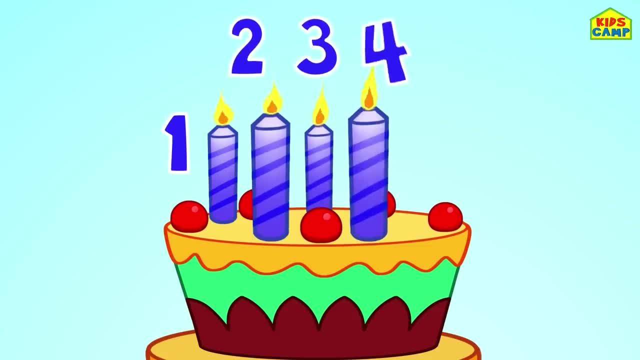 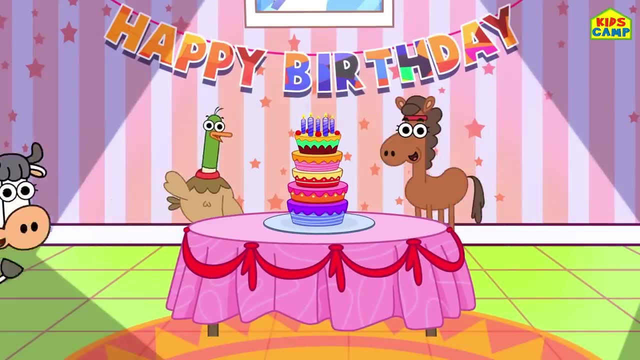 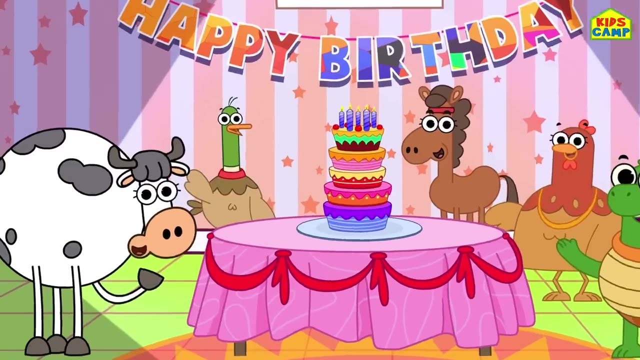 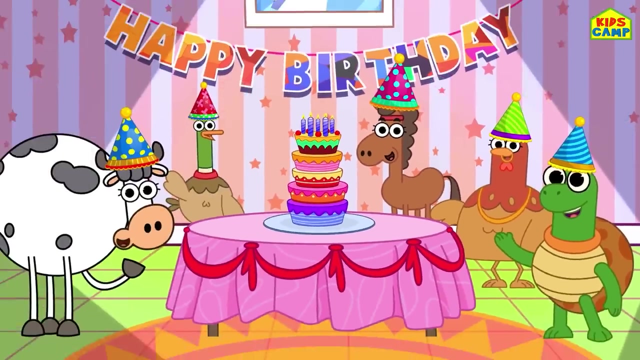 One candle, two candles, three candles, four candles, five candles. Yay, Wow, Everyone's here. Hi everyone. We need party hats. How many party hats do we need? One, two, three, four, five, Five party hats. 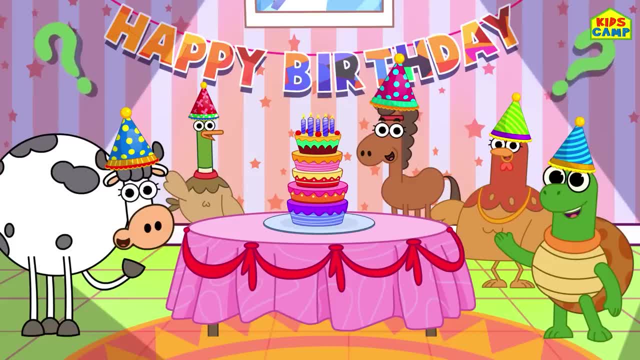 Hmm, What else do we need? Hmm, Something's missing. That's right, We need balloons. One, two, three, four, five, Five balloons. Woohoo, This is now starting to look like a birthday party. Everyone's got presents for Eva. 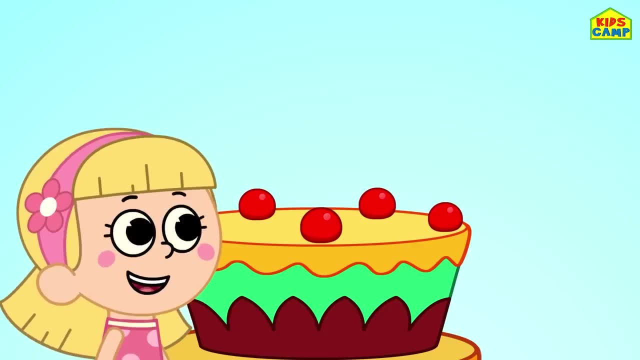 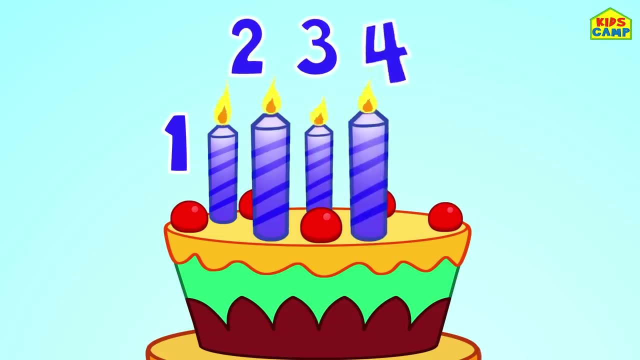 82!, 82!, 83!, 83!, 84!, 84!, 85!, 86!, 87!, 86!, 87!, 88!, 88!, 89!, 90!, 90!, 91!. 92!, 93!, 93!, 94!, 95!, 96!, 97!, 98!, 99!, 99!, 100!, 100!, 200!, 1!, 2!, 1! 2!. 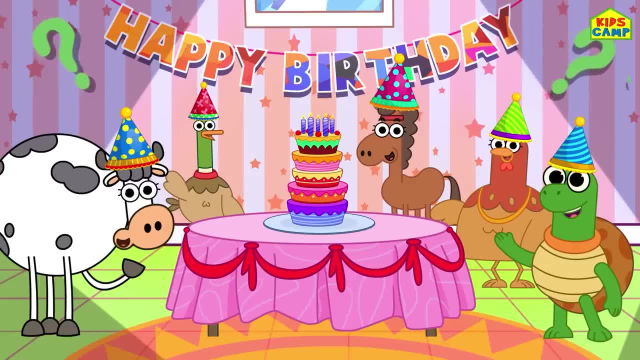 3!, 3! 3! 2! 3! 1! 2! 1! 2! two, three, four, five, Five balloons- Woohoo, This is now starting to look like a birthday. 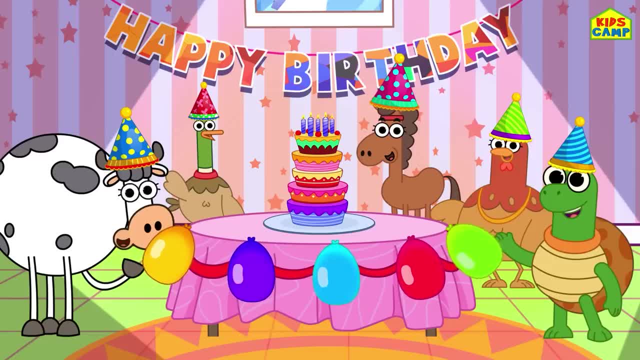 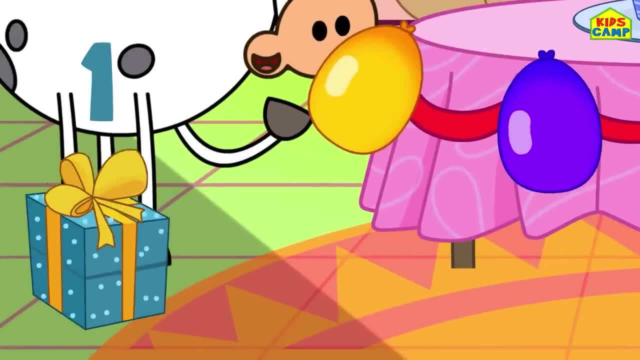 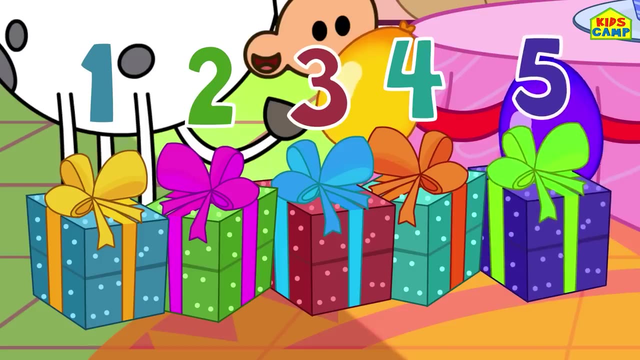 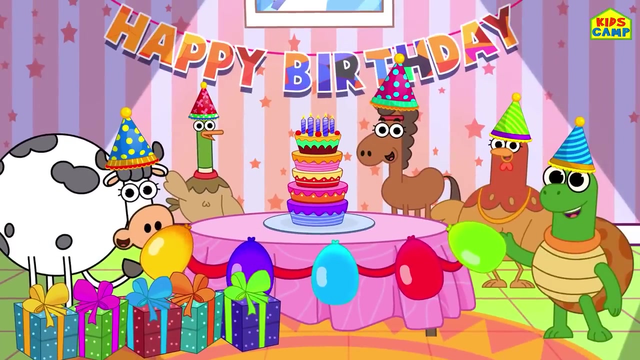 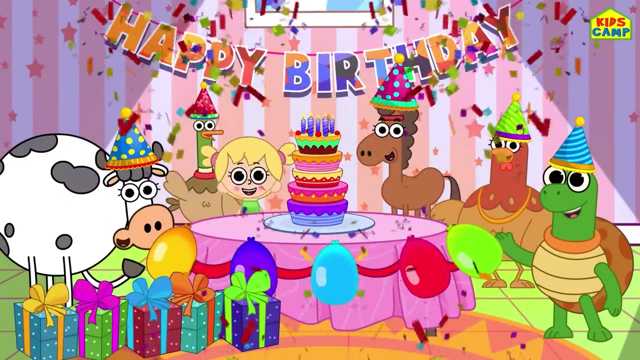 party. Everyone's got presents for Eva. Let's keep them here And count. Here we go: One, two, three, four, five, Five presents. Let's get this party started. Where's Eva? There she is Surprise. Happy birthday Eva. This was so much fun, And so is counting. Let's 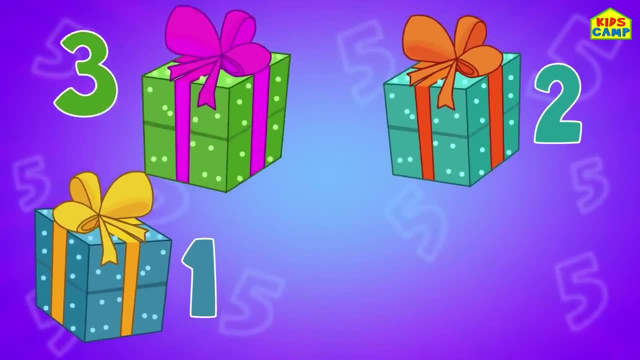 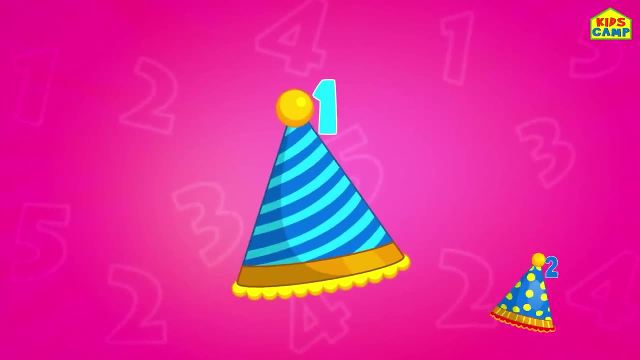 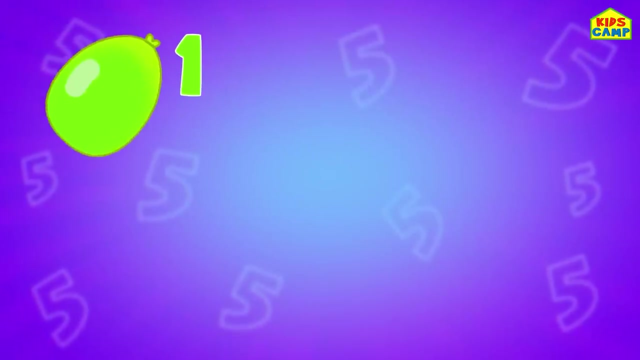 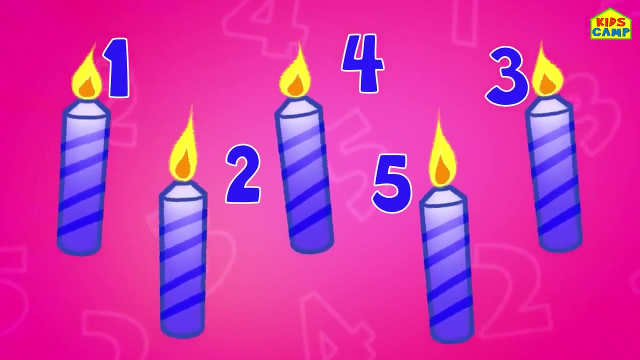 do it again. One, two, three, four, five, Five presents: One, two, three, four, five, Five. party hats: One, two, three, four, five, Five. balloons: One, two, three, four, five, Five. candles: One, two, three, four, five. Five presents: One, two, three, four, five Five presents: One, two, three, four, five Five presents: One, two, three, four, five, Five layers of cake. This was so much fun. It was the best party ever. Bye, bye. 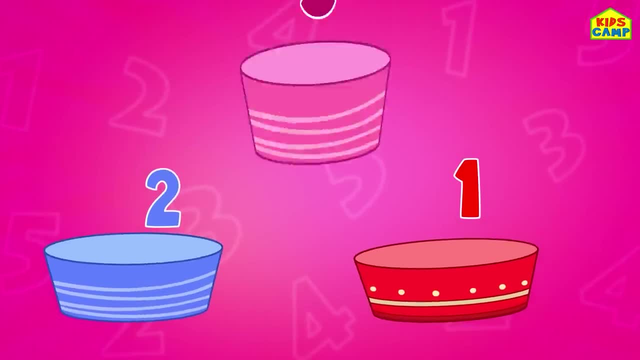 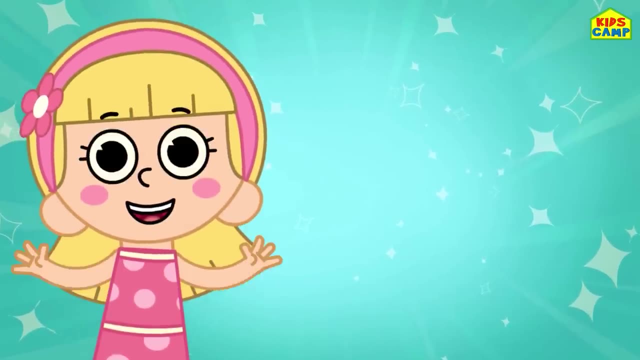 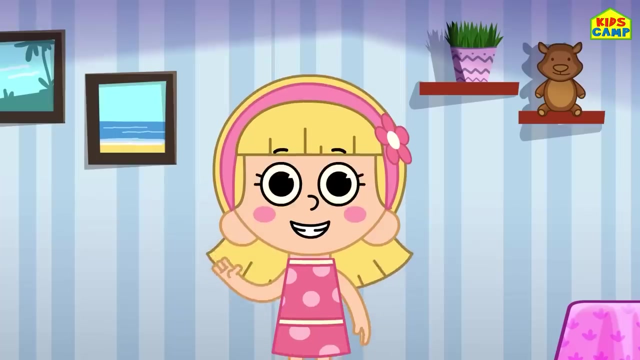 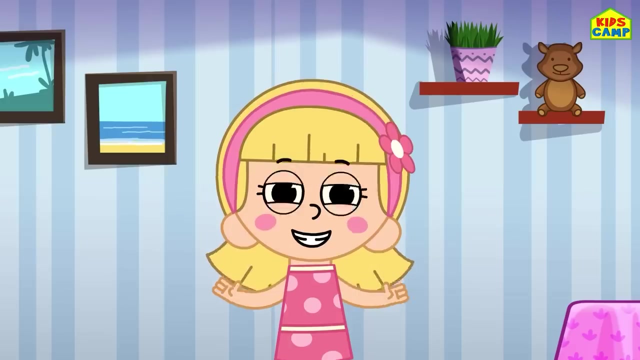 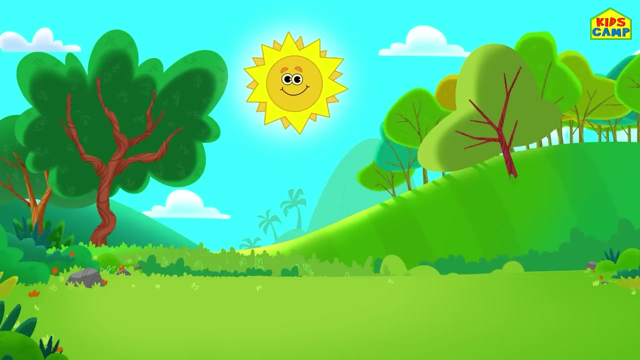 Hi, I'm Ellie, and today we are going to learn opposites. What is an opposite? An opposite is when two words contradict each other. For example, if it's daytime, the opposite of day is night. Right Ready, Here we go. 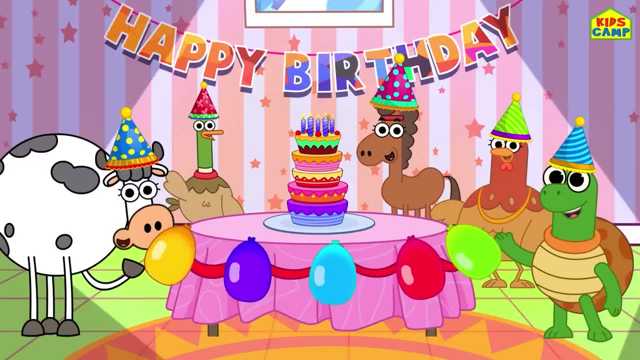 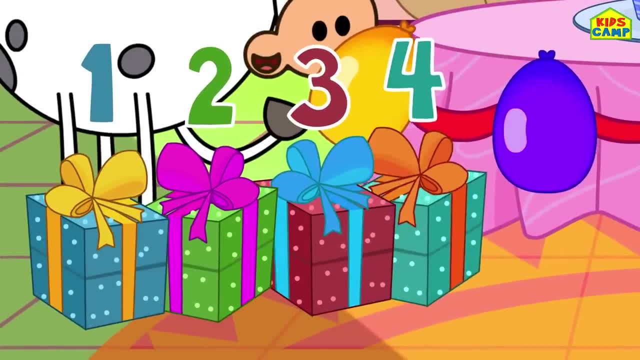 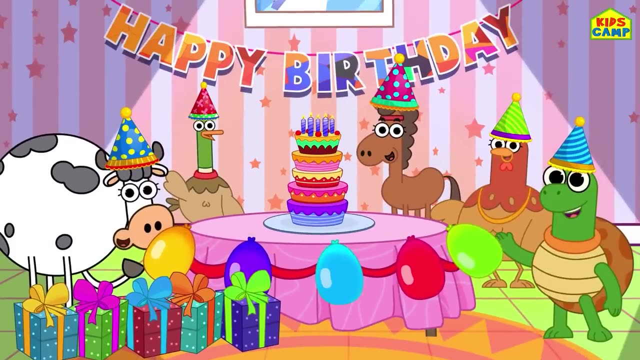 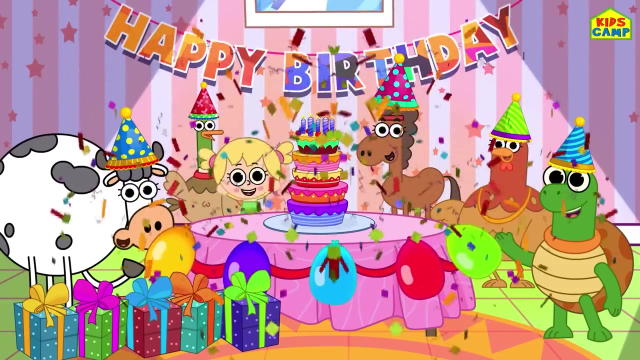 Let's keep them here And count. Here we go: One, two, three, four, five, Five presents. Let's get this party started. Where's Eva? There she is. Surprise. Happy birthday, Eva. This was so much fun. 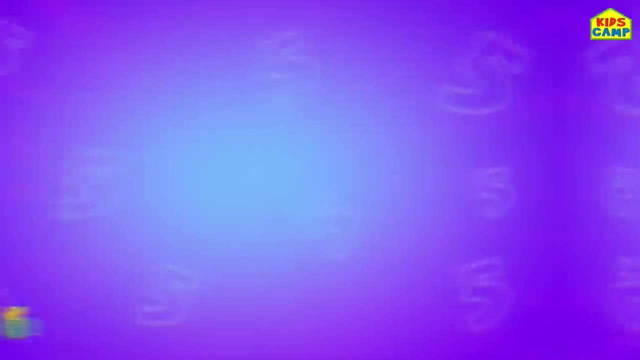 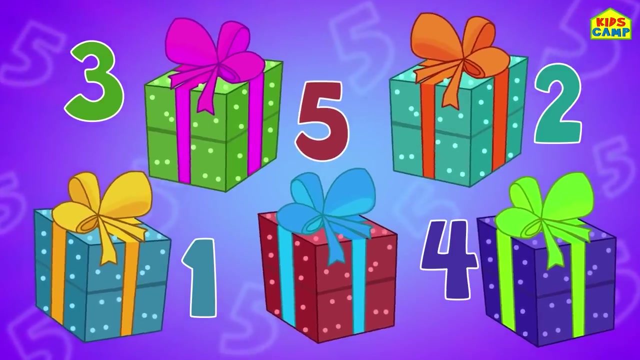 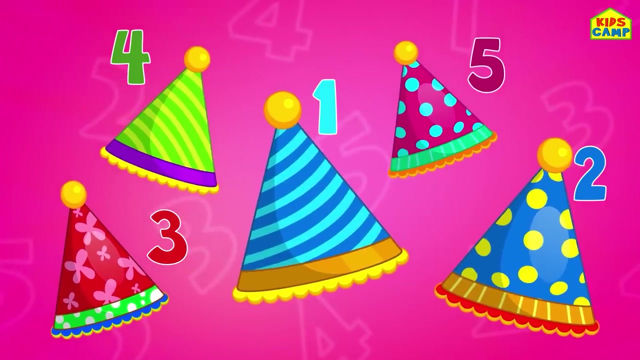 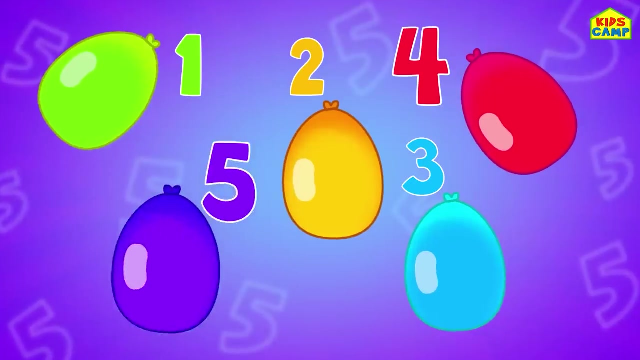 And so is counting. Let's do it again. One, two, three, four, five Five. presents: One, two, three, four, five Five. party hats: One, two, three, four, five, Five balloons: 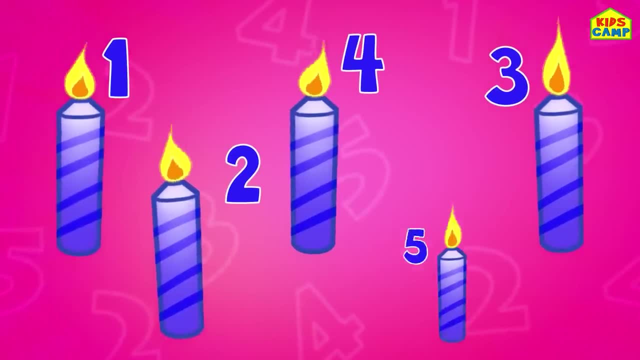 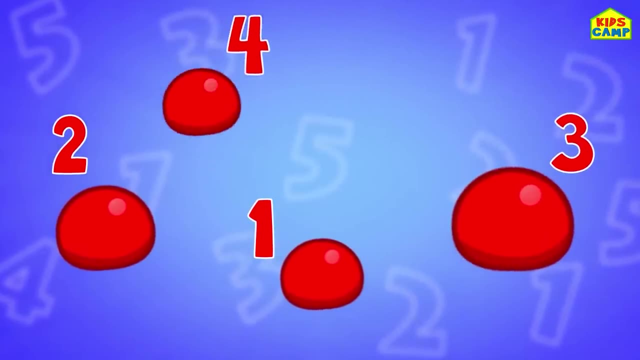 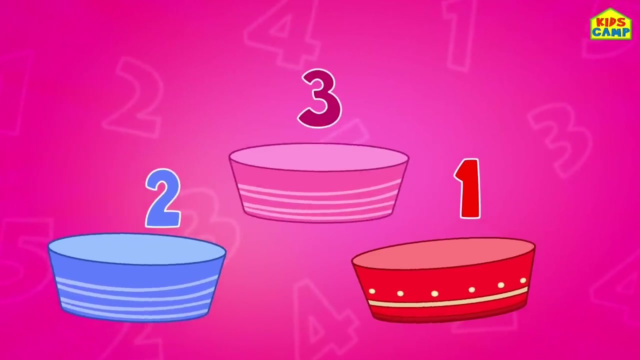 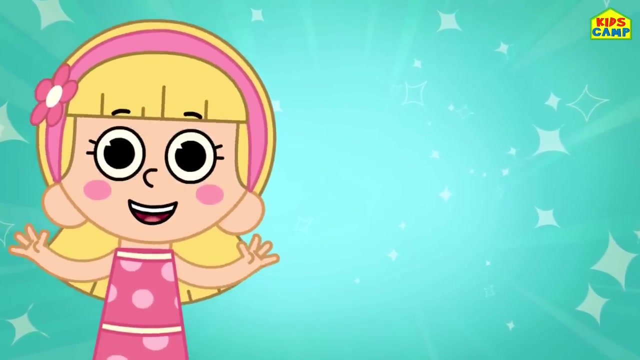 One, two, three, four, five, Five candles: One, two, three, four, five. Five. cherries: One, two, three, four, five. This was so much fun. It was the best party ever. Bye-bye. 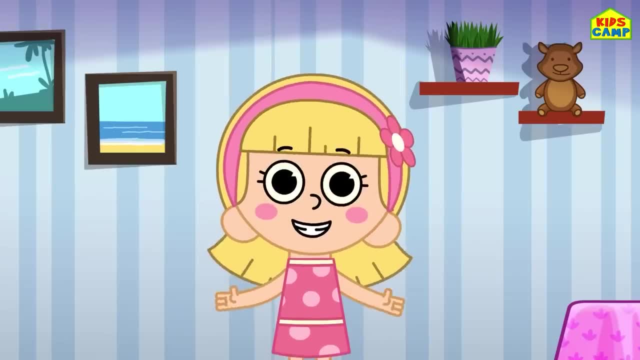 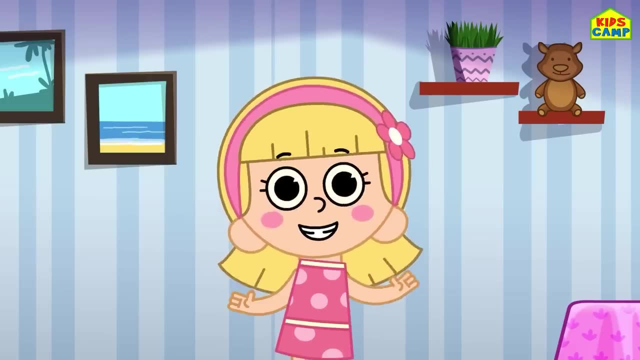 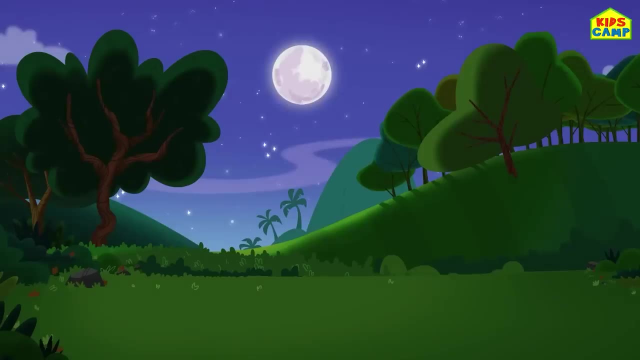 Hi, I'm Ellie, And today we are going to learn opposites. What is an opposite? An opposite is when two words contradict each other. For example, if it's daytime, the opposite of day is night. Right Ready, Here we go. 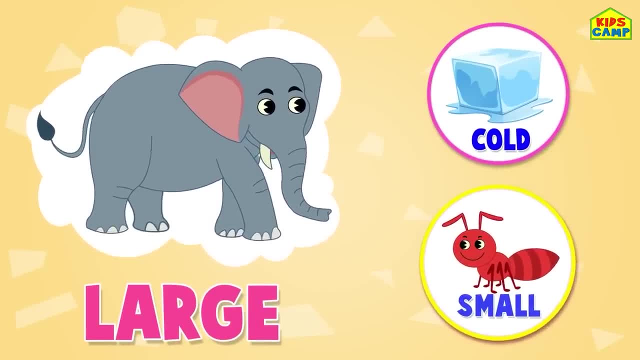 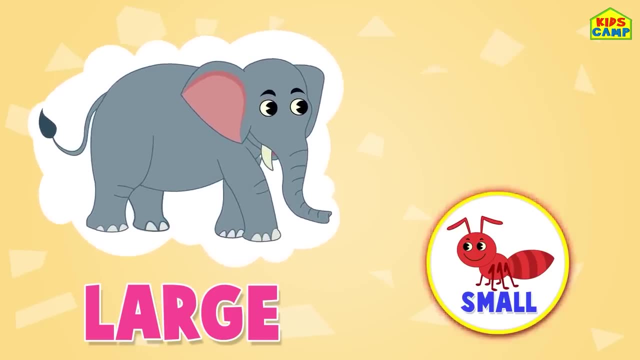 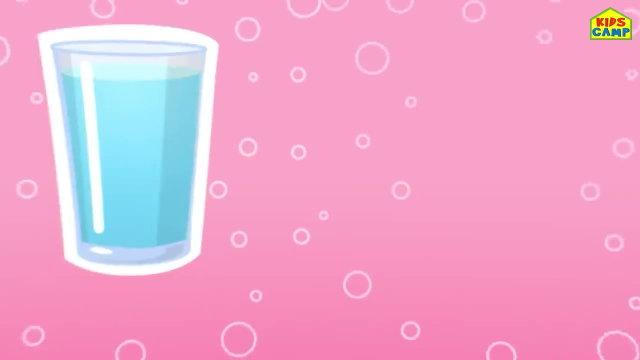 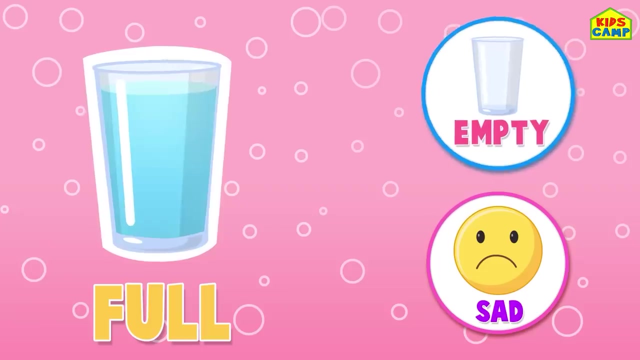 What is the opposite of large? Is it small Or cold? It's small, That's right. The opposite of large is small. What is the opposite of full? Is it sad Or is it empty? The opposite of full is empty. 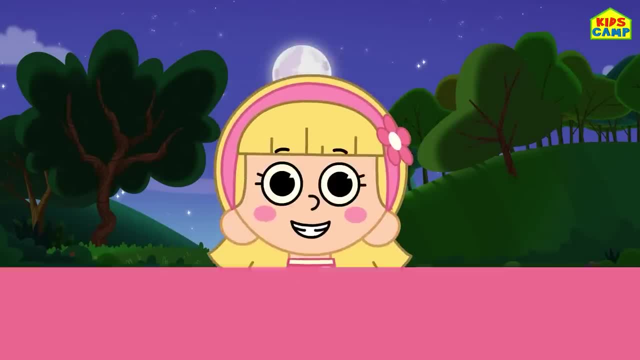 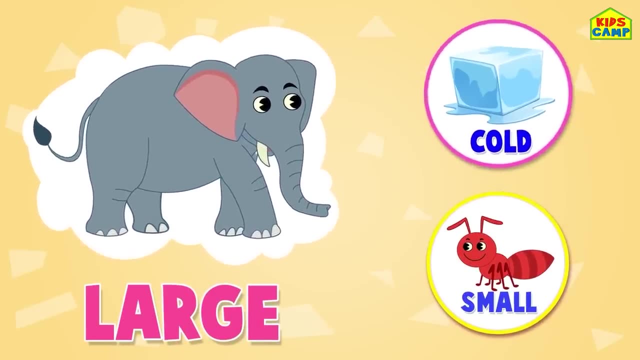 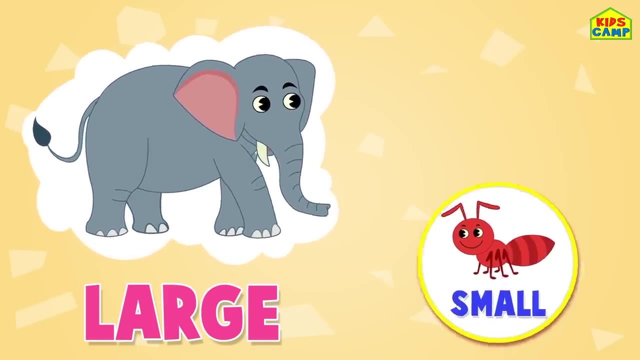 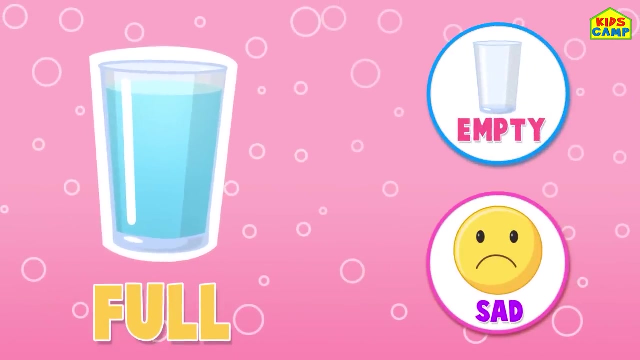 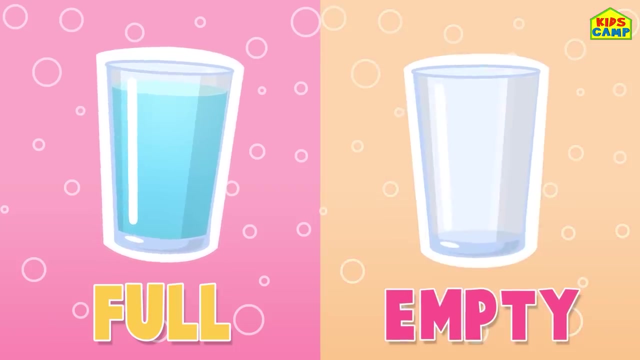 What is the opposite of large? Is it small or cold? It's small, That's right. The opposite of large is small. opposite of full: Is it sad or is it empty? The opposite of full is empty, That's right. 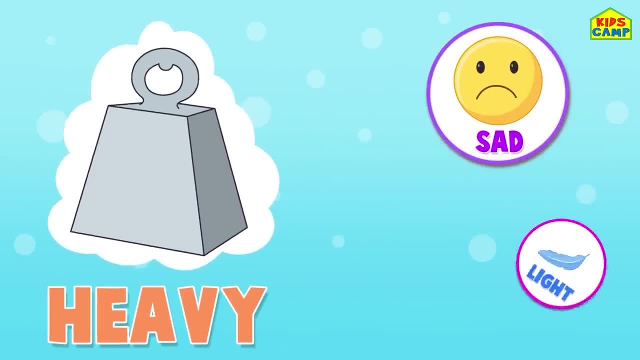 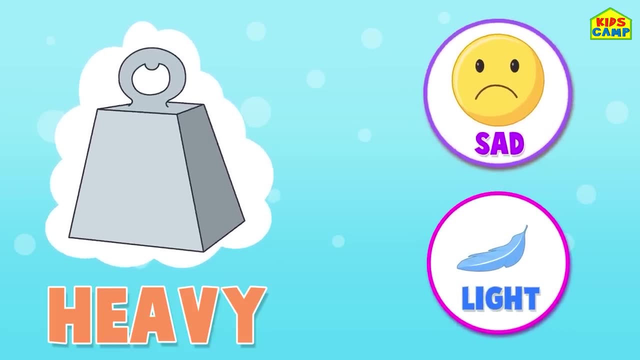 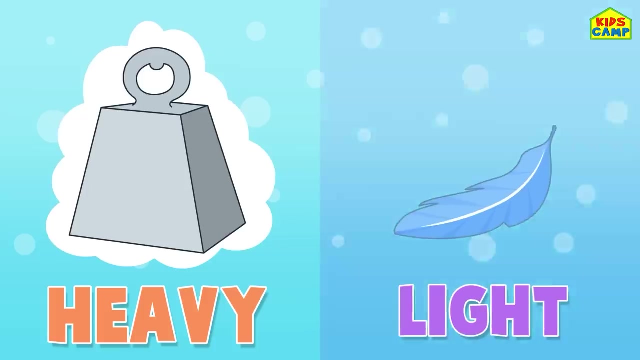 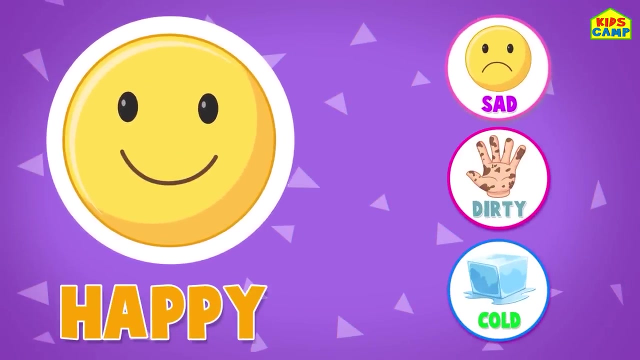 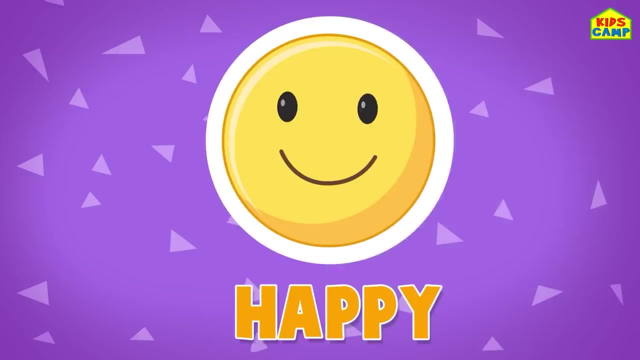 What is the opposite of heavy? Is it light or sad? It's light. The opposite of heavy is light. What is the opposite of happy? Is it sad, is it dirty or is it cold? It's sad, That's right. The opposite of happy is sad, And I feel happy right now, Yay. 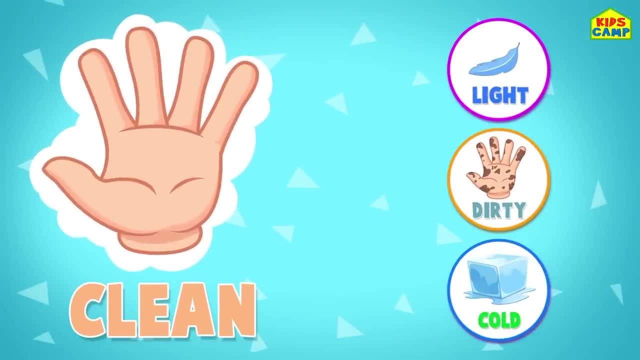 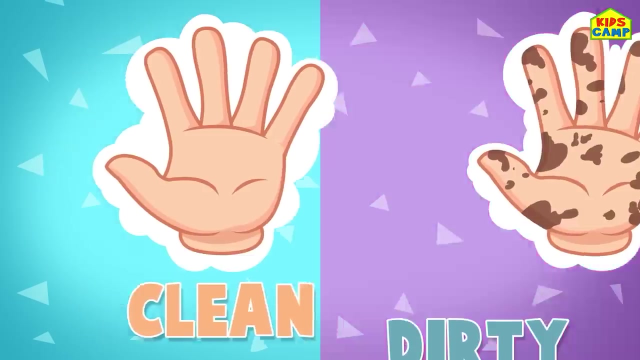 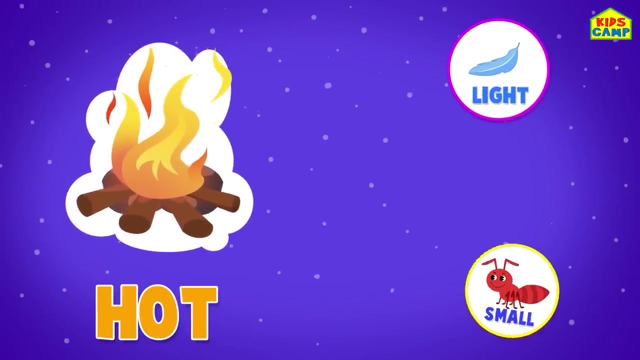 What is the opposite of clean? Is it cold, is it light or is it dirty? That's right, friends, It's dirty. You should always keep your clean clothes in the fridge. hands clean and not dirty. what's the opposite of hot? is it light, is it small or is it cold? 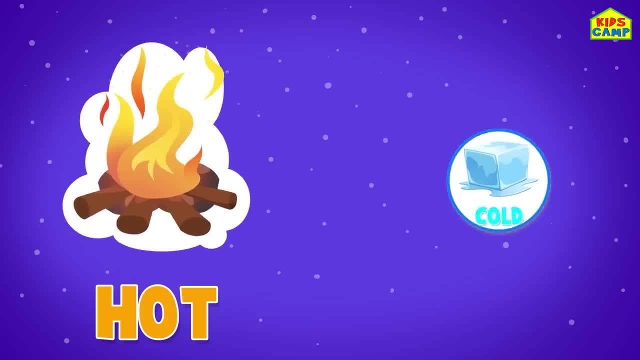 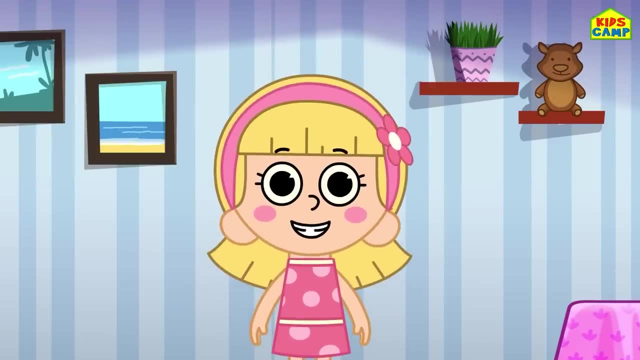 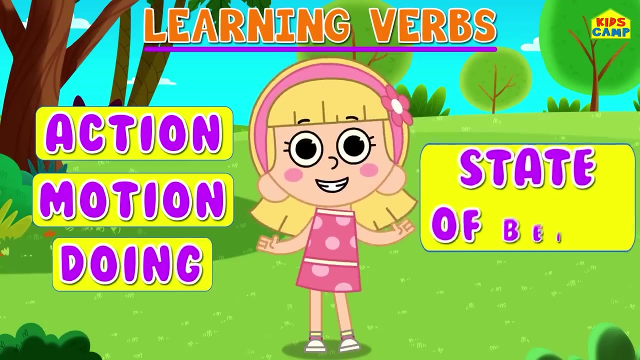 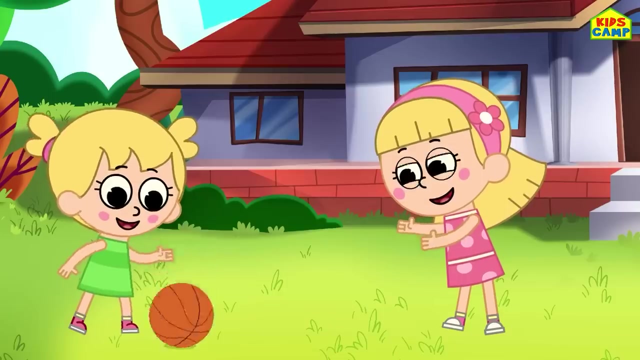 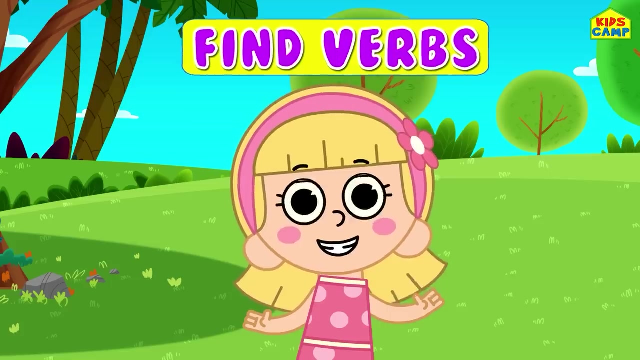 it's cold, that's right. the opposite of hot is cold. good job, friends. well done hi. verbs are words that show action, motion, doing or a state of being, and I am on a playground and I'm playing with Eva. what we are going to do today is find verbs. are you ready? we have to. 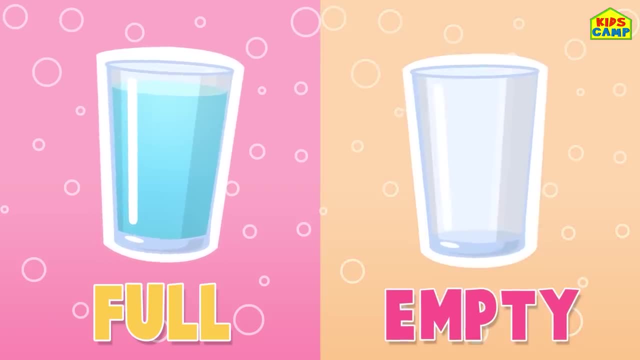 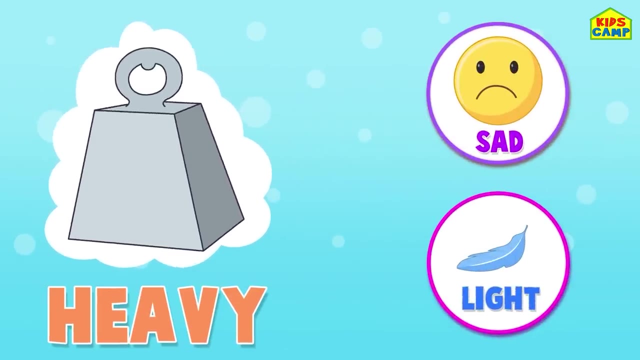 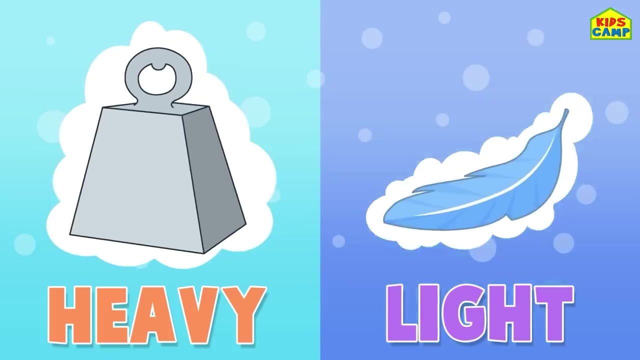 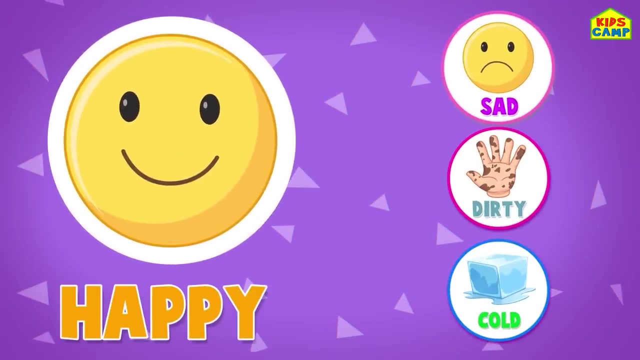 That's right. What is the opposite of heavy? Is it light Or sad? It's light. The opposite of heavy is light. What is the opposite of happy? Is it sad? Is it dirty Or is it cold? It's sad. 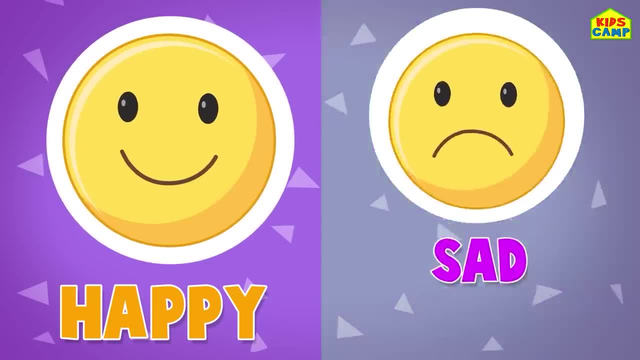 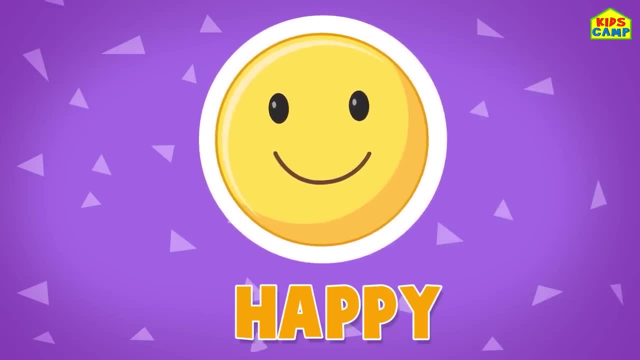 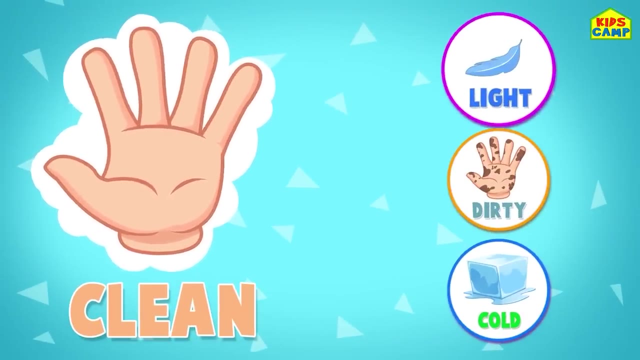 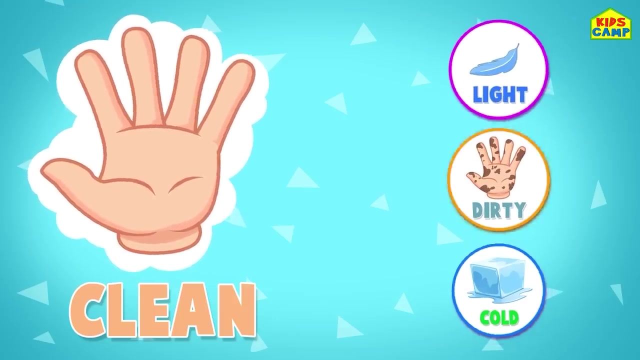 That's right. The opposite of happy is sad, And I feel happy right now, Yay. What is the opposite of clean? Is it cold, Is it light Or is it dirty? That's right, friends, It's dirty. You should always. 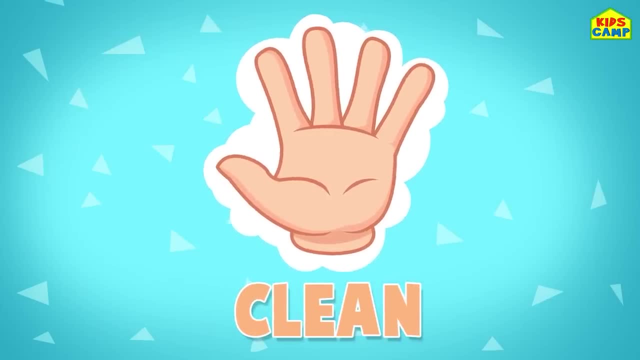 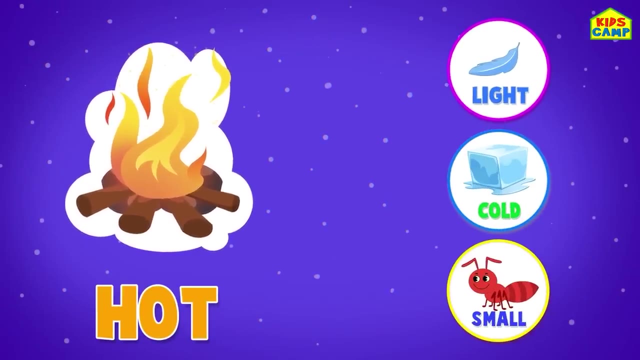 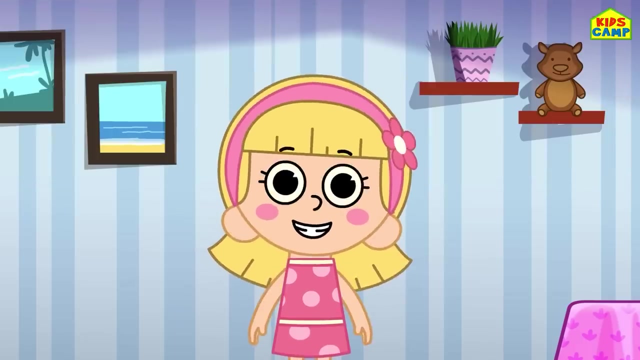 keep your hands clean and not dirty. What's the opposite of hot? Is it light, Is it small, Or is it cold? It's cold. That's right. The opposite of hot is cold. Good job, friends. Well done Hi. 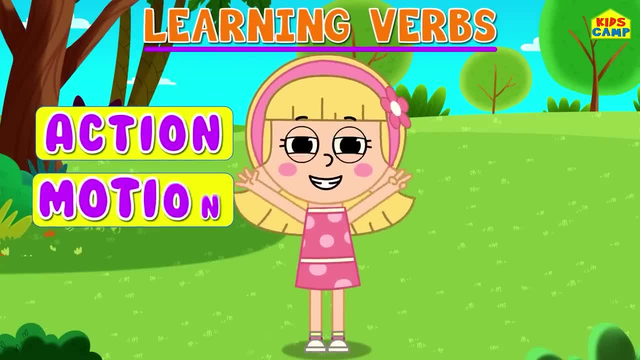 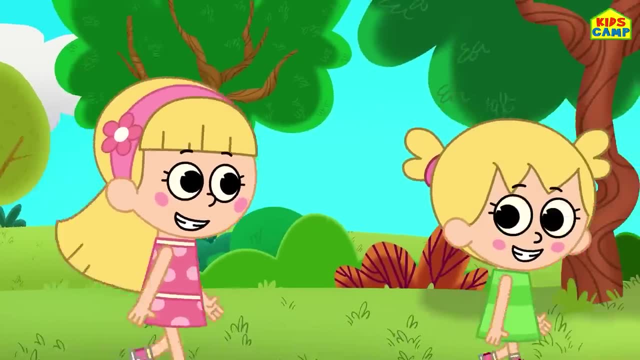 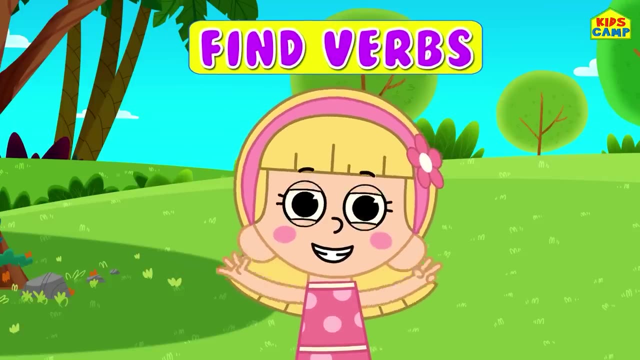 Verbs are words that show action, motion, doing or a state of being. And I am on a playground And I am playing with Eva. What we are going to do today is find verbs. Are you ready? Let's get started. 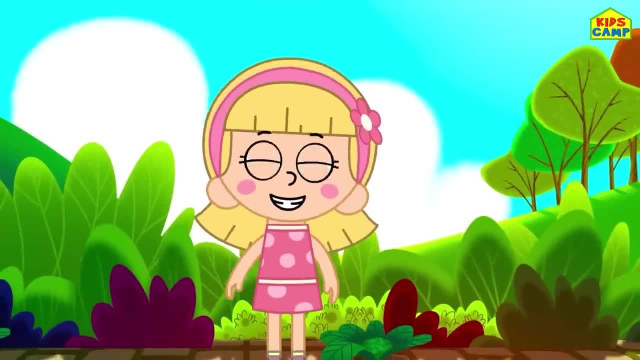 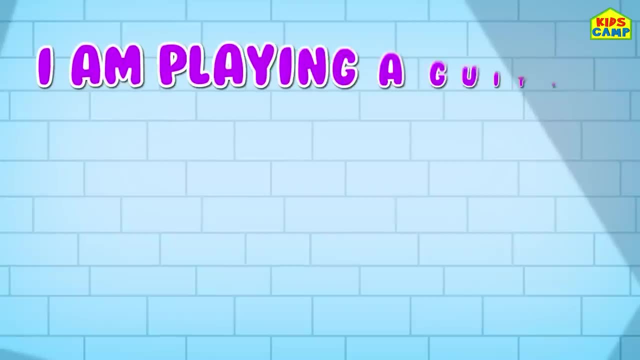 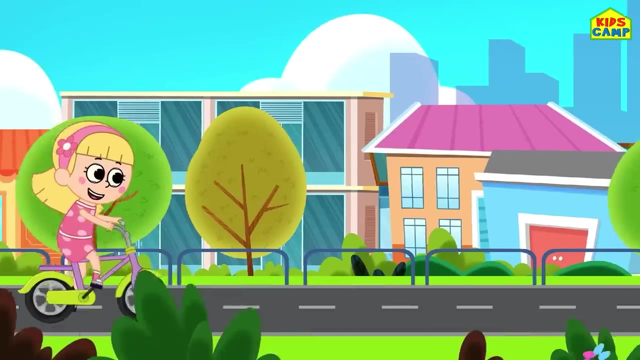 Right away. I am playing the verb. Can you find what's the verb in the sentence? I am playing the guitar. Playing is the verb here. That's right. What's the activity I am doing here? I am riding a bicycle. 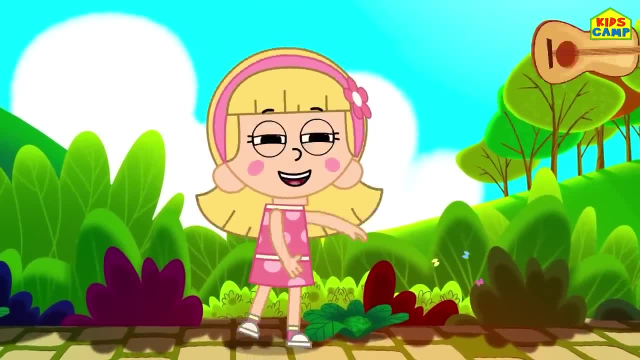 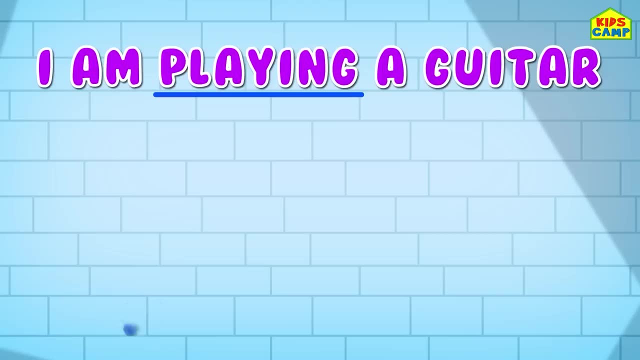 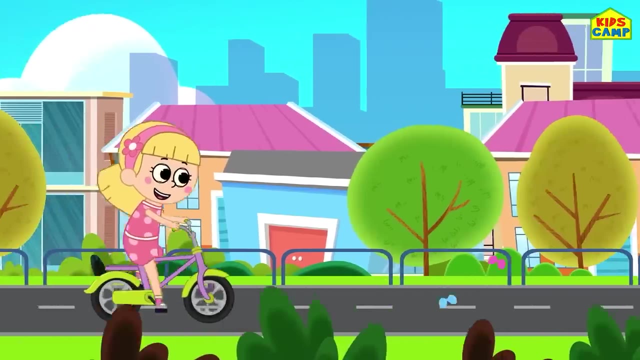 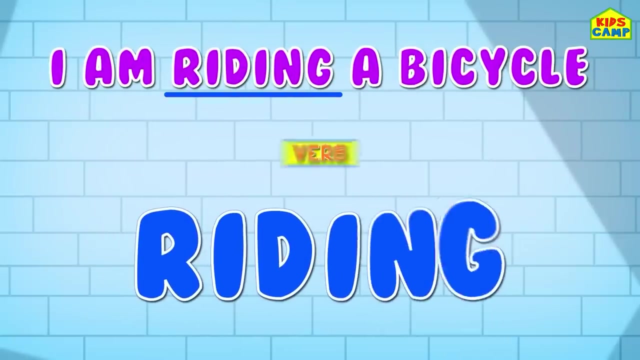 look for the world. can you find what's the world in the sentence? I am playing the guitar. playing is the world here. that's right. what's the activity I'm doing here? I am riding a bicycle. that's right. riding is a verb. look at my little sister, Eva she. 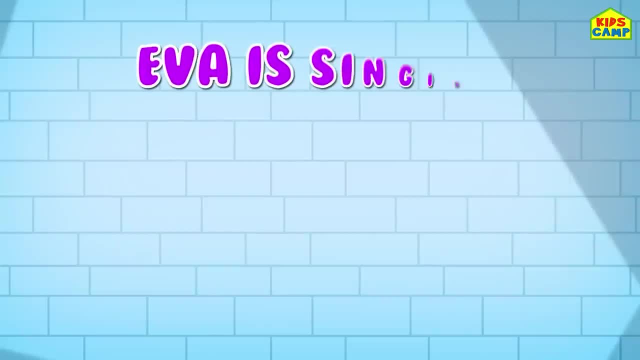 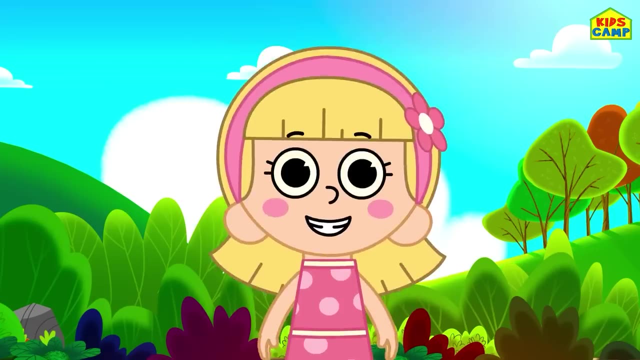 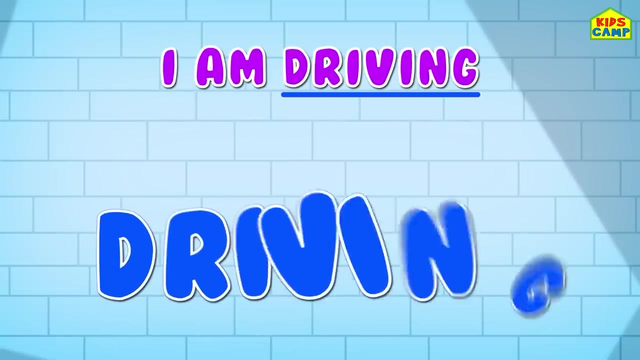 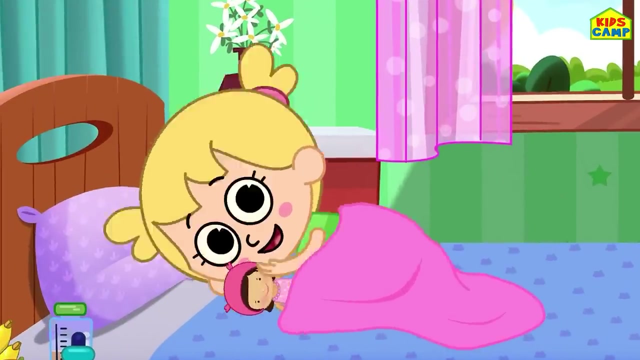 loves to sing. that's right, Eva is singing. singing is the world here? good job, friends. look at me. I am driving. that's right, driving- is the world here? and what is it that we do the first thing when we get up in the morning? that's right, we crush our cheese. 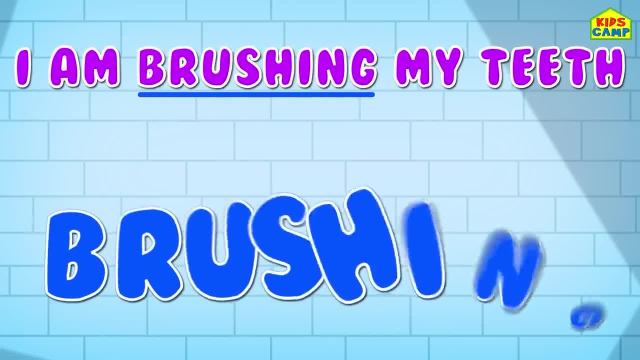 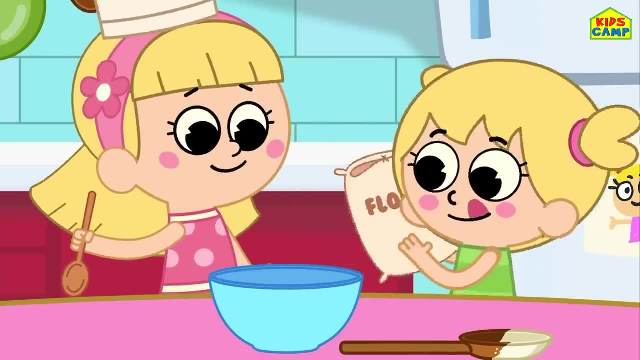 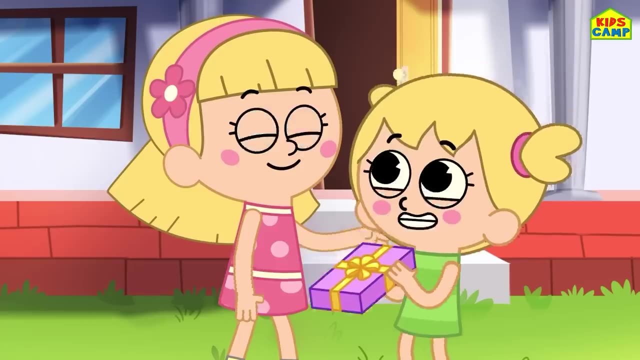 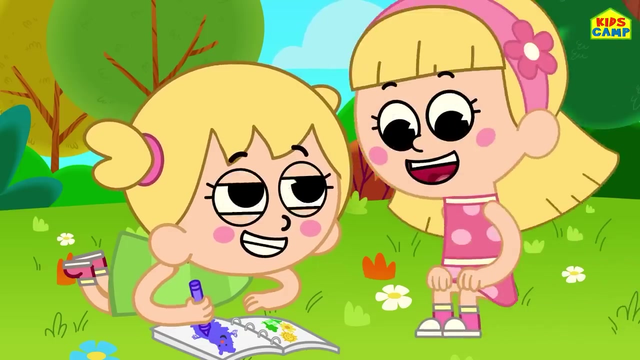 I am brushing my teeth- Brushing is the verb here, Eva- and I love to cook. I am cooking- Cooking is the verb here- And I've got a new box of crayons. I love to use my crayons to draw and color. 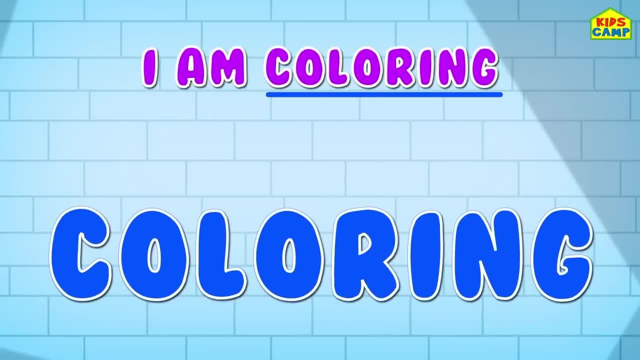 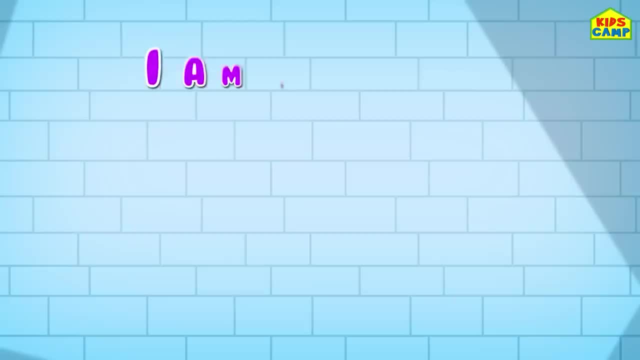 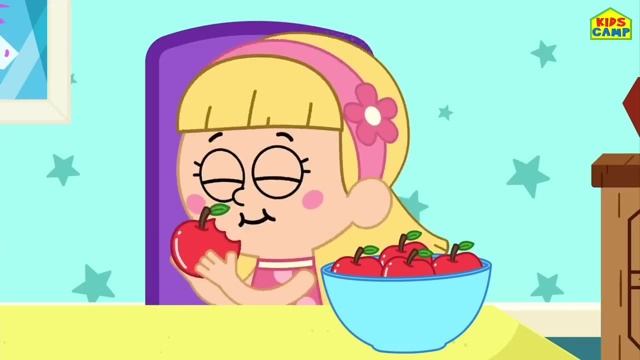 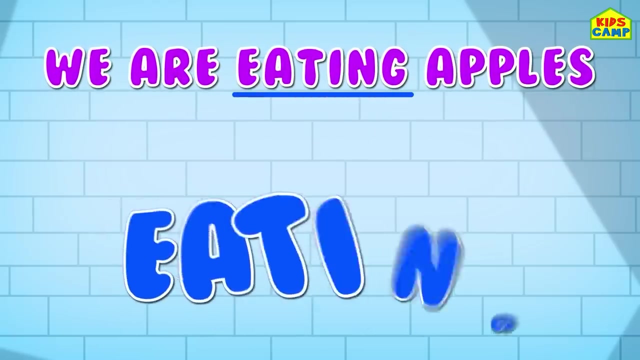 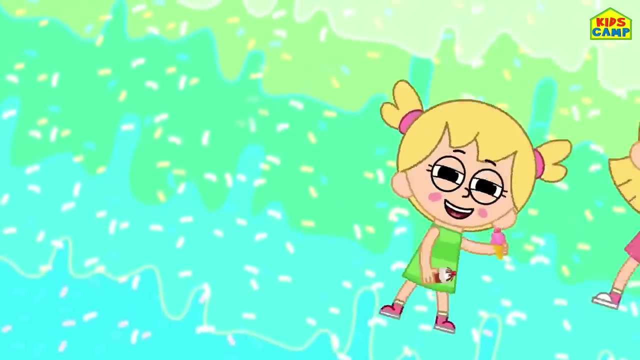 I am coloring. Coloring is the verb here. I am clapping. Clapping is the verb here. We are eating apples. We are eating apples. Eating is the verb here. That's right. We are dancing. We are dancing. Dancing is the verb here. 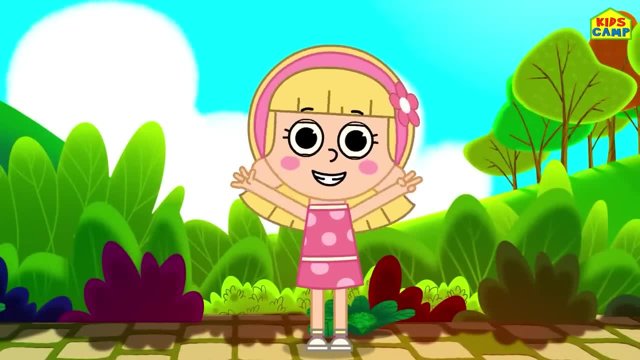 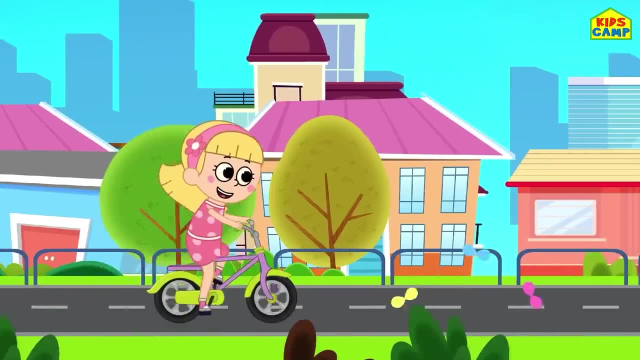 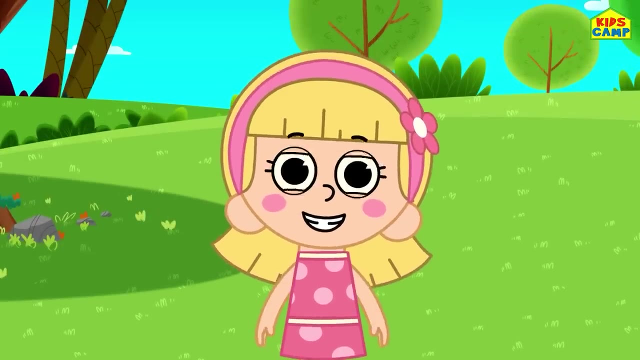 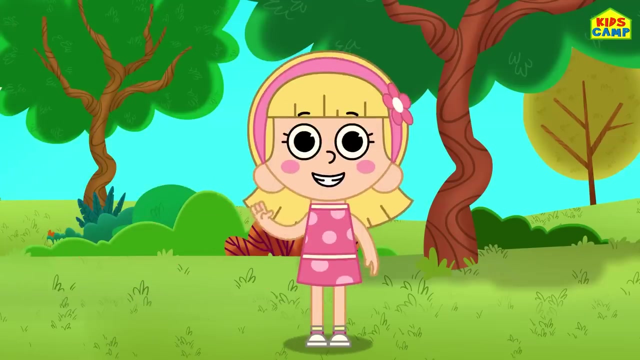 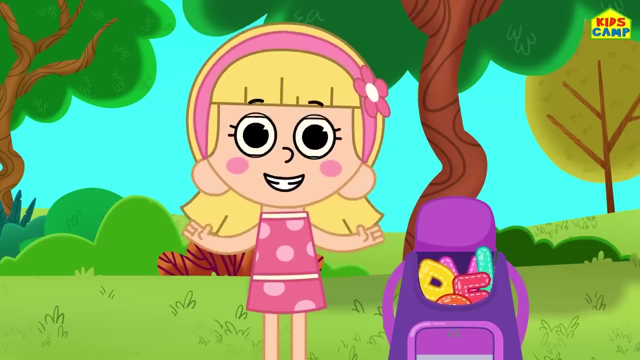 Wow, This was so much fun. What do you like to do? Do you like to cook, play guitar, paint, sing or ride a bike? Let me know. Until then, keep watching Kids' Camp. Bye-bye, I'm Ellie and I have a bag of alphabets with lots of scrambled and jumbled letters. 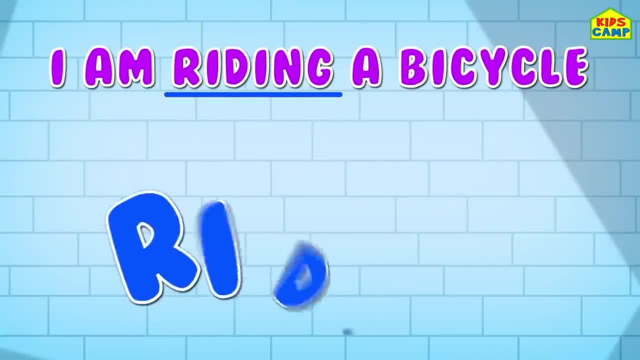 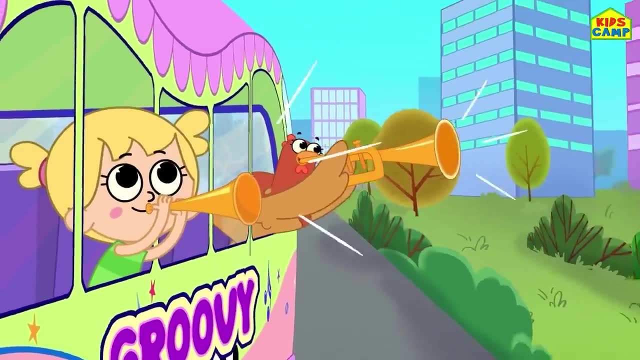 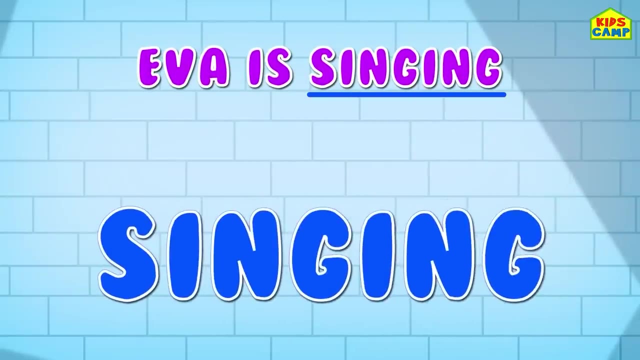 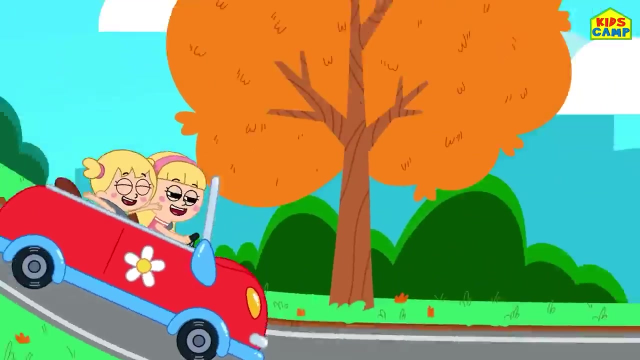 That's right, Riding is a verb. Woohoo, Look at my little sister, Eva. She loves to sing. That's right, Eva is singing. Singing is the verb here. Good job, friends. Look at me, I am driving. 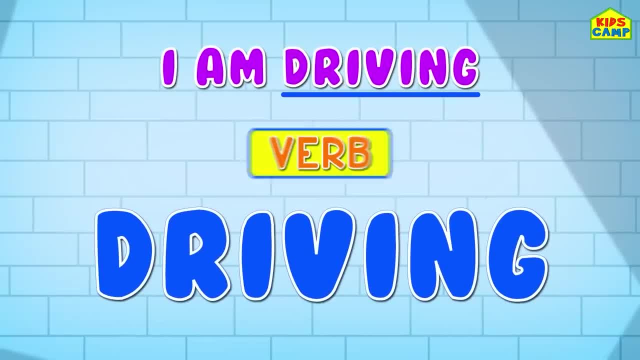 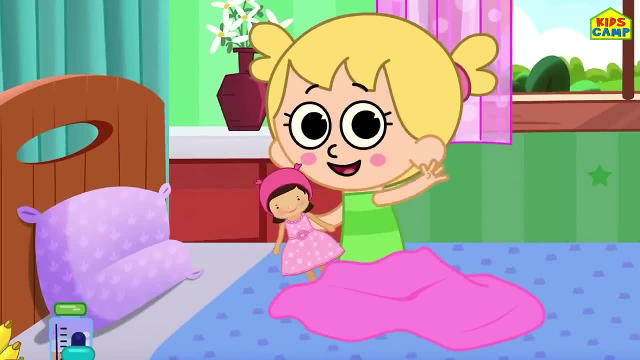 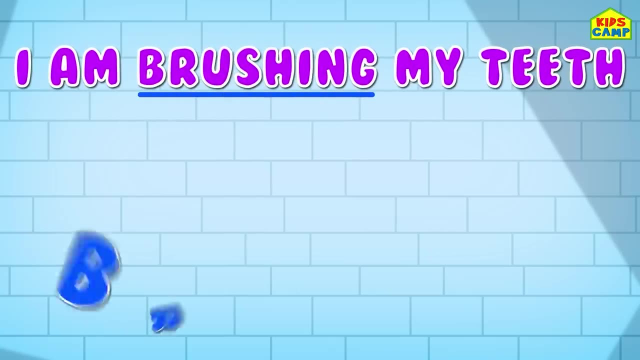 That's right. Driving is the verb here. And what is it that we do? the first thing when we get up in the morning? That's right. We brush our teeth. I am brushing my teeth. Brushing is the verb here, Eva, and I love to cook. 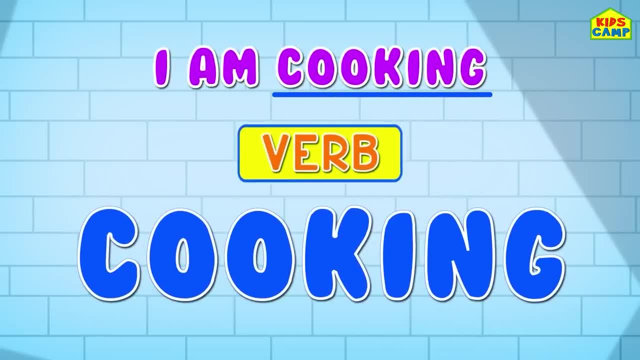 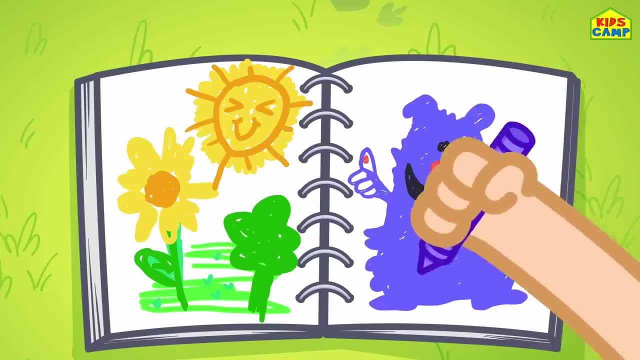 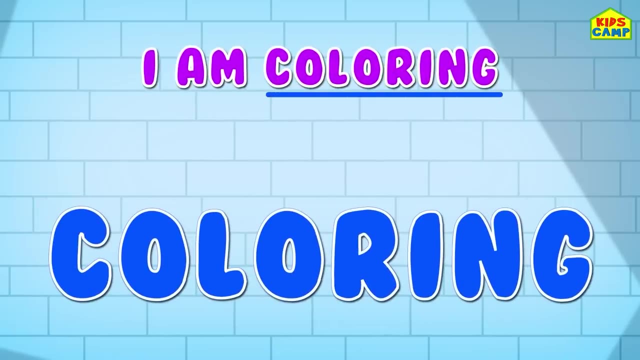 I am cooking- Cooking is the verb here- And I've got a new box of crayons. I love to use my crayons to draw and color. I am coloring. Coloring is the verb here. Woohoo, I am clapping. 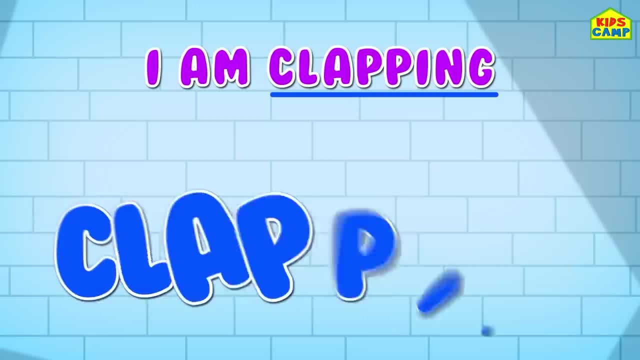 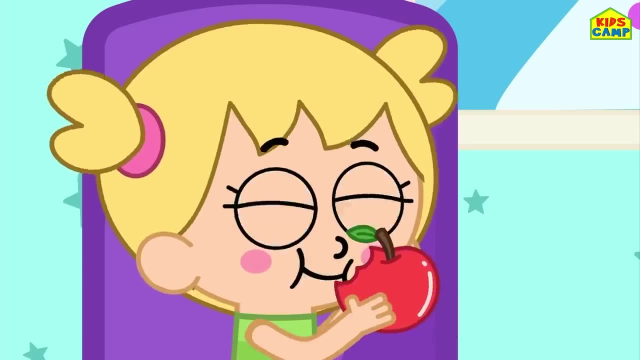 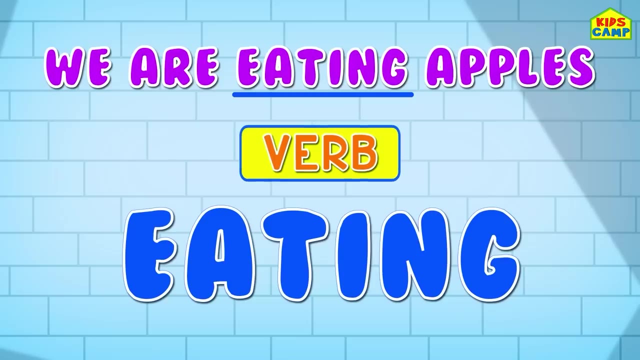 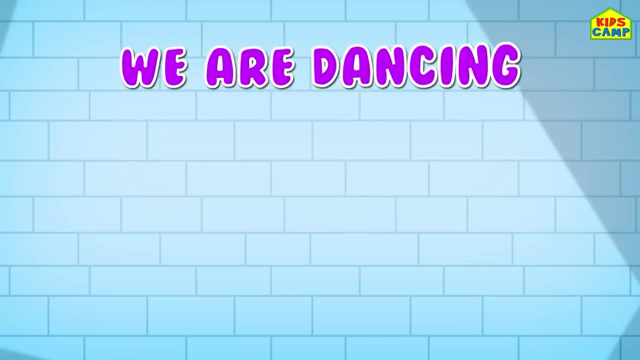 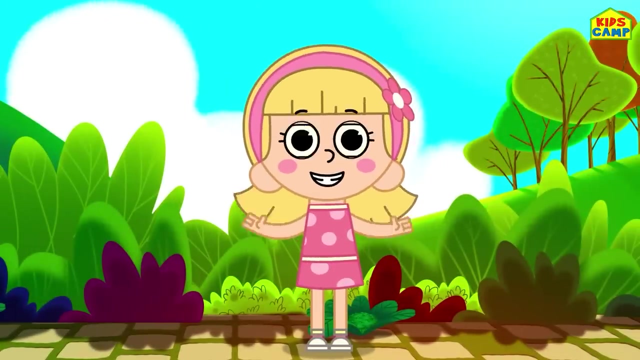 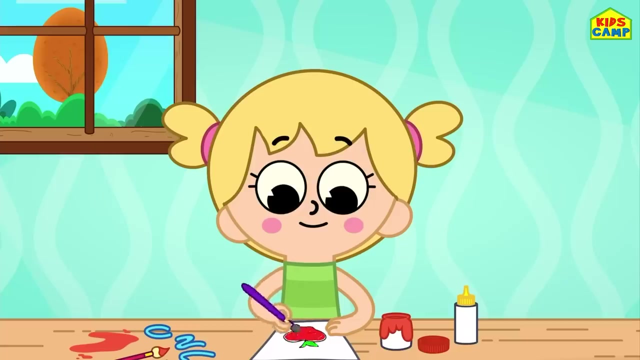 I am clapping. Clapping is the verb here? Woohoo, We are eating apples. We are eating apples. Eating is the verb here, Woohoo, That's right, we are dancing. dancing- is the world here? wow, this was so much fun. what do you like to do? do you like to cook, play guitar, paint? 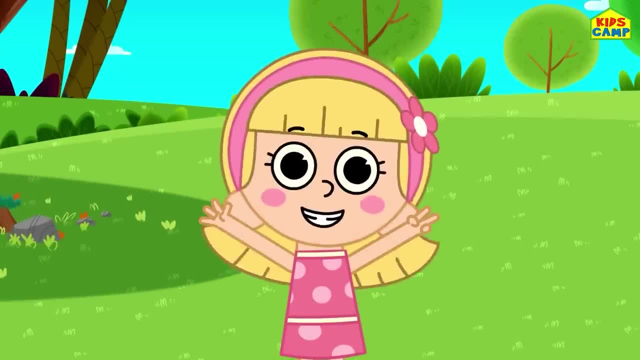 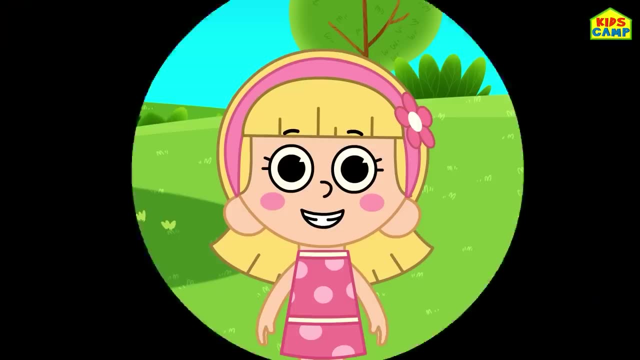 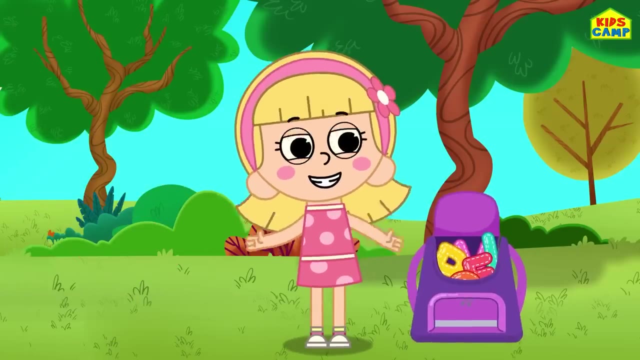 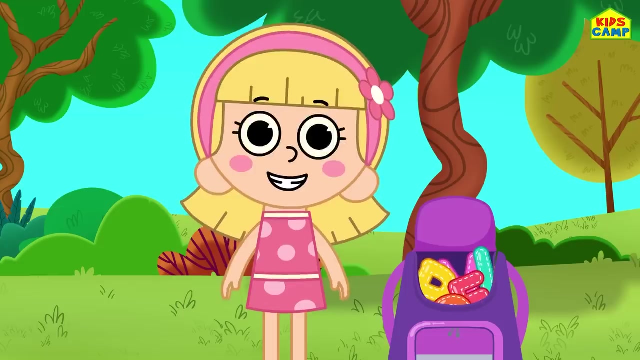 sing or ride a bike. let me know. until then, keep watching kids camp. bye, bye, hi kids. i'm ellie and i have a bag of alphabets with lots of scrambled and jumbled letters. we have to unscramble them to find the correct word. fun game, let's start. 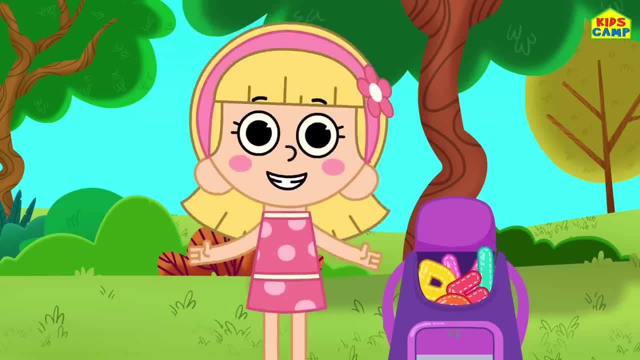 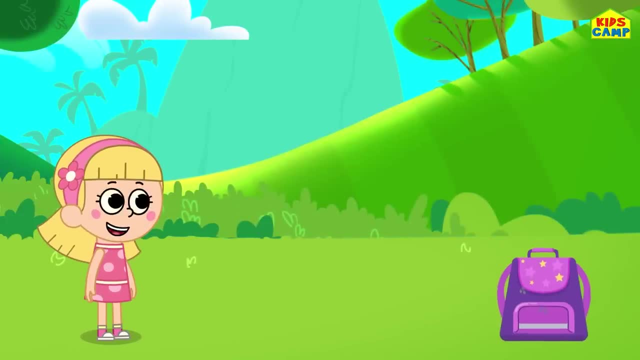 We have to unscramble them to find the correct word. Fun game. Let's start. Alright, What is this? Hmm, I wonder what it is. Ah, P, L, A, E, P. Hmm, what word could this be? 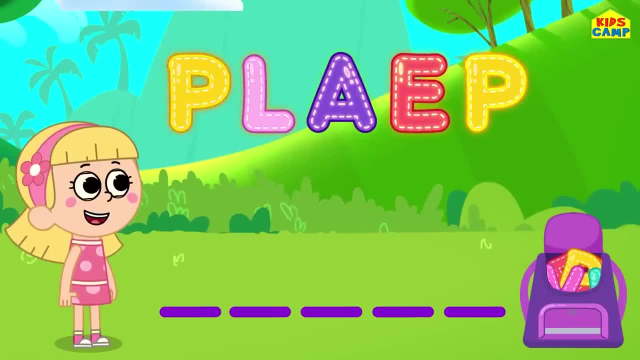 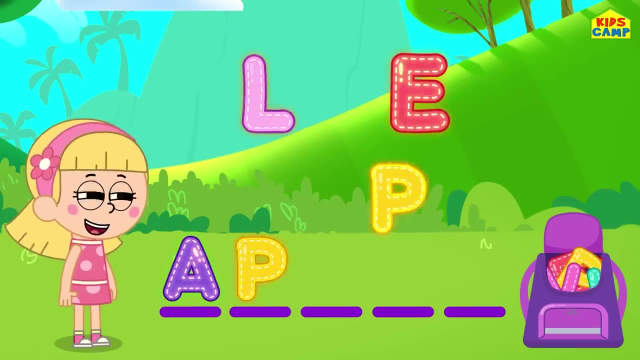 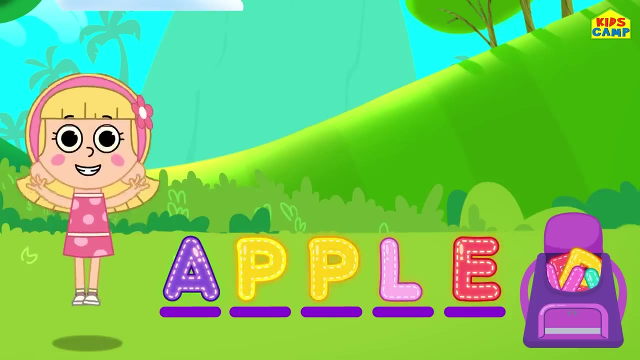 Oh, I know This is an apple. It starts with the letter A, P, P, L and E. That's right, We got it right. kids, It's an apple. Woohoo, We got the first word correctly. 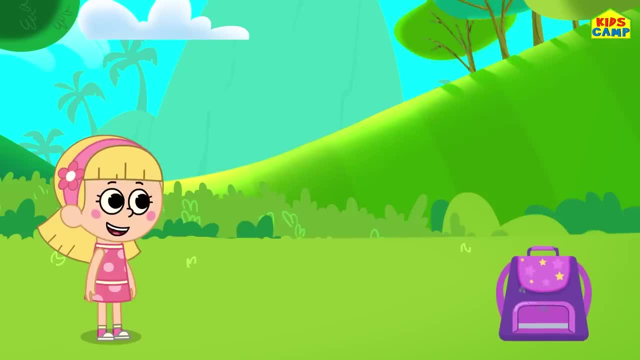 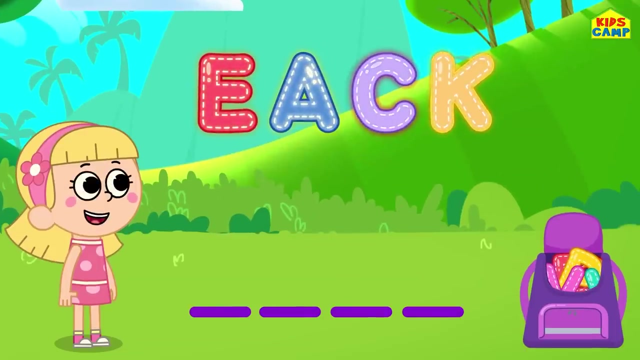 We got the first word correctly. What's next? Hmm, I wonder what could this be? The letter E, A, C and K? Hmm, this looks familiar. That's right, It's a cake. Yes, yes, I know this one. 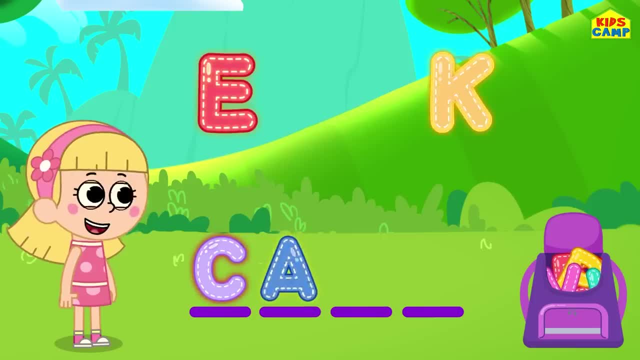 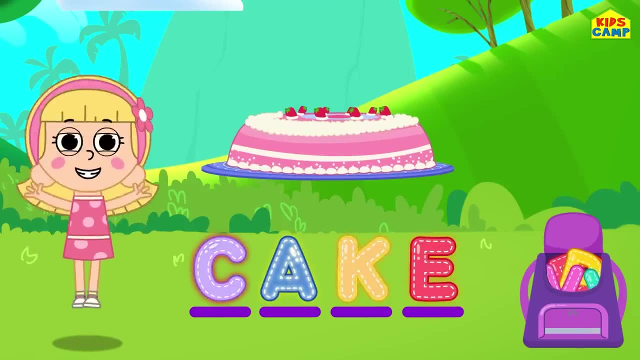 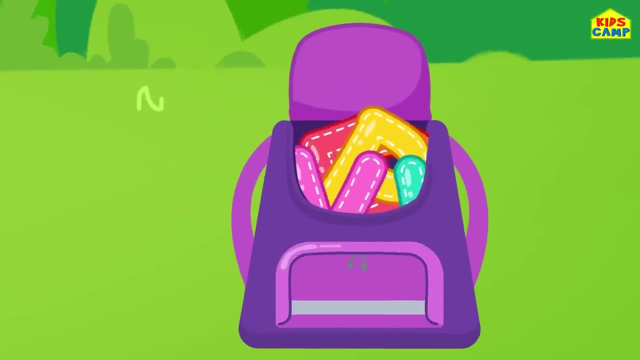 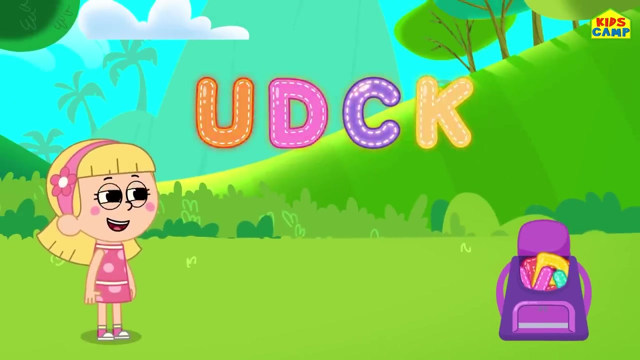 It starts with the letter C, A, P, L and E, A, K and E. Yay, We did it again. What's the next word? Any guesses? Hmm, we have the letters U, D, C and K. 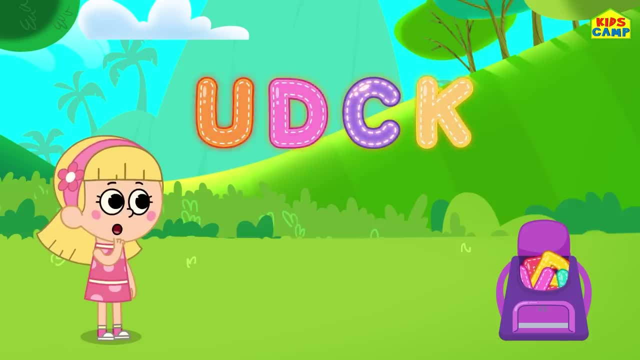 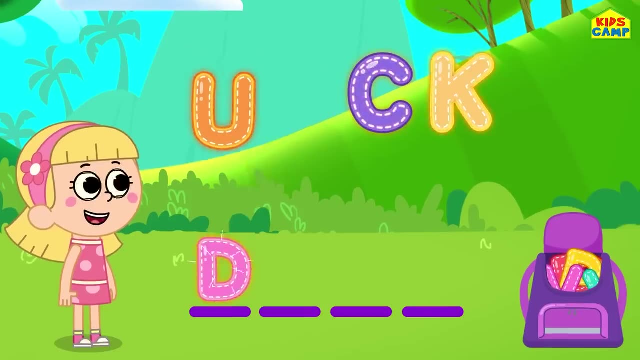 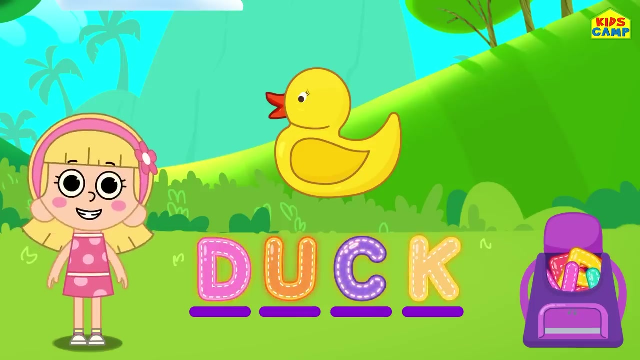 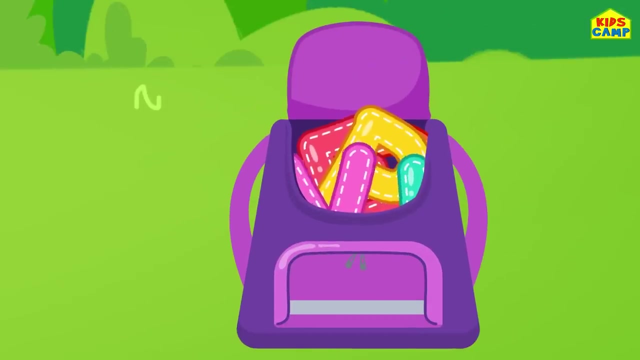 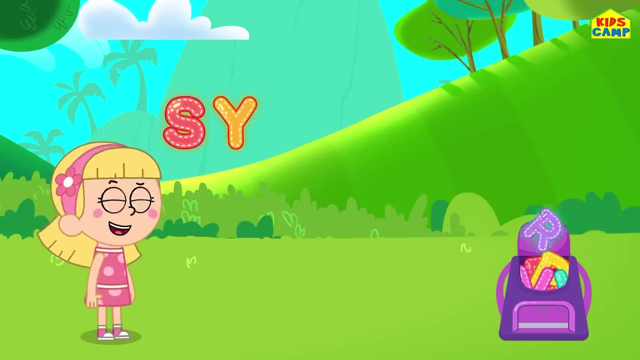 What is this? Hmm, it's a duck. It starts with the letter D, U, C and K. Duck, Woohoo. Alright, let's go to the next one. What does my bag of letters have now? The letters S, Y, R, A, C, O and N. 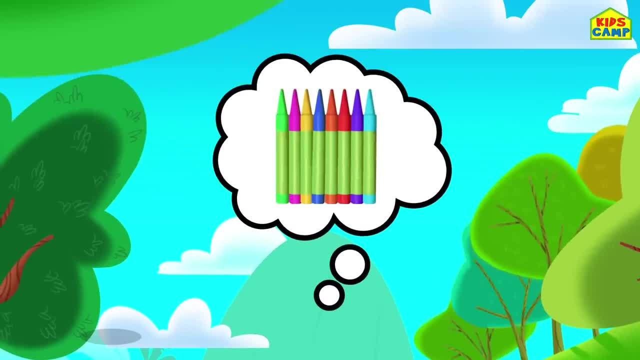 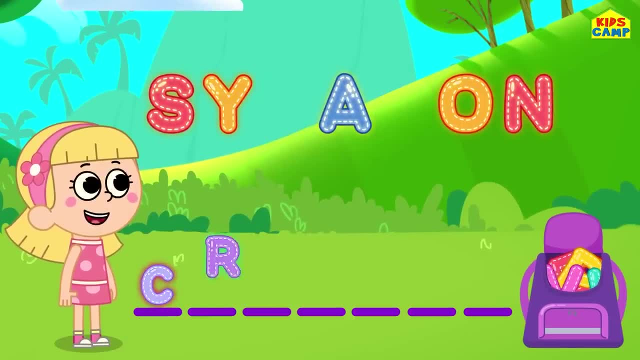 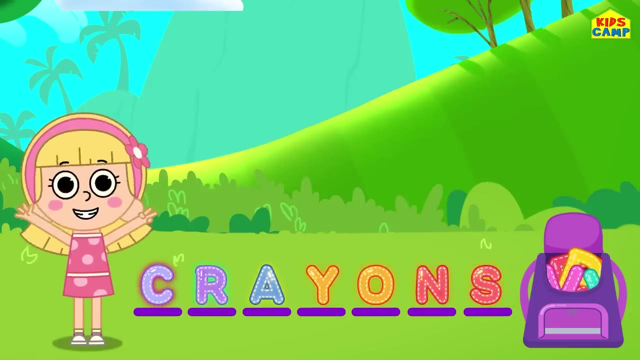 What could this be? These are crayons. That's right, kids, I love crayons. It starts with the letters C R A Y O N S Crayons. That's right, Woohoo. 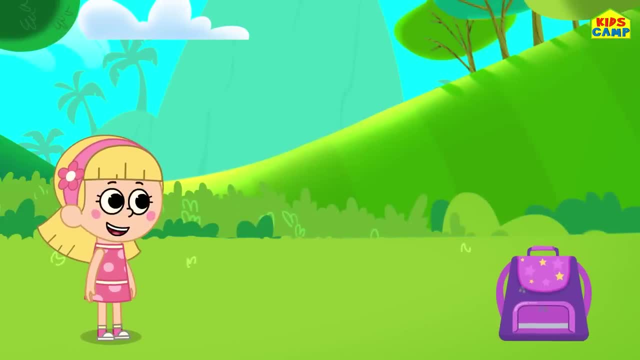 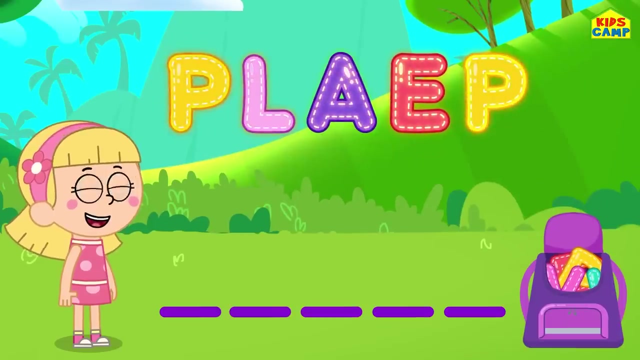 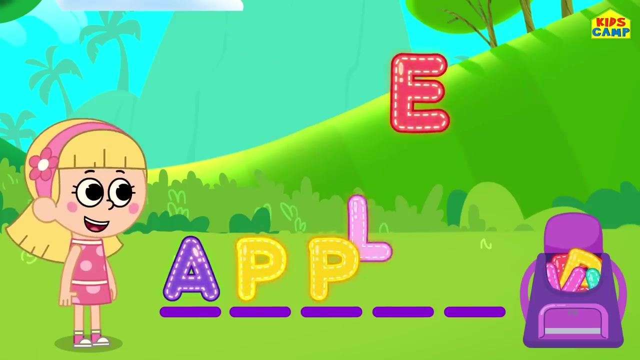 all right. what is this? hmm, i wonder what it is. ah, p, l, a, e, p. hmm, what word could this be? oh, i know, this is an apple. it starts with the letter a, p, p, l and e. that's right, we got it right. kids, it's an apple. 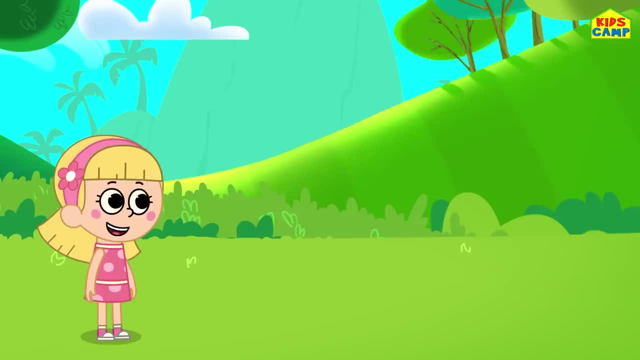 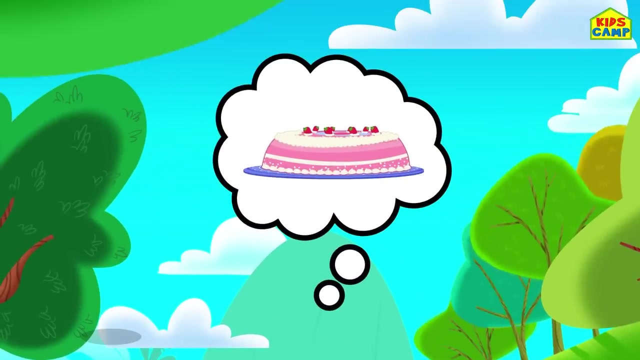 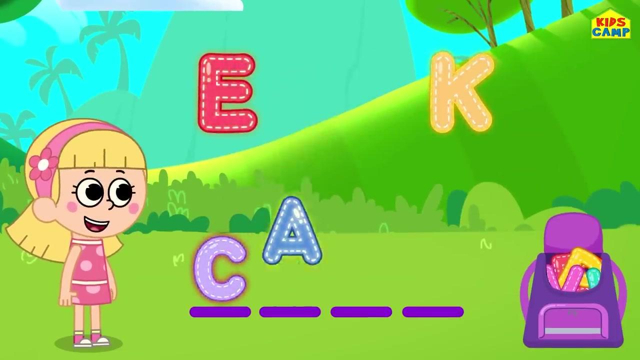 we got the first word correctly. what's next? hmm, i wonder what? could this be the letter e, a, c and k? hmm, this looks familiar. that's right, it's a cake. yes, yes, i know this one. it starts with the letters c, a, k and e. yay, we did it again. 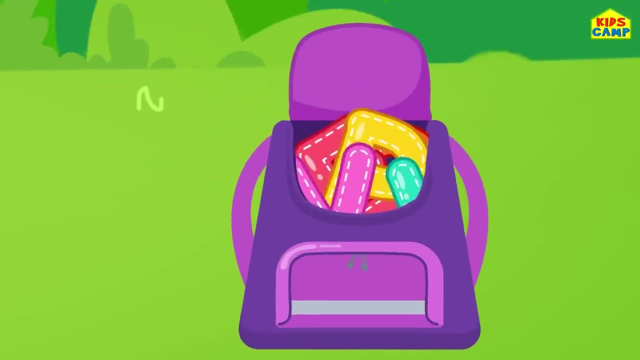 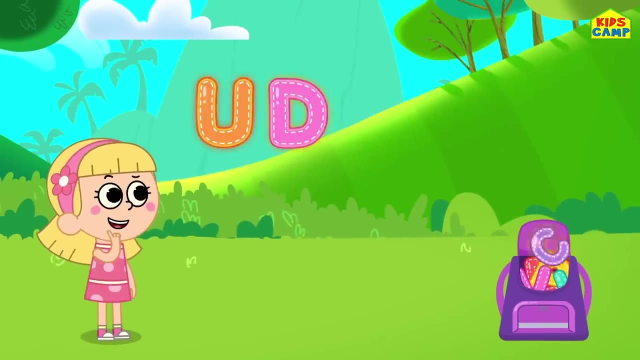 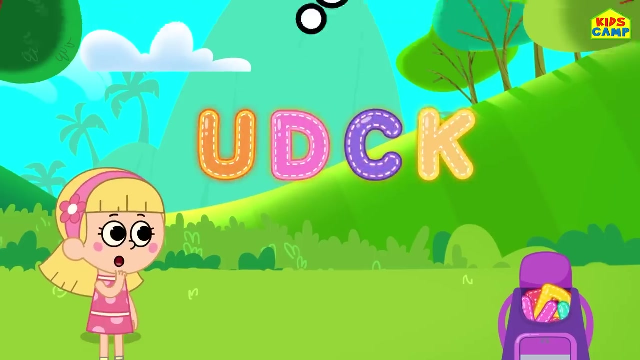 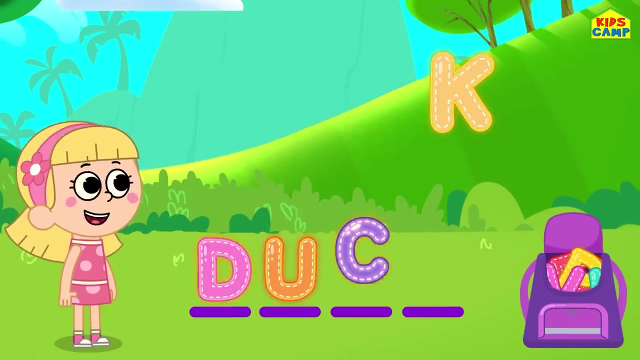 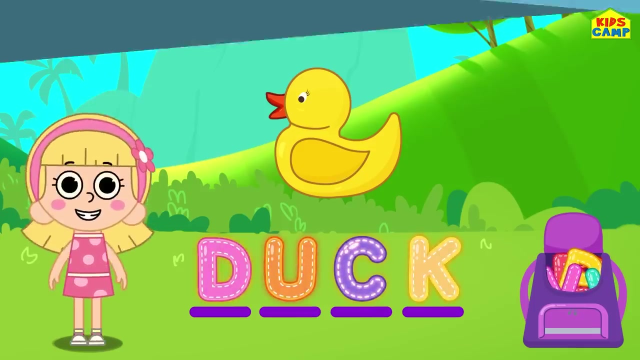 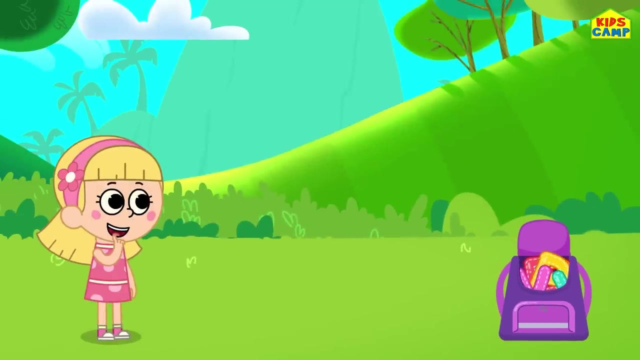 what's the next word? any guesses? hmm, we have the letters u, d, c and k. what is this? hmm, it's a duck. it starts with the letter d, u, c and k: duck, woohoo, all right, let's go to the next one. hmm, what does my bag of letters have now? 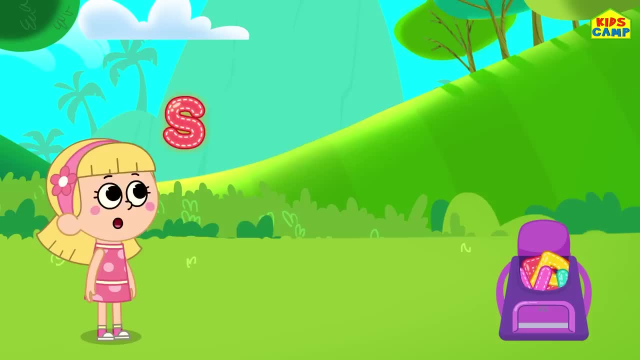 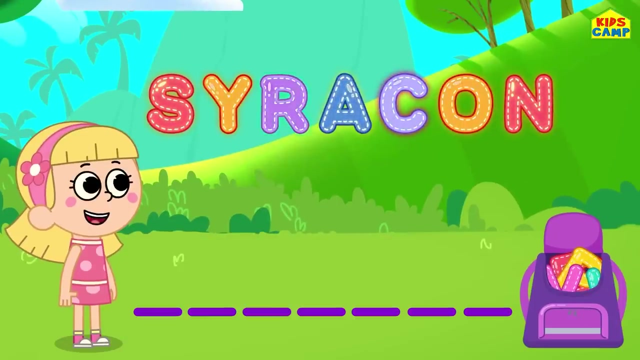 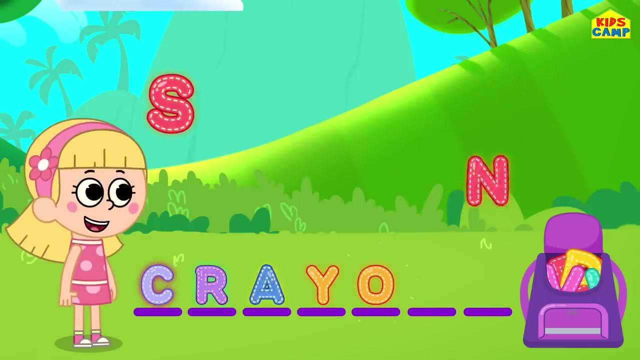 hmm, the letters s, y, r, a, c, o and n. what could this be? these are crayons, that's right, kids, i love crayons. it starts with the letter c r a y o n e s crayons, right, kids. today we are going to do the letter d, d c r a, a, c, o and an n. 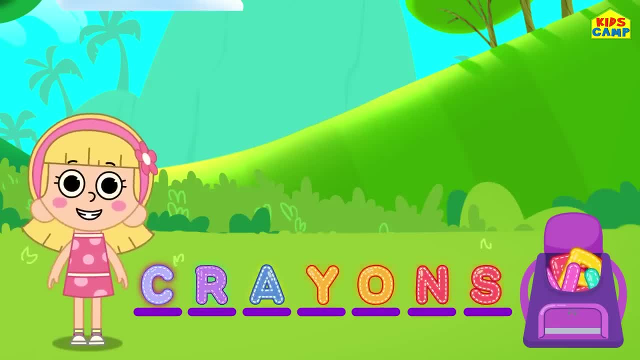 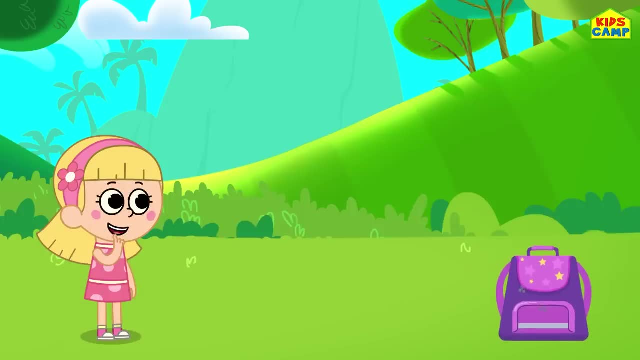 we will know those letters soon. Crayons, That's right. Woohoo, One more. What will come out of the bag of letters? What letters? R T R C O A, Hmm, what could this be? 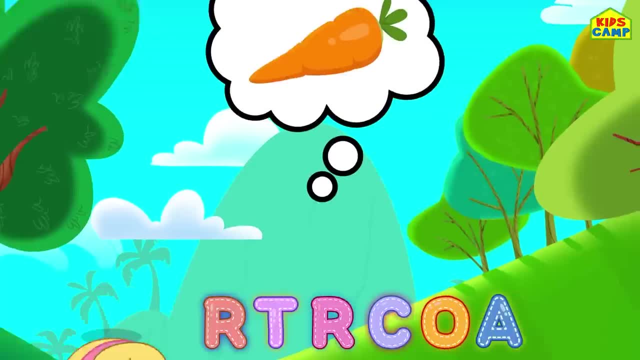 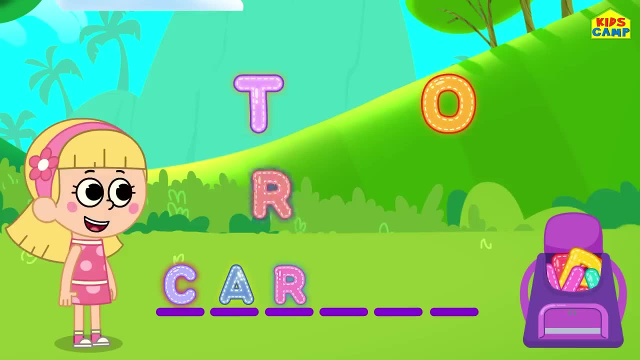 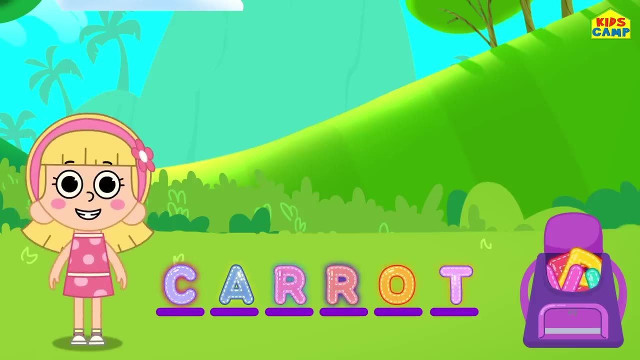 It's a carrot, That's right. That starts with the letters C, A, R, R, O and T, That's right. Carrot, Woohoo. Good job, kids, Well done. This was so much fun. Bye, bye. 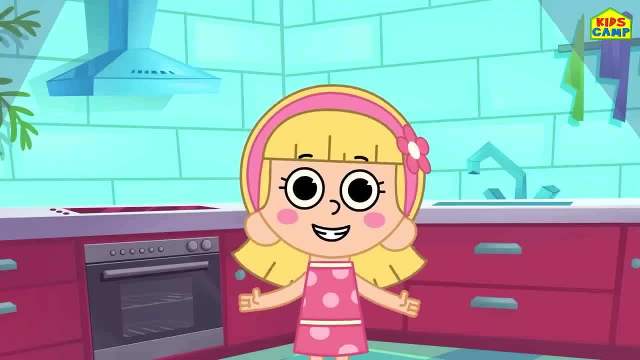 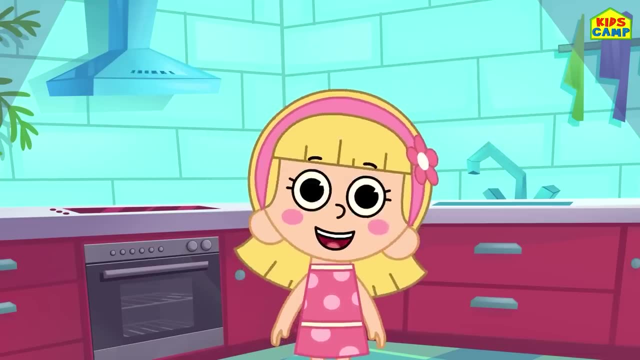 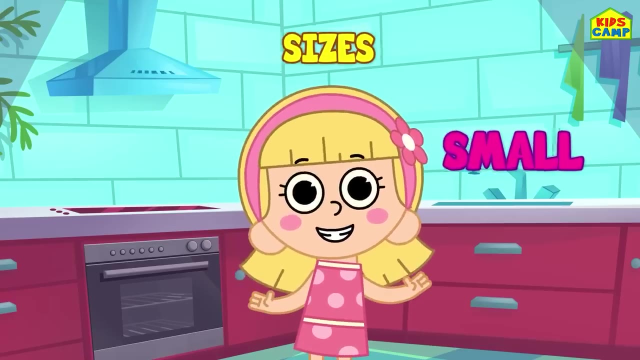 Hi friends, I'm Ellie And I'm making some yummy treats for Eva. Okay, But first we have to sort them according to their sizes: Ready, Big or small. Will you help me, friends? Yes, Then let's get started. 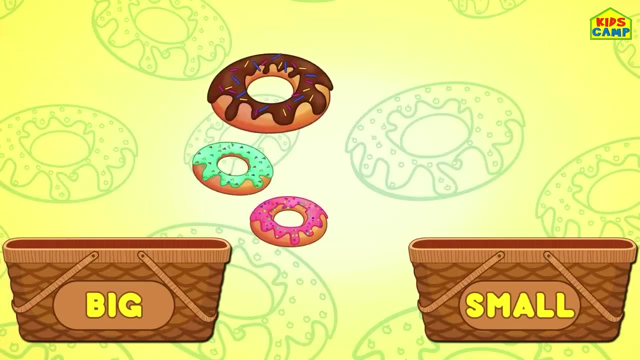 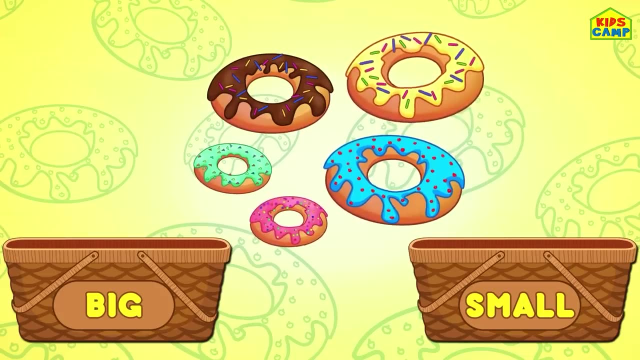 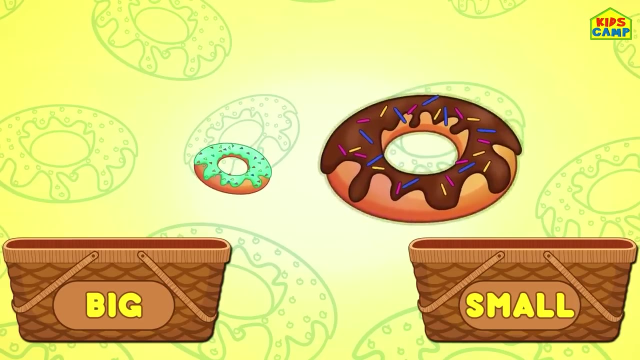 Right away. Wow Donuts- Yummy, I love them. Let's sort them according to their sizes. This chocolate donut looks bigger than this one, That's right. The bigger donut goes into the basket labeled big, That's right. 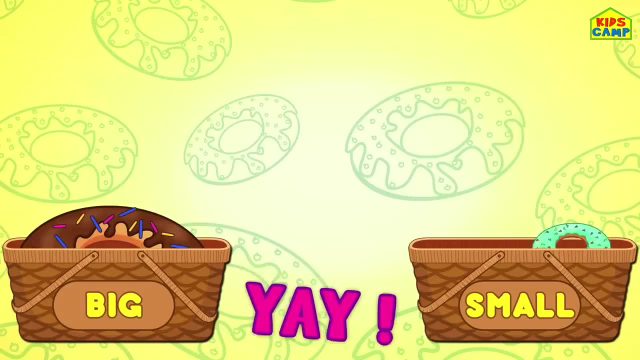 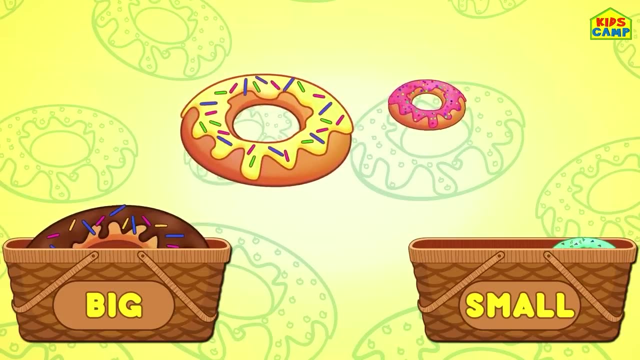 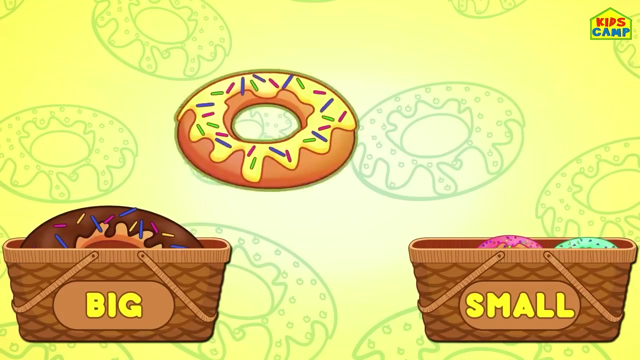 And the small donut goes into the basket labeled small. Yay, Let's compare these two. The pink donut is smaller than the yellow donut, That's right. The smaller one goes into the small basket And the bigger donut goes into the big basket. 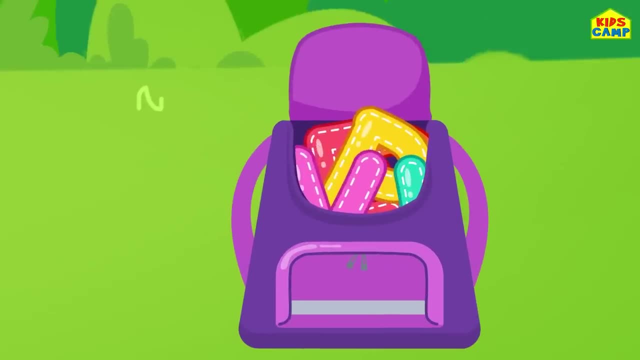 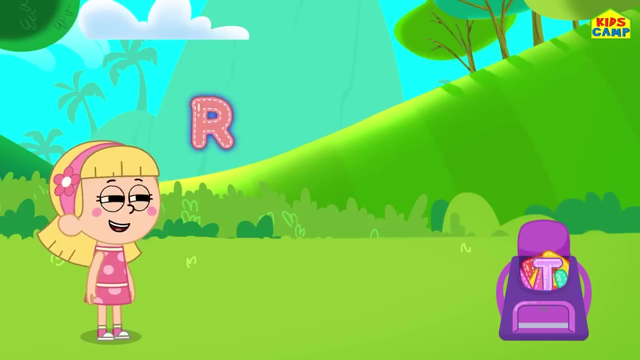 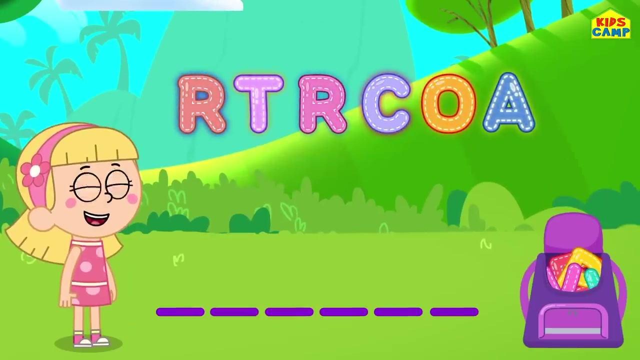 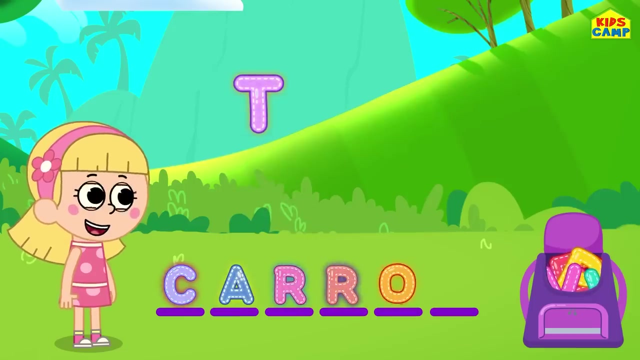 One more. What will come out of the bag of letters? What letters? R, T, R, C, O, A? Hmm, what could this be? It's a carrot, That's right. That starts with the letters C, A, R, R, O and T. 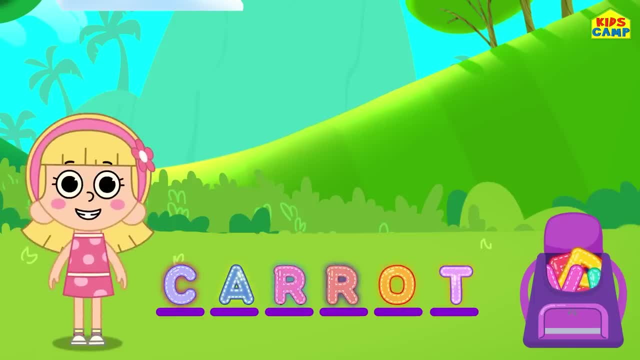 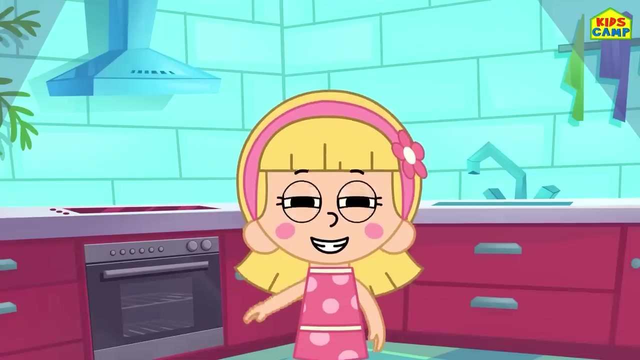 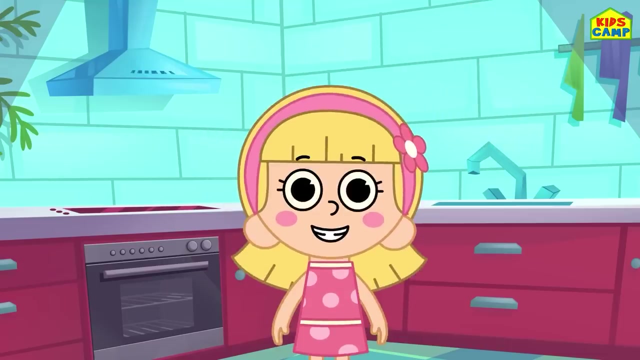 Yay, That's right, Carrot. Woohoo. Good job, kids. Well done. This was so much fun. Bye-bye, Hi friends. I'm Ellie And I'm making some yummy treats for Eva, Okay. 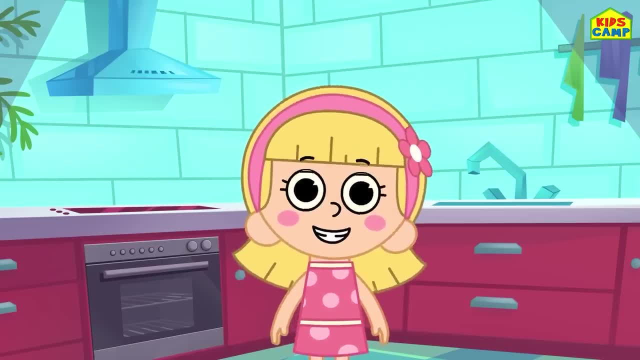 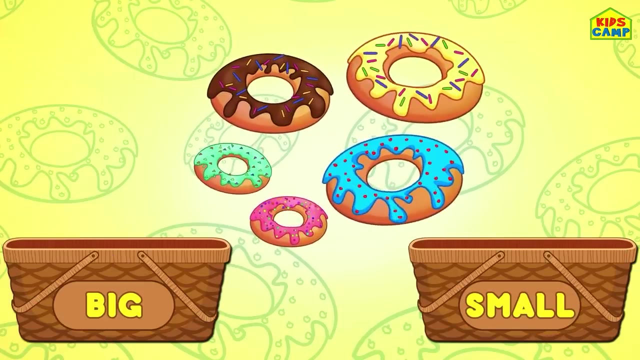 But first we have to sort them according to their sizes. Ready, Big or small? Will you help me, friends? Yes, Then let's get started right away. Wow, Donuts, Yummy, I love them. Let's sort them according to their sizes. 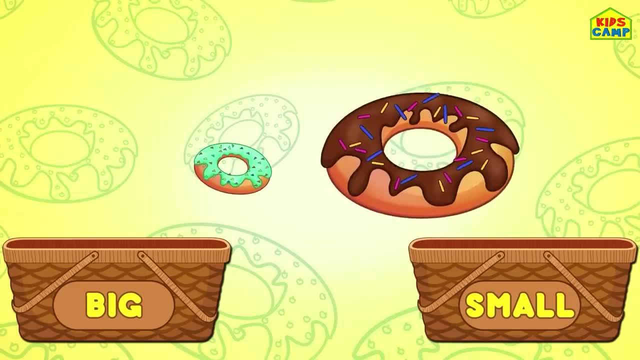 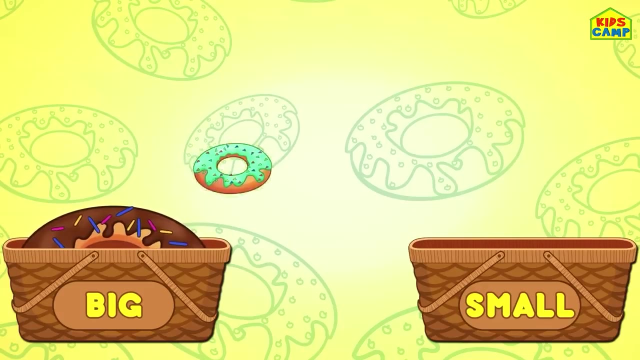 This chocolate donut looks bigger than this one, That's right. The bigger donut goes into the basket labeled big, That's right, And the small donut goes into the basket labeled small, Yay, Hmm, Let's compare these two. 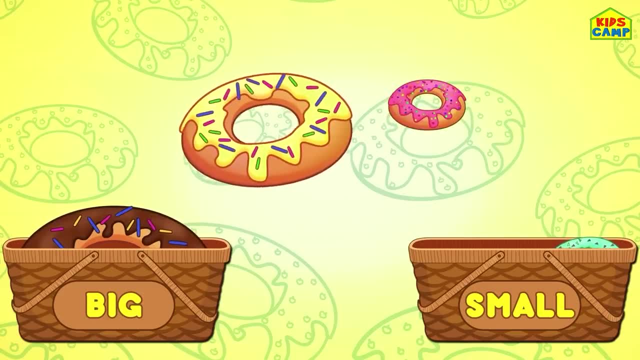 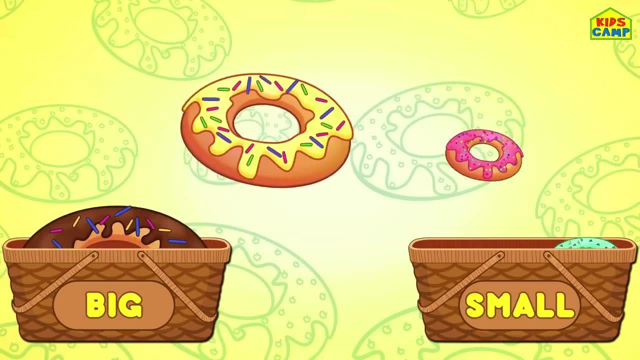 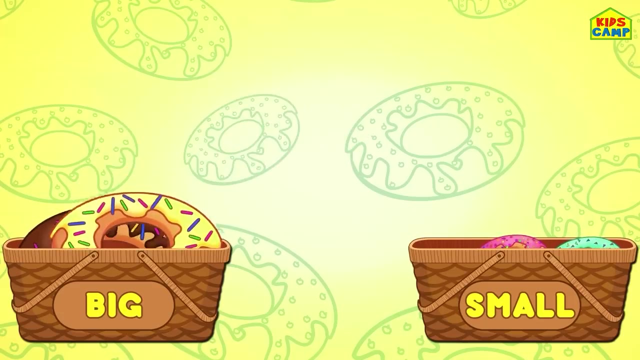 The pink donut is smaller than the yellow donut, That's right. The smaller one goes into the small basket And the bigger donut goes into the big basket. That's right. Yay, Yay, Yay, Yay. 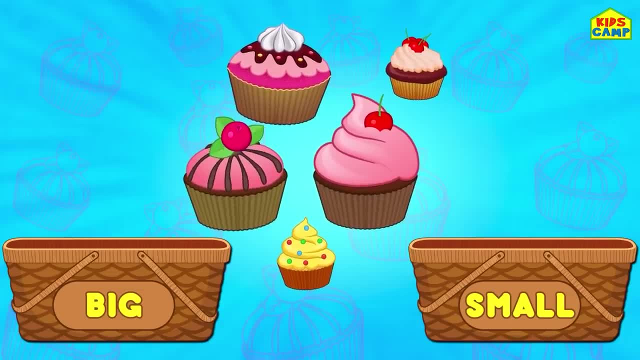 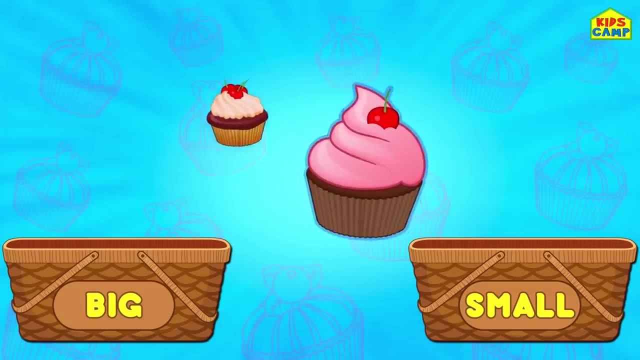 Yay, I see a lot of cupcakes. Wow, Let's sort them according to their sizes. The pink cupcake is bigger than the other cupcake. The bigger donut goes into the big basket. That's right, Yay, Yay. 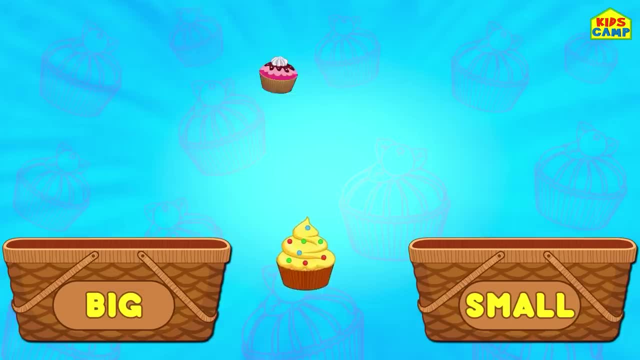 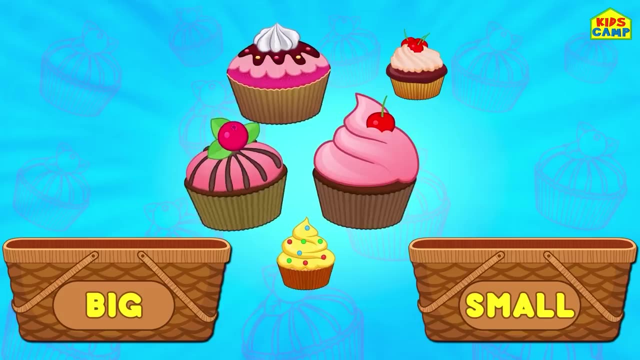 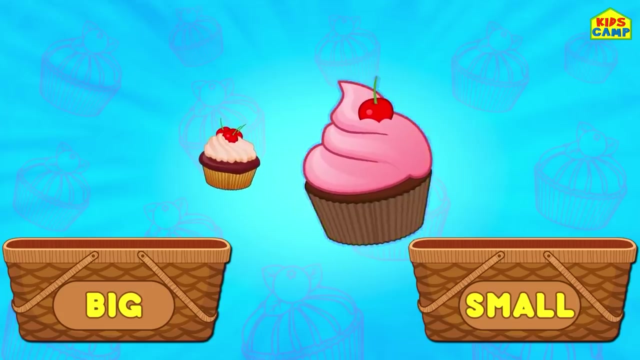 That's right. Yay, Yay, Yay, Yay, Yay. I see a lot of cupcakes. Wow, Let's sort them according to their sizes. The pink cupcake is bigger than the other cupcake. The big pink cupcake goes into the big basket. 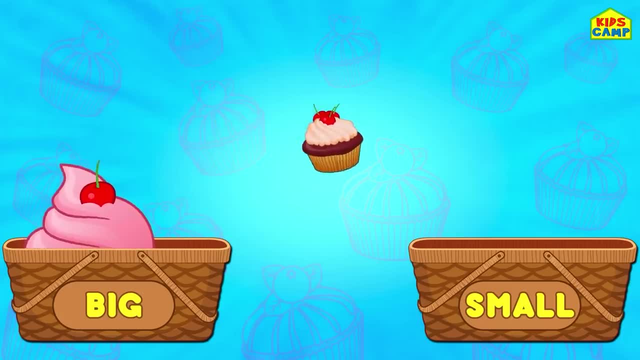 And the smaller one goes into the small basket. Wow, Wow, Ooh, more cupcakes. Let's compare these: The pink cupcake is bigger, The yellow cupcake is smaller, The yellow cupcake goes into the small basket and the big one goes into the big basket. 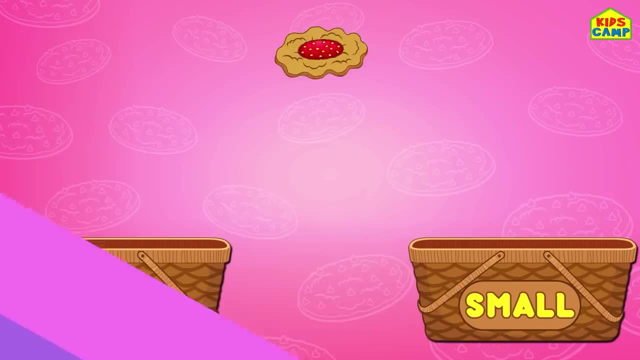 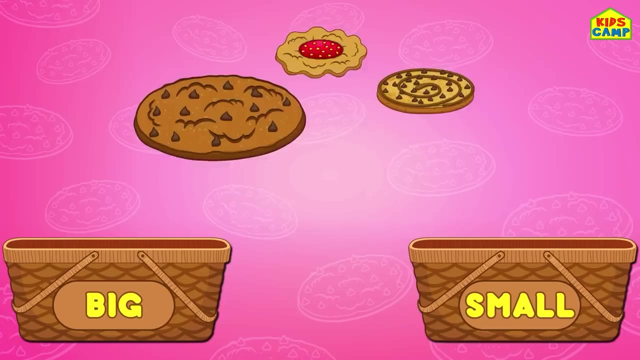 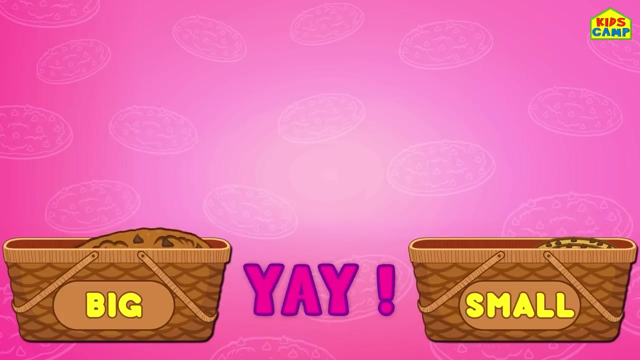 Yay, What's next? Cookies. Wow, Let's sort the bigger cookies from the smaller ones. The smaller cookie goes into the small basket and the bigger cookie goes into the big basket. That's right. Yay, This smaller cookie goes into the small basket. 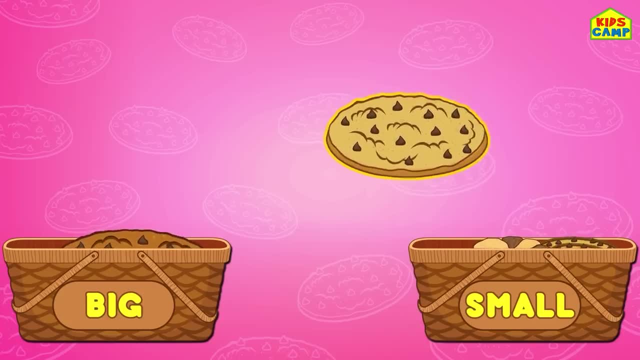 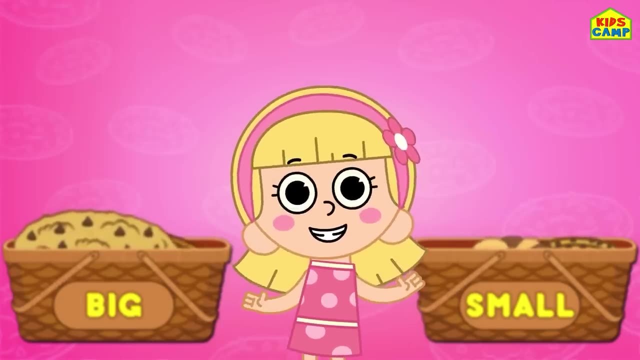 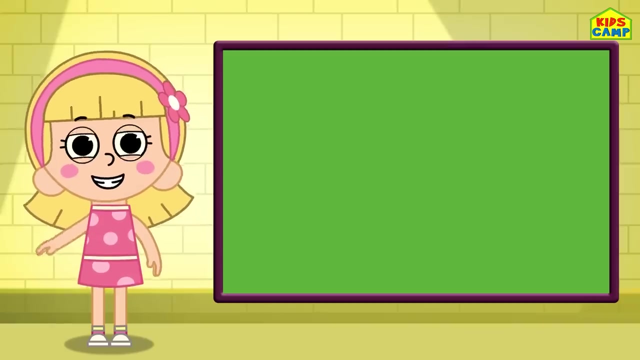 and this big one goes into the big basket. Wow, We sorted all these treats according to their sizes. Good job everyone. Woohoo, Hi kids. I'm Ellie and today we're going to play Find the Objects, Yay. 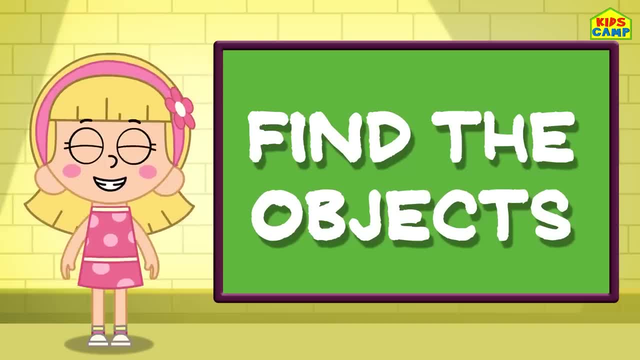 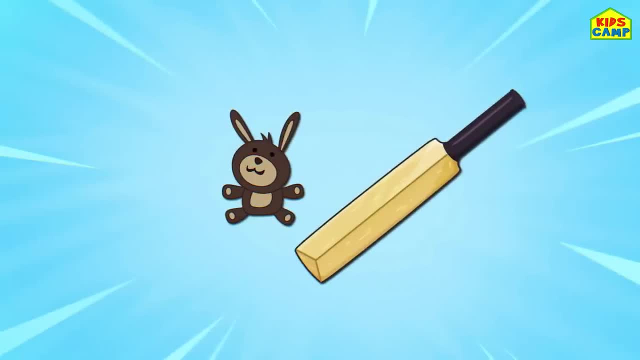 That's right, Let's get started. Woohoo, Let's find the bat and the teddy Ready. Here we go. Can you find the bat and the teddy? Where could it be? Can you see the bat and the teddy anywhere? 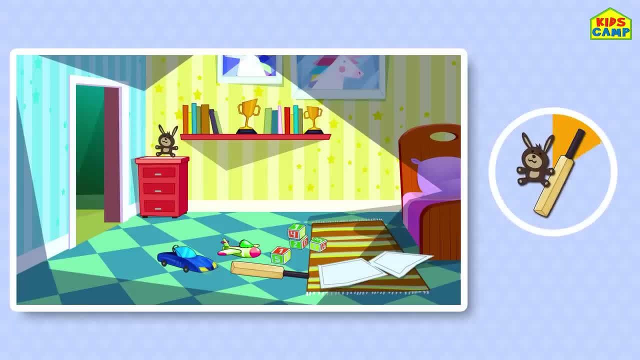 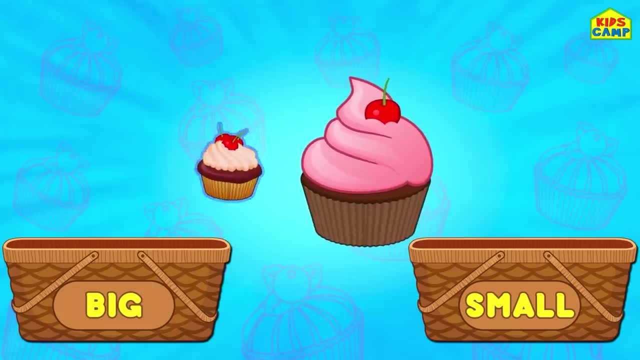 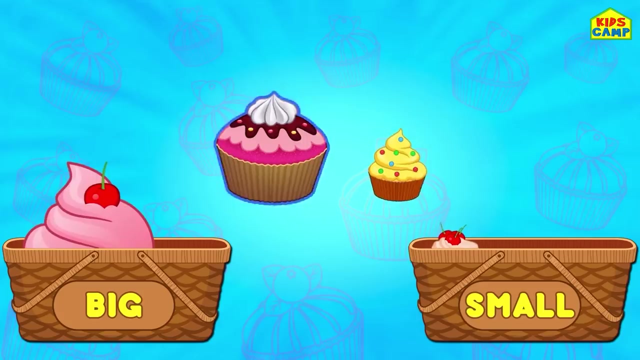 Yay, Yay, Yay. The big pink cupcake goes into the big basket And the smaller one goes into the small basket. Wow, Oh, more cupcakes. Let's compare these: The pink cupcake is bigger, The yellow cupcake is smaller. 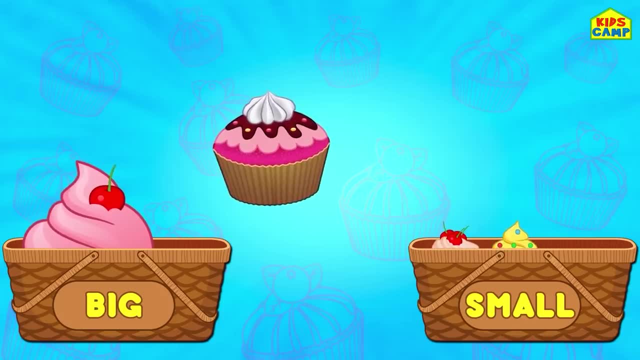 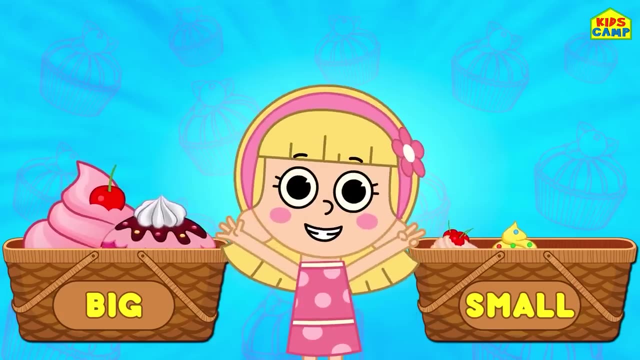 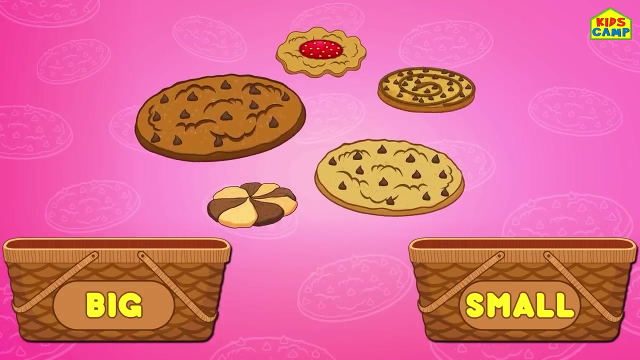 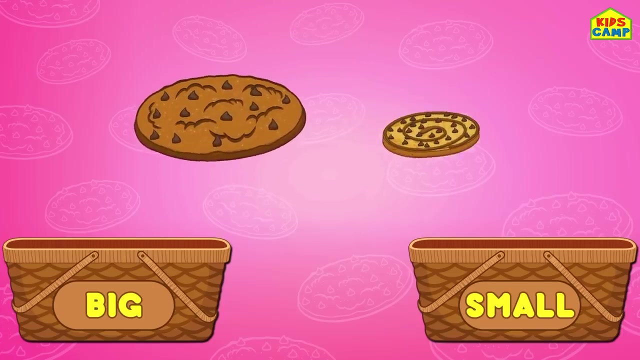 The yellow cupcake goes into the small basket And the big one goes into the big basket. Yay, What's next? Cookies- Wow, Let's sort the bigger cookies from the smaller ones. The smaller cookie goes into the small basket. 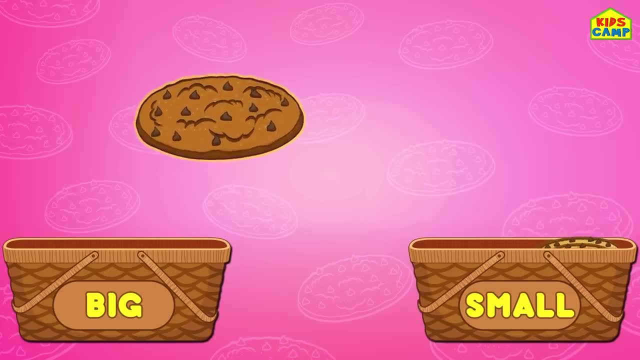 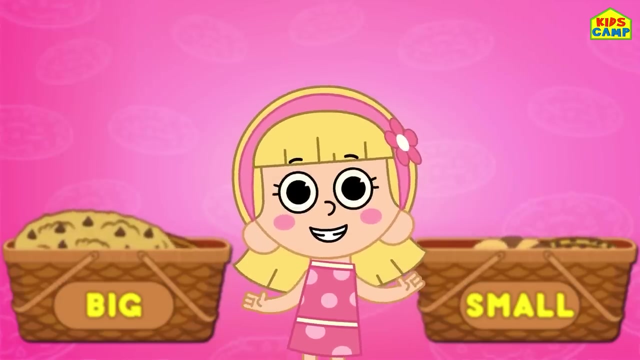 And the bigger cookie goes into the big basket. That's right, Yay, This smaller cookie goes into the small basket And this big one goes into the big basket. Wow, We sorted all these treats according to their sizes. Good job everyone. 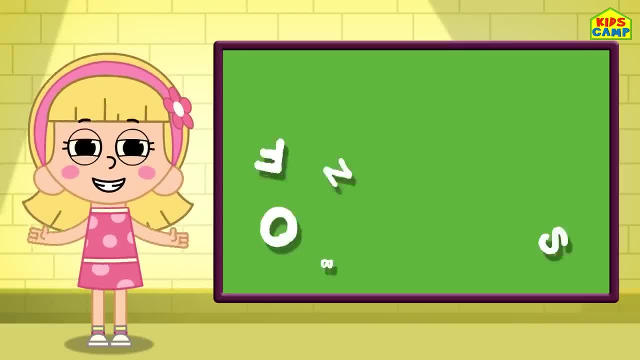 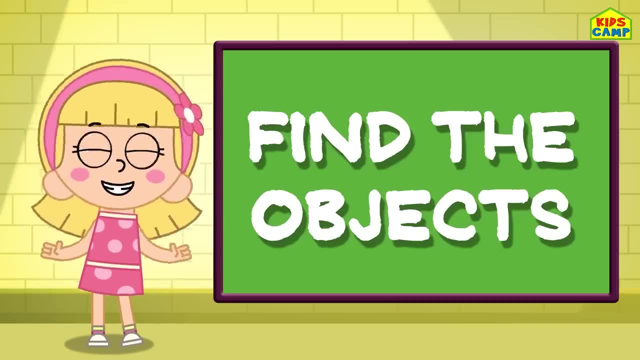 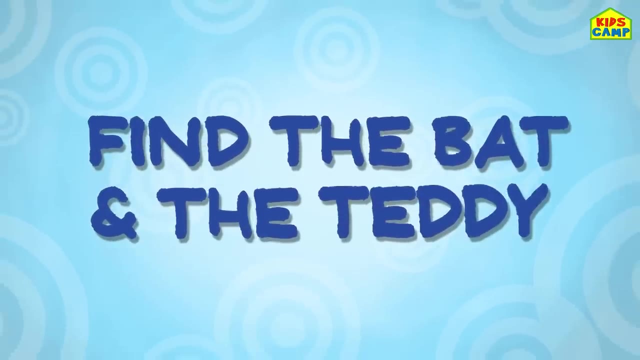 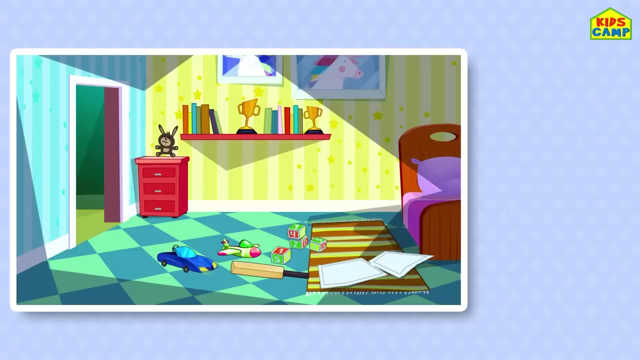 Hi kids, I'm Ellie, And today we are going to play How to Find the Objects. Yay, That's right, Let's get started. Woohoo, Let's find the bat and the teddy. Ready, Here we go. 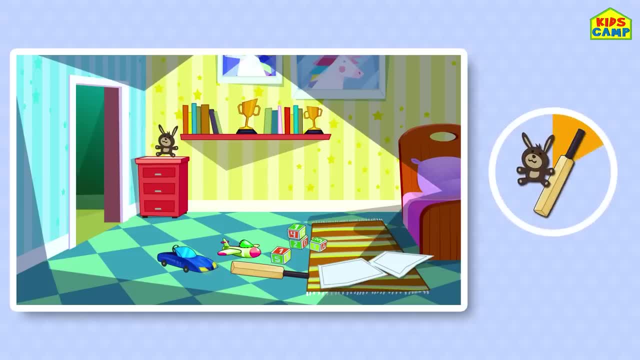 Can you find the bat and the teddy? Where could it be? Can you see the bat and the teddy? Can you see the bat and the teddy Anywhere? Keep looking Time's up. Aha, There it is. 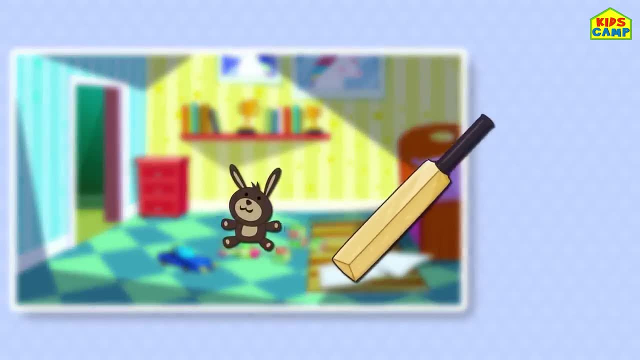 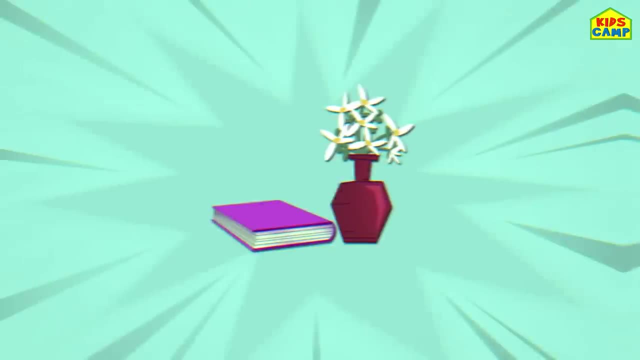 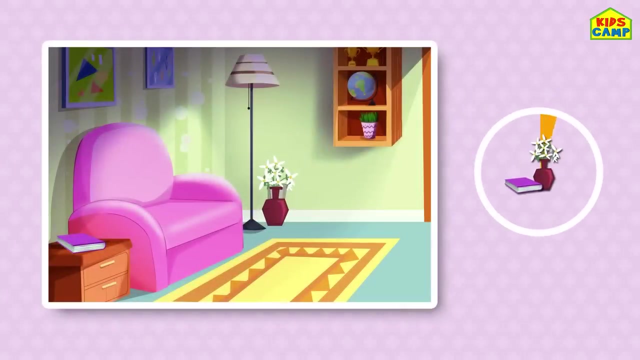 Yay, We found the bat and the teddy. Find the flowers and the book. Let's look for it. Can you spot the flowers and the book? Where could it be? Where could it be? Not on the sofa? Where is it? 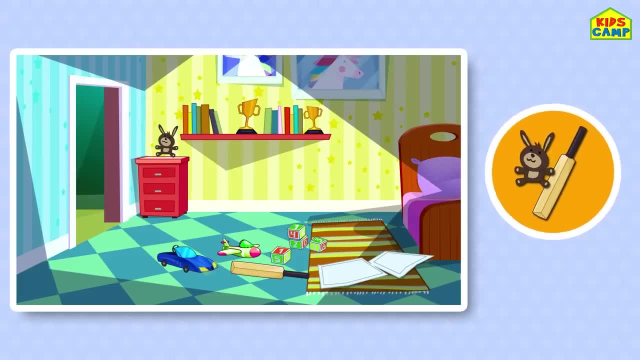 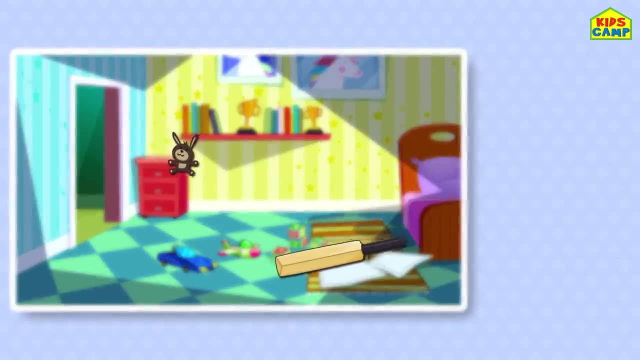 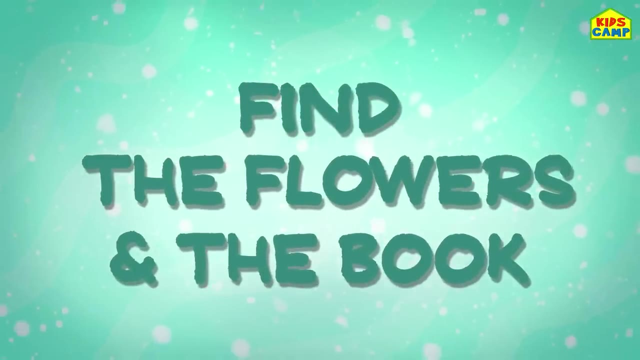 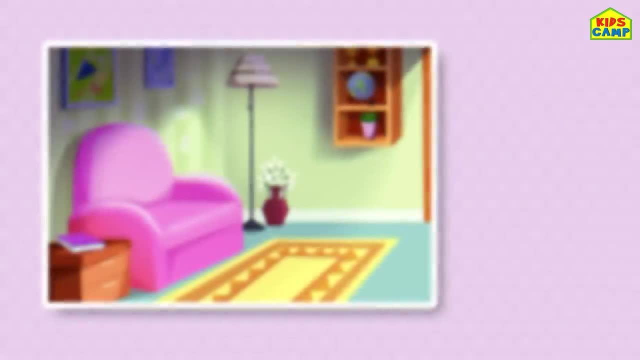 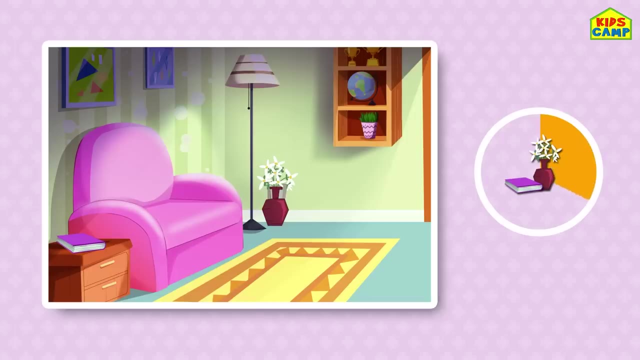 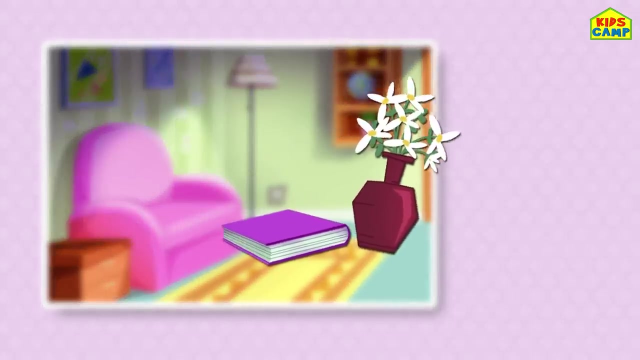 Yes, Close your eyes, Let's look for it. Ok, Let's draw some lines. Can you spot the flowers and the book? A yellow Ming- Are we ready? Ready? Zooming, Let's find the flowers and the book. We found the flowers and the book. Find the ball and the pink doll. 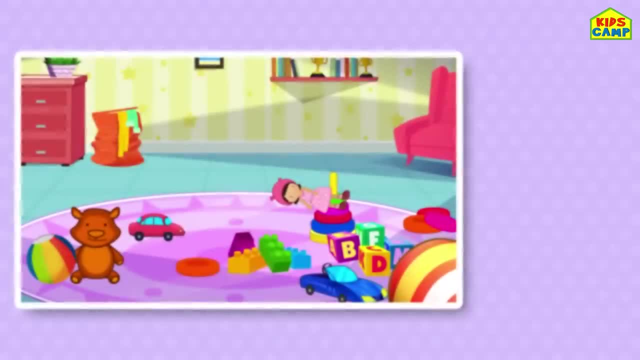 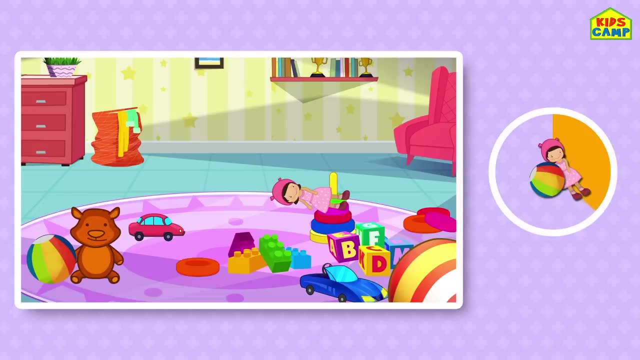 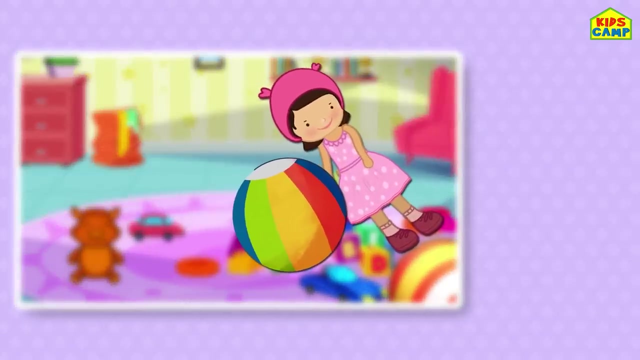 Ready. Can you spot the doll and the ball? Where could it be? where could it be? Keep looking, Our time's almost up, Time's up. Did you find it? Yes, there it is. We found the ball and the pink doll. Yay, Find the red toothbrush and the toothpaste. Ready kids. 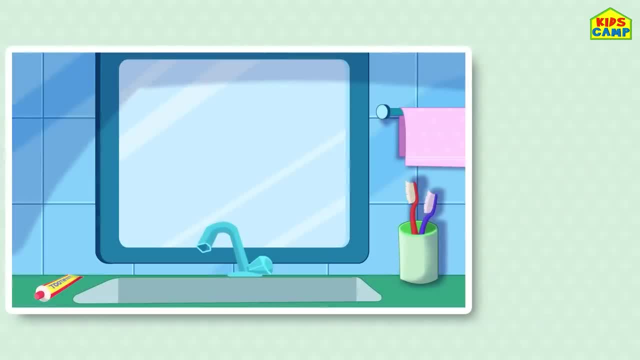 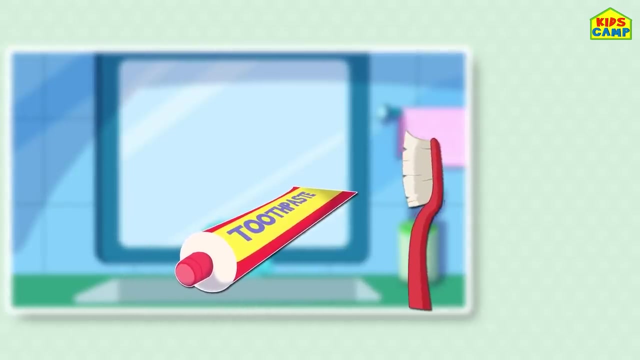 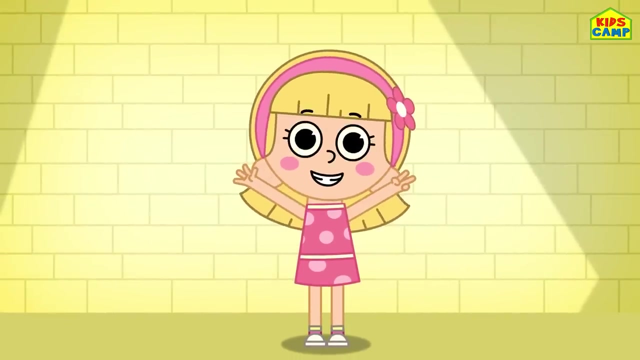 Look for it. Look for it. Can you spot the red toothbrush and the toothpaste? This one is easy. Keep looking Time's up. Woohoo, you did find it There. it is The red toothbrush And the toothpaste. This was so much fun, kids, We found all the objects. 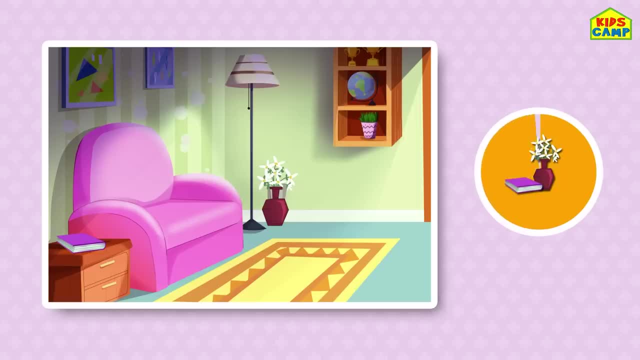 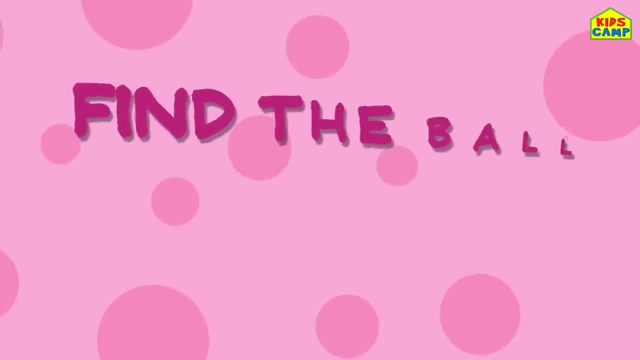 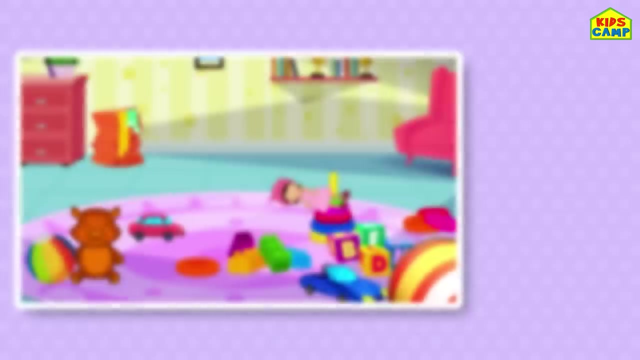 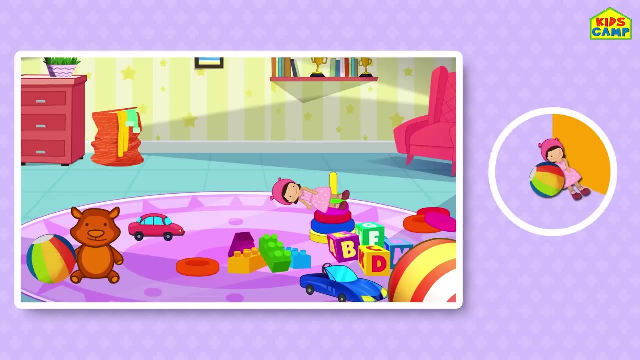 Keep looking. Time's up. There it is. We found the flowers and the book. Look, Find the ball and the pink doll Ready. Can you spot the doll and the ball? Where could it be? Where could it be? Keep looking. 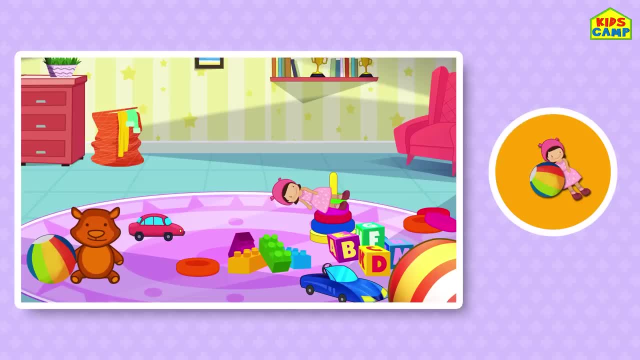 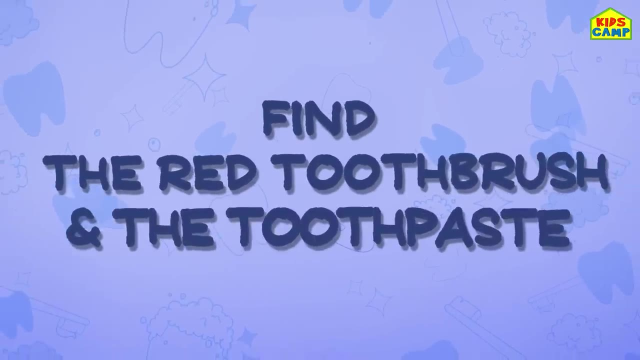 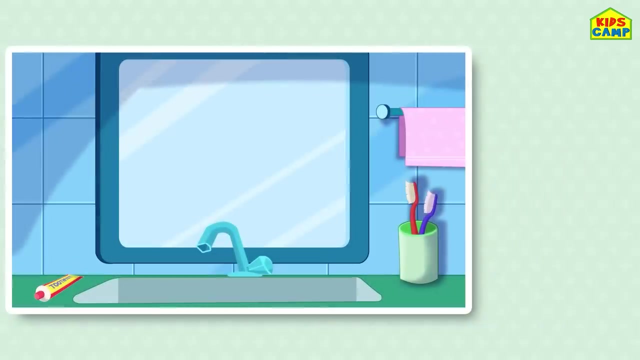 Our time's almost up, Time's up. Did you find it? Yes, There it is. We found the ball and the pink doll. Yay, Find the red toothbrush and the toothpaste. Ready kids Look for it. Can you spot the red toothbrush and the toothpaste? 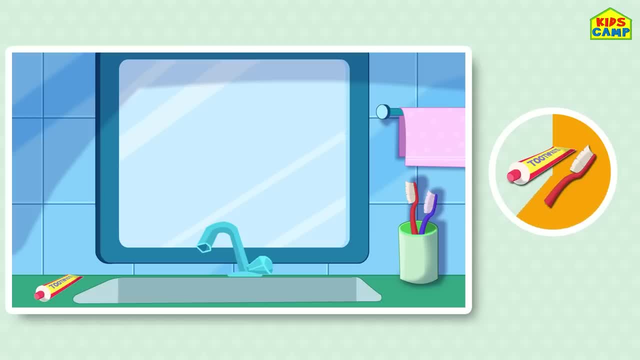 This one is easy. Keep looking. Where is it Here? it is Time's up, Time's up. You did find it There. it is The red toothbrush and the toothpaste. This was so much fun, kids. We found all the objects. 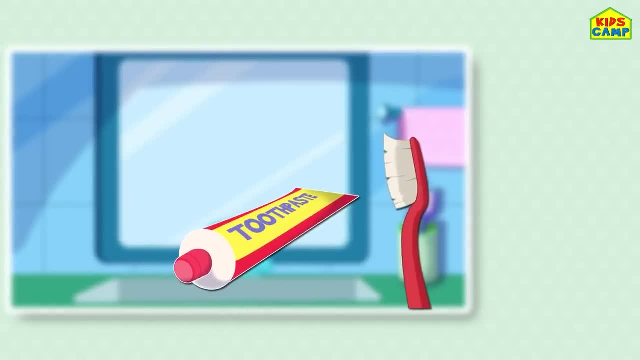 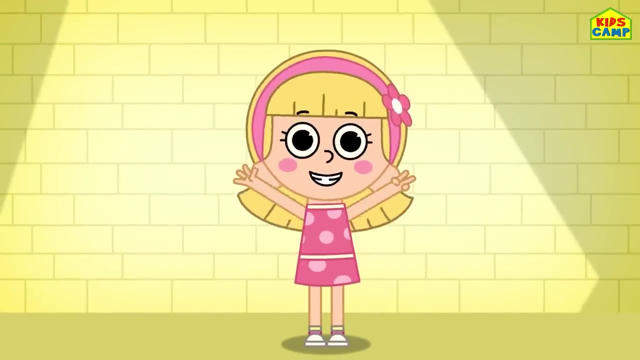 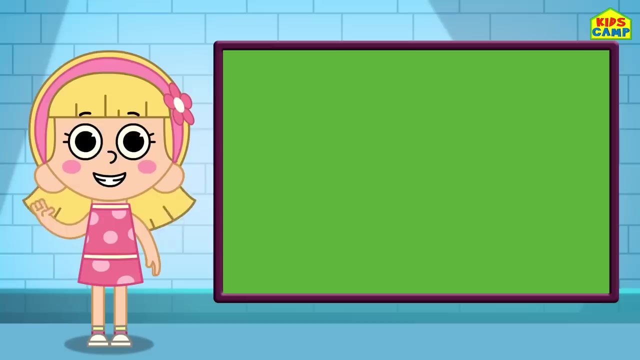 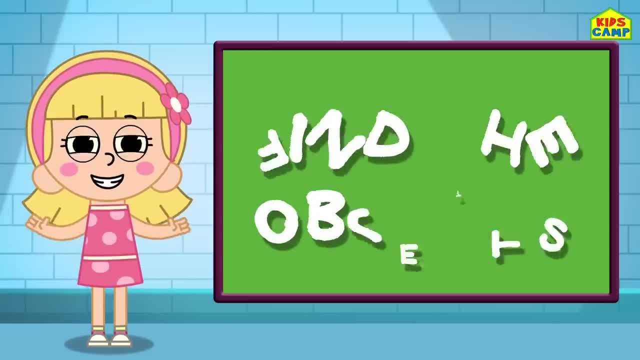 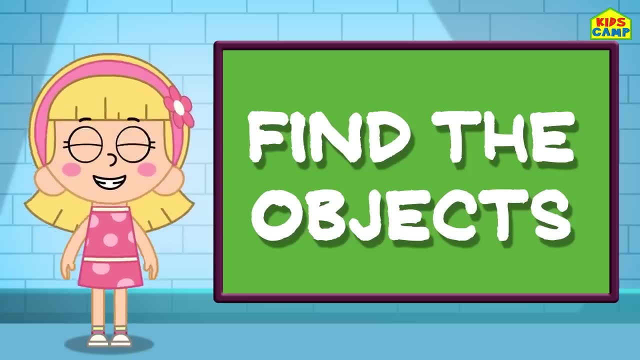 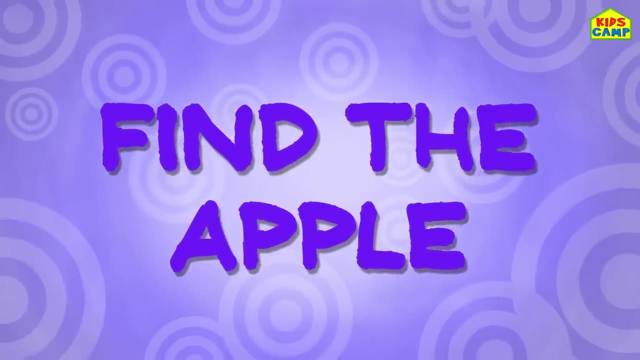 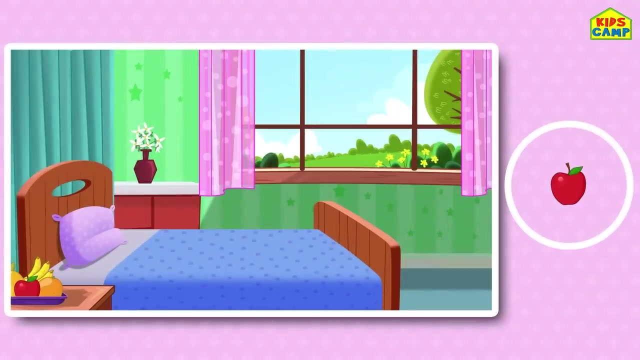 Bye, And today we are going to play Find the Objects. Yay, Ready, Let's get started. Find the apple. Hmm, that's easy. Let's look for the apple. Where's the apple? Is it on the bed? 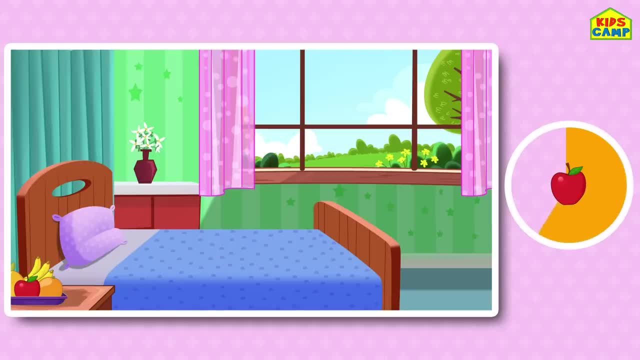 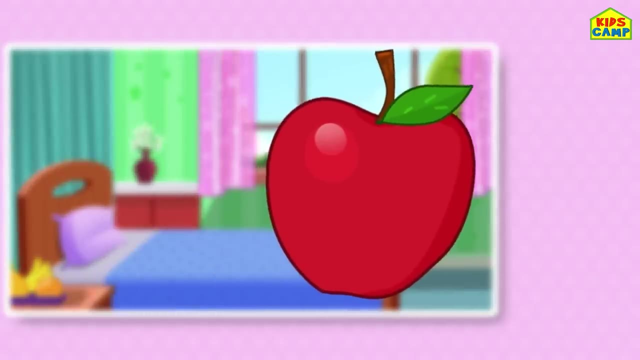 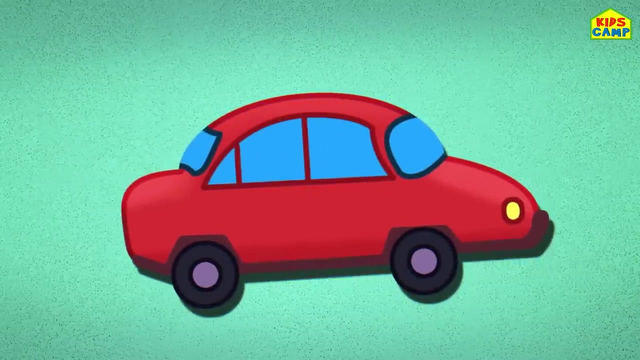 No, Where is it? Keep looking Time's up. Did you spot the apple? Yes, there it is. Good job, kids. We found it. Find my car. We have to look for my red car. Can you spot it? 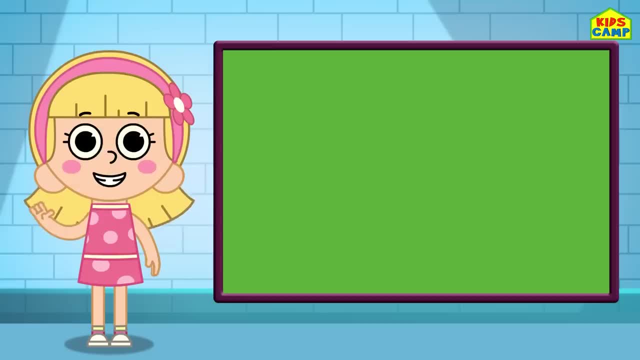 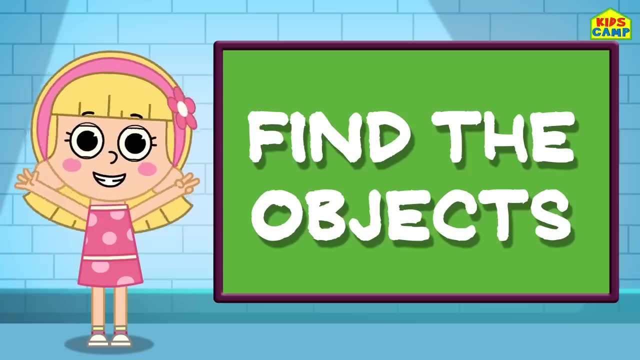 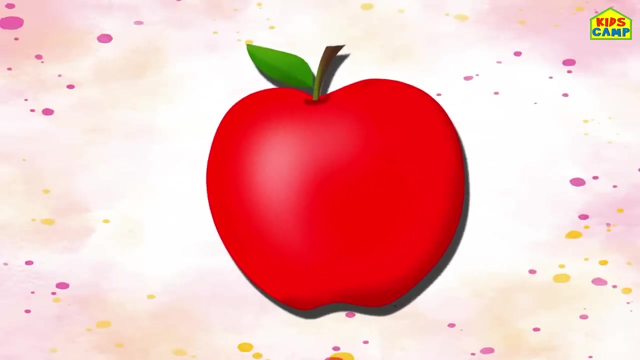 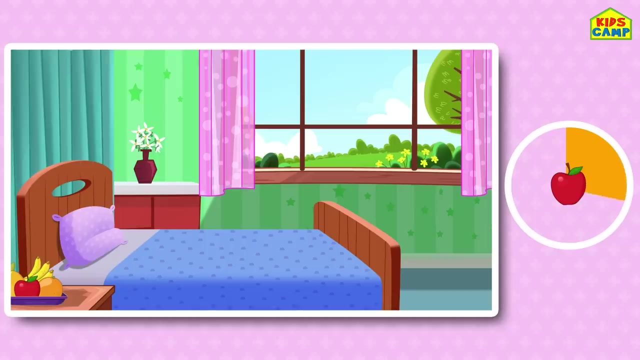 See you soon. Hi kids, I am elly and today we are going to play. find the objects. Yay, Ready, Let's get started. Find the objects, Find the apple. Hmm, that's easy. Let's look for the apple. Where's the apple? Is it on the bed? 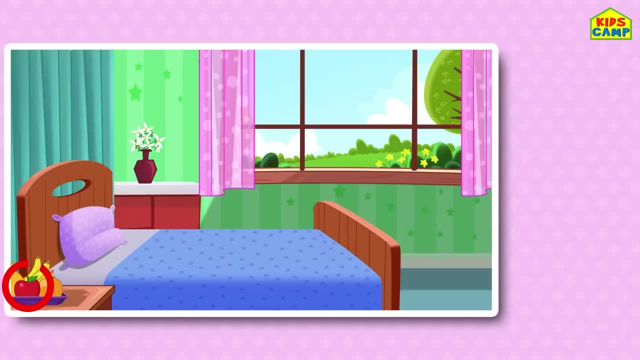 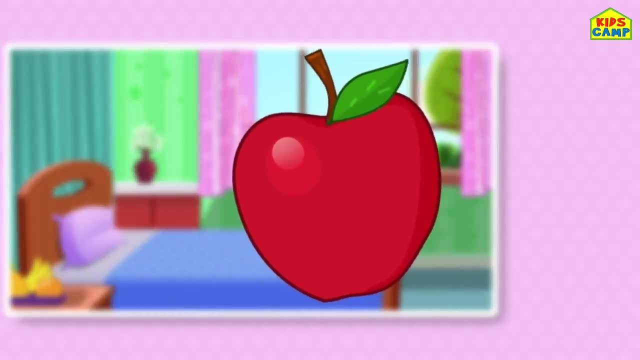 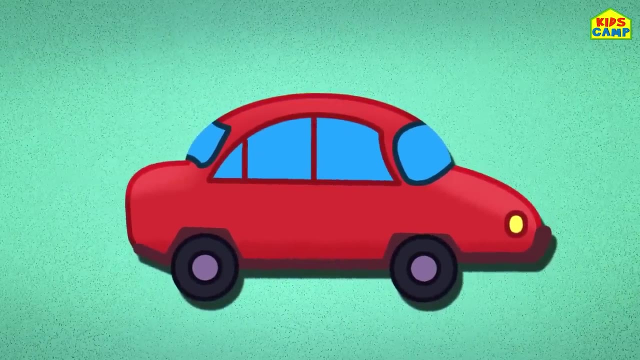 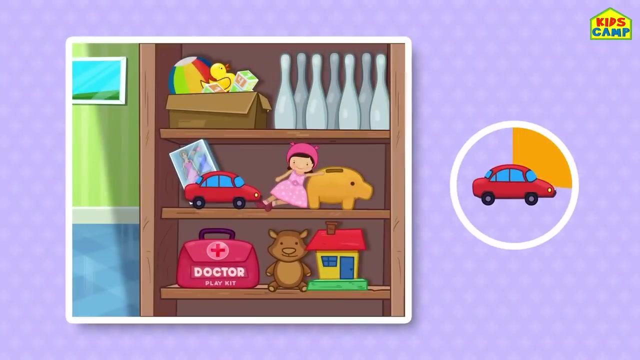 No, Where is it? Keep looking, Time's up. Yes, there it is. Yay, Good job kids, We found it, Find my car. We have to look for my red car. Can you spot it? Hmm, where is it? There's so many toys on the shelf. Uh oh, time's up. 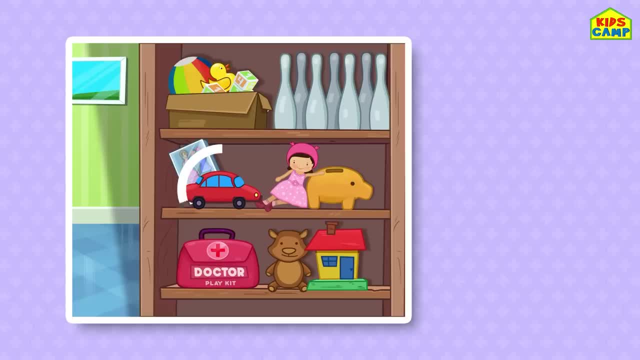 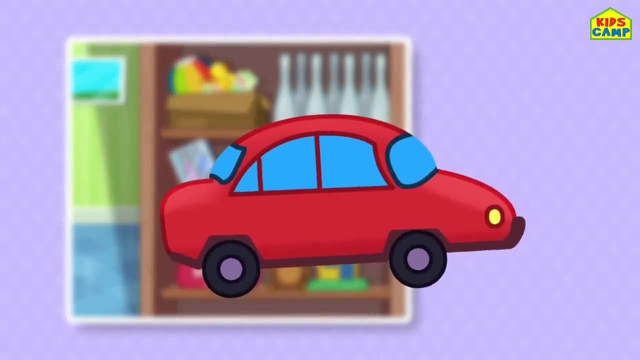 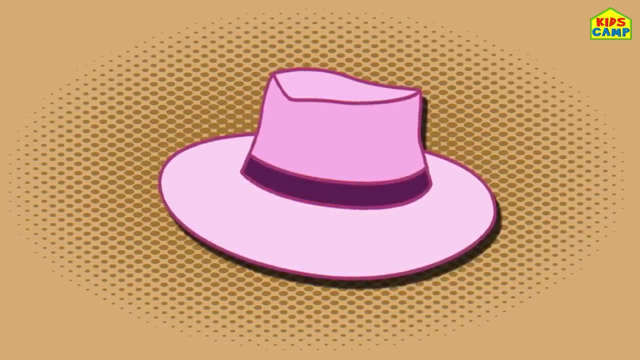 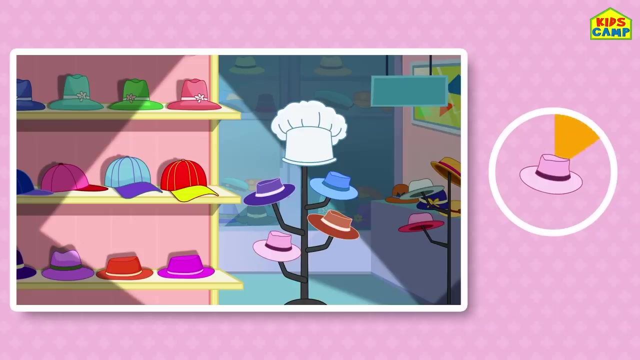 Did you spot it? Yes, that's right, That's where it is. That's my red car, Vroom, vroom. Find my hat, My pink colored hat. Can you look for my hat? Oh my, there are so many hats. Can you spot the right one? Come on, Time's up. 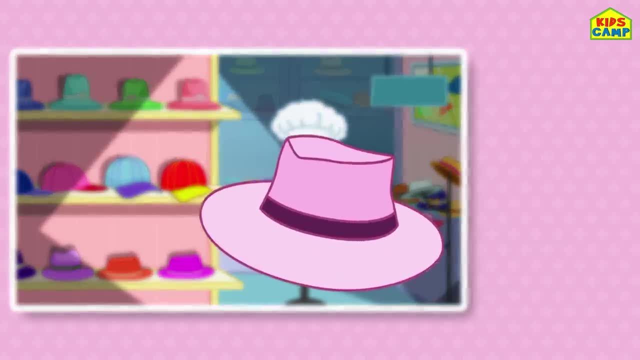 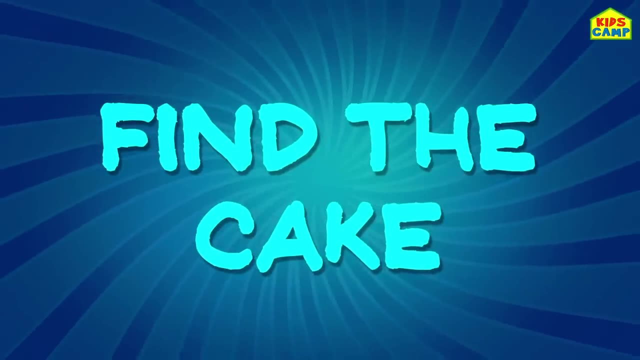 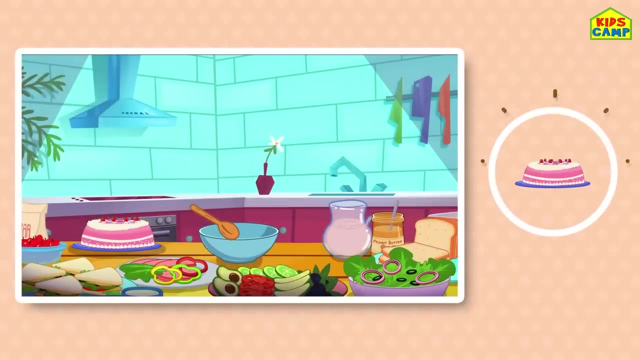 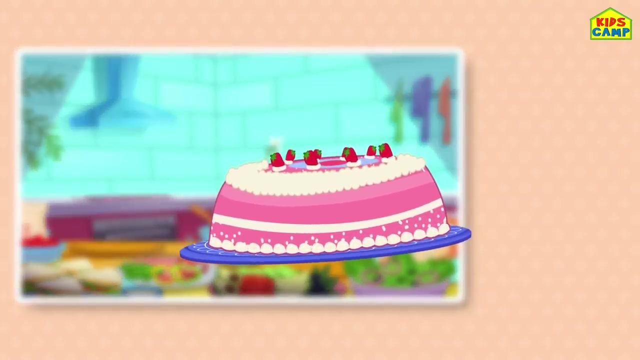 Yes, that's the one. Yay, Good job, kids, You found it. Woohoo, Find the cake. Hmm, delicious, Let's look for the cake. Wow, there is so much food on the table. Can you look for the cake? Where's the cake? Time's up. That's right, There it is. You found the cake. 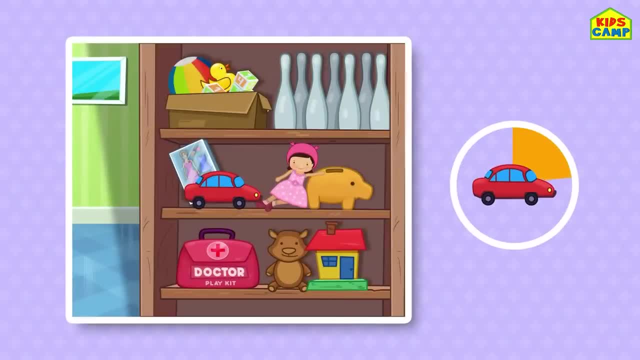 Hmm, where is it? There's so many toys. There's so many toys on the shelf. Uh-oh, time's up. Did you spot it? Yes, that's right, That's where it is. That's my red car. 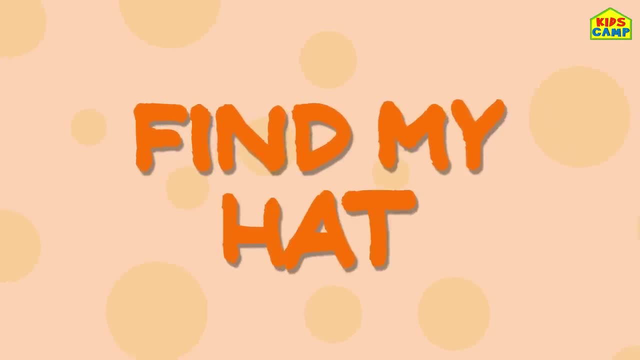 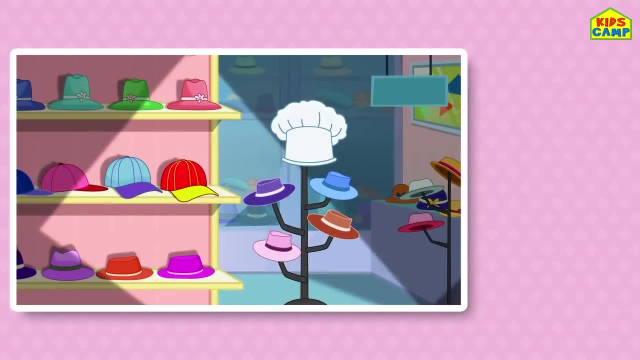 Vroom, vroom. Find my hat, My pink-colored hat. Can you look for my hat? Home, home, home. Oh my, there are so many hats. Can you spot the right one? Come on, Time's up. 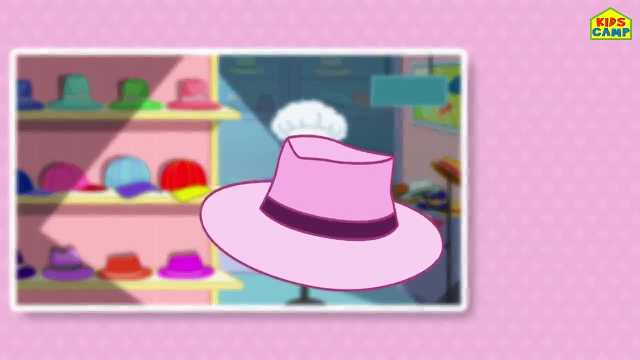 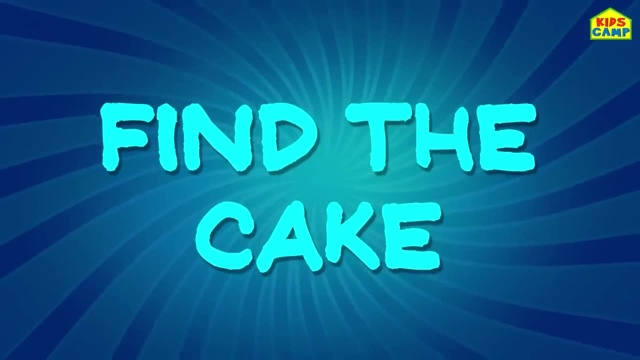 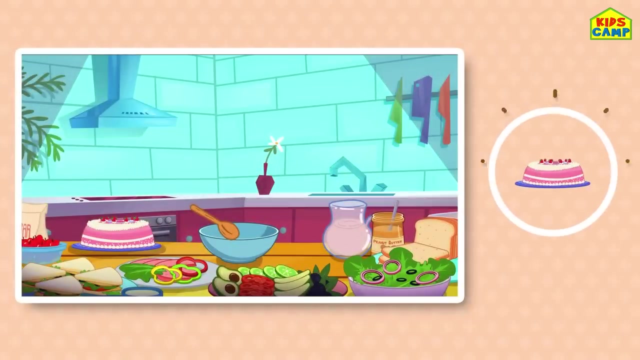 Yes, that's the one. Good job, kids, You found it. Woo-hoo, Find the cake. Hmm, delicious, Let's look for the cake. Wow, there is so much food on the table. Can you look for the cake? 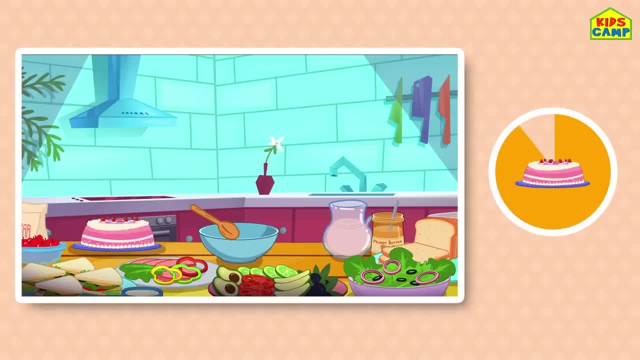 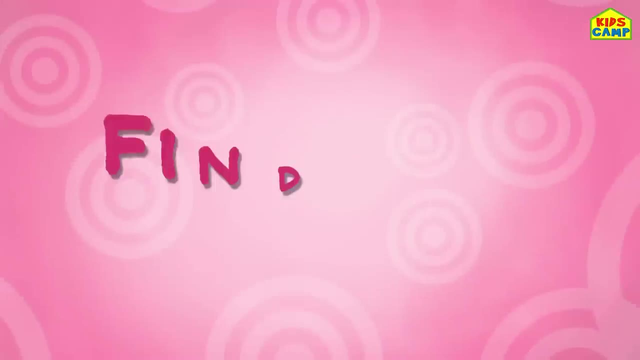 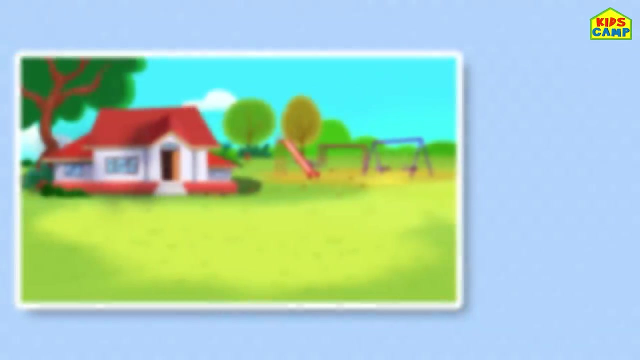 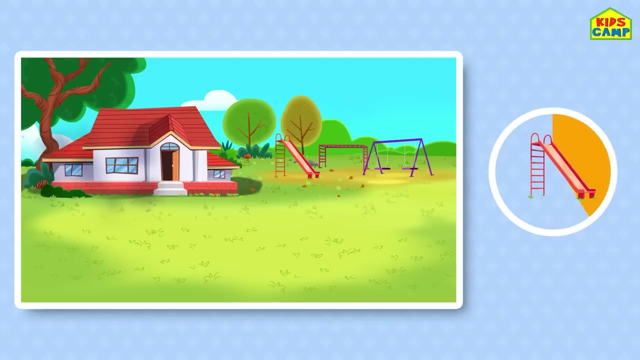 Where's the cake? Time's up. That's right, There it is. You found the cake Looks delicious. Find the slide. Wow, I love the slides. Where's the slide? Can you spot it? Keep looking, Time's almost. 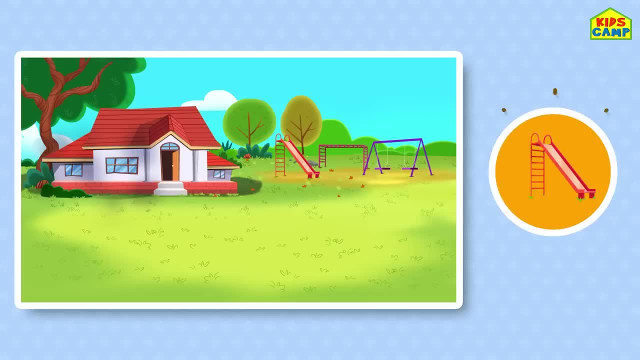 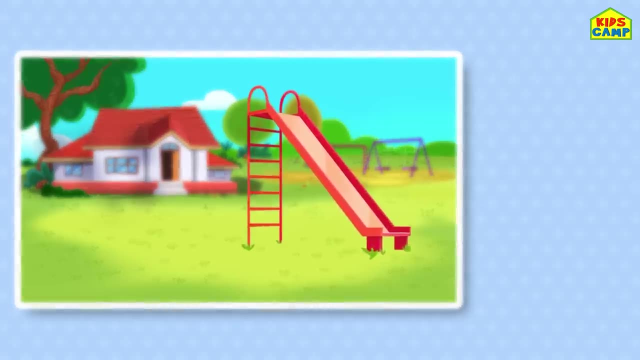 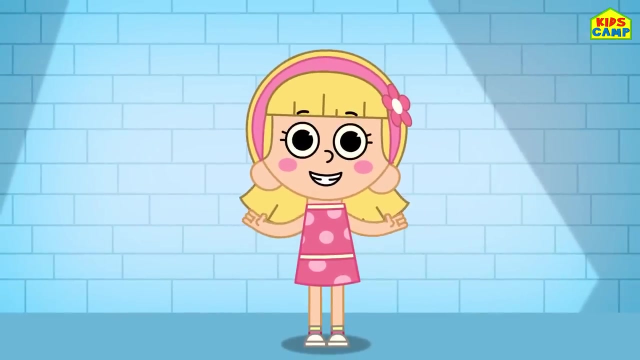 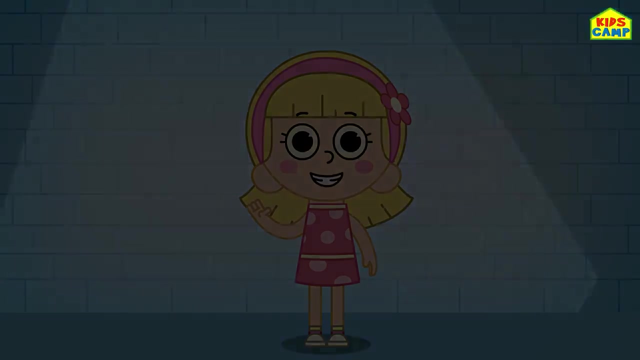 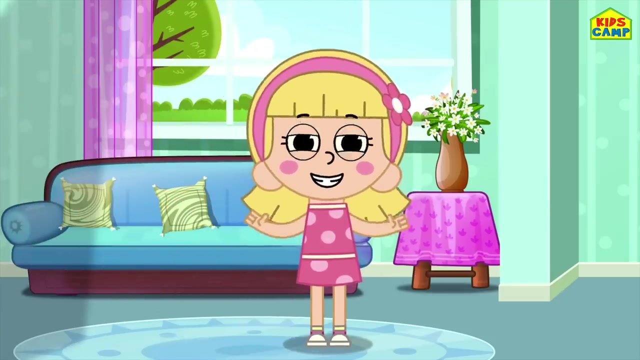 up. Uh-oh, Time's up. Yes, that's right, We found the slide. Woohoo, Good job. We had so much fun finding the objects. See you soon. Bye-bye. Today we are going to play with puzzles, Don't we all love puzzles? That's right, Let's start. 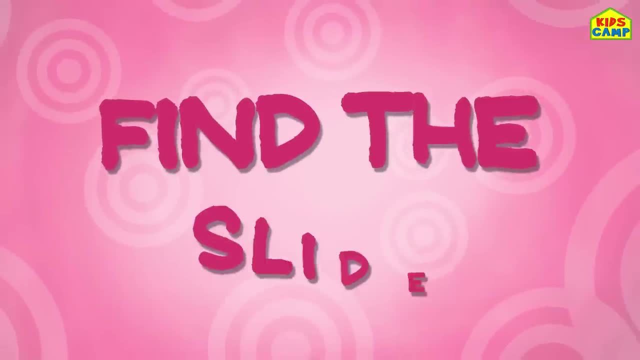 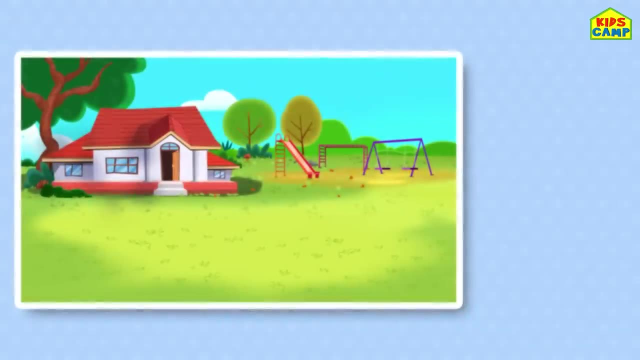 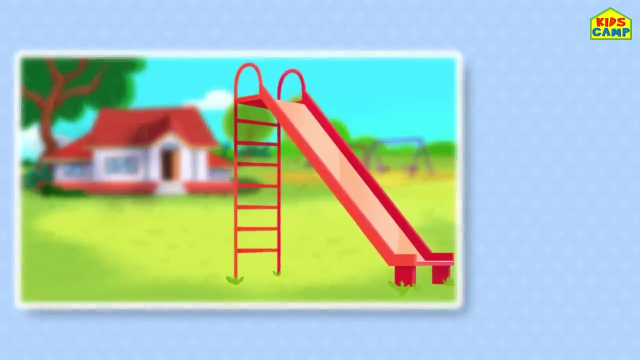 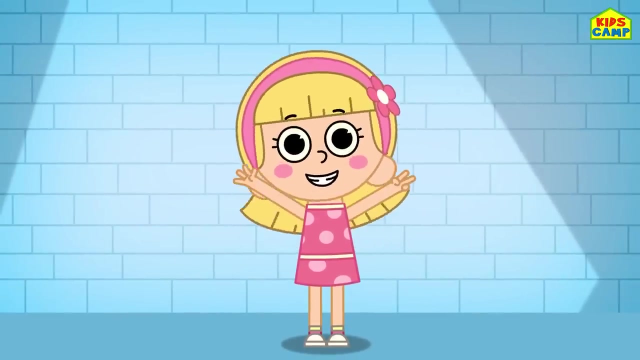 Looks delicious. Find the slide. Wow, I love the slides. Where's the slide? Can you spot it? Keep looking. Time's almost up. Uh, oh, time's up. Yes, that's right, We found the slide. Woohoo, good job, We had so much fun finding the objects. See you soon. 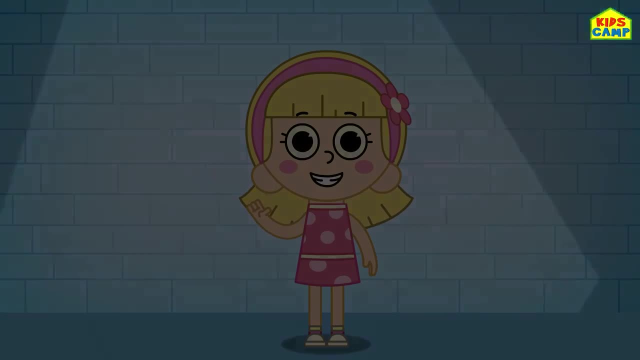 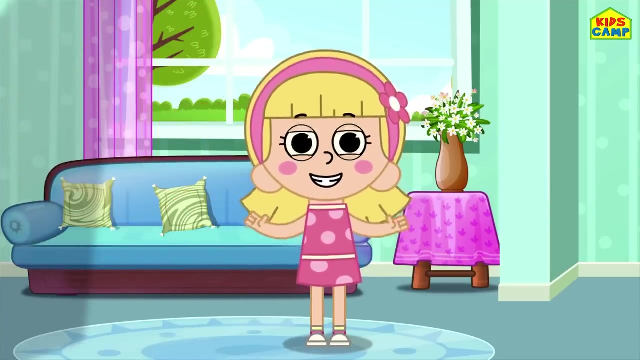 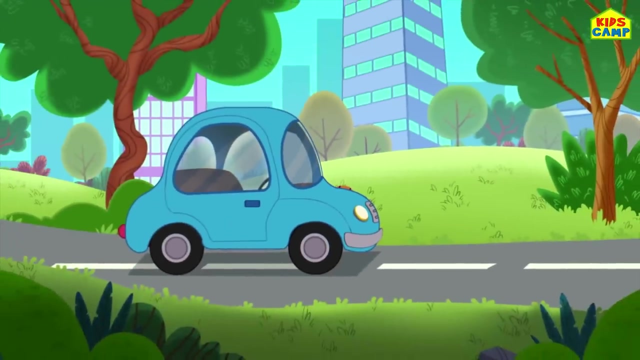 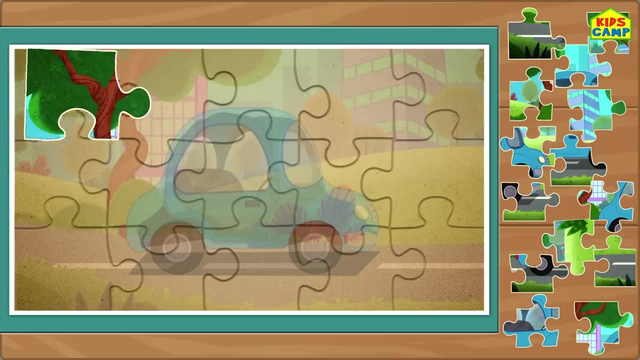 Bye, bye. Hi kids, I'm Ellie And today we are going to play with puzzles. Don't we all love puzzles? That's right, Let's start. Oh, that's a car. Let's put all the pieces together. Let's start with the corners. That's right, It goes right there. 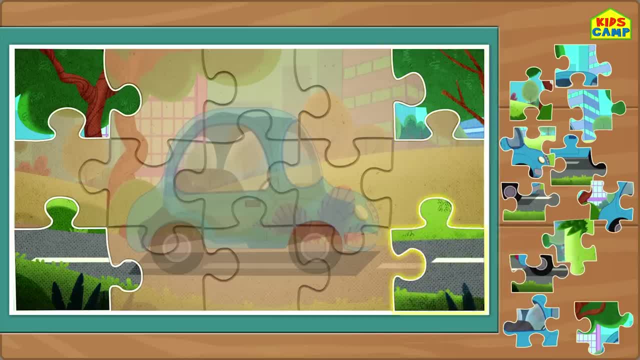 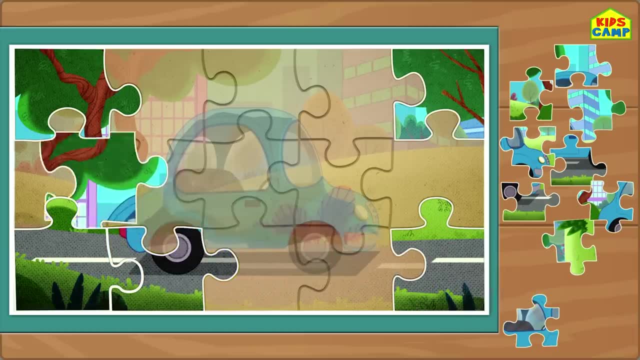 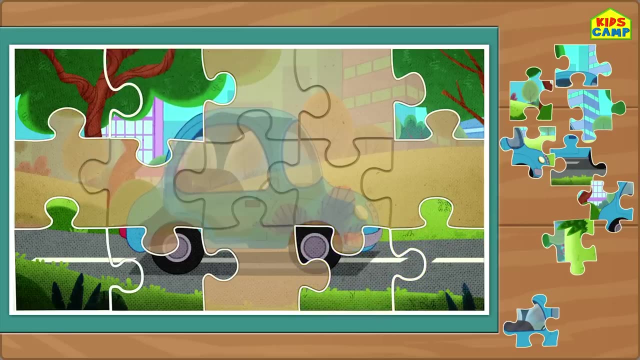 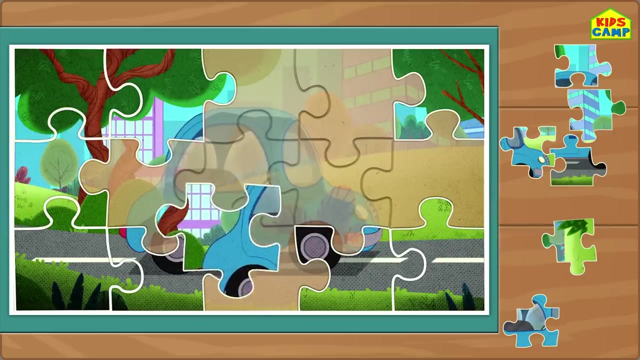 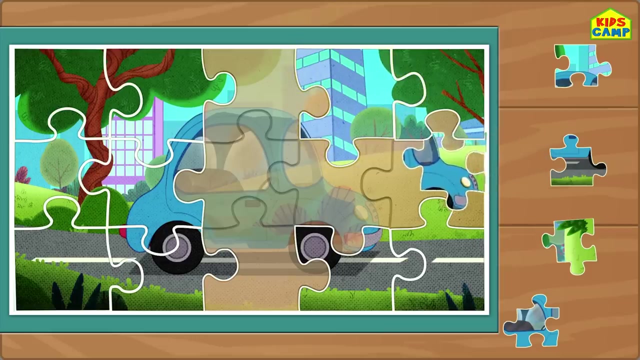 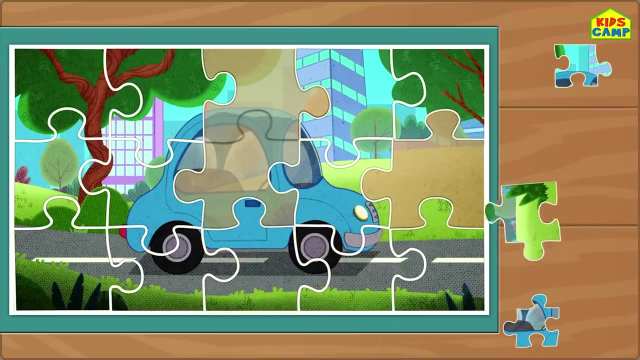 That's right. Perfect, We got all the four corners. No, that goes up there. That's right. Another wheel, perfect. Great. Uh, oh, That's right. Wow, This is so much fun. I like puzzles, don't you? No, no, that doesn't seem right Now. it is Perfect. And the last piece. 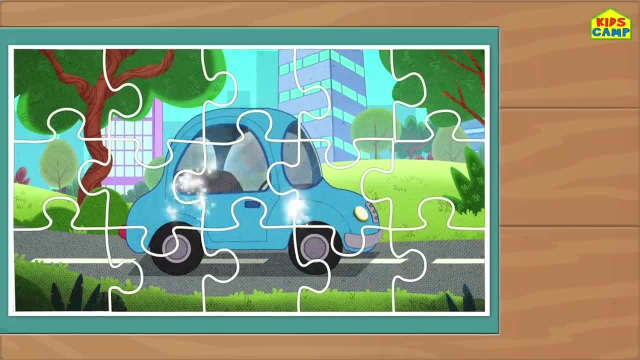 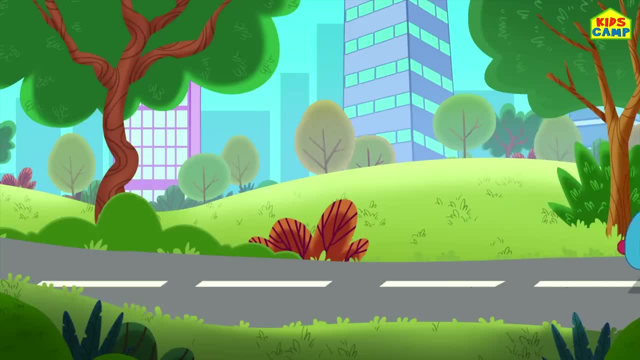 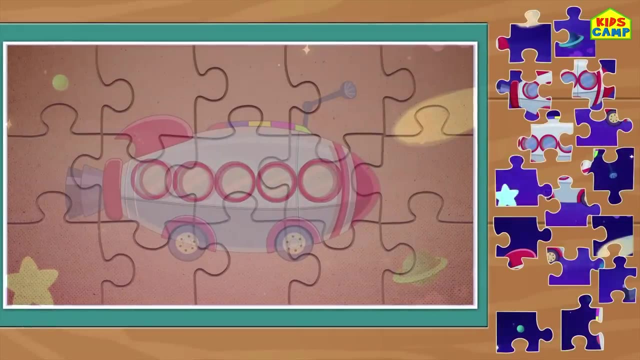 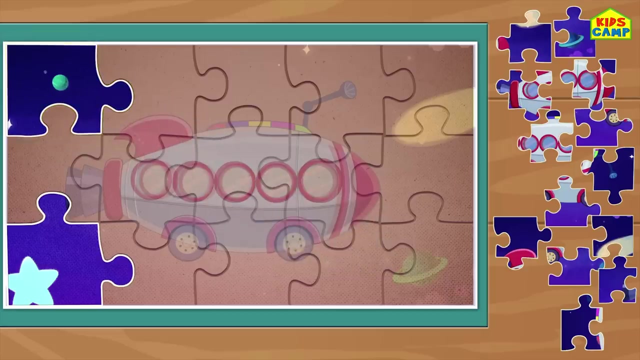 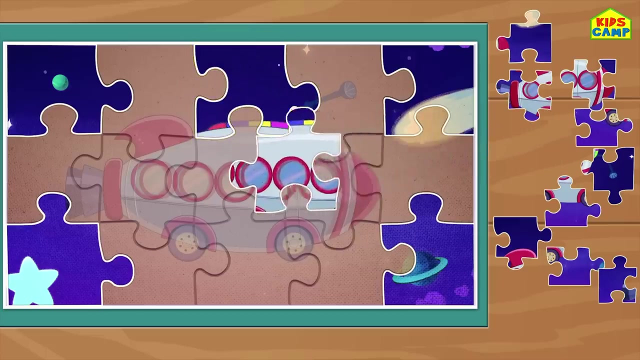 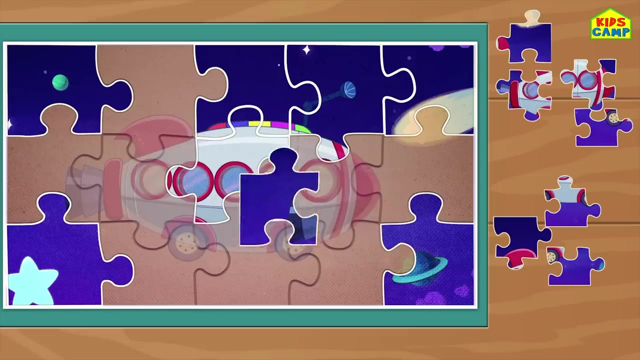 Woohoo, we did it. kids, There goes my car, Vroom, vroom, And Now we have a spaceship. Let's start with the corners. That's right, That's right. Yay, we got all the four corners. Uh oh Yes, Wow, the windows. Perfect, Woohoo. 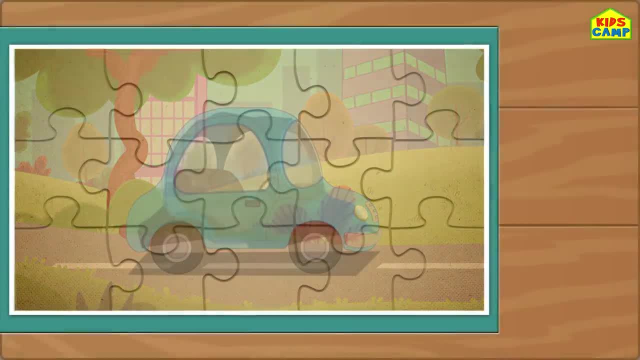 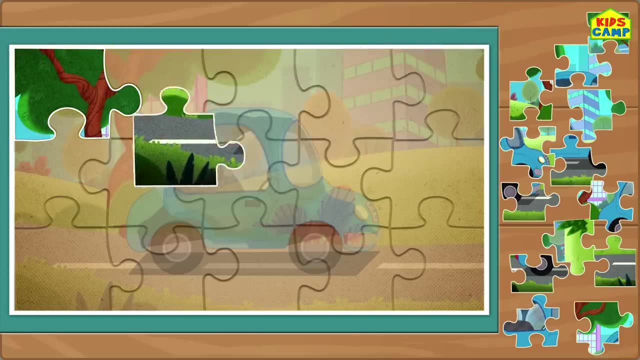 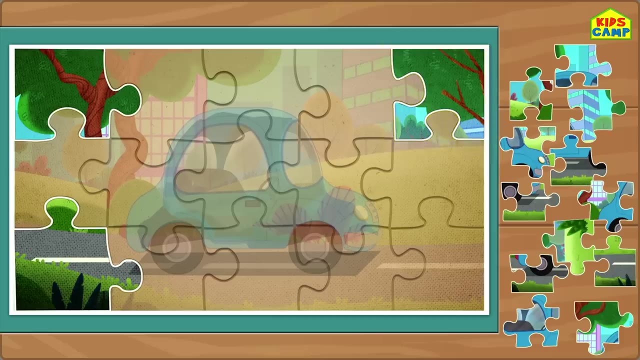 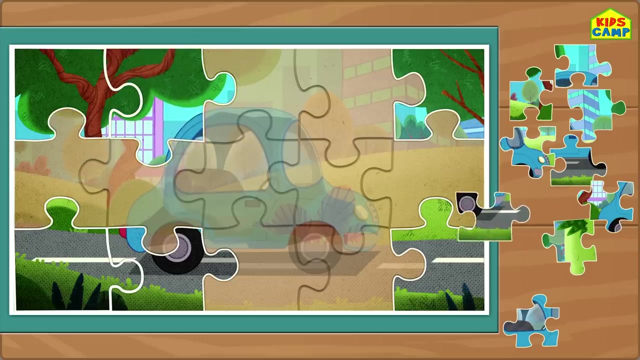 Oh, that's a car. Let's put all the pieces together. Let's start with the corners. That's right. It goes right there. That's right. Perfect, We got a car. That's right. Let's start with all the four corners. No, that goes up there. That's right. Another wheel. 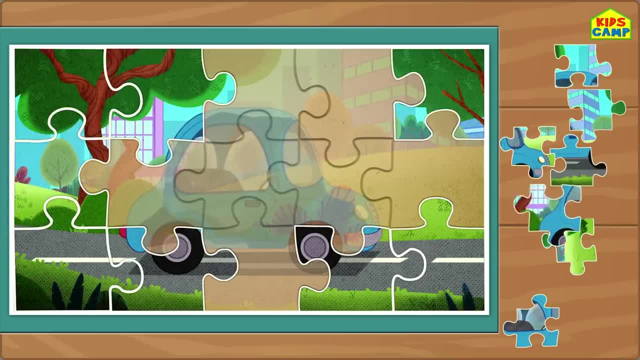 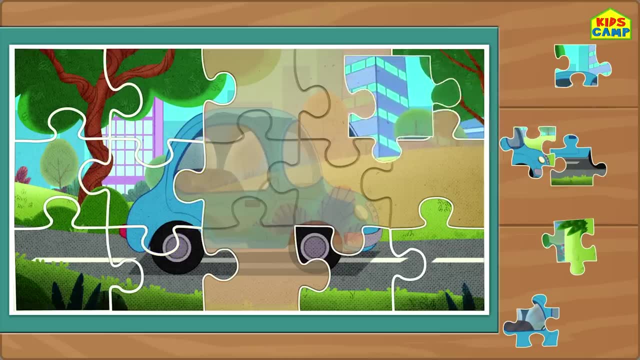 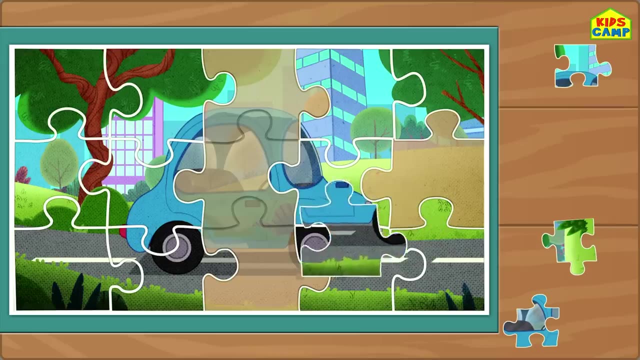 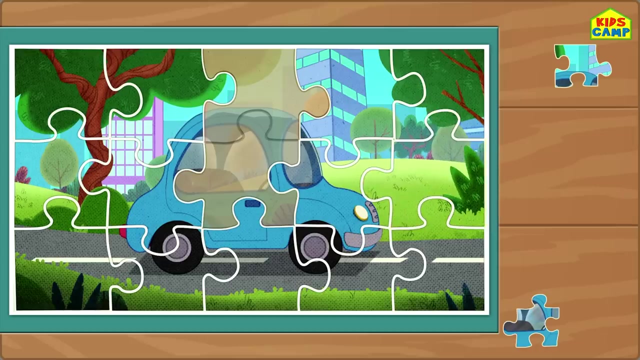 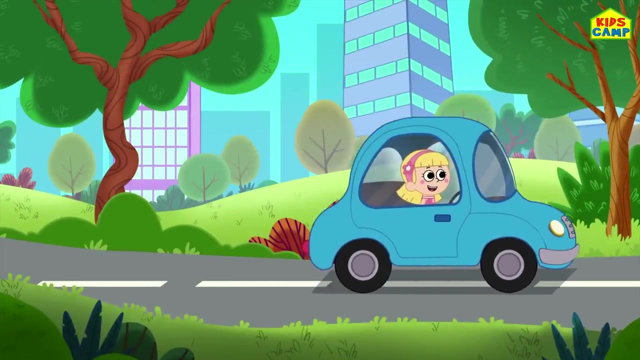 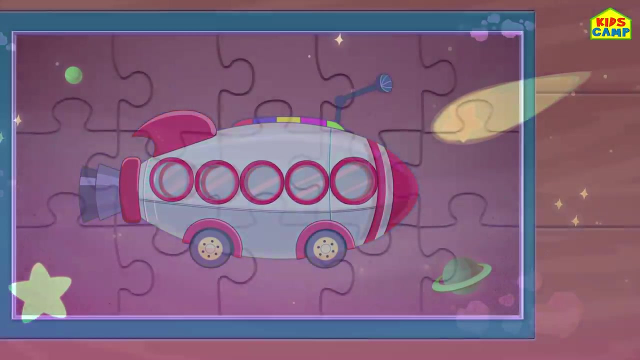 Perfect, Great, Uh-oh, That's right. Wow, This is so much fun. I like puzzles, Don't you? No, no, That doesn't seem right. Now it is Perfect. And the last piece? Woohoo, We did it. kids, There goes my car, Vroom, vroom, And now we have a spaceship. 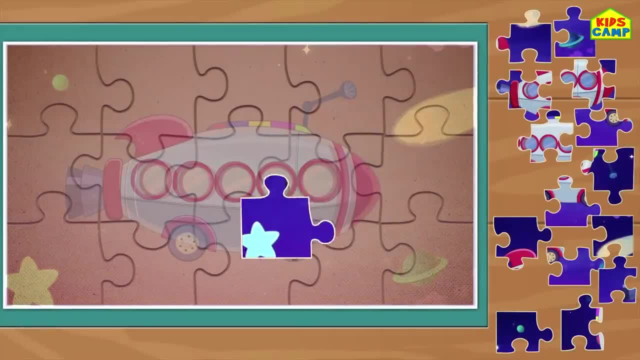 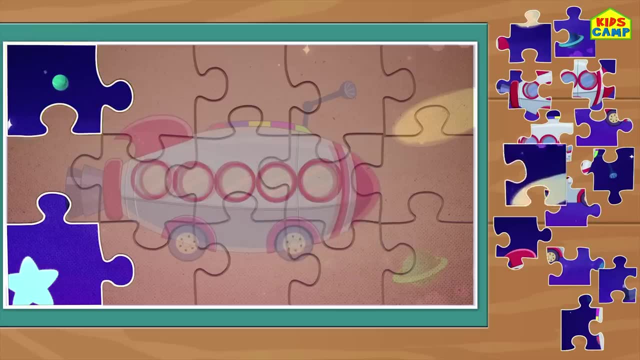 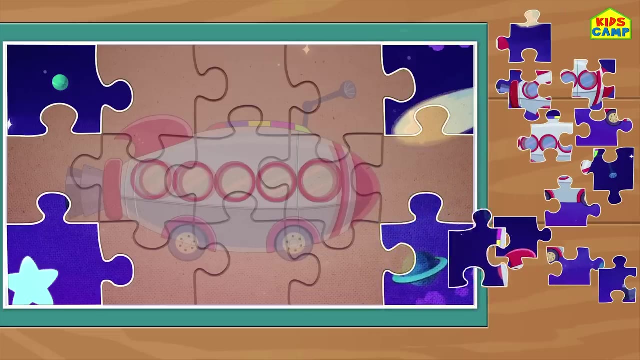 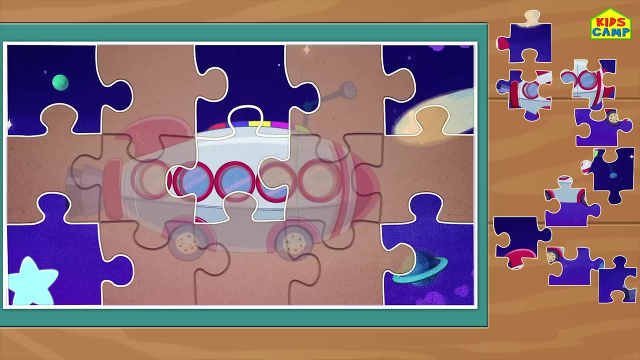 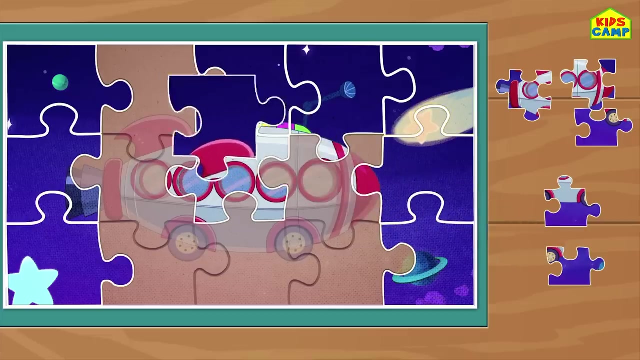 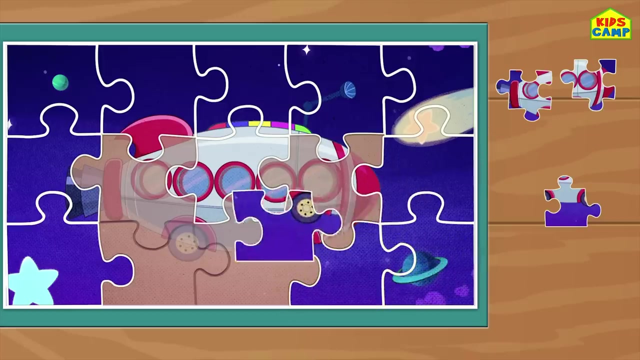 Let's go. Let's start with the corners. That's right. Yay, We got all the four corners. Uh-oh, Yes, Wow, The windows Perfect. Woohoo, That's right, We're almost done. Just a few more to go. Perfect, A few more. 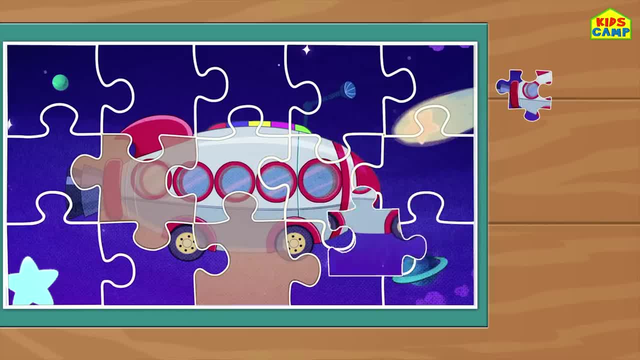 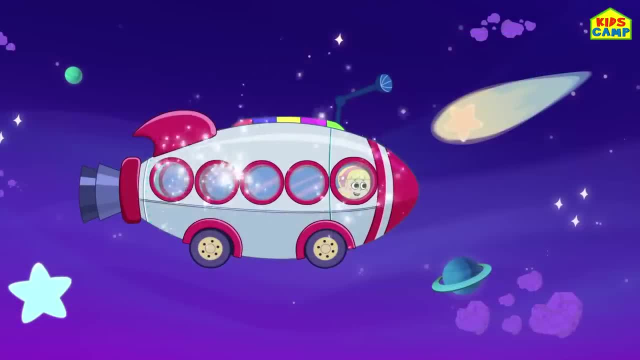 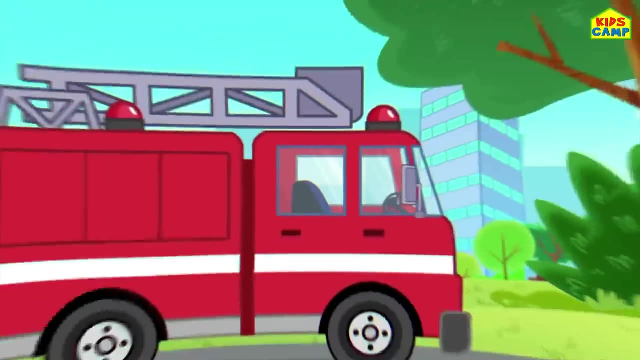 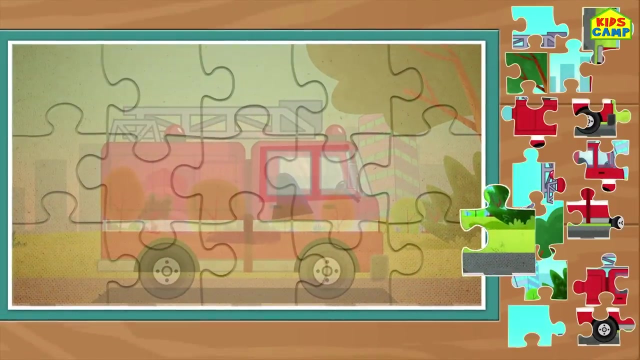 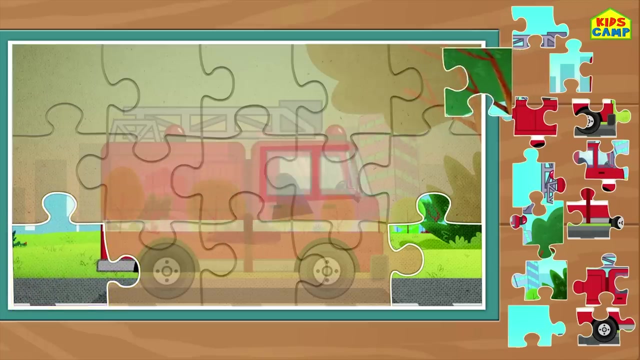 pieces. Wow, This looks so good. And the last piece: Our spaceship is completed And here I go: Woohoo, A fire truck. Once again, let's start with the four corners. Good job, kids, We're learning. 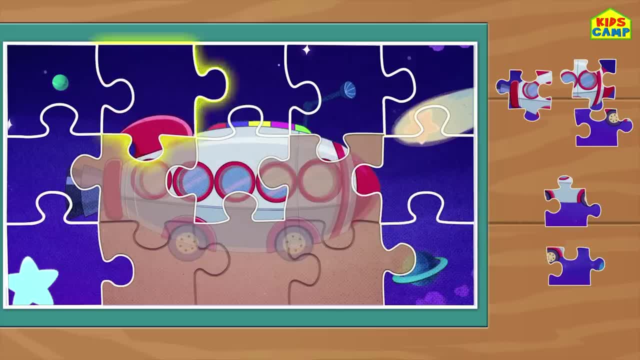 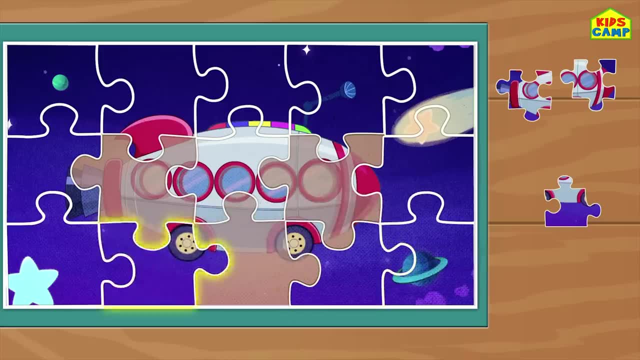 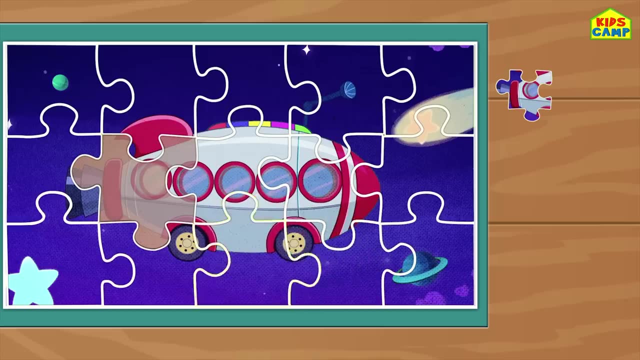 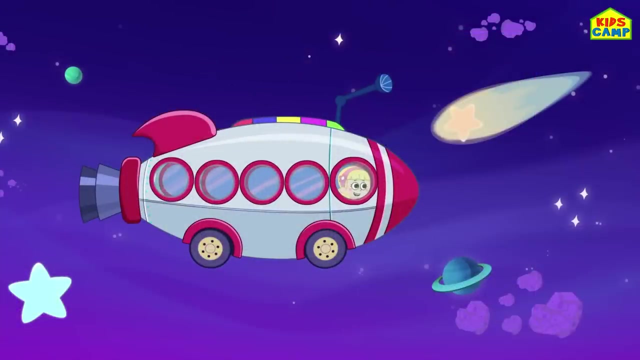 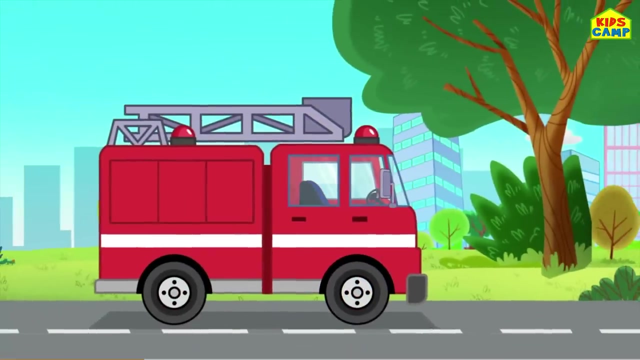 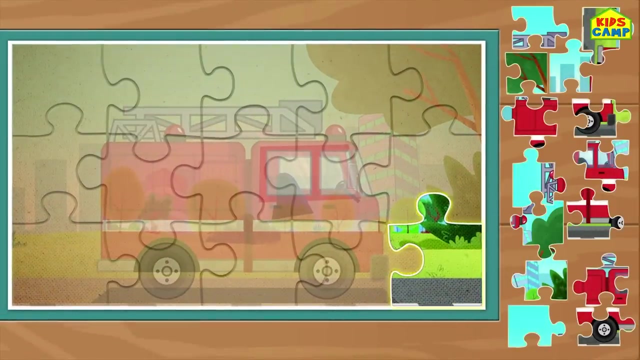 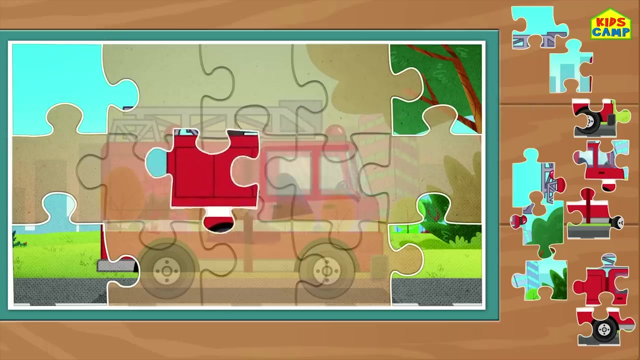 That's right, We are almost done. Just a few more to go Perfect. A few more pieces- Wow, this looks so good. And the last piece: Our spaceship is completed. And here I go- Woohoo, A fire truck Once again. let's start with the four corners. Good job, kids, we are learning. 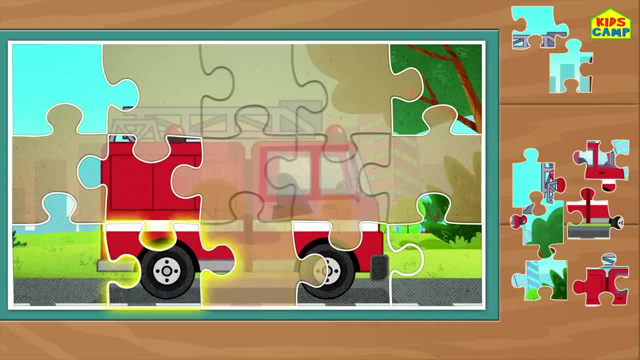 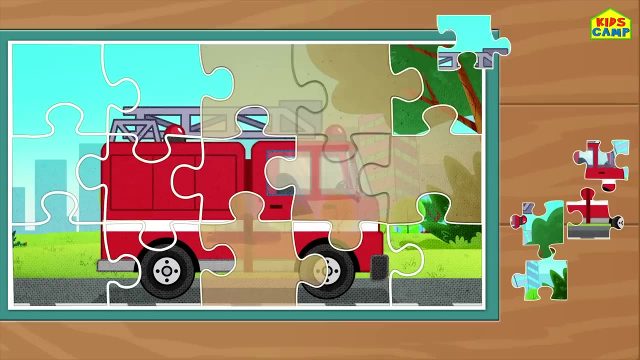 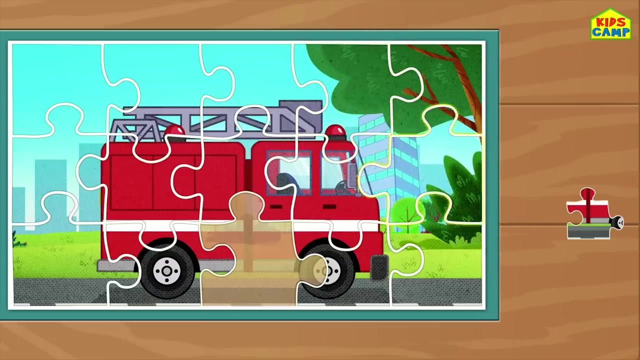 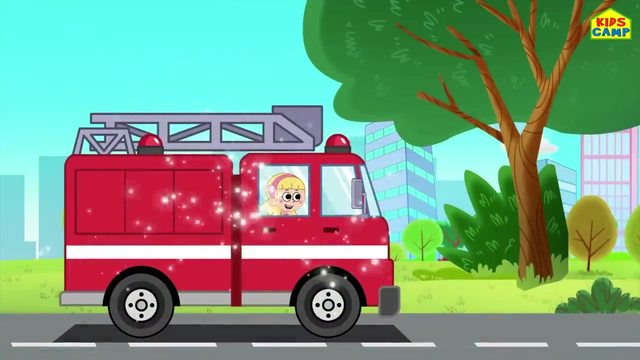 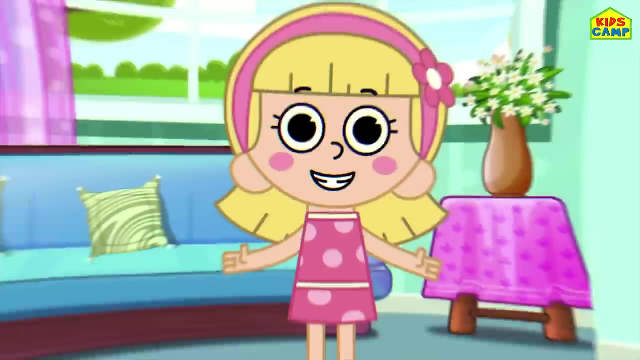 Oh, the wheels. And the second wheel. Oh, the center piece. Wow, we almost got it. A few more pieces That fits correctly. Oh, we gotta spin that around. Perfect. And the last piece. We did it. Our firetruck is ready to go, Wow, Yay, This was so much fun solving puzzles. 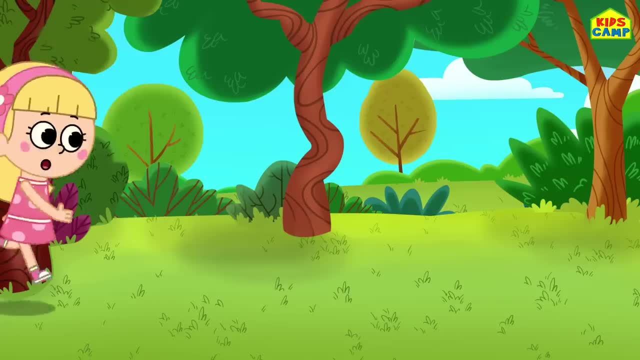 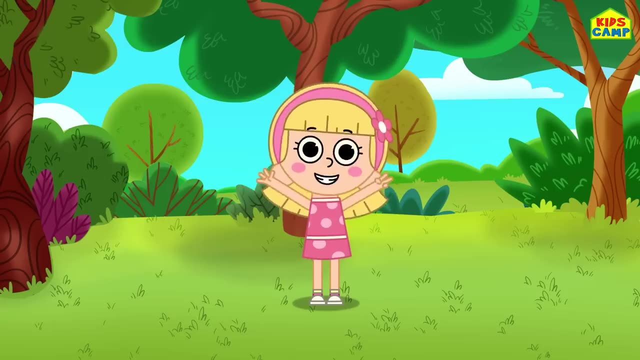 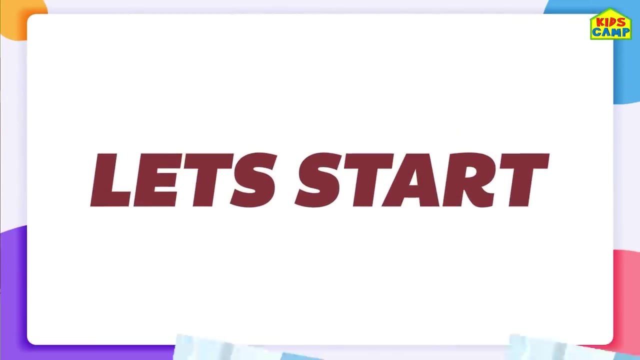 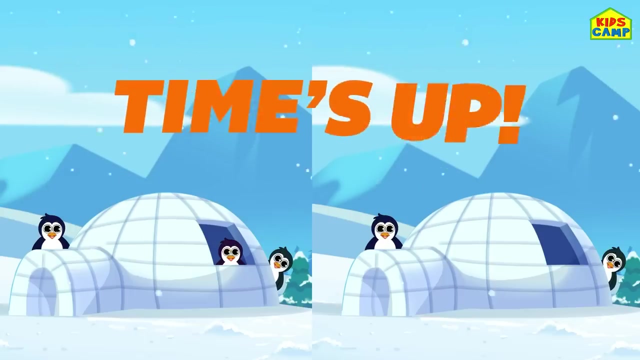 See you soon. Hi, I am Ellie And we are going to play a fun game. We have to spot the differences And this is going to be such a fun game. Ready, Let's start. Can you spot the difference? Time's up. 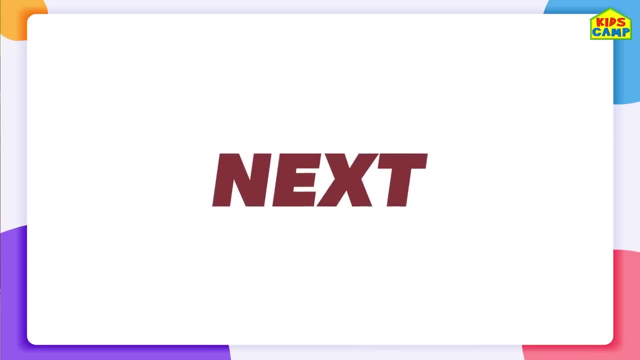 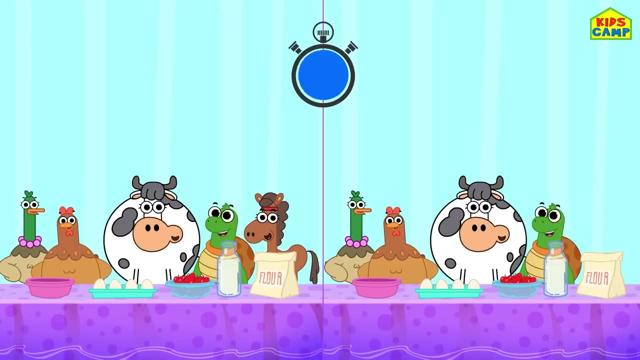 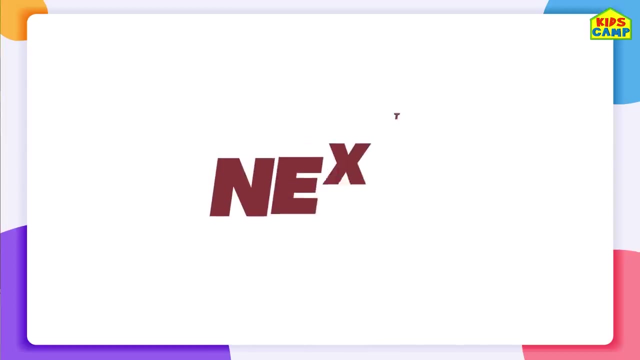 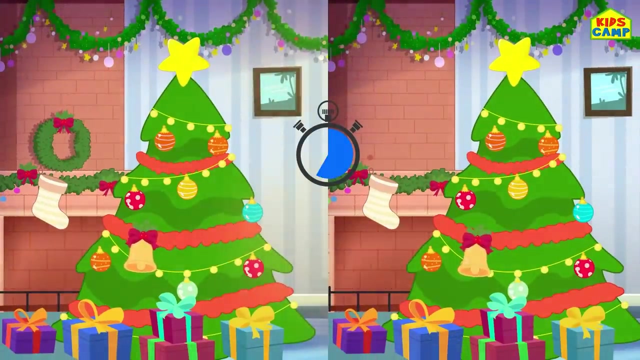 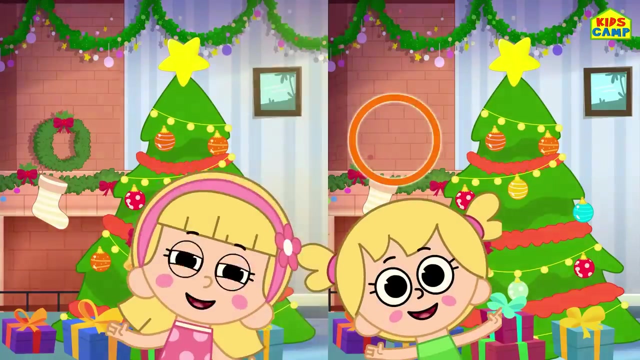 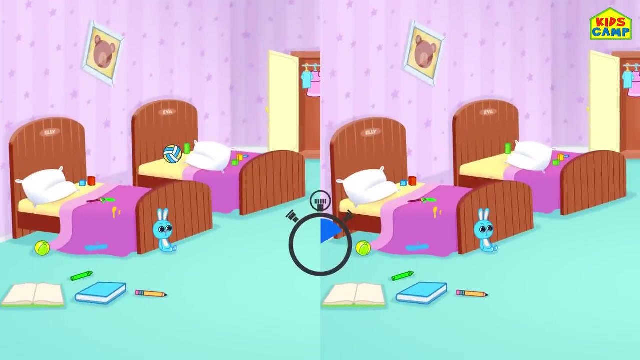 That's right. Next one: Can you spot the difference? Time's up, That's right. Yay, Can you spot the difference? Keep looking Time's up, That's right. Next one: Can you spot the difference? Keep trying. 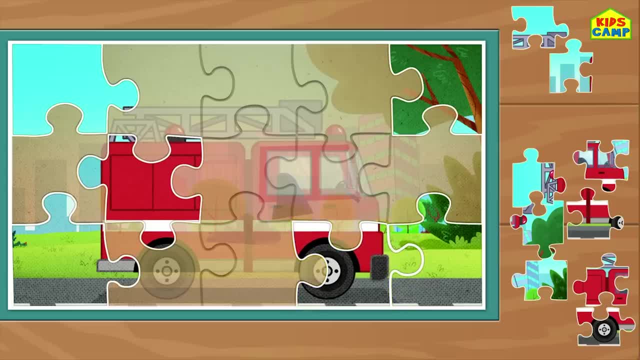 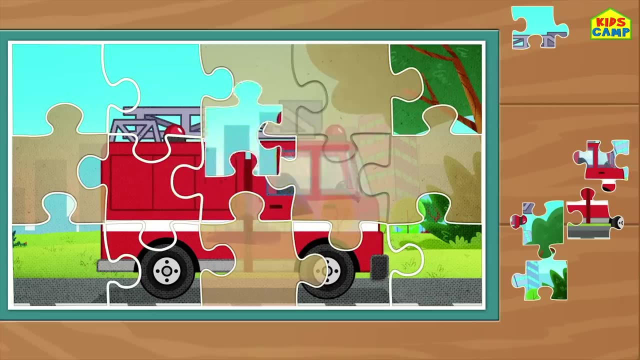 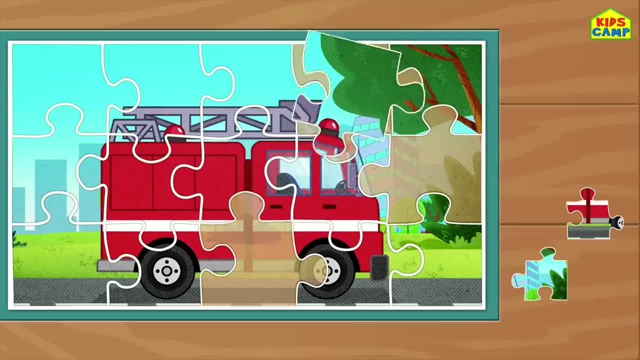 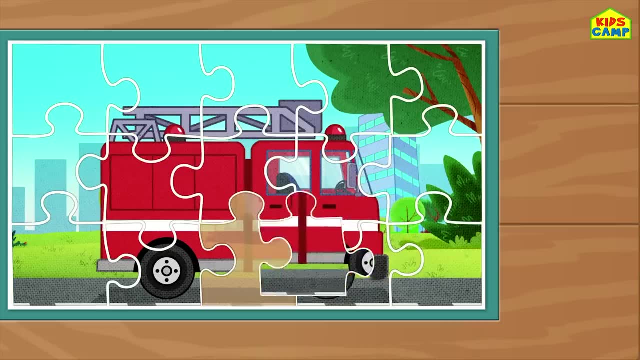 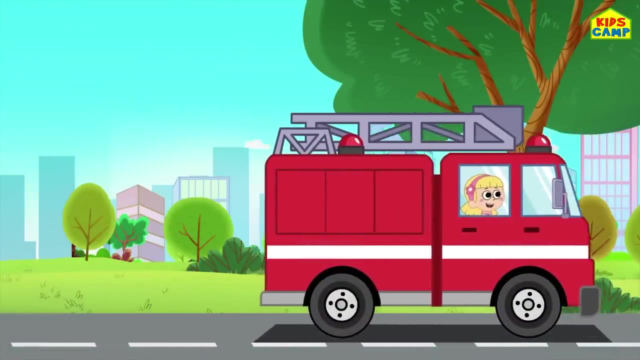 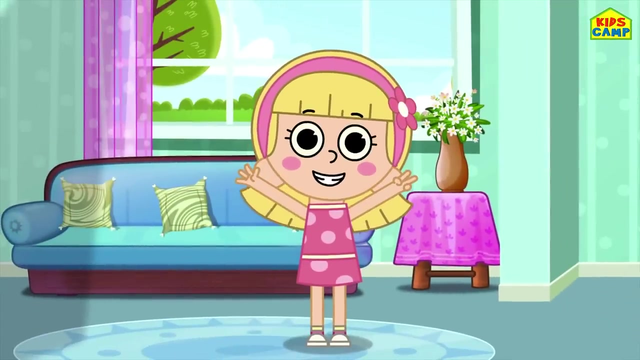 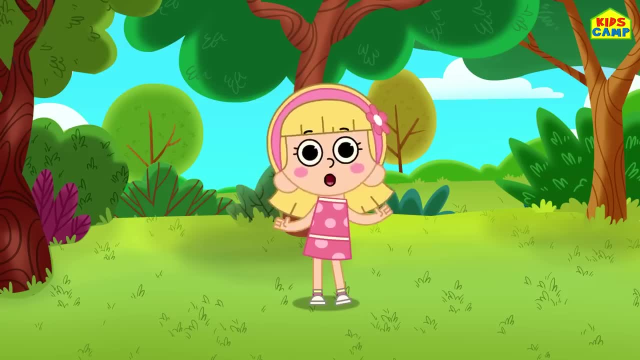 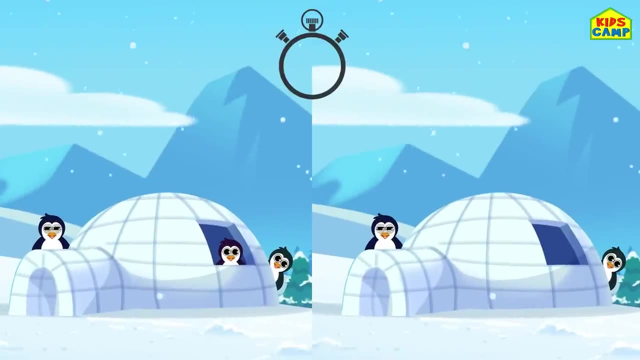 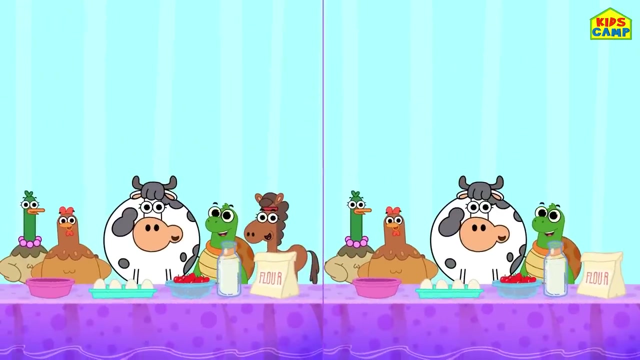 We have to spot the differences And this is going to be such a fun game. Ready, Let's start. Can you spot the difference Time's up? That's right. Next one: Can you spot the difference Time's up? 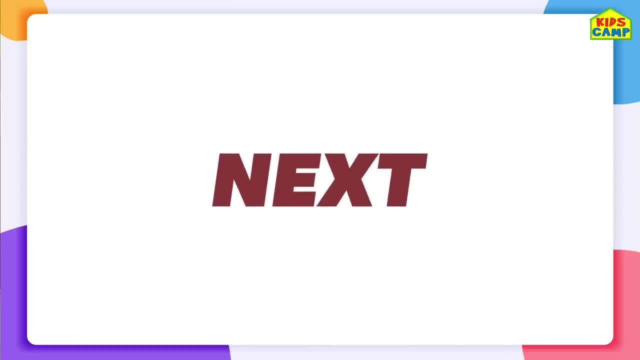 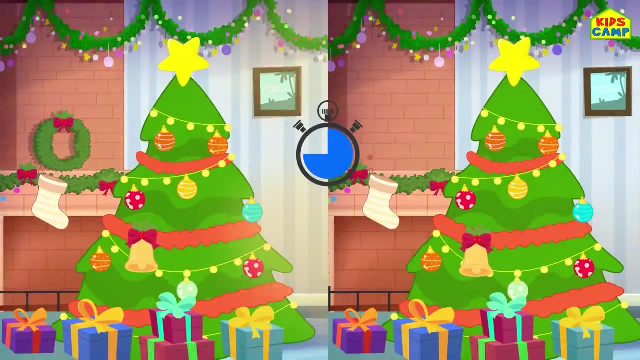 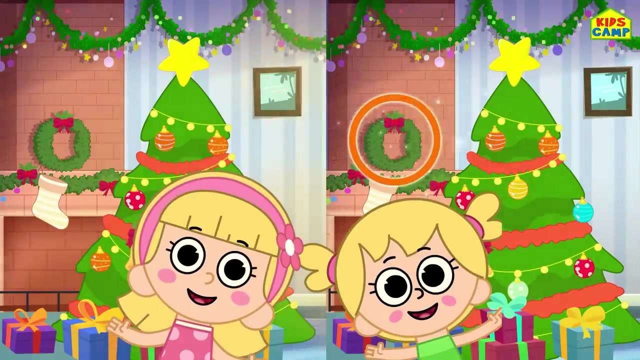 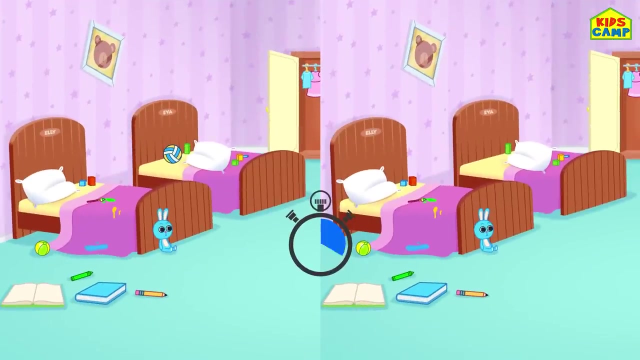 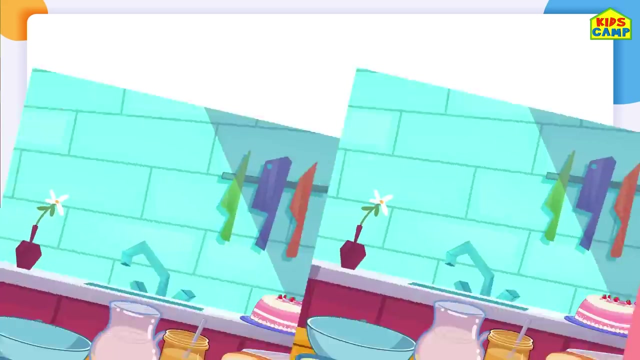 That's right. Can you spot the difference? Keep looking Time's up? That's right. Next one: Can you spot the difference? Keep trying Time's up? That's right. Next one: Can you spot the difference? Keep trying. 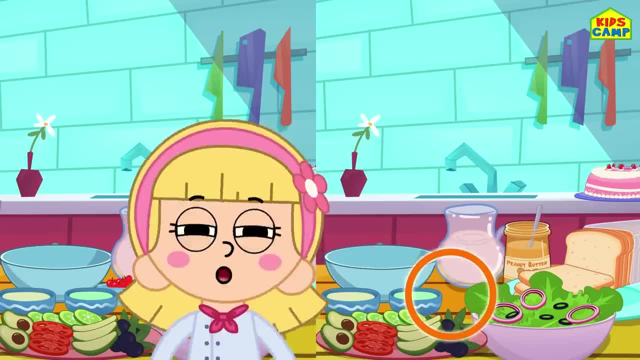 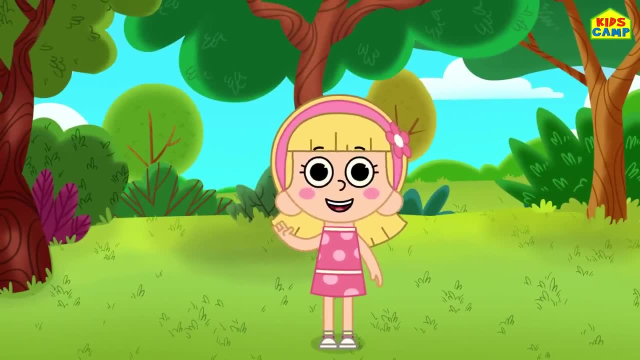 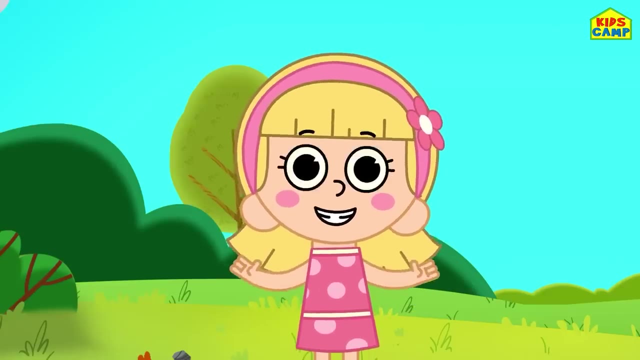 Time's up. Woohoo, You guys did it. Yay, This was so much fun. Bye-bye, Hi friends. I'm Ellie And I've learnt some new words. That's right. Do you also want to learn with me? Yes, Let's get started. 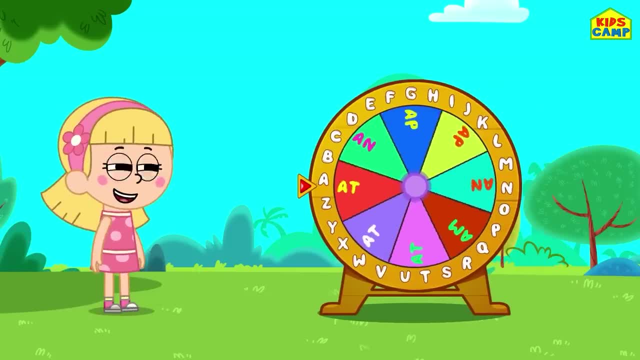 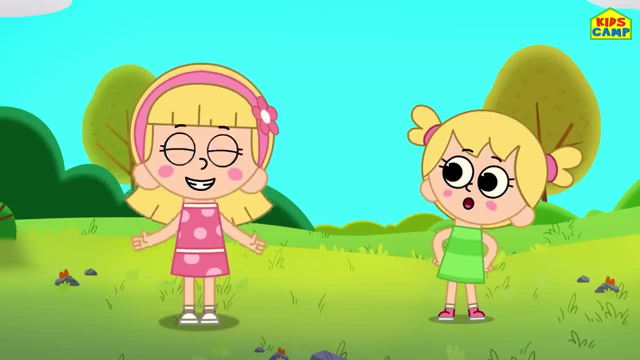 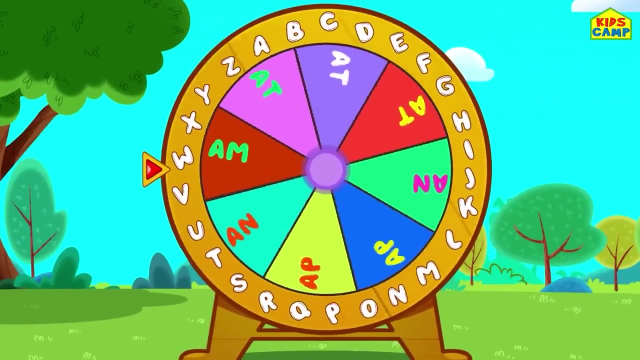 This is the word wheel. We have to spin the wheel and match the letter to make the correct word, And we also have clues. This is going to be so much fun. Let's get started. Let's spin the wheel, Woohoo. 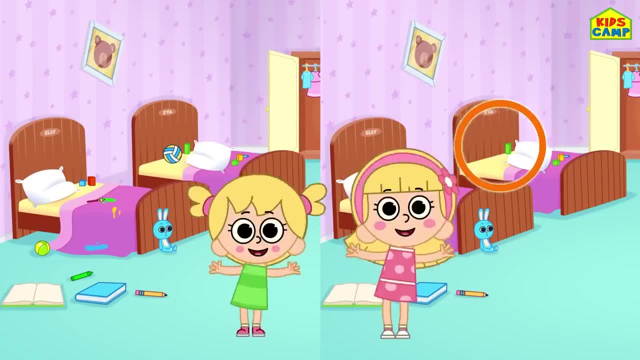 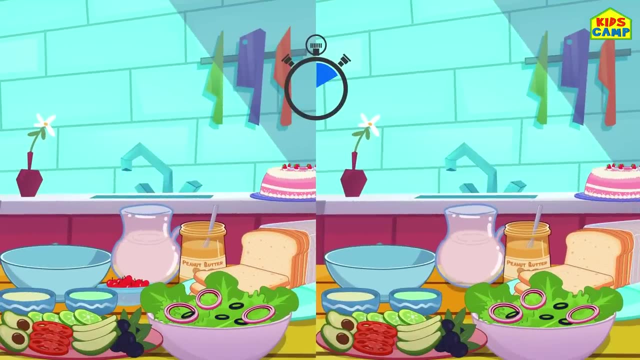 Time's up. Yay, Can you spot the difference? Keep trying Time's up. Yay, Can you spot the difference? Keep trying Time's up. Can you spot the difference? Can you spot the difference? Can you spot the difference? 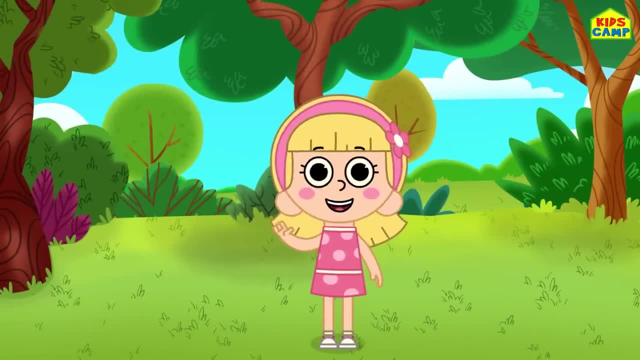 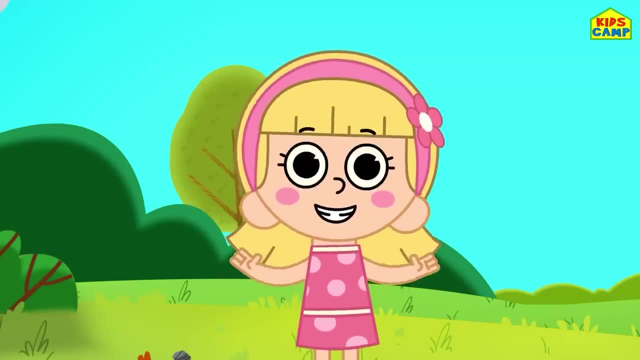 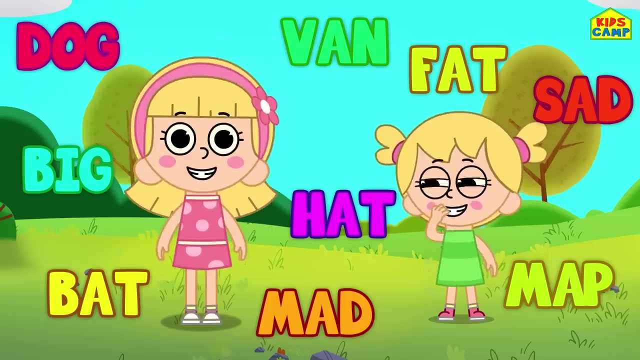 Yay, This was so much fun. Bye-bye, Hi friends. I'm Ellie and I've learned some new words. That's right. Do you also want to learn with me? Yes, Let's get started. This is the word wheel. 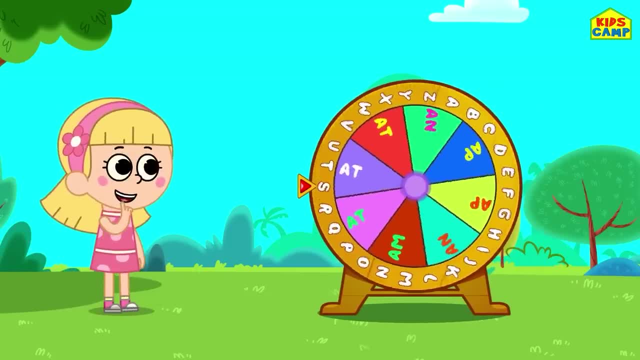 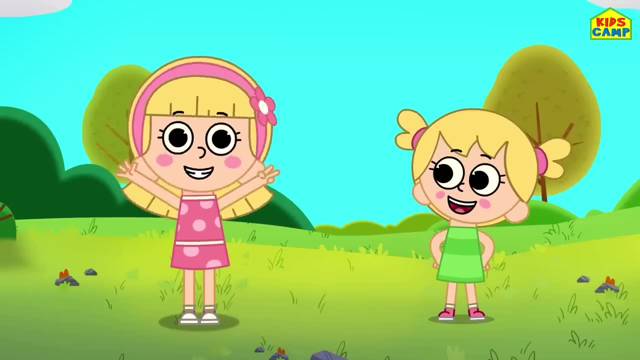 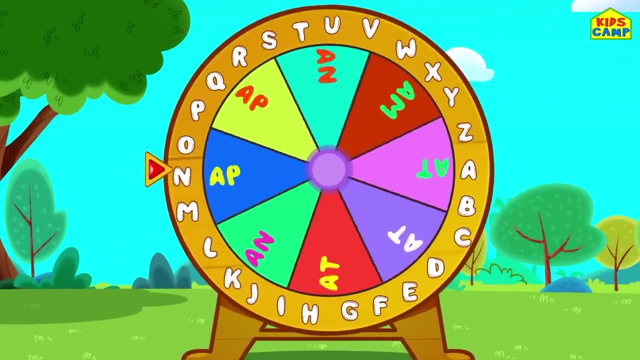 We have to spin the wheel and match the letter to make the correct word, And we also have clues. This is going to be so much fun. Let's get started. Let's spin the wheel. Woohoo, Is that a word? 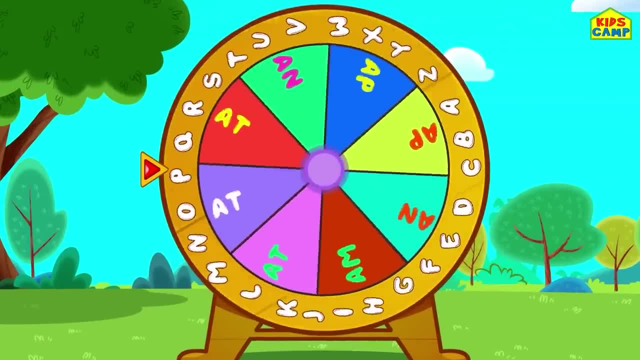 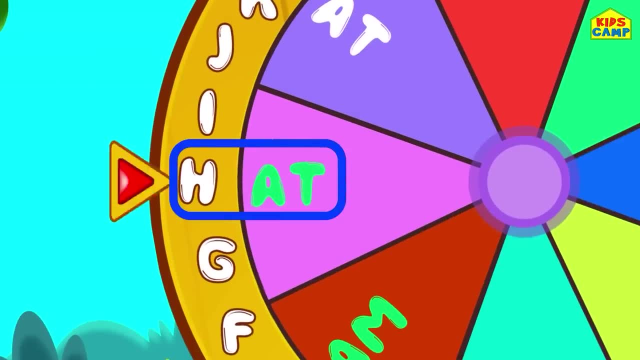 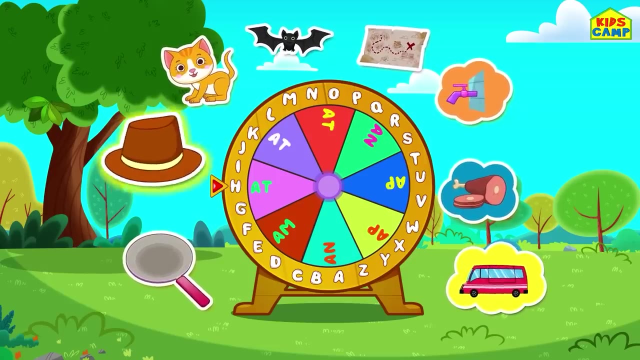 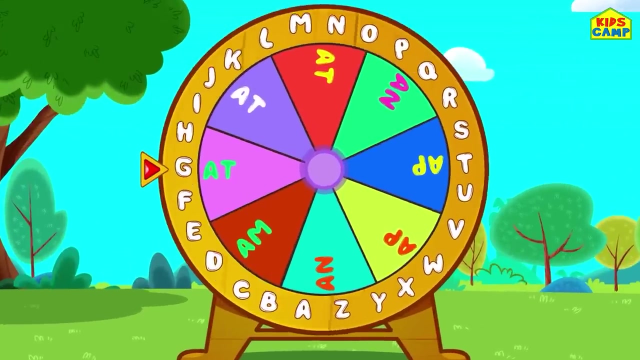 No, Let's keep spinning. Is that a word? H-A-T hat? That's right, That's how you spell a hat. We found the first word. Let's look for more. Let's spin the wheel, Woohoo. 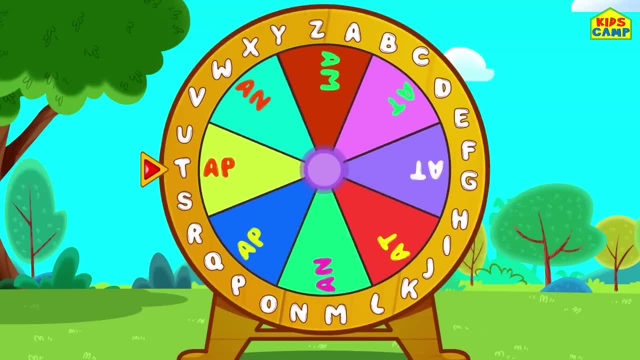 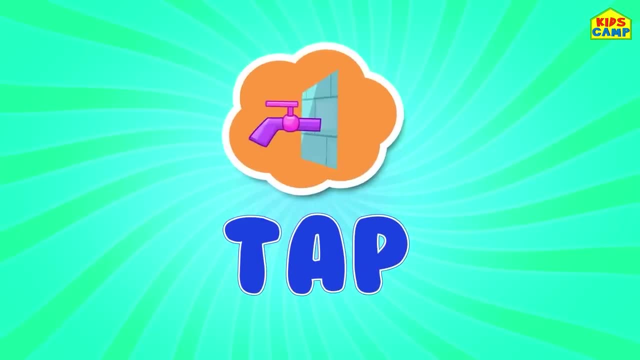 Is that a word? T-A-P? tap, That's right, That's a word, A tap. Wonderful, We've found one more. Let's look for some more. Keep spinning. Woohoo, Is that a word? P-P-A-P? 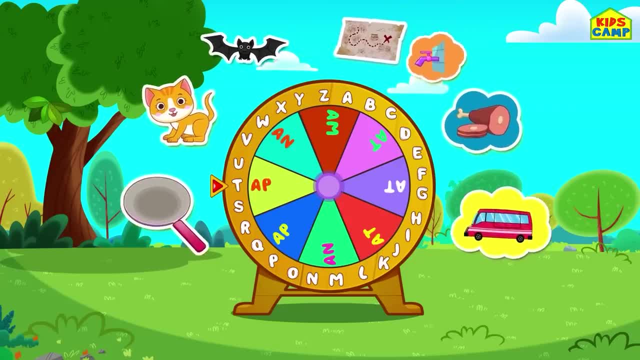 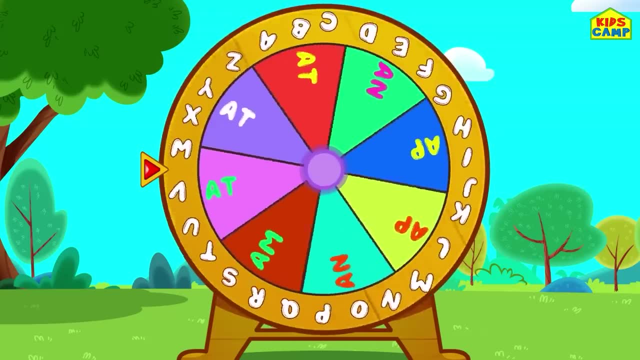 Yes, it's a word. Let's spin the wheel. Let's get started. Let's get started, Let's spin the wheel. Woohoo, Is that a word? No, Let's spin the wheel, P-P-A-P. 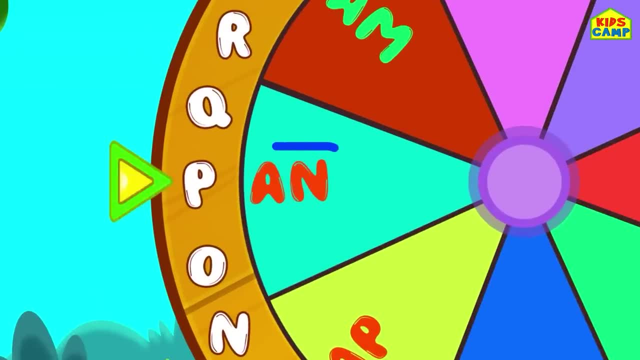 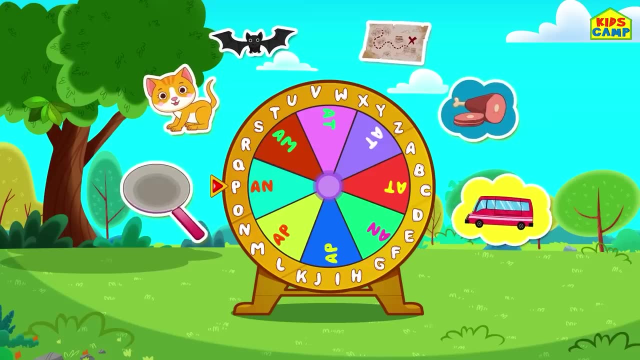 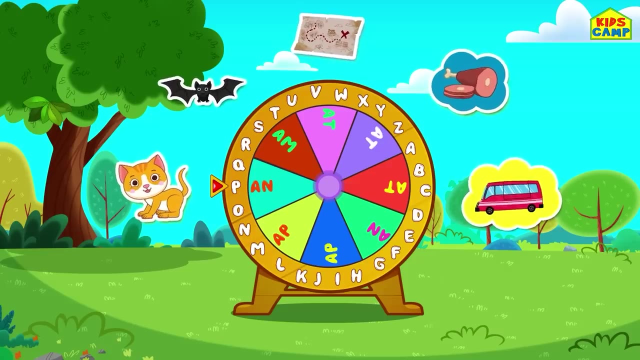 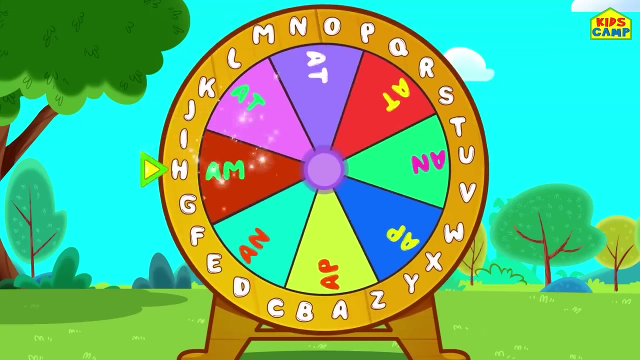 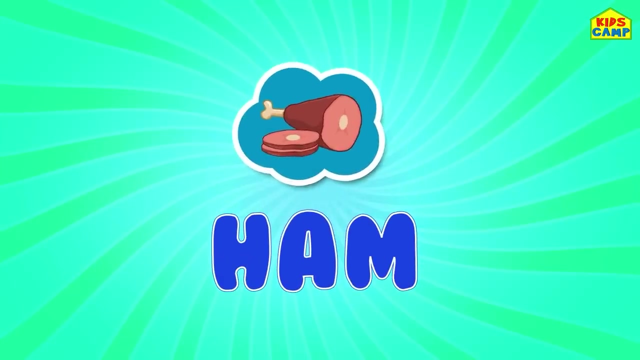 That's right, That's a word. P-A-N Pan- Yes, that's a word. Wow, we found another one. What's next? Let's keep spinning. Yay, Is that a word? H-A-M Ham- That's right, that's a word. Yummy. 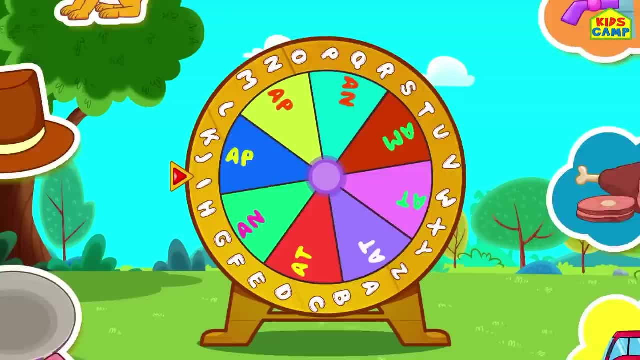 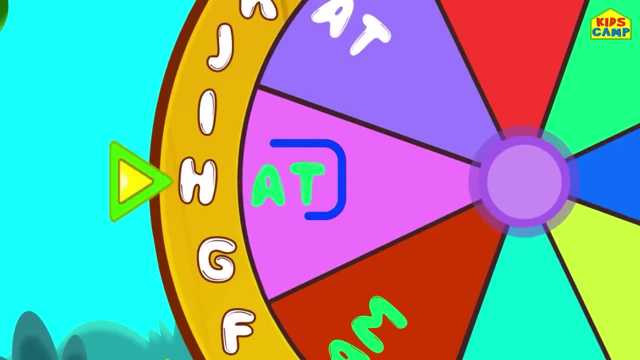 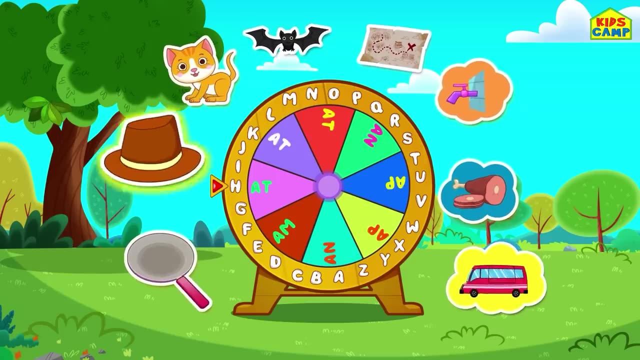 Is that a word? No, Let's keep spinning. Is that a word? H-A-T hat. That's right. That's how you spell a hat. We found the first word. Let's look for more. Let's spin the wheel. 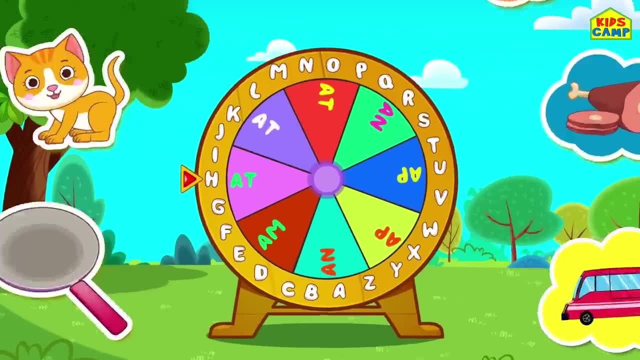 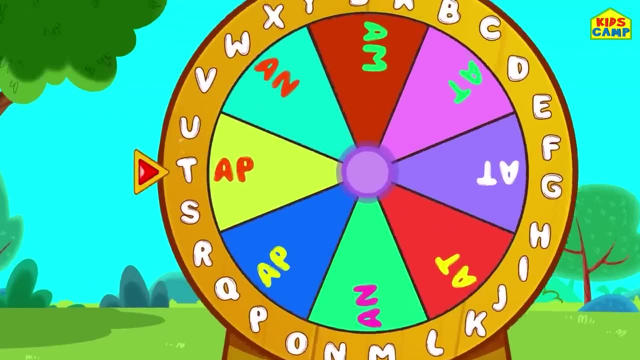 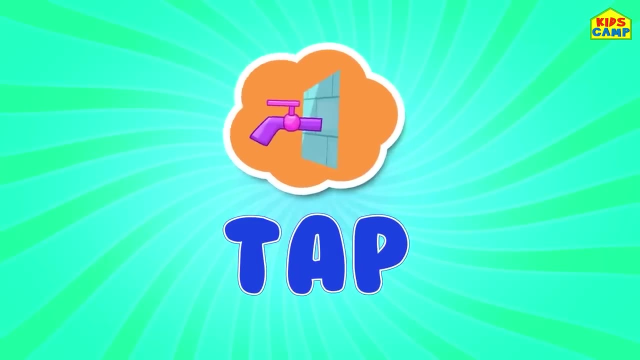 Woohoo, Is that a word T-A-P. tap? That's right, That's a word: A tap. Yay, Wonderful, We found one more. Let's look for some more. Let's spin the wheel, Woohoo. 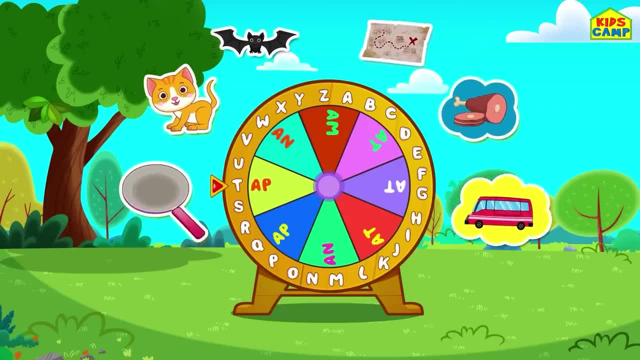 Is that a word? T-A-P. tap, That's right. That's right. Yay, We found another one. Let's spin the wheel. We found one more. Let's look for some more. Keep spinning, Woohoo. 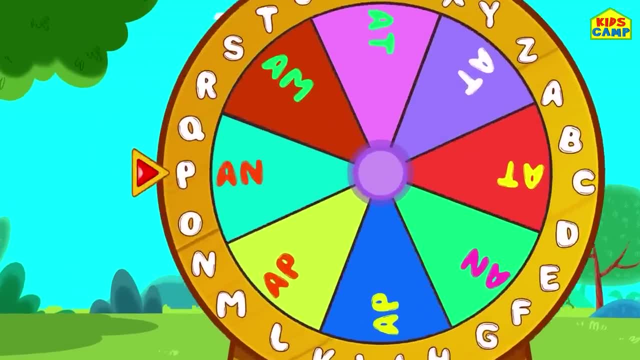 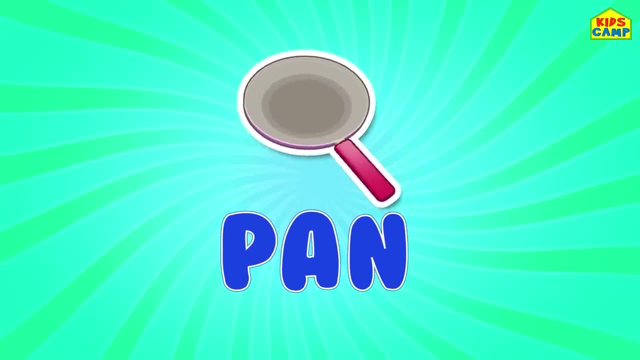 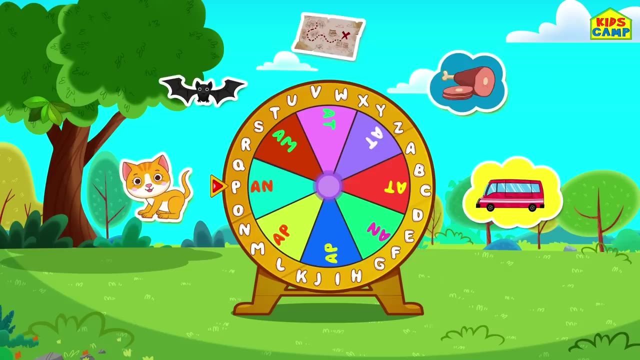 Is that a word? P-A-N Pan? Yes, that's a word. Wow, We found another one. What's next? Let's keep spinning. Yay, We are back. Wow, We're back. Yay, We are back. 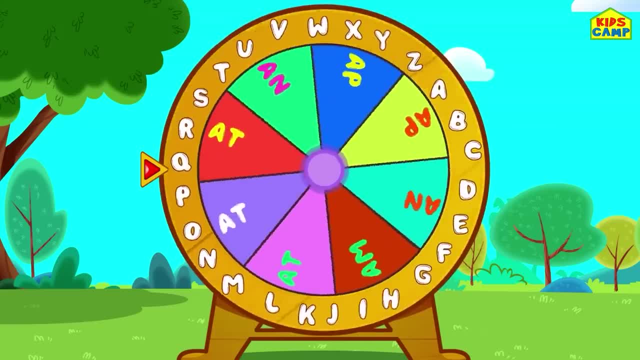 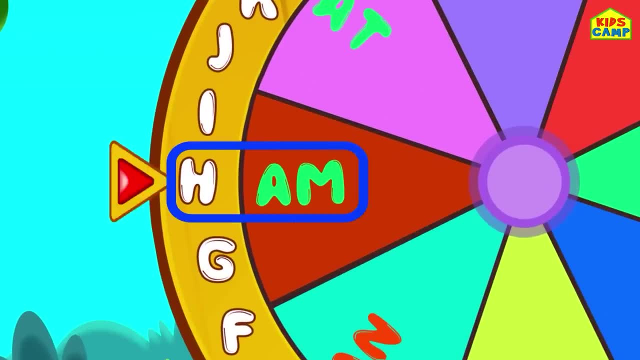 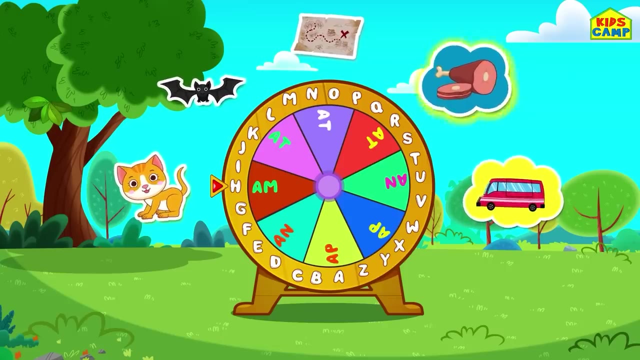 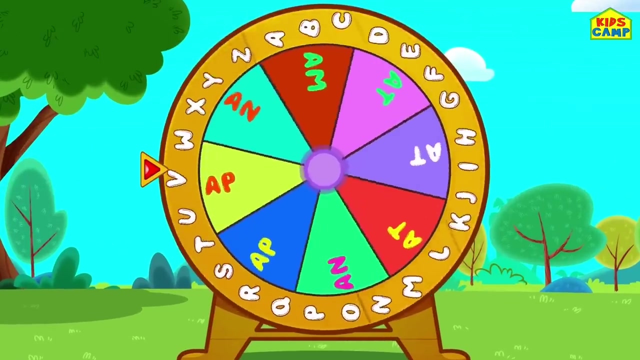 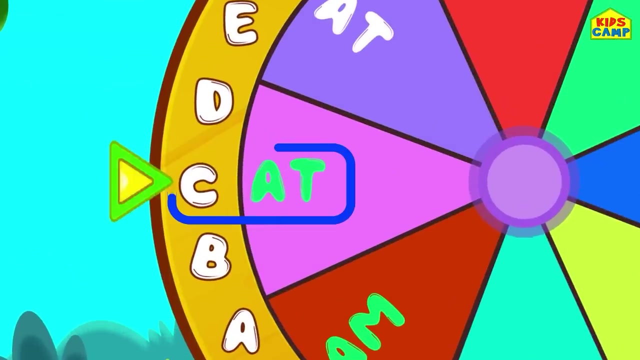 We're back. Is that a word? H-A-M. Ham, That's right, That's a word. Yummy, We found another one. Let's find some more friends. Let's spin the wheel. C-A-T. That's a word. Cat. 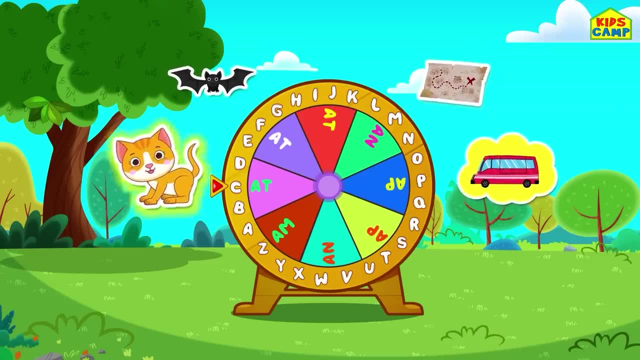 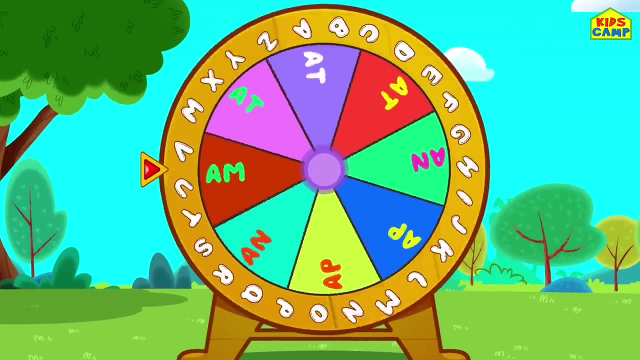 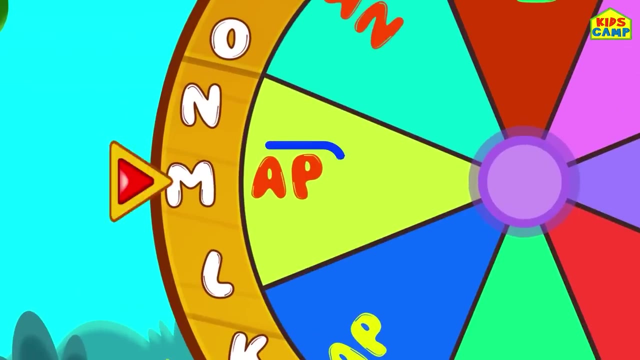 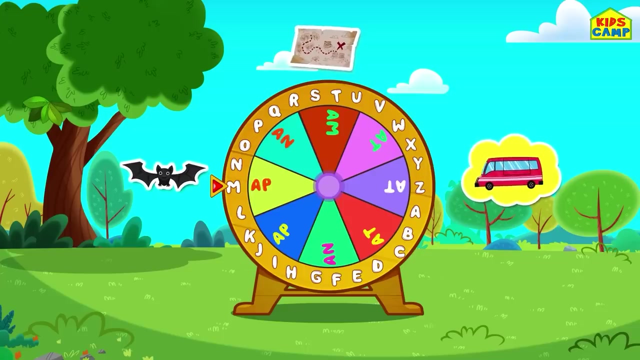 What's next? Let's spin the wheel again. Word wheel: Keep spinning. Uh-huh, We found another word: M-A-P Mouse, That's right. Map is a word. We found the word map. Good job, friends. Let's keep spinning the wheel. 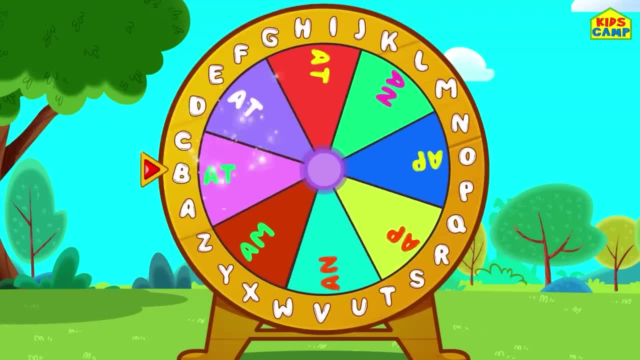 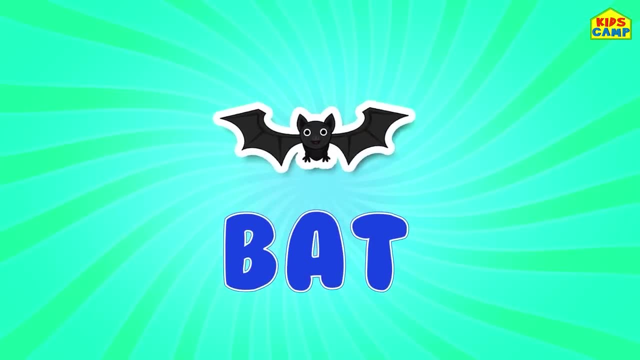 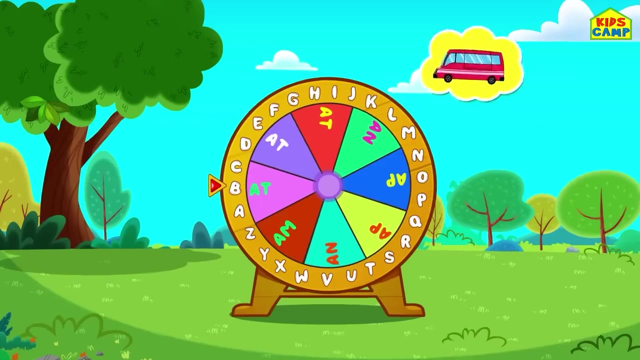 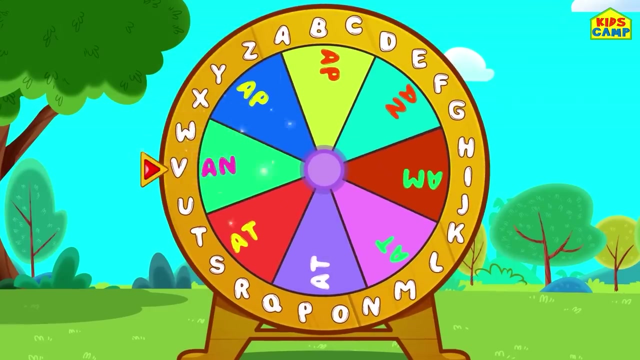 What's next? That's a bat B-A-T bat. That's right, We found another word: A bat. Good job, What's the last word? Let's keep spinning the wheel. It is A van B-A-N. 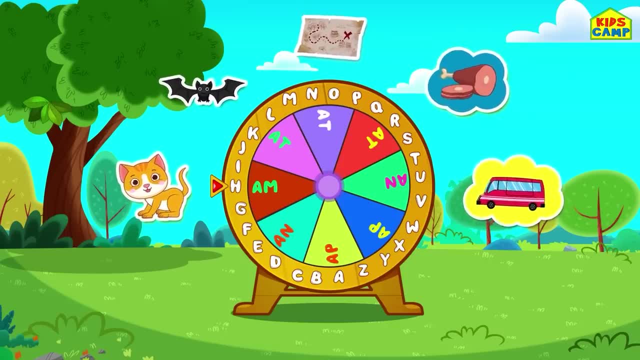 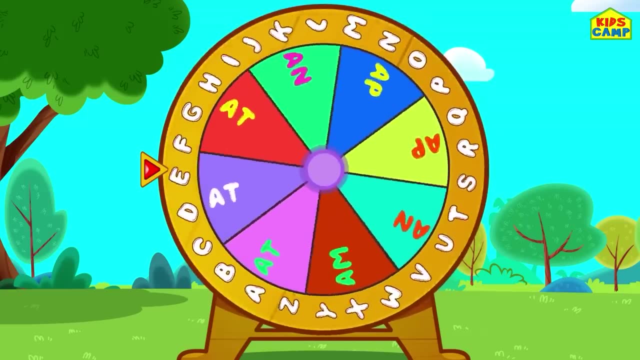 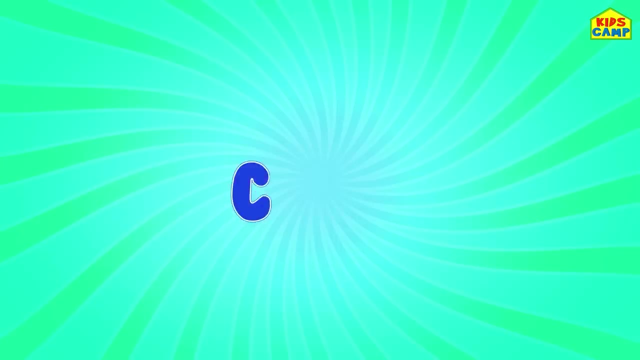 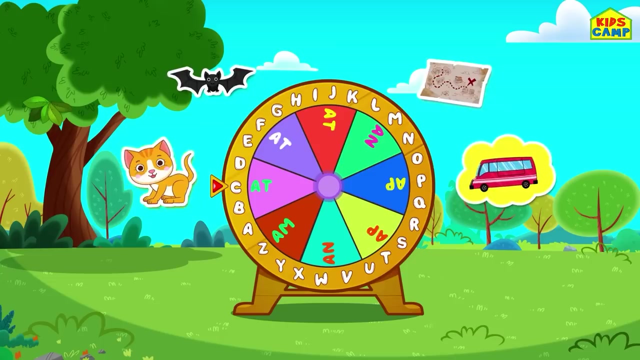 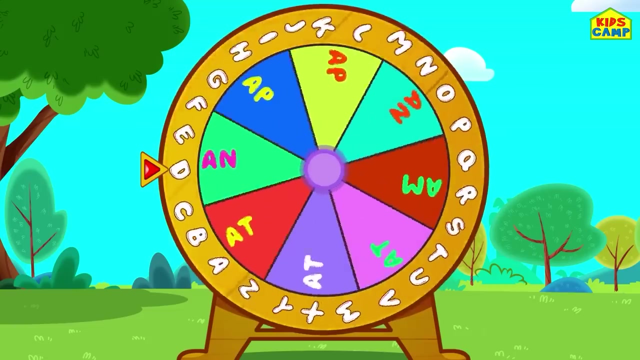 We found another one. Let's find some more friends. Let's spin the wheel C-A-T. That's a word. Cat Woohoo, What's next? Let's spin the wheel again. Word wheel: Keep spinning, Uh-huh, We found another word. 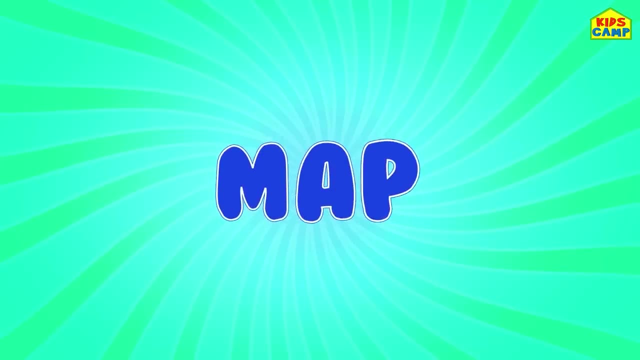 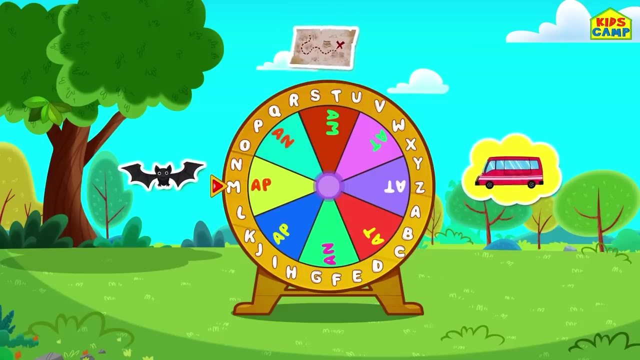 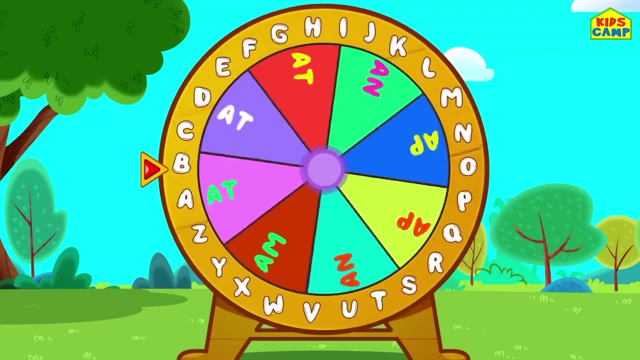 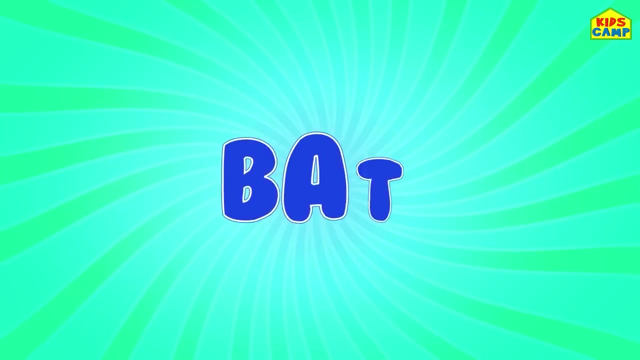 M-A-P Map. That's right. Map is a word. We found the word map. Good job, friends. Let's keep spinning the wheel. What's next? That's a bat. B-A-T Bat. That's right, We found another word. 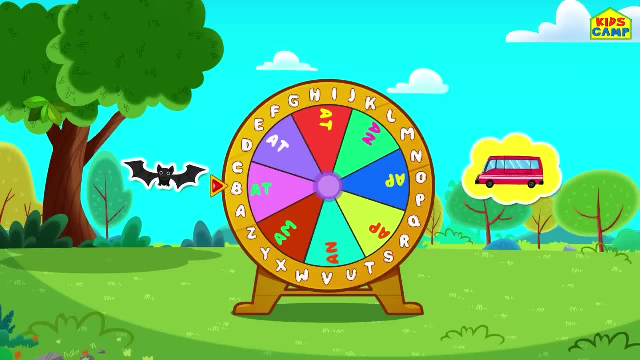 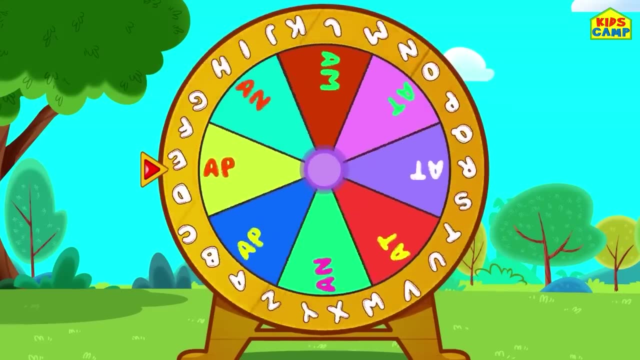 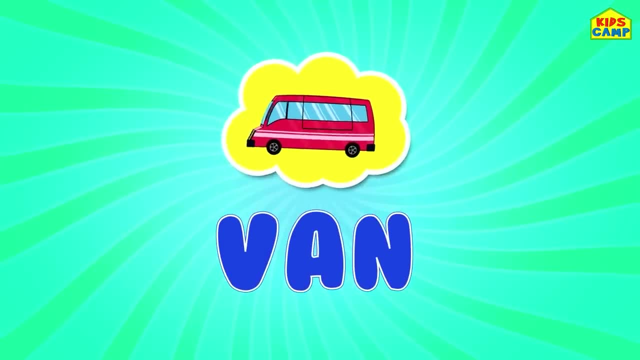 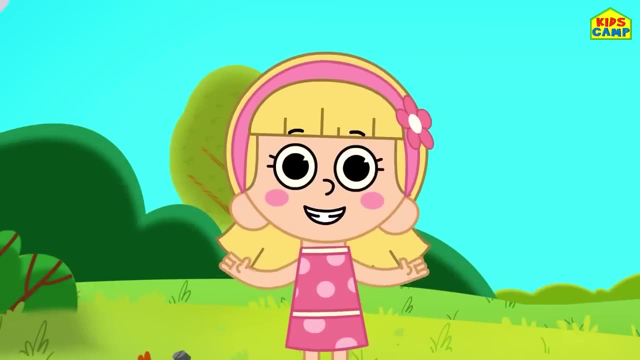 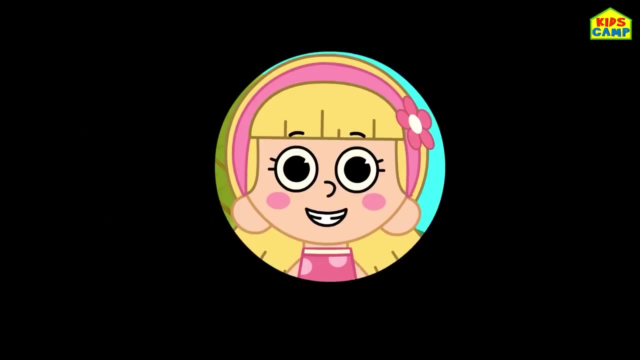 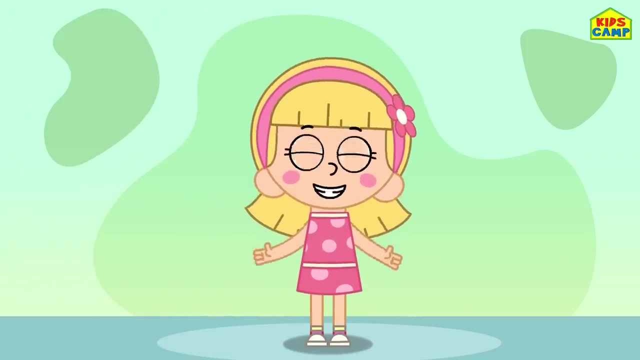 A N WAN. That's right. Woohoo, We got all the words. We had lots of fun today. Yay, We learned some new words today. Bye, Hi kids. I'm Ellie And I'm going to put up some pictures in Eva's bedroom. 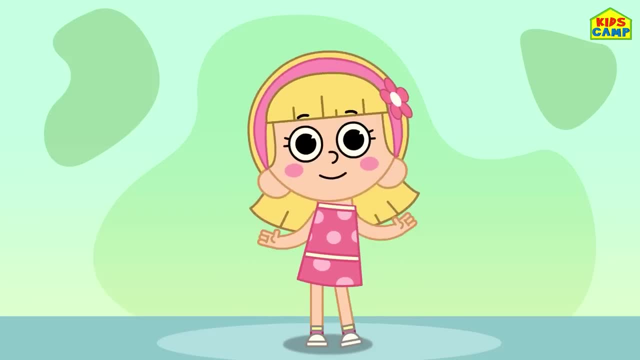 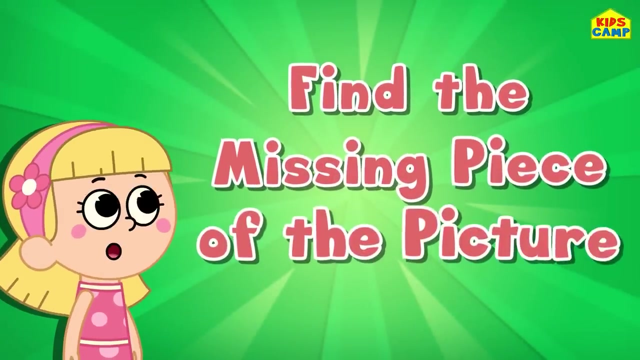 But there's just one tiny problem. There seems to be a missing piece in each picture. Can you help me find it? Woohoo, Let's get started. This is going to be a fun game. Let's find the missing piece. 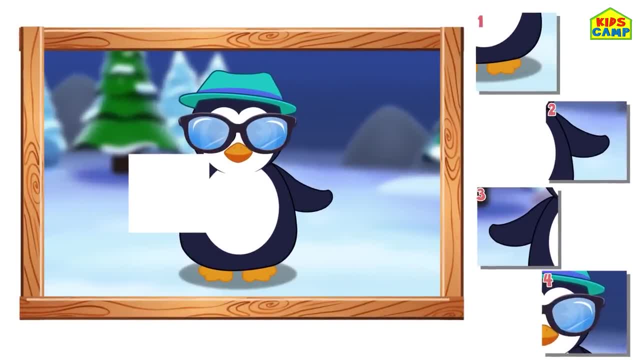 Hmm, Do you know which one is the right piece? Let's try. Let's try. Is number 2 the right piece? No, it isn't. Is number 1 the right piece? Uh-oh, It isn't. Is number 4 the right piece? 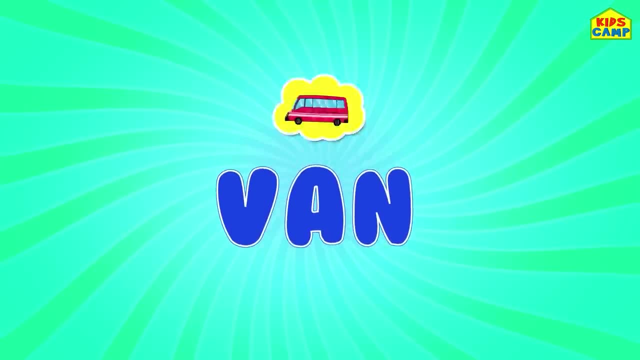 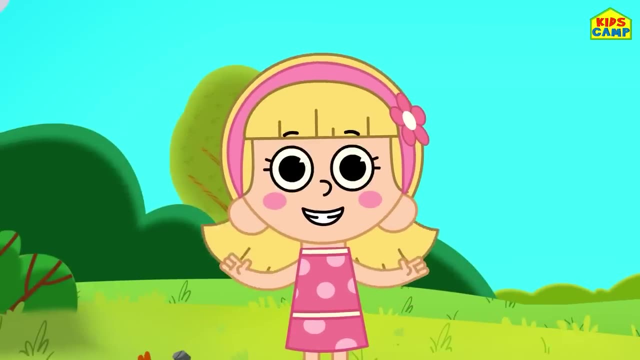 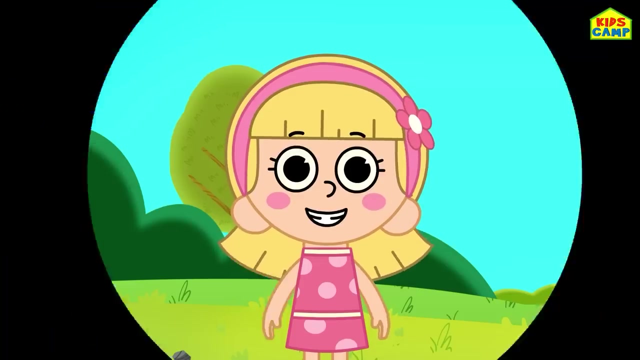 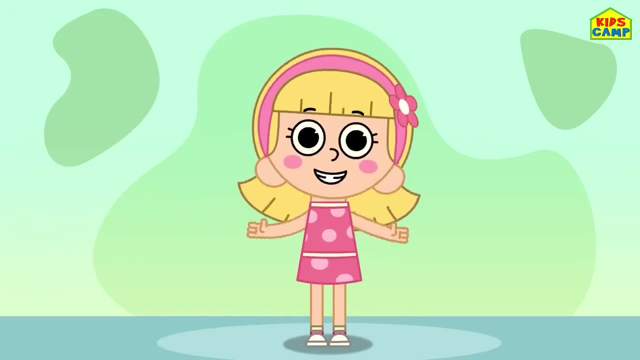 Van. That's right. Woohoo, We got all the words. We had lots of fun today. Yay, We learned some new words today. Bye, Bye, Bye. Hi kids, I am Ellie. I am going to put up some pictures in Eva's bedroom. 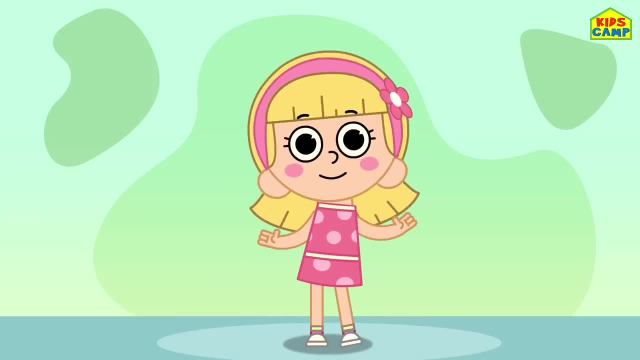 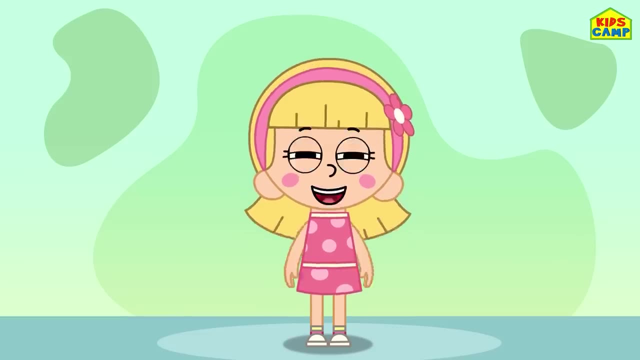 But there is one tiny problem. There seems to be a missing piece in each picture. Can you help me find it? Woohoo, Let's get started. This is going to be a fun game. Let's find the missing piece. We found the missing piece. 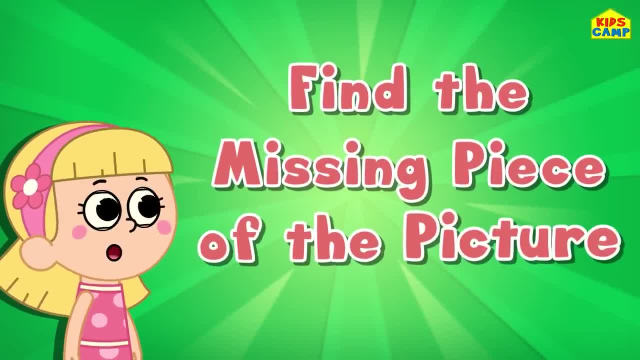 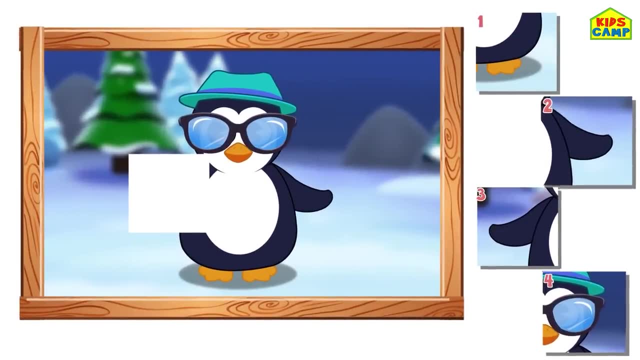 Two. We found the missing piece: Basic painting. do you know which one is the right piece? let's try. is number two the right piece? no, it isn't. is number one the right piece? oh, it isn't. is number four the right piece? no, let's try. number 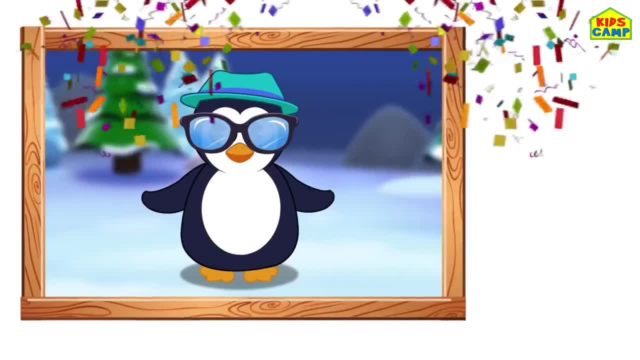 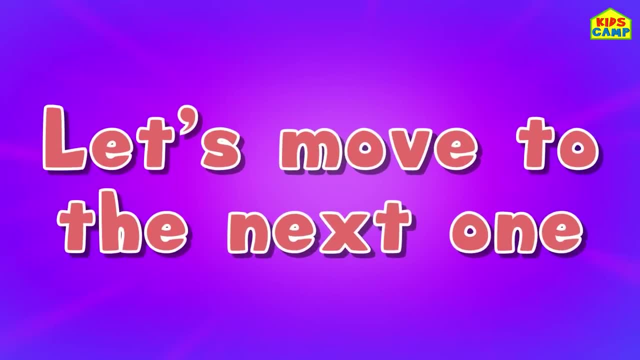 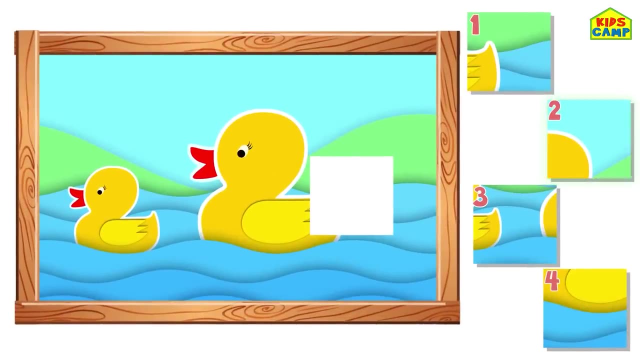 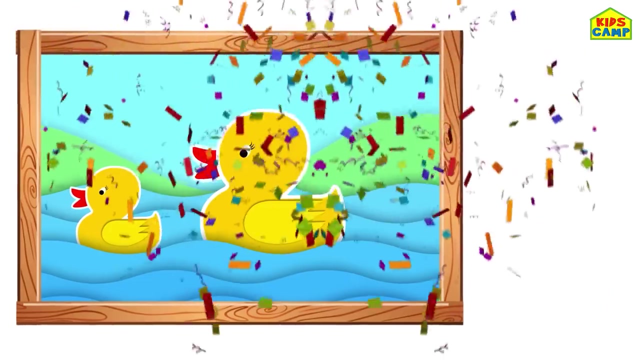 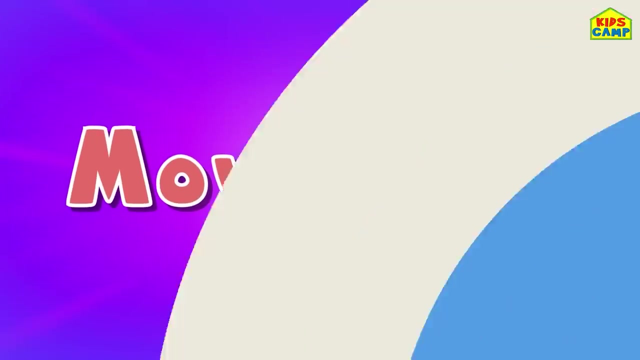 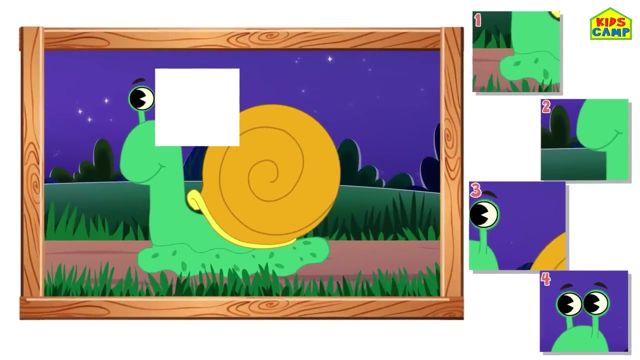 three. yes, we got the right one. good job, kids. let's move to the next one. what is missing from here? let's try number two. no, let's try number four. no, no, let's try number one. we got it. hmm, what's missing here? let's find out. let's try number two. no, that doesn't fit right. let's. 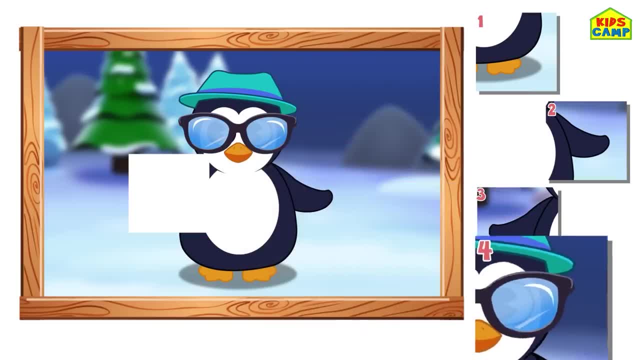 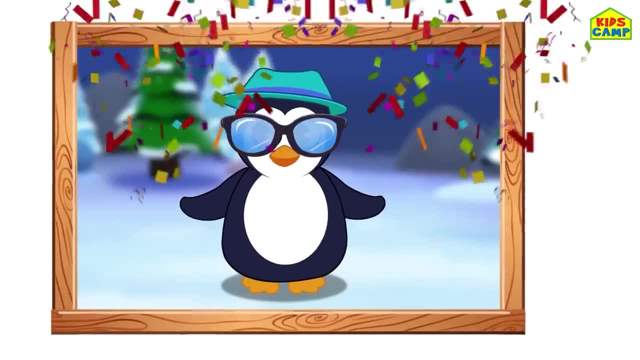 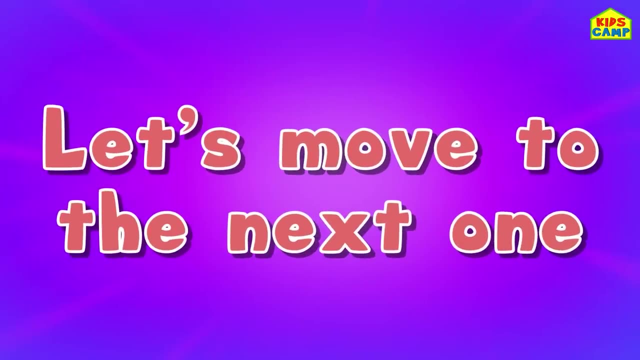 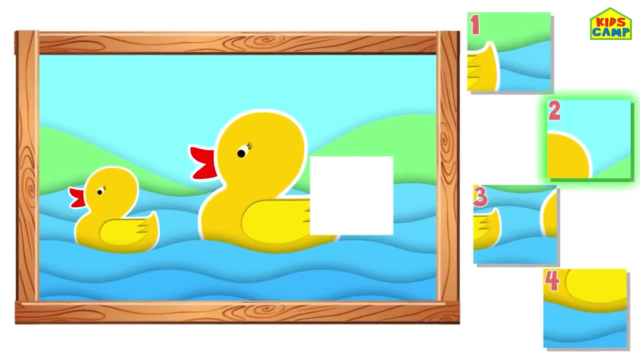 No, Hmm, Let's try number 3!. Yes, We got the right one. Woohoo, Good job, kids. Shhh, Let's move to the next one. What is missing from here? Let's try number 2!. 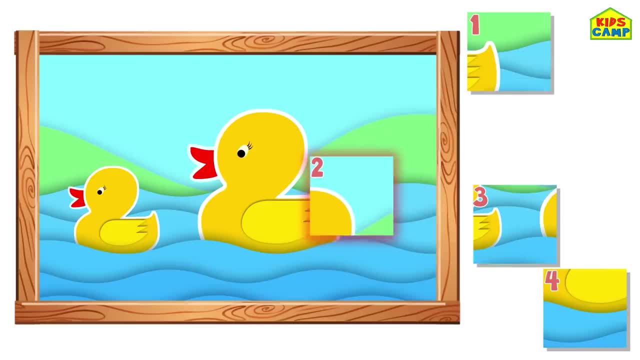 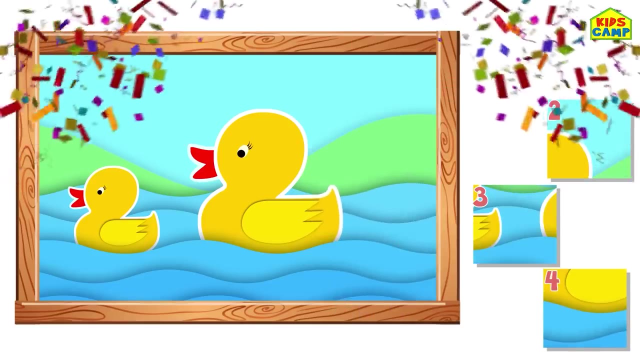 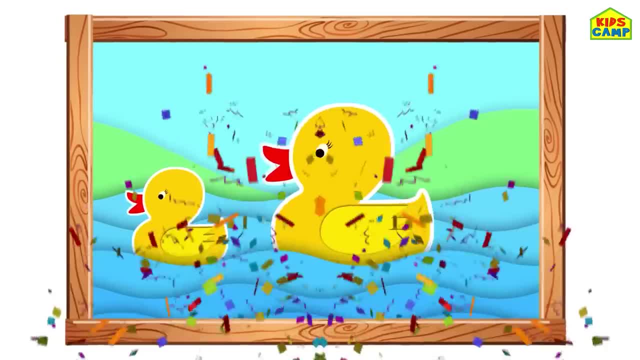 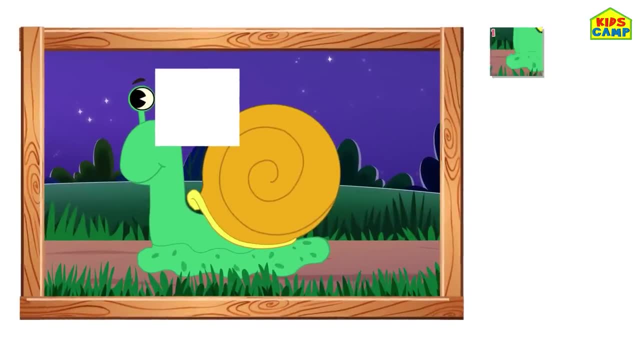 Yay, That fits right. We got it. Woohoo, We got it, Woohoo, Shhh Moving on, Shhh Moving on. Hmm, What's missing here? Hmm, What's missing here? Let's find out. 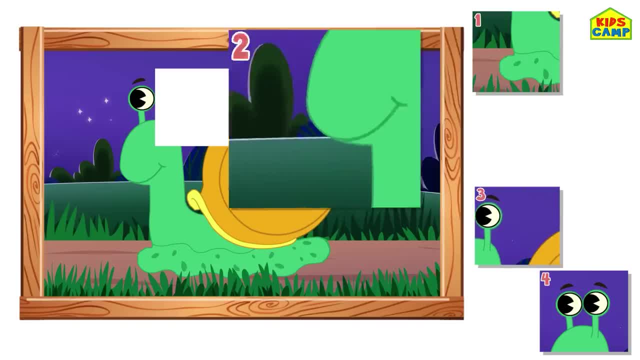 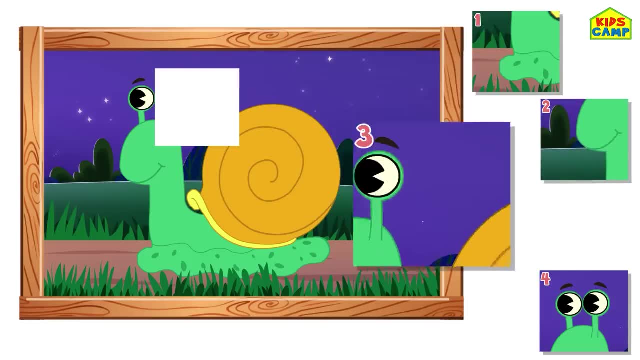 Let's try number 2!. Let's try number 2!. No, That doesn't fit right. No, That doesn't fit right. Let's try number 3!. Let's try number 3!. Wow, We did it. Wow, We did it. 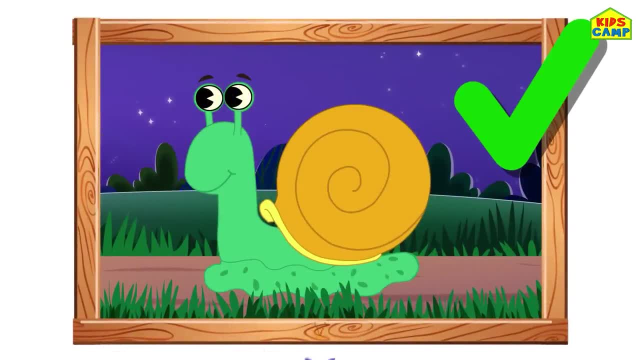 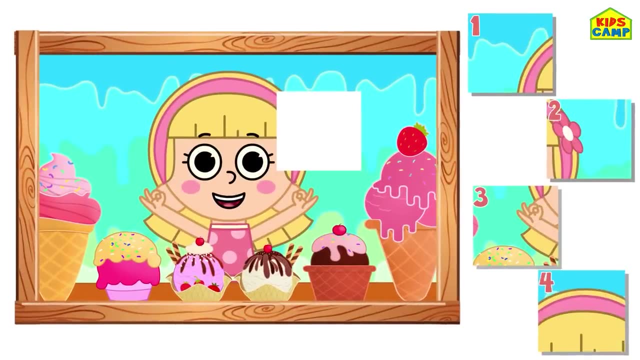 We got that one right. Ready to go up on the wall. Ready to go up on the wall, Moving on. Hmm, What's missing here? Hmm, What's missing here? Let's try number 1!. No, That doesn't seem right. 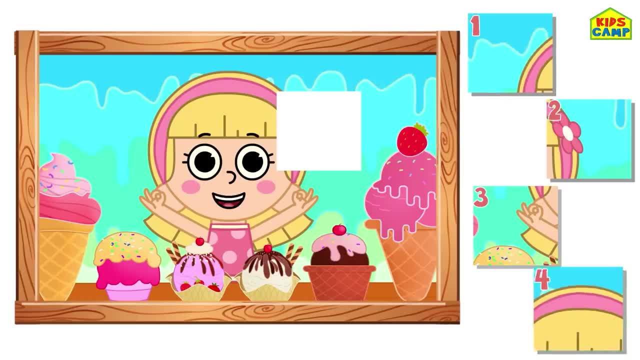 No, That doesn't seem right. Let's try number 4!. Let's try number 4!. No, No, Let's try number 3!. Let's try number 3!. No way, No way. Let's try number 2!. 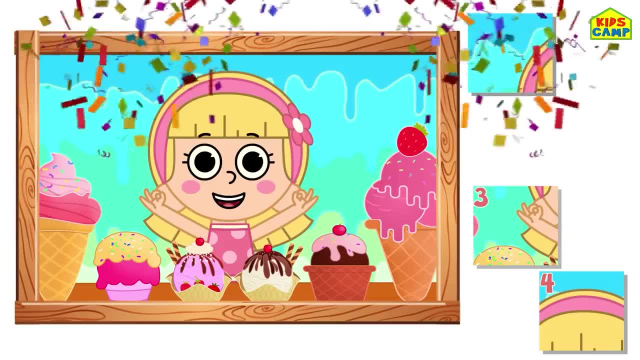 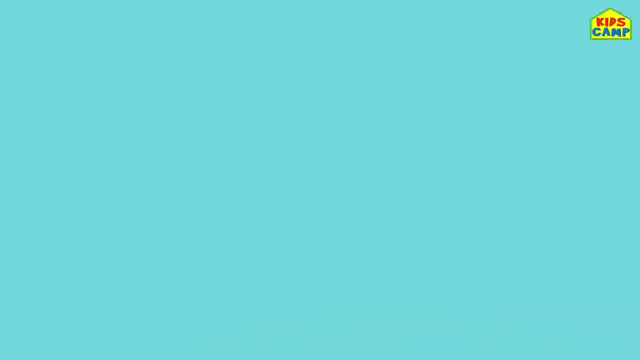 Let's try number 2!. Yes, This fits right. Woohoo, We did it again. Woohoo, We did it again. Good job kids. Yay, They already look so good up on the wall. They already look so good up on the wall. 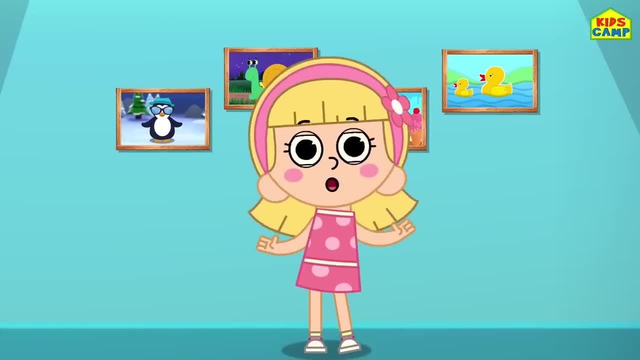 Eva's gonna love this. Eva's gonna love this. Thank you so much for helping me out. This was a fun game. Keep watching Kids Camp for more learning videos. Keep watching Kids Camp for more learning videos. Until then, bye-bye. 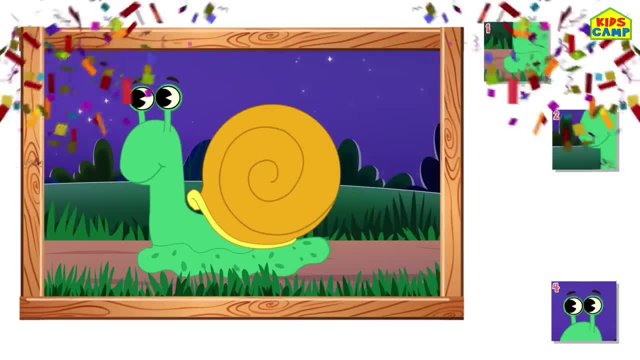 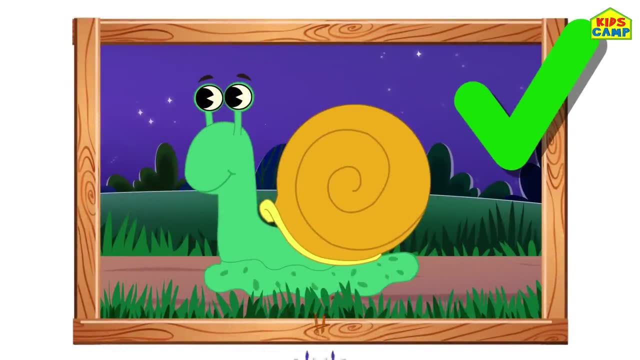 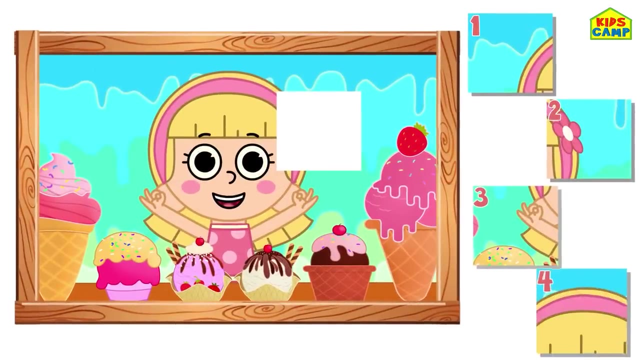 try number three. wow, we did it. we got that one right, ready to go up on the wall moving on. hmm, what's missing here? let's try number one. no, that doesn't seem right. let's try number four: no, no. let's try number three: no way. 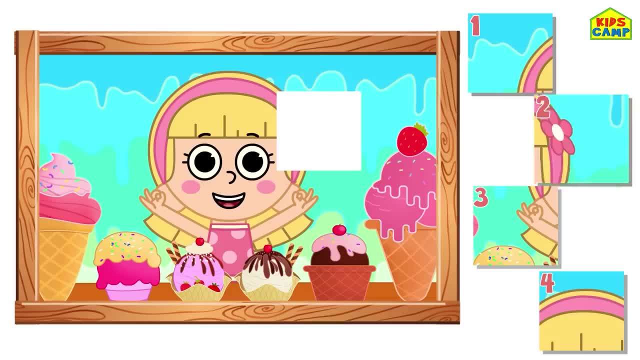 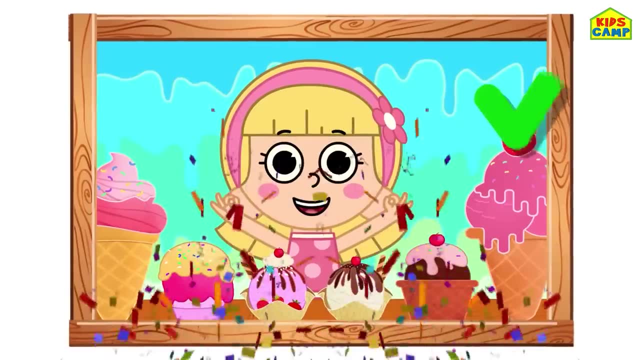 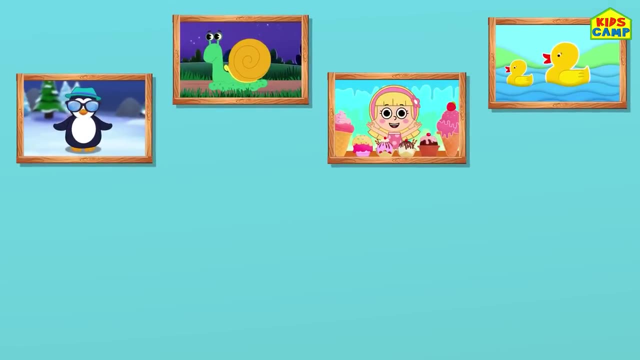 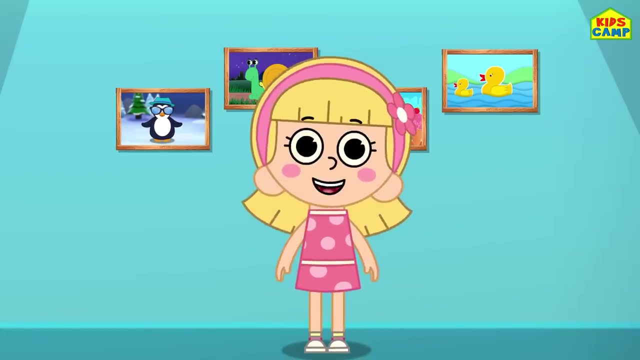 let's try number two. yes, this fits right. woohoo, we did it again. good job, kids. yay, they already look so good up on the wall. eva's gonna love this. thank you so much for helping me out. this was a fun game. keep watching kids camp for more learning videos. 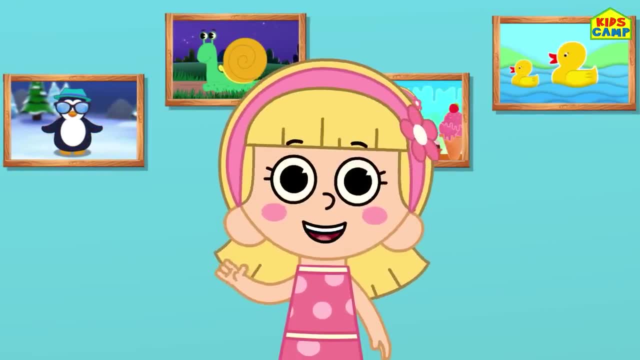 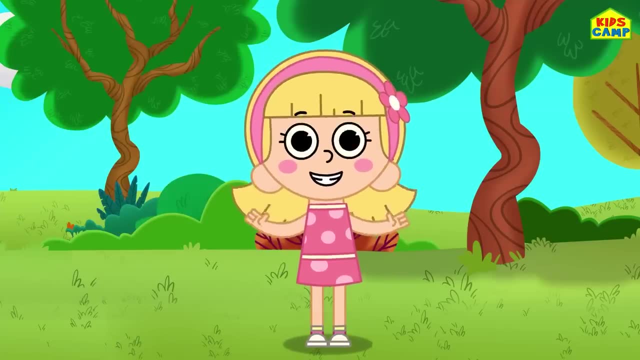 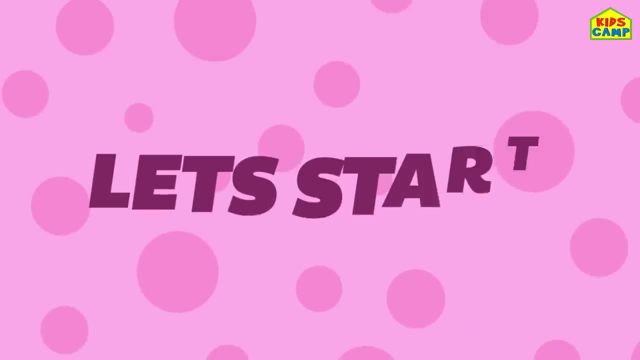 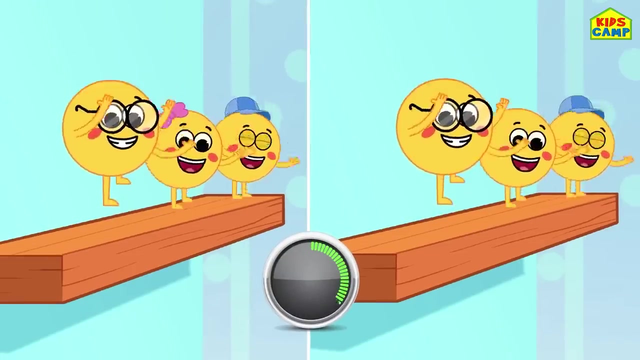 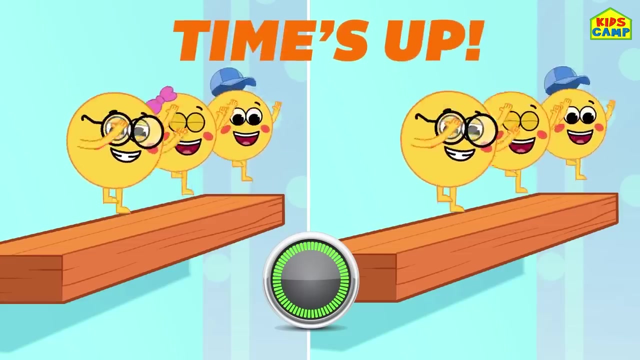 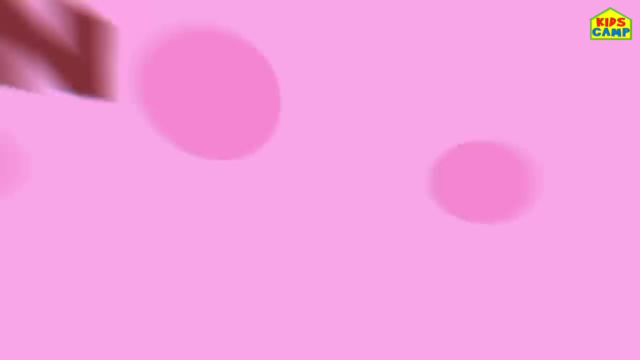 until then, bye, bye, hi, i'm ellie and we are going to play. spot the difference. ready, let's go. woohoo, let's start. can you spot the difference? time's up, that's right. good job, kids. let's go to the next one. can you spot the? 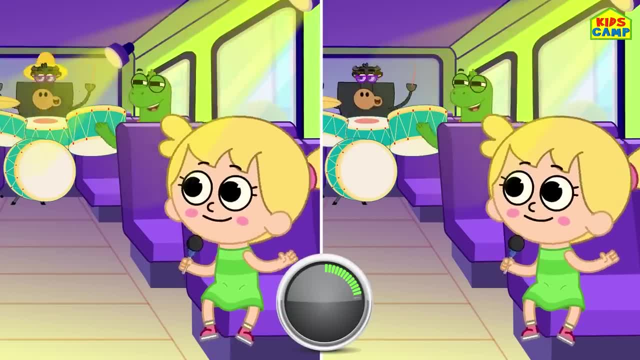 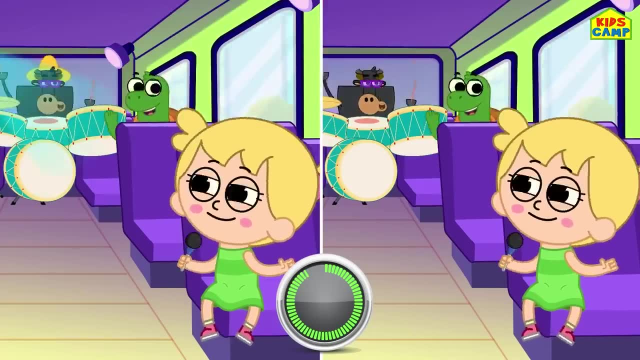 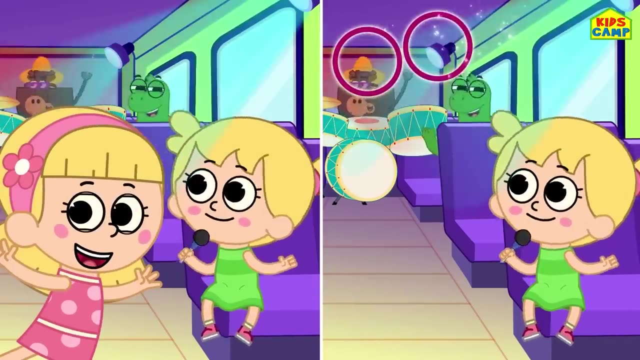 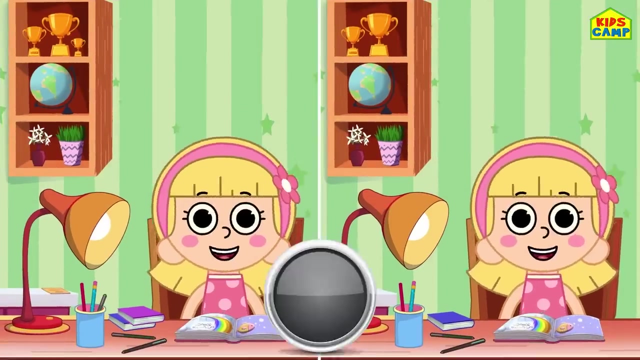 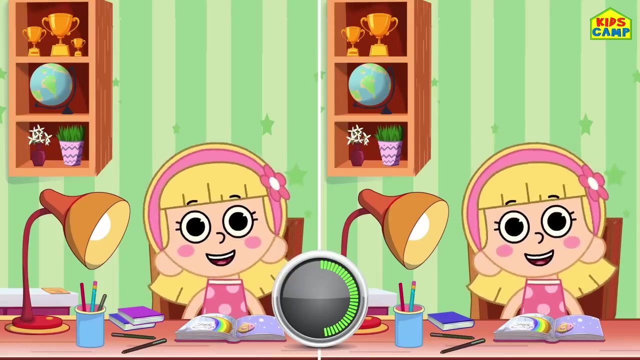 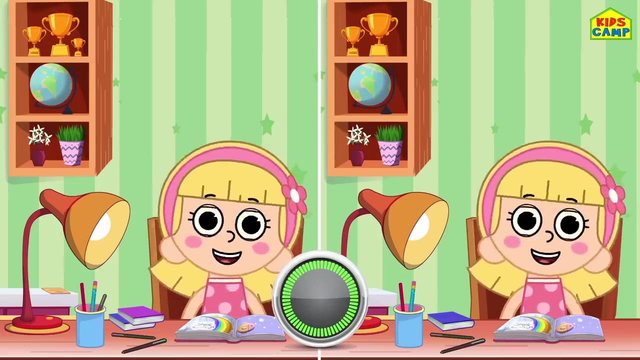 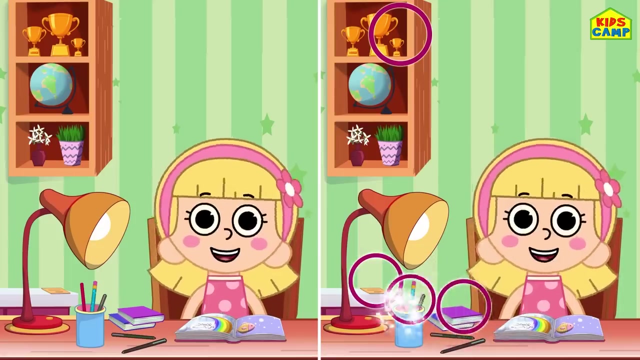 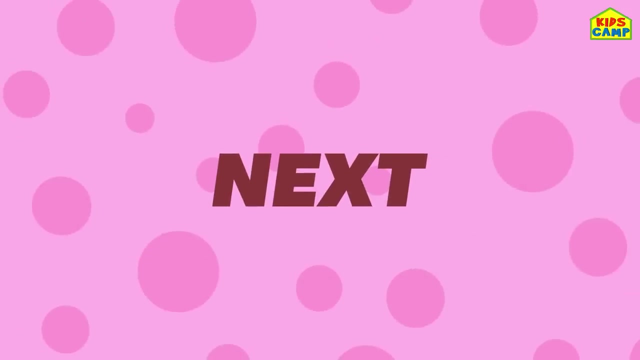 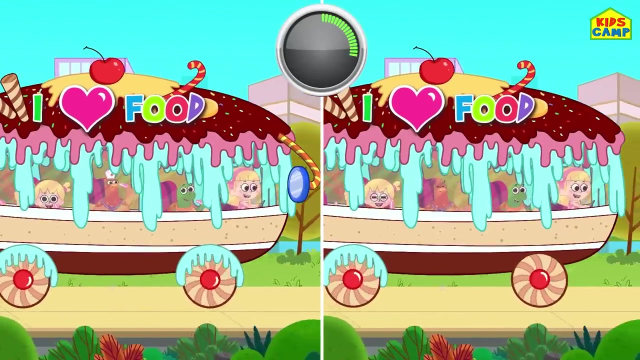 keep looking time's up. Time's Up, that's right, Let's do the next one. Can you spot the differences? Keep looking Time's up, That's right, You got it. You got it. Next one: Can you spot the differences? 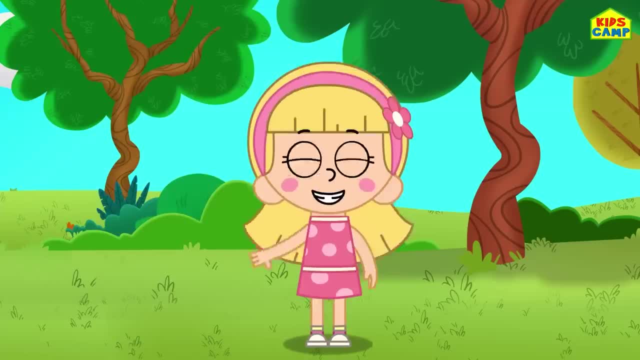 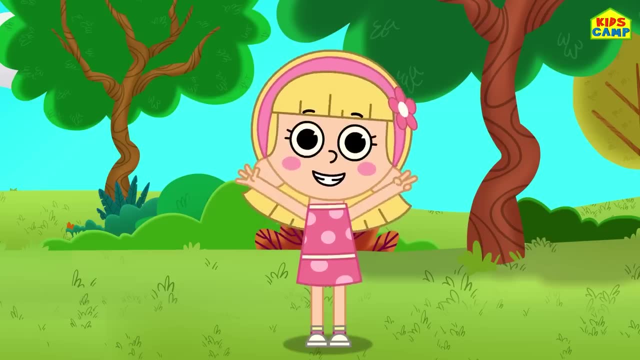 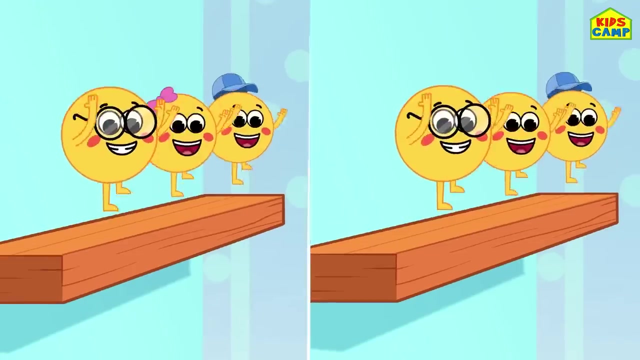 Until then, bye-bye. Until then, bye-bye. Hi, I'm Ellie And we are going to play. Spot the Difference Ready, Let's go? Woohoo, Let's start. Can you spot the difference? Can you spot the difference? 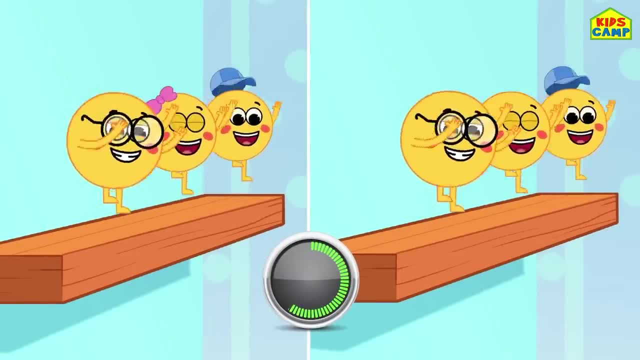 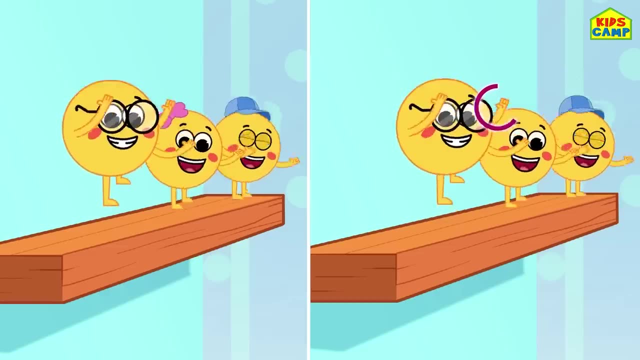 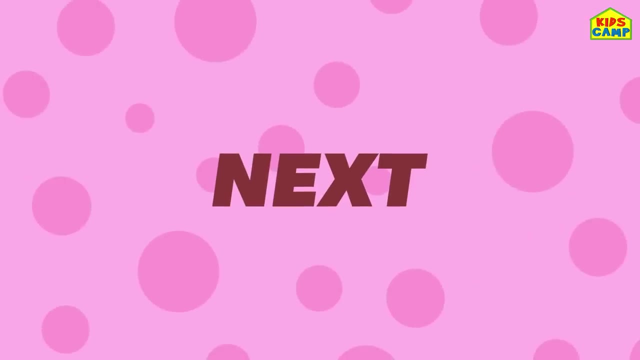 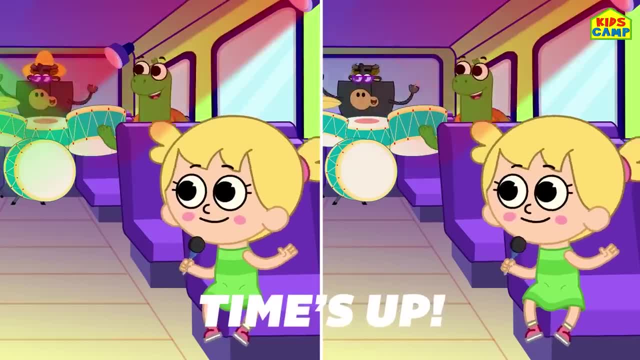 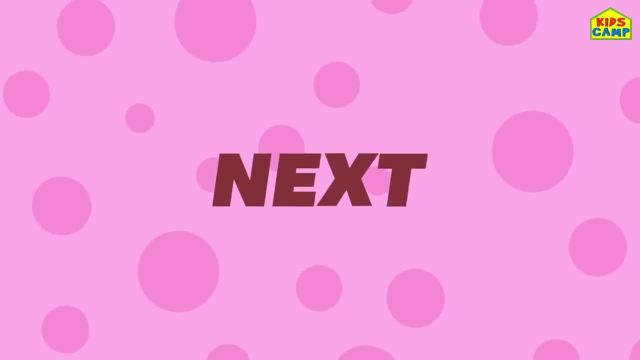 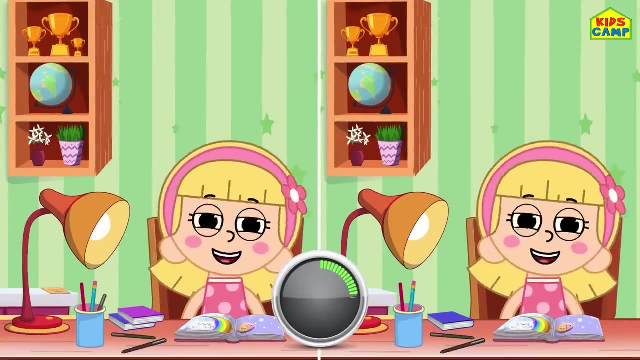 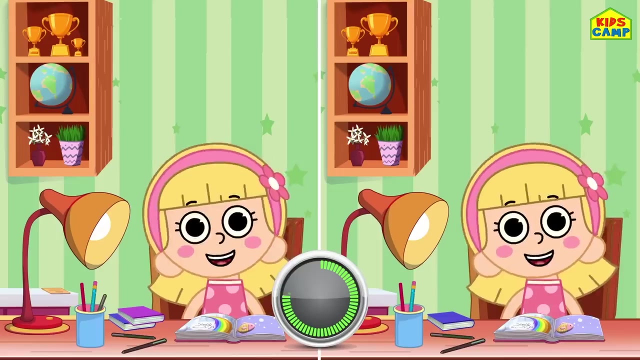 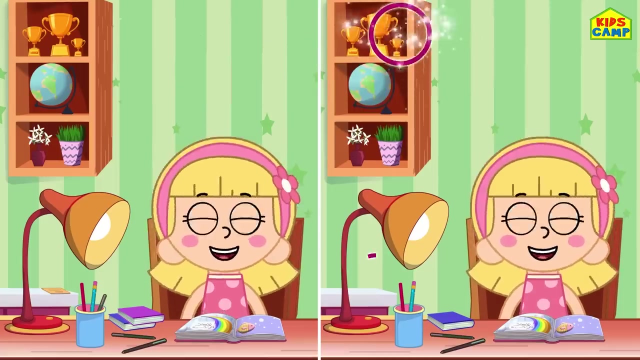 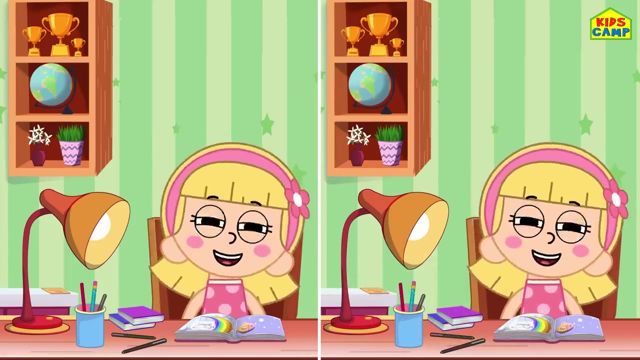 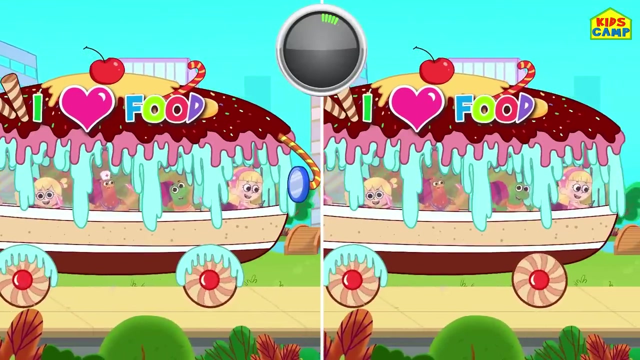 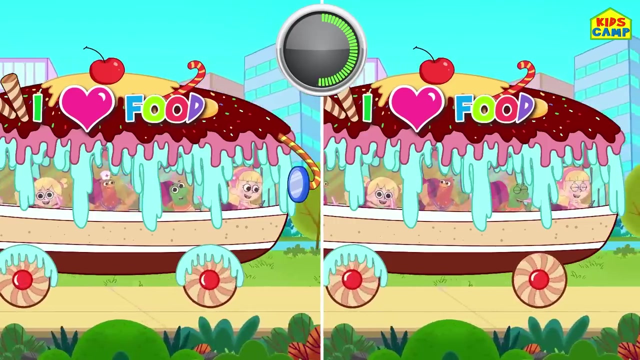 Time's up. That's right, Let's do the next one. Can you spot the differences? Keep looking Time's up. That's right, You got it. Next one: Can you spot the differences? Keep trying. Can you spot the differences? 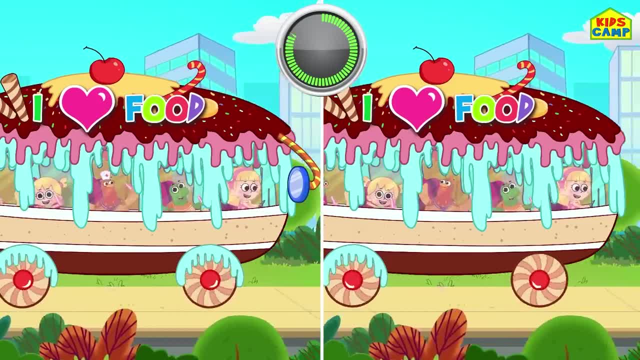 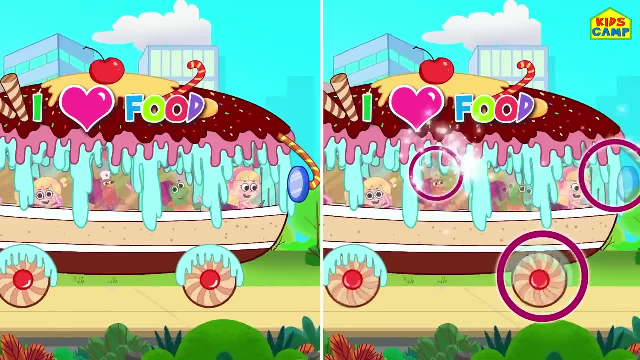 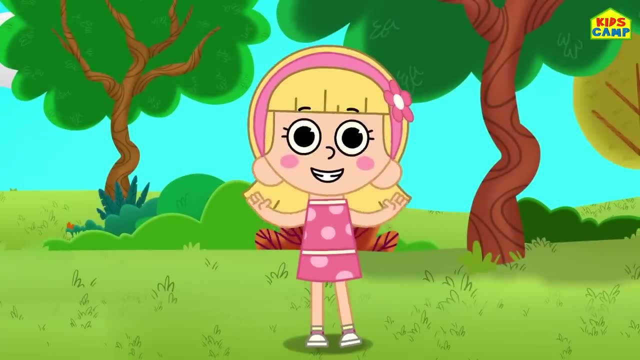 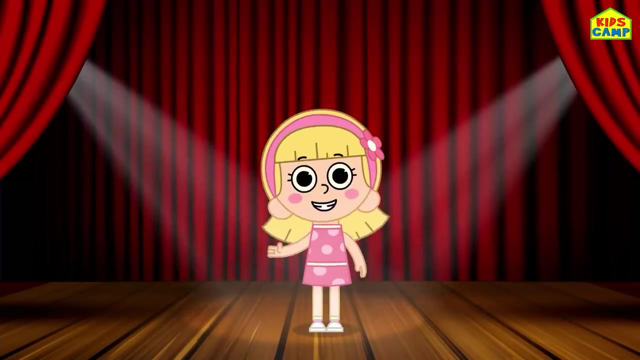 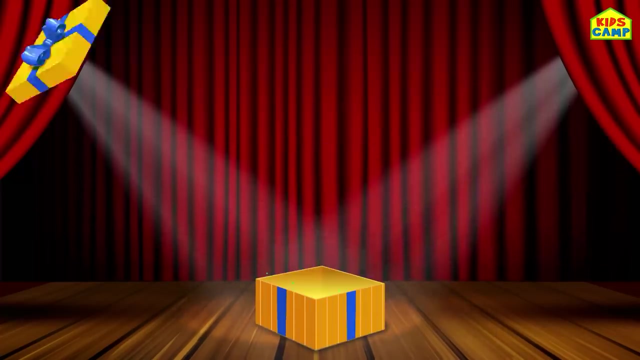 Can you spot the differences? Can you spot the differences? Time's up. You got it. Good job kids. Good job kids. This was so much fun. This was so much fun. Keep watching Kids Camp. Bye, Here we go. 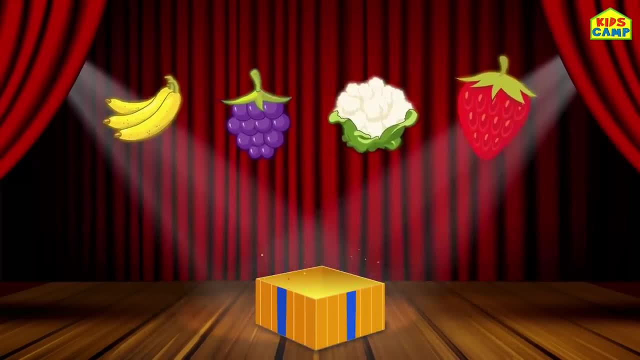 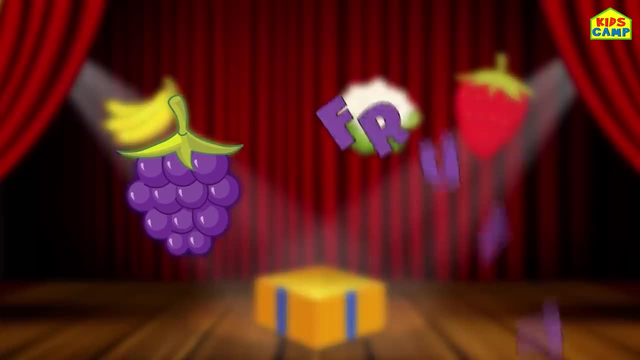 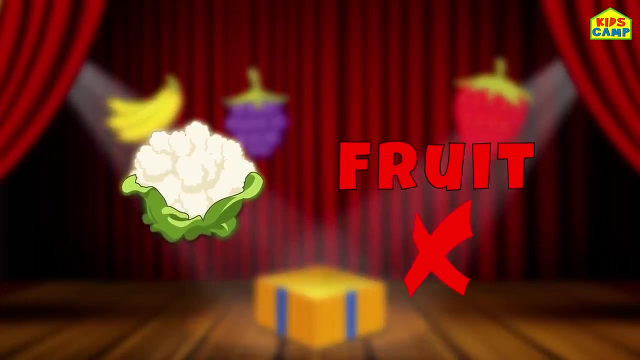 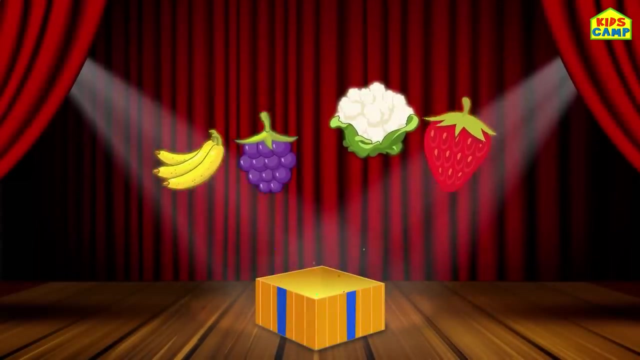 Let's go Spot the odd one out. Spot the odd one out. Is this a fruit? Yes. Is this a fruit? Yes. Is this a fruit: No. Is this a fruit. Is this a fruit? Yes, Yes. 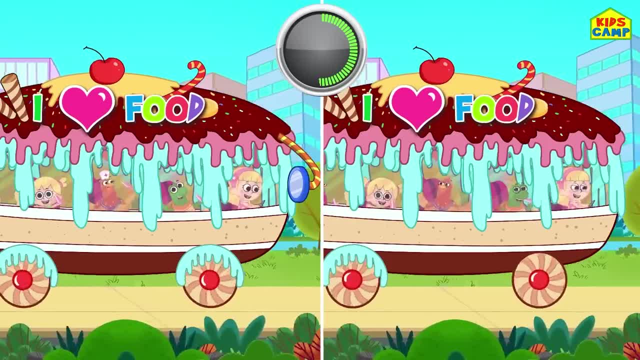 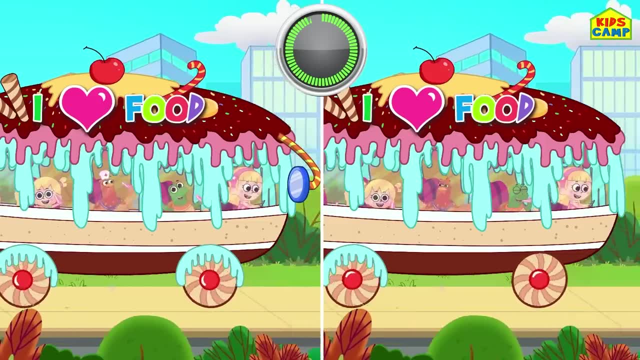 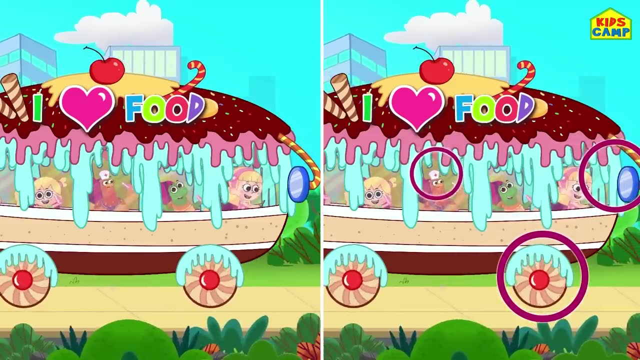 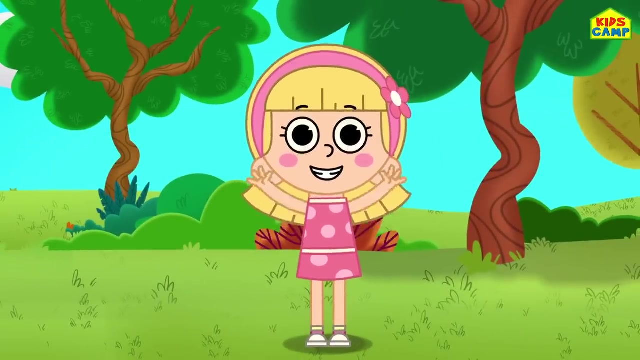 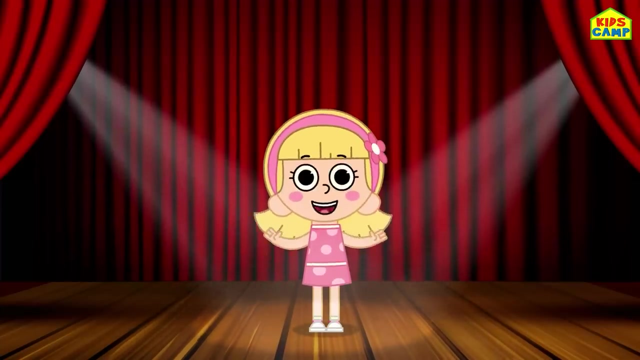 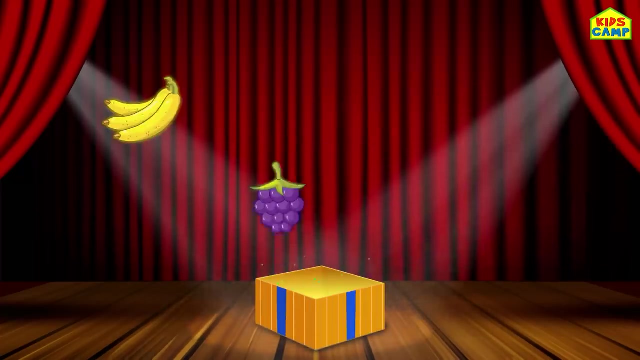 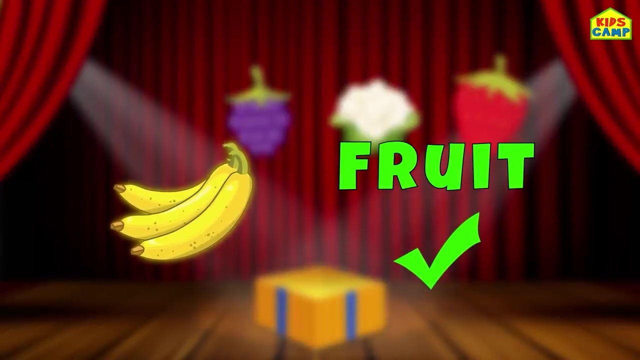 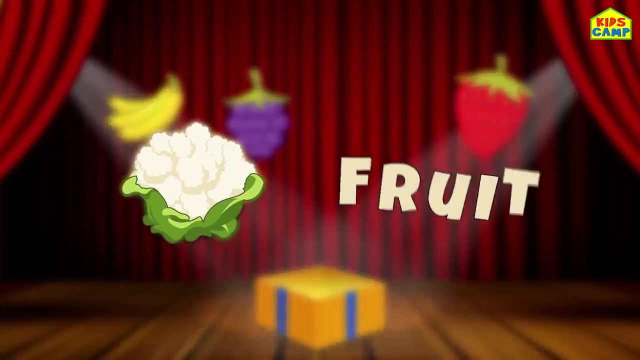 Keep trying Time's up. You got it. Good job, kids. This was so much fun. Keep watching Kids Camp Bye-bye. Yes, Is this a fruit? Yes, Is this a fruit? No, Is this a fruit? 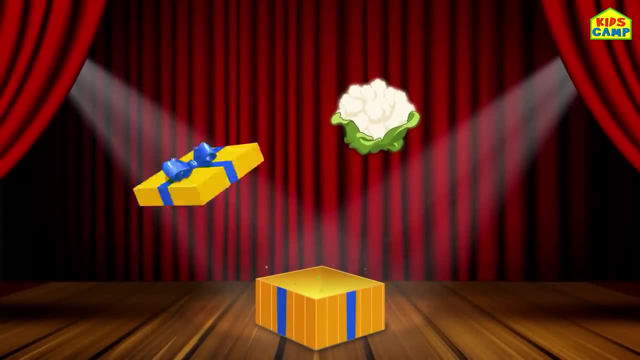 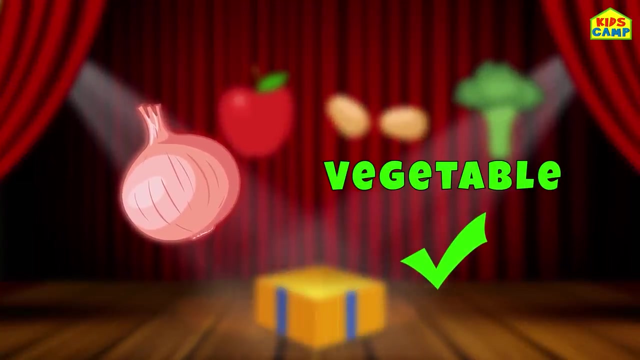 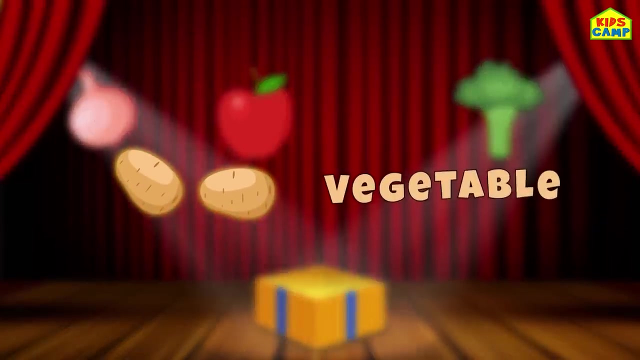 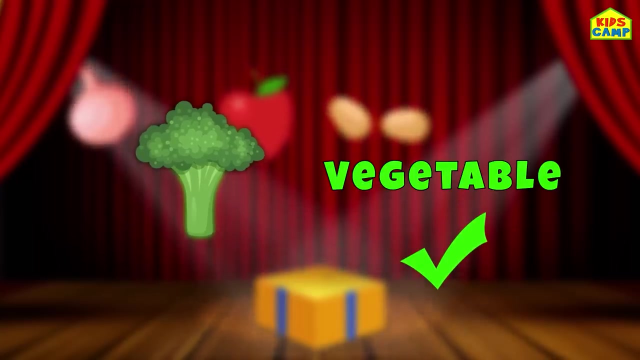 Yes, Here we go. This is the odd one out- Yay, Is this a vegetable? Yes, Is this a vegetable? No, Is this a vegetable? Yes, Is this a vegetable? Yes, Yay, We spotted the odd one out. 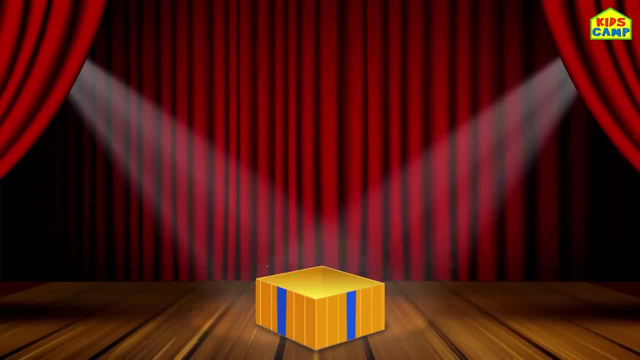 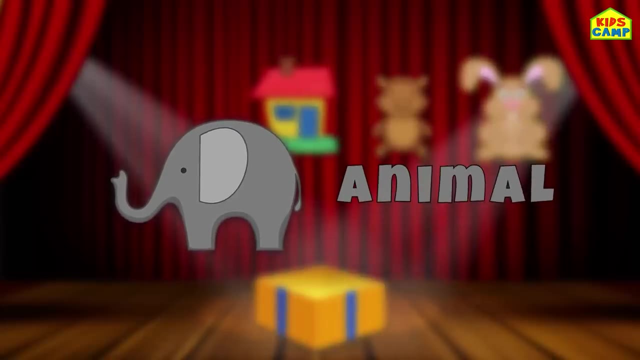 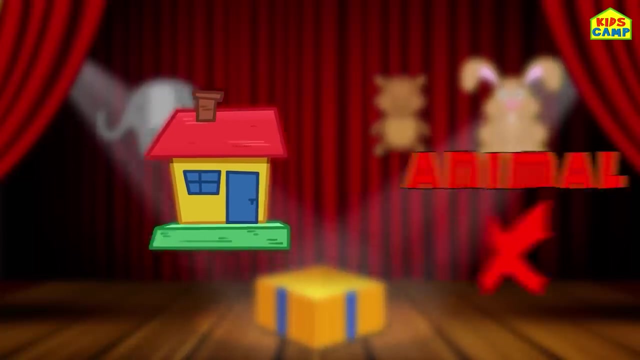 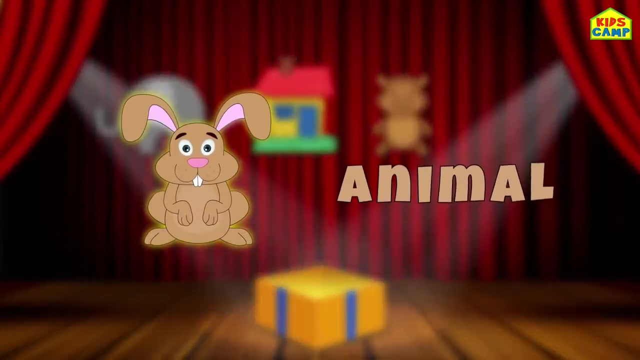 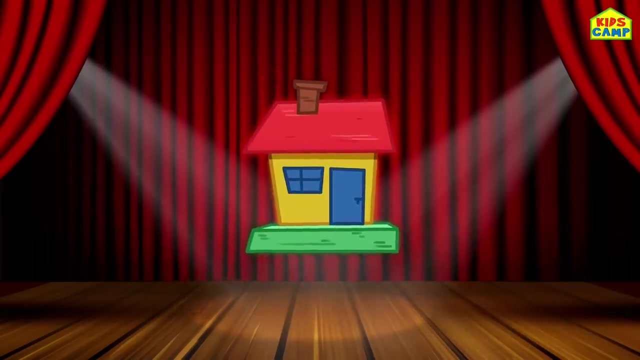 What next? Ooh, Is this an animal? Yes, it is. Is this an animal? No, Is this an animal? Yes, Yes. Is this an animal? Yes, it is. We spotted the odd one out there as well. Good job, kids. 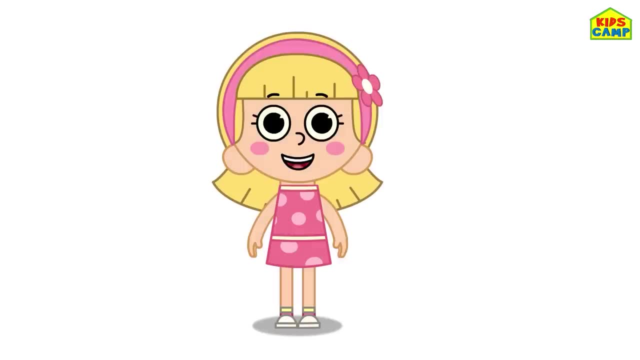 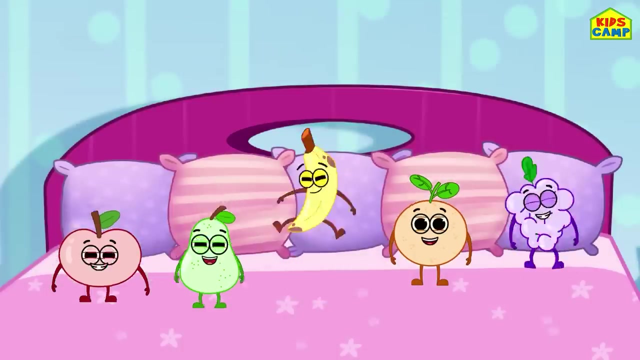 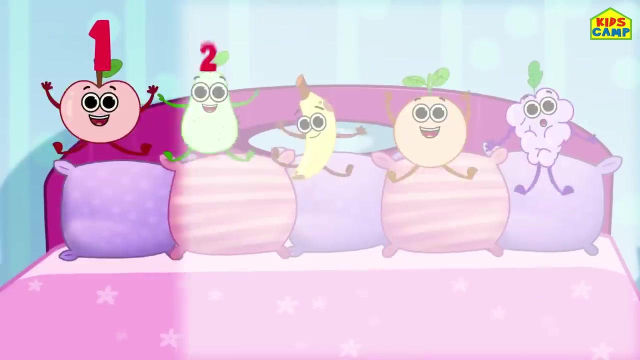 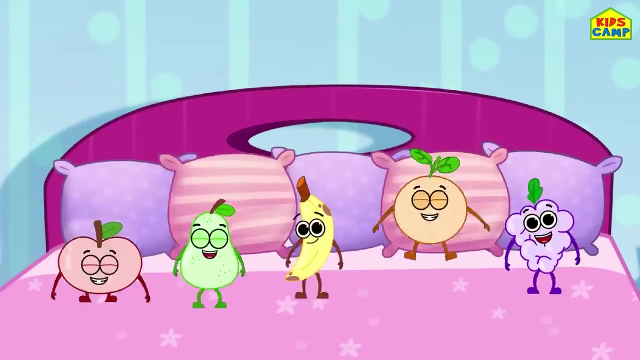 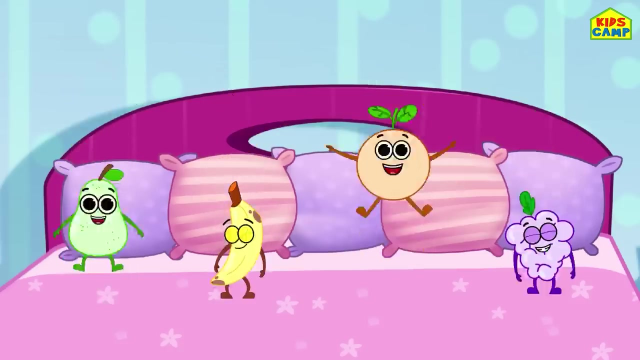 Hi, I'm Ellie. well, hello boys and girls. today we're going to learn how to do simple math subtraction. that's right, we have five fruits. look at them jumping on the bed so cute. one, two, three, four, five. wow, five fruits. oops, one of them fell down. oh, how many fruits do we have on the bed now? 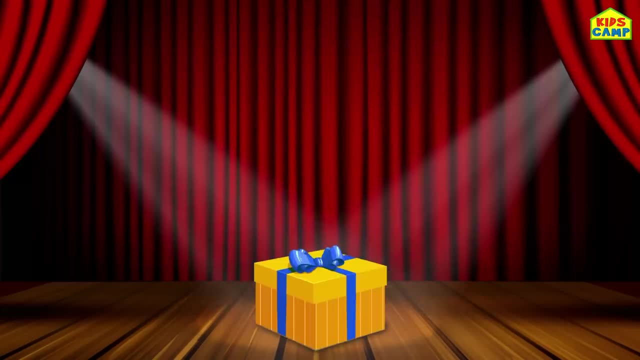 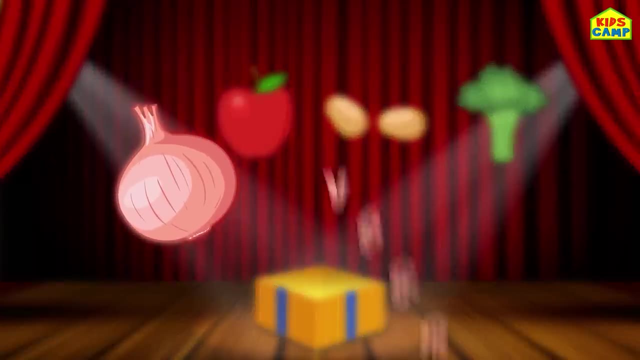 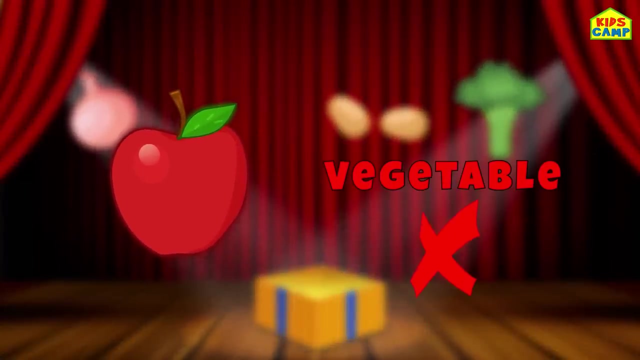 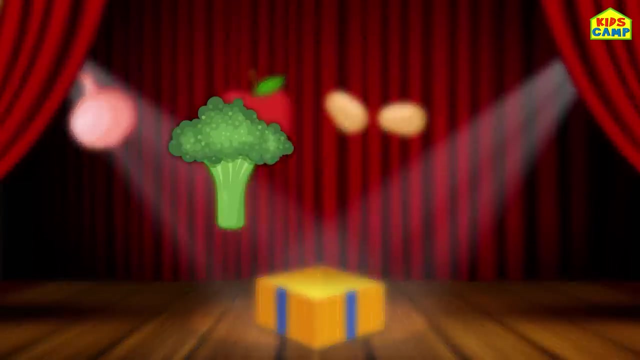 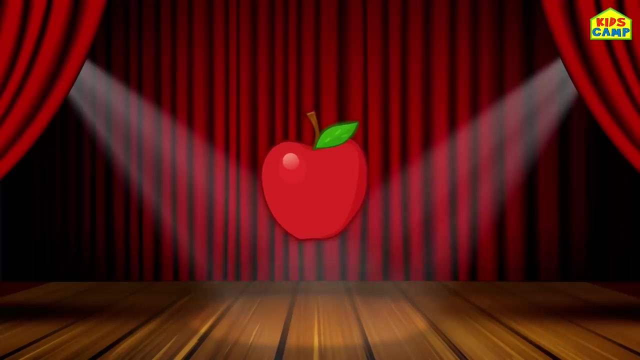 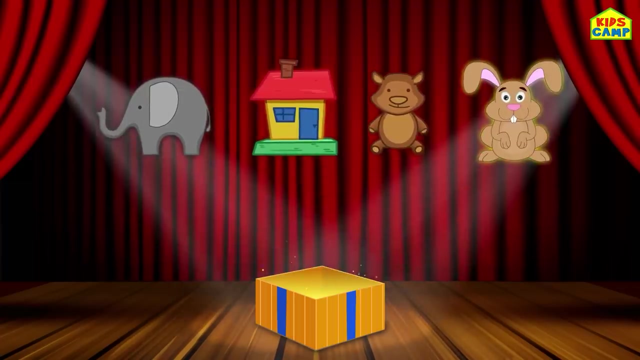 Here we go. Hmm, is this a vegetable? Yes. Is this a vegetable? No, Is this a vegetable- Yes. Is this a vegetable? Yes. Yay, We spotted the odd one out. What next? Ooh, Is this an animal? 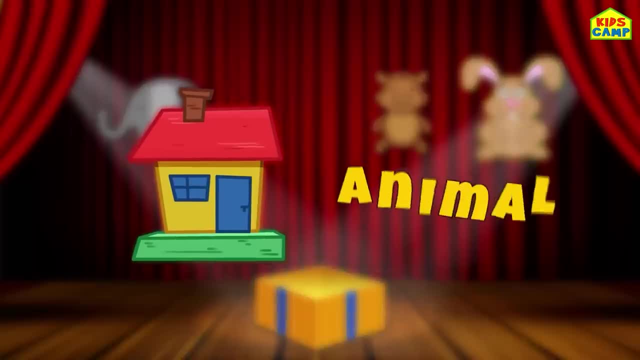 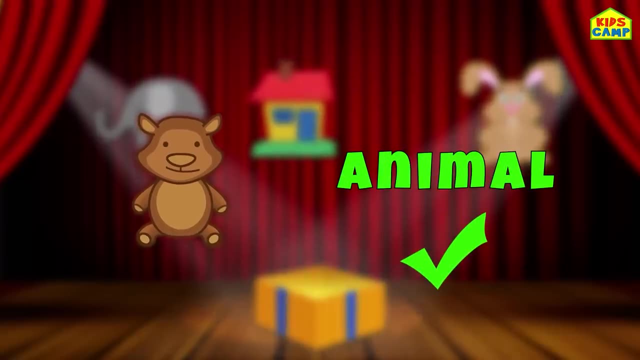 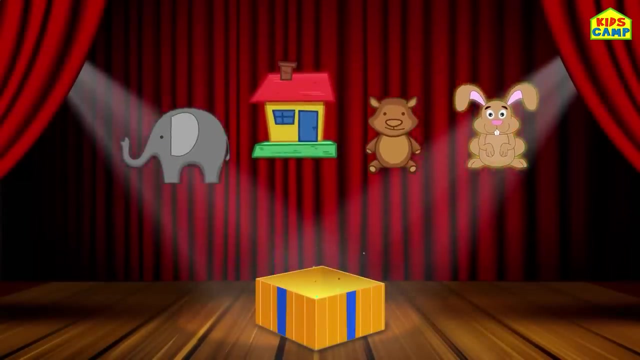 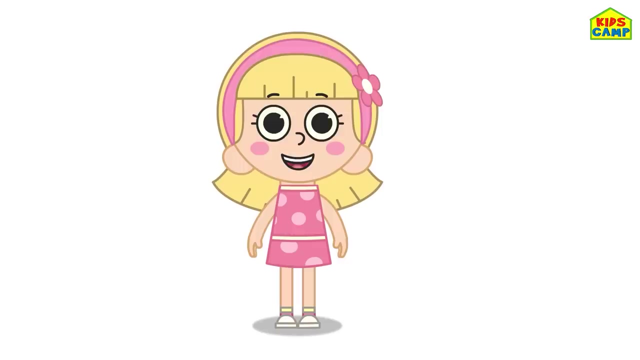 Yes, it is. Is this an animal? No, Is this an animal? Yes, yes, Is this an animal? Yes, it is. We spotted the odd one out here as well. Good job, kids. Hi, I am Elly. Well, hello boys and girls. 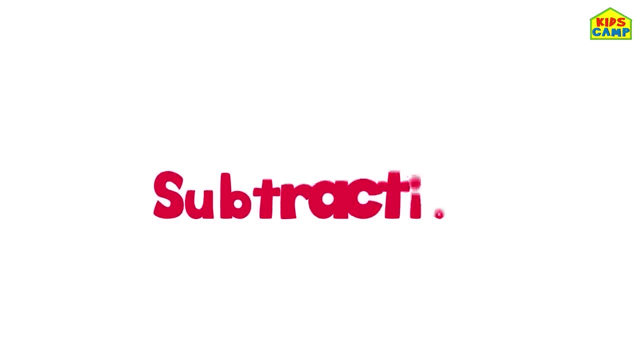 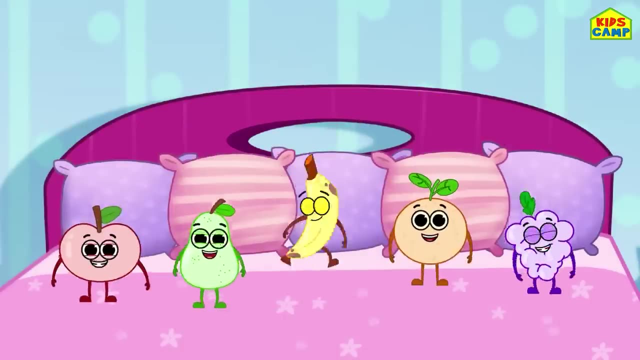 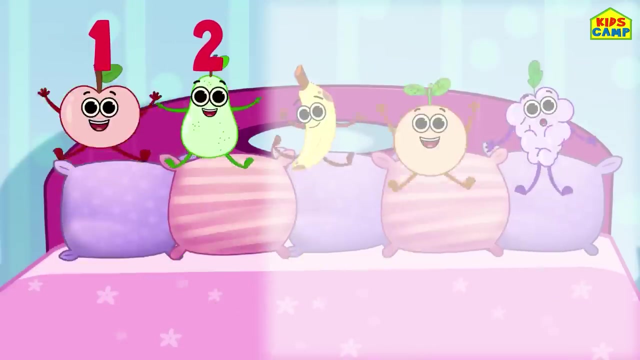 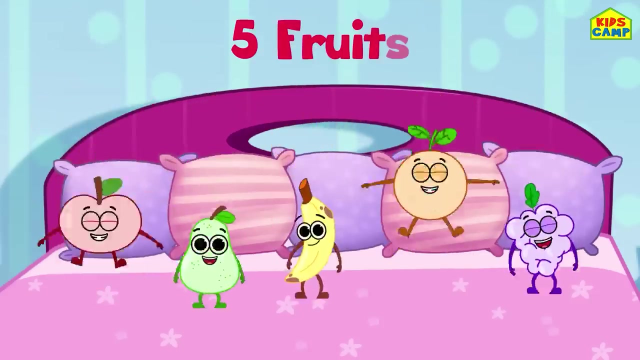 Today we are going to learn how to do simple math Subtraction. That's right, We have 5 fruits. Look at them jumping on the bed, So cute. 1, 2, 3, 4, Five, Wow, Five fruits. Oops, One of them fell down. 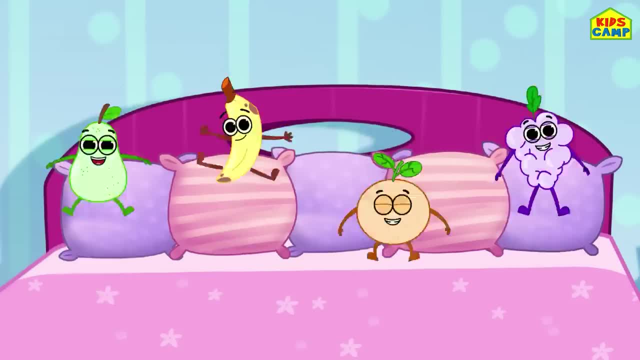 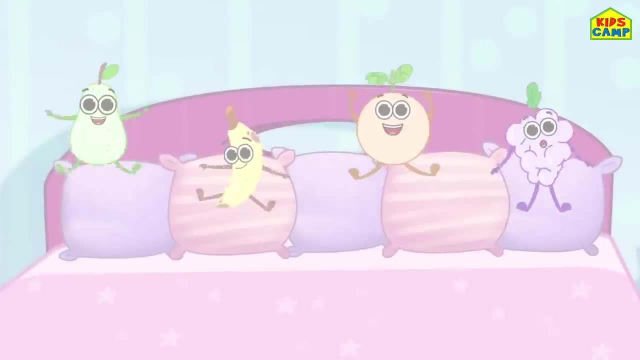 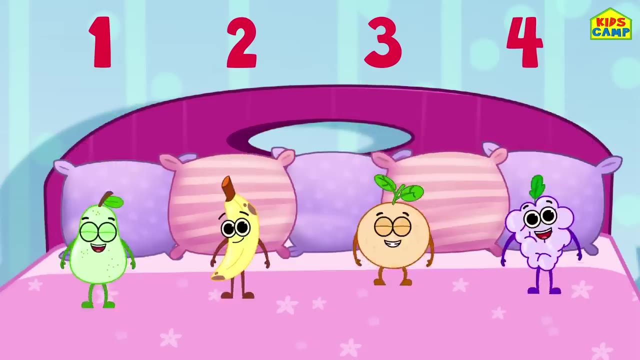 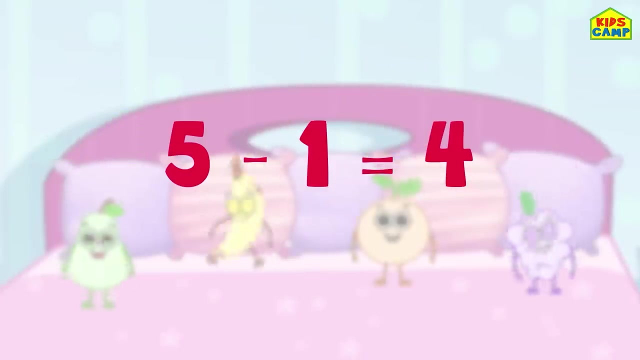 Ooh, How many fruits do we have on the bed now? Five minus one is We have one, two, three, four. We have four fruits jumping on the bed. That's right. Five minus one is four. We have four fruits jumping on the bed. 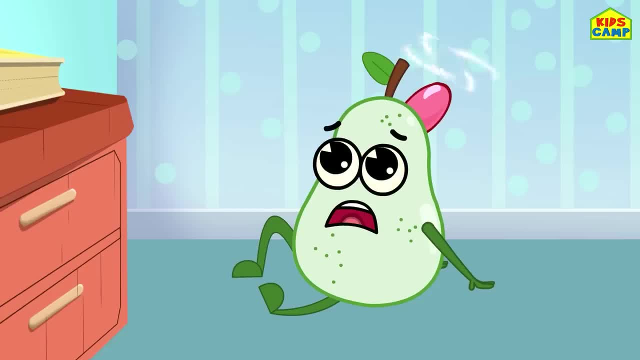 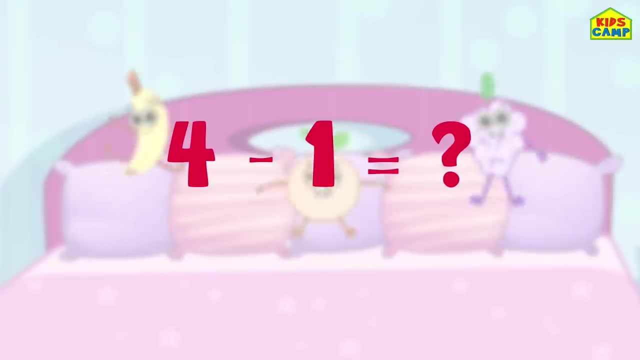 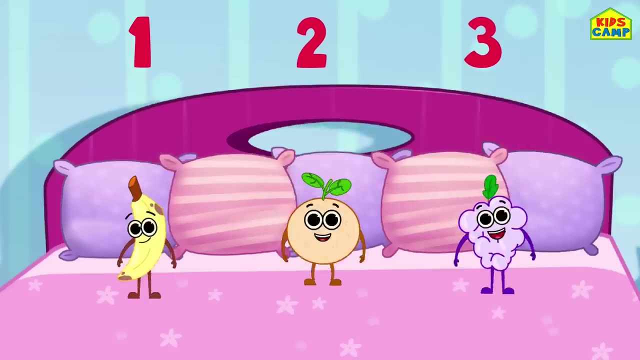 Oops, One fell off. Oh, How many fruits do we have jumping on the bed now? Four minus one is. Is it two? Is it one? Is it three? Let's count One, two, three. We have three fruits jumping on the bed. 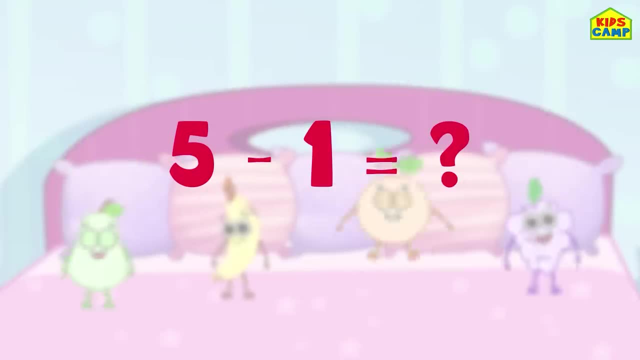 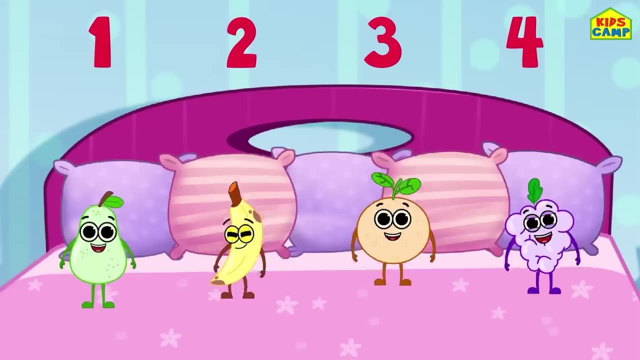 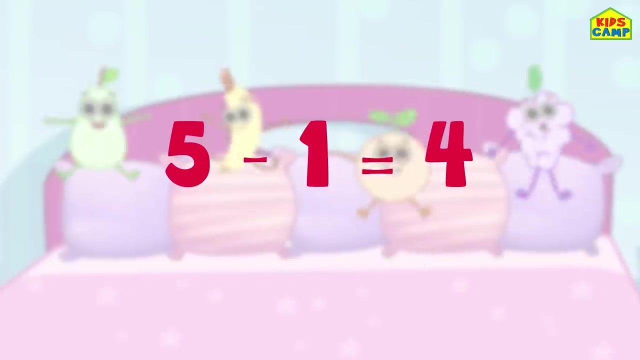 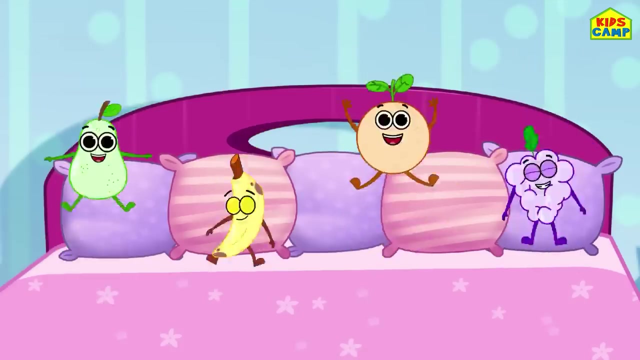 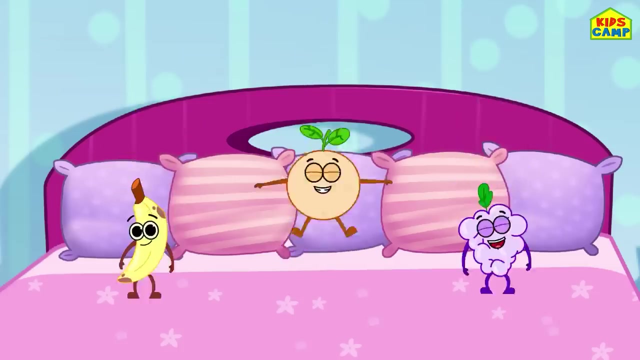 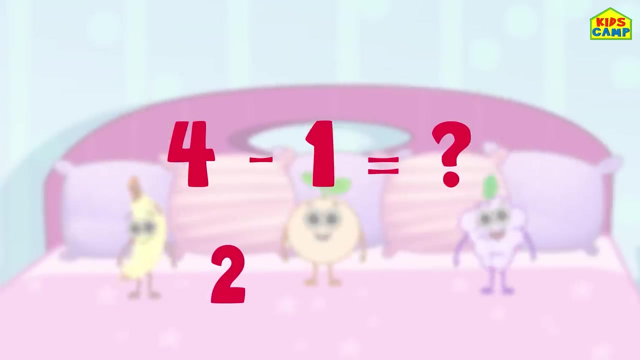 five minus one is: we have one, two, three, four. we have four fruits jumping on the bed. that's right. five minus one is four. we have four fruits jumping on the bed. oops, one fell off. oh, how many fruits do we have jumping on the bed now? four minus one is: is it two, is it one, is it three? 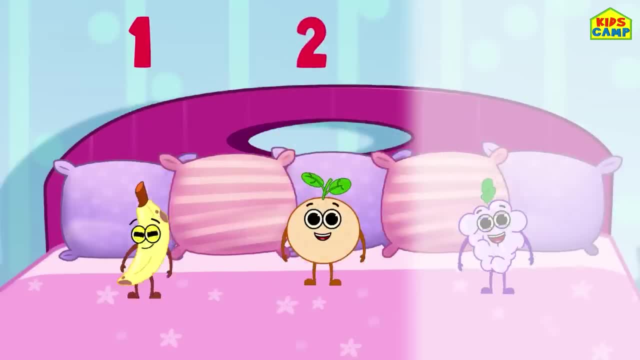 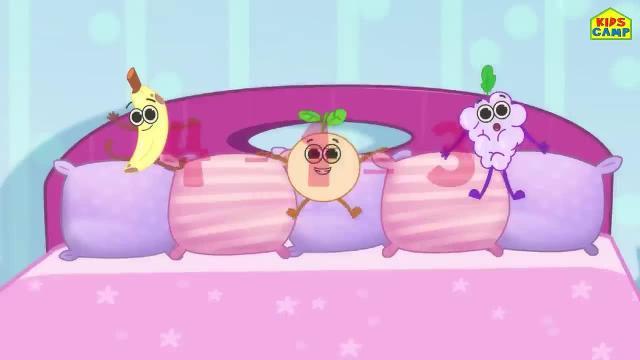 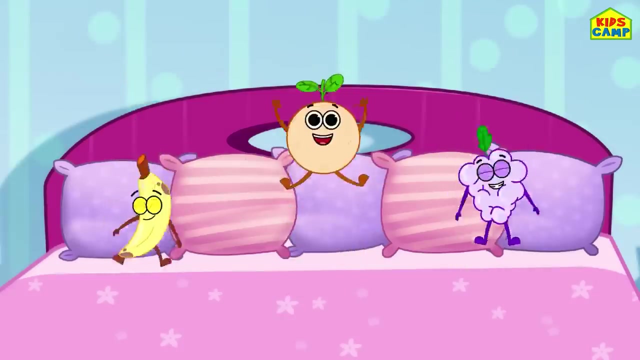 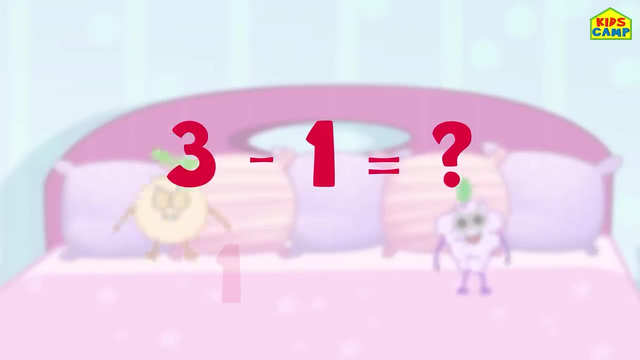 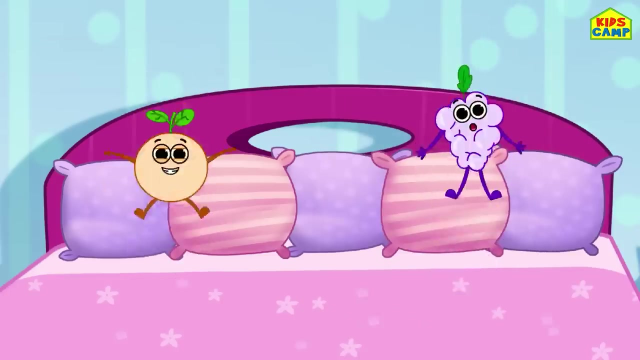 let's count one, two, three. we have three fruits jumping on the bed. four minus one is three. yay, oops, one more fell off. oh, three minus one is. is it one, is it two, or is it three? one, two: we have two fruits jumping on the bed. three minus one is two. 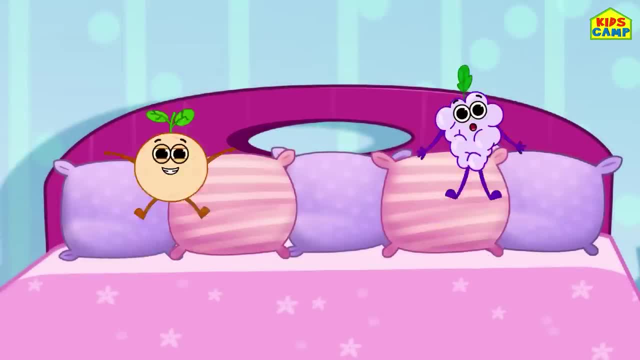 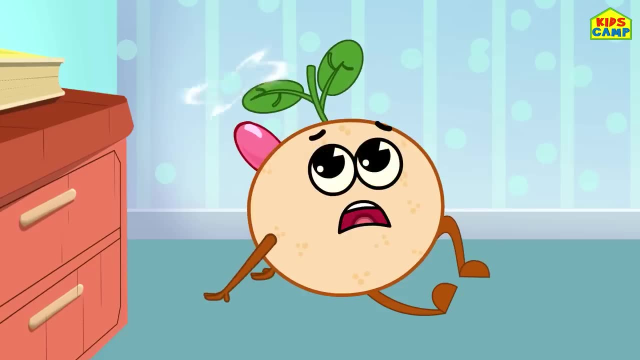 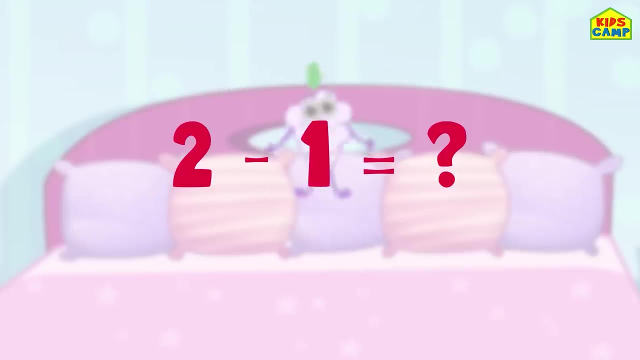 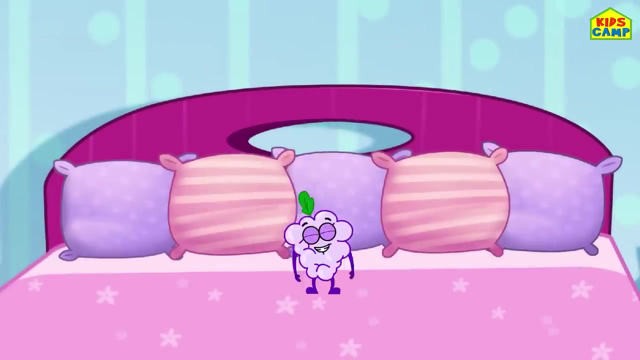 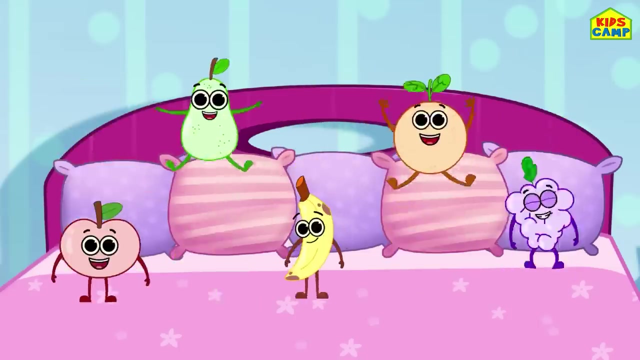 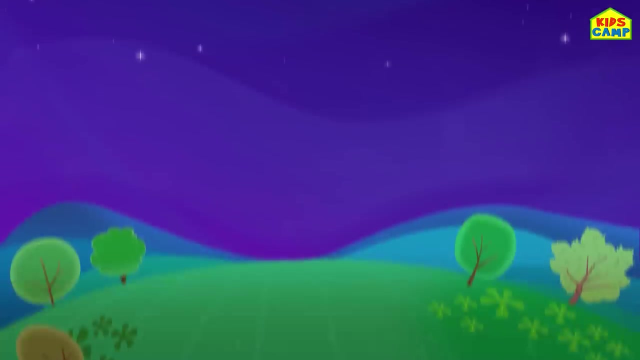 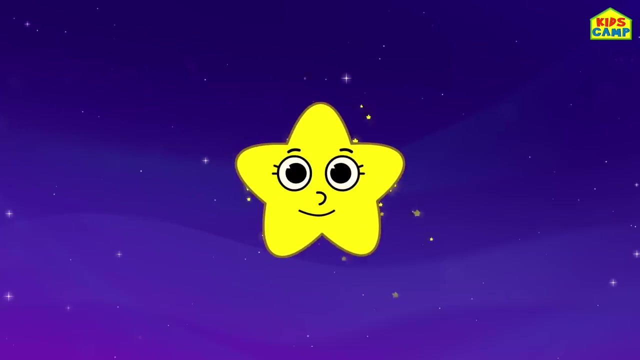 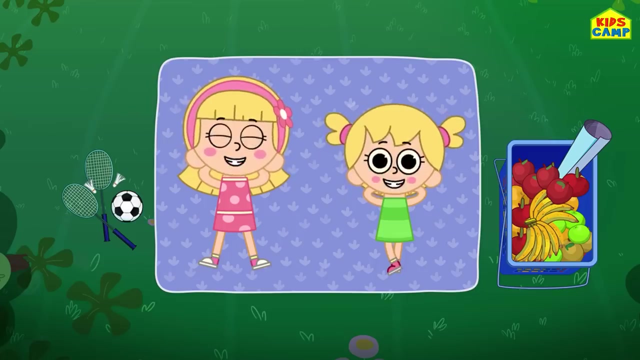 woohoo, wow, one more fell off. ouch. hmm, how many left on the bed? two minus one is one. let's put all the fruits back on the bed. yay, we did it. good job, kids. bye, good job kids. look eva, twinkle, twinkle little star. tell me what we hinkle you are. 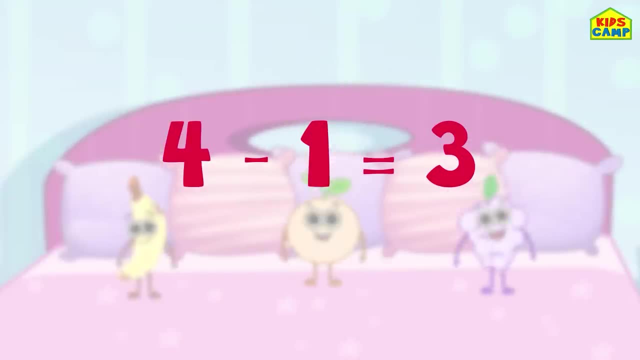 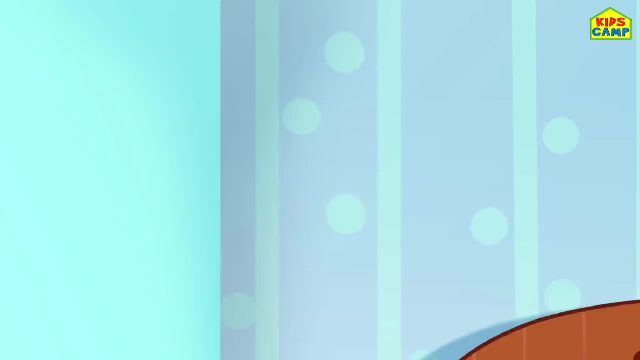 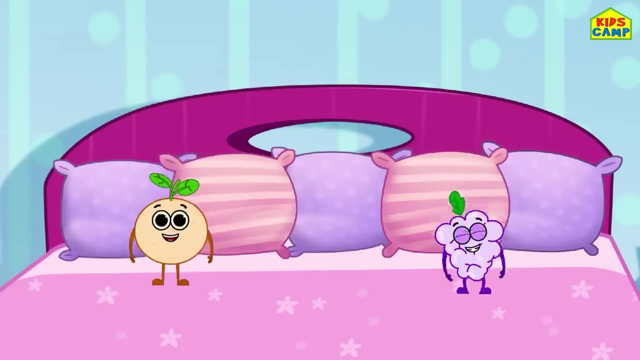 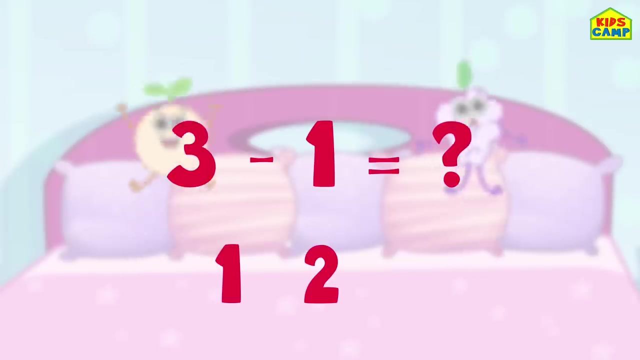 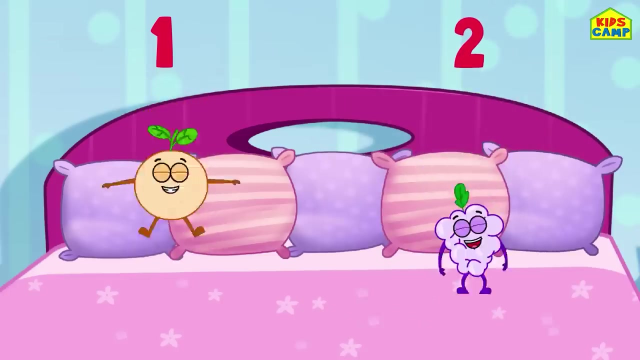 Four minus one is three. Yay, Oops, One more fell off. Oh, One. Three minus one is: Is it one, Is it two, Or is it three? One, two. We have two fruits jumping on the bed. 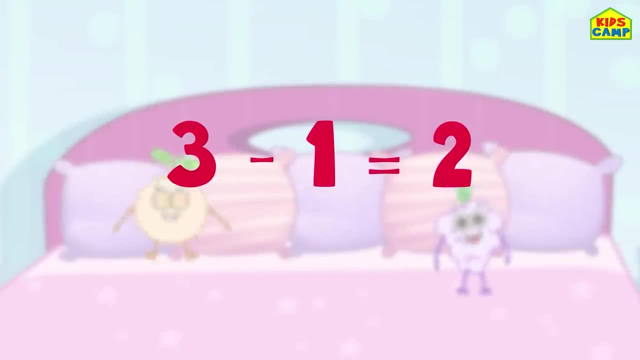 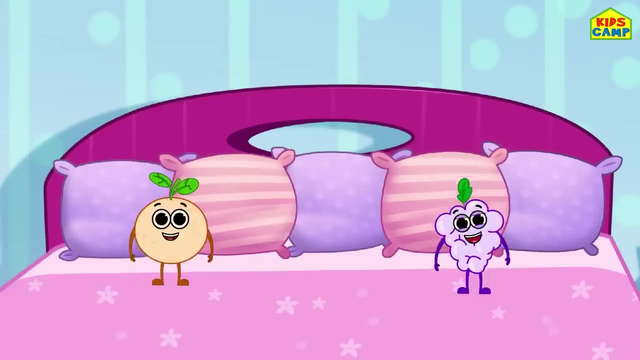 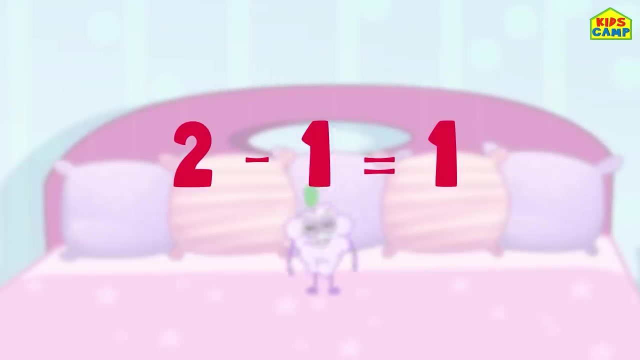 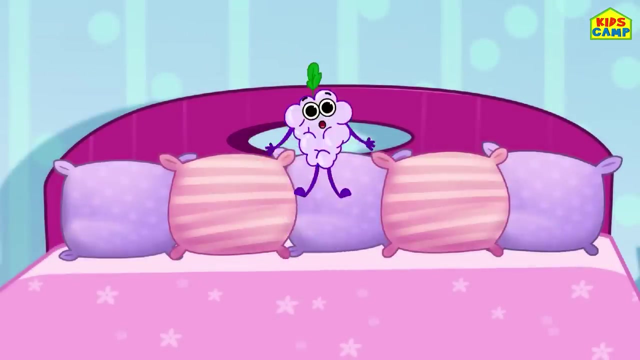 Three minus one is two. Yay, Woohoo, Wow, Oh. One more fell off. Ouch, Hmm, How many left on the bed? Two minus one is One. Let's put all the fruits back on the bed, Yay. 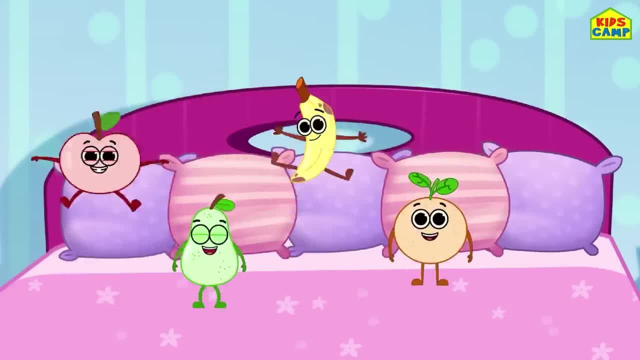 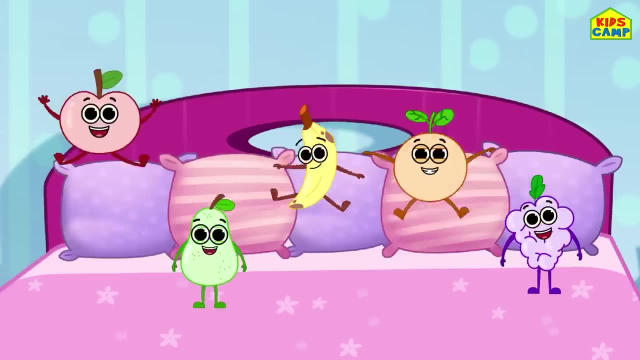 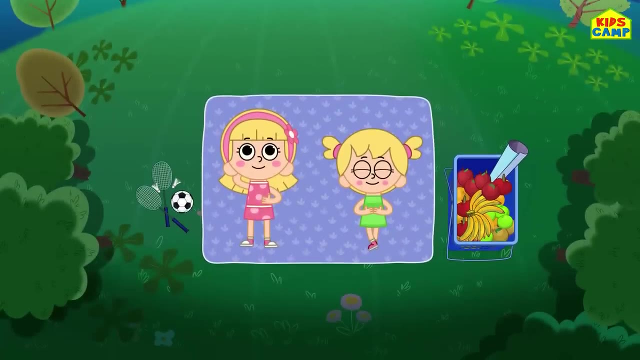 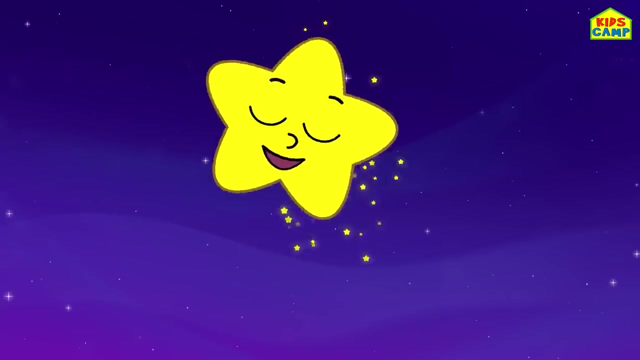 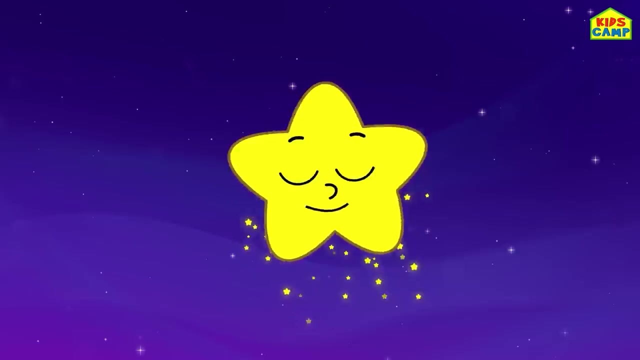 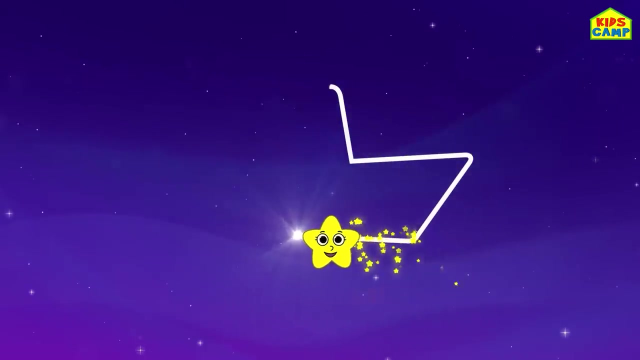 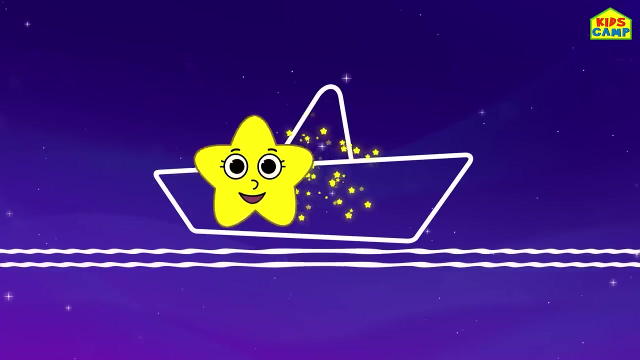 We did it. Good job, kids. Bye-bye, Look, Eva, Twinkle, twinkle little star, Tell me what vehicle you are. Wow, This is so exciting. Woohoo, What is that? I think it's a boat. The boat sails in the vast ocean. 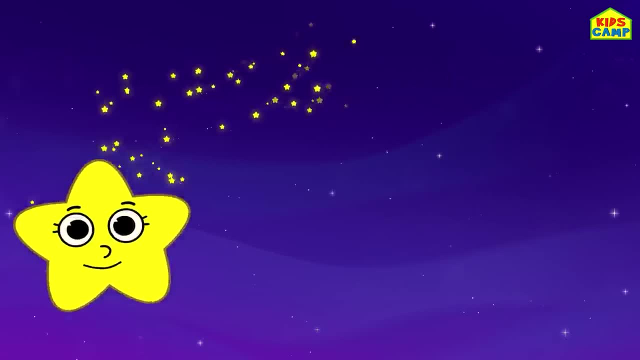 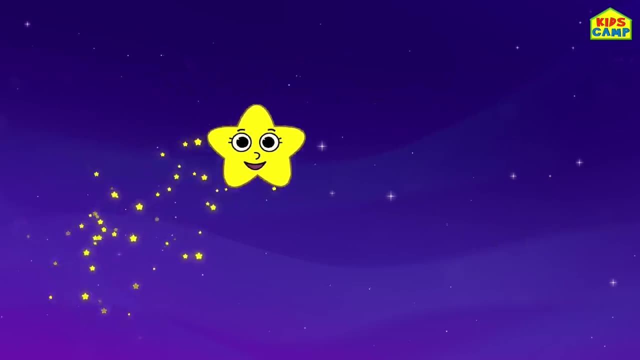 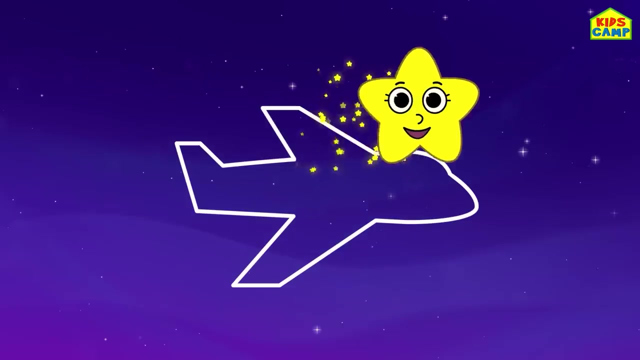 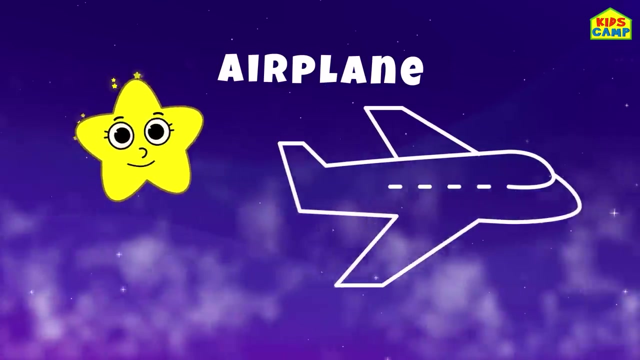 Twinkle, twinkle little star. Tell me what vehicle you are. Twinkle, twinkle little star. Twinkle, twinkle little star. Here comes another one. Wow, Look, it's an airplane. An airplane flies high in the sky And can take us anywhere in the world. 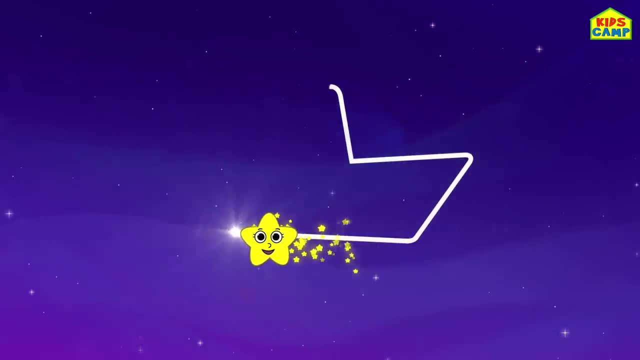 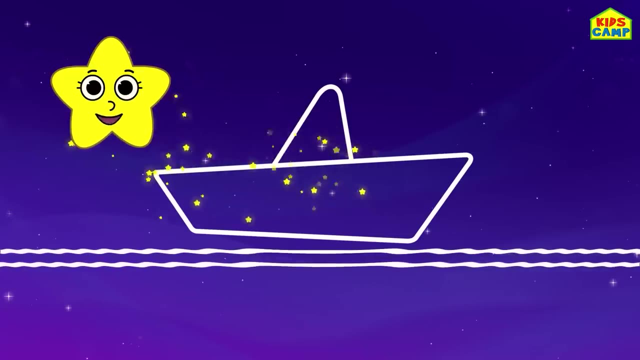 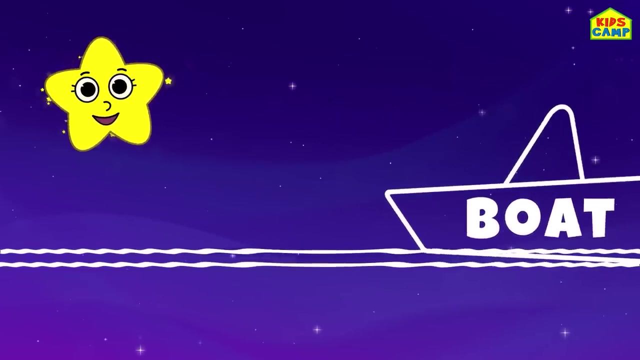 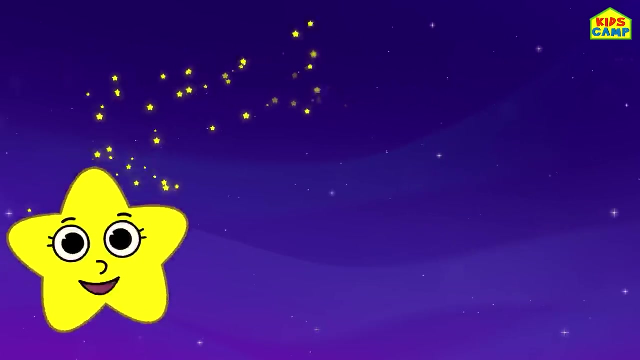 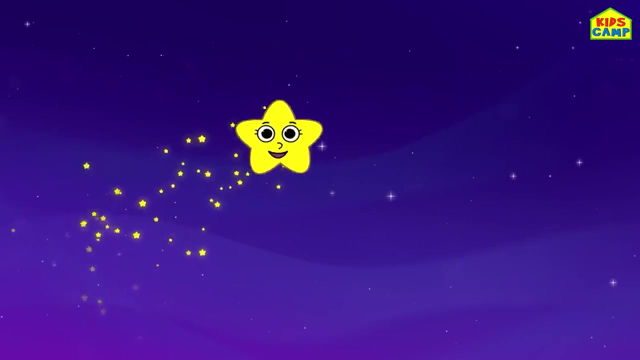 wow, this is so exciting. thank you. wow, this is so exciting. wow, this is so exciting. Woohoo, What is that? I think it's a boat. The boat sails in the vast ocean. Twinkle, twinkle little star. Tell me what vehicle you are. 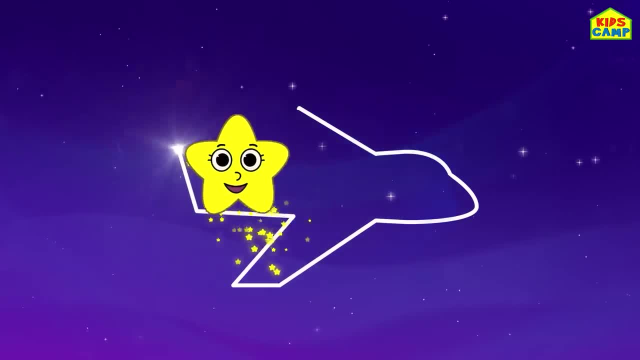 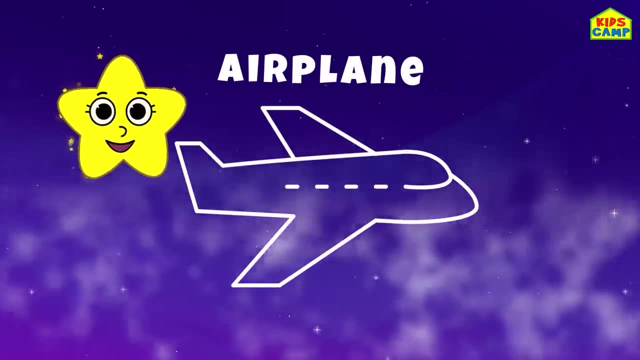 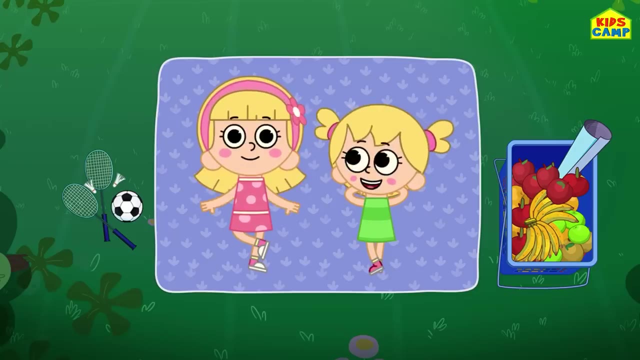 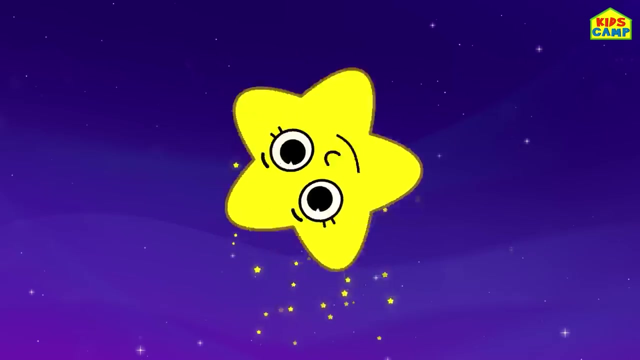 Here comes another one. Wow, Look, it's an airplane. An airplane flies high in the sky and can take us anywhere in the world. Wow, We are getting good at this Twinkle, twinkle little star. Tell me what vehicle you are. 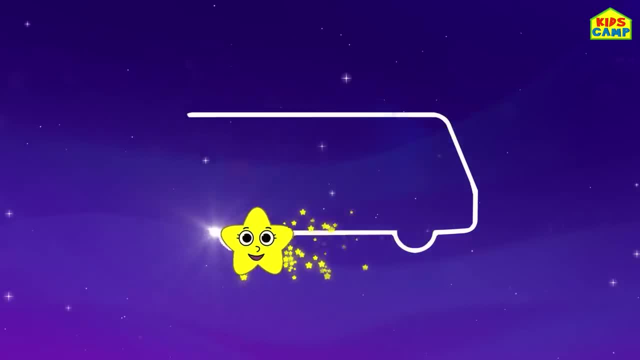 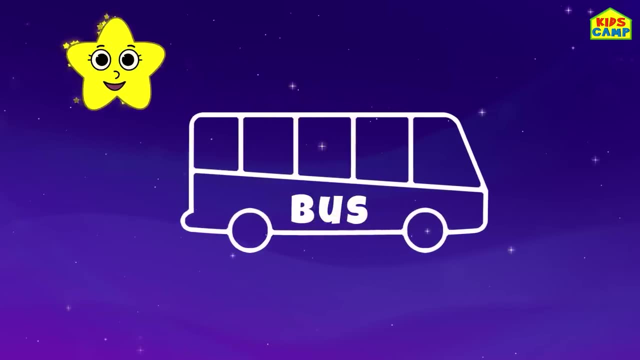 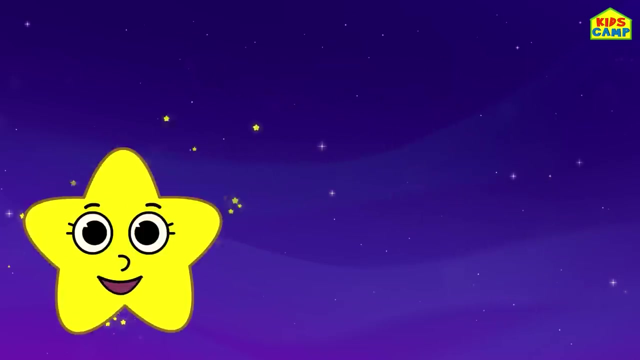 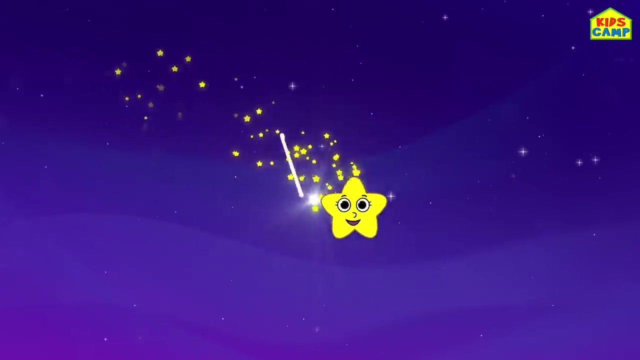 Look, look One more. It's a bus. You're right, Ellie. We go to school in the bus. It's so much fun. Yay, Twinkle, twinkle little star. Twinkle, twinkle little star. Tell me what vehicle you are. 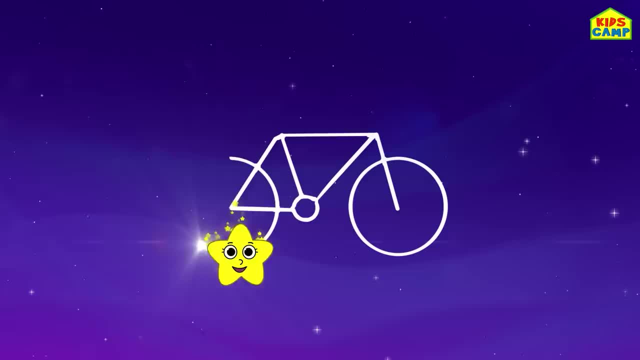 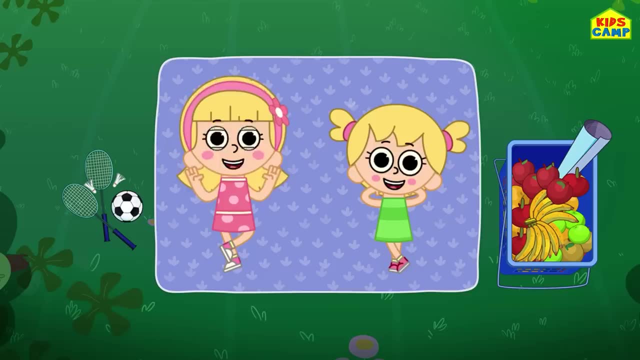 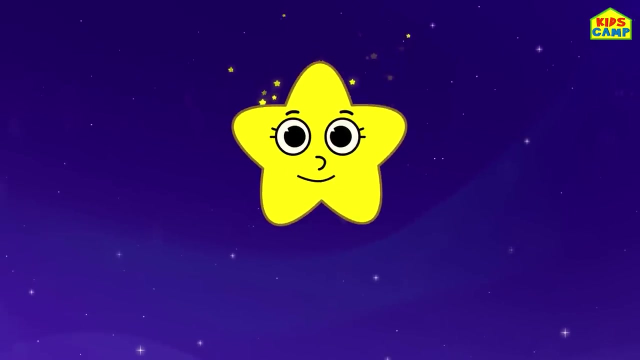 Hey Look One more. Is that a bicycle? Yes, yes, I love cycling. It also keeps us fit and healthy. Yay, We did it. We had so much fun learning vehicles. Good bye, Woohoo, Hi friends, I'm Ellie. 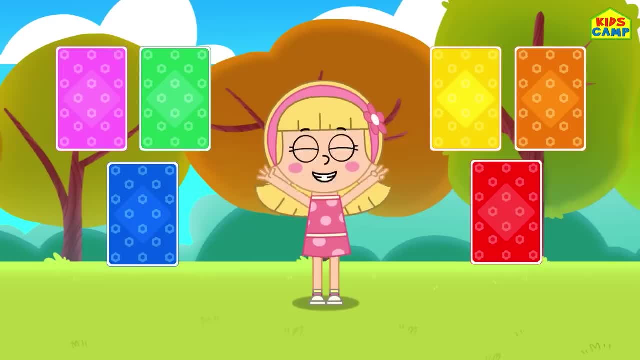 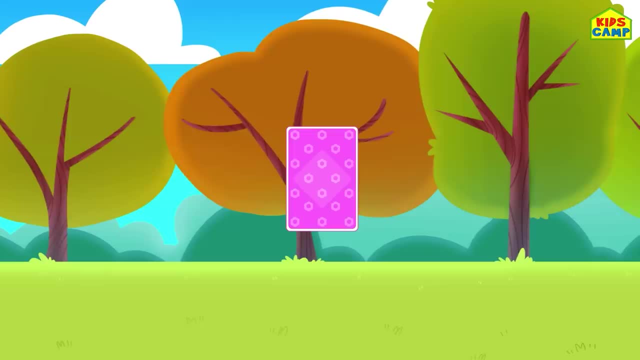 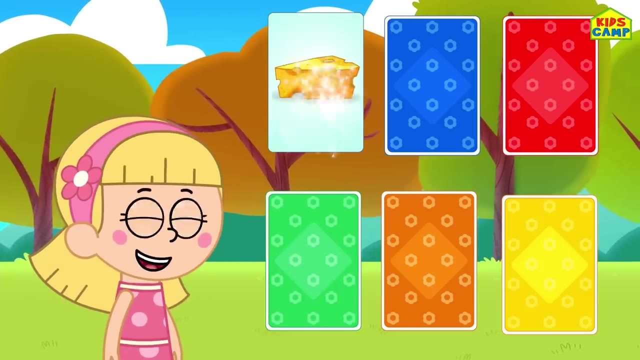 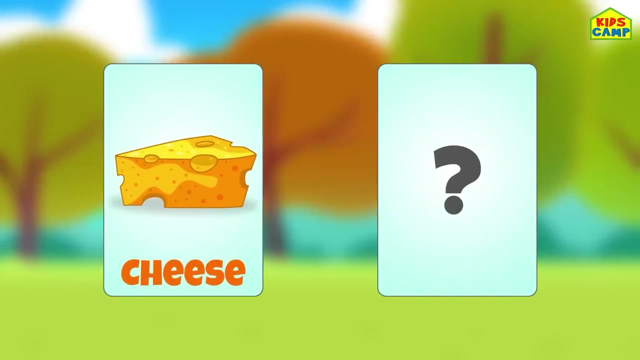 Let's play a fun card game. We have six colorful cards. Let's flip them over and start the game. Yay, Whee. Let's start with the pink card. Ooh, What is this? It's cheese. We need to find what cheese is made of. 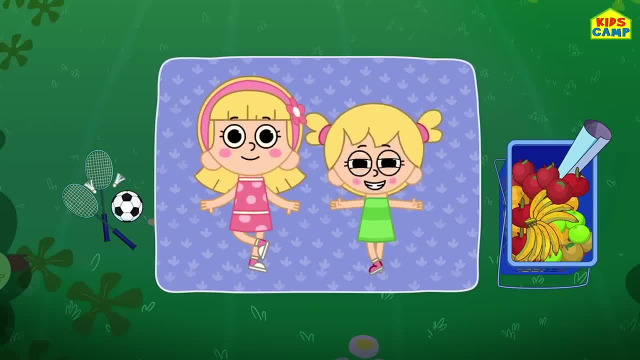 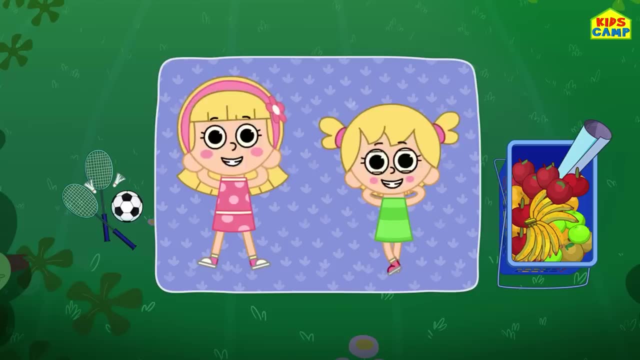 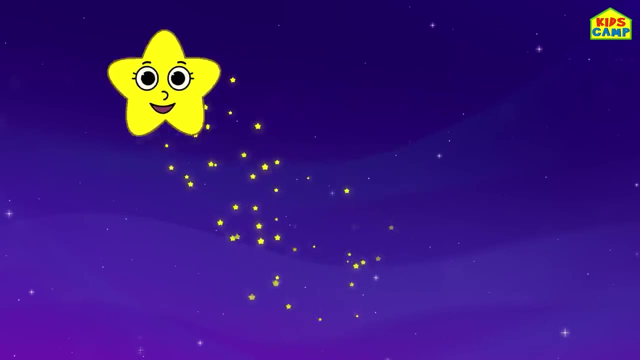 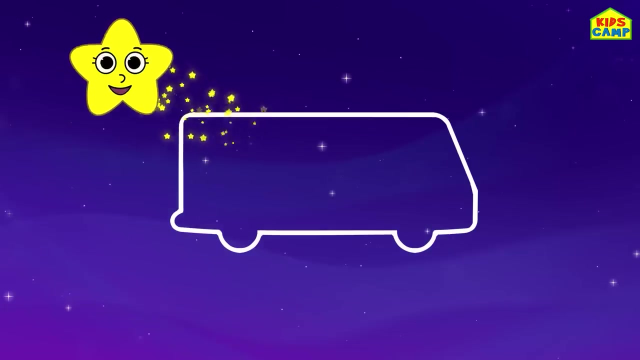 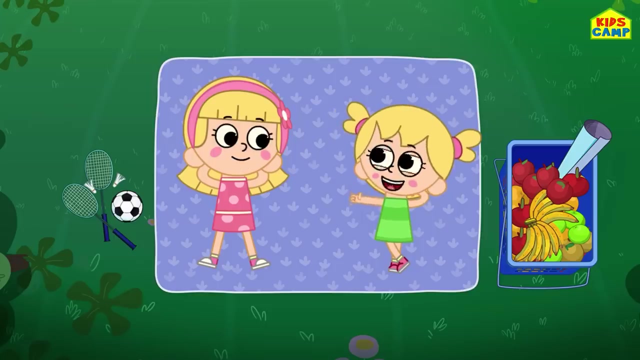 Wow, We're getting good at this. Twinkle, twinkle little star, Tell me what vehicle you are, Look, look One more: It's a bus. You're right, Ellie, We go to school in the bus. It's so much fun. 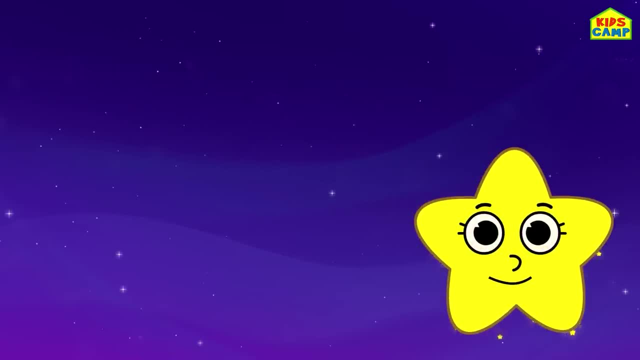 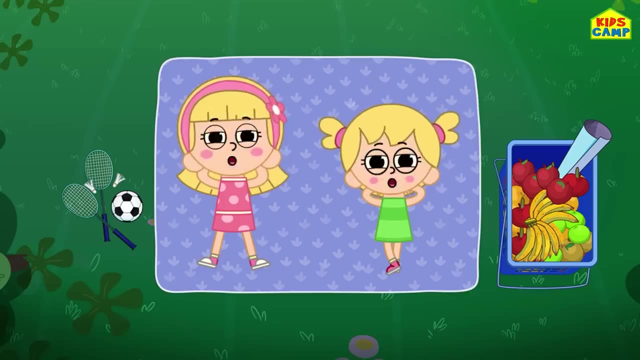 Yay, Twinkle, twinkle little star. Twinkle, twinkle little star. Twinkle, twinkle little star. Tell me what vehicle you are. Tell me what vehicle you are. Tell me what vehicle you are. Hey Look, One more, Is that a bicycle? 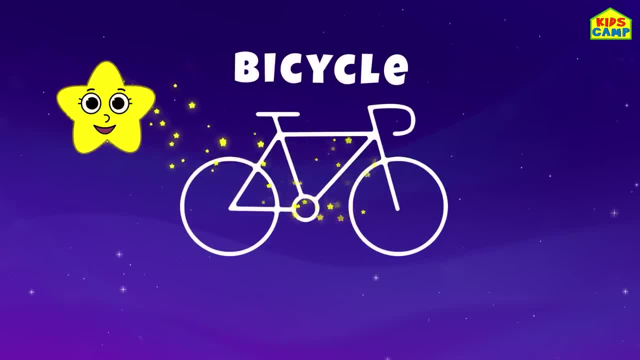 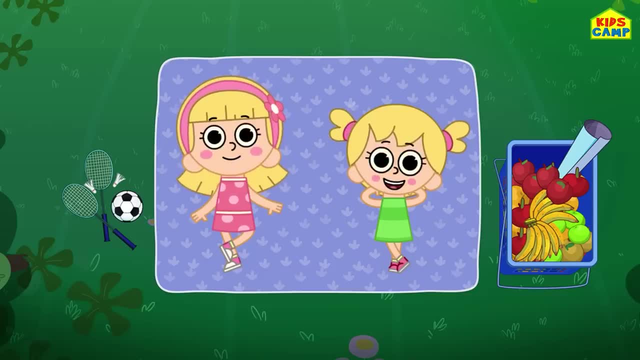 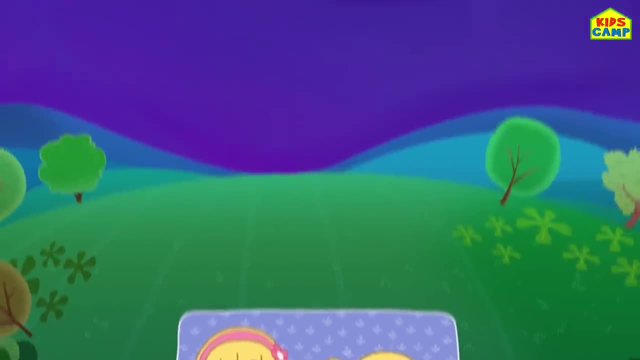 Yes, yes, I love cycling. It also keeps us fit and healthy. Yay, We did it. We had so much fun learning vehicles. We had so much fun learning vehicles. Good bye, We had so much fun learning vehicles. We had so much fun learning vehicles. 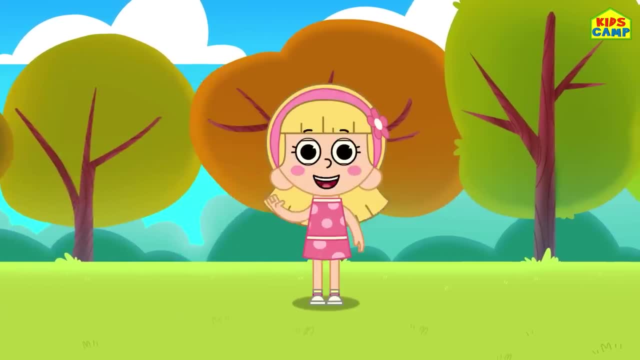 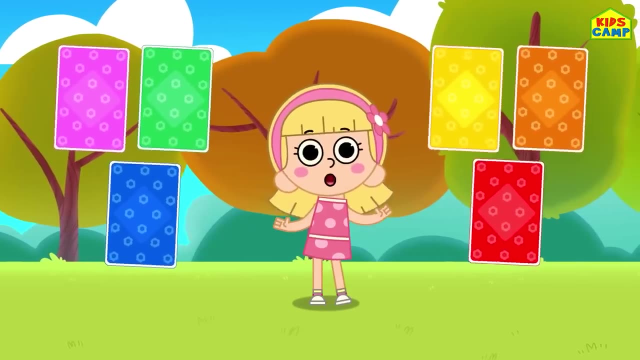 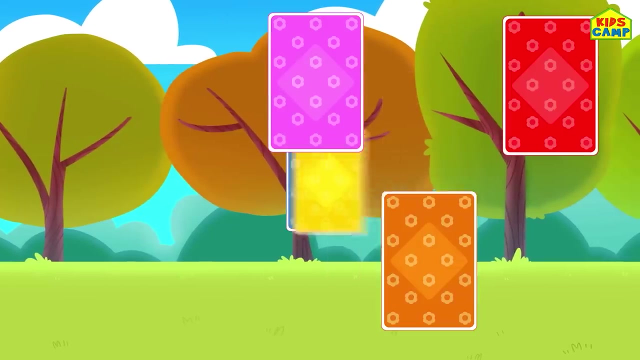 Yay, Woohoo. Hi friends, I'm Ellie. Let's play a fun card game. We have 6 colorful cards. Let's flip them over and start the game. Yay, Yay, Whee, Whee. Let's start with the pink card. 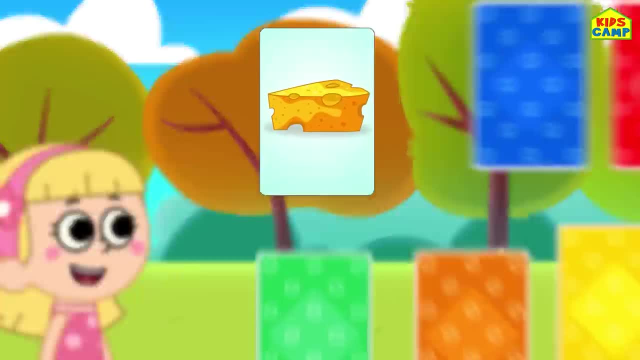 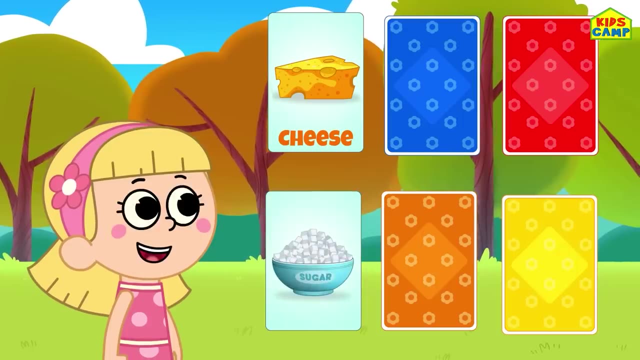 Let's start with the pink card. What is this? It's cheese. We need to find what cheese is made of. We need to find what cheese is made of. Uh oh, What is this? It's sugar. Is cheese made from sugar? 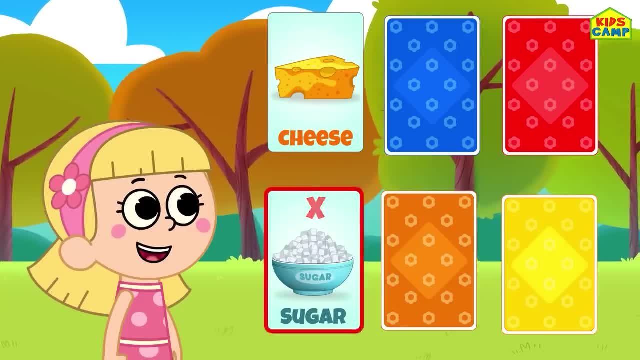 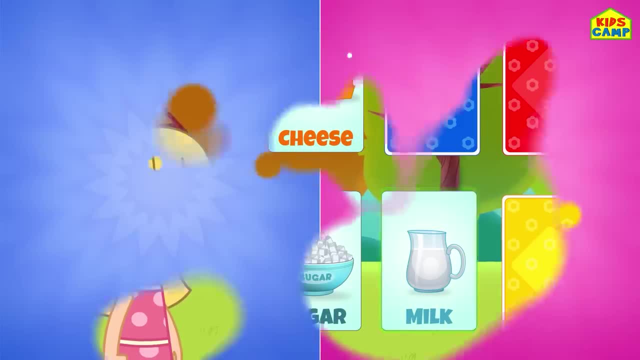 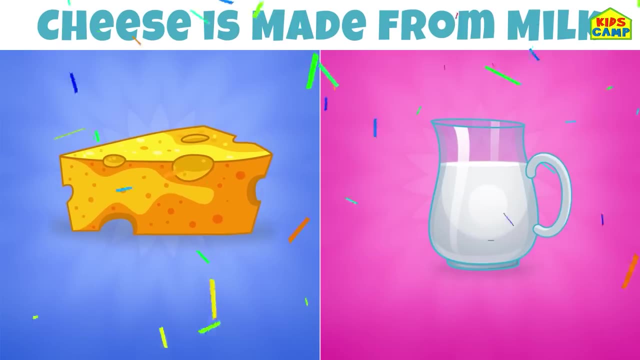 No, I don't think so. Let's flip another card. Let's flip another card. It's milk. Yes, We got that right. Cheese is made from milk. Yay, Right, kids, Yummy, Let's find out what's next.